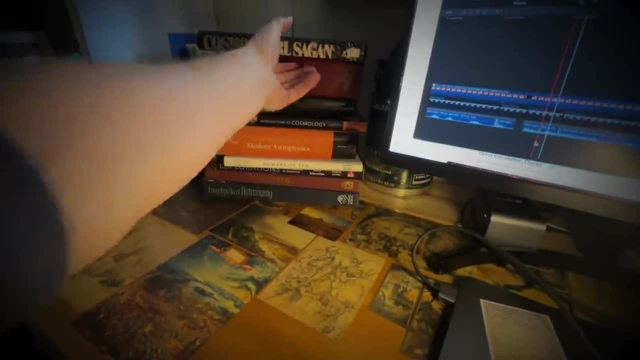 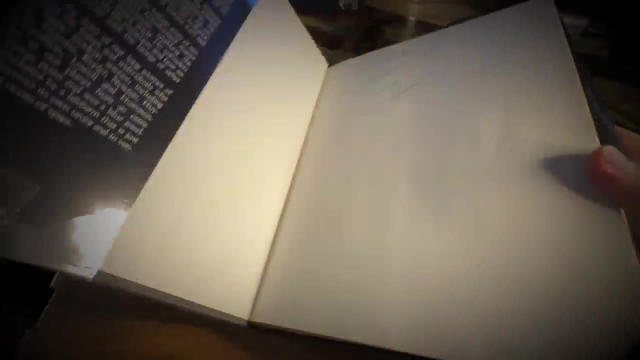 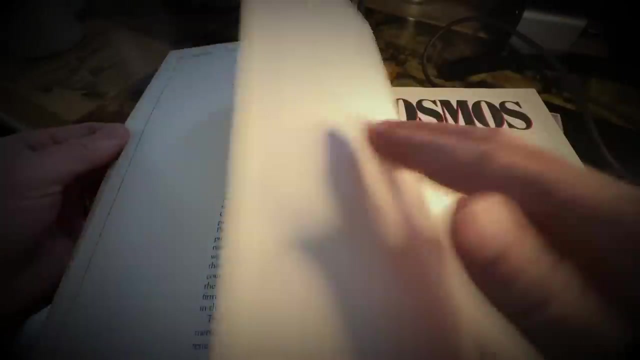 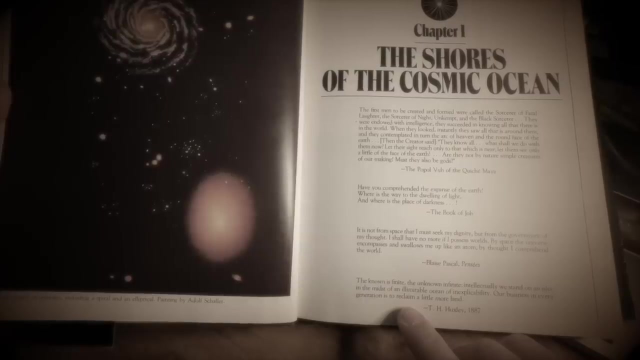 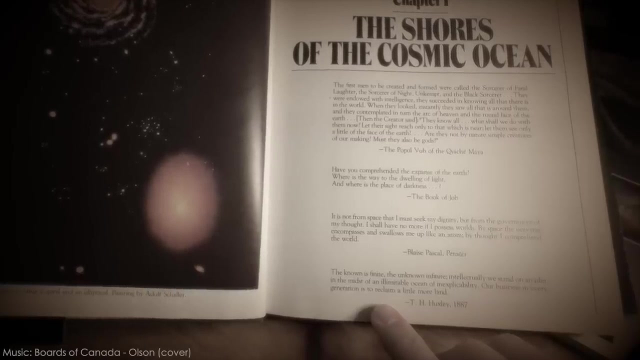 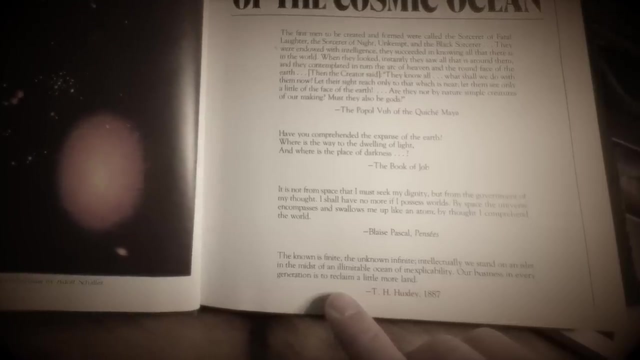 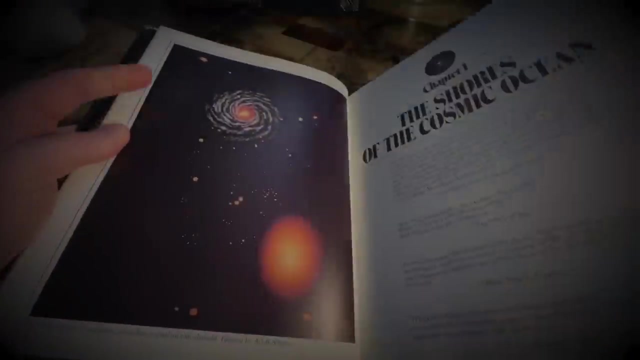 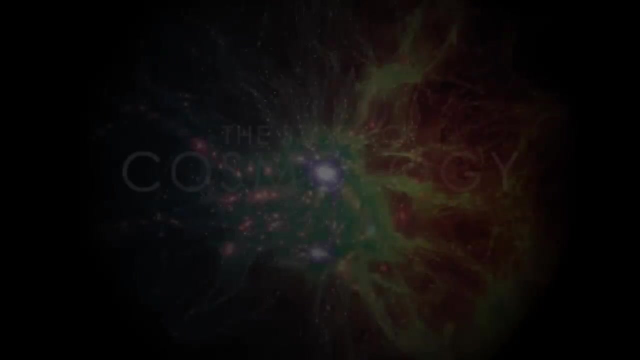 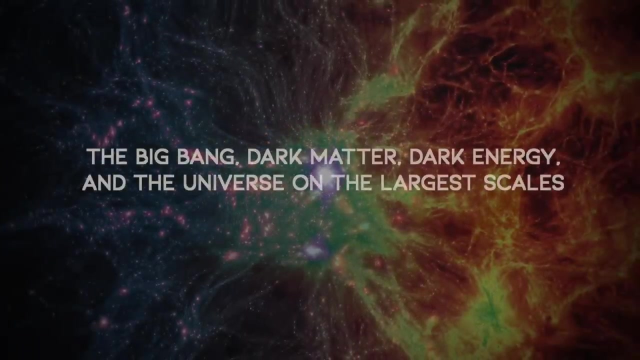 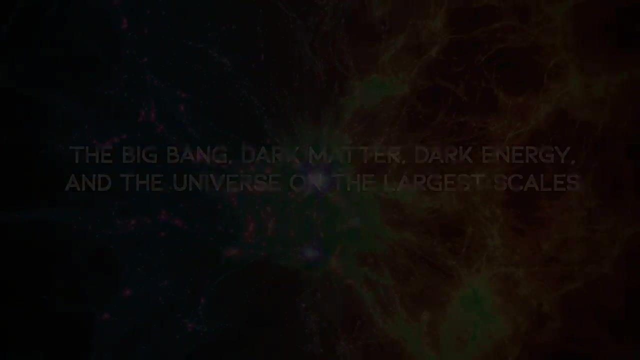 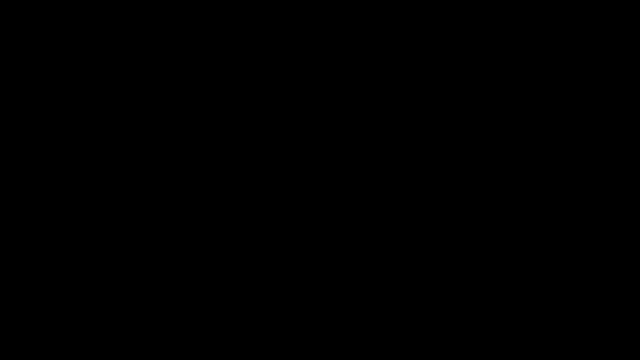 The known is finite, but the unknown infinite. Intellectually, we humans stand in the midst of an illimitable ocean of inexplicability. Our business in every generation is to reclaim a little more land. Thank you very much In the first instant of time. 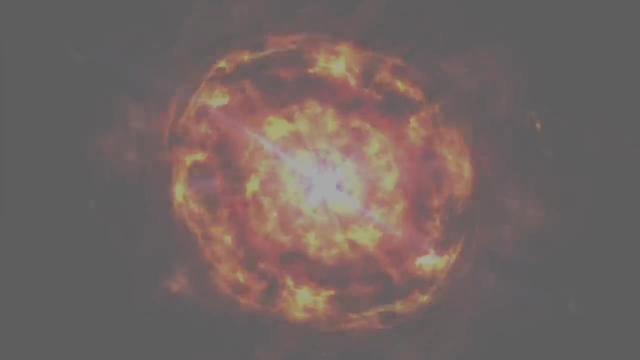 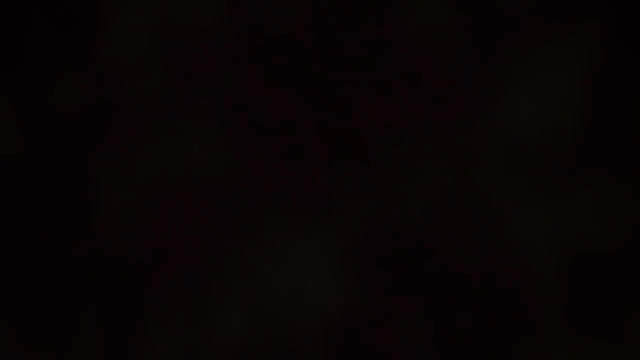 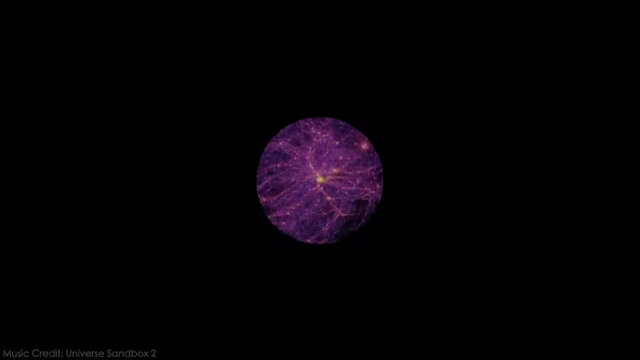 all of existence was intertwined fields of near-infinite energy. Particles didn't exist, Matter didn't exist. Everything was fluid, unified, and energies like this haven't been seen in the universe anywhere ever since Less than a trillion trillionths of a second later. 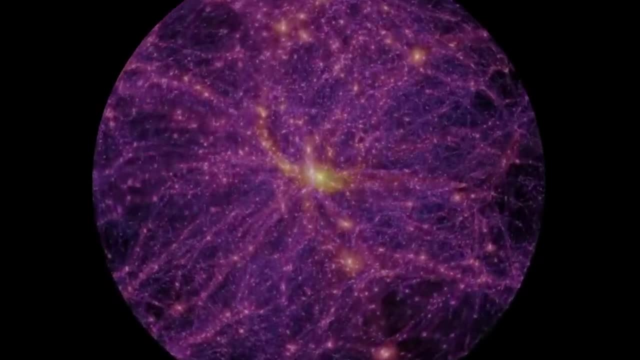 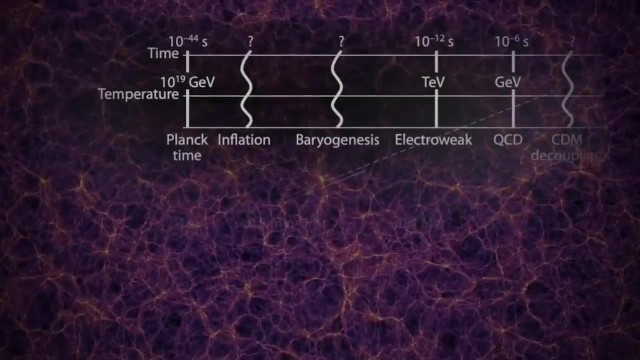 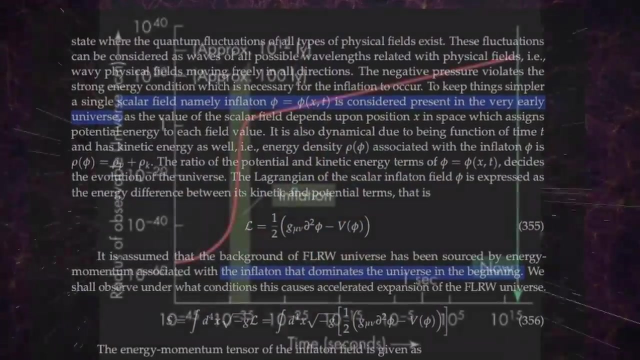 in an already expanding universe. an additional event called inflation happened Under the influence of water, what cosmologists cleverly called the Inflaton particle. the metric of spacetime itself suddenly stretched exponentially, and these overlapping energy fields began evolving into the physics we know today. 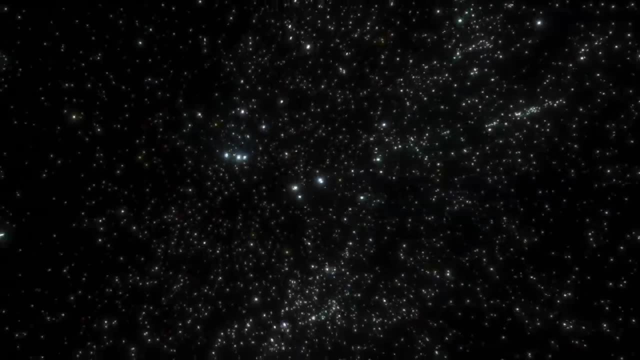 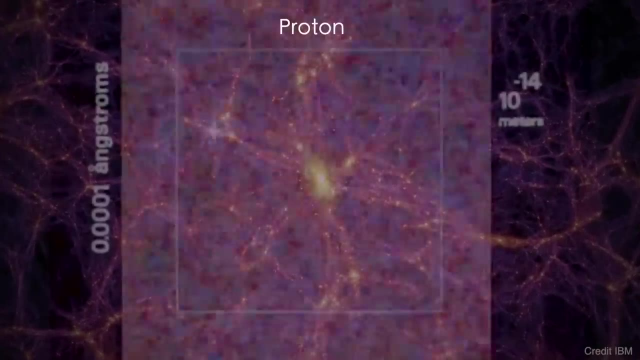 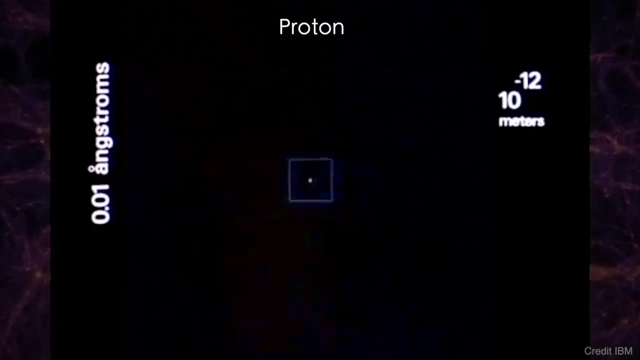 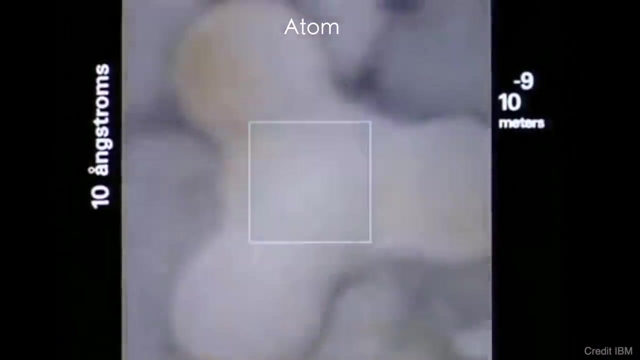 Before this inflation, this observable universe, our local pocket of the universe, was only the size of half the width of a proton. inflation expanded this to 10, to the power of 78 times this volume. so this is a huge order of magnitude. and let's put it on more human scales here. our volume of space went from about 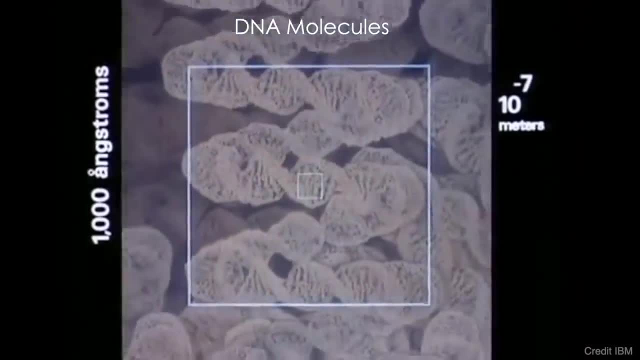 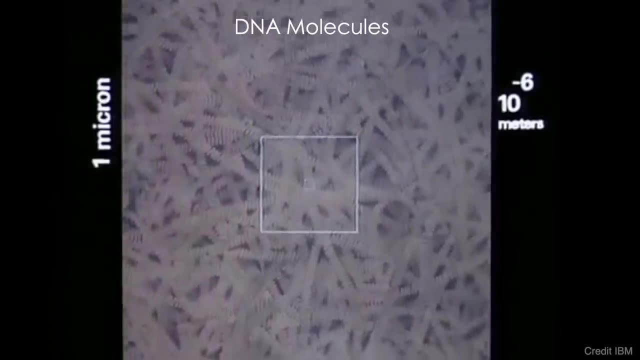 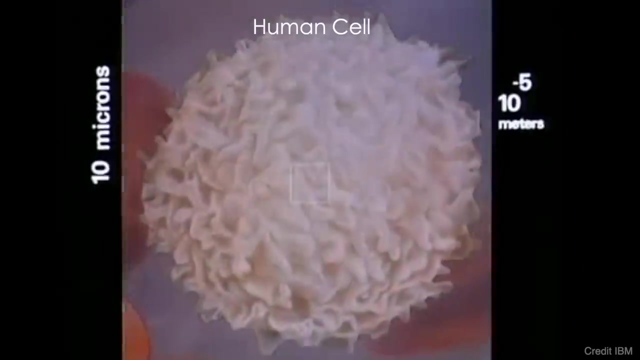 the size of a proton inflated to a grain of sand. but even that doesn't do it justice. most of us don't have an intuition of just how small the quantum realm is, myself included. so I think a better visualization to the picture to the tune of something more anthropomorphic. 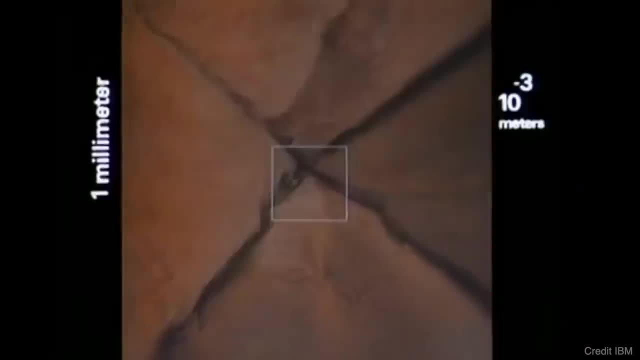 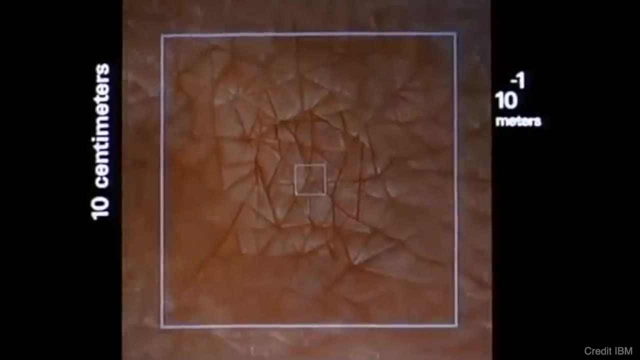 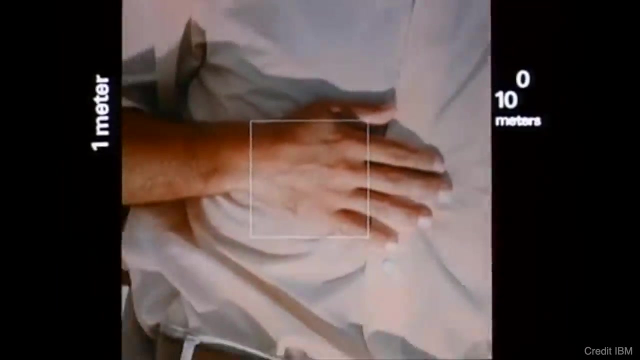 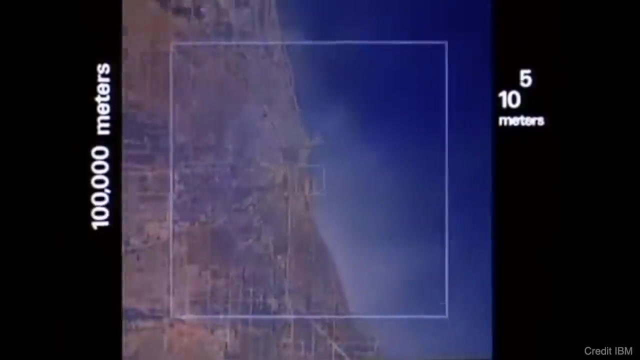 more human centered, would be still something really small, microscopically small, but still imaginable- like a plant cell- and this is about a 50th of the width of a human hair, or about a thousandth of a metronome millimeter. Under this same scale of inflation, that plant cell would have ballooned to 10,000. 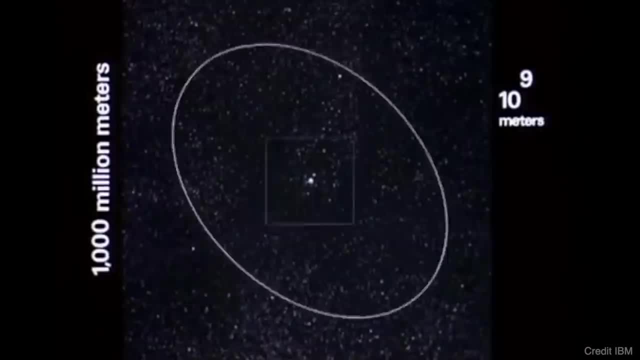 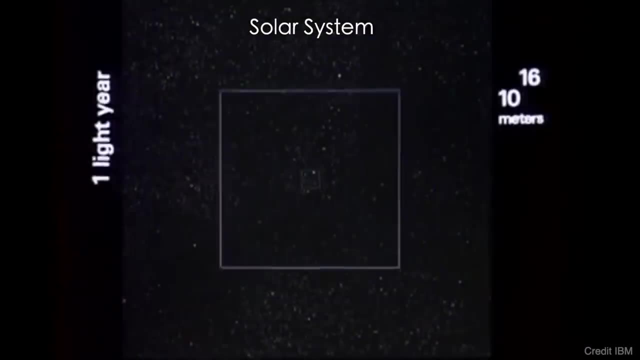 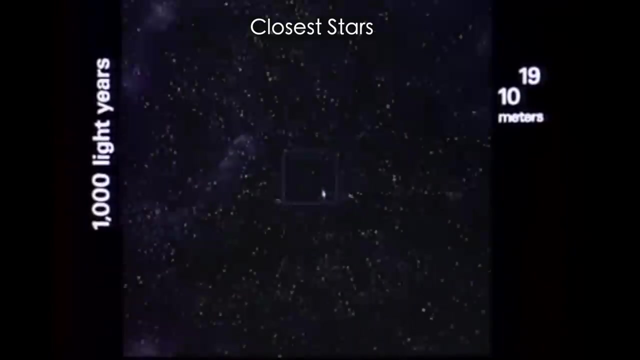 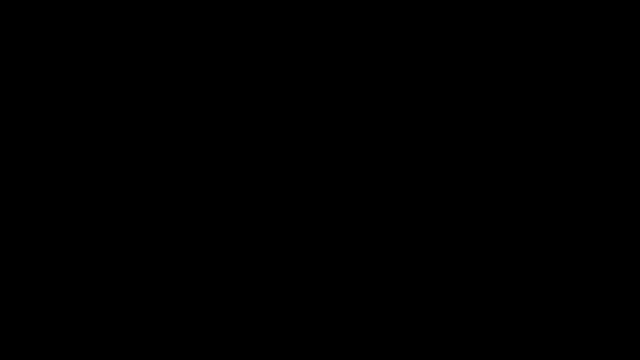 light years across. Then, to put that in even further context, that 10,000 light year chunk of our Milky Way galaxy holds about 350,000 stars. But because the universe really was only the size of a proton before, inflation at scales like this, well, within the quantum realm of things, 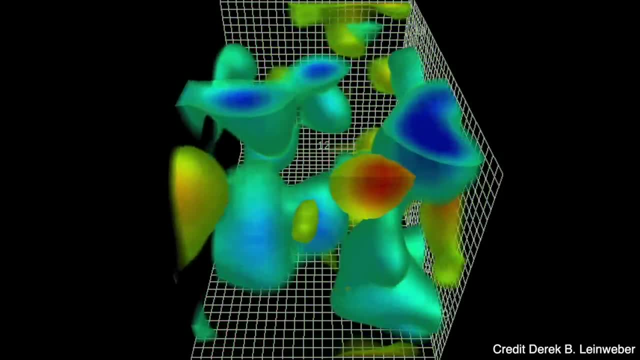 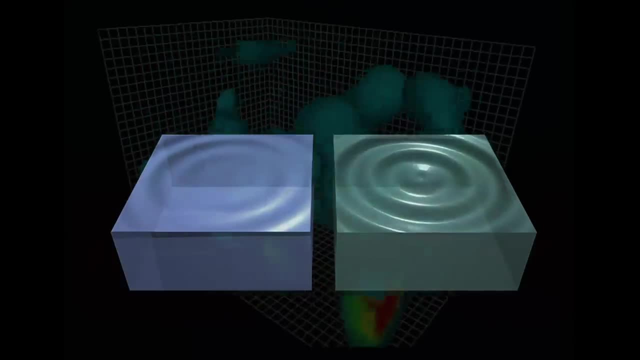 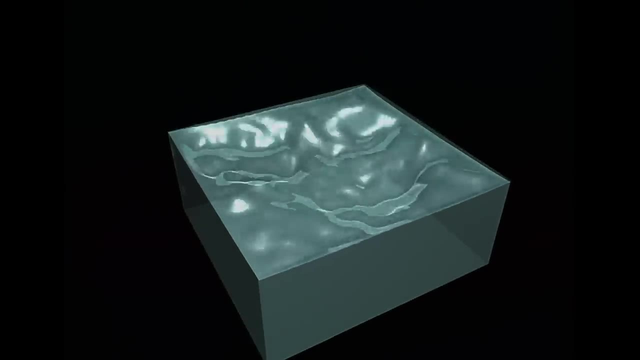 tiny fluctuations in the quantum field energy are always randomly bubbling in and out of existence And these came into play. It's believed that, along the rapid scaling of space-time, the fluctuations, these quantum field energies, permeated the universe and they were inflated. 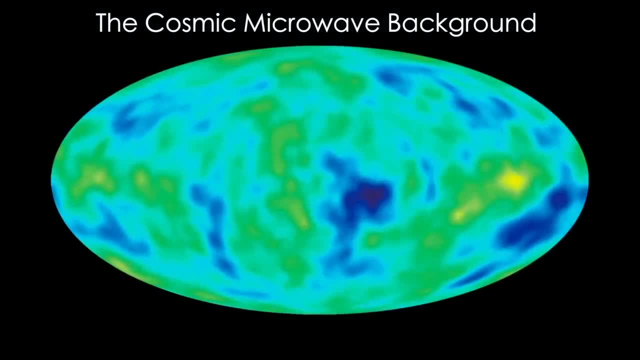 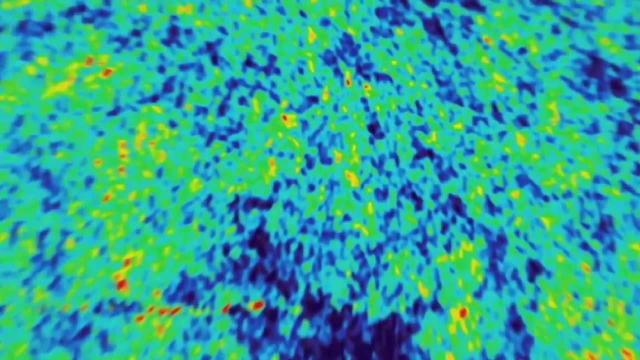 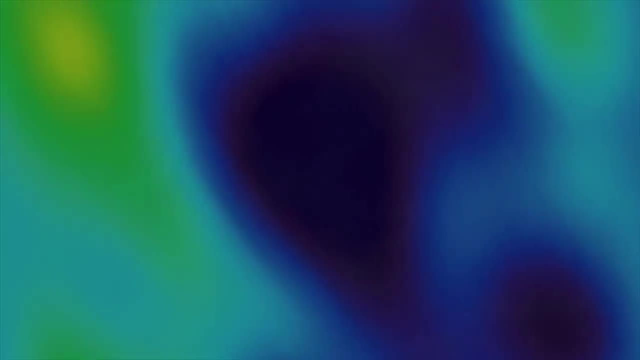 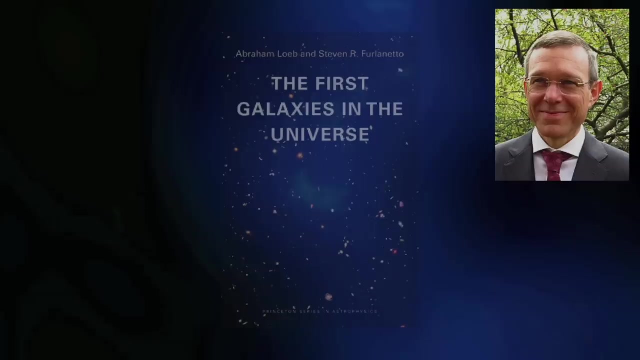 along with it. So this: when inflation hit and blew up the proton to a grain of sand or the human cell to 10,000 light years across, these fluctuations were permanently froze into the structure of the universe And, as Harvard astronomer Avi Loeb propounds in his book The First Galaxies. 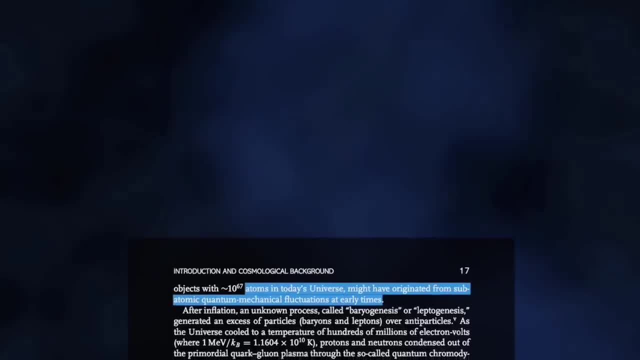 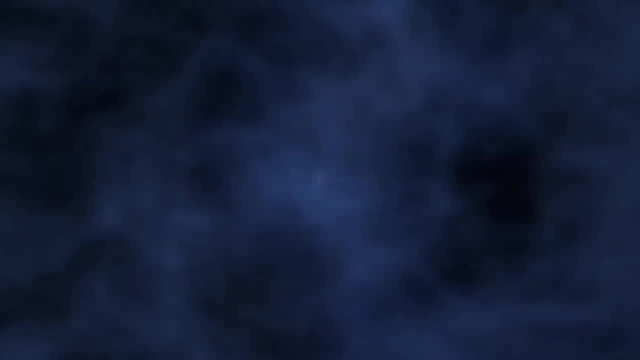 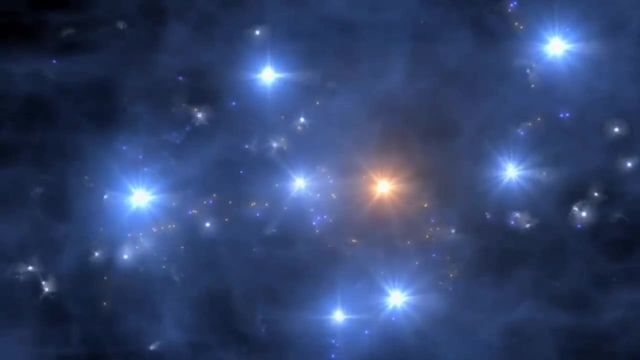 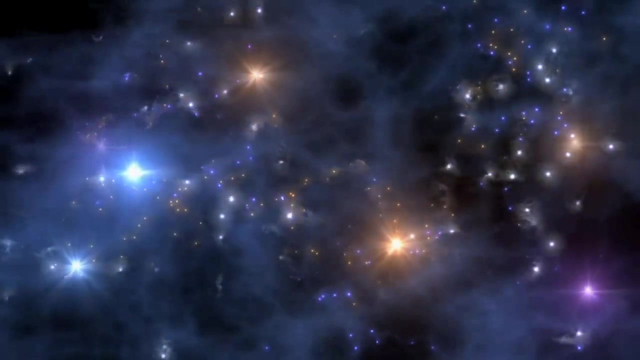 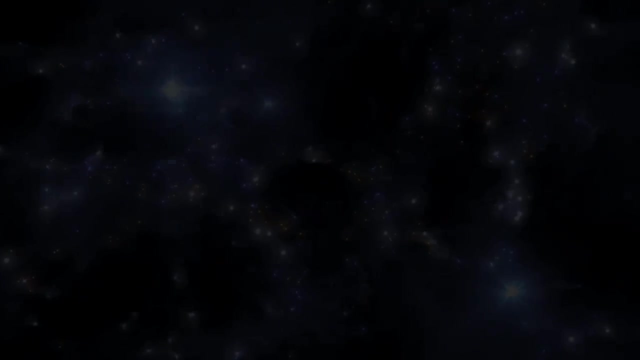 he thinks these quantum perturbations actually led to the inhomogeneities that ultimately birthed the gravitational fluctuations around which the center of galaxies clustered around In the early universe, And he thinks these quantum perturbations were actually what seeded the first stars and then the first galaxies. This then set the universe on its course towards our current state. 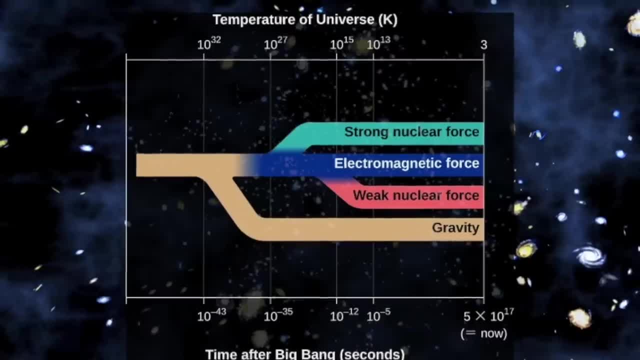 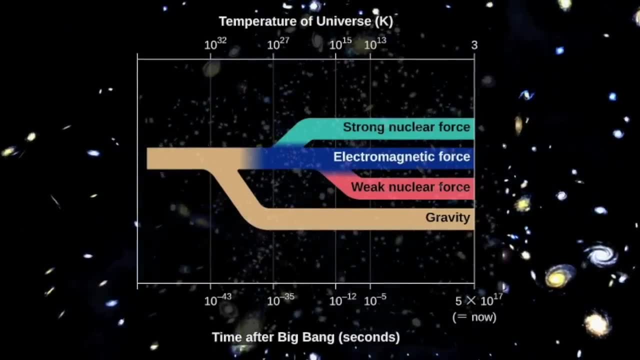 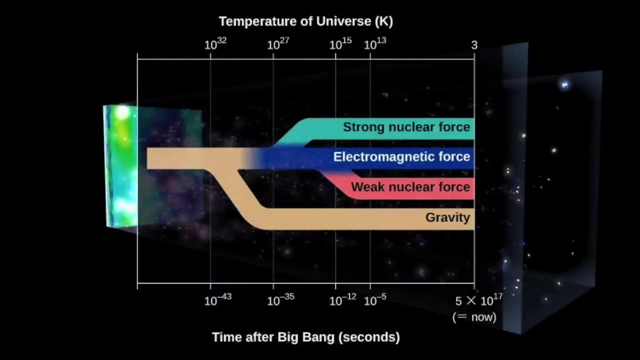 It ripped gravity and the atomic forces apart. They were unified at a certain point before this, this instant, after the big bang. Then the atomic forces themselves went ahead and split into the strong, then the weak, then the electromagnetic forces. Once the electro-weak force split, 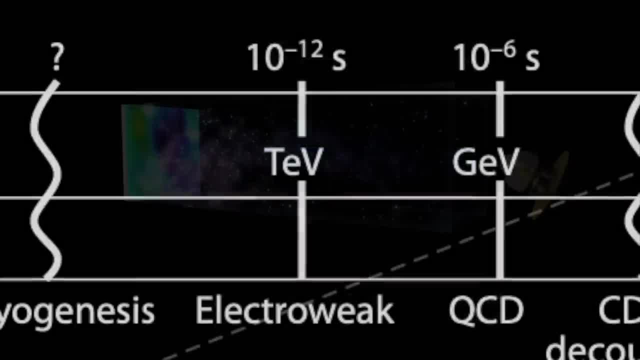 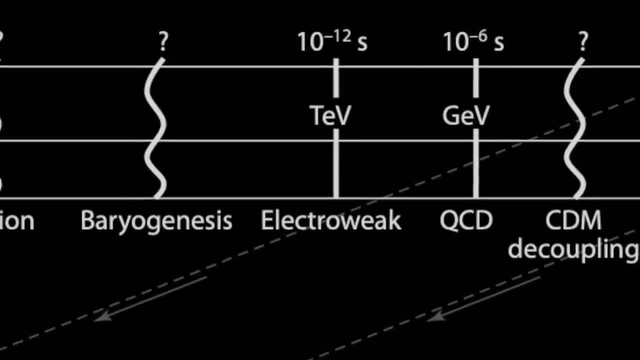 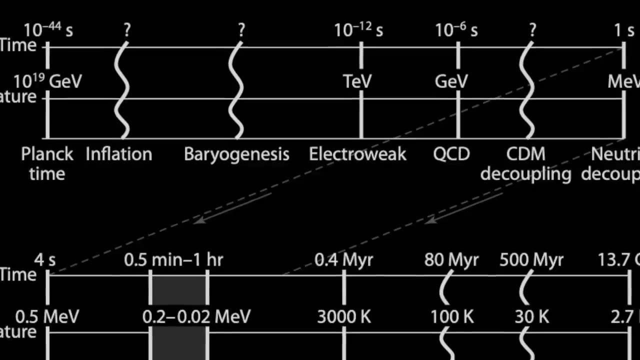 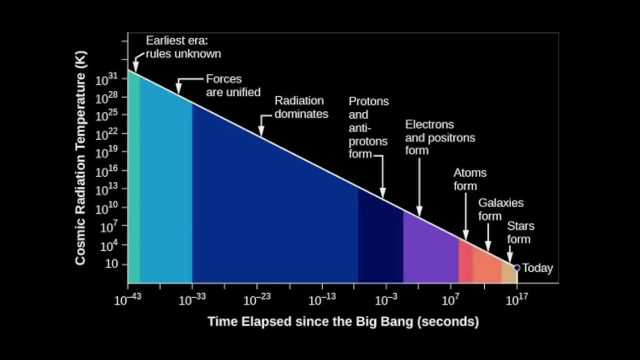 And all this, all this that just happened was less than a billionth of a second after the big bang Into the birth of our universe, And so if we play that out a billion more times to make a full first second of the universe, By then it. 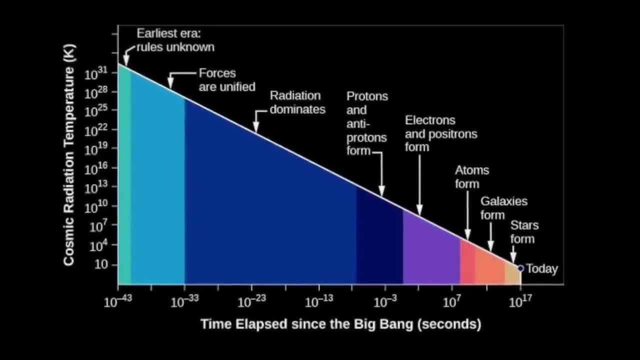 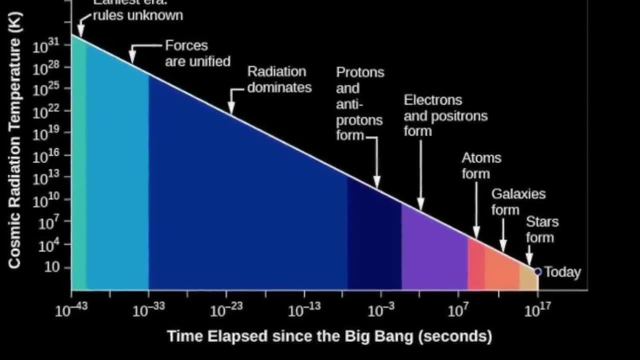 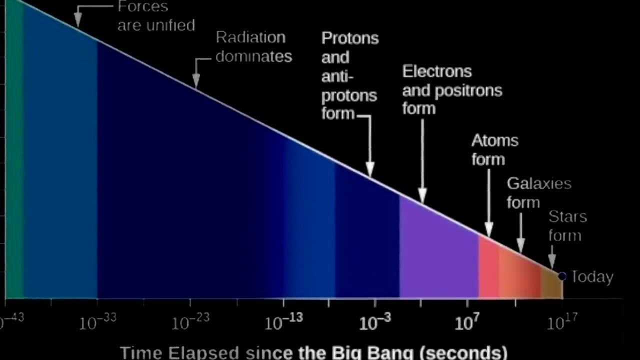 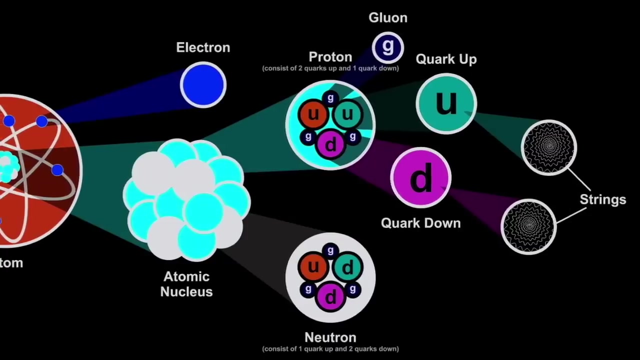 solidified all the current abundances of particles and photons and energies that we know now- Particles and their anti particles like electrons and positrons. they popped into existence at this point, but instantly began annihilating each other, and this left an oddly fortunate for us surplus, because it's the 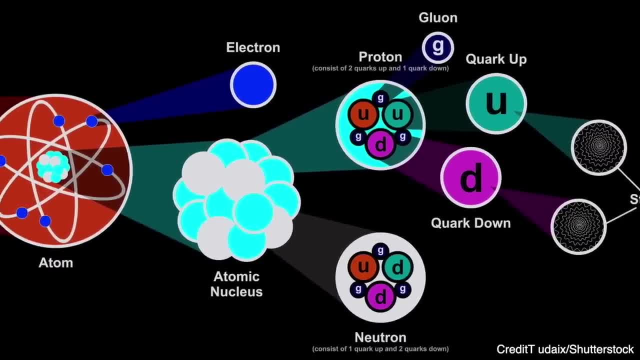 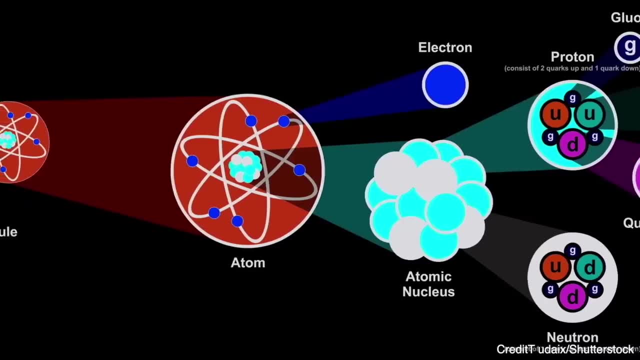 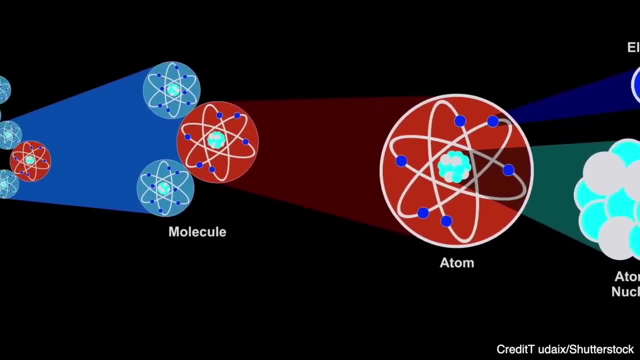 particles- not the anti particles- that were made of The leftover quarks from these annihilations, then snapped together into triplets to become protons and, for about the first 20 minutes of the universe, still at billions of degrees. mind you, it was hot enough to fuse the. 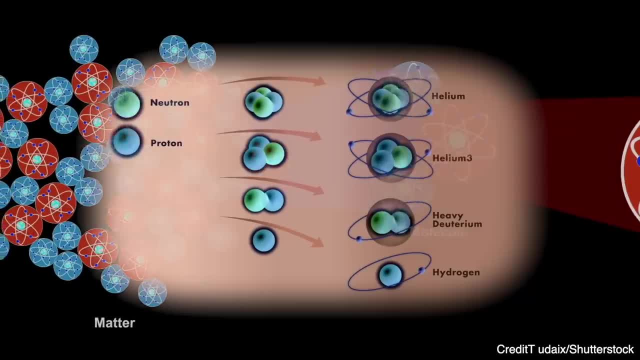 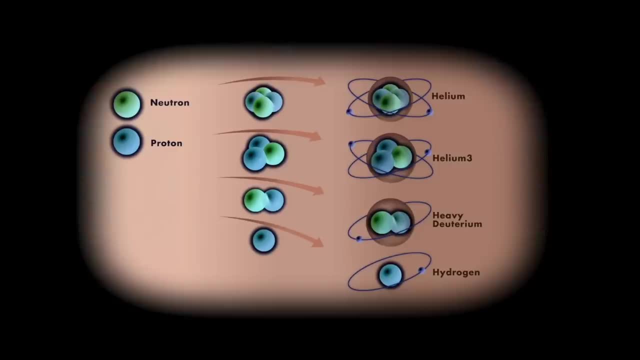 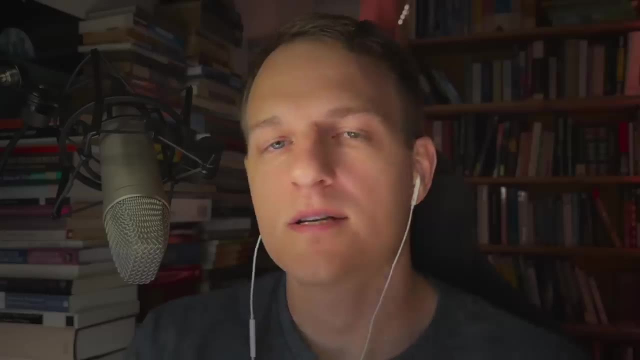 protons themselves into doubles and triplets, making helium and lithium in small amounts, although most of the universe was still single proton atoms without their electrons. so we call that ionized atoms of hydrogen, and it's even speculated that at this point, within still the billions of degrees and 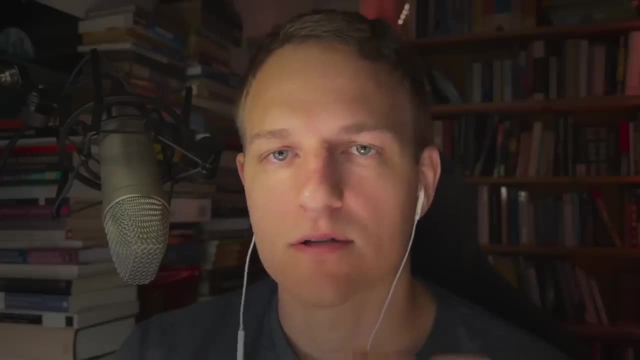 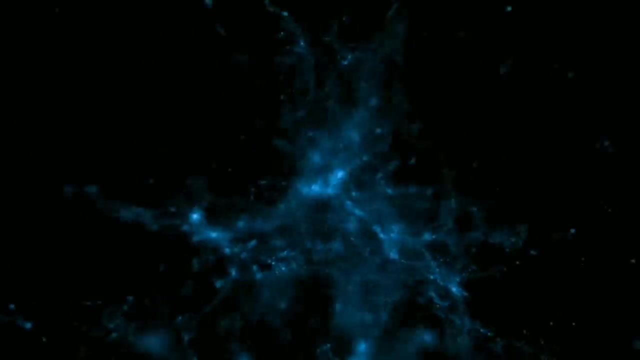 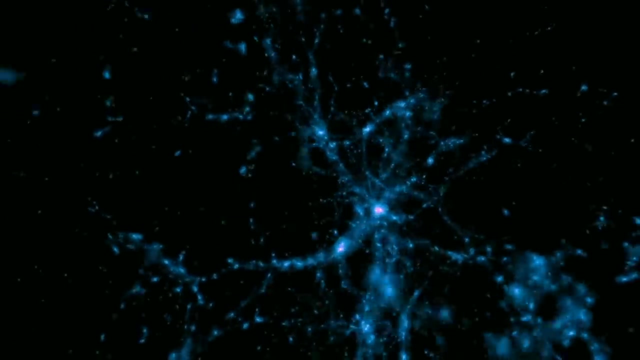 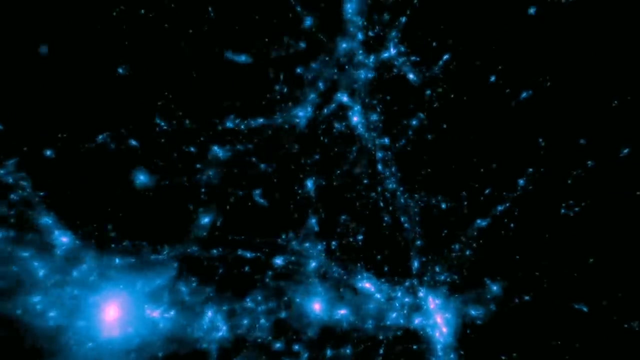 swarming energies in the conditions of this early state of the universe, that primordial black holes could have formed. Those omens could have actually been the origins of the first galaxy cores interacting with the frozen in Quantum fluctuations becoming massive, ultimately massive gravitational attractors that the first stars might 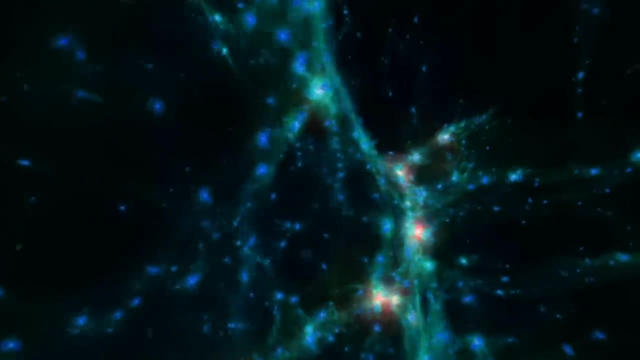 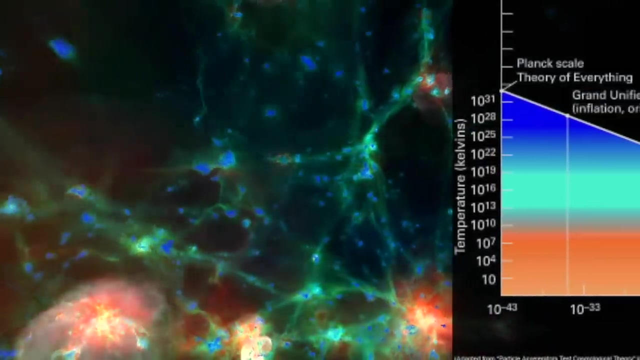 begin to orbit. millions of years later, So at just 20 minutes old, the universe had swollen, broken and collapsed. This was the very start of the amount of energy we could haveね broken its unity, sown quantum fluctuations into the largest scales imaginable. birthed and then annihilated particles and even possibly created the first singularities. By about the first hour, billions of degrees had cooled down to just millions and nuclear fusion had stopped and freezing the abundances of hydrogen mostly, probably about 75% of the hydrogen. 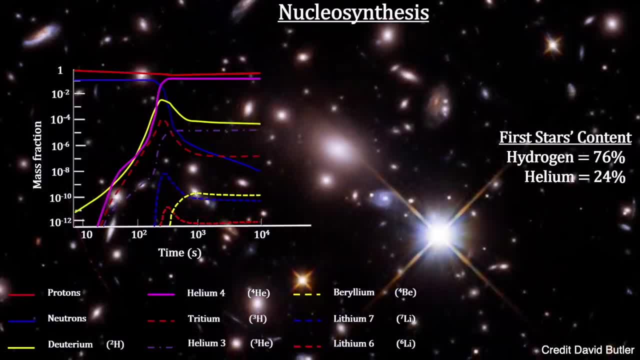 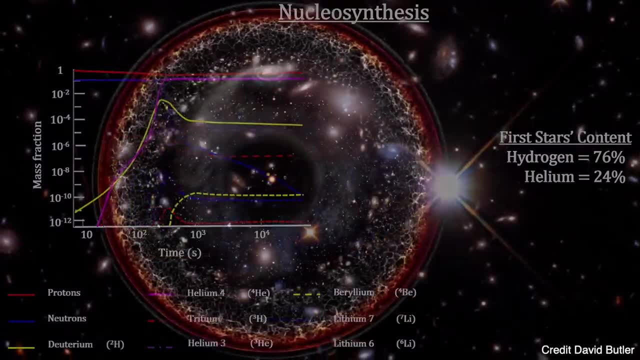 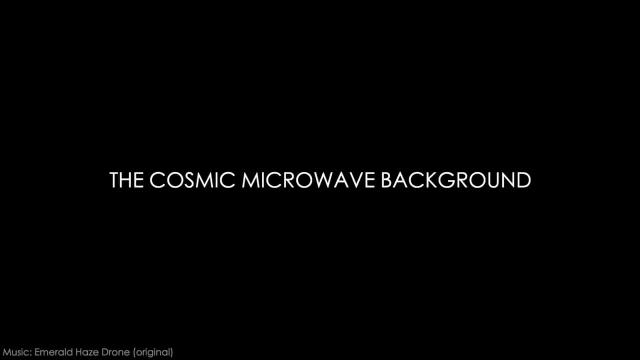 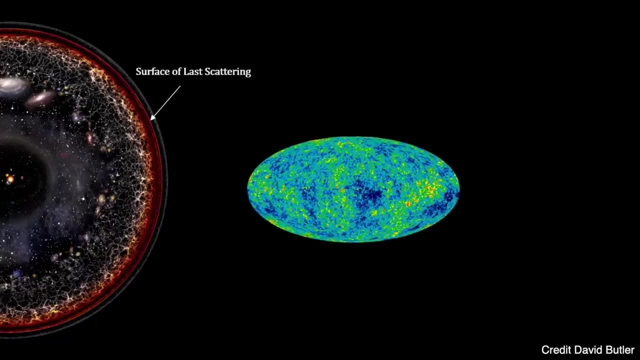 with the remaining 20 or so percent being helium and then a few percent of the heavier three-proton nuclei, lithium. But the entire universe wasn't cool yet by any means. It was now just a white-hot plasma of high-energy radiation. 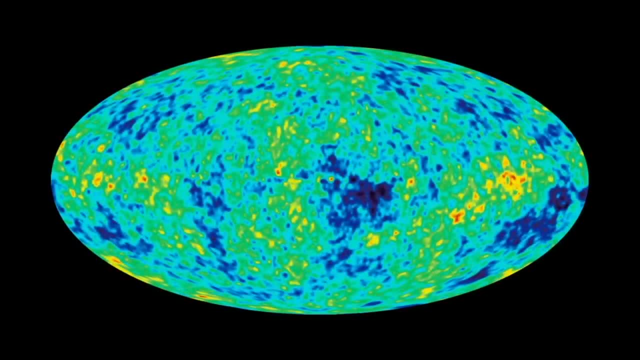 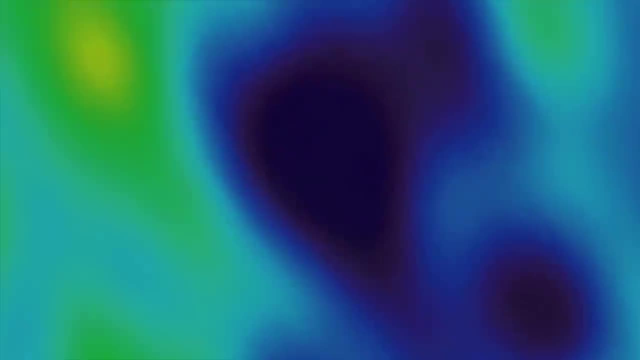 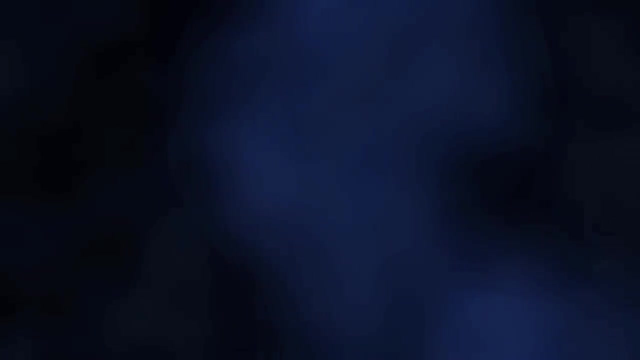 coupled to a dense, cacophonous sea of protons and electrons. In fact, this universe was still at such high energies. it's calculated that there were more photons released here in the next few thousand years from this furnace at the beginning of the universe. 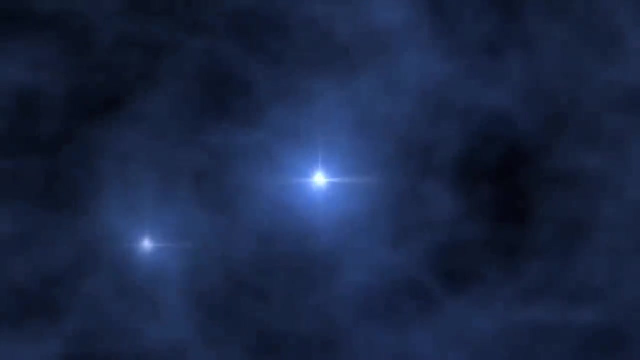 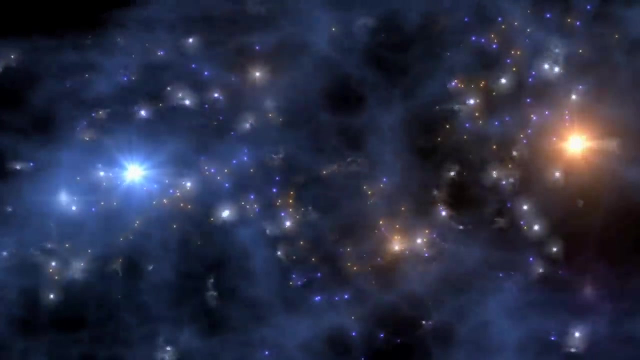 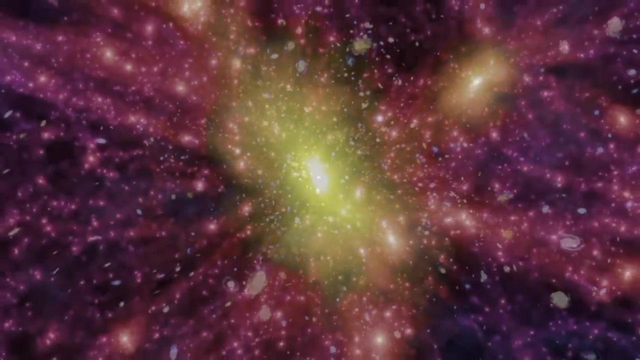 than the sum of all photons from all stars, all astrophysical phenomenon in the 14, billion years since, And despite the fact, despite the fact that there was continually more space for this cosmic flood of radiation to expand into and cool off. 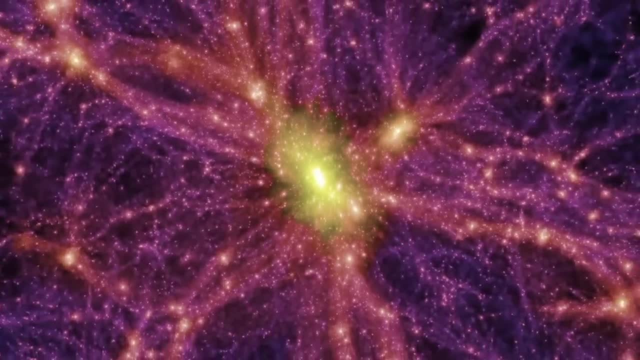 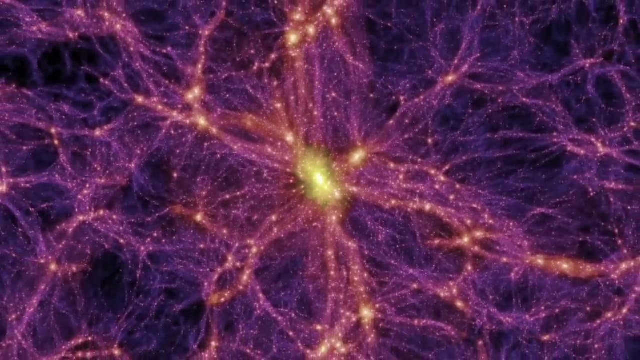 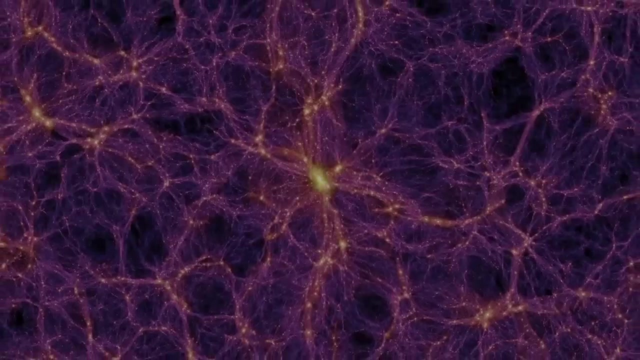 into what is kind of a metaphysical question, of course, but it still took hundreds of thousands of years to do so. It went from millions to tens of thousands to gradually just a few thousand degrees kelvin, And in this first hundred thousand years of the universe. 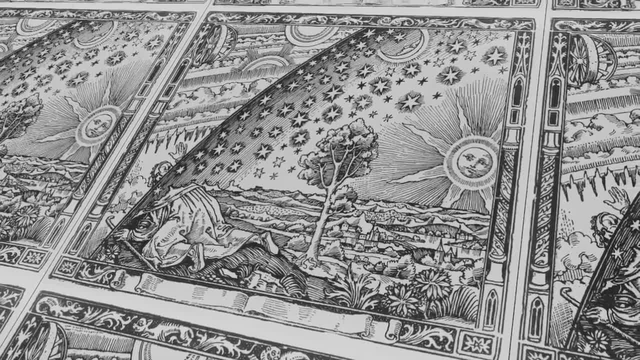 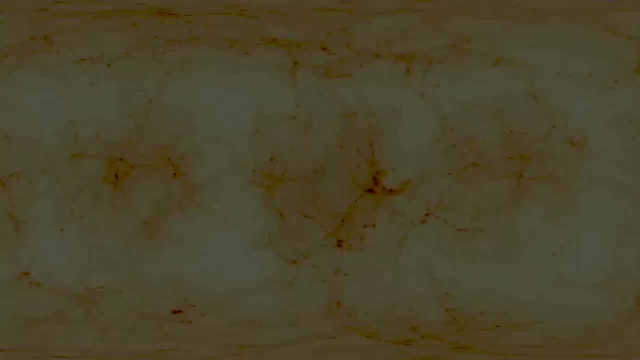 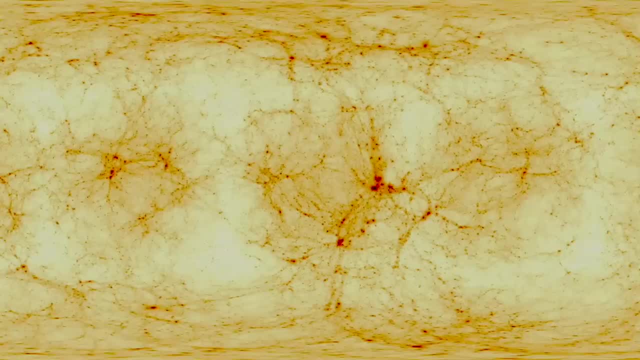 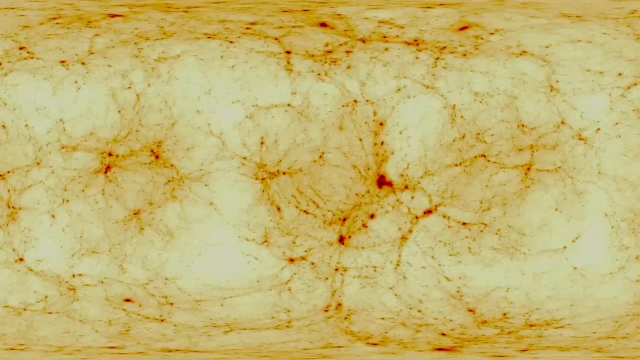 any point in space, whether you're inside it or some metaphysical being standing outside. it would have looked like one continuous, unimaginably bright star. millions, millions of light-years across Matter and radiation, were part of this universe and were perpetually just ricocheting off each other. 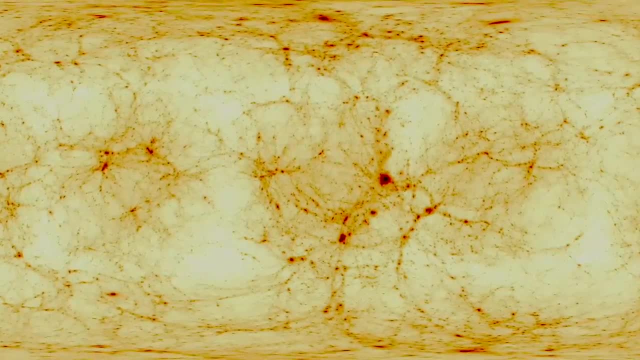 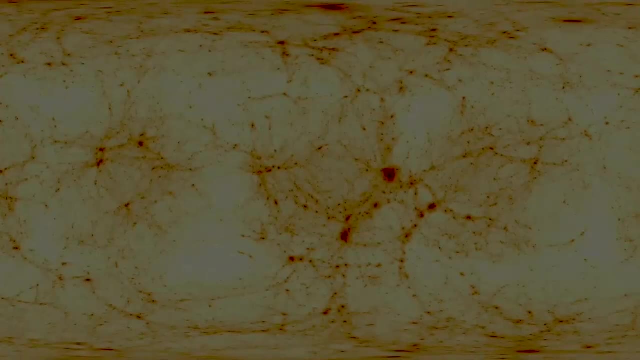 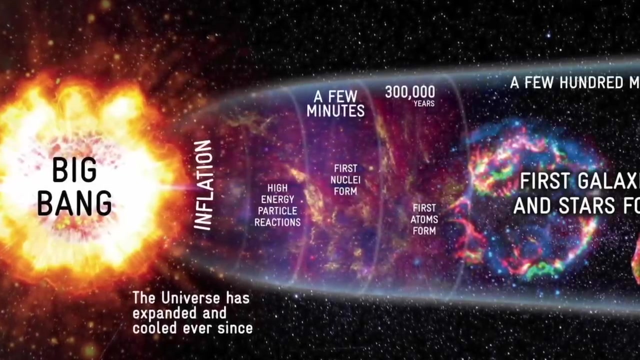 And only at the end of this period of hundreds of thousands of years would they be able to cool off enough to dim the cosmic lights just a little. Finally, at about 400,000 years after the big bang, the environment allowed electrons to bind to protons. 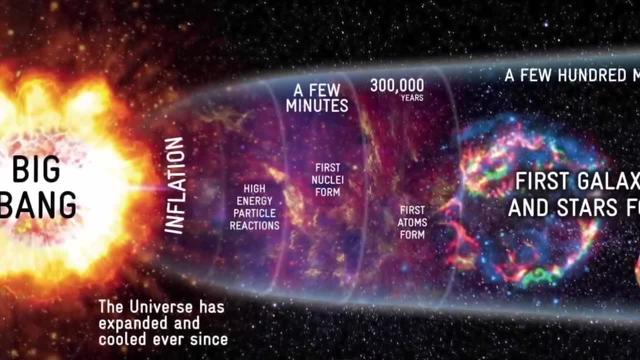 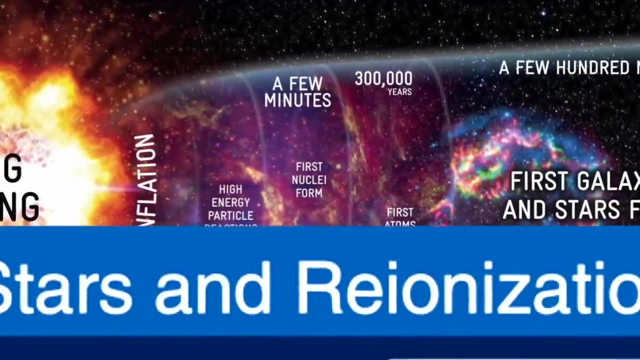 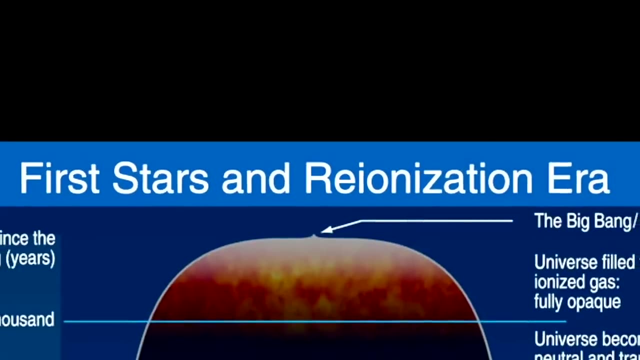 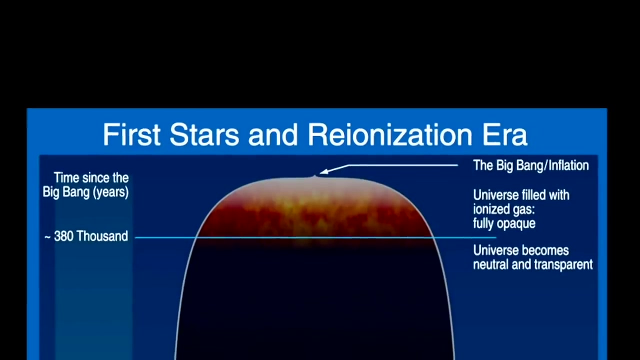 forming the first atoms in the glow of the cosmic furnace We have existed within until this point started to quiet down a bit For the first three million years. all we'd see if we were some unfortunate being left to drift in the near-infinite, boundless field of simmering down matter and radiation. 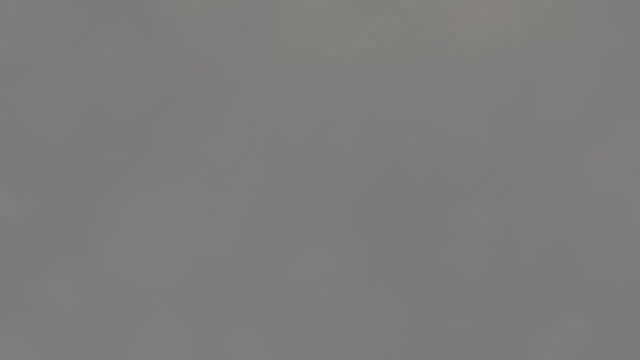 all we'd see is this omnipresent wall of white light- white initially, though, and then gradually fading. It would probably seem like we were at the center of some massive hollow star whose interior walls were glowing towards us but also receding at the speed of light. 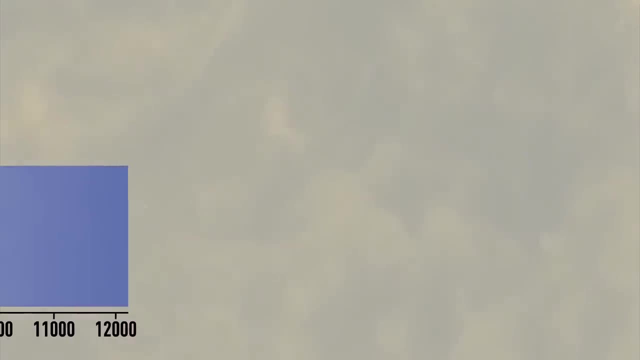 Once this initial grain of sand that we talked about had continued expanding to eight millimeters, eight kilometers, eight light years, eighty million light years by about that point, that wall of receding light being about forty million light years away from us. 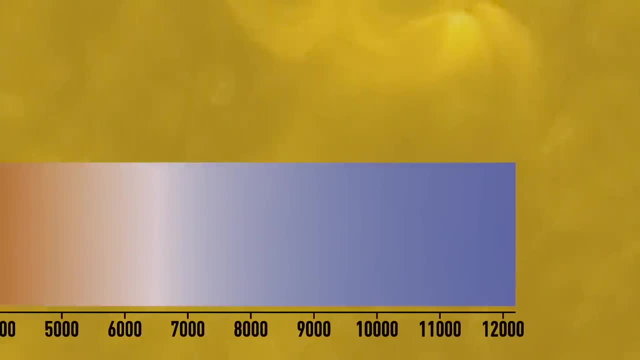 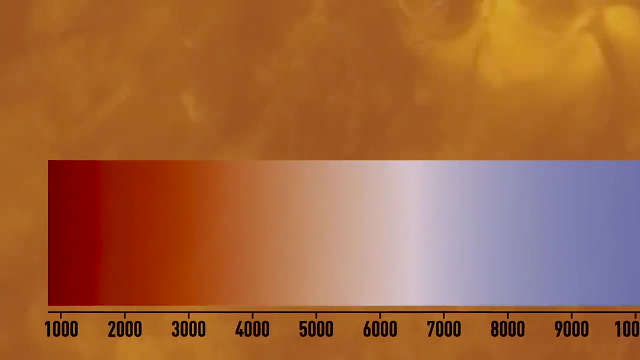 things were now cooling and their light was becoming dimmer and redder. Then, as it receded over hundreds of thousands of years, it would dim and grow yellow-orange and, as this orange cloud finally gave way to more, more of a diffuse gas, 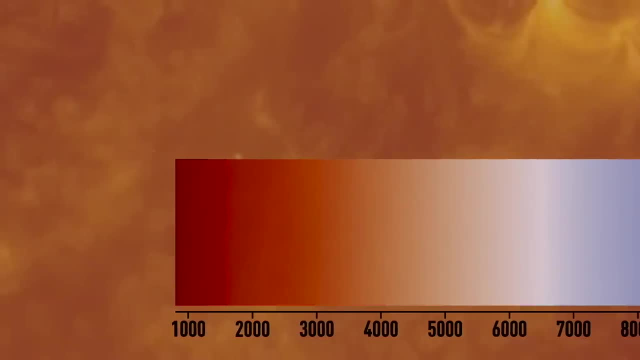 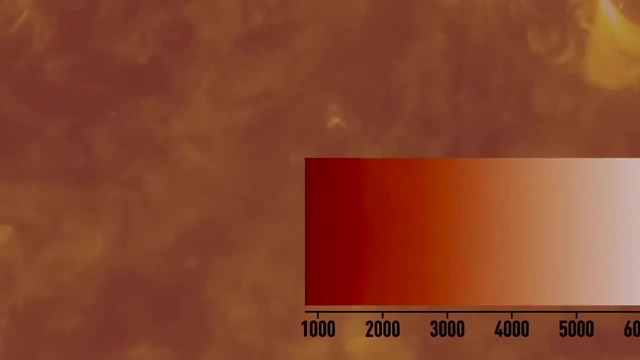 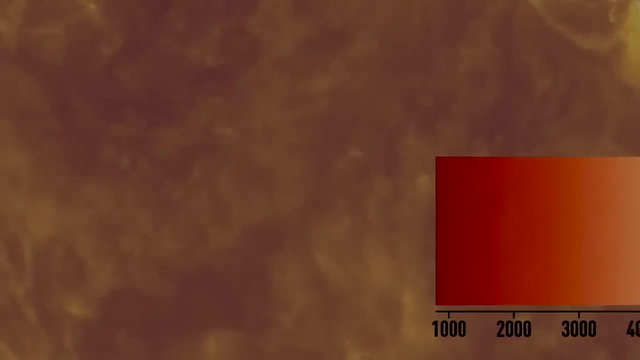 getting redder and fainter with each passing millennia, its light, and eventually even its warmth, would extinguish altogether. And it's here, at the beginning of time, and in just the first few million years of existence, that the universe entered. 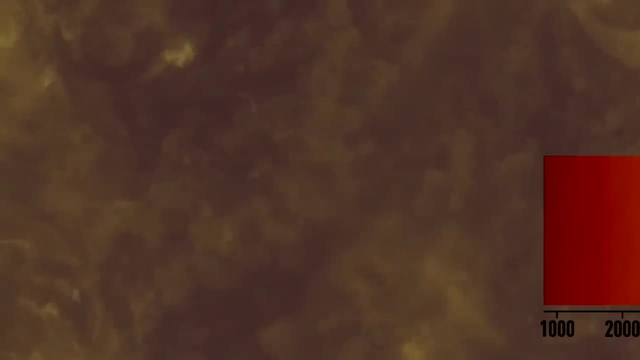 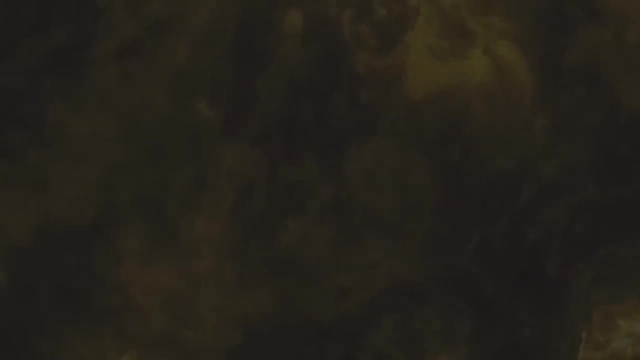 into what's called the Dark Ages. Nothing but darkness, Nothing but diffuse clouds of hydrogen and helium, cooled off until they lost their glow and warmth and were expanding diffuse matter. All light from that ancient background wall. 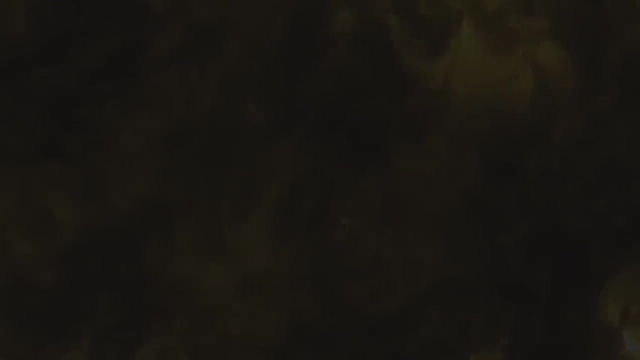 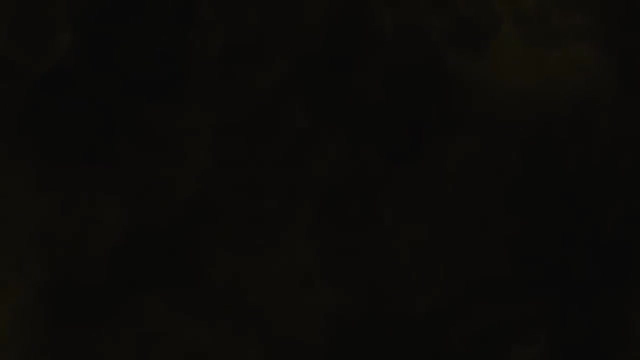 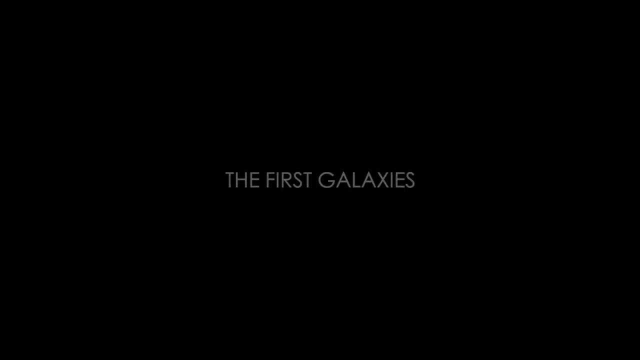 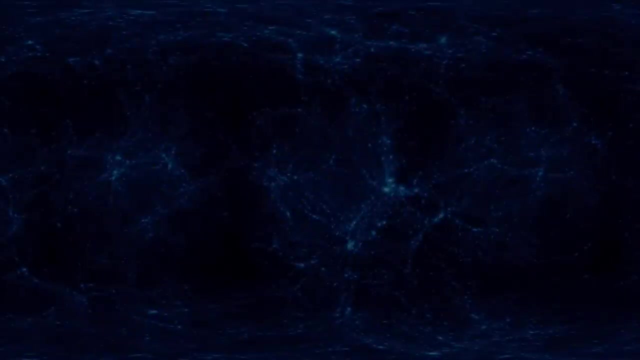 traveling away, had long, long since dissipated, No new light would form for almost a hundred million years after this Just black. Since then, that matter that emitted that warm glow has in the intervening time, 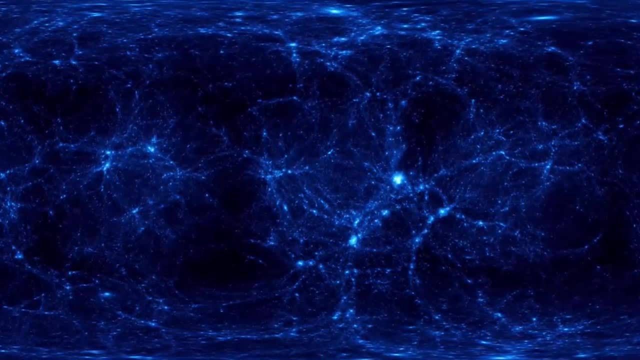 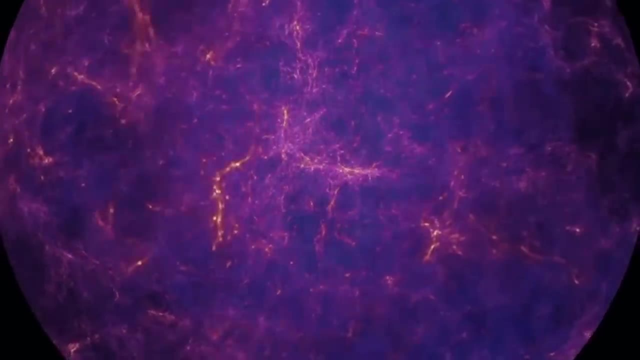 mostly condensed into galaxies, with the remaining matter being superheated into intergalactic intercluster gas in the intercluster medium, And those galaxies are now calculated to be about 46 billion light years. 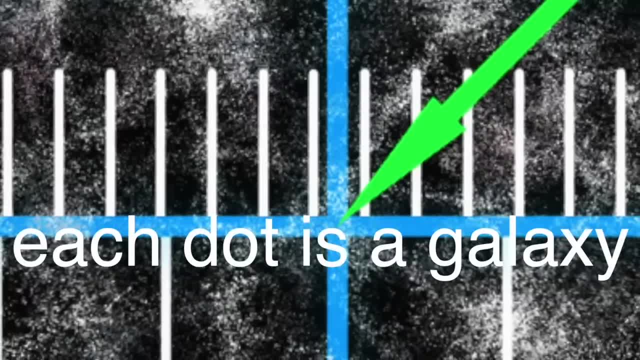 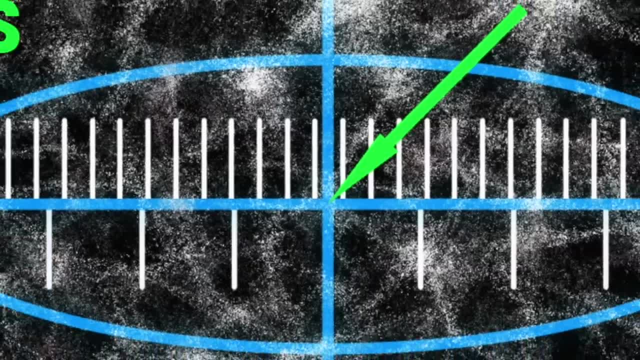 from us today. That's a shift of about a little over a thousand times further away than that 40 million light year distant wall of 40 million light years from us today. That's a shift. 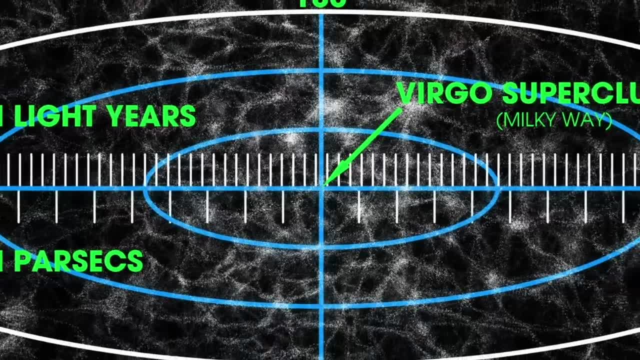 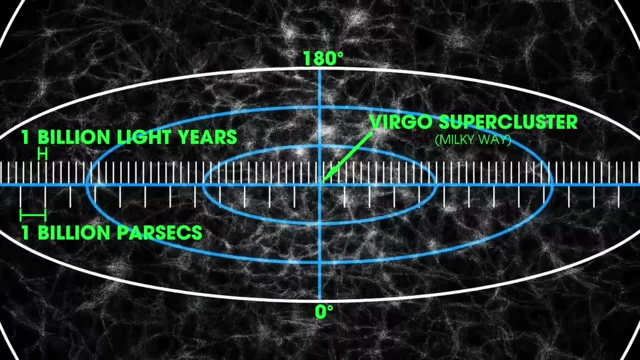 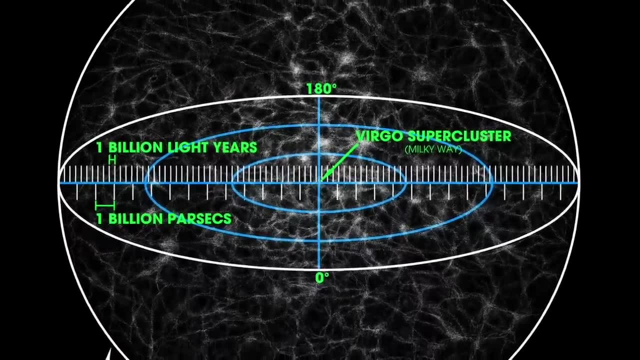 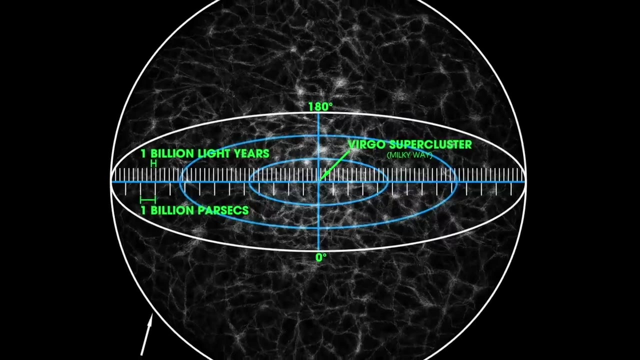 of about a little over a thousand times distance. wall of finally dimming light was. But the universe might not be as infinite as this makes it seem. The actual size of the whole universe: 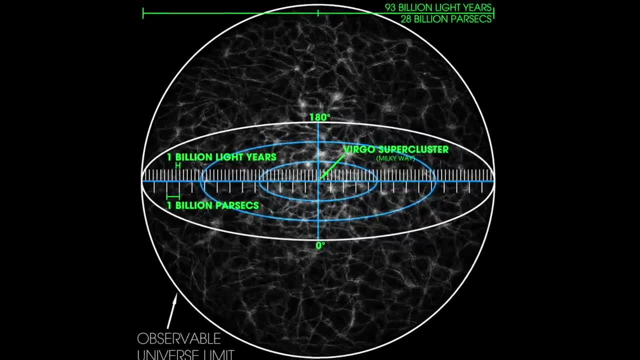 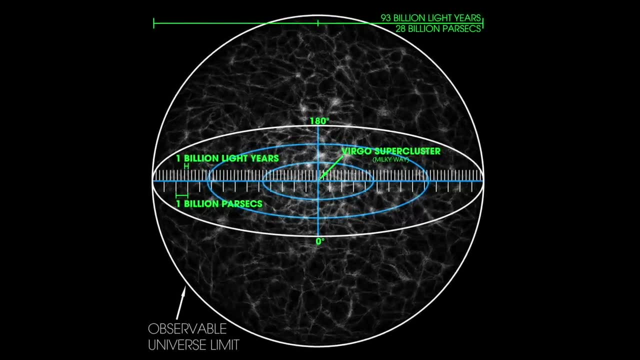 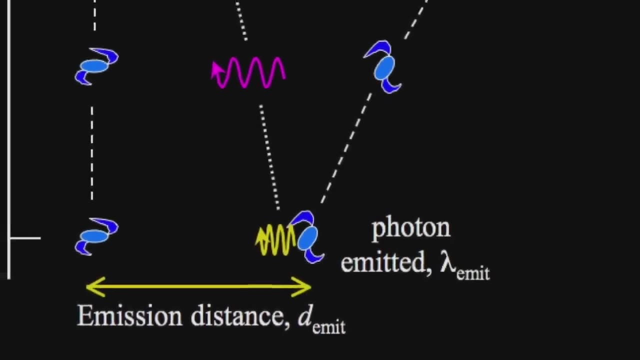 see, this is where the distinction between the observable universe and the true universe, capital U universe, is important, Because light, at a certain point, is being one of the fundamental speed limits. 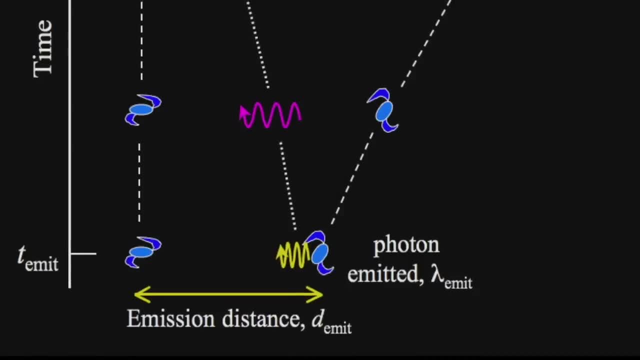 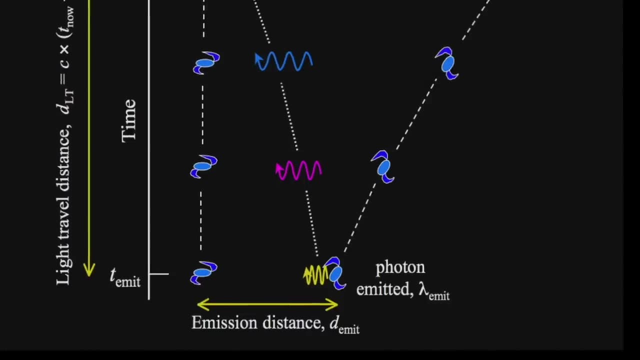 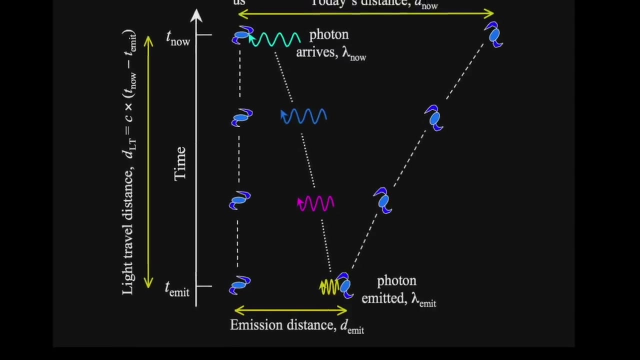 of the universe, constraints in the physical limitations of the universe. Light cannot travel faster than its own speed. Now, with space stretching, it can cover distance, cover distances further than a static universe. 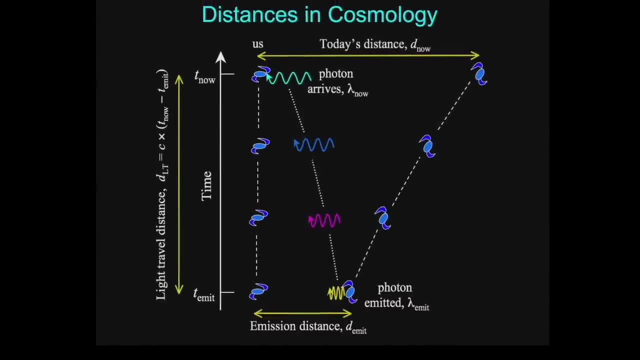 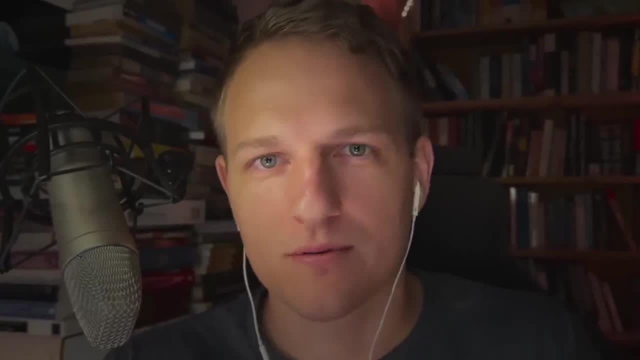 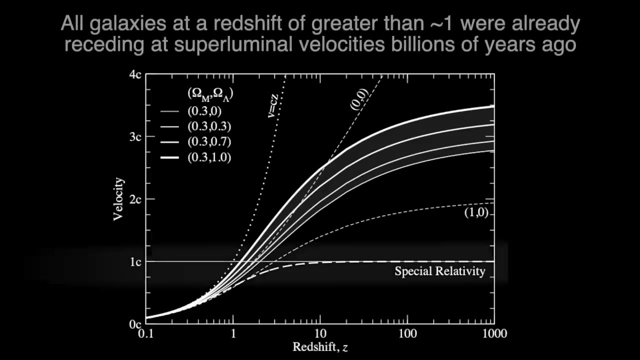 would allow light to travel Because, as it travels, almost like walking very fast on an airport escalator or one of those moving sidewalk fancy situations, Although the distance between two objects will continually. 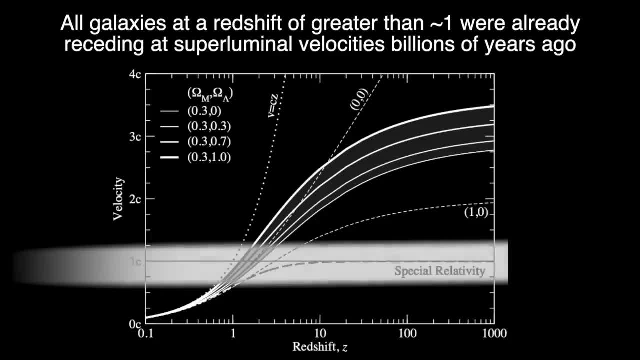 expand The distance between the emitting object, the object, the galaxy, let's say that emitted the light, and the light, the, the head of the light beam itself will have also expanded, So it'll. 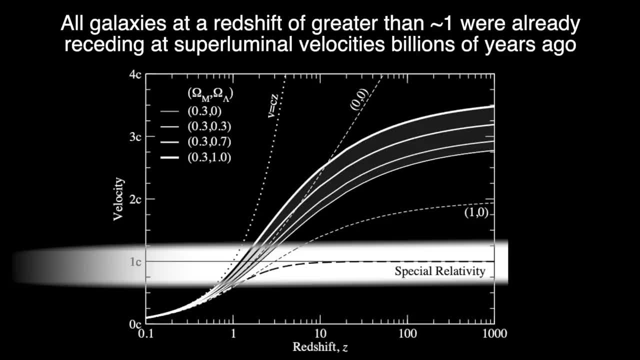 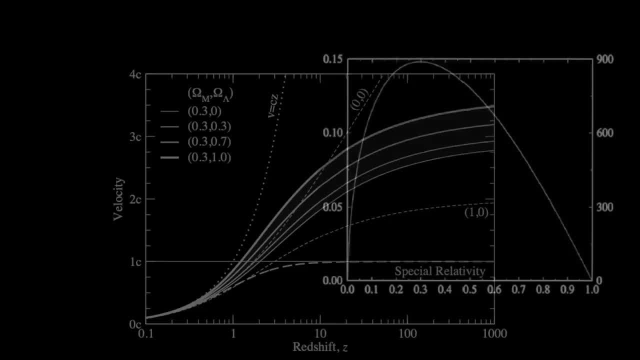 have expanded into a distance larger than that, light would have traveled from the emitted galaxy in just a static universe itself. So it seems from the emitting galaxy's perspective that the light is receding away. 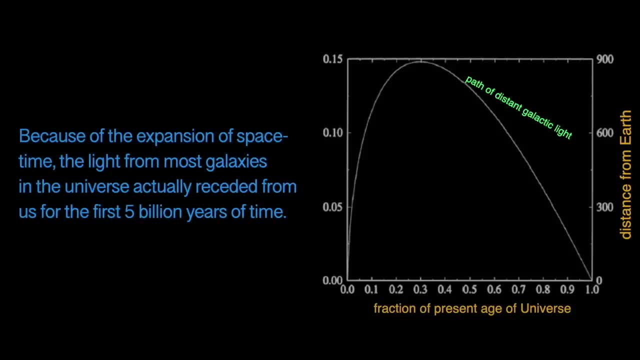 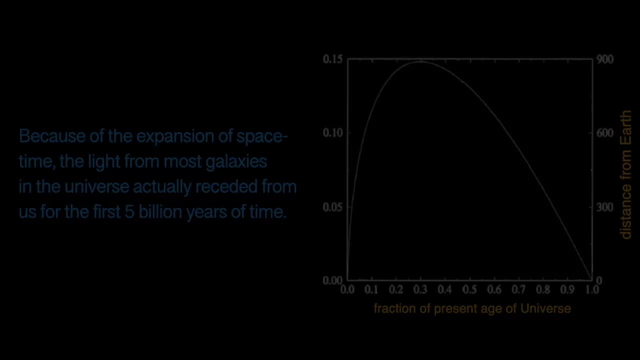 at greater than possible light speed would ever allow for, And, in fact, one of the furthest galaxies until some of the amazing discoveries that we're about to mention today was at what's called 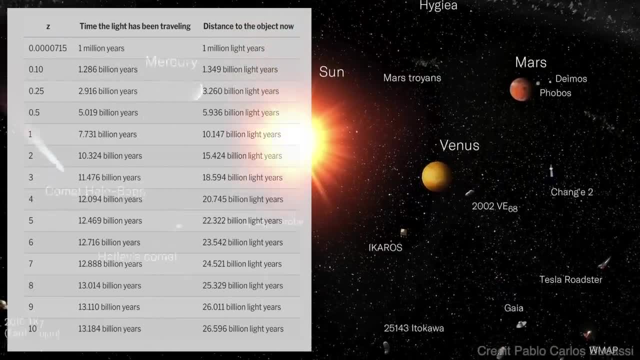 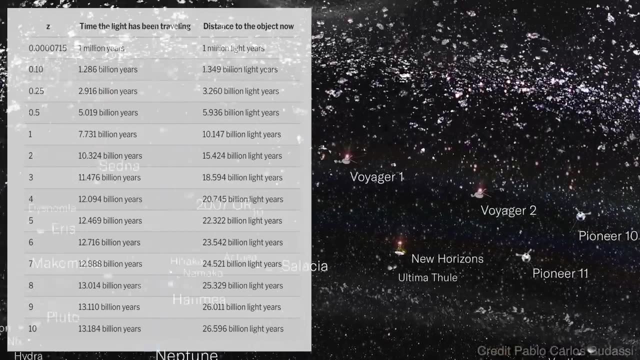 a red shift of 11.1.. And that meant that that galaxy, that emitting galaxy, was so far away from us even back then, at the earliest, within a few hundred million years of the universe. 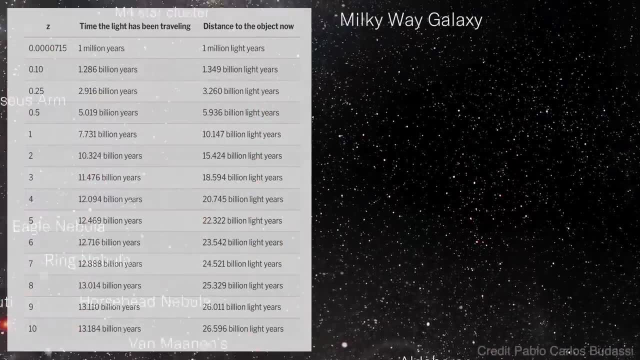 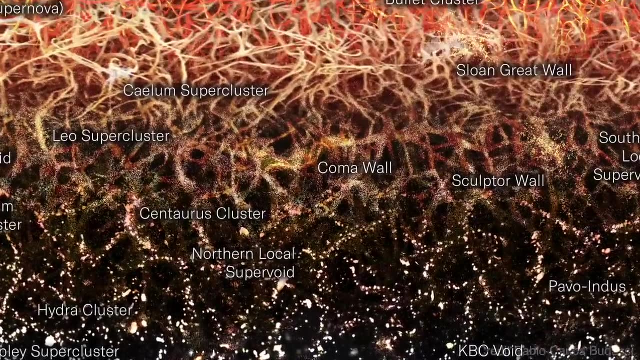 It was traveling. the expansion of space was causing it to travel and us to travel from it, at a speed four times greater than the speed of light. Now, of course, light can't keep up with that. 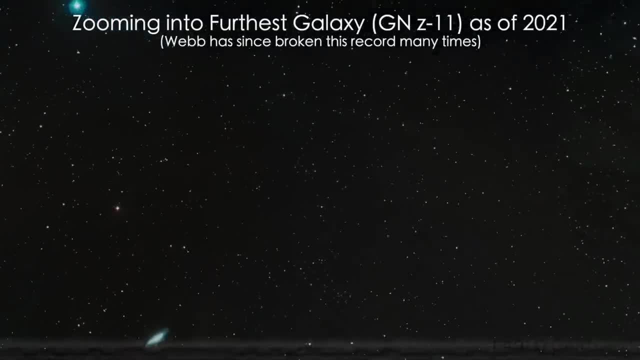 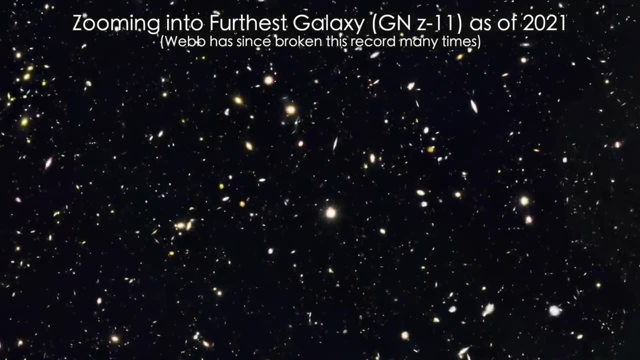 So at some point that distant galaxy will recede, just like that wall of light, into a redder fainter out of the visible spectrum, into obscurity at the edge of our observable. 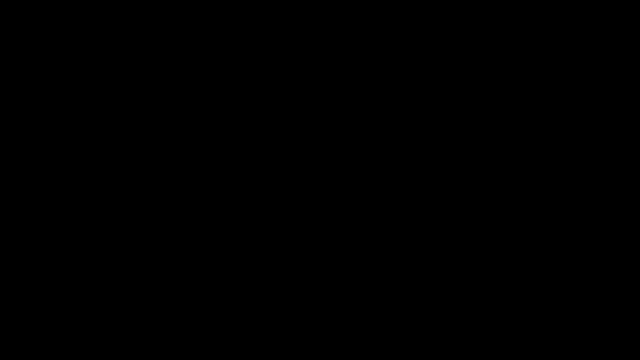 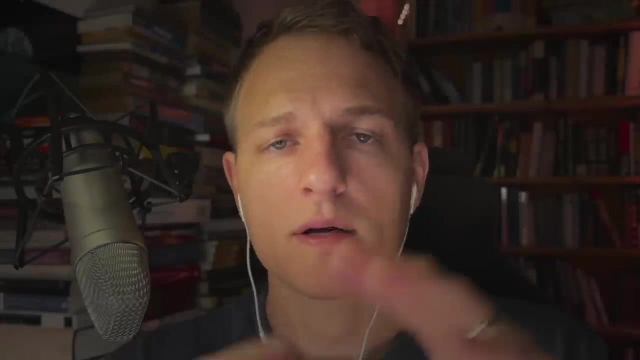 universe, And so that's all to try to give you an idea that our pocket of the universe is limited by the galaxies whose photons we will, and at a certain point there's a boundary at which we will not. 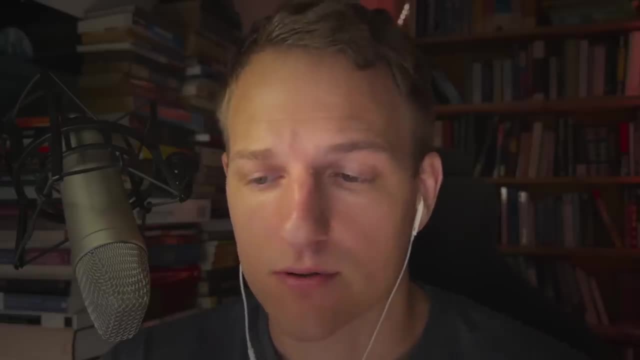 ever be able to see photons a certain distance from us, And they're so far that and receding so fast that their light, despite traveling towards us, will never cross what's called the event. 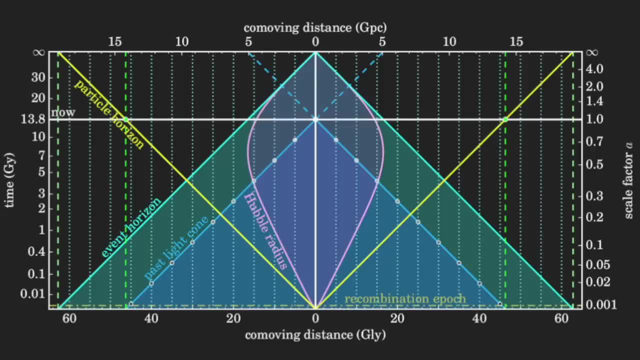 or particle horizon of the universe. So the size of the universe isn't known, And in fact it's thought that, according to even mainstream cosmological models, the universe may not even have a physical boundary. 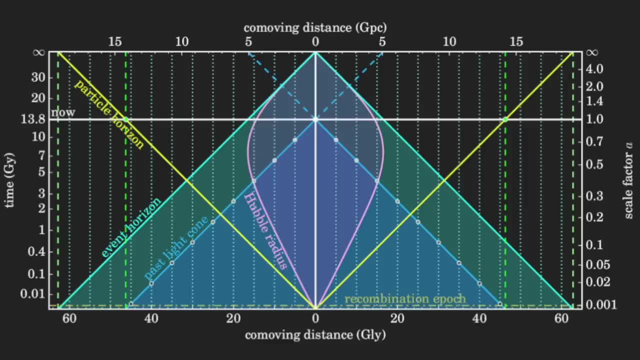 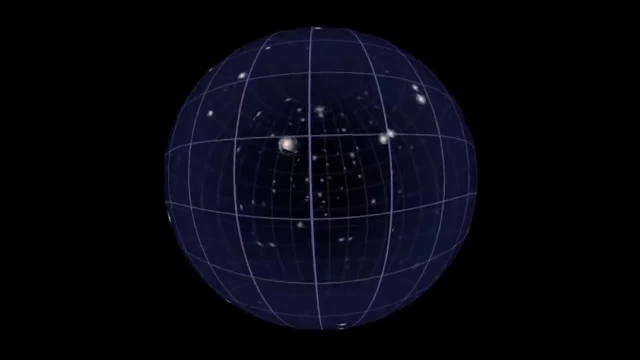 in the first place. So every point in the universe, whether it's inside our observable universe or outside it, has its own radial lines that will never reach any sort of boundary. So it's really important. 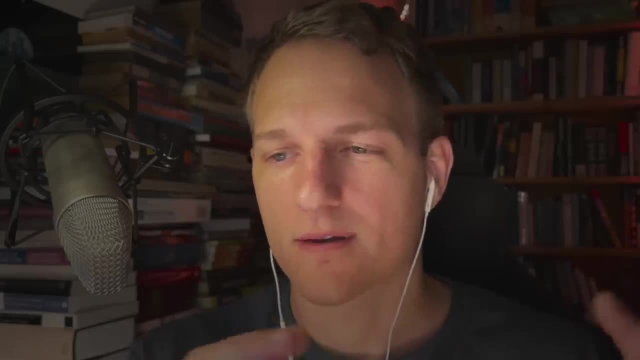 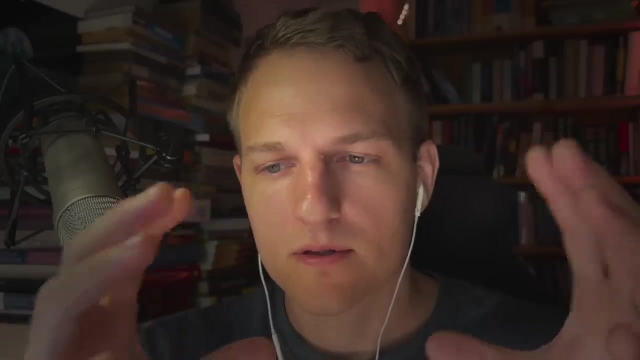 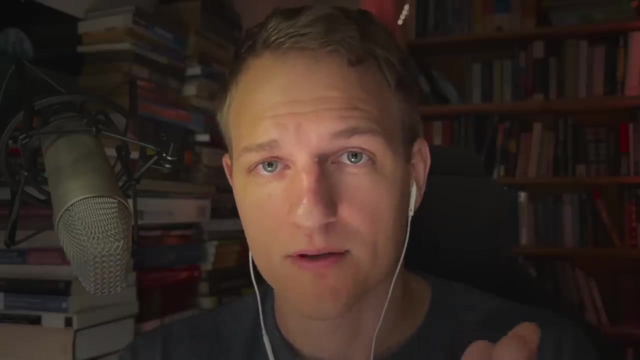 to understand that we will never be able to see distant galaxies beyond a distance that cosmologists have calculated was about 46, billion light years away from us now, So meaning. 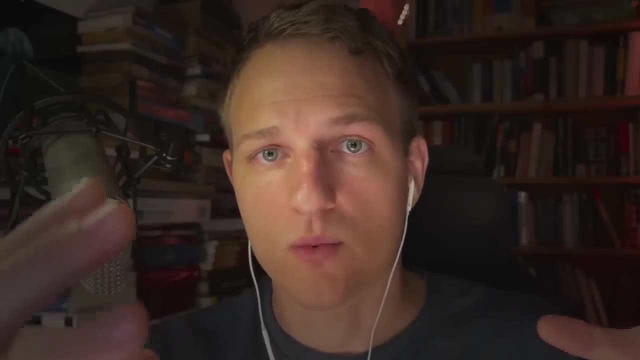 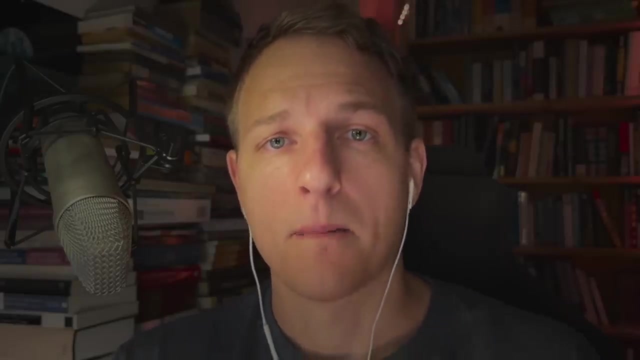 the diameter of the, the sphere in which our that, that defines our observable universe, is about 93, billion light years across. It's way more than just the 13.7, billion years. 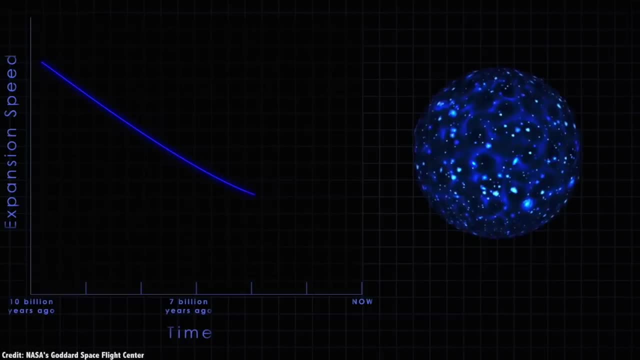 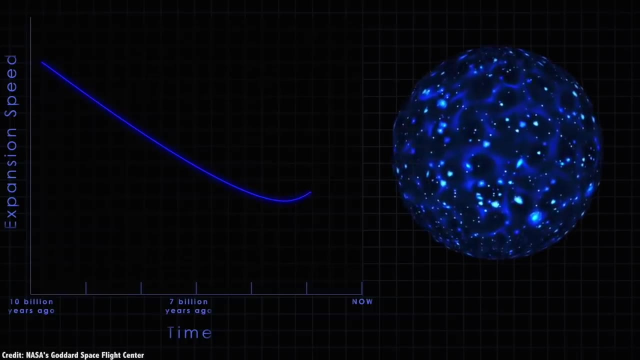 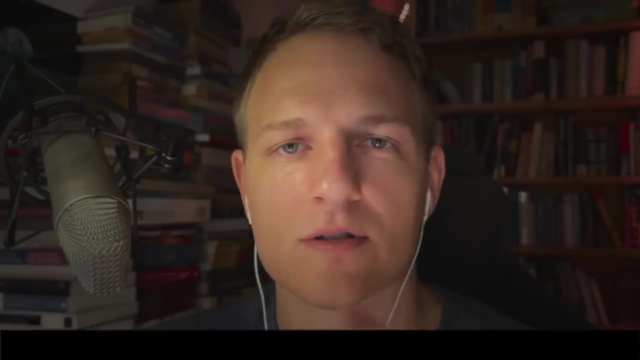 that light could travel since the beginning of the universe And that's due to the expansion of space, as will be documented diving into later. But even then that's just a speck. 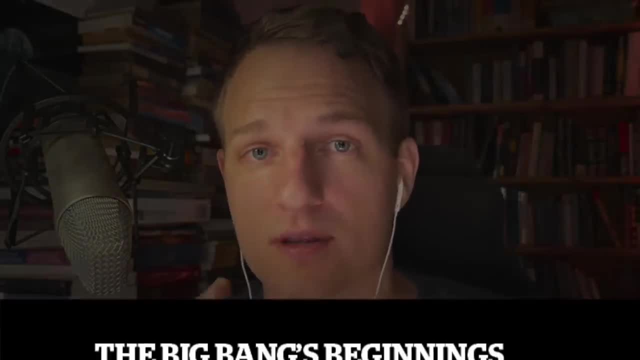 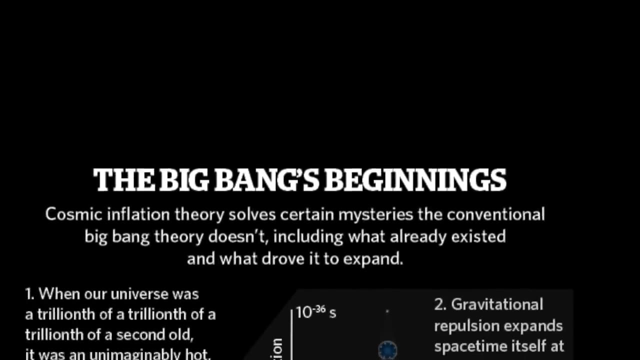 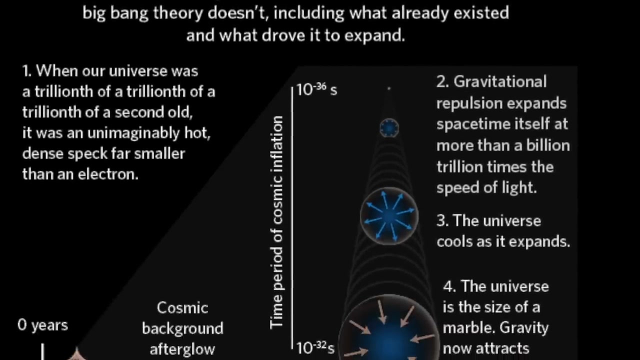 according to even mainstream cosmological models, that's just a speck, a small fraction of the subset of the potentially larger, proper universe that we live within. but of course, 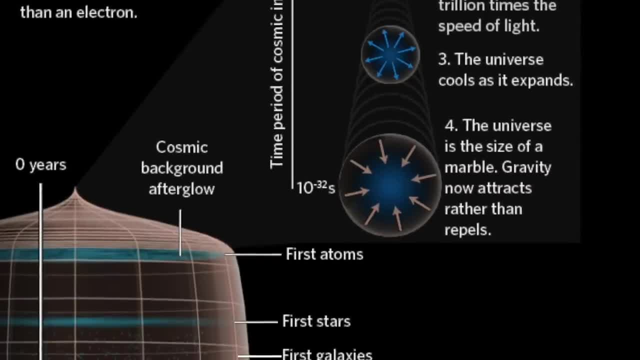 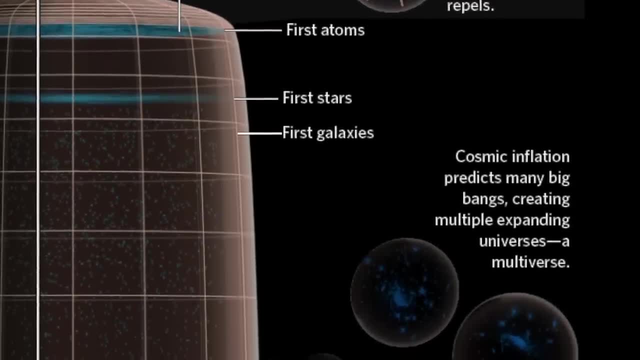 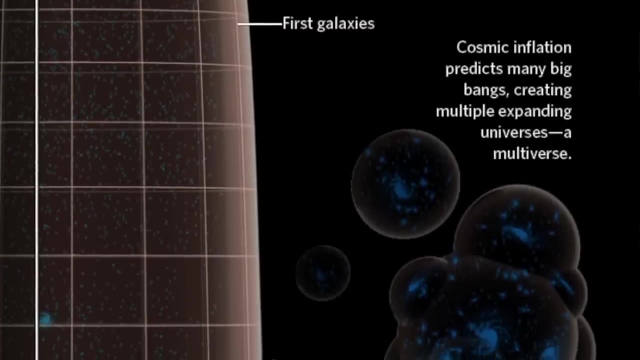 we can never observe or detect, and there's even some cosmologists that would take that as far as to say that, if not being billions of times larger than our observable universe, 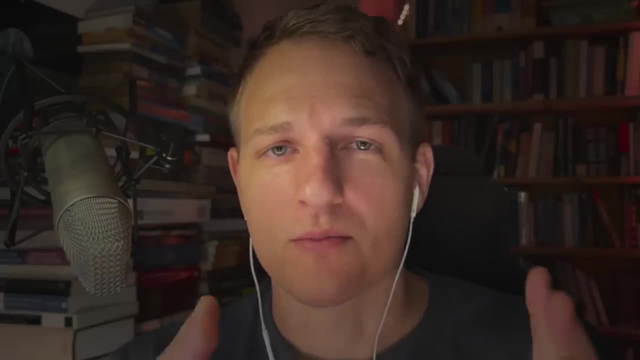 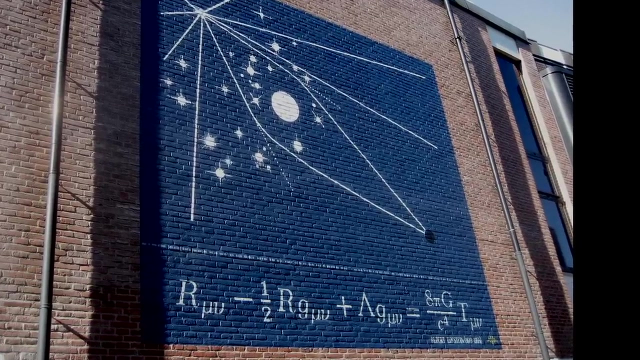 it might just be infinite. Another really interesting, fascinating possibility, given well, giving you information about the universe, the parameters which cosmologists use to try to characterize the fundamental nature. 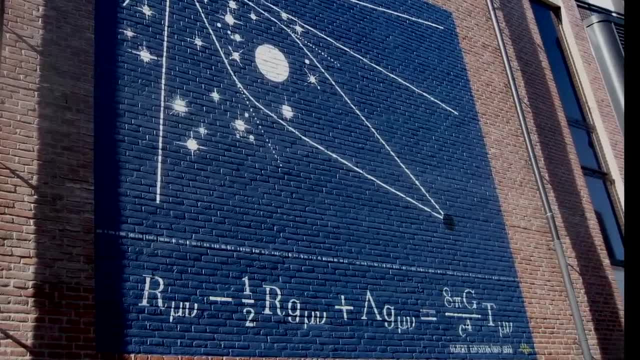 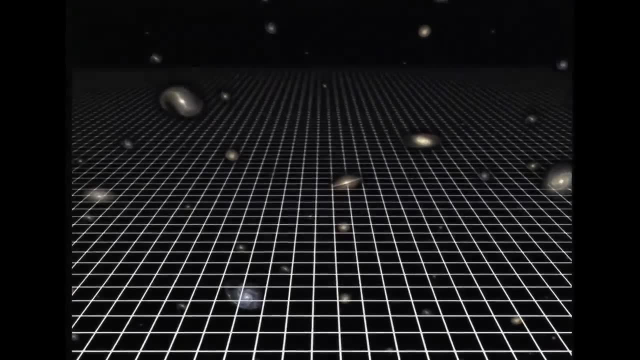 of space-time at the farthest and grandest scales of the universe is the curvature of space-time itself. and if our universe is flat, like they think, then we do have a universe. 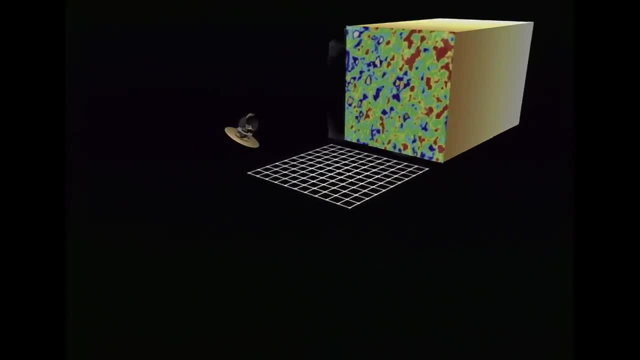 in which it is expanding outward and in which there is no limit. but if it is, maybe maybe we're- and this is a huge possibility- detecting and our observations and our data. 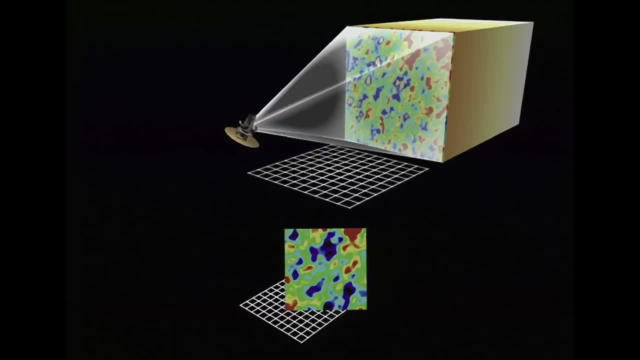 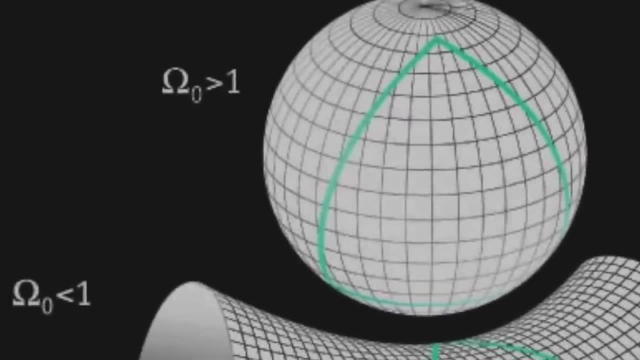 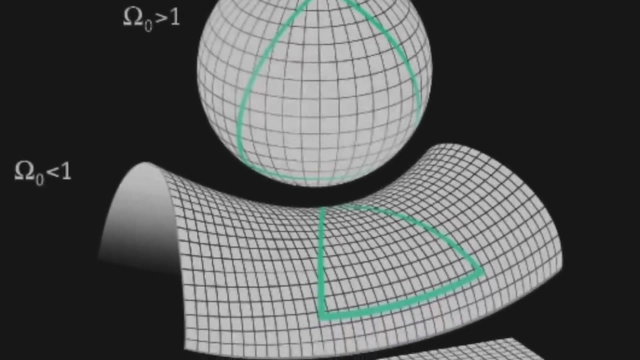 of the deepest galaxies and phenomena in the universe is inaccurate or we're being we're misreading it, then the curvature might actually be flat. curvature would be flat. 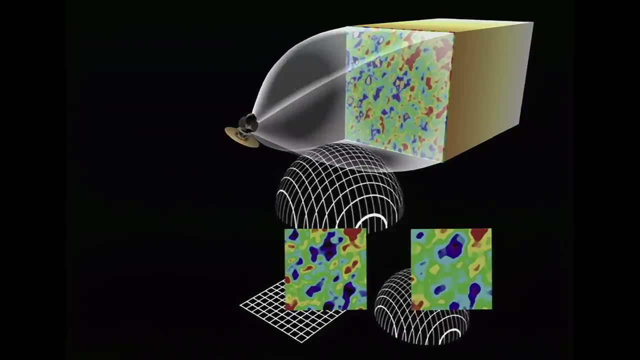 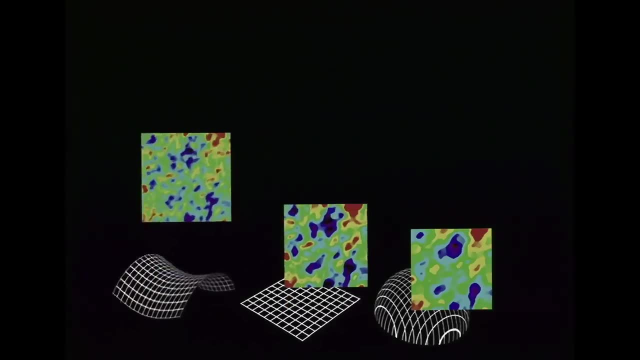 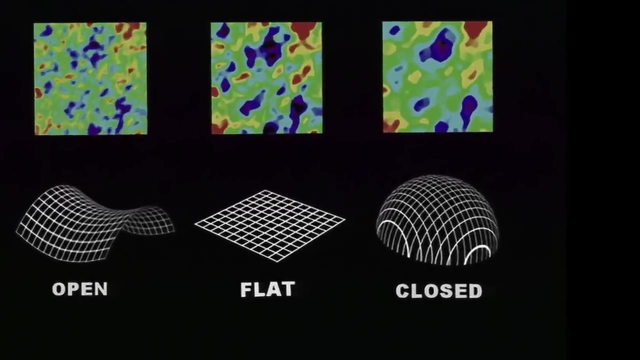 positive curvature would be essentially the 3D analog, three-dimensional analog of a two or the four-dimensional analog, rather, of a three-dimensional globe that has curvature in which 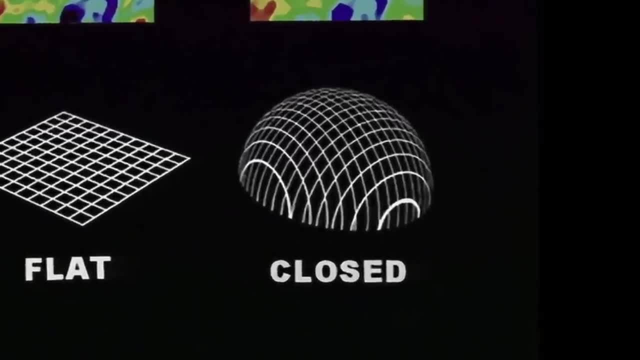 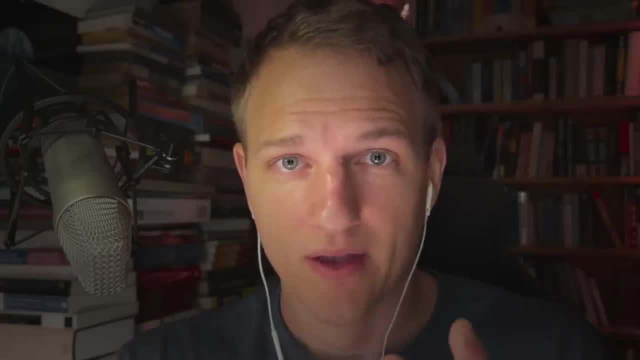 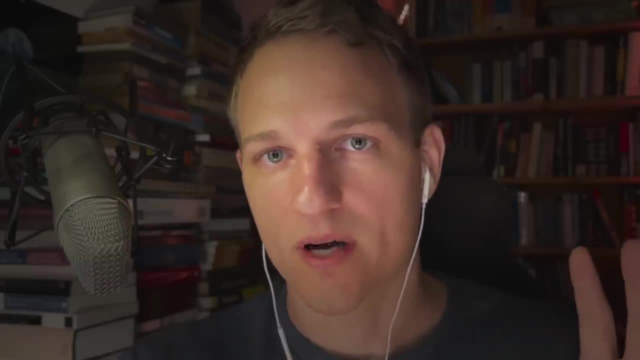 overlaps, laps back onto itself, which, if it does have a positive curvature, the universe we live in. that means that it actually isn't 43, or 46, billion. light-years in radius, but it's actually smaller than that in the furthest galaxies that we're as traveled along a curvature for such a long time. 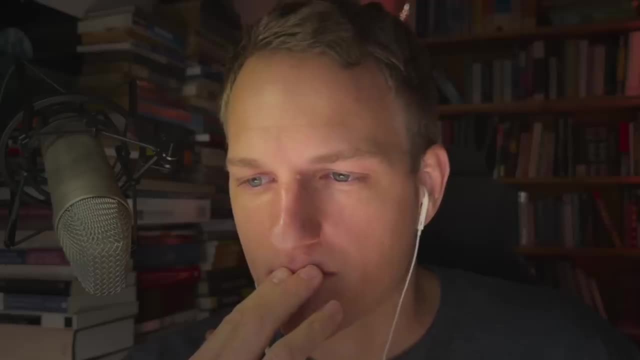 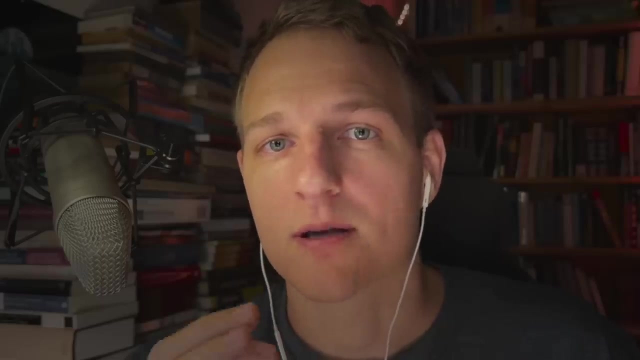 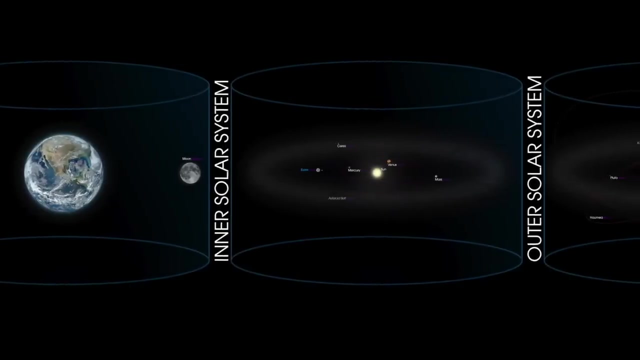 that it loops back onto itself like a sphere, so some distant galaxies might be duplicate images of nearby galaxies, and this is one of the. 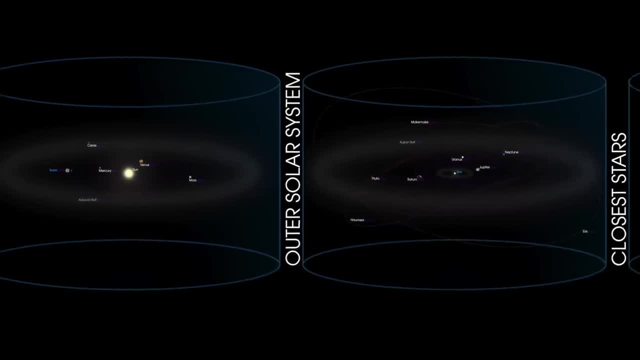 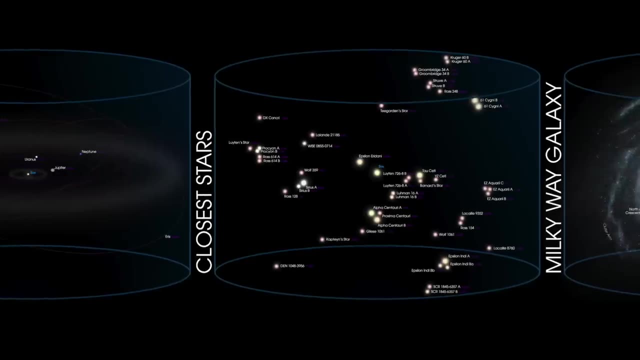 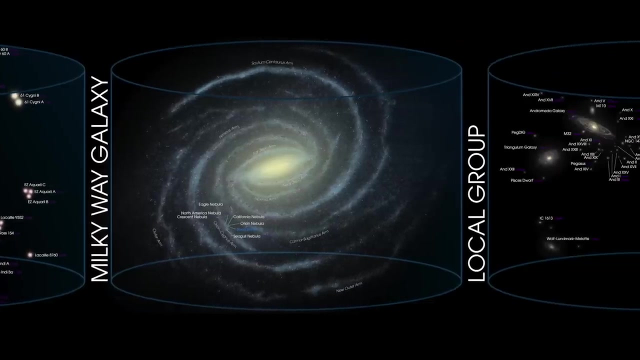 many things we still haven't confirmed. another thing is another aspect of the universe is its structure and its hierarchical structure: neighborhoods of local clusters. 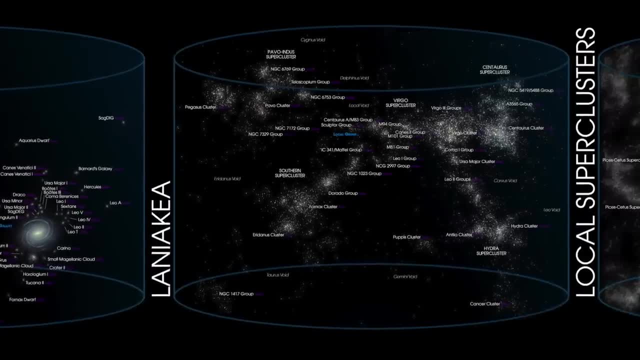 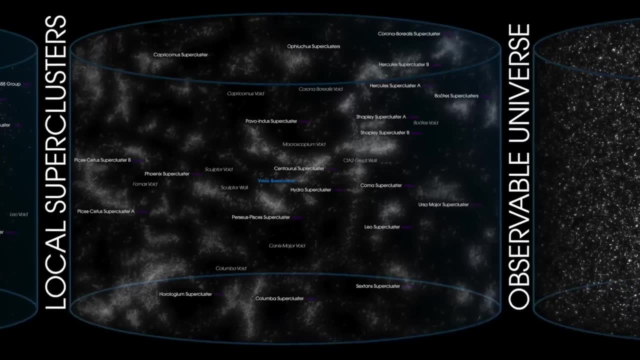 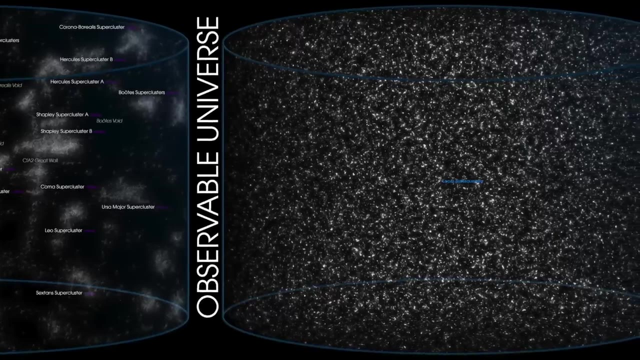 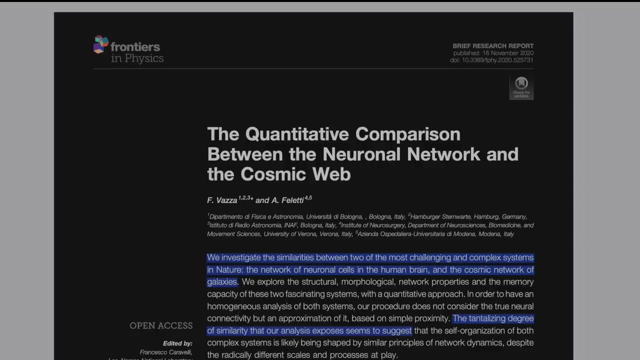 then larger super clusters. these get on the scales of hundred tens to hundreds of millions of light years across. and at that point these, these 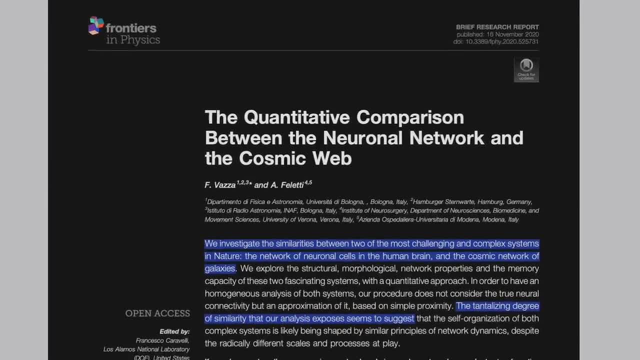 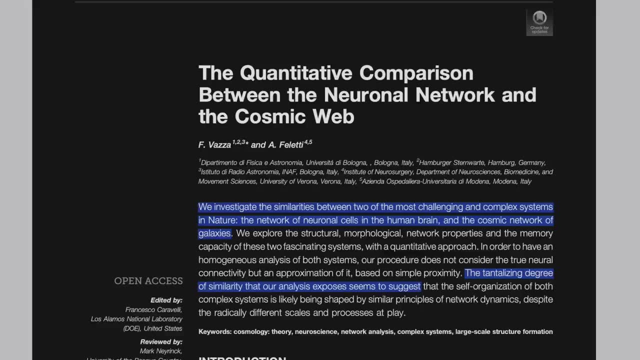 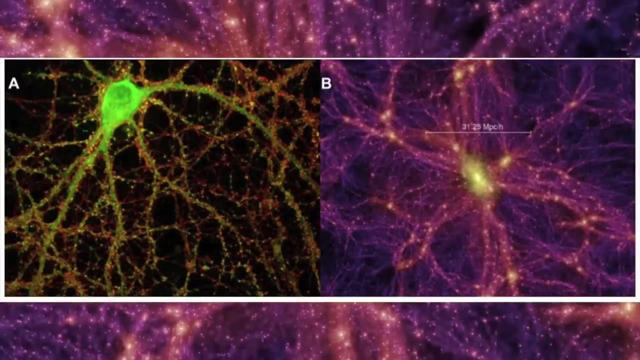 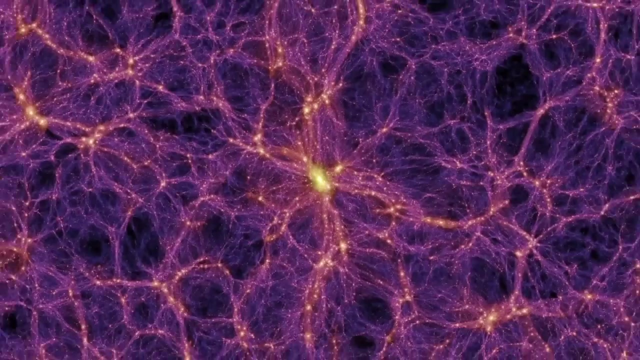 structures. if you scale that out far enough, the groups of filaments form into walls and sheets. it's thought that at this point this is 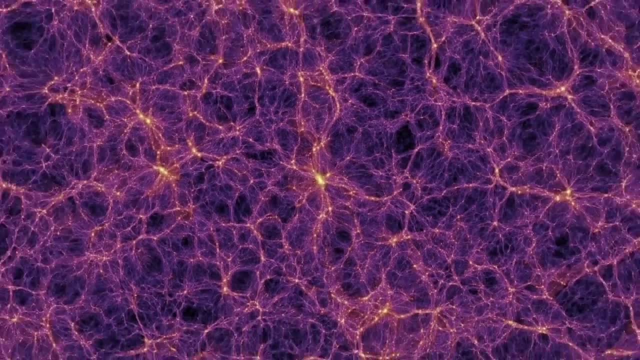 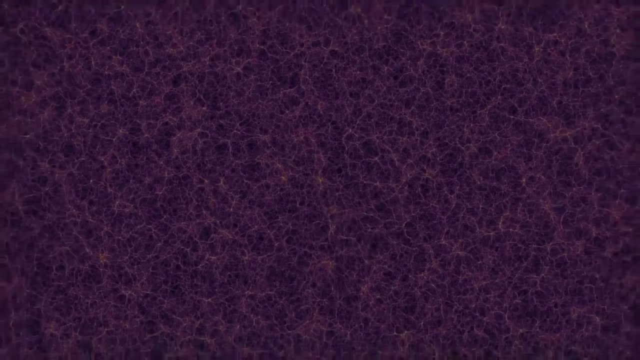 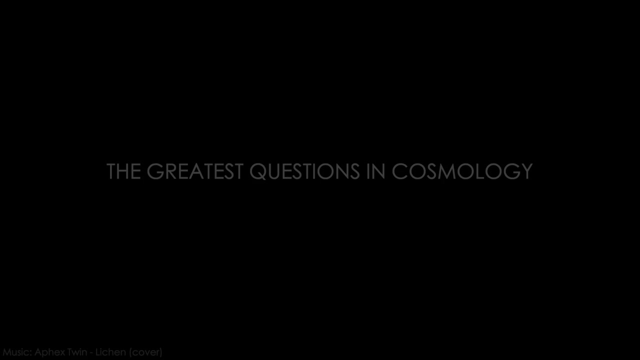 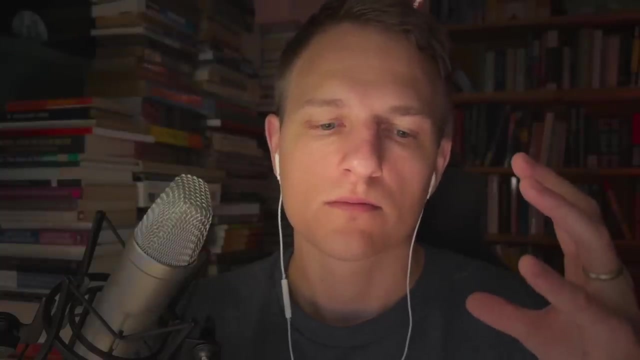 what's called the end of other galaxies. there are no swirling centers of mass around which super clusters swirl, but we didn't know this until. 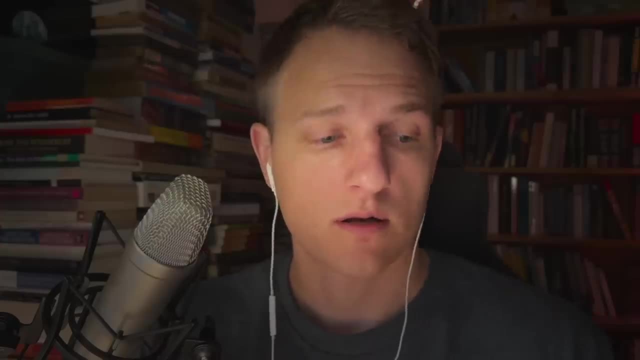 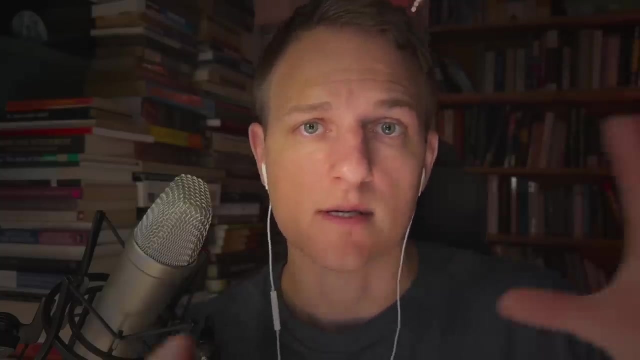 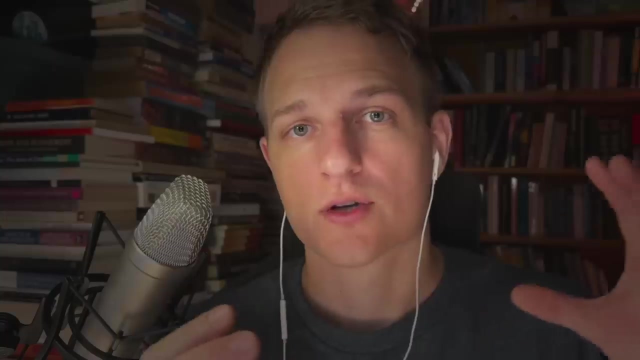 recently. it wasn't until the nineties that cosmologist sent steps to be able to see and piece together maps of our observable universe on. 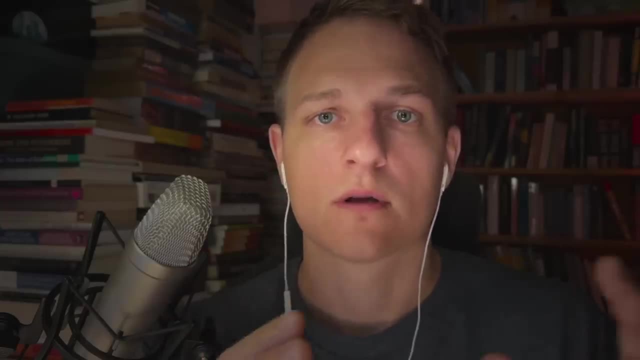 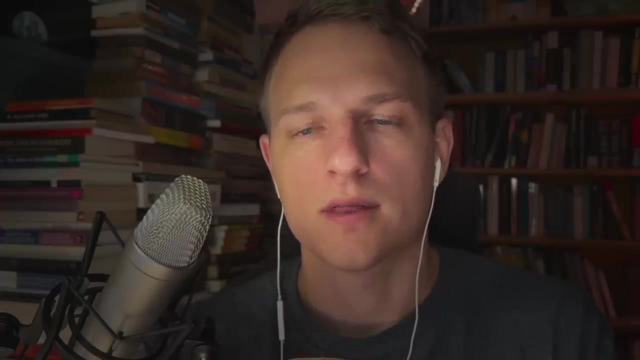 these grandest scales and really determined that it is a homogenous, smooth sponge foam, like so much about the universe. still we have so many. 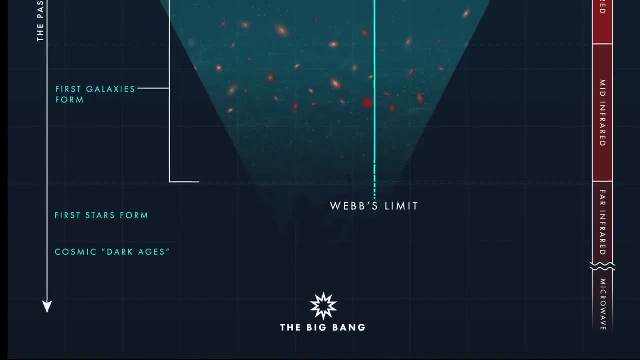 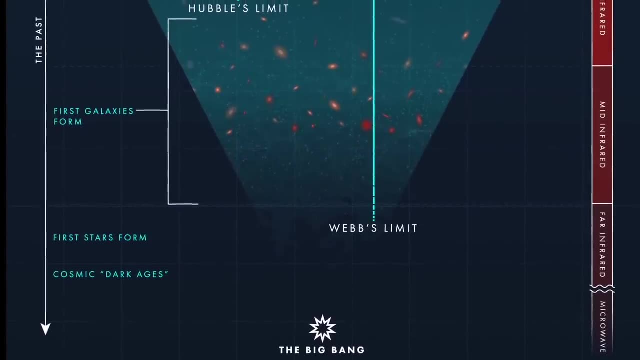 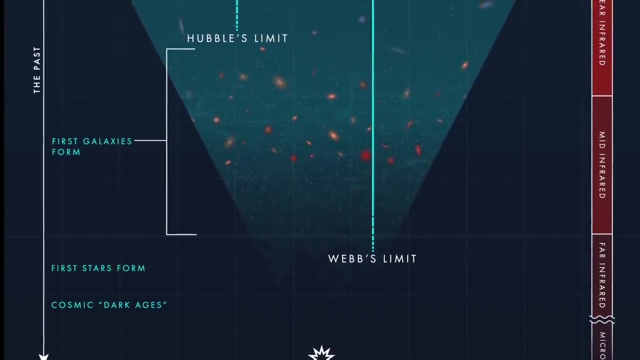 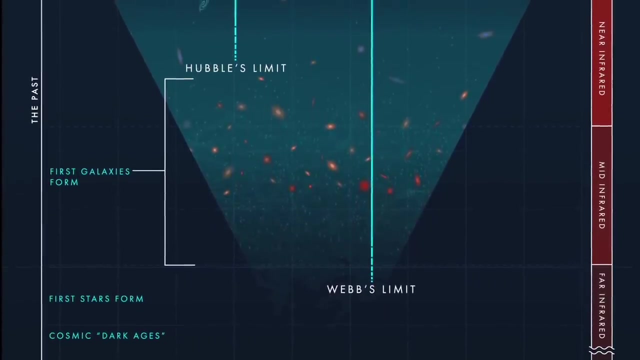 things that we are literally in the dark about. we have the dark ages- we don't know when- the first seconds of the universe and 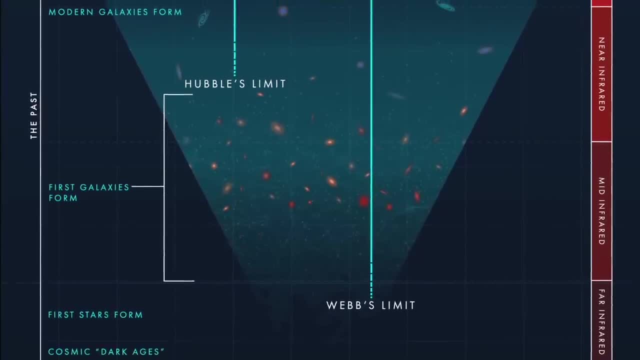 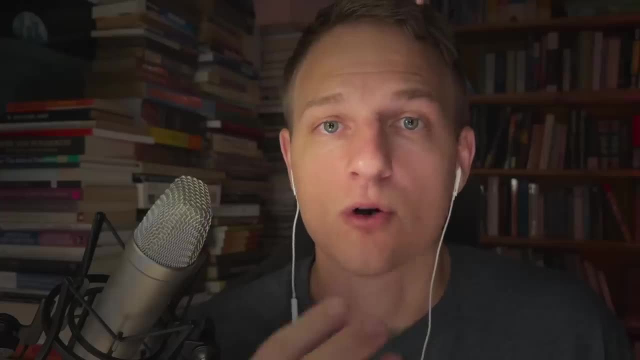 these were the seeds around which matter collapsed into and coalesced and became the gravitational wells sitting at the cores of the air corralled. 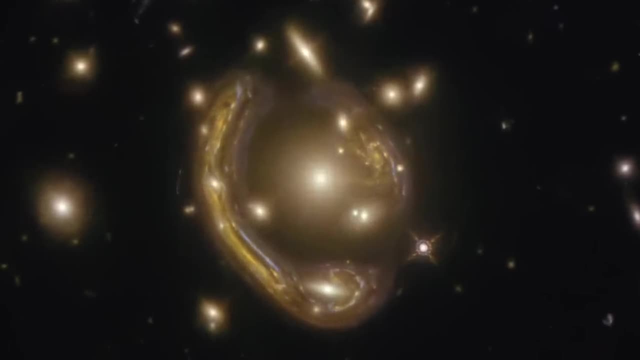 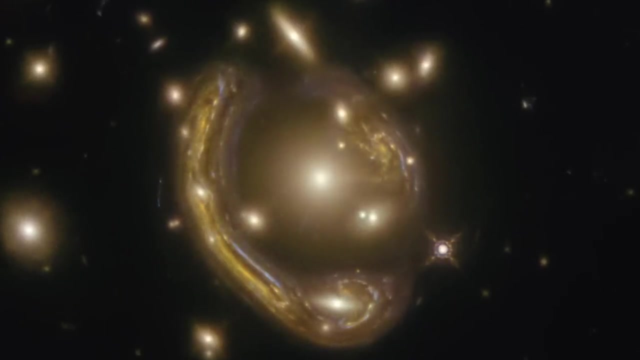 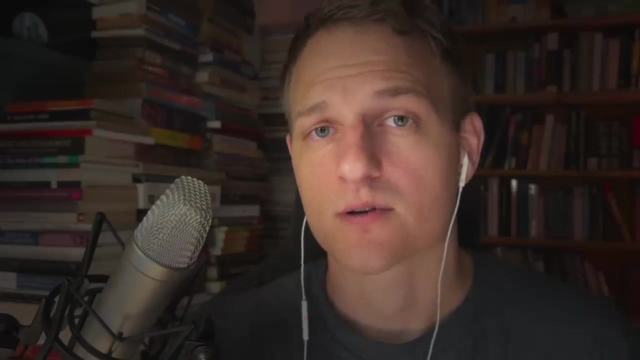 in these spheres of undetectable, non inert, non interactive matter. we don't know, finally, what dark energy is. we have no idea what this. 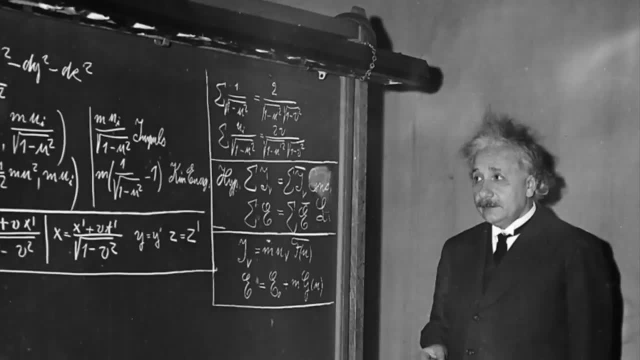 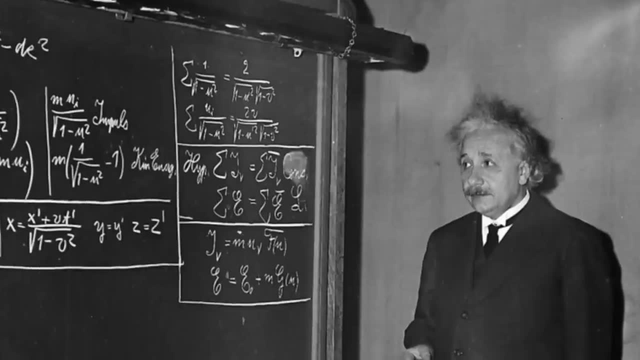 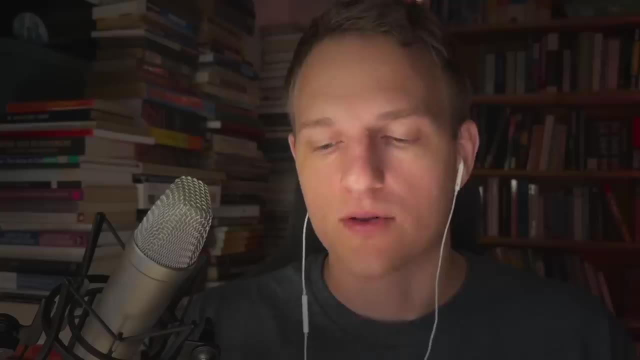 is, it seems to, in the early nineteen hundreds, when he came up with special and then, ten years later, general relativity and started applying. 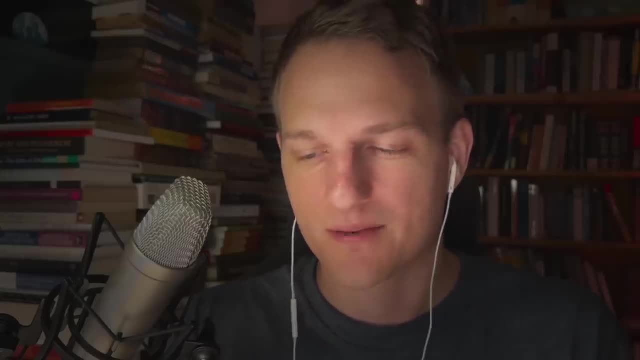 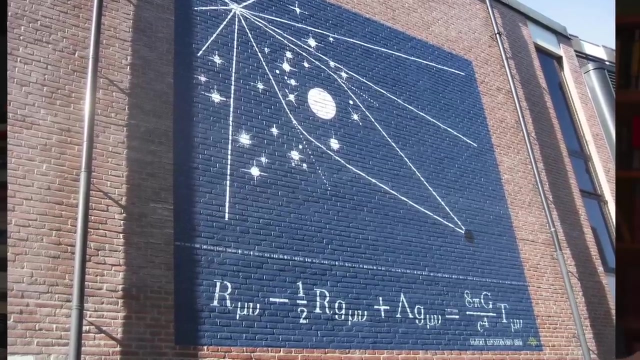 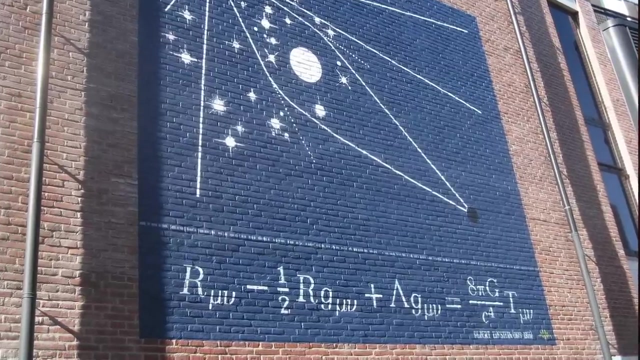 them to astrophysics and astronomy cosmology. even though this Einstein inserted into his equations called lambda, he used the variable the Greek letter lambda. 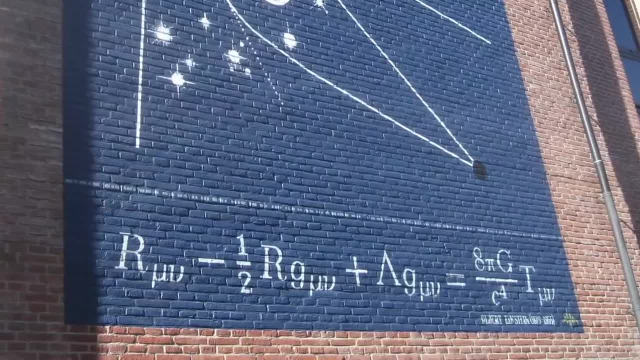 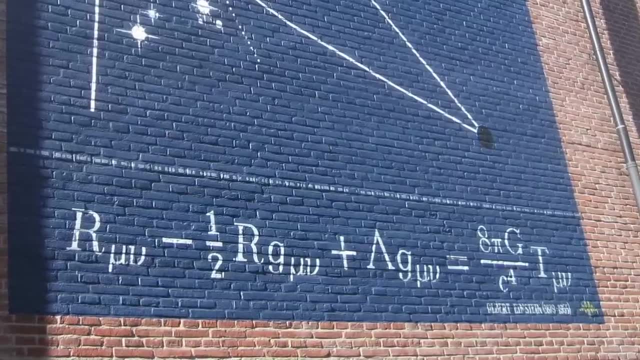 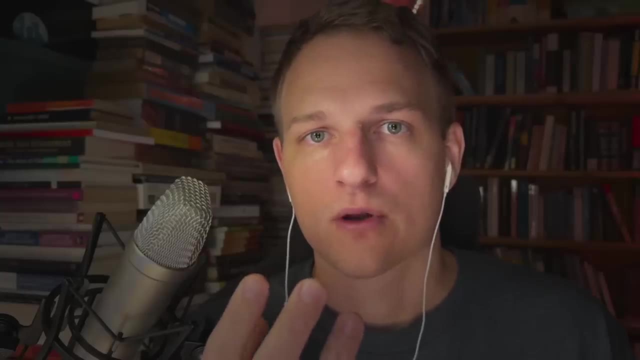 to offset the gravity of matter that bends space time. and he said in a almost anti gravity, pressure and outward force, propelling and counteracting. 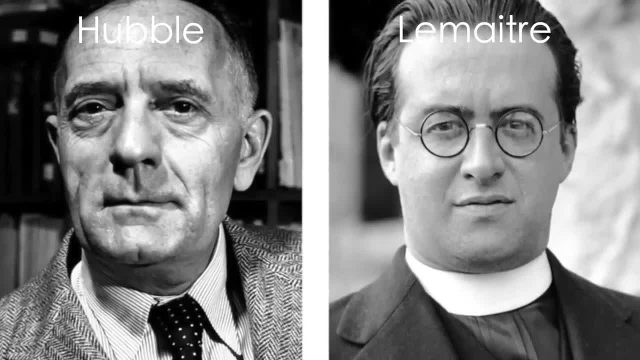 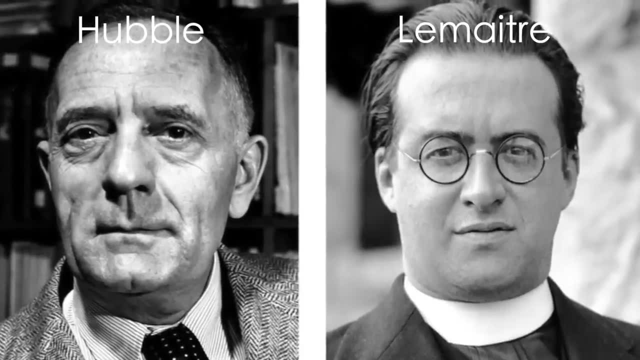 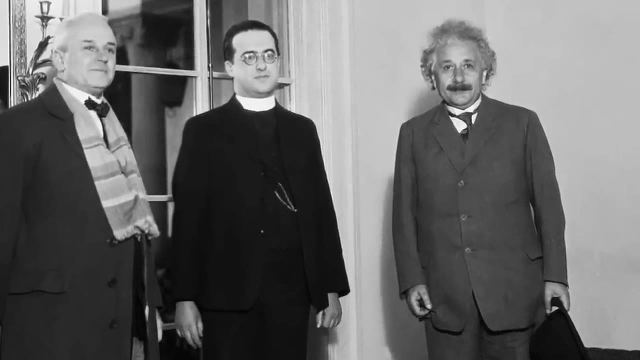 gravity. he then dropped it when he realized Hubble- Edwin Hubble- a few years later in La Matra, and expansion doesn't really tie into. 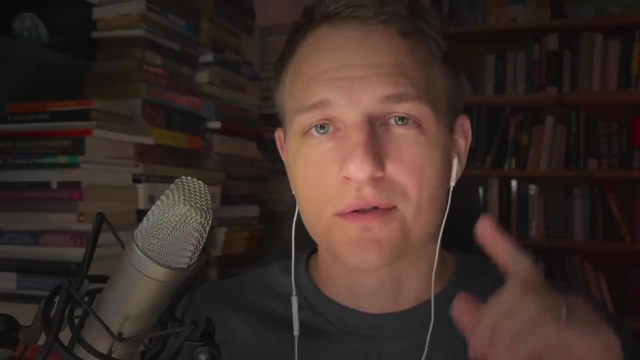 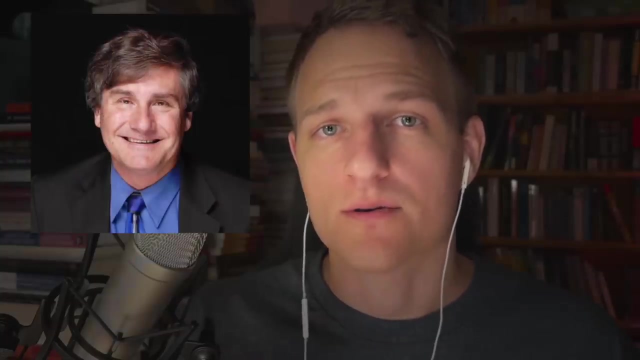 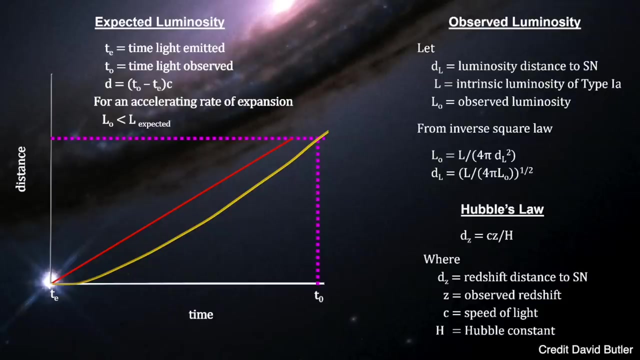 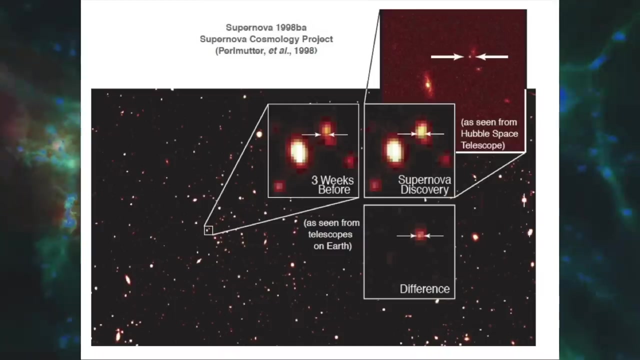 dark energy. so we dropped it. and then, a hundred years later or so- about maybe 70,, this guy, along with a team of distant 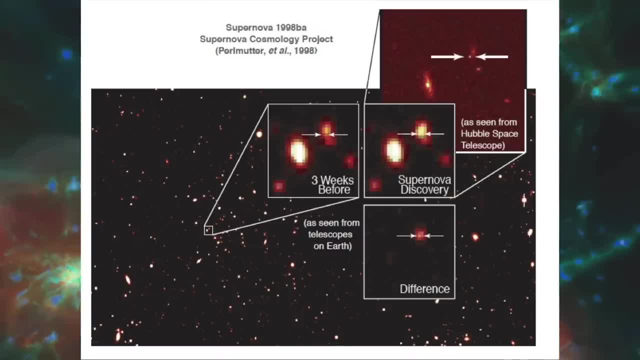 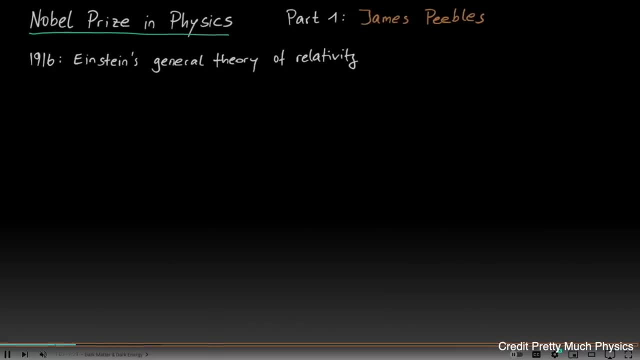 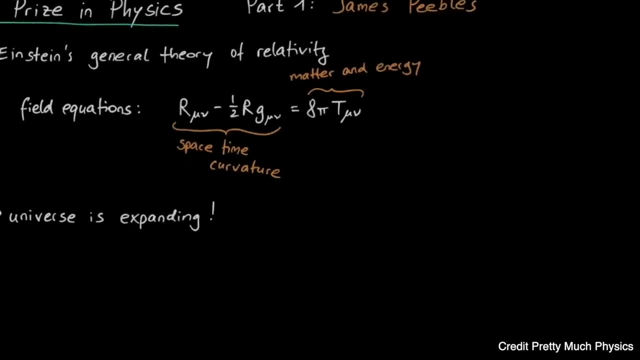 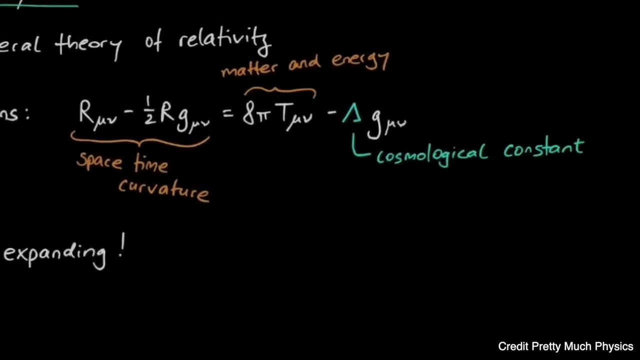 supernovae pointed to an expansion that was far faster than what the momentum from the early inflation of the universe would have led to this. 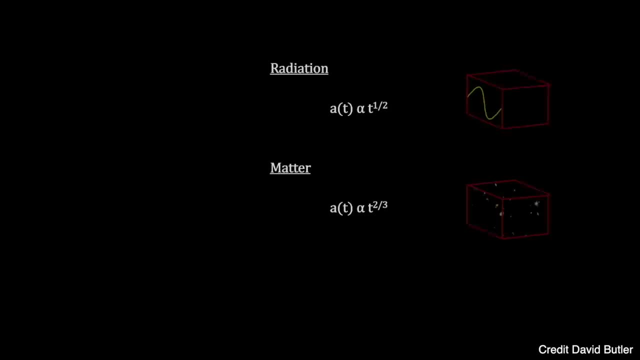 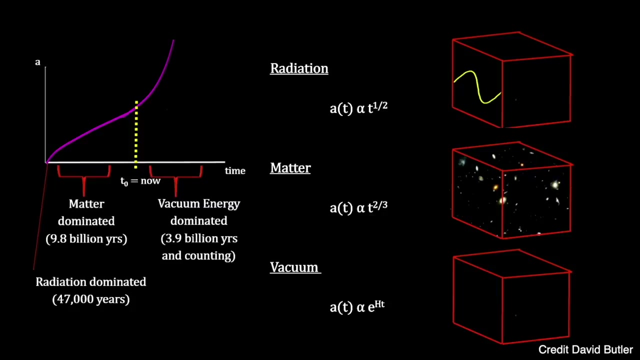 forced cosmologists to a vacuum energy that expands the metric of space itself, much like the inflaton particle that Filipenko on Lex Friedman's podcast. 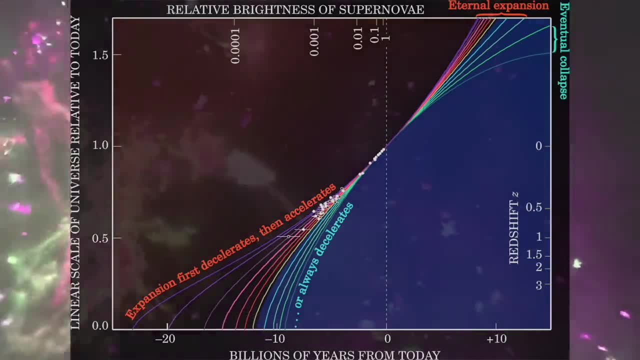 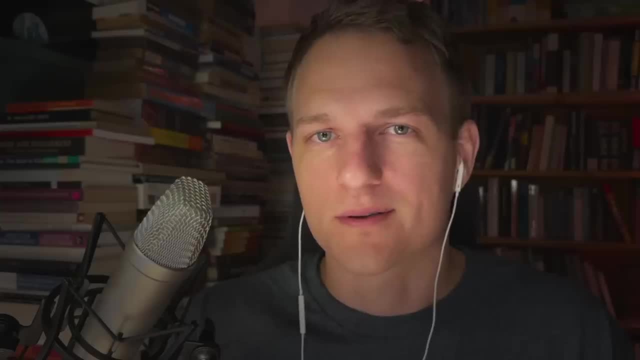 actually talked about, maybe dissipated into other particles there, so many things that we are very much ignorant about, and there's also, though, a lot. 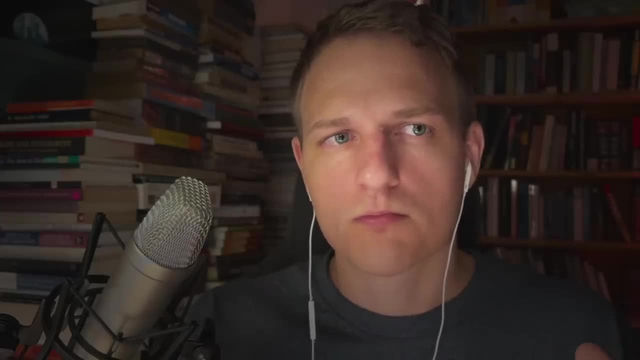 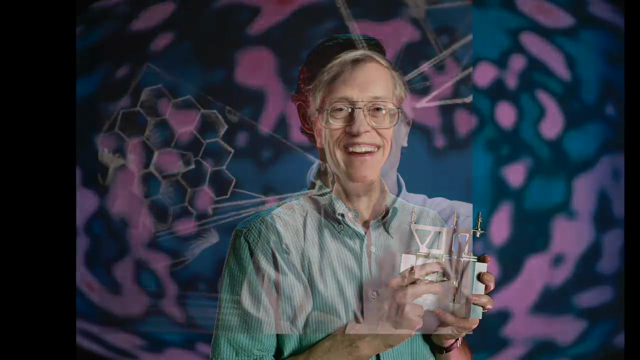 of breakthroughs that happened in the nineties in around the same time, as led by scientist John Mather, the Coby satellite in nineties. 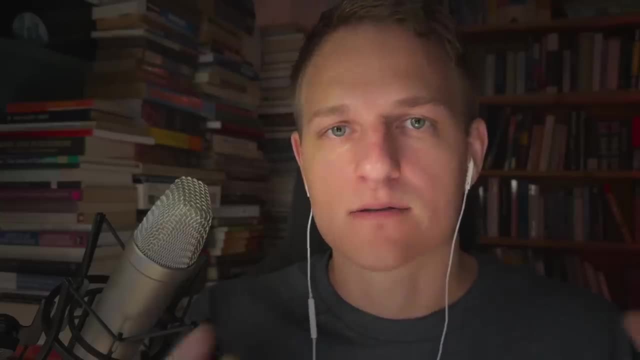 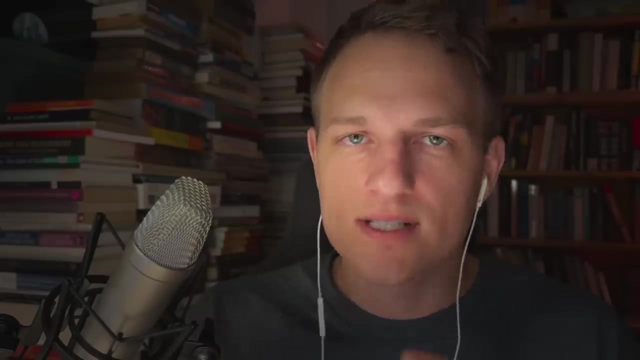 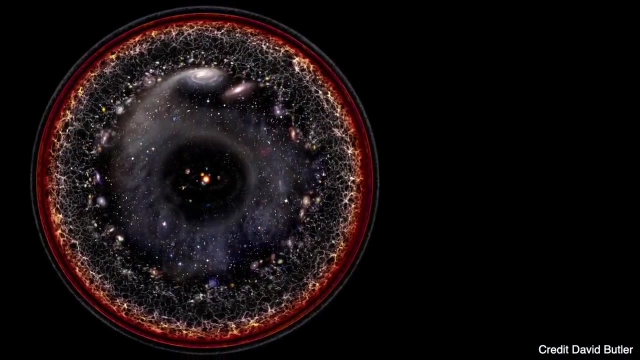 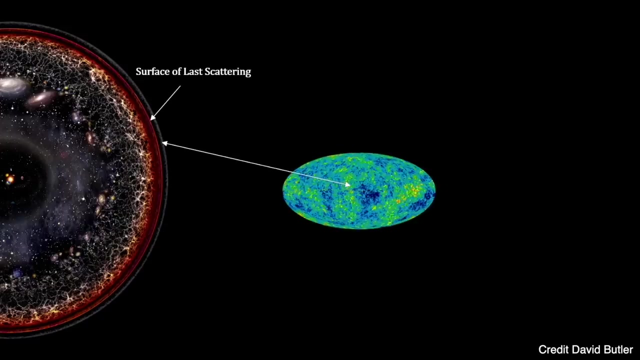 measured the cosmic background light that we just mentioned that was emitted from that early haze of white into longer microwave wavelengths. such good data from 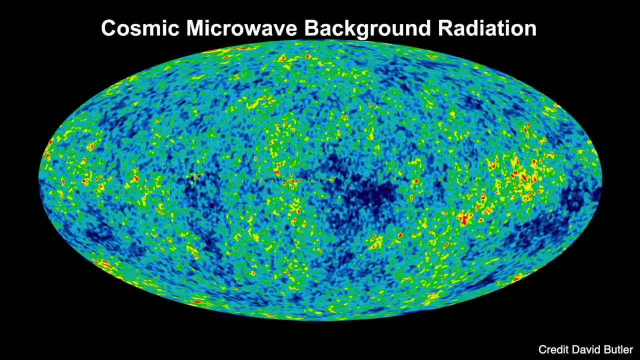 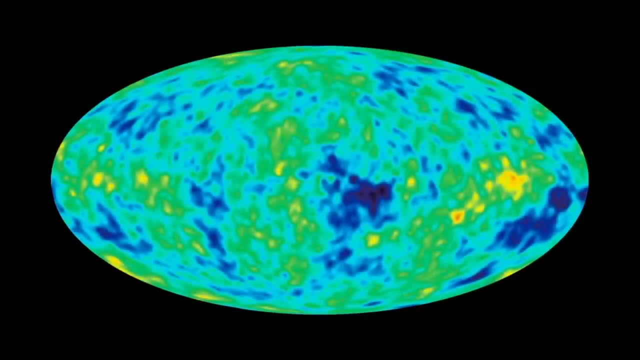 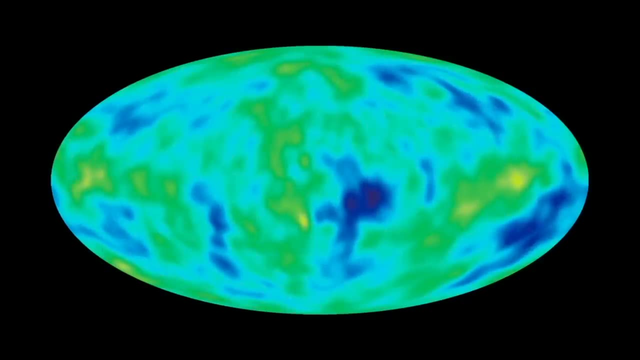 this Coby microwave detecting satellite actually helped resolve those large oscillations like this that we see. it's been refined and really measured. it helped. 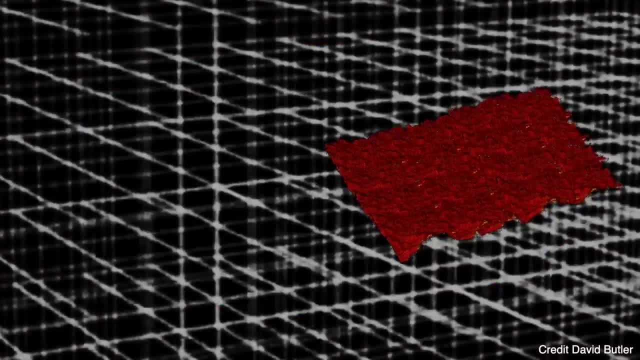 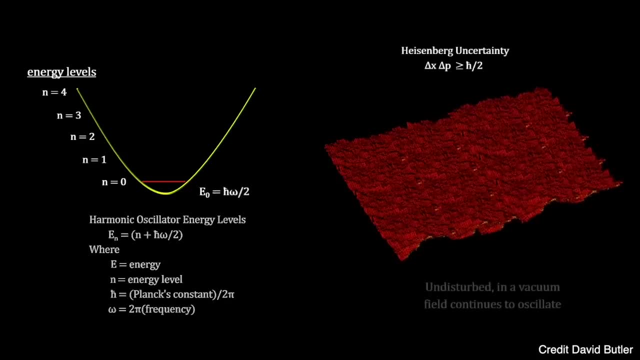 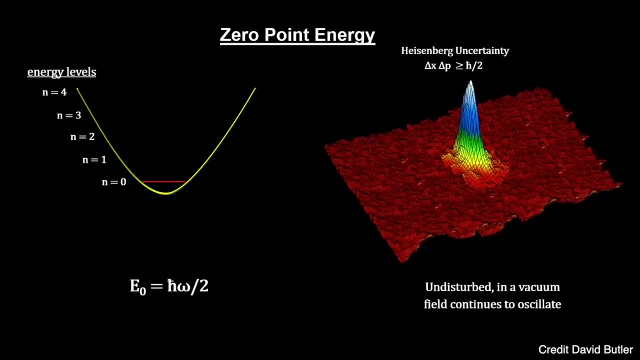 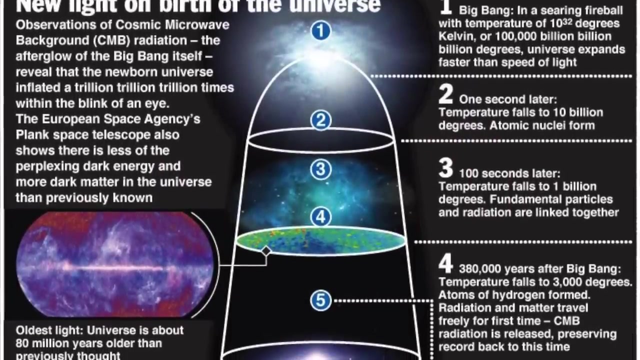 us see that these oscillations might have been these fluctuations that were seeded by the quantum field, fluctuations frozen into a structure on the largest. 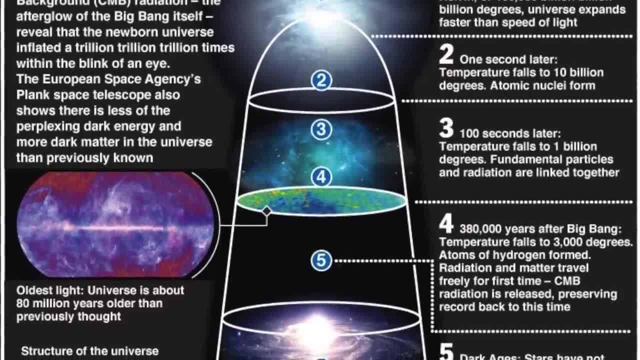 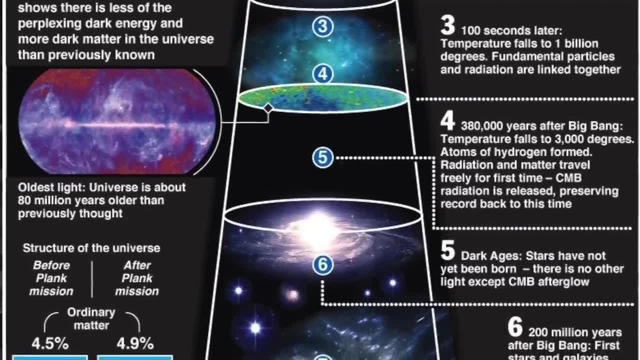 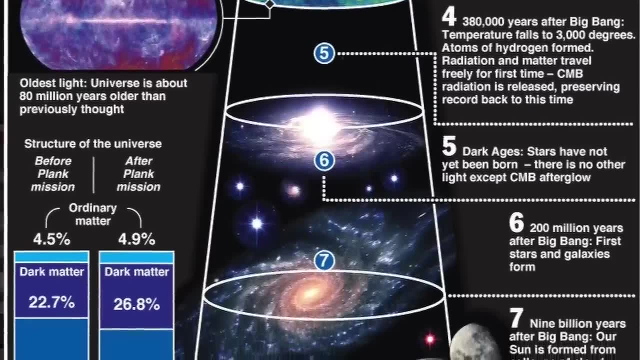 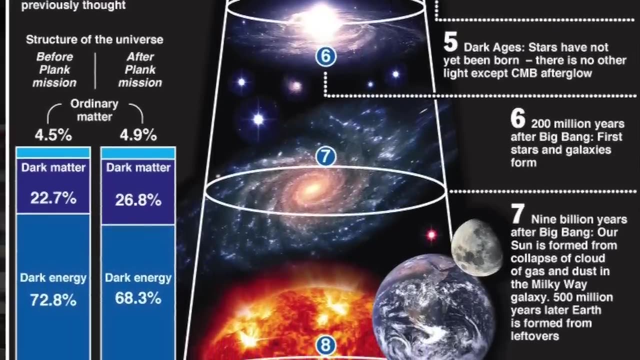 of scales over the next millions of years, cooled down from thousands to hundreds, to tens of degrees above absolute zero. so this ice cold field, 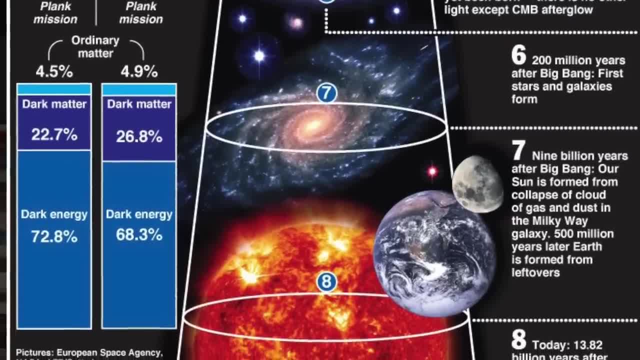 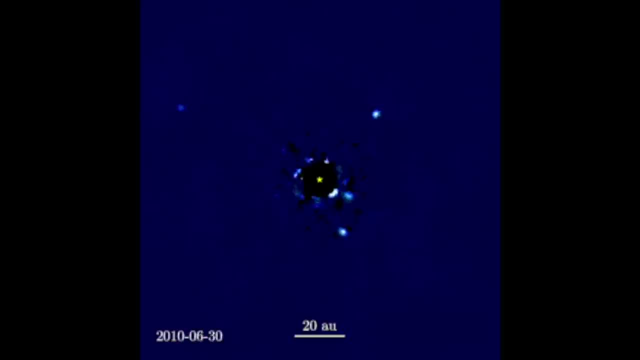 of hydrogen mostly drifted of the universe. also around the same time, in the nineties, scientists discovered the first exoplanets, the first planets orbiting. 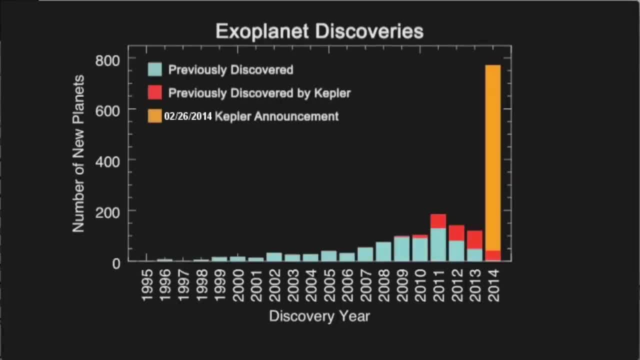 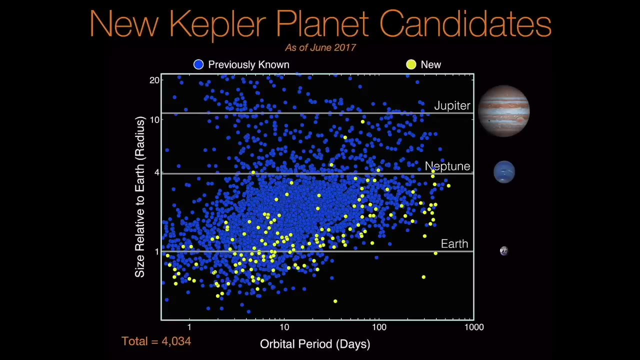 stars far outside our own solar system. these were. the technology was fixed on discovering more, and hundreds, and then eventually thousands of more were discovered. 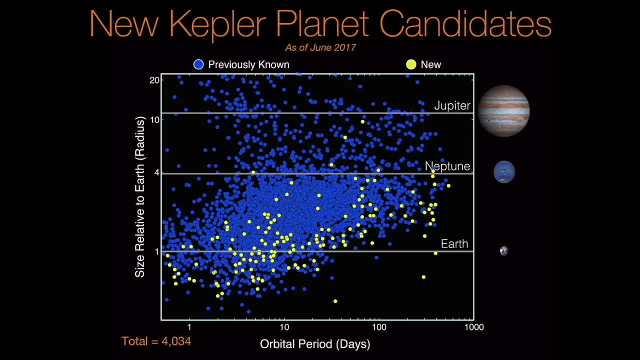 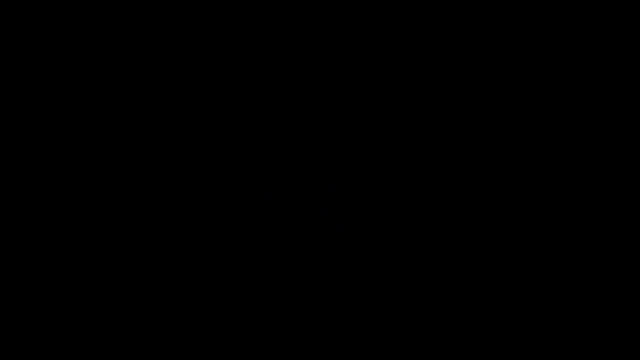 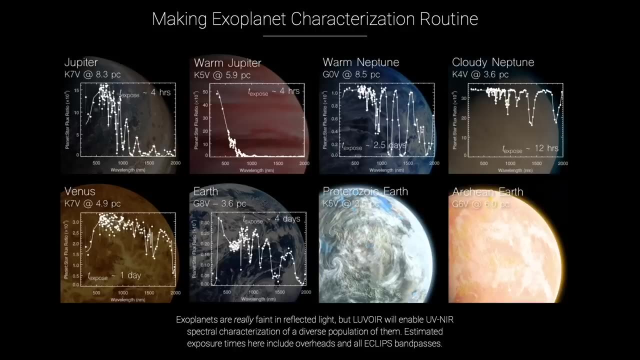 in the race to find alien life on planets began. it's actually now lots of them whose atmospheres we've been able to measure. show. 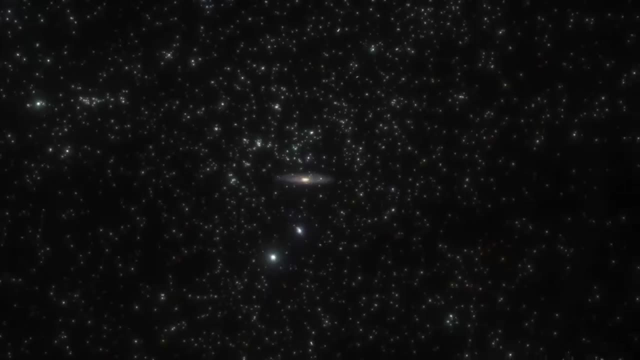 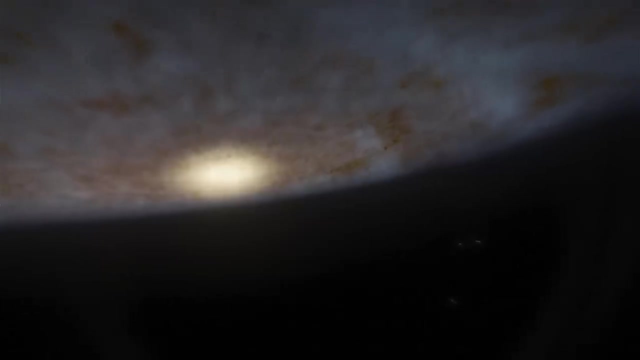 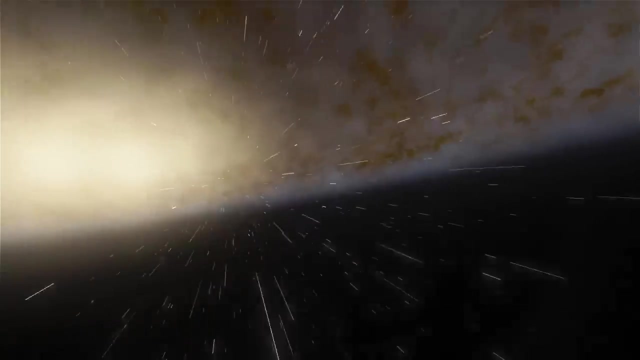 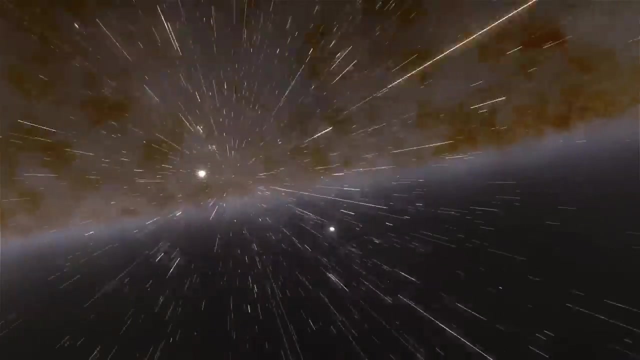 that show that they aren't very hospitable to life, but the math that might stop you in your son. and then one in five of 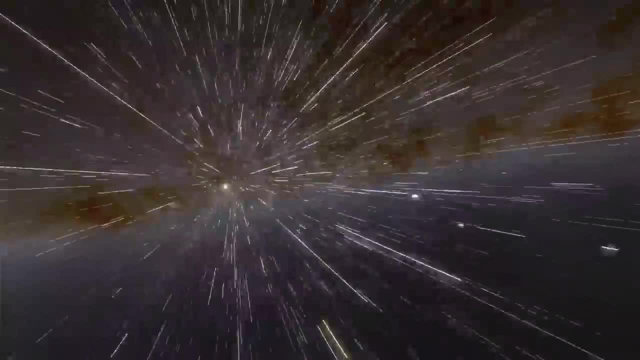 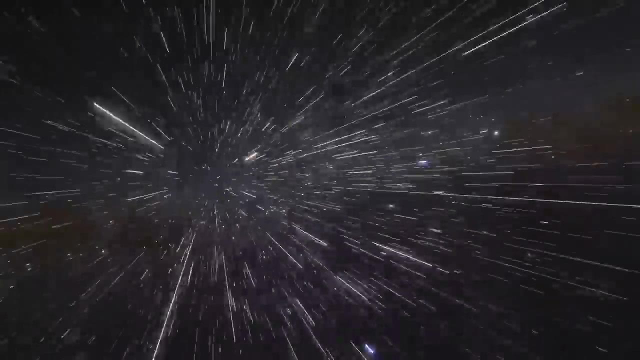 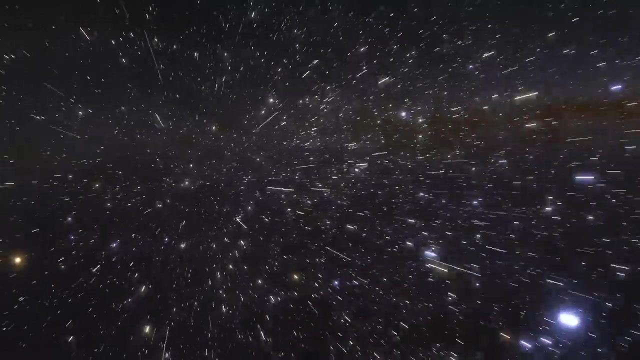 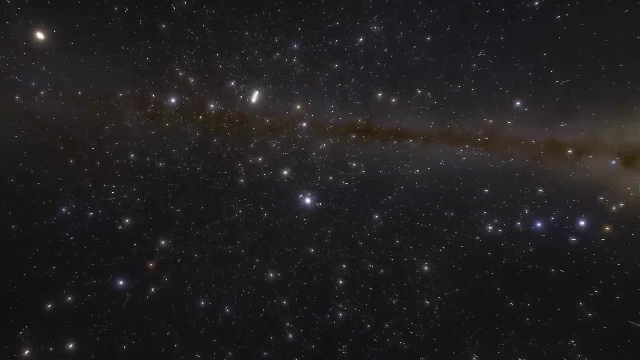 those have earth like planets around them. that means that about five to six billion planets like earth exist just in our underground. seeing the first. 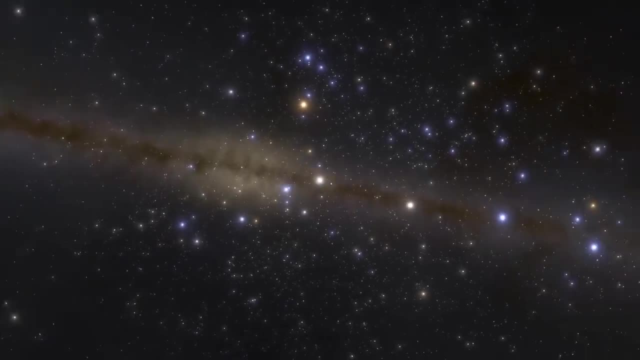 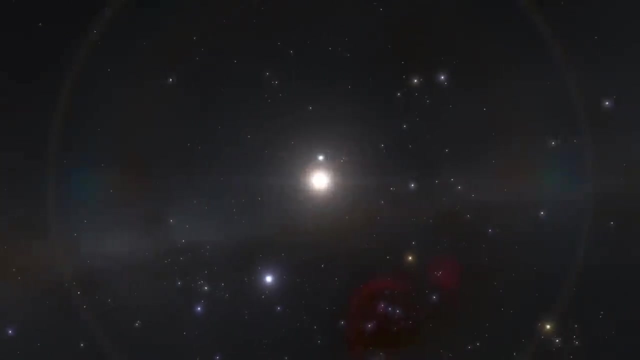 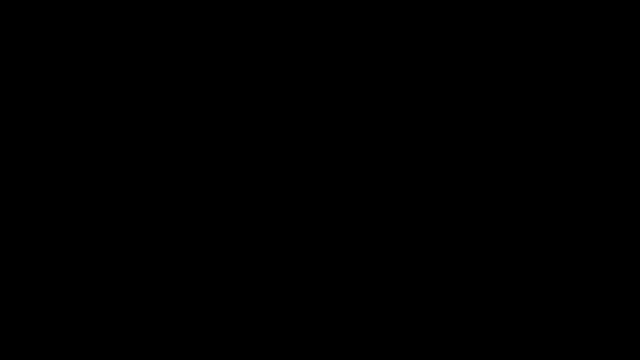 hydrogen fields that might have turned into the first stars, the first exoplanets, and the tantalizing evidence of the sheer volume of planets that 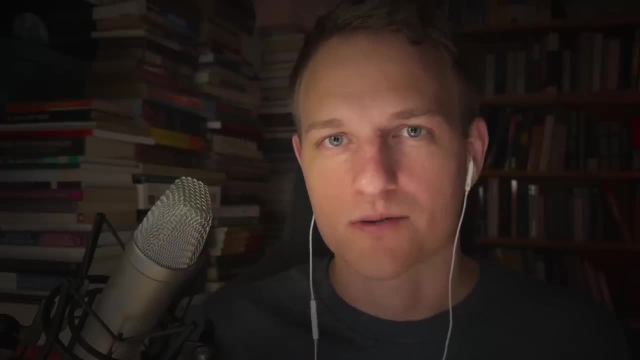 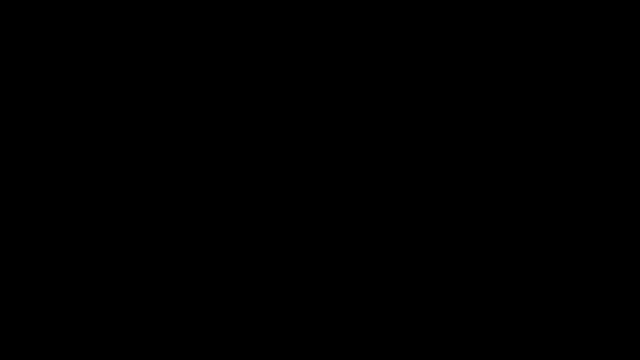 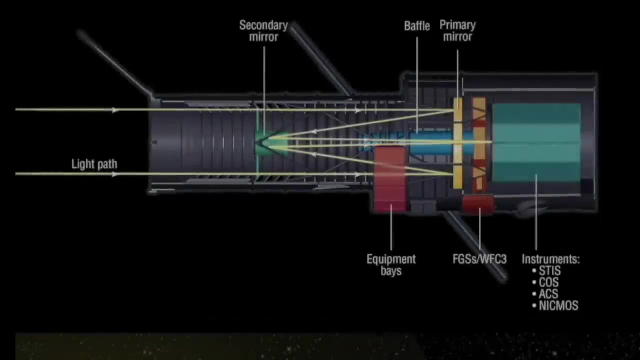 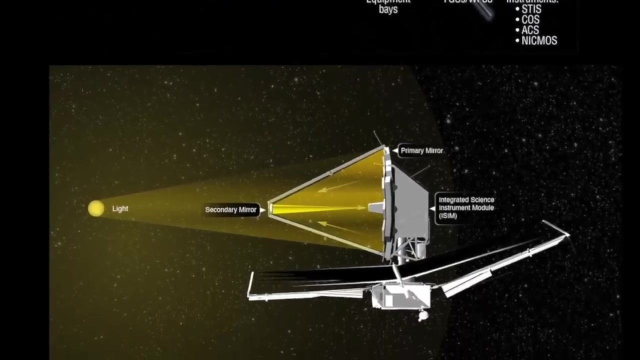 are these huge domains of ignorance about the cosmos that we live in that the james web space telescope was born. so much of telescopes. 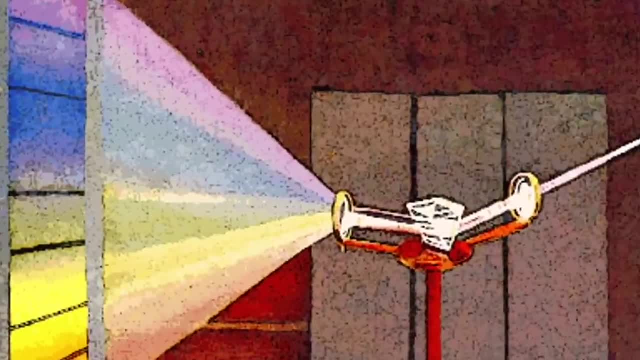 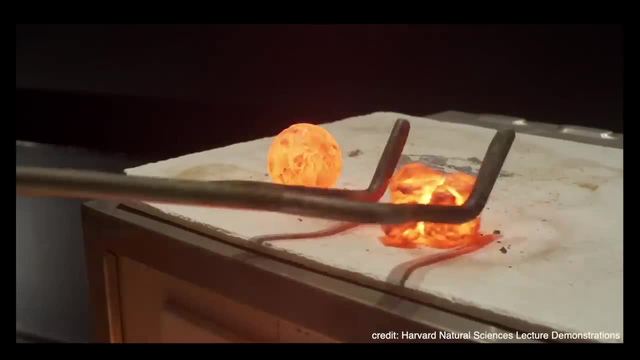 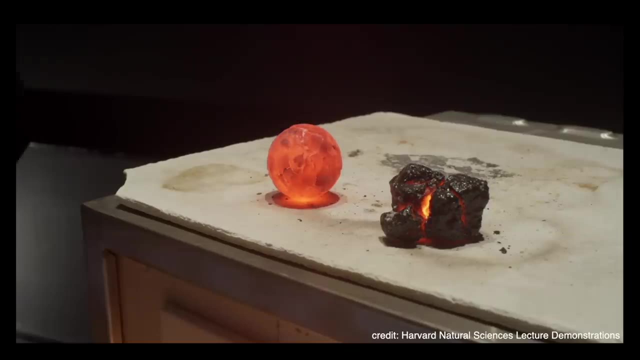 involve the simple gathering of, and of course we apply physical experiments on done here on earth and now in satellites in space, and the laws 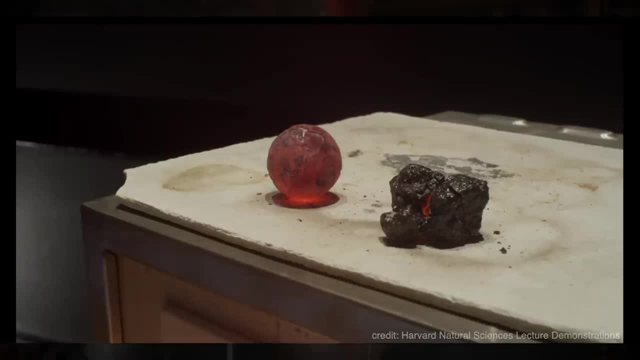 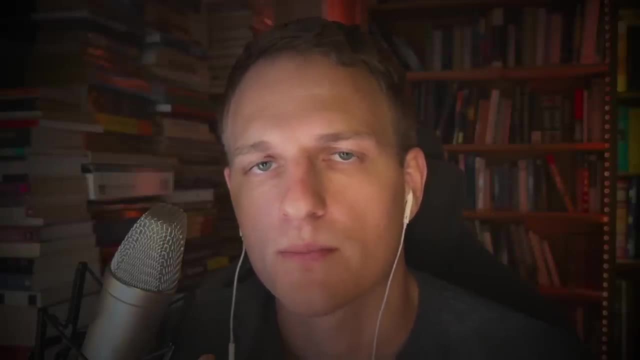 of nature that we determined from that to the atoms basic structure are nuclei. they're nuclei with protons, neutrons, call them nucleons together and 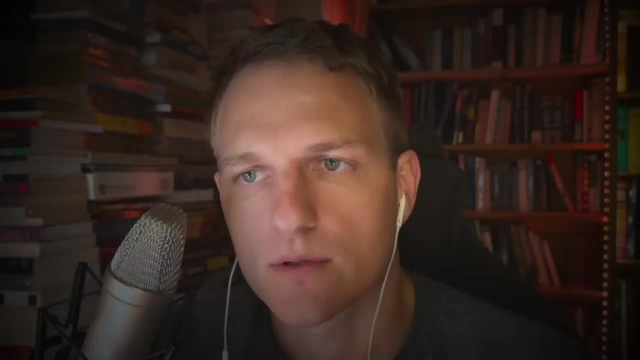 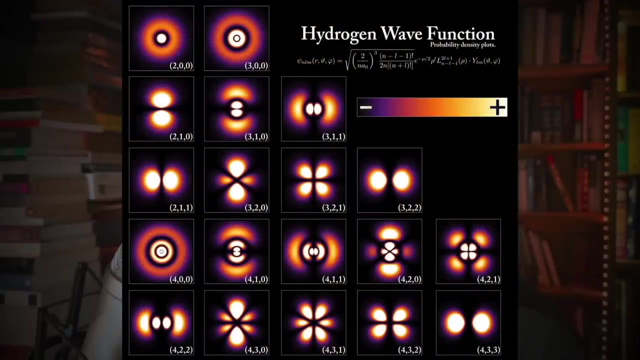 they're orbited by these really tiny particles with high energies called electrons and neutrons, but around any given in any given element it's defined. 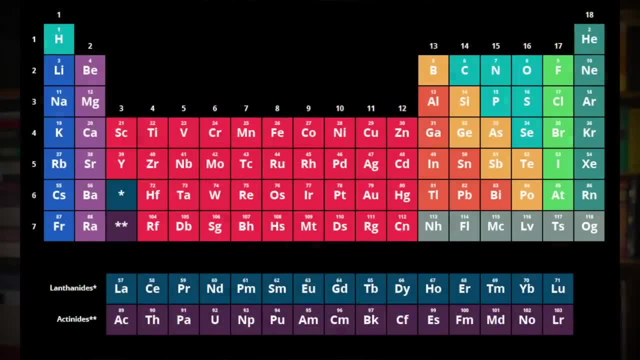 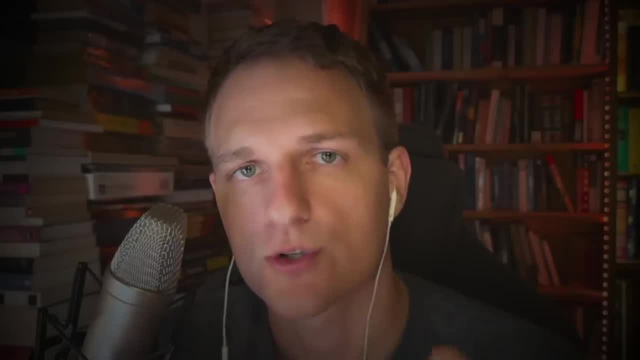 by how many protons it has, and usually with protons you have a roughly similar number of neutrons in a feedback loop of sorts. 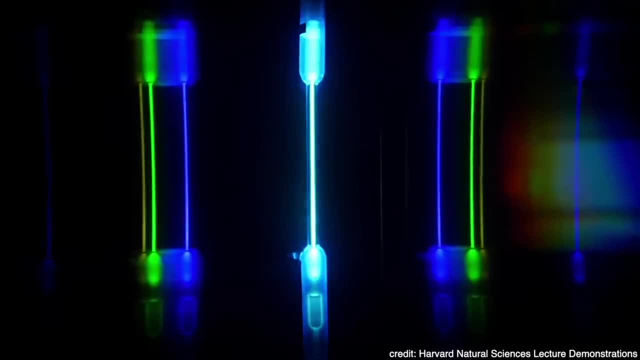 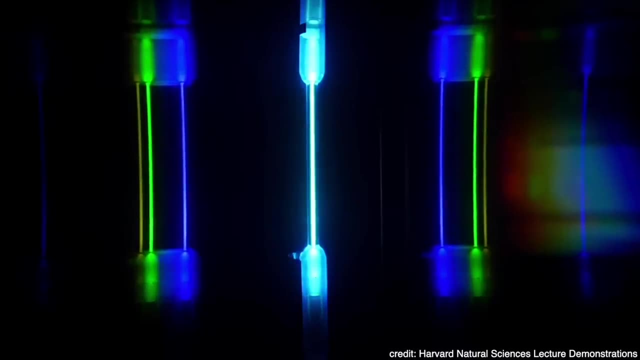 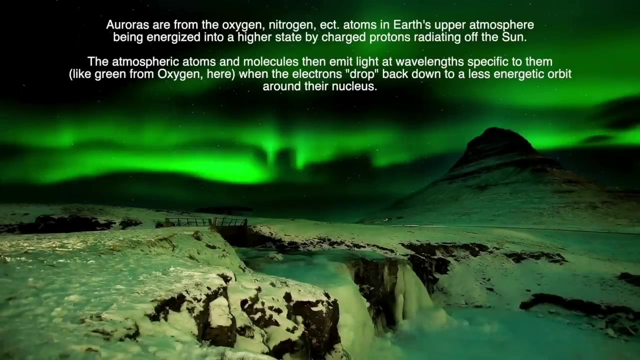 with each other, such that the electrons energy, in order to change up or down through absorbing different wavelengths well, can only absorb and be able. 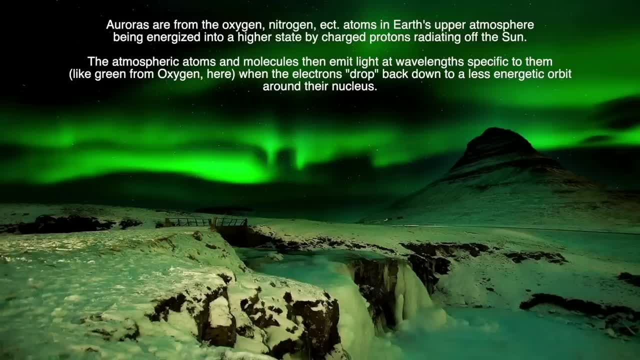 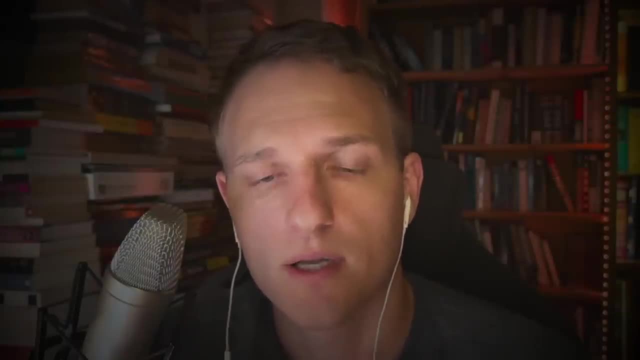 to. they come from the fact that, as you have a different nucleic configuration, different configuration from different amounts of protons, given different nucleus, you 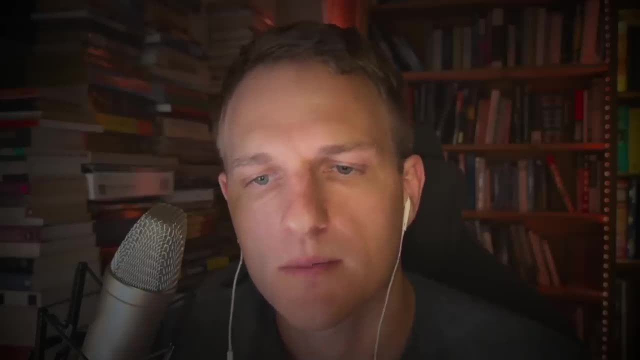 know, oxygen too, and of course that makes it bigger, creates a much stronger positive charge that the electrons have to interact with in a loop. 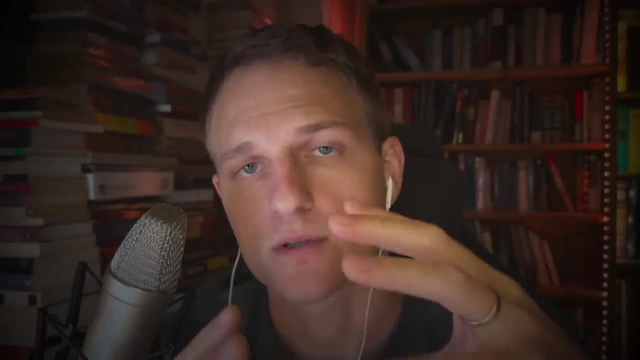 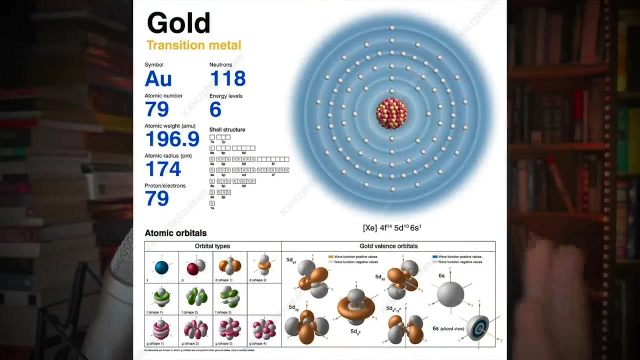 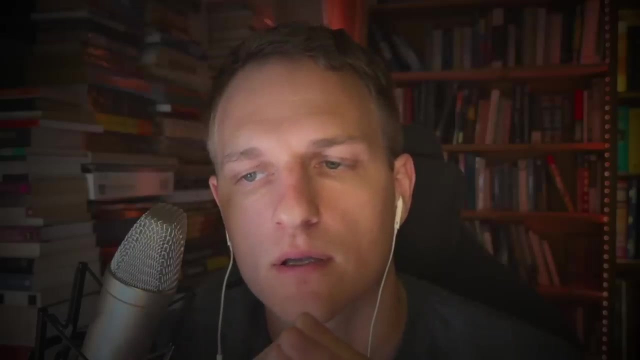 now, and so, therefore, for us, with all its protons, then the tiny little single proton hydrogen nucleus, the hydrogen nucleus is well, it's important. 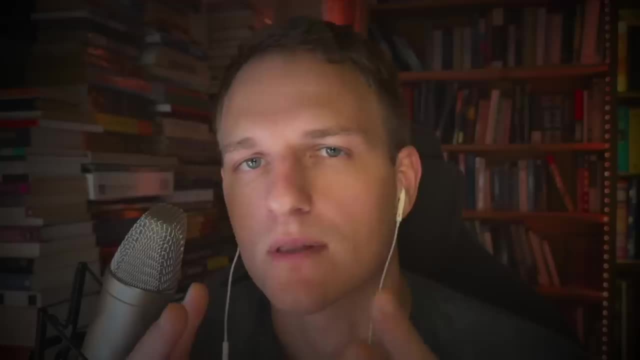 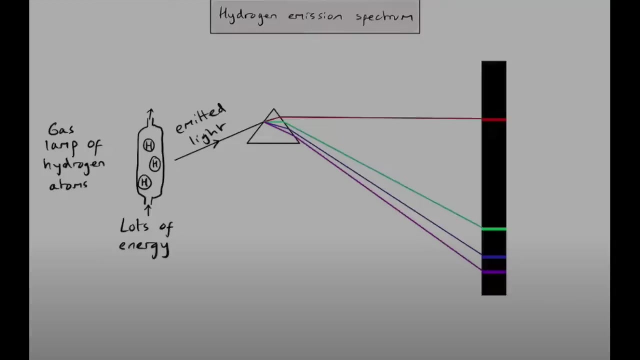 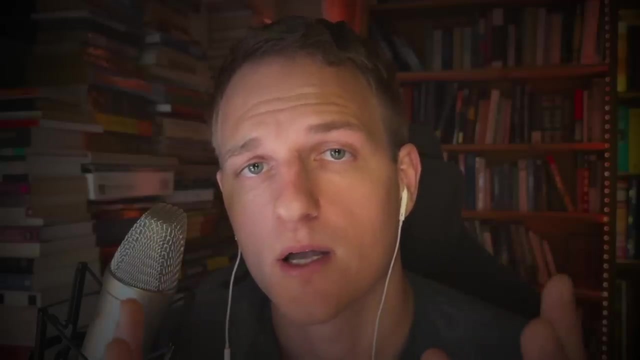 for cosmology and astronomy, but I don't think I have a very specific characteristic set of spectral lines and because most of the early universe 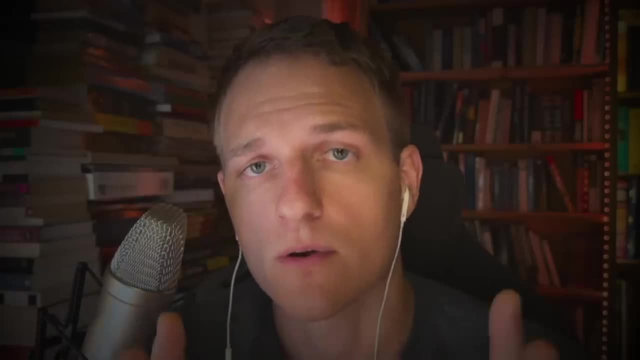 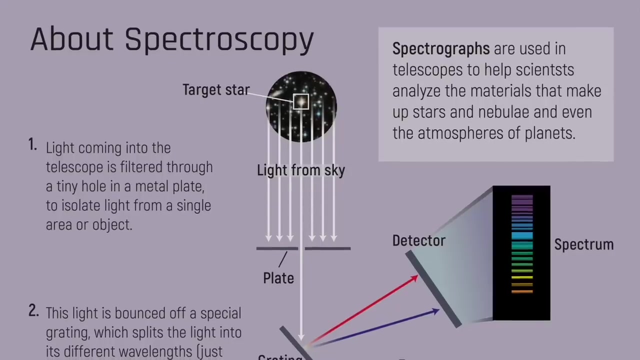 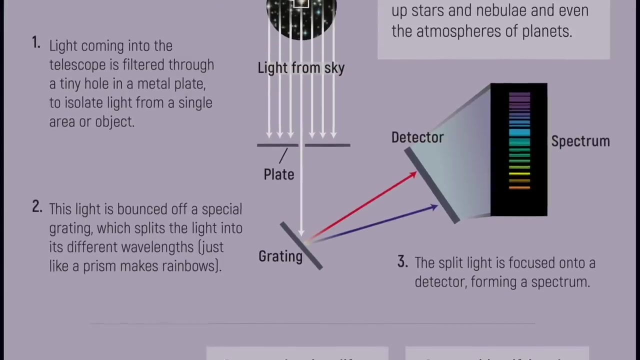 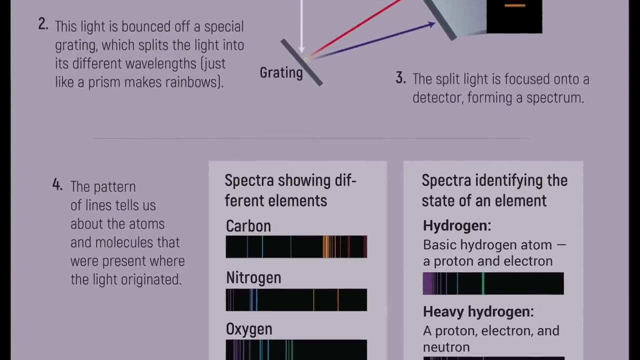 was hydrogen, because, other than some a little bit of helium and lithium, hydrogen spectral series of lines looks like and they want to know that. 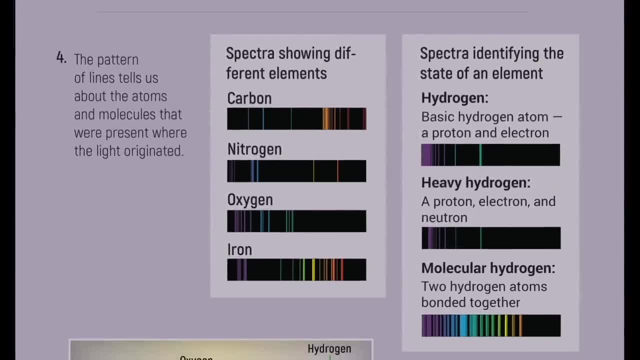 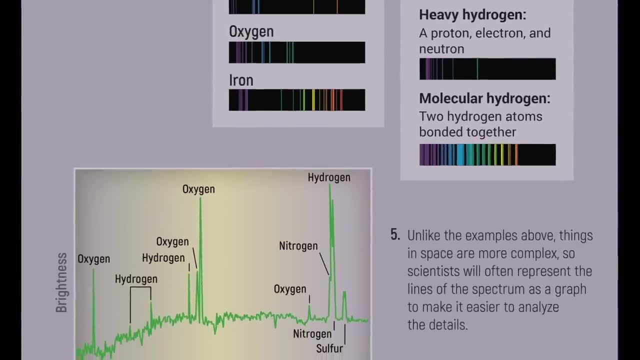 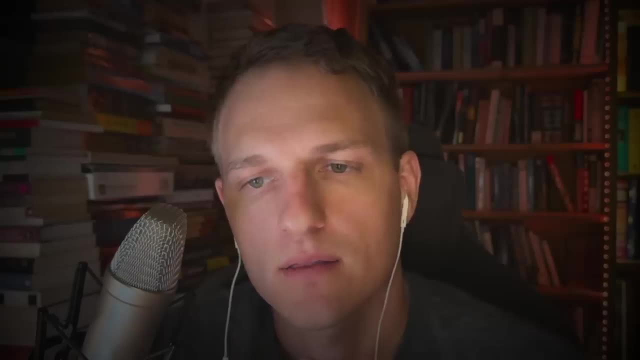 because they can look for that in the light from the distance by peeking through the light. they want to analyze properties of hydrogen and. 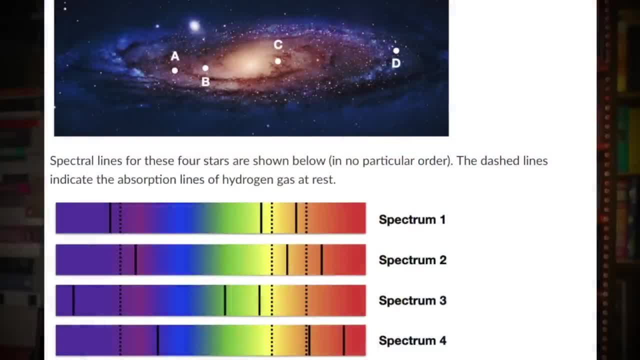 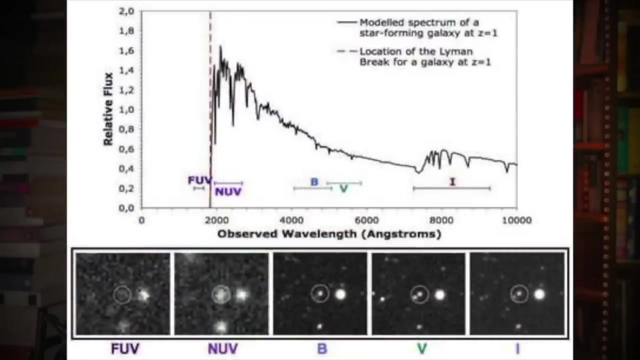 turns out that there's very specific properties of hydrogen lines that are able to tell us how far away for time, and other features like 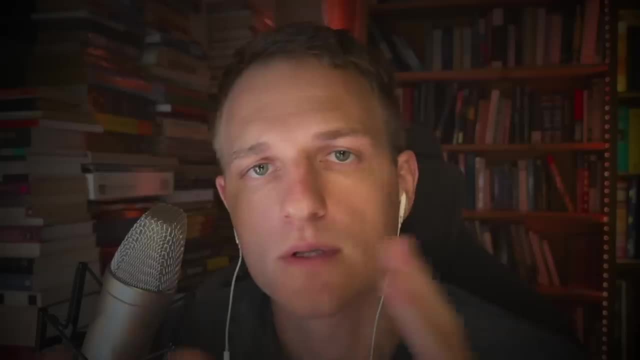 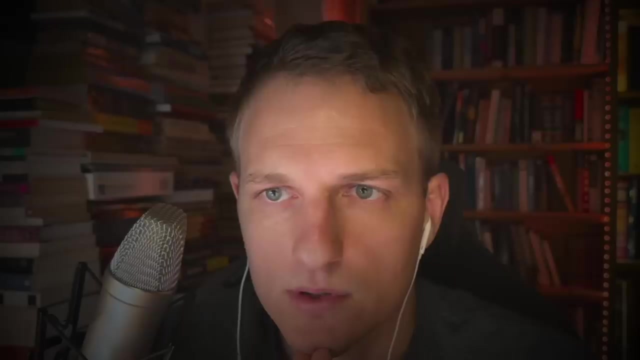 the abundances of hydrogen in a given galaxy. that's being observed, and so the structure of the atom and how it interacts with light. the 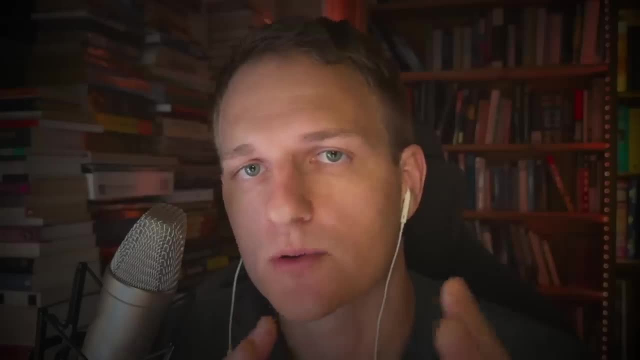 theory of cosmology and the universe we live in is built upon the easiest way i found to describe atoms and how they interact with. 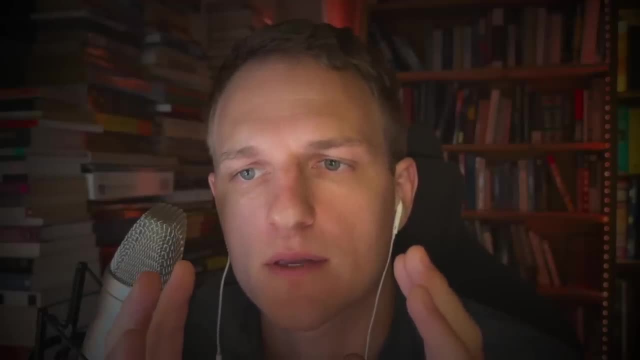 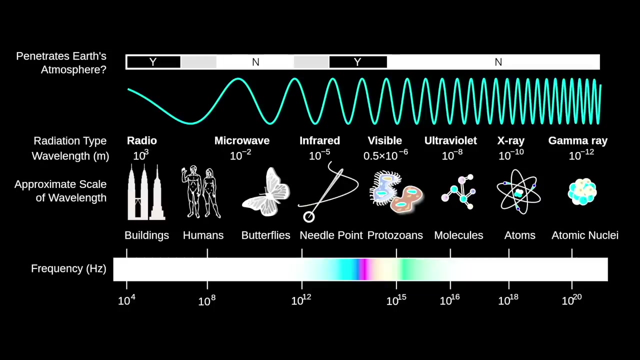 light and emit at the lowest end. let's think of, let's think of how light impacts matter if we shine light on it. we have. 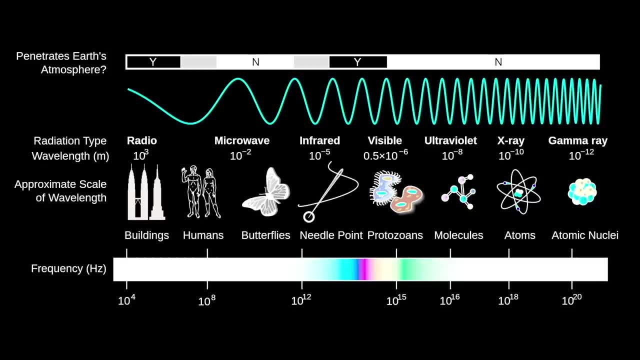 different types of light right at the end and blue being the shortest. then, as we get even higher frequencies, we go into the uv and 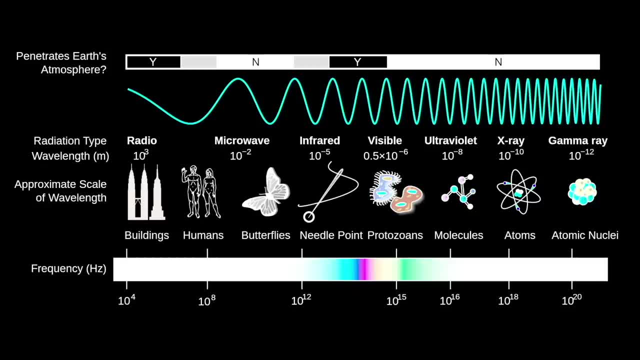 at that point uv bleeds into the x-rays and gamma through you. it ionizes the atoms in your body and small doses like machines. 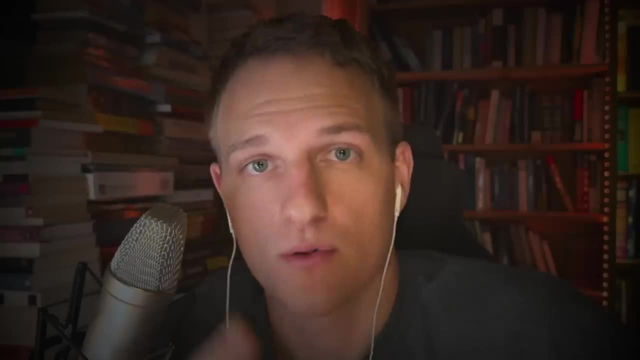 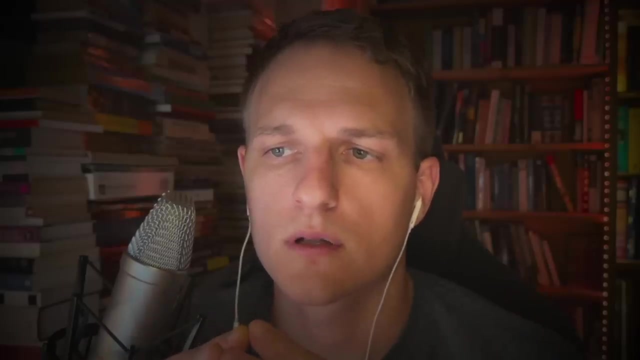 use. as far as we know now, for with 100, years of observation, it doesn't work in the way I found to describe light and 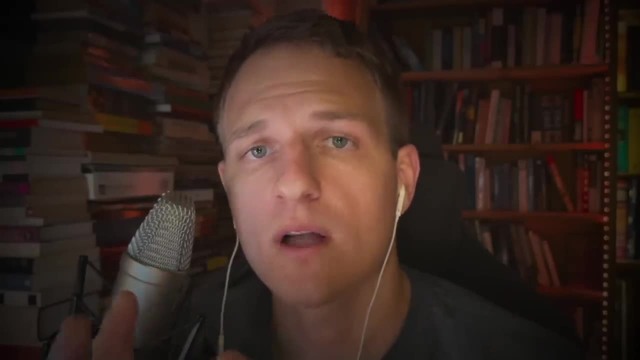 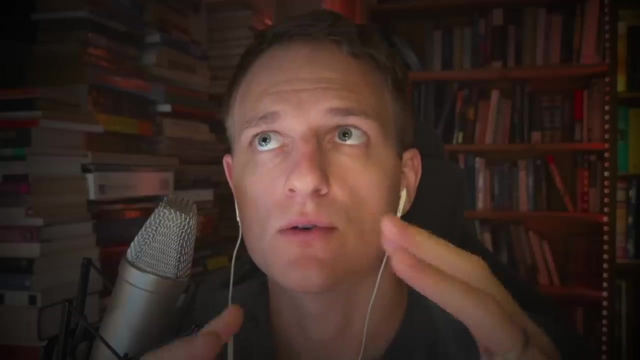 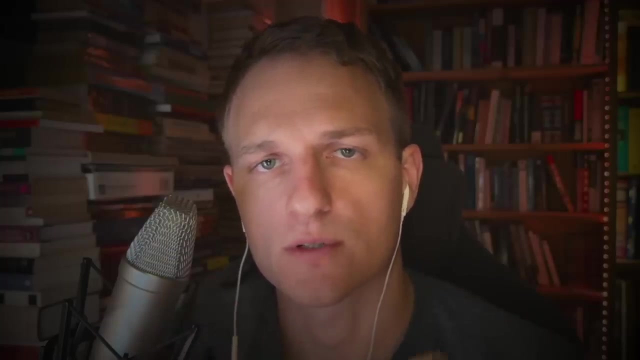 to understand it, conceptualize it's the way it's broken up, is actually to break it into regions of energy electron with a negative sometimes. 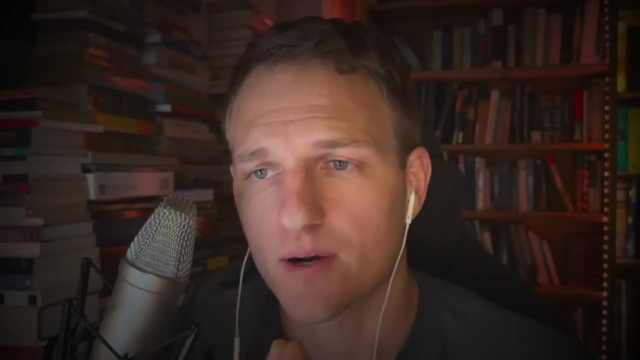 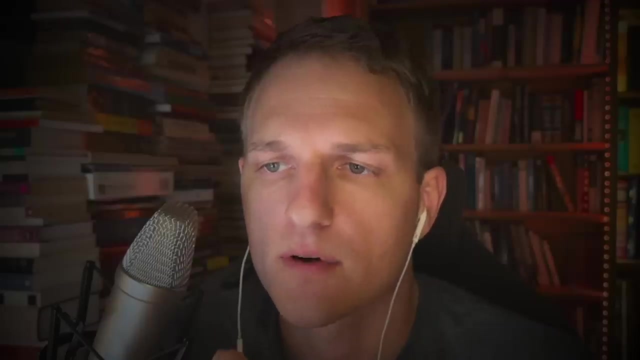 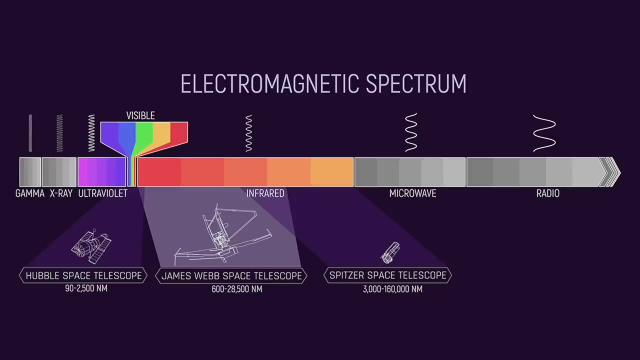 or many times. it's multiple protons in the nucleus, multiple electrons surrounding it at different energy levels, and we have groups of atoms of light. 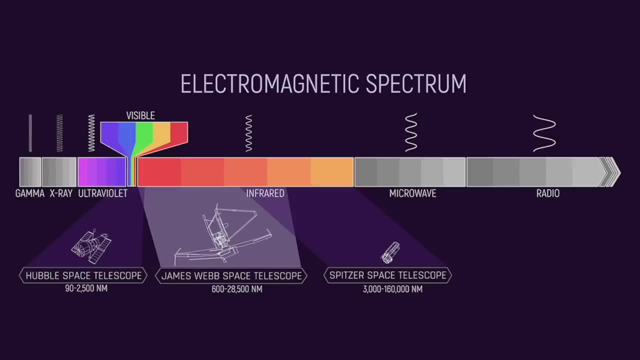 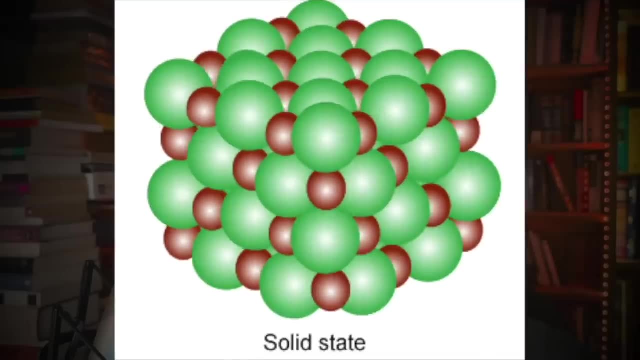 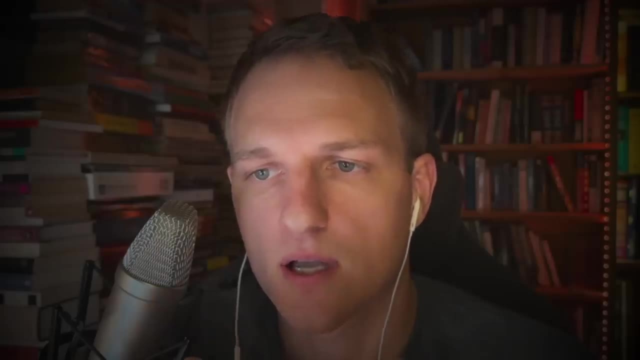 that can jiggle around and any time a light, any time an atom is above zero degrees, absolute zero, it has some sort of intrinsic. 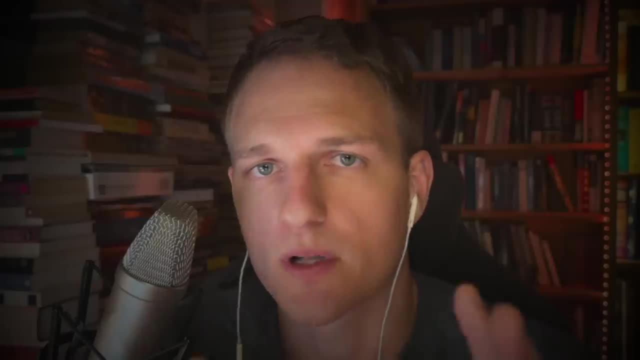 vibration. some sort of all atoms will have some sort of ambient energy and vibration movement to them that will cause them to spontaneously emit protons. 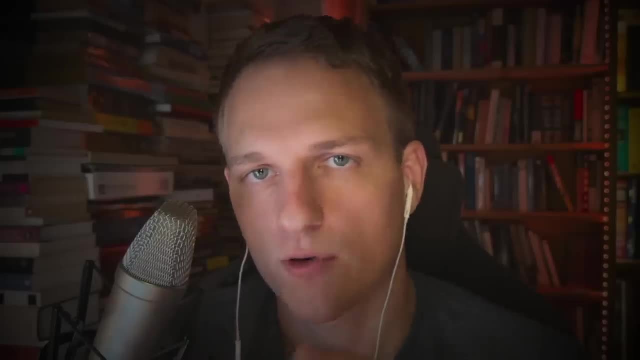 or photons, and the hotter you get more and more high energy photons, low energy, radio and microwave photons for cold gas and space, and then 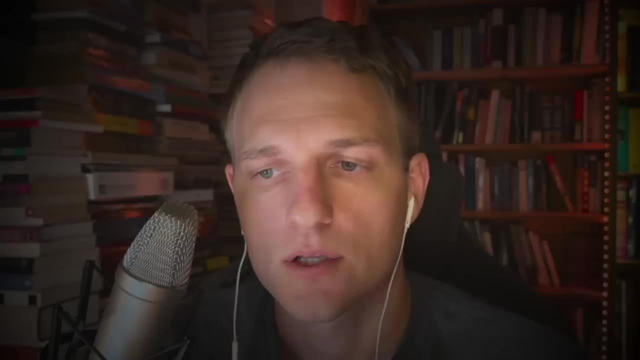 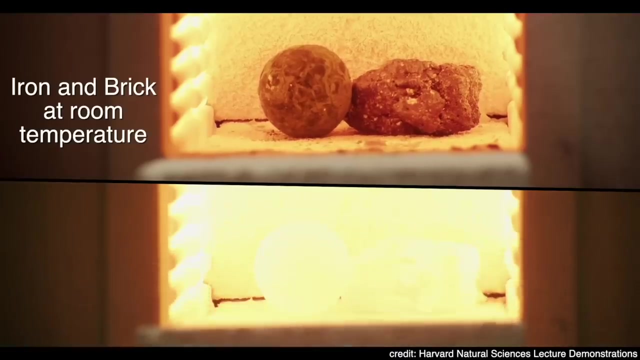 as you go through our atmosphere and get hotter towards the photons that the atoms on earth are emitting, cause they're starting to really get. 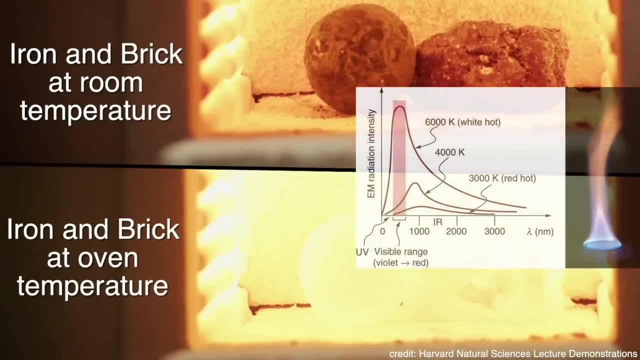 a lot more ambient temperature here and, of course, as you go to hundreds, that'll almost get to the point where light visible, light being. 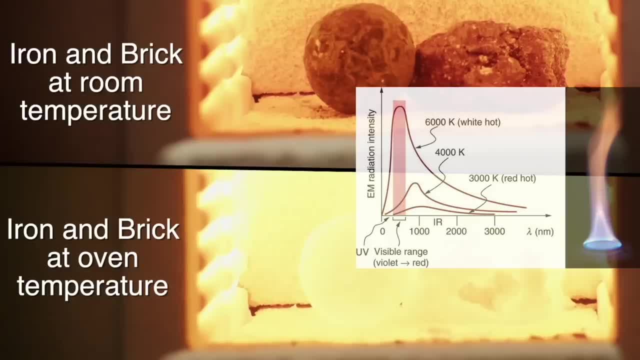 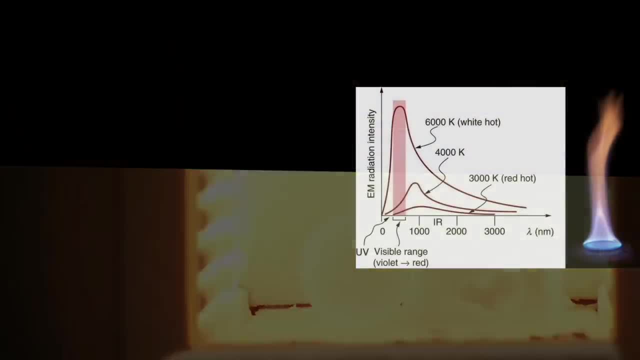 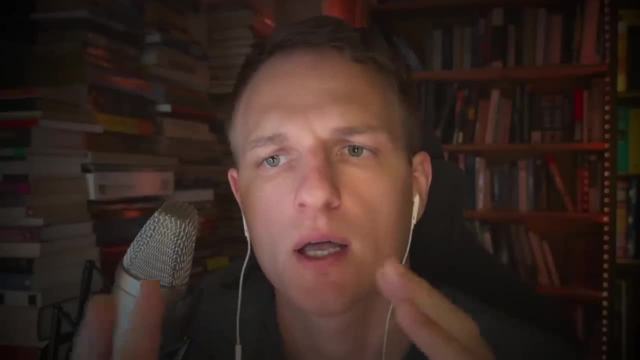 much more energetic than infrared and way more energetic than microwaving radio waves is emitted, and so the best large scale oscillations within a 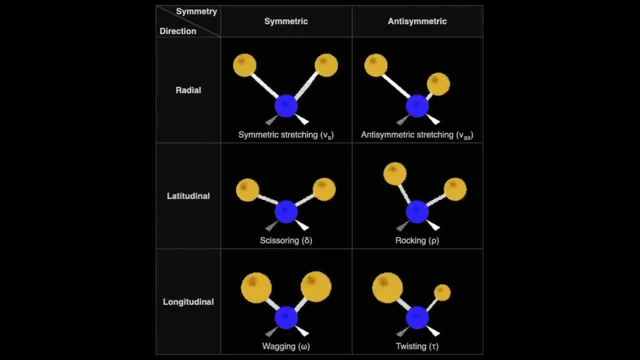 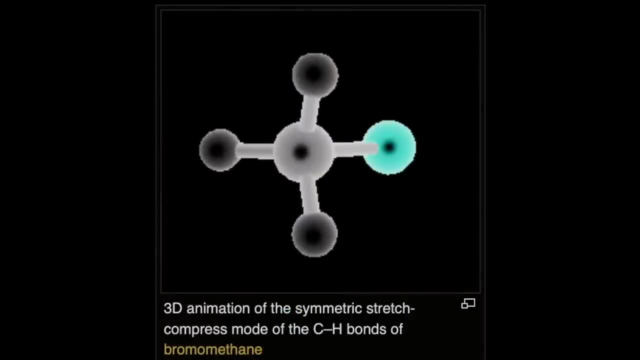 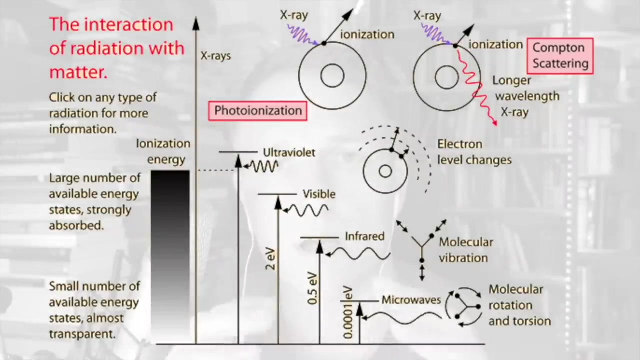 structure that's going to create a lower frequency than the higher frequency vibrations of the individual atoms, those and in molecules in particular, and not 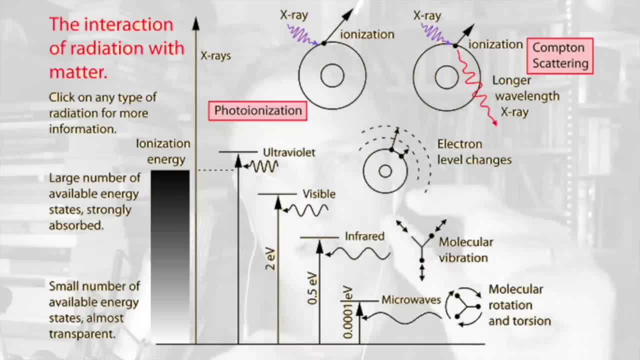 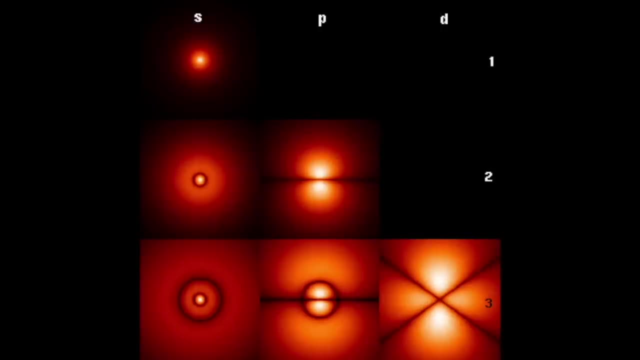 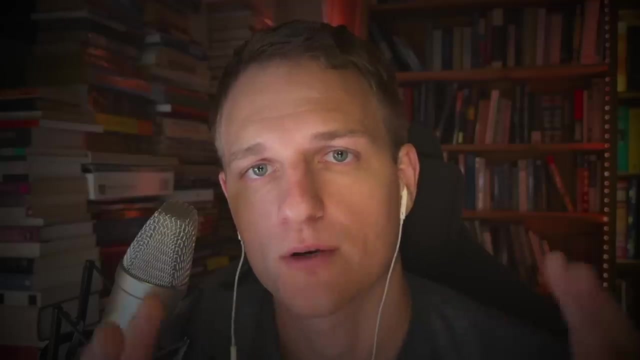 the vibrations of the whole atoms, but the way more intense, higher frequency, high energy vibrations of the electrons themselves, orbiting or spinning or moving. 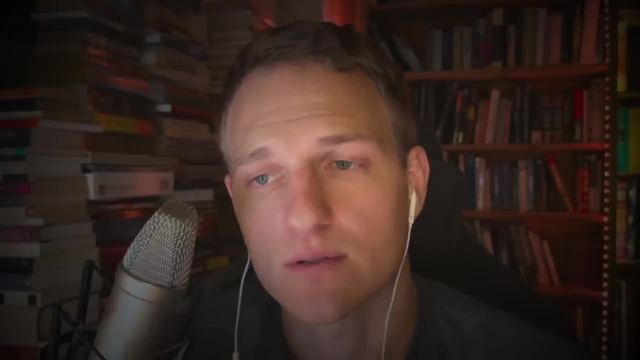 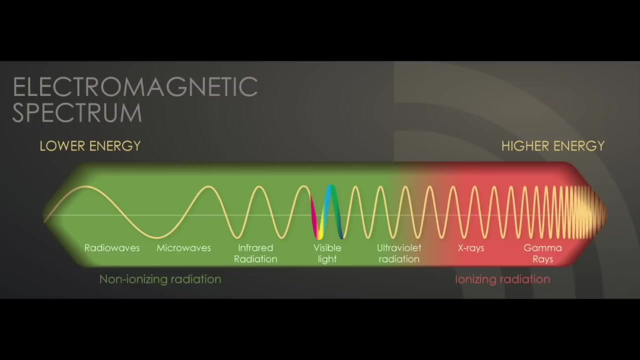 with some sort vibrations being UV or being optical up to UV, and then you have ionization which is free, basically free moving electrons. that 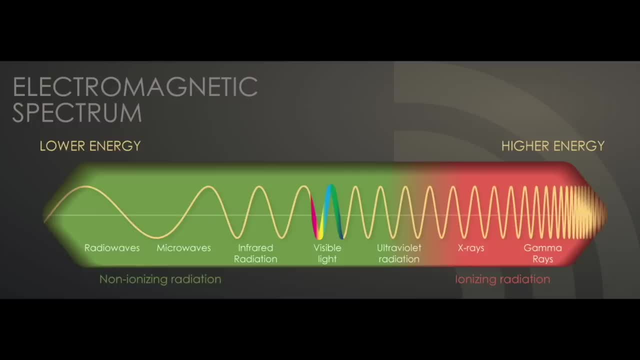 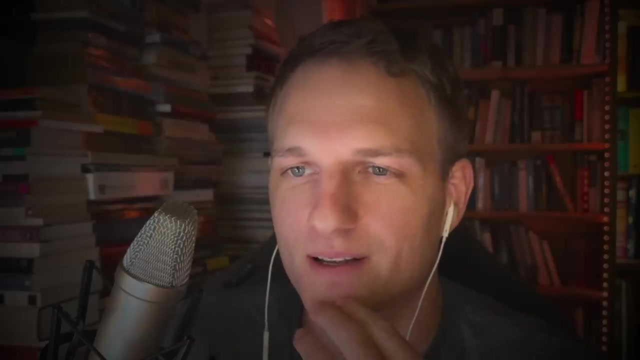 have so much energy that they're broken free. they, I guess sometimes. I hope that made some sense to you. hopefully I put enough pictures to make you to to register it. 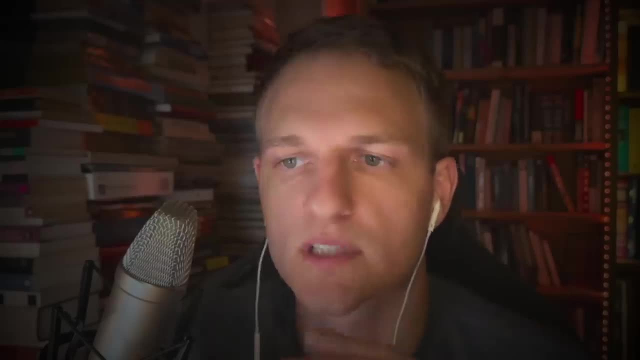 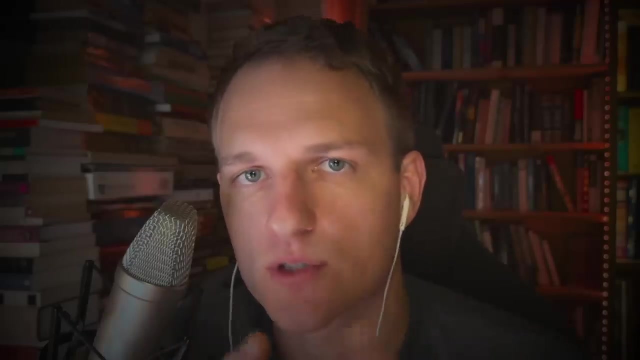 but that's how I understand it at least. it's important, because of how the universe shows us light, for us to be able to understand what's going on, whether it's whether it's looking at the. 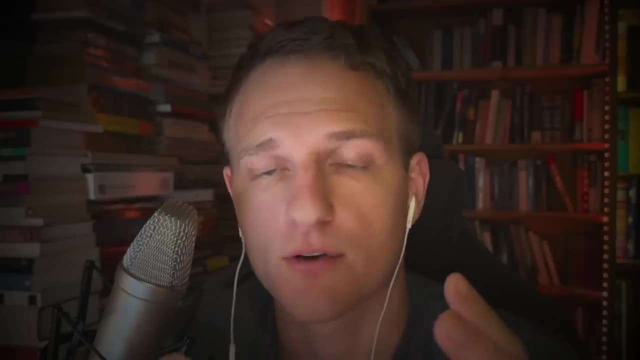 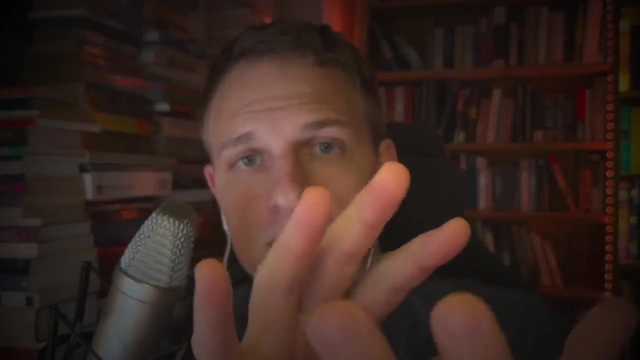 atmospheres of exoplanets and how they filter their own sun's light on the way towards us, if the orientation of the solar, that exoplanet, distant star system is oriented so that 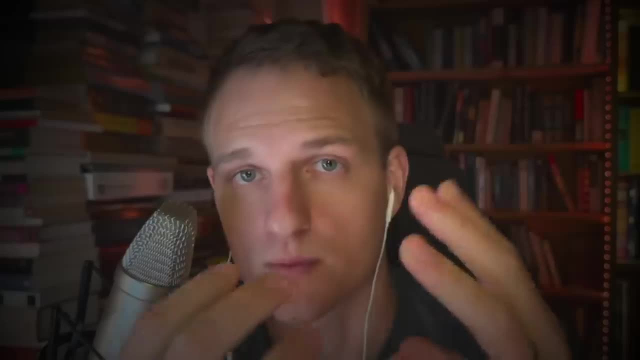 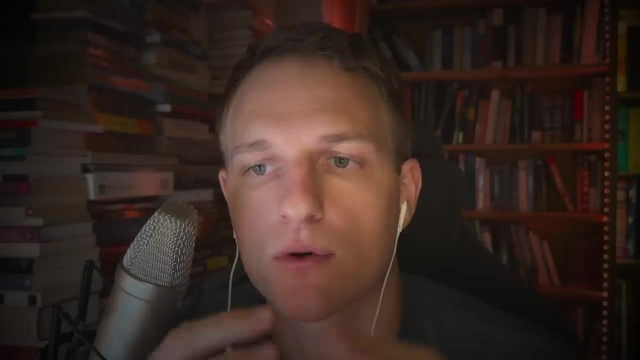 the planets are orbiting in front of their sun, with respect to us, and then the makeups of gas, nebulae, other stars- we can see the spectra of other stars and, in fact, anything that emits light. 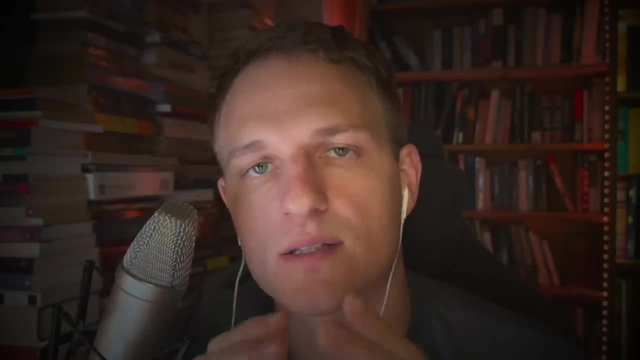 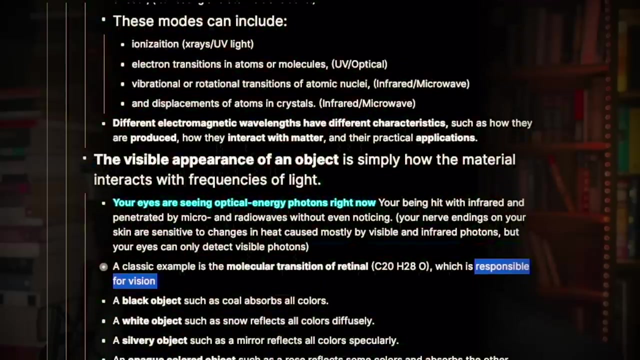 in the universe we can break into a spectrum and see tons of characteristics and details about- and this relates to the, the visible appearance for us of an object you know. for example, you know: 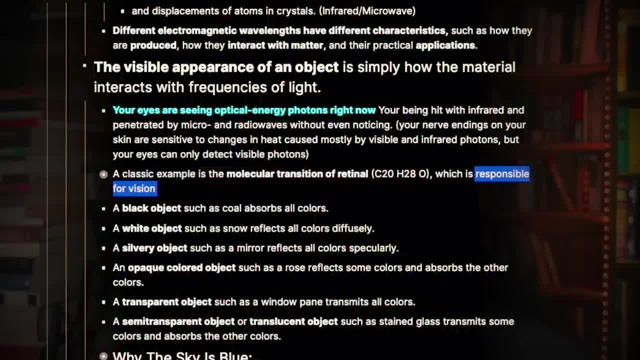 what's interesting is the. so the molecular transition of what's called retinal, which is the molecule responsible for vision in our eyes, is is what makes our vision work, is the molecule right here. 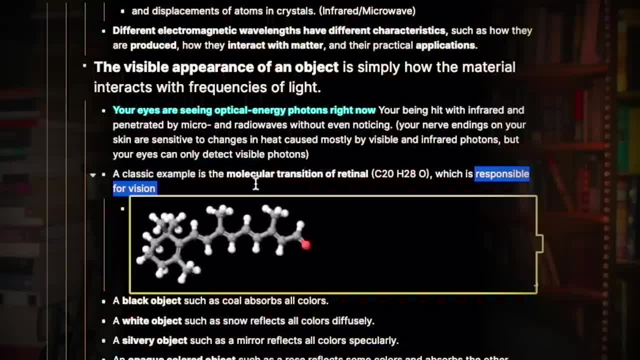 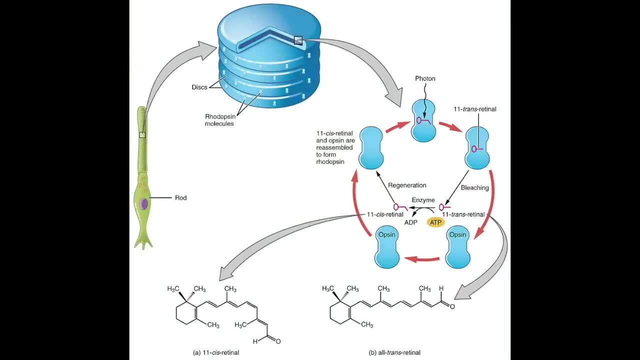 so it undergoes a series of transitions and of course you could see, with all those atoms it's got 20 carbon, 28 hydrogen and one oxygen, one little oxygen atom. the combination of of of. 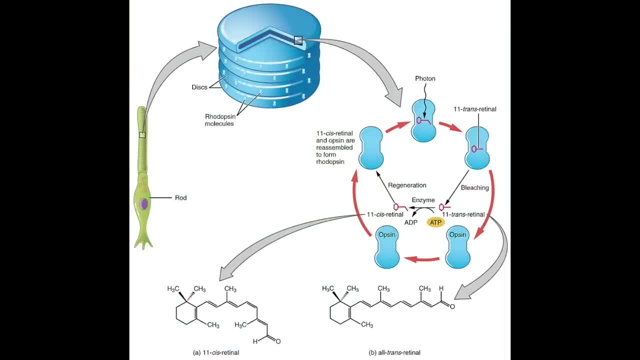 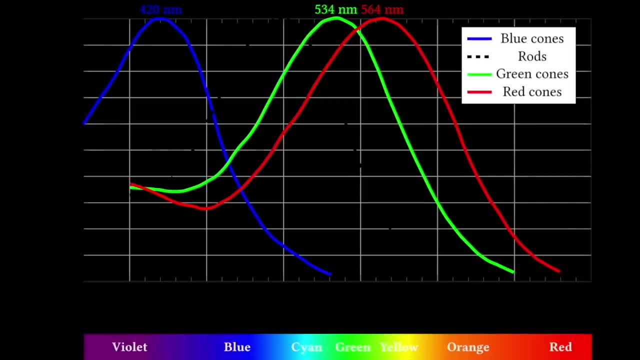 different frequencies between. so you know, the spectra, the absorption and emission spectra of of those elements and individual atoms combined into molecules is completely dependent on what the shape of the molecule is, what the atom. 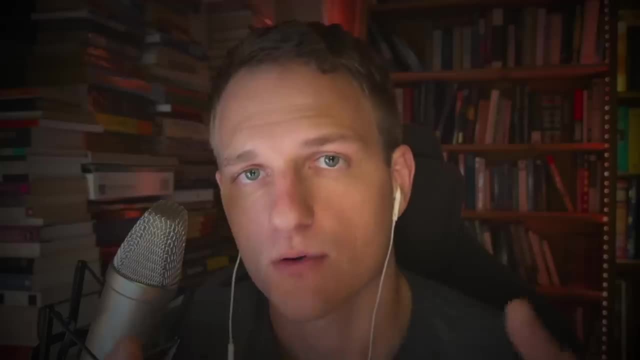 atoms are, how they're configured, how many there are, of course, how many electrons in each atom atomic uh orbit there are, and in certain, you know, ring-shaped molecules they even share electrons, which is a really cool phenomena. so that different. 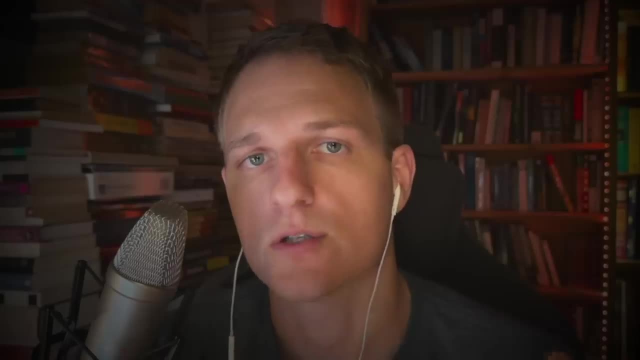 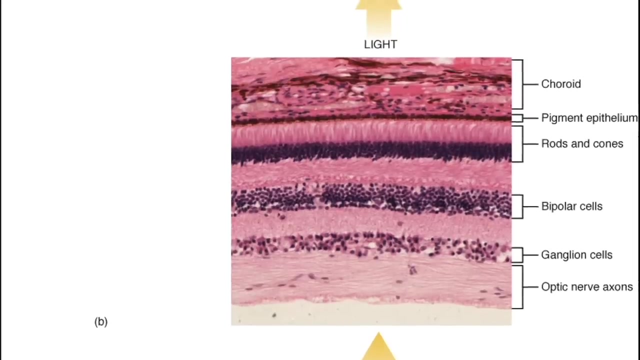 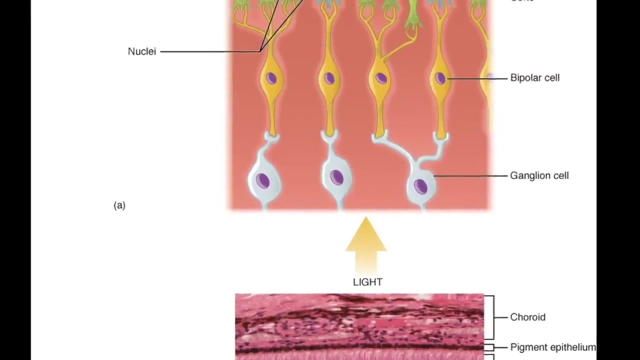 structure, even itself, can change the frequency of different types of frequencies, that of light that they absorb. so each molecule, even beyond the elements, beyond the atoms, each molecule combined of different atoms, has its own characteristic spectral absorption and emission lines and are the molecular transition of retinol is when sunlight or any light that falls within our 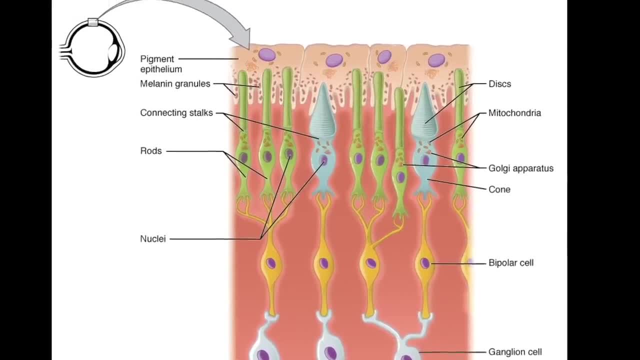 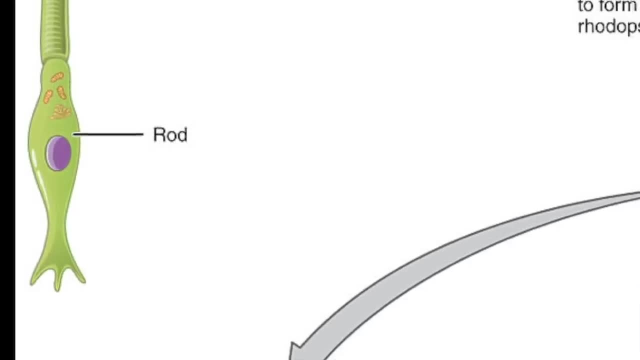 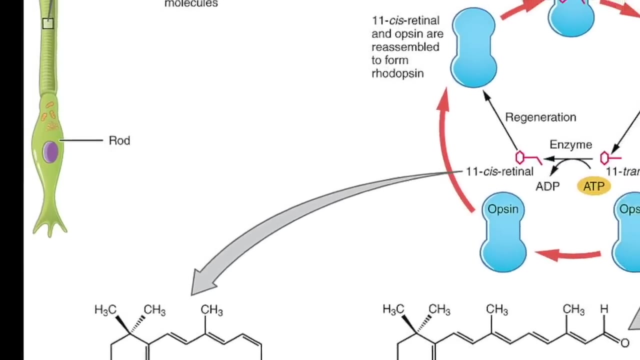 visible range that we can see hits our eyes. it stimulates these molecules that send neural signals to our brain to register it as some sort of stimuli from outside, of course, unless we're in a simulation and it's all in our brains like the matrix. but yeah, it's just interesting that. 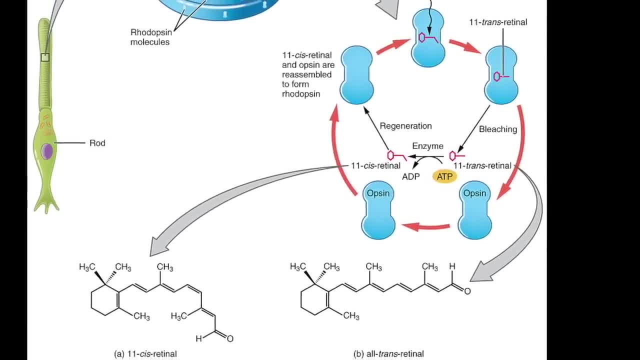 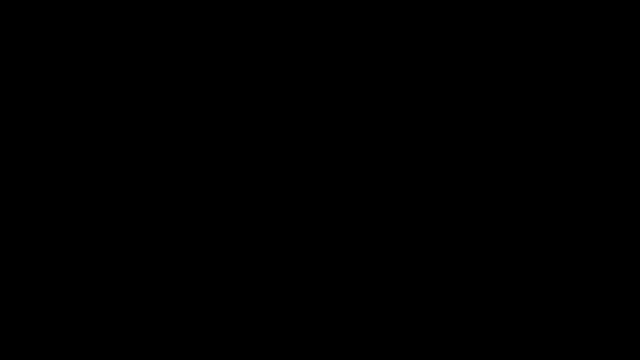 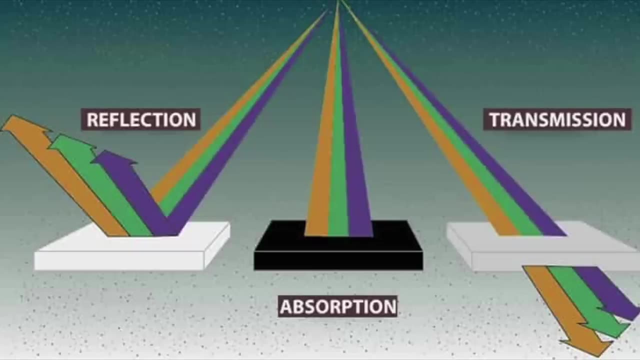 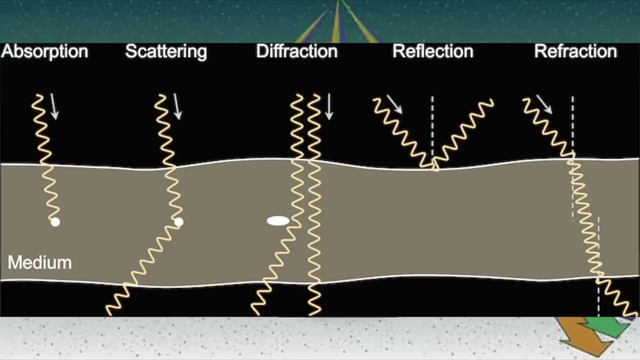 that's, you know the mechanism for how we now we see no black object. just in general terms, how objects appear to us. a black object like we talked about as such as coal, has no reflectivity. a purely brought black object, it will absorb all colors. a white, 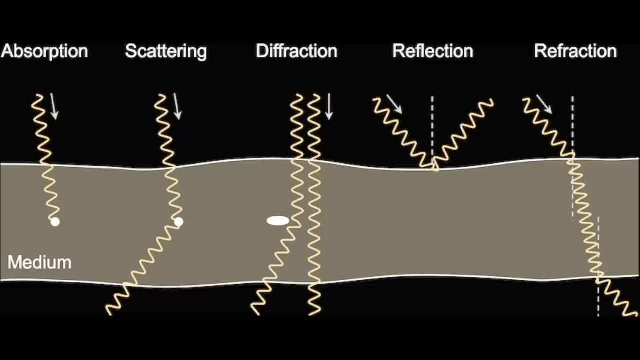 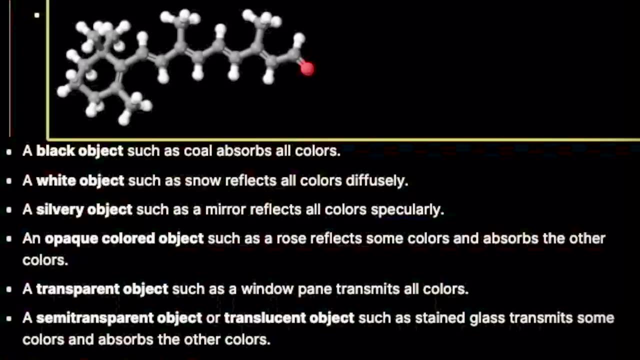 object reflects all colors, like snow. a silvery object, such as a mirror, reflex colors specularly an opaque colored object. so something- I mean anything- that has a specific color to it, basically absorbs all the colors, but the color you see, a rose, absorbs every other color, but it's red wavelengths if it's. 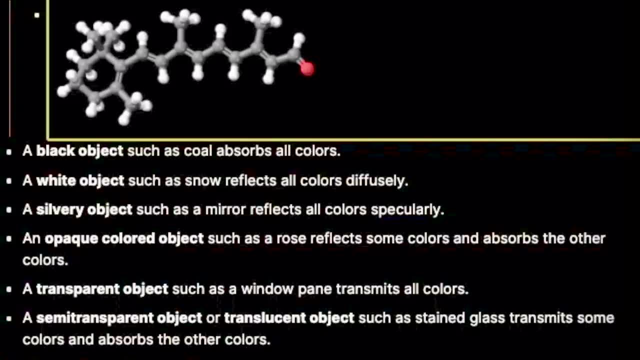 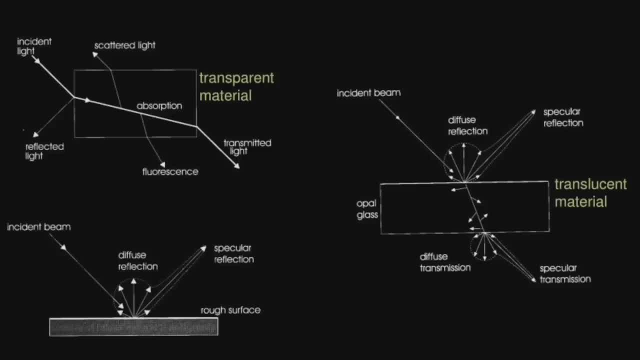 a red rose, for instance, the transparent object emits or, sorry, allows the transmission through itself of all colors, like glass. and then stained glass, for instance, a semi-transparent object or colored liquid will emit only, will absorb all the colors and only allow the color that you we see it as to pass. so a blue liquid would only allow blue light coming into. 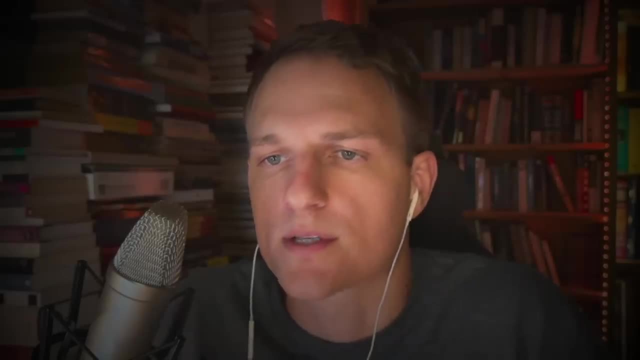 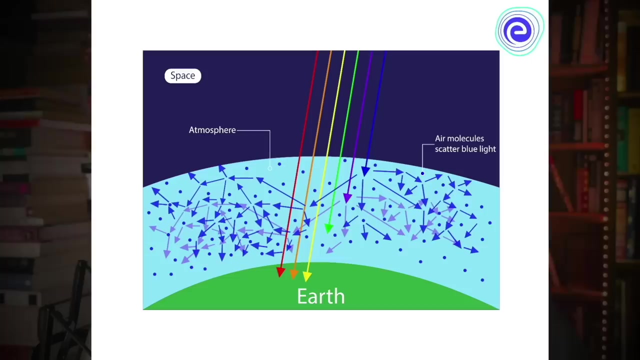 it to pass, and even the sky. the reason the sky is blue has a molecular as an explanation, based in how light interacts with molecules in our atmosphere. it's because the sunlight has plenty of red and blue, mostly peaks in green, but it has plenty of all-color. the reason this guy 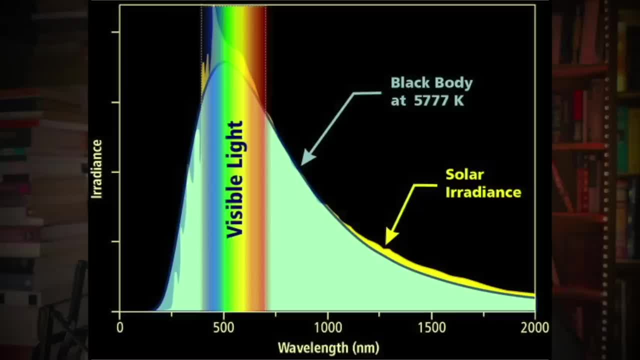 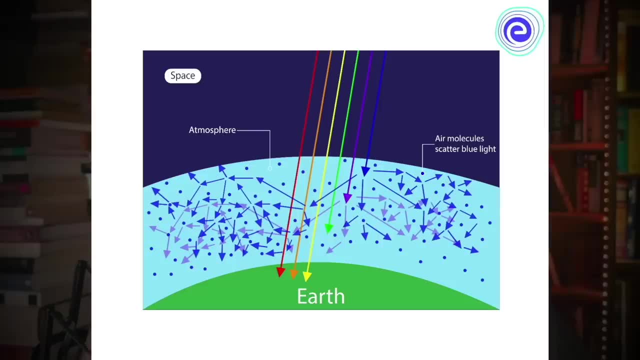 is not purple or orange or green and it's blue, is actually because blue, being the highest energy at the lowest, smallest wavelength of the visible spectrum that we can detect, is scattered. it just happens to be scattered by the particular molecules that we have have in our atmosphere. it's scattered really well and, apparently, as there's a law, i forget. 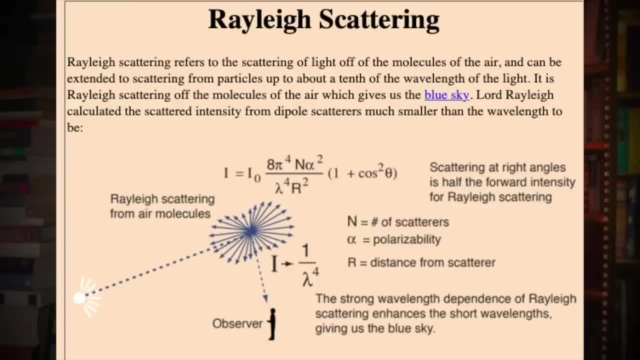 i guess i didn't write it here, but there's a wall, a law that says that light of wavelengths of shorter frequencies are scattered, with a scattered more on the order of magnitude of like four times uh, so like four thousand or forty thousand times as much. sorry, it won't be ten ten. 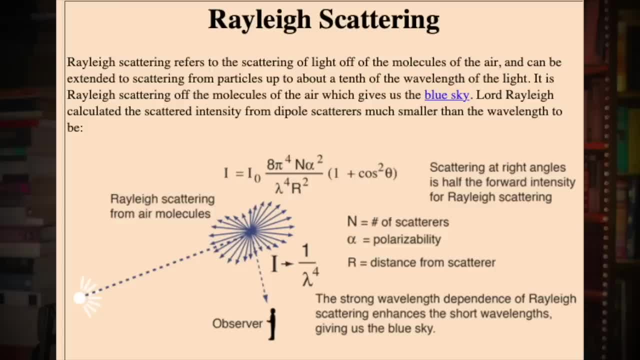 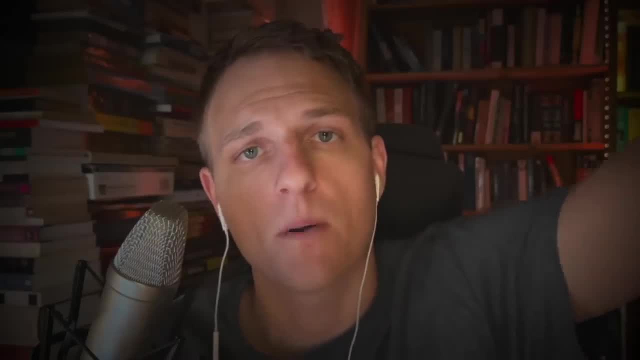 ten thousand. i was way off there- it's. it's ten times, but it scatters ten times more than red light. so as we look at the sun, even though the sun has all these colors, we perceive all the colors mostly, are coming through, although some of the blue light is getting stripped out because it's 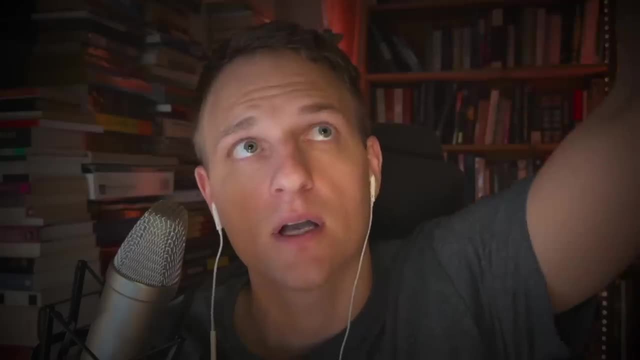 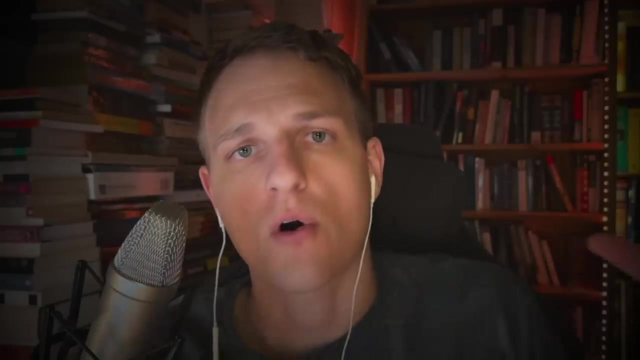 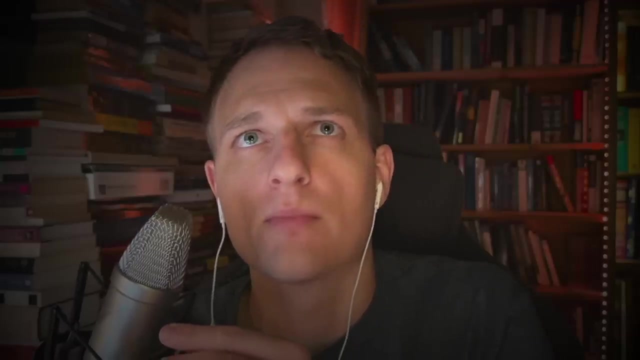 getting scattered way more than the red, and we're seeing the white sunlight as it hits us when it's overhead, but all the blue light is being scattered all over the atmosphere at 10 times the rate. red is you and that's why. so all the blue light we're seeing from the sky is actually sunlight. that's been 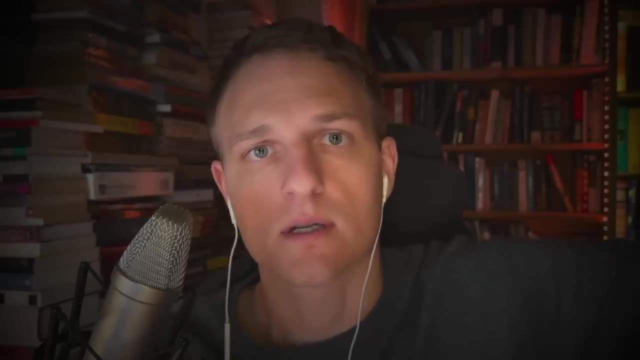 deflected and scattered way off in the distance and bounced back towards earth and uh, because blue does that more than red. that's why the whole sky looks like it's blue, because all those molecules- oxygen and nitrogen- prefer- just based on their shapes, uh, and how they interact with light, they prefer, they tend to, uh, to not anthropomorphize it too much. 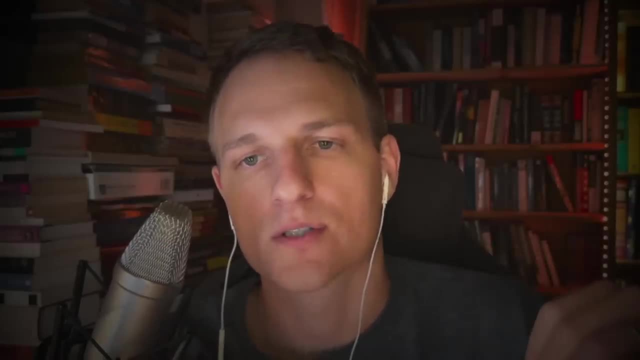 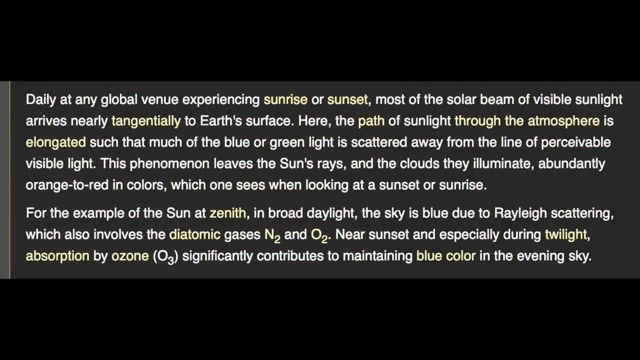 they just tend to scatter blue light way more than red, and then red sunsets occur, i believe because it goes through so much more atmosphere that at uh uh do i remember why red sunsets occur. i think it has something to do with the angle of the sun being really low to the horizon. 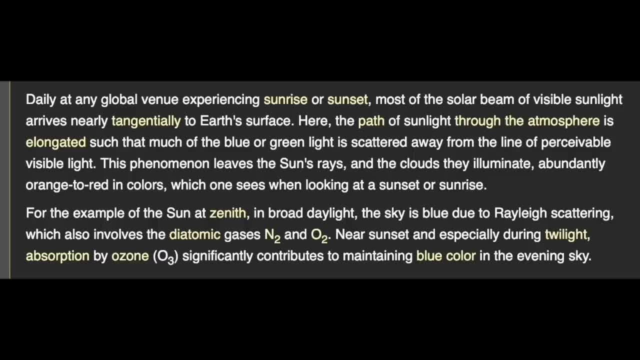 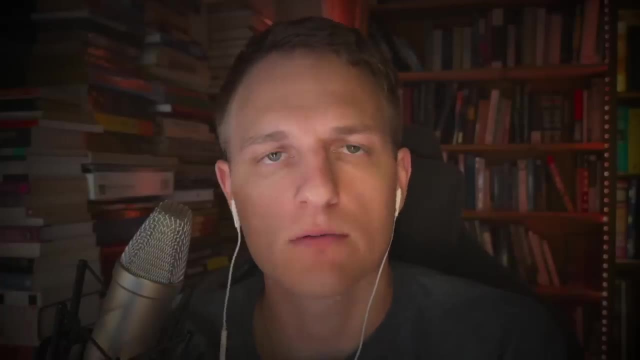 so it has to go through way more atmosphere and i believe there's maybe another effect at a really low angle that comes into play that allows more scattering of longer wavelengths like red. but the quantum mechanics, the nature of light, the black bodies and the uv catastrophe, that's all important because 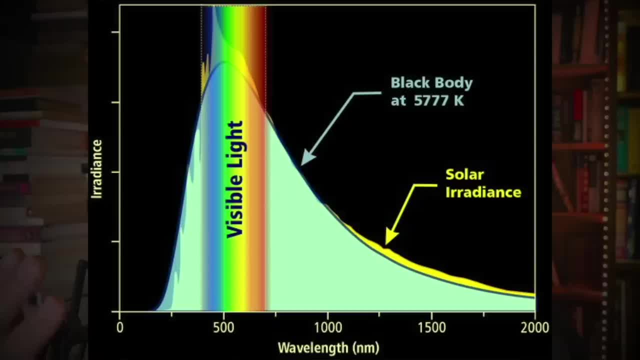 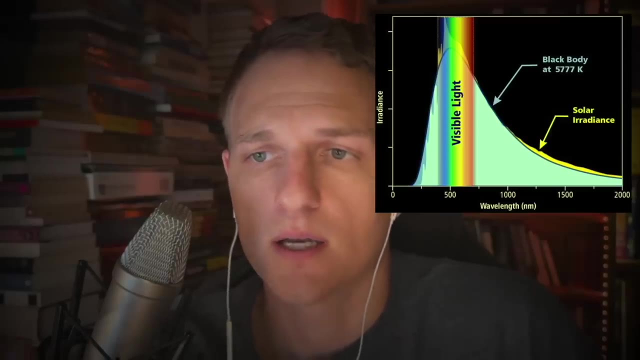 stars are modeled as black bodies and they make, apparently they make really really good, um, very accurate, very close approximations to black bodies. when physics, uh, when all scientists make a decision about the assumptions for any particular model, what they do is they usually make a reasonable trade-off between the acceptable model, errors and the difficulty of calculation of the 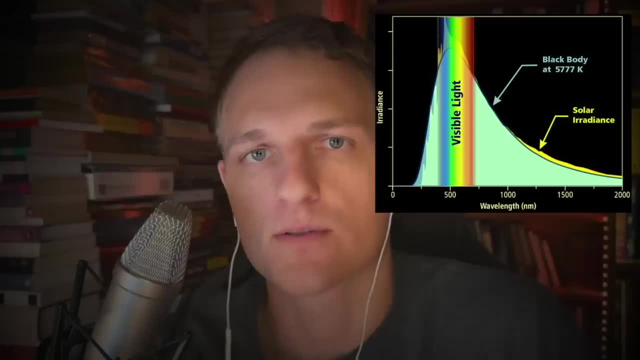 mathematical curve. they're trying to fit to the phenomenon. So if there's a curve that just roughly corresponds to it and then there's a curve that's a very close fit but you know infinitely more complex to calculate, they're probably going to use the one. that just is more. 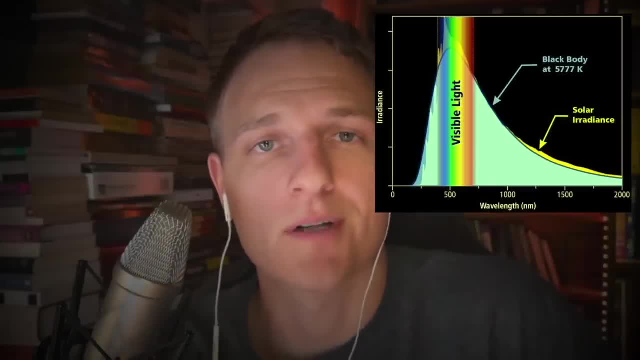 of a rough fit because it's close enough, it's good enough and it'll save them a lot of work. Maybe that's why our AI systems in the future will help modeling the real world way better. But they've used for centuries- for at least a century, I guess, they've used a black body curve. 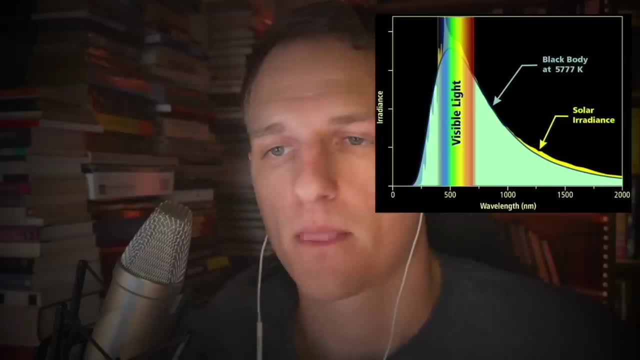 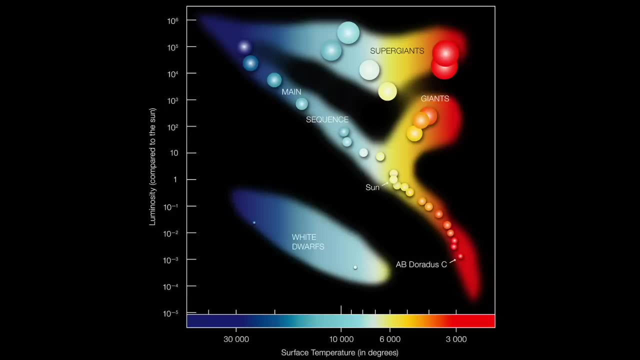 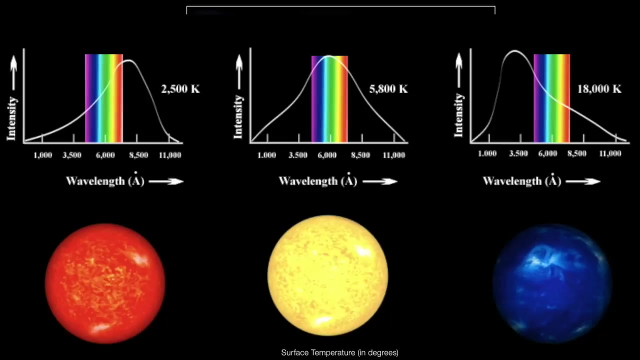 to simulate a process. They'll approximate the sun's spectral emissions and there's what's called an HR diagram. that is roughly a relationship, a very well-defined relationship, between the color of a star- whether it's blue, orange or white or yellow- and the temperature of a star. 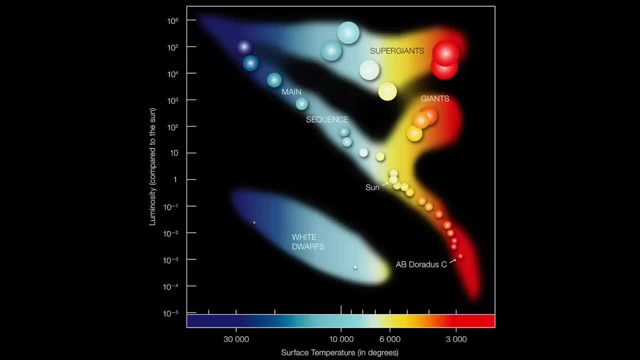 And that's That comes from the black body relationship of color, of temperature to the peak wavelength of that black body curve, or now known as the Planck curve. And there's another law that goes along with Planck's, called the Wien's displacement law. that tells you exactly at what wavelength 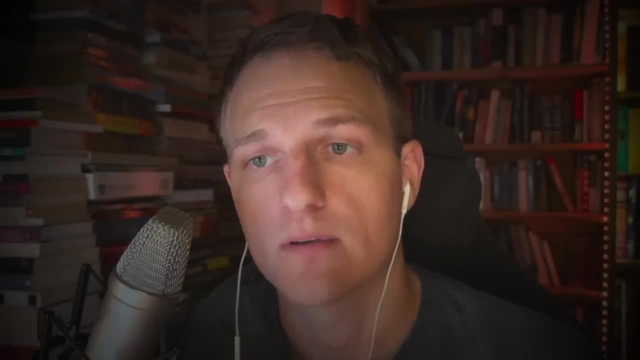 that black body will peak for any given temperature, regardless- and this is cool because it's regardless- of what that material is. It's not just a matter of how much heat is made up of. so it could be if it has enough atoms. essentially, it could be all perfectly one element, and they won't emit that one absorption line. They'll emit a ton of a continuous spectrum just because there's so many geometries going on and there's so many vibrations and rotations of molecules emitting different wavelengths and energies. 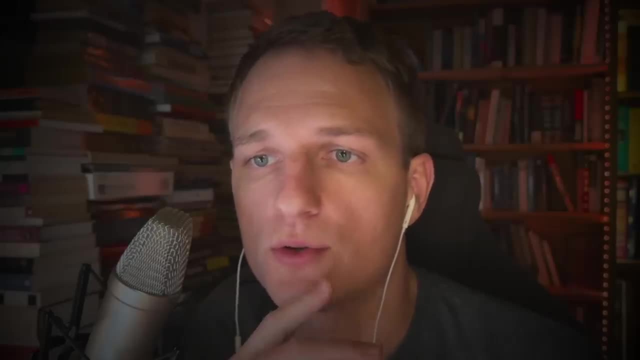 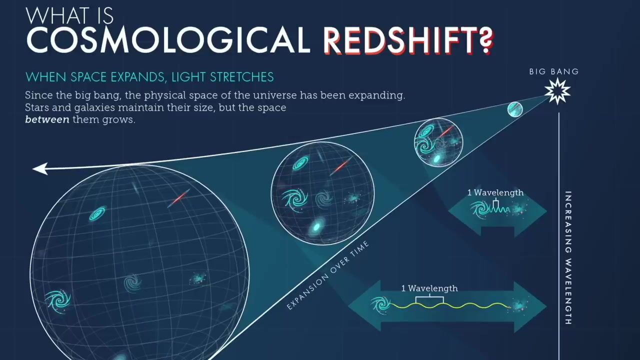 So even scientists were even able to estimate how hot the sun is, But lava is based on its color, which is, I thought, pretty cool, and there's tons of other examples of how useful black bodies really are. I think I put this in here because the main point I wanted to make was that, while I was 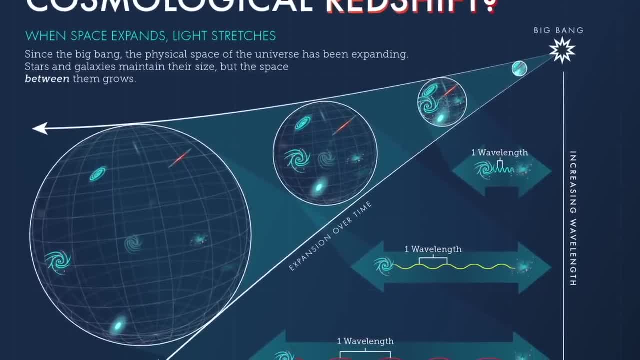 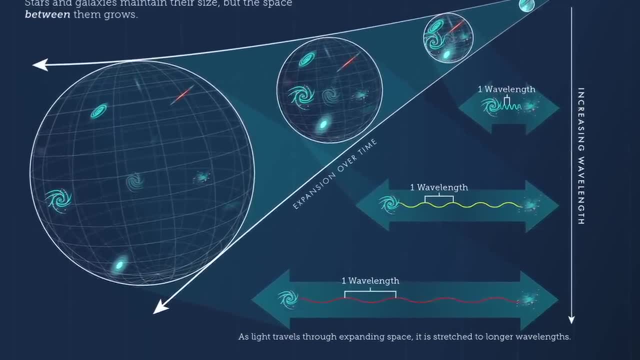 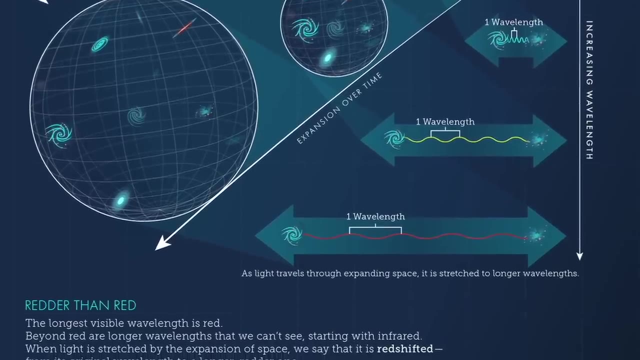 studying why the Webb telescope was built specifically to be infrared. I could understand that. you know maybe well, one of the big explanations was that when things are redshifted, when things are far enough away, of course, the expansion of space causes the what was. 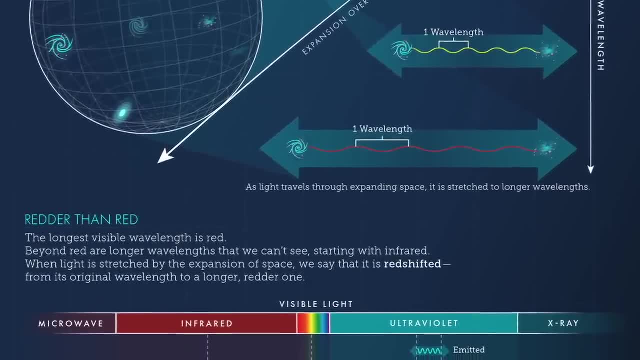 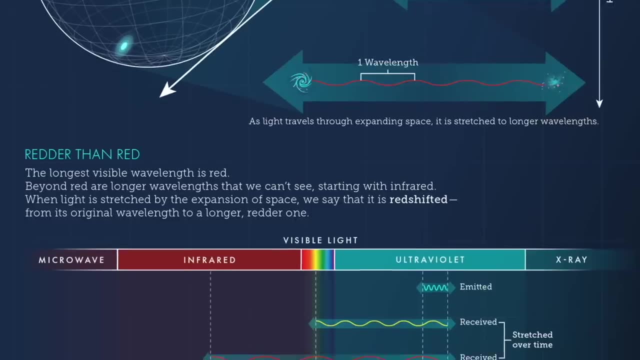 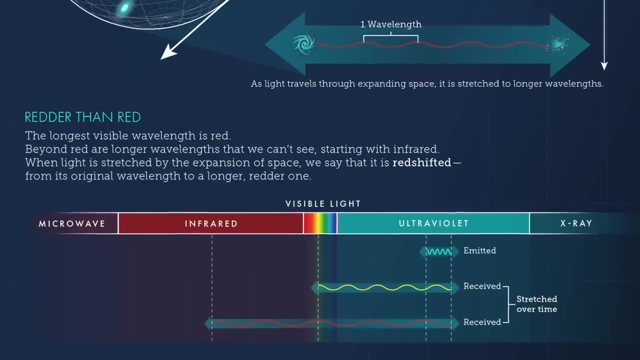 initially emitted as UV or visible light is now stretched into the infrared, and so they're actually invisible galaxies. It looks black to. if Hubble hadn't been equipped with its infrared sensors, it wouldn't be able to detect half the galaxies. It would be a mess. 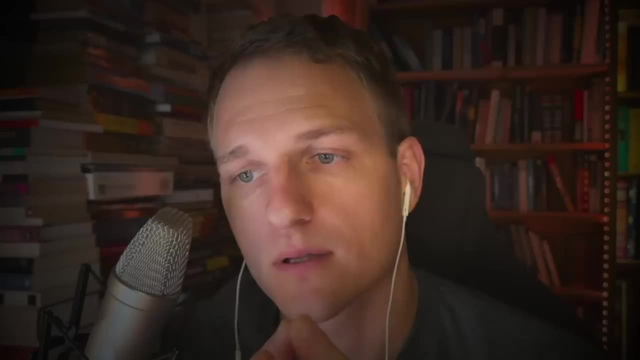 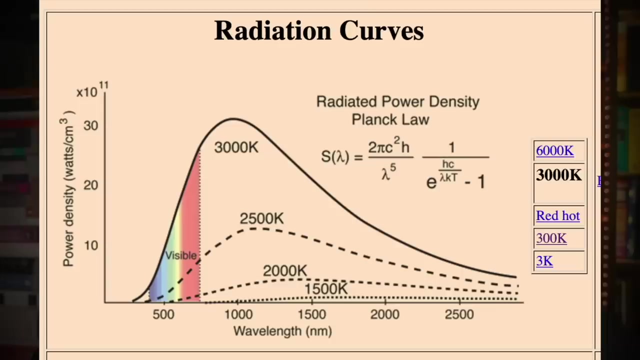 It would be a mess in its deep field. But that doesn't explain why the light was mostly UV and white to begin with. It's why galaxies were mostly emitting most of their light. It's why they peak in the optical and UV light range. 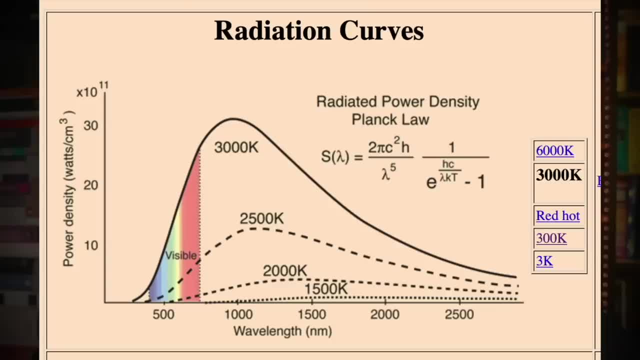 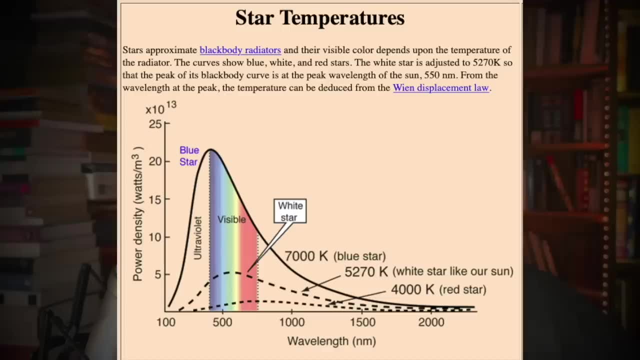 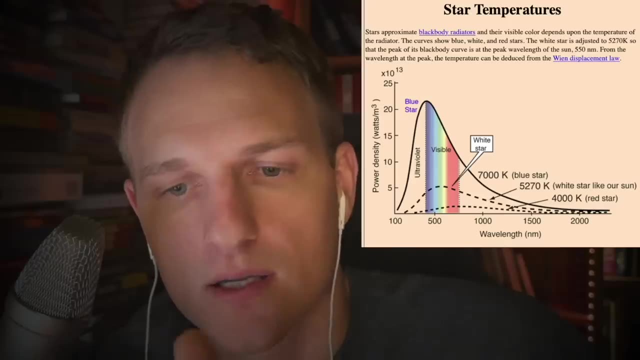 It's why a lot of galaxies- unless they're very, very high energy galactic galaxies, like galactic cores, quasars or supernovae, don't emit a ton of X-ray radiation. It's because of that ultraviolet catastrophe that drop-off in the peak as it gets hotter. 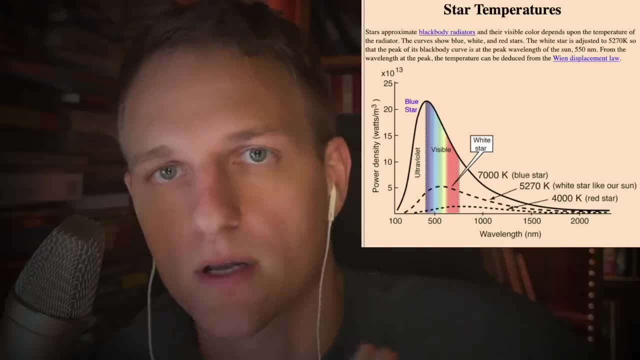 and hotter as the temperatures get hotter. So it turns out that most matter, most stars, stellar matter, of course, makes up galaxies. so most galaxies composed of stars in the universe emit ultraviolet light. That's why they're called galaxies. 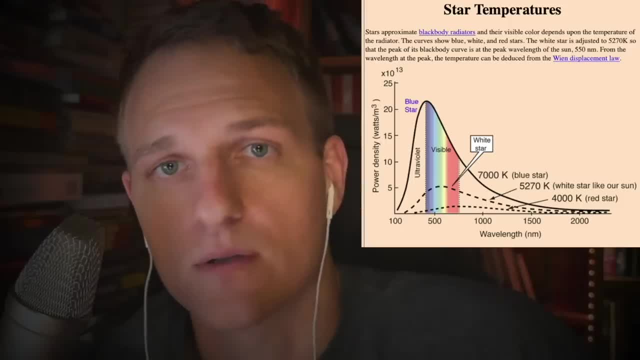 That's why stars in the universe emit almost all of their radiation, which has a ton of spectral line information in it that tells us the composition and the- you know- densities of stars and the temperatures They- well, they emit at temperatures that peak in the visible and UV wavelengths. 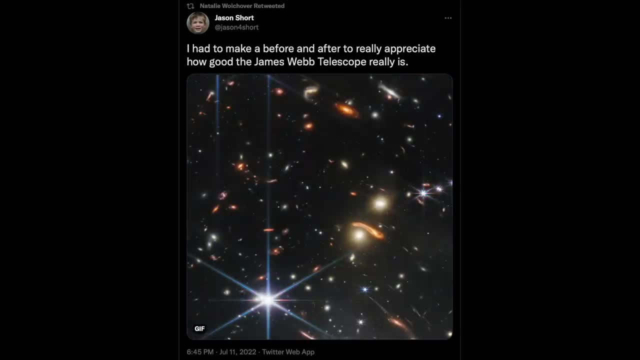 So I was always wondering why, like why aren't we using optical telescopes to look for you know ancient, really distant X-rays that's been shifted into the optical? Or why aren't you know infrared? why aren't we using radio telescopes to look for stuff? 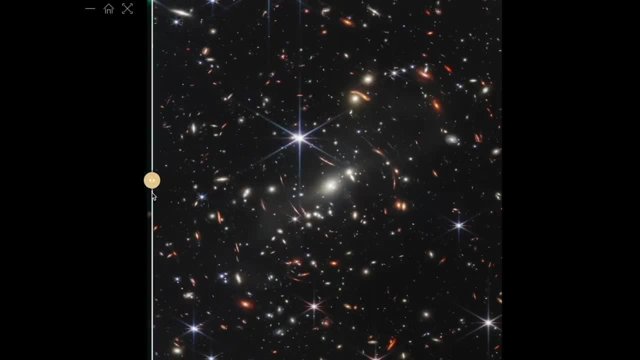 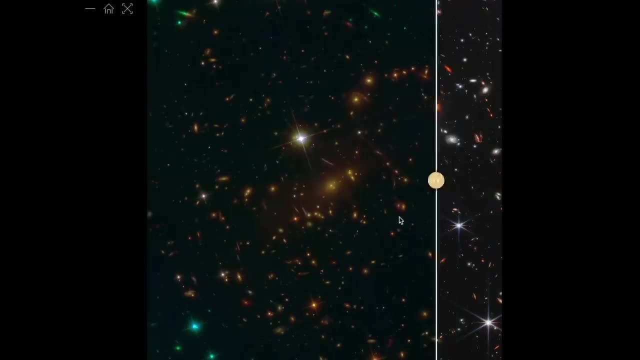 that's been shifted into the radio And it turns out- you know we are to some extent doing that- but the bulk of the galaxies that we're going to see, the first stars we might see at the beginning of time in the 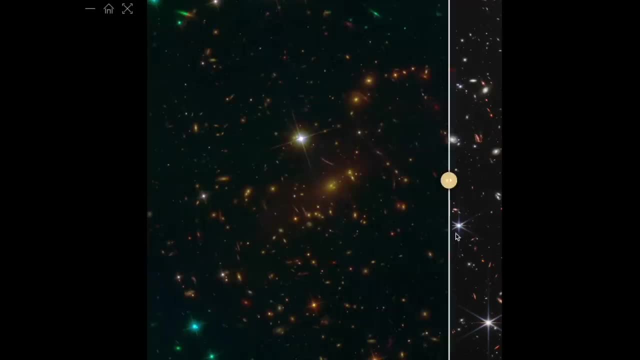 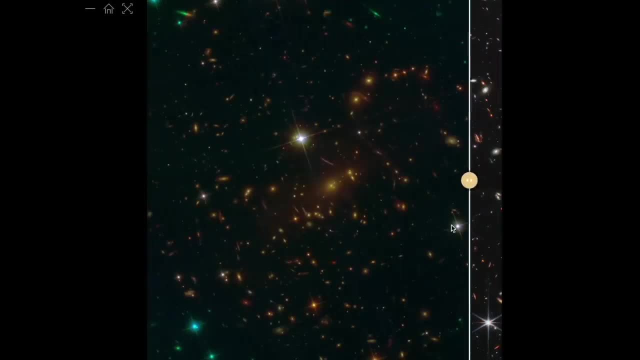 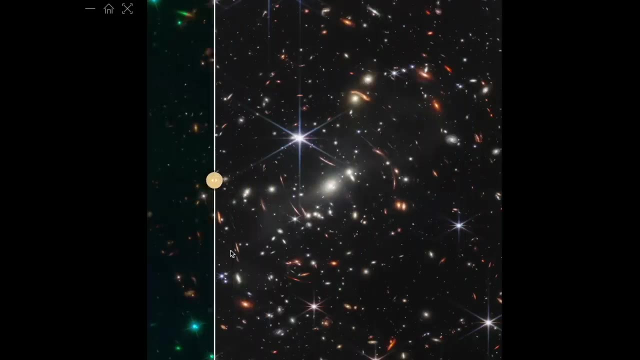 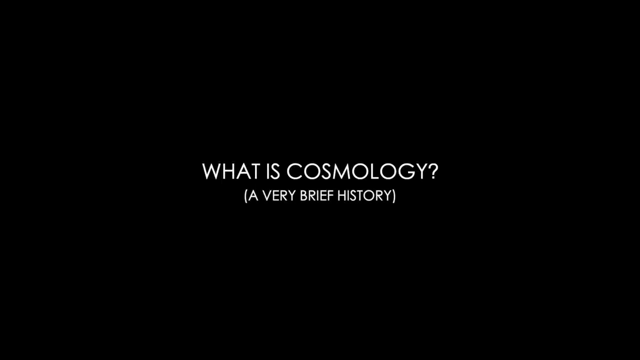 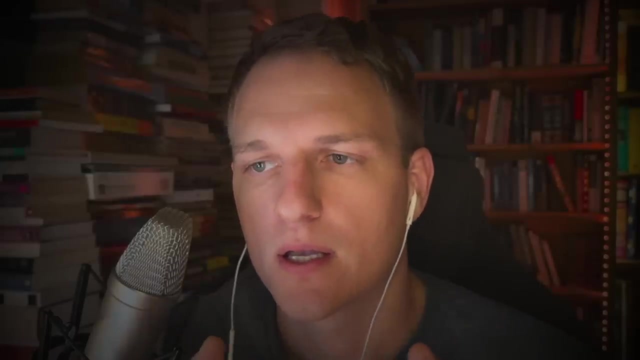 from them peaked in the visible, exactly in accordance with the black body Planck curve. So that's been shifted since then. So what is cosmology? It's the study of the origin. It's the study of the origin and the evolution of the entire universe. 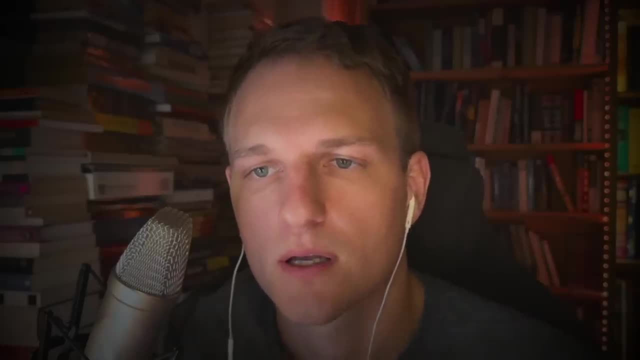 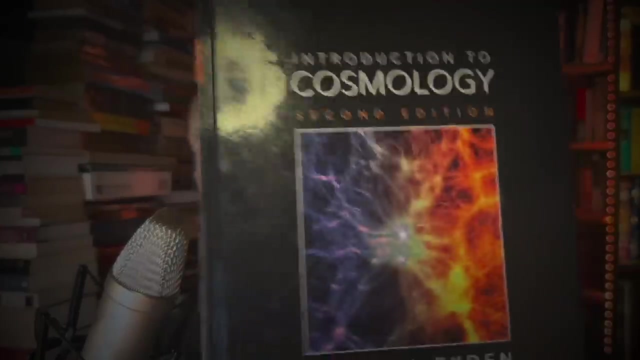 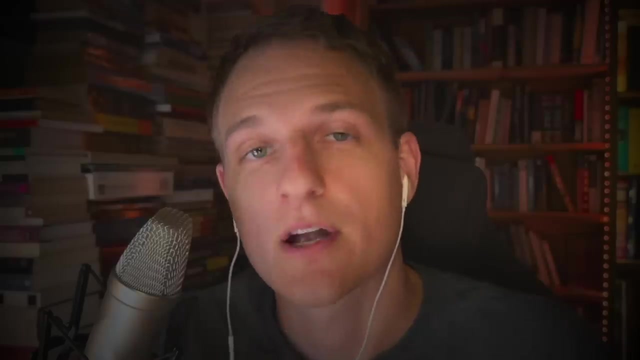 It's the biggest picture we have of our existence. I think that's why it's so fascinating. This is actual an actual cosmology book here, an introduction to cosmology. There's a scary amount of math in here. I actually wasn't expecting that. 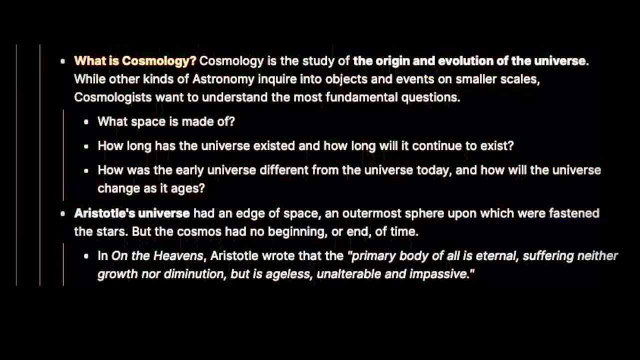 Cosmology. It tackles all the big questions: What's space made of? How long has the universe existed and how long will it continue to exist? How was the early universe- one of the big ones Webb is asking- different from the universe? 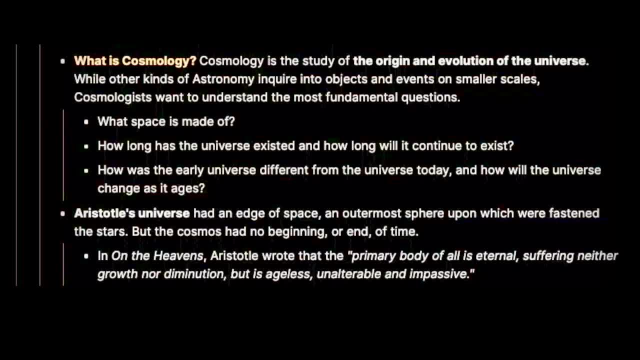 of today. Aristotle's universe, as we kind of alluded to, was different way, different than ours, But it has some features. Earlier ideas were still transmitted, The ones that stood the test of observation have informed our current understanding of the universe. 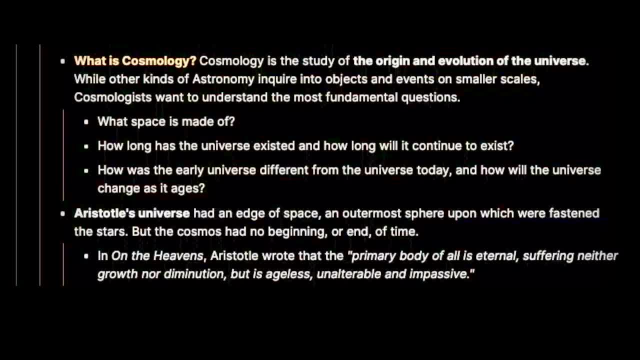 Aristotle's universe had an edge of space, an outermost sphere upon which were fastened the stars. But the cosmos that he understood it had no beginning, so it had an infinite existence in time. And on the head of the universe there was no beginning, so it had an infinite existence. 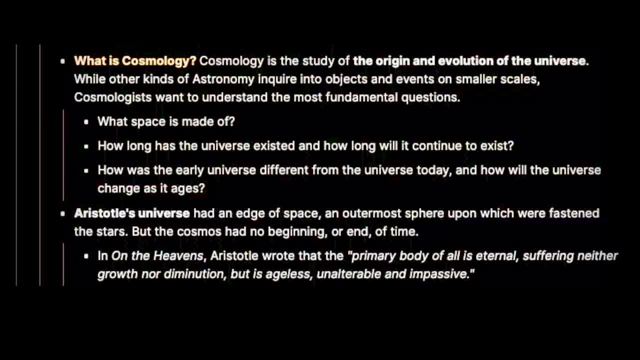 in time And on the head of the universe. there was no beginning, so it had an infinite existence in time. Then, in the heavens, Aristotle wrote that. he wrote that the primary body of all is eternal suffering, neither growth nor diminution, but is ageless, unalterable and impassive. 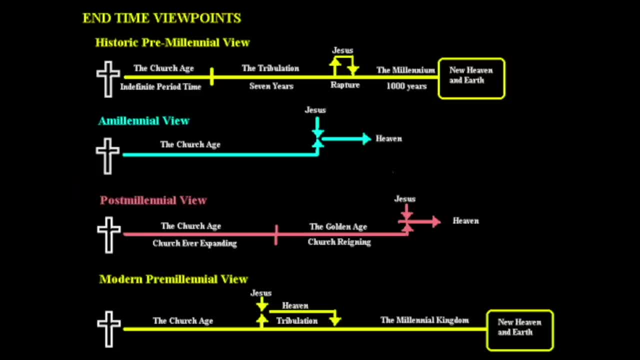 Then the Judeo-Christian worldview, coming out of Eastern Mediterranean, did away with eternity, but it maintained the idea of cosmos. Cosmos with that was finite and without change. so it didn't change, but it was. it did have a definite beginning and a definite end, and that would be the what's that. 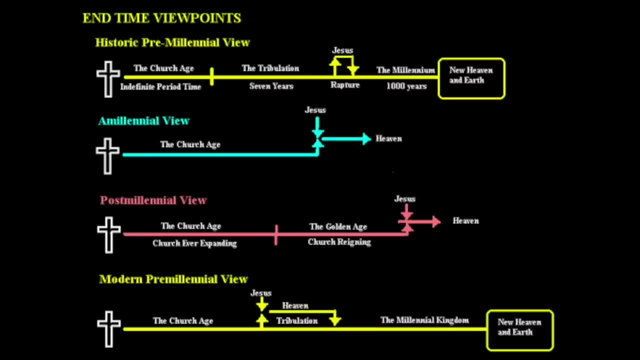 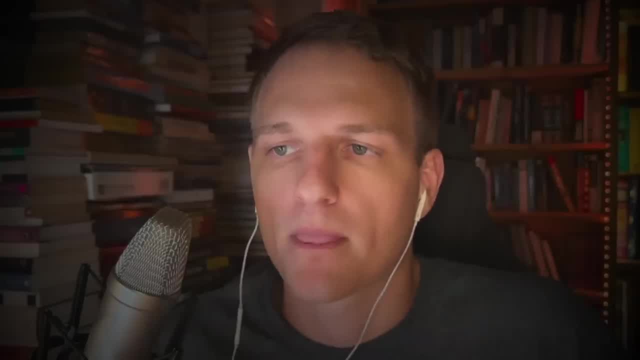 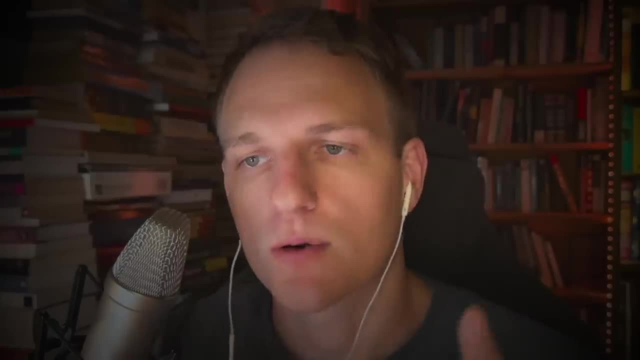 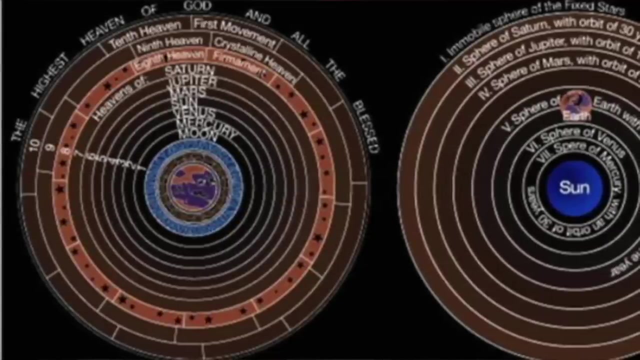 called eschatology. according to this and many other ancient traditions, the universe was created from nothing and has remained at the same ever since, but then Copernicus, in 1543, he demoted the earth to a mere planet around the Sun, like we talked about, and that changed the way we looked at things. this wasn't. 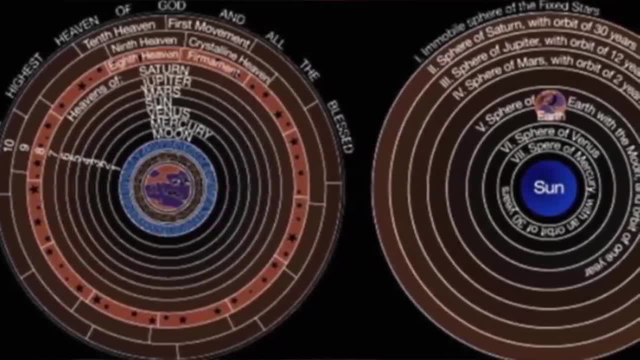 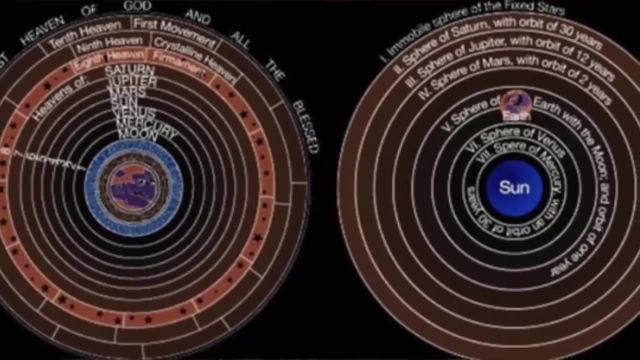 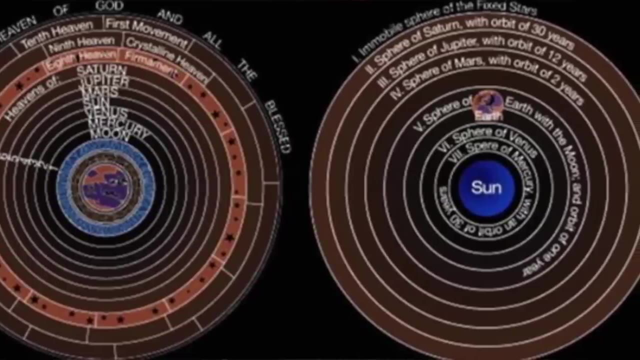 changing the earth to tell him belief, though, that the universe was both spatially finite and static in time. so what Copernicus thought of still was like, yes, the things. everything didn't revolve around the earth, but in fact the earth spun and we revolved around the. 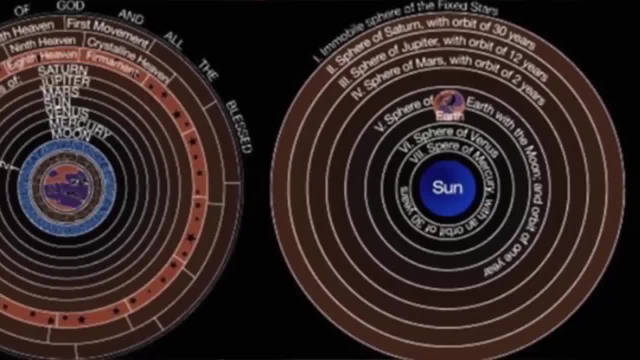 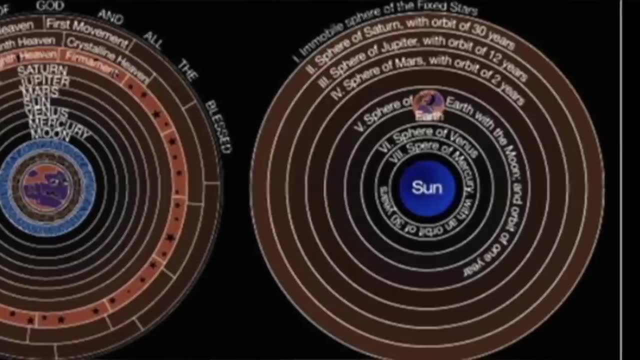 Sun, but it was still a spatially finite universe. there was an edge to it and over time it didn't evolve, it was eternal, it stayed the same. and then you know- I'm not going to go into too much detail on that, but I think it's. important to understand that the universe was created from nothing. and then Copernicus: in 1543 he demoted the earth to a mere planet around the Sun, like we talked about, and that changed the way we looked at things. this was changing the way we looked at things. this was 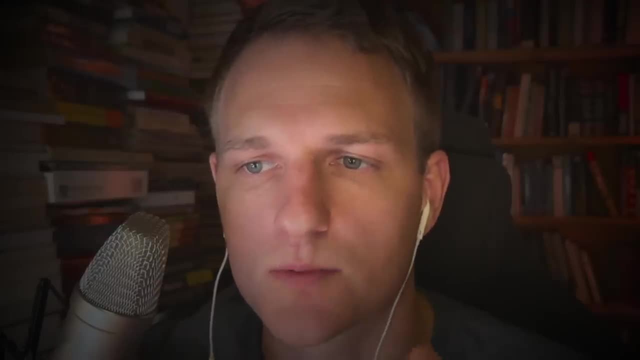 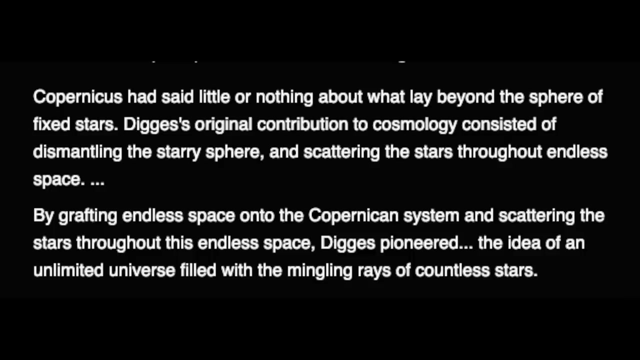 maybe half a century after Copernicus. Thomas Diggs became the first Copernican to pry the stars off their crystalline sphere, that in that finitely static edge of space, and what this effectively did was spread them throughout space. it was the first time scientists, people, had consciously really 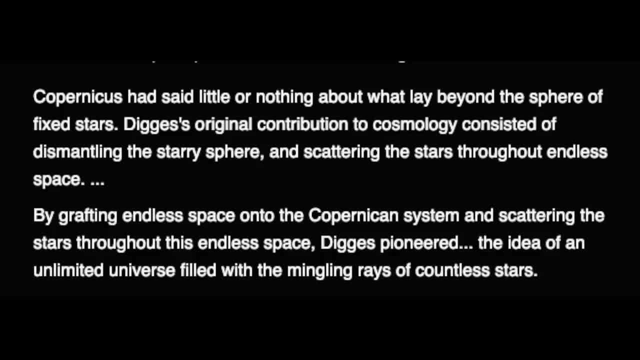 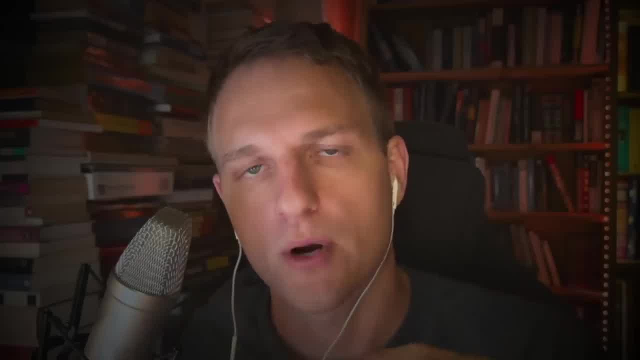 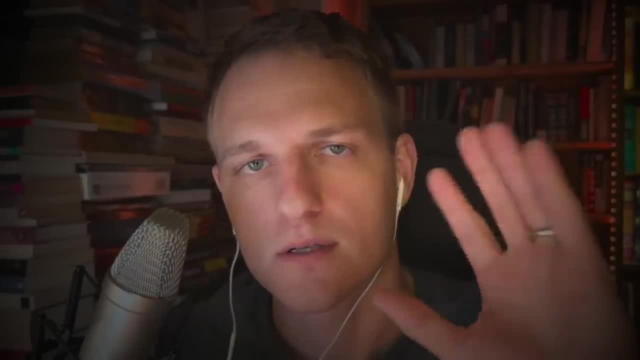 thought that possibly the stars might be at different levels than the earth and different distances, and they might exist the way in a three-dimensional- not paradigm- rather than just a two-dimensional, you know, stuck to the two-dimensional surface of this distant sphere, but even then the universe was. 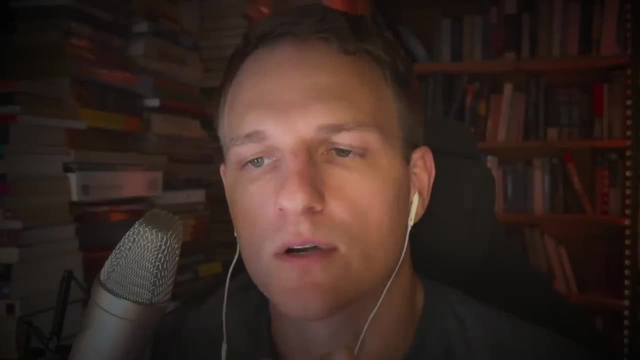 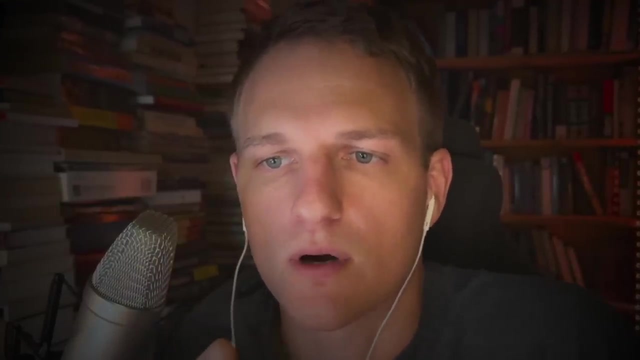 still viewed as unchanging with time. Newton even argued the same view. a century later he discovered that the universe was still unchanging with time. but even then he discovered that the universe was still unchanging with time. the ideas to you know the, the actual math behind how the planets orbited. but 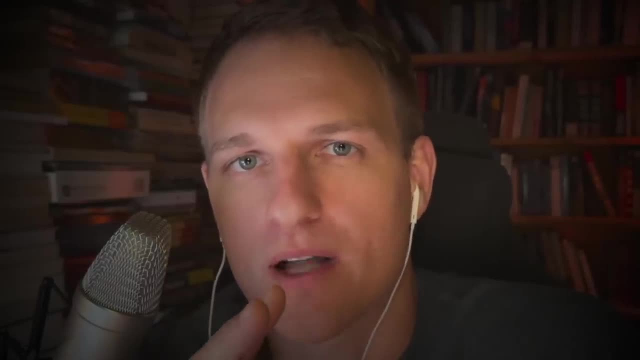 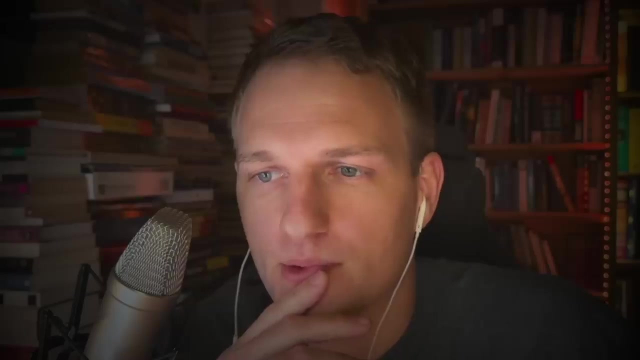 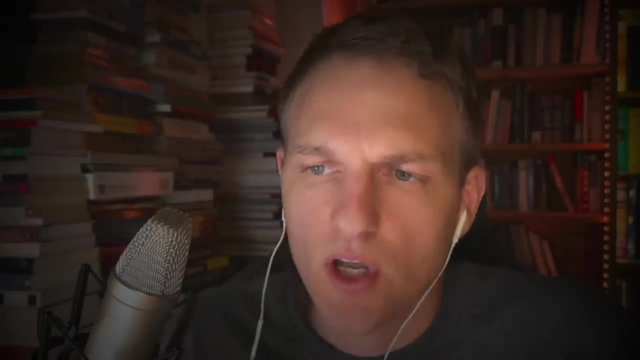 he discovered the ideas to, you know the, the actual math behind how the planets. even then, he couldn't bring himself to imagine a universe that had motion beyond just the planets around the Sun, and so this universe, he assumed, remained the same from one aeon to the next. there's one paradigm in in this book. 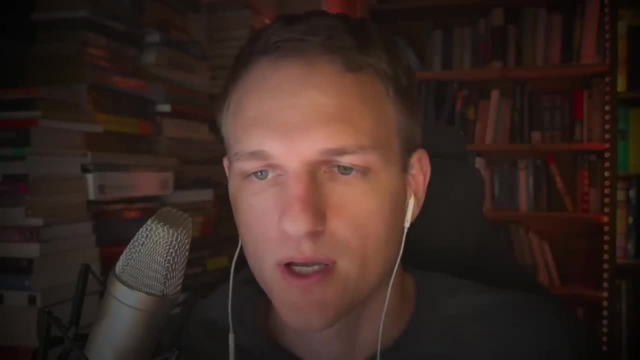 the universe that had motion beyond just the planets around the Sun. and so this book here- I mean it's not from this book, it's just age-old paradigm- called our paradox, called Olbers paradox. it was a paradox that was meant to refute the argument that the universe was infinite, basically. 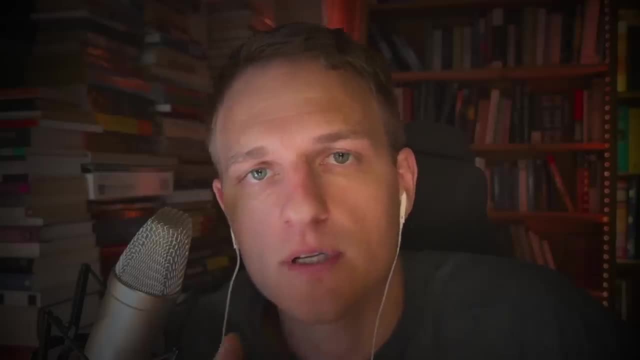 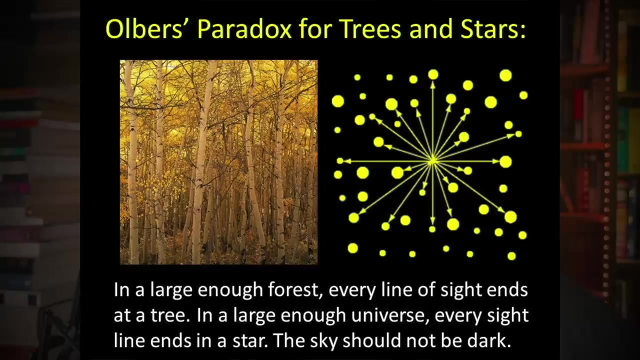 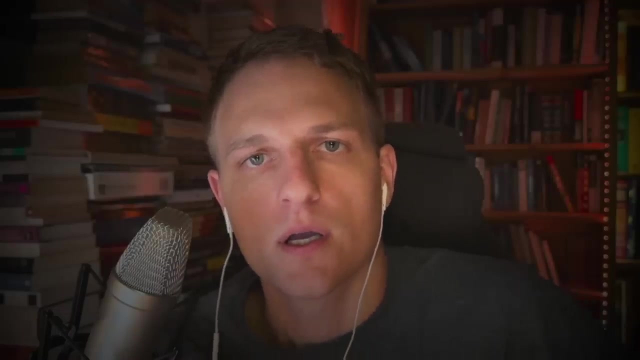 really just a way of saying that if it was infinite in space and time, then why isn't the night sky perfectly bright, as bright as the surface of a Sun? it says that if there has been infinite time for an infinite field of stars to exist, then why hasn't the light from all those distant stars come in our field of view? 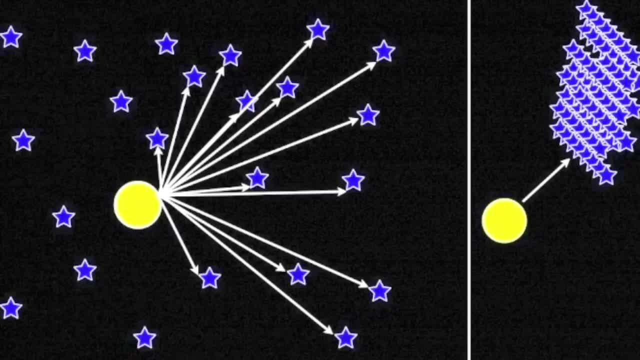 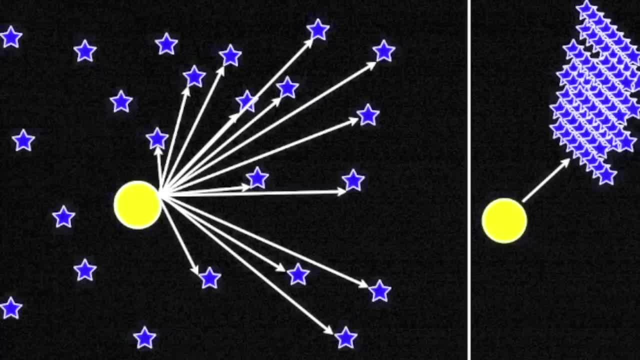 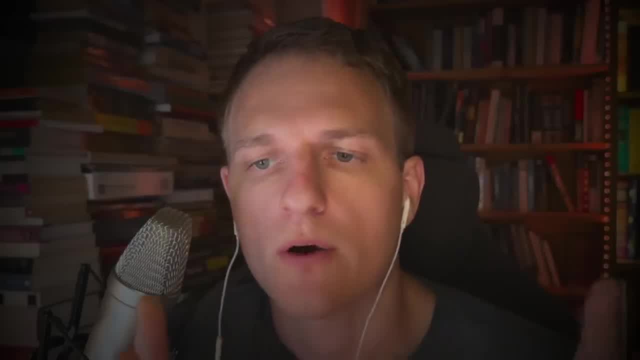 of the stars and over came along a couple hundred years later and he tried to formalize that and saying: well, we can rule out that the universe is infinitely large, full of you know, in an uniform and matter, and that it's infinitely old. if it was all of those, there would be the light from even the most distant stars. 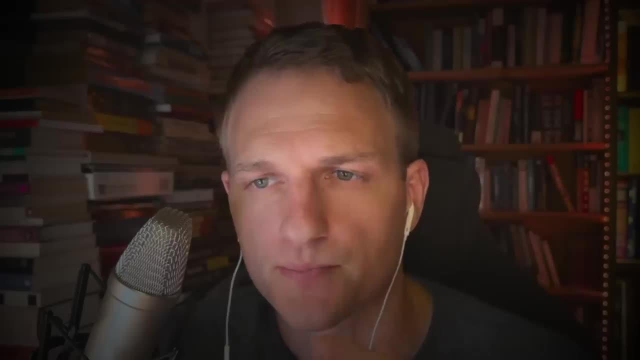 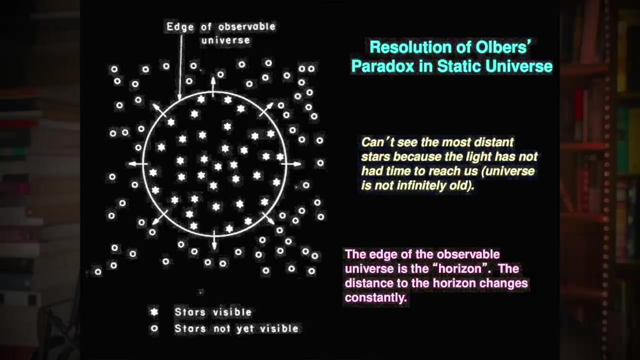 would have had time, because you know at that time they would. they were well by Olber's time, in 1800s, they knew that light had a finite speed. he theorized that the- uh, infinite time of the universe would allowed, would have allowed infinite time for the light to travel and therefore it would have reached our 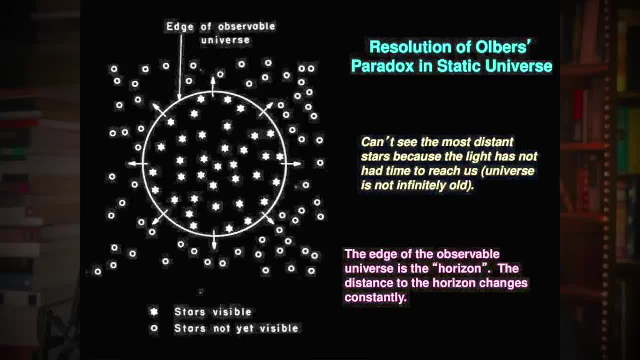 eyes. and if the universe wasn't just a few, you know, a few stars, few thousand stars, and then it just ends into blackness. if there was a continuing field of stars, all those would have contributed to filling up the entire night sky with light. All the black voids anywhere would have at some point. 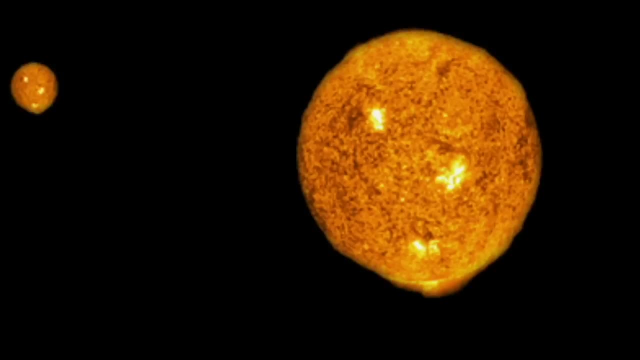 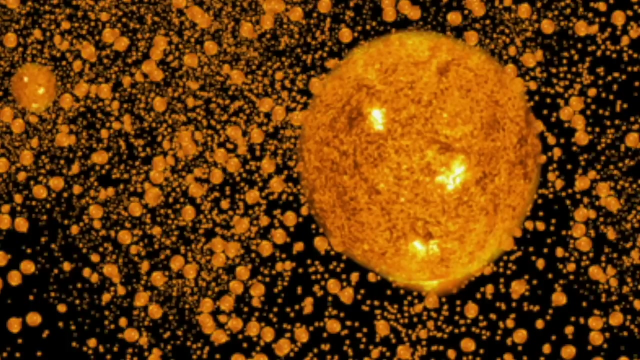 at some distant enough point, been occupied by a star on its apparent position relative to us, our view from Earth, And so we could tell from that paradox, at least logically, the universe isn't old, or at least there isn't a uniform field of stars beyond a certain point. 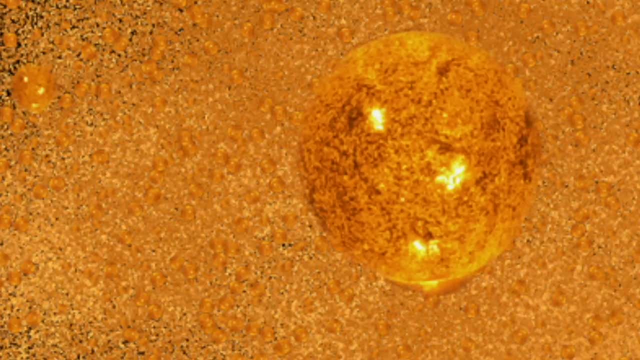 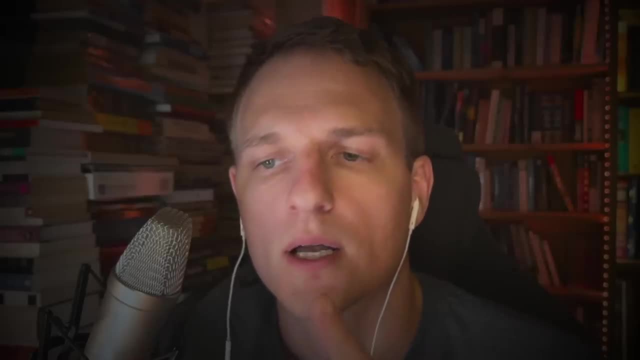 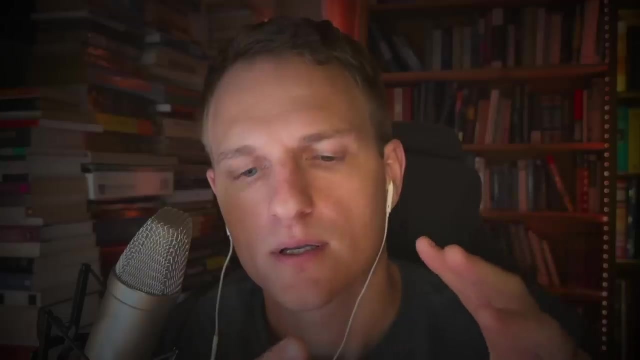 They must end at a certain point, which might mean there's a finite space to the universe too, And so I thought that was a pretty cool idea. It's one of the first instances where we start to view the universe as having potentially other systems. 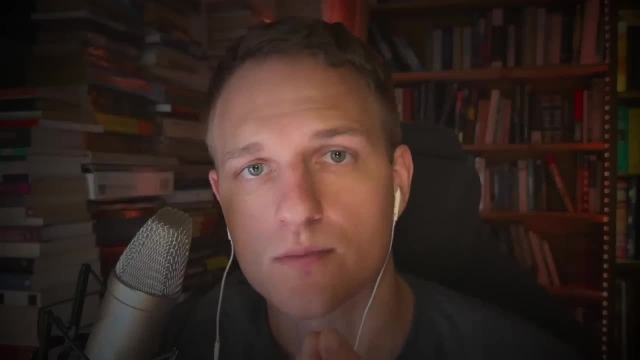 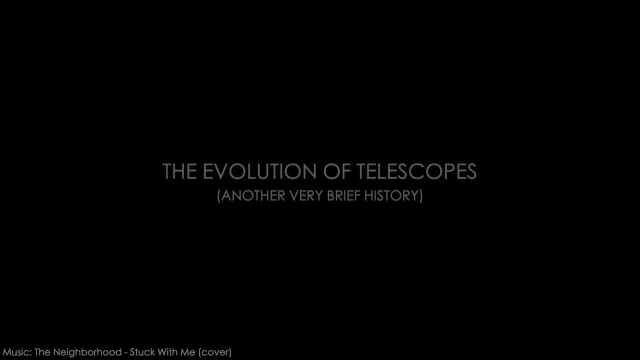 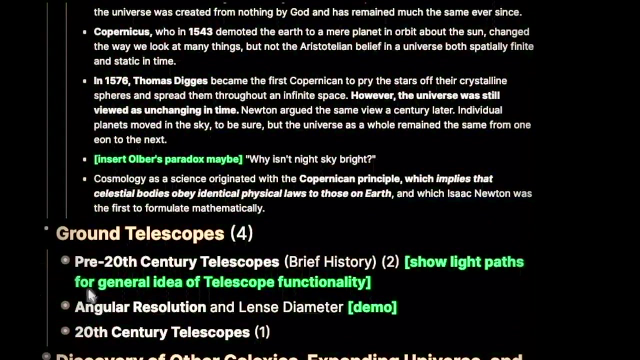 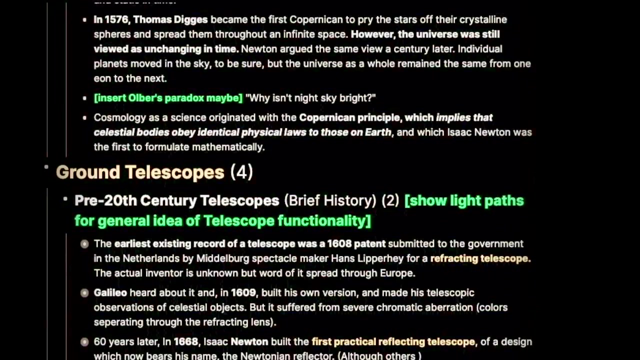 and the stars being other star systems like our own, with planets and at different, varying distances, with glowing suns that themselves might possibly move and not be like stuck statically to this crystalline, unchanging sphere, And cosmology progressed, starting with around Galileo. 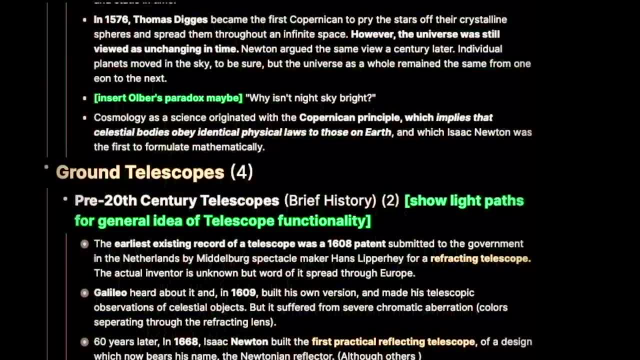 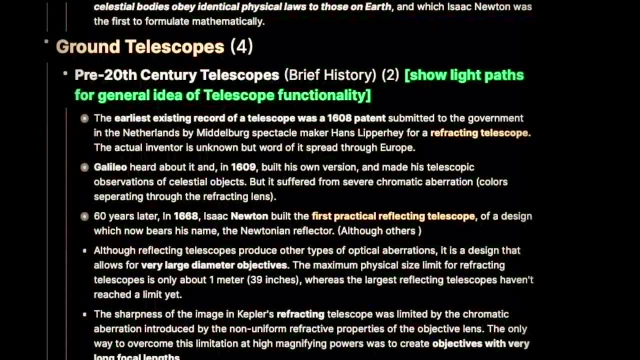 And then, about 75 years after Galileo, Newton took Galileo's. it wasn't Galileo's invention, but he was one of the first to hear of a telescope, you know, a lens being ground so that you could look, magnify distant objects. 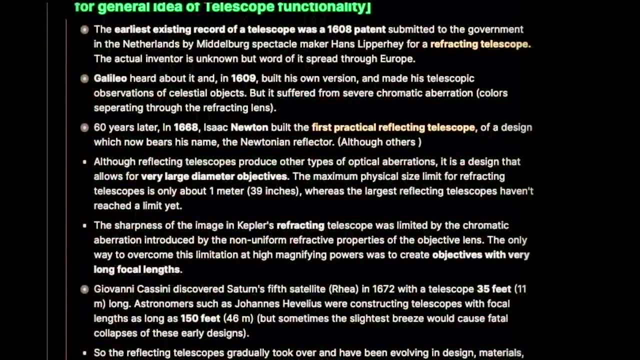 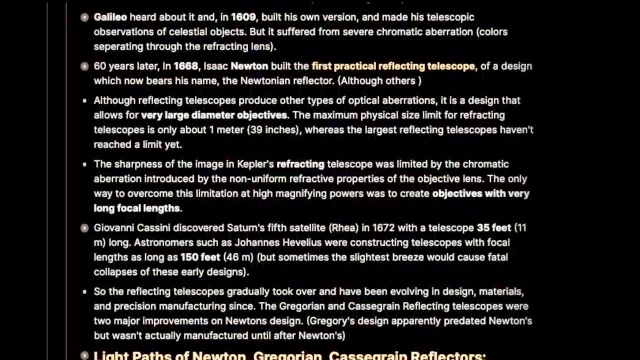 And then Newton, 60 to 70 years later, perfected really designs that were used for the next couple hundred years. after that He came with the first practical reflecting telescope, which meant it didn't just come on, come in straight to, let's see if I got a picture of it here. 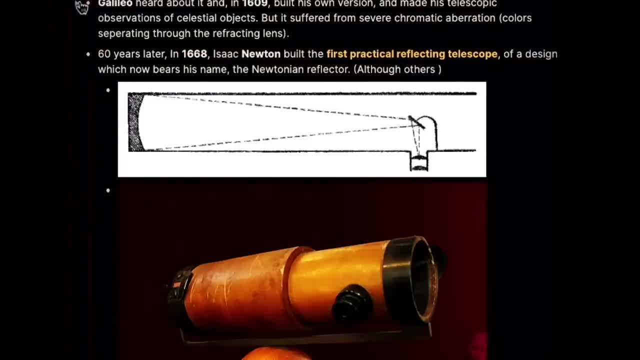 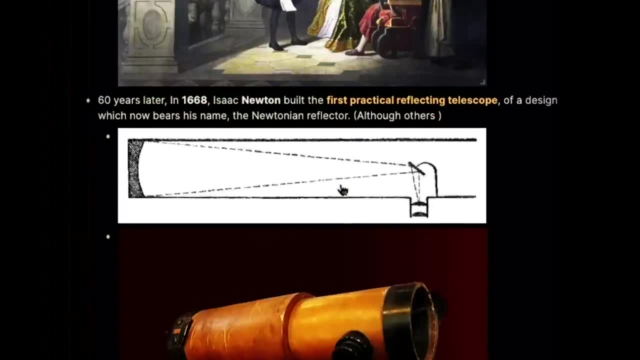 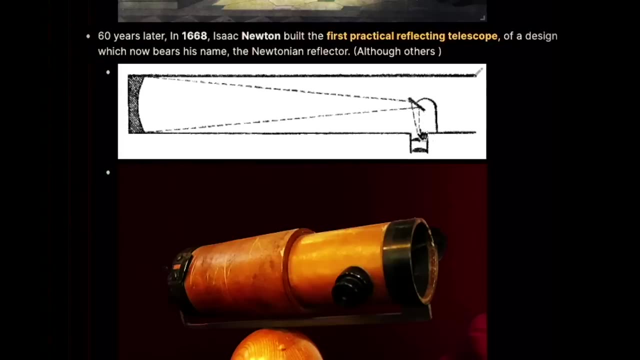 Yeah, it didn't come straight to your eye like Galileo's, So you didn't just point it and look right behind where you were pointing It was actually came in through the lens and got reflected off this little mirror here, in which focused it perfectly on your eye. 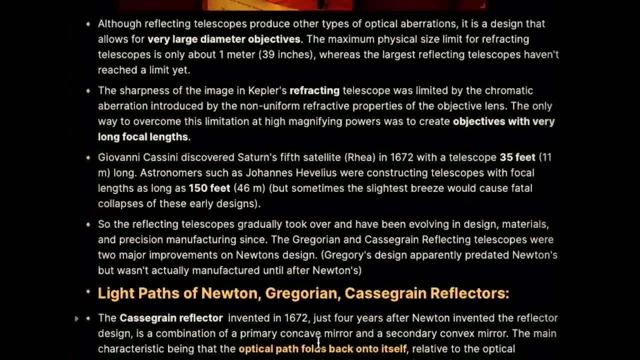 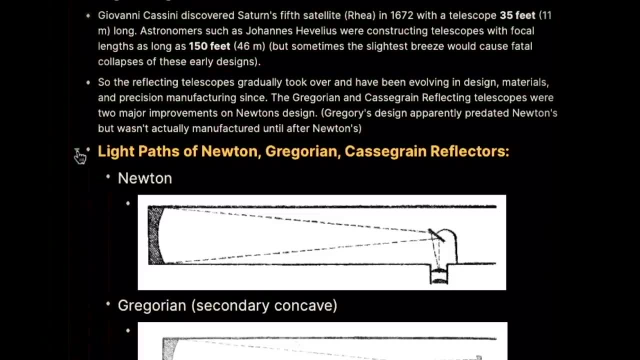 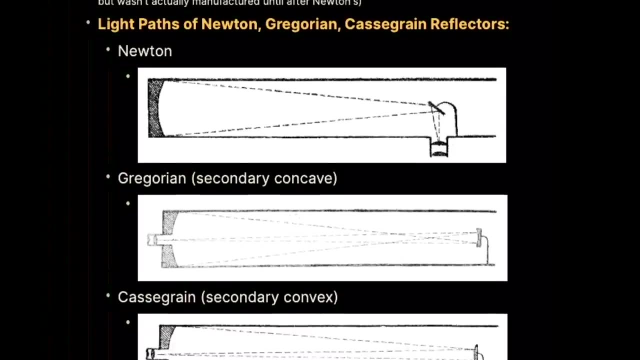 on the side of it. So these eventually got crafted more and more to allow sharper and sharper images. The lenses were ground smoother, They were ground with more magnification, And then we had some modifications like this, where you could actually you had the 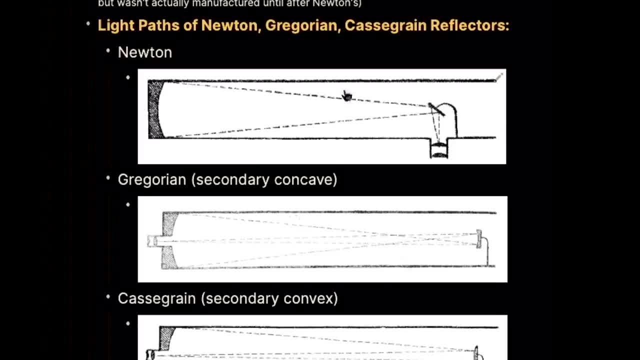 so you had light coming in here, bouncing off there, not quite focusing on here, but this was set up so that the focus would ultimately come right to your eye. The light of the Gregorian telescope developed not too much longer after Newton. These were all in the early you know: 17,, late 1600s, even. 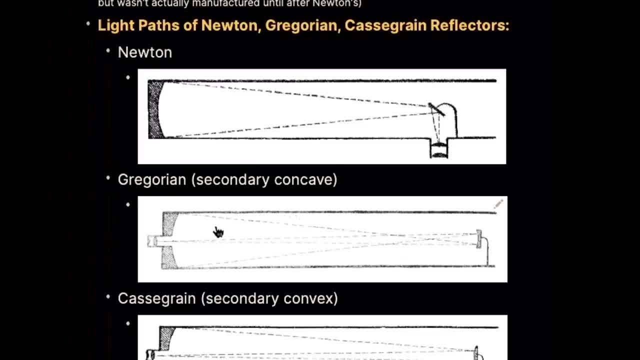 These designs have been around for 300 years or, yeah, even more than that. It's amazing that they're still mostly just kind of elaborated upon. The design hasn't really changed that much, And this one just has a. the light comes in from the right. 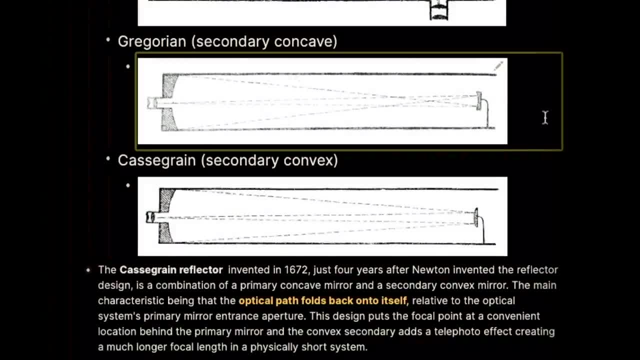 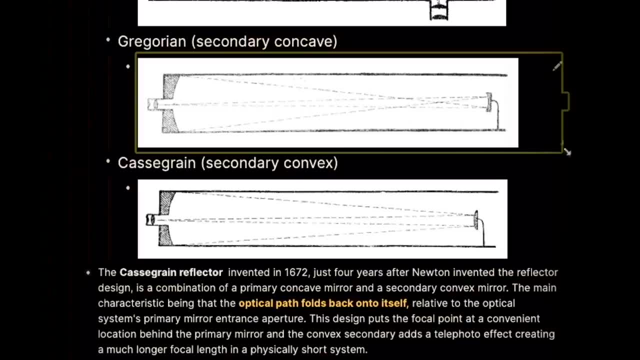 And see if I can make it larger- And bounces back off onto the mirror but then reflects right back to the observer. So it's not a direct. it's built to look like Galileo's refracting telescope, but it's actually a refracting telescope. 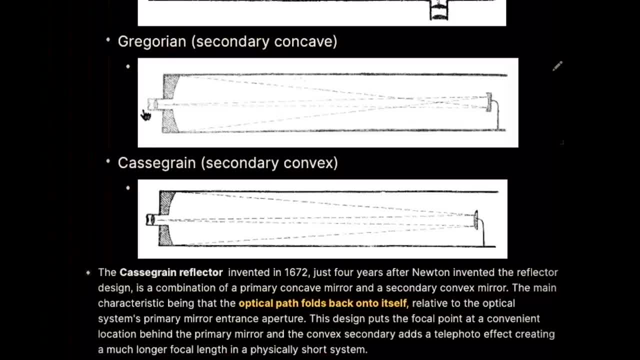 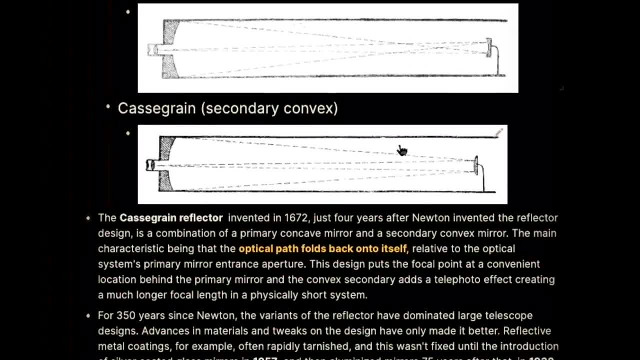 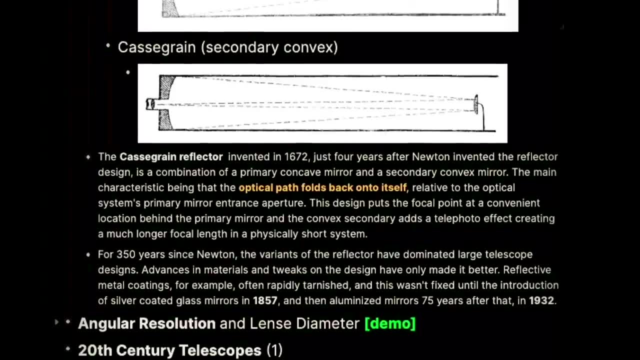 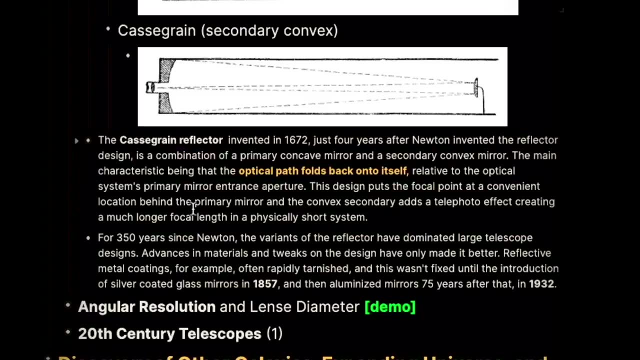 And then this one is the same design except the lenses. the mirror here is concave or convex rather than concave. The Casagrande reflector actually invented in 1672, so even before Newton. And this is actually the. 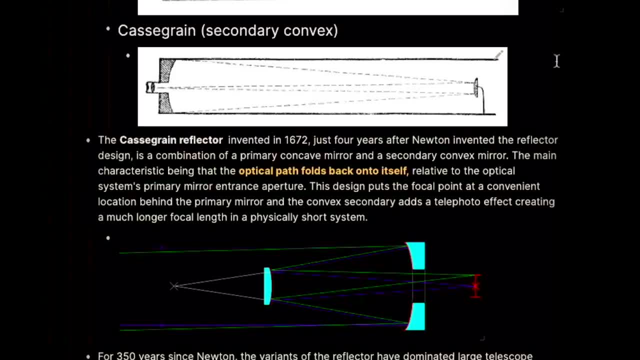 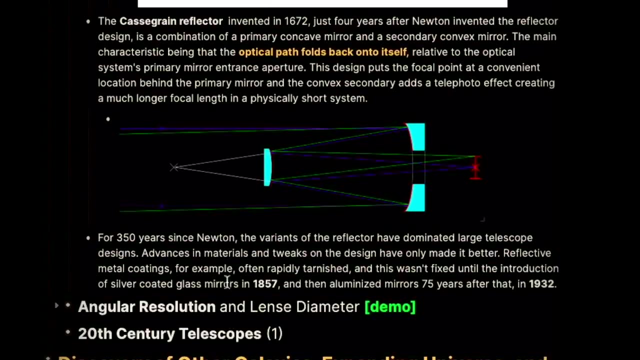 so the optical path, by folding back on itself, allows it to have the same magnification as a hyperlong reflector telescope would. So, other than, like some materials and tweaks on you know, the types of metal they use for reflecting, and glass material science. 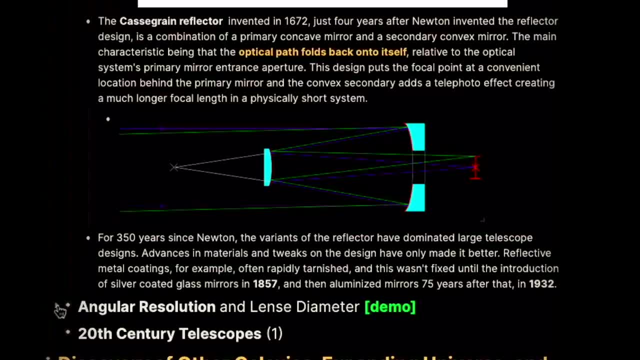 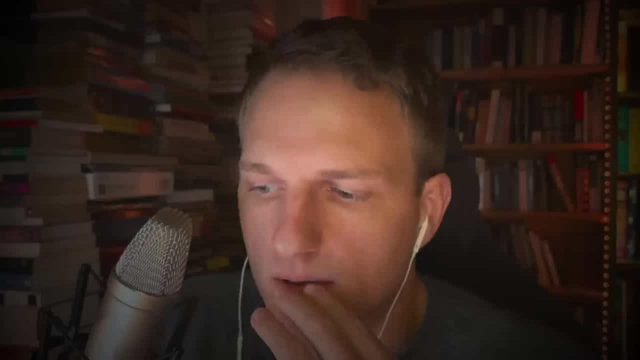 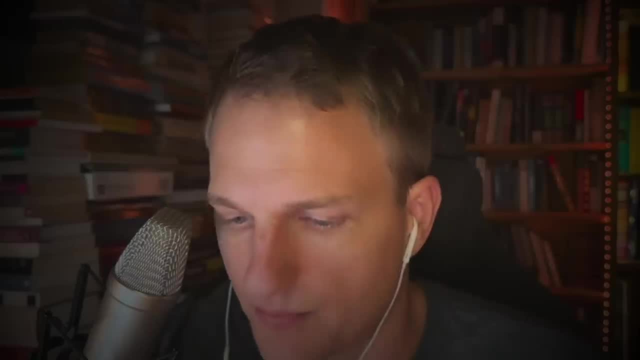 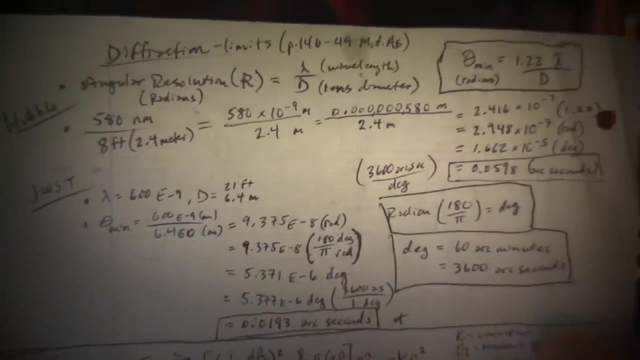 it really didn't change that much for 350 years And 50 years is phenomenal. Now here, we could see the. now, here we could see the. now, here we could see the. so if you guys could see that right there, we see that the. 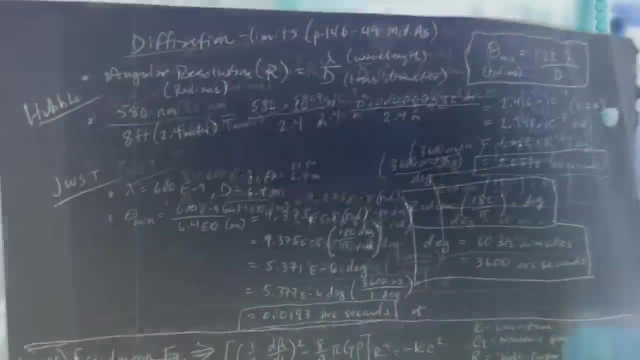 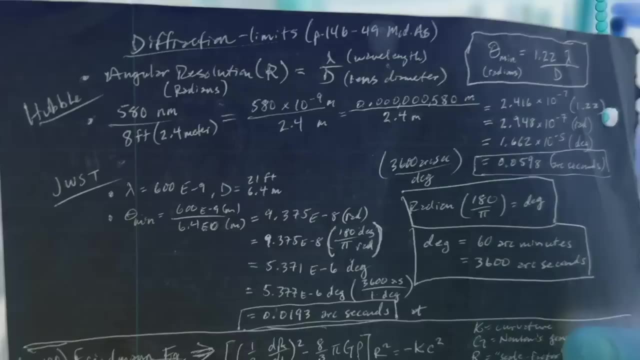 the angular resolution is strictly dependent. The angular resolution is strictly dependent. It's one of the great, you know features of math that we're able to see like a very precise relationship between the lens diameter, the diameter of the Primary lens that's collecting the light, and how sharp the image looks. 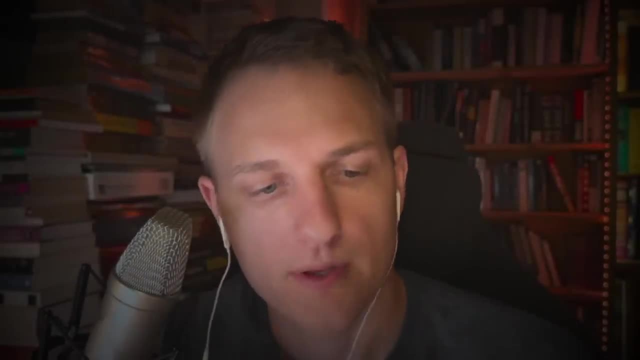 And what we see here is that, You know for Hubble, It has to do with the wavelength too, so it's a relationship between the angular resolution Is the wavelength divided by the diameter of the lens, which means for a smaller wavelength, like visible light, smaller than 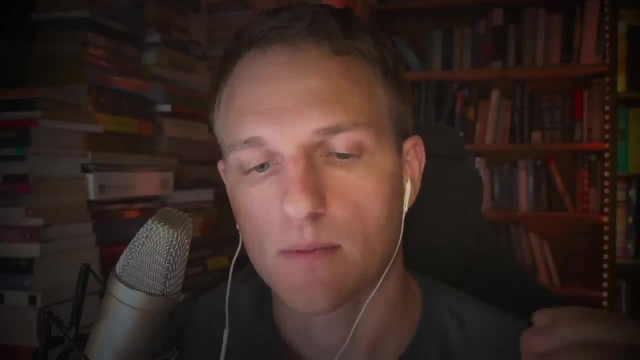 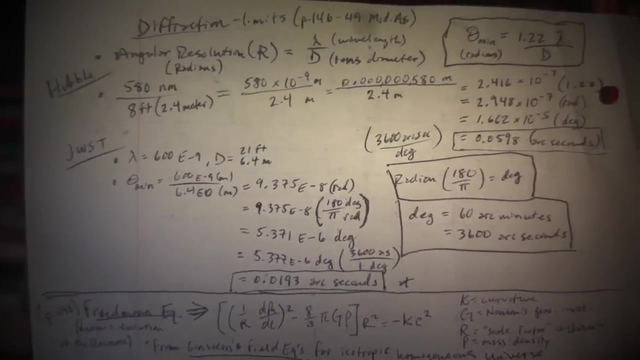 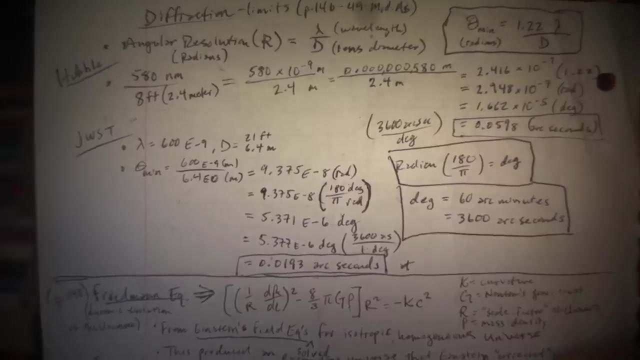 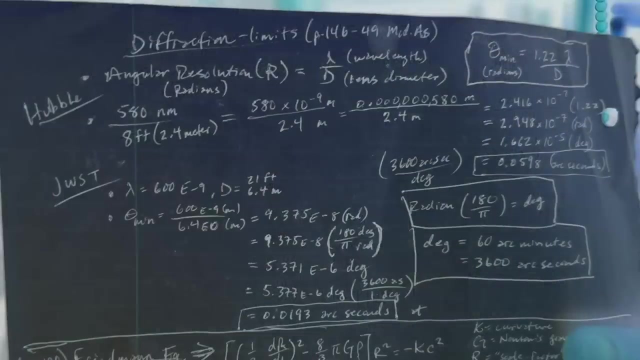 longer wavelength infrared light. that web sees. What you want is to have a smaller angular resolution, Small as possible, so for any given diameter. what that means is that For any larger wavelength you need a larger diameter mirror, or else, as you Get a larger and larger wavelength going out of 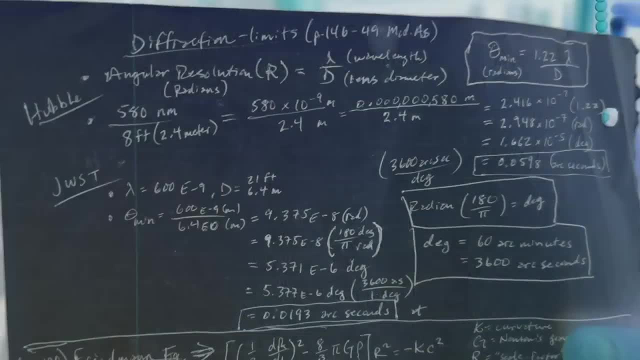 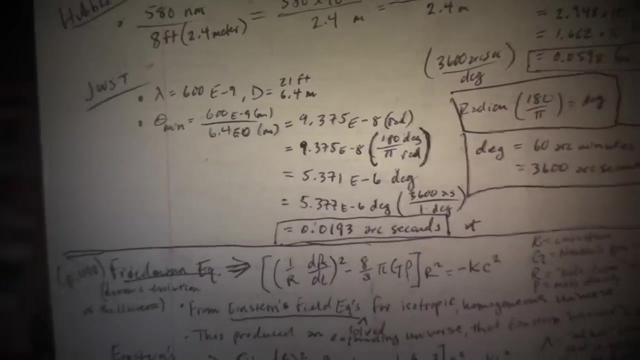 You know, Relative to visible light. if you go to infrared light the resolution will decrease because the numerator is getting larger there. so as you have Infrared light, you need a much larger mirror. then, for instance, Hubble, which is focused on primarily Observing shorter wavelengths from the visible light. so it needs a smaller mirror, but it still needs a. 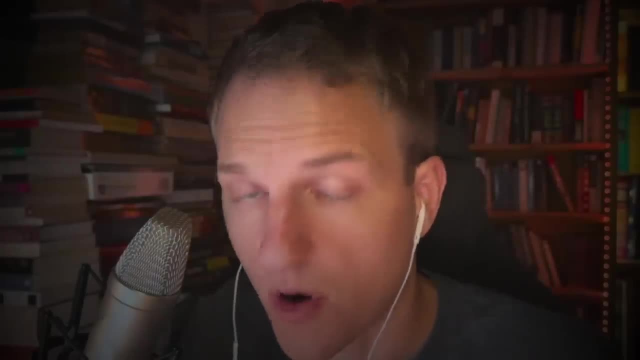 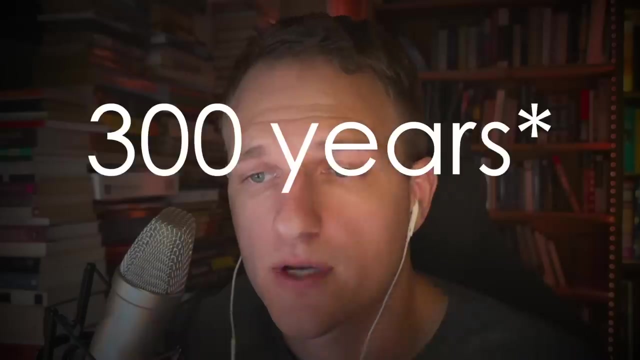 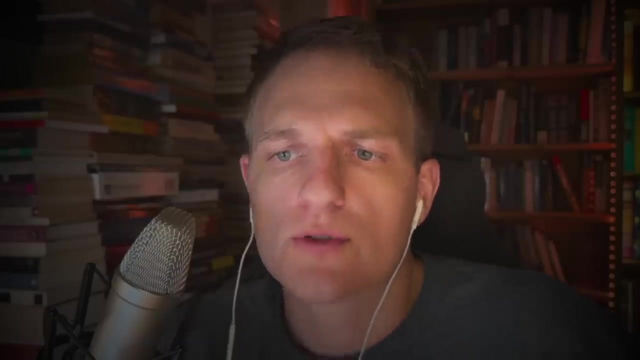 It does need those mirrors to be Polished to within a fraction of lambda the wavelength, which is insane. now How smooth that has. to be so for the last century, last 300 centuries, we've been using reflectors of some sorts, but There's been a new type that the web actually is using, and it's incredible because the 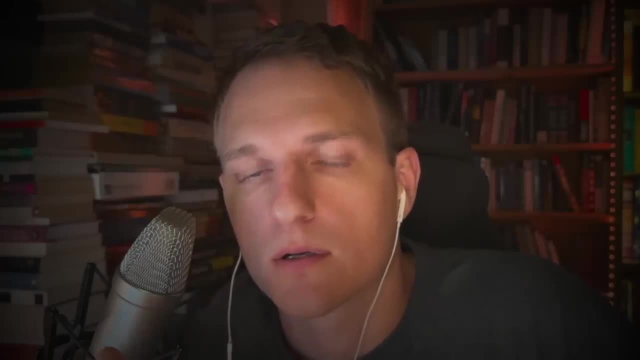 Optics are such that it's able to have the The, the light, fold back on itself so many times that it, for web in particular, It creates the effect of having the same effect as having the magnification, magnification of a Four, I believe, of something like a four hundred foot. 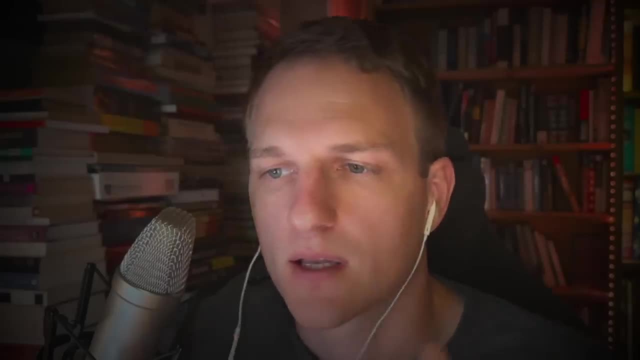 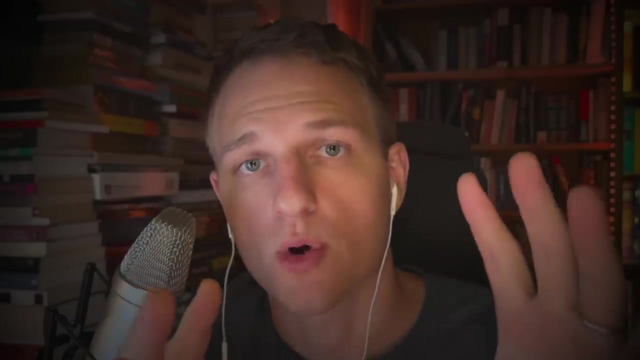 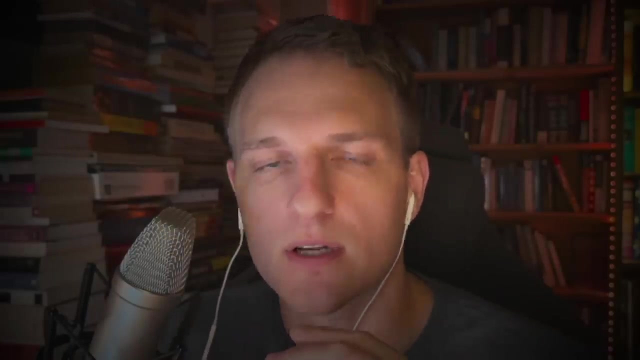 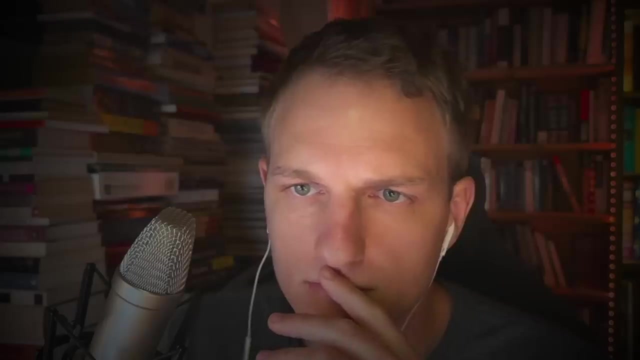 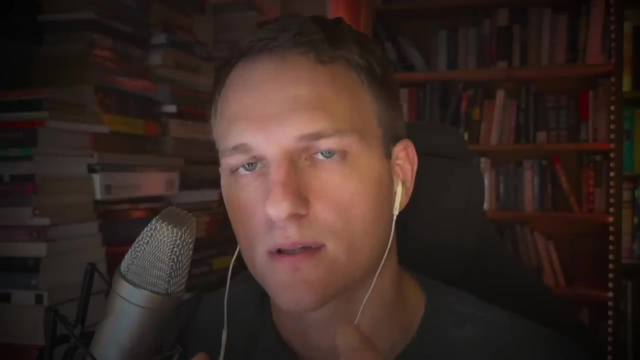 Long focal lens, All within a design of about 20 feet, because it's as the main primary mirror, And then it has the secondary mirror suspended about 20 feet away, Which is giving it just amazing, amazing resolution. and So a quick run-through the astronomy, cosmology that is leading up to 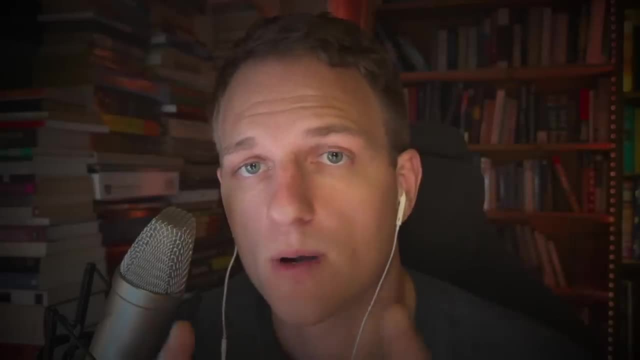 You know everything you're gonna see in the headlines for web and the telescope, Defining galaxies as far back a time and time as it'll be going, Like I said in the intro, every almost every month, You should be expecting web to be making brand new discoveries in the 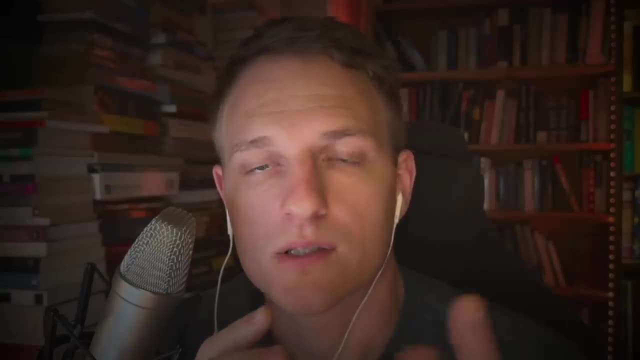 And that's because it's seeing in the eye, Infrared it's, and it has its massive mirror, extremely polished. It has high-tech, state-of-the-art sensors, and We're gonna be seeing things that are changing the way, or It really is. they were trying to. they made a point in multiple articles I read saying that. 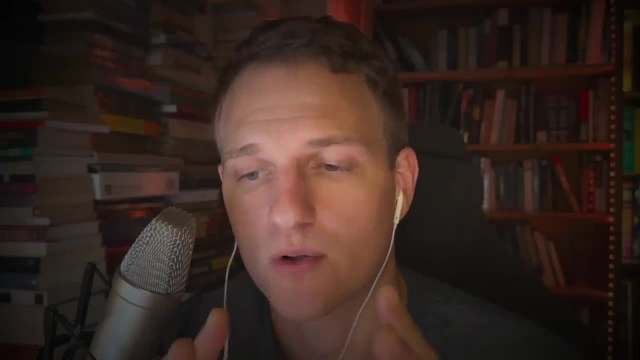 They're not trying to reinforce the status quo of cosmology. They want to just get the best Observations they can and see if the current Cosmological model, called the lambda cold dark matter model- Big Bang model, to complete the whole phrase- is. They want to see whether it stands or falls with the 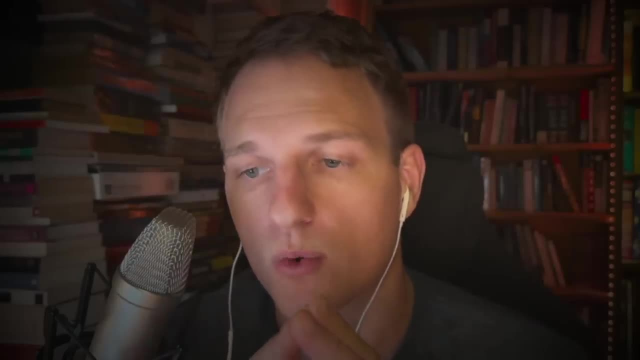 amazingly high resolution observations that web will be Performing, and so I think it's important to understand the background behind our current understanding, our current theories of Of how the universe came to be. I mean, why we think it came from the Big Bang, Why don't we think it's just a steady state, and it's always been that way. 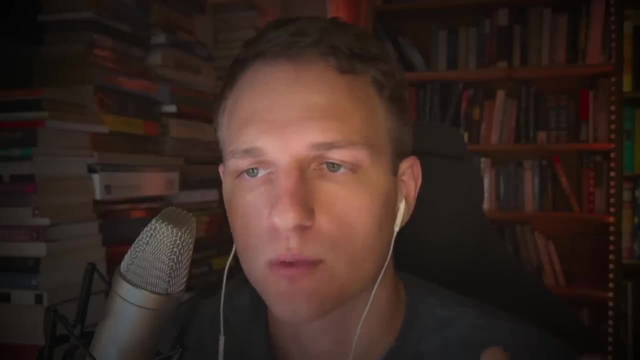 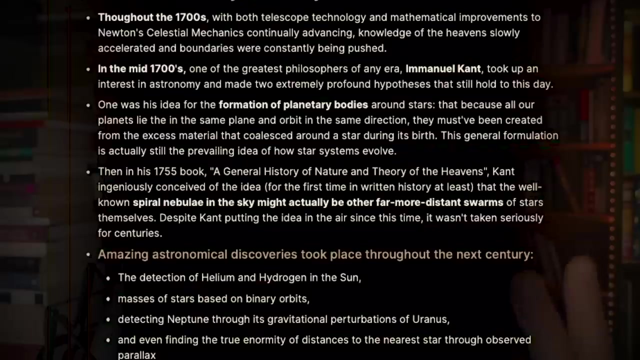 How we think galaxies evolve, stars, how exoplanets are made, how many other earth-like planets there might be out there. And then, of course, how many? how many alien species on different planets would that possibly mean there might be? How much time? how many other? 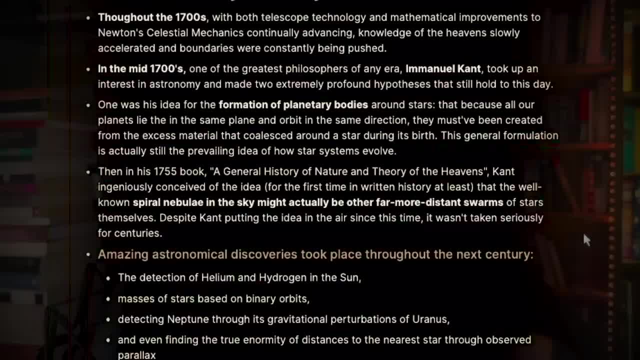 Galaxies are similar to ours, it turns out we're we're actually in a pretty unique galaxy. most of the galaxies in the universe rely Lie within these massive super clusters, and they have these, these elliptical Features that mean that star formation is fairly non-existent in them. It's already, they've already developed most of their stars already. 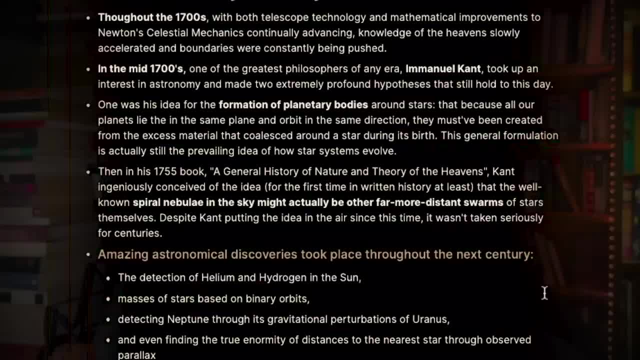 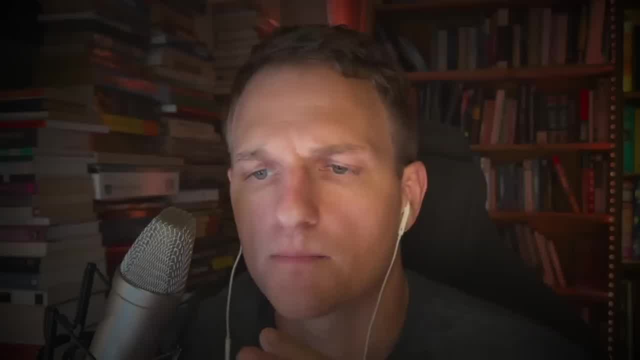 already and turns out the spiral structure we believe that we exist within. that our Milky Way is is a transitory phenomenon in in galaxies that are able to still have star birth ongoing, the waves of the arms- the, rather than the arms of the spirals, create waves and shock waves of. 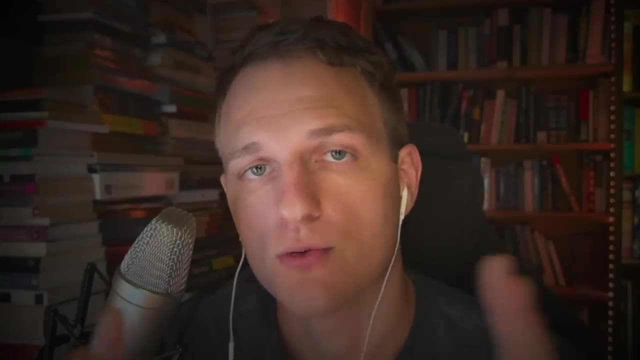 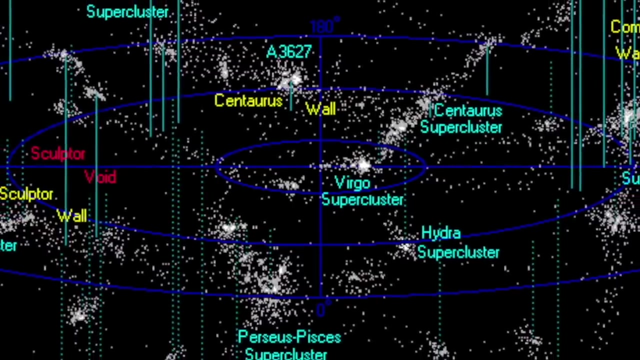 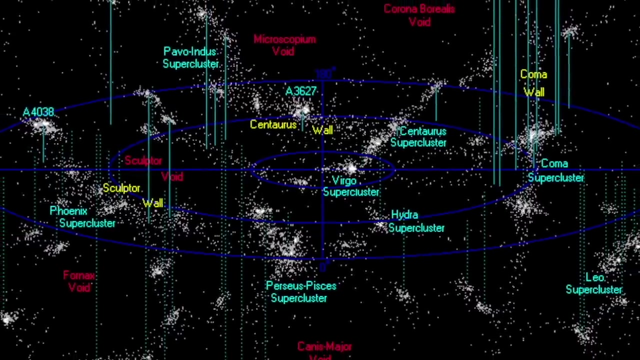 energy that hit these fields of stars, That create new stars to be birthed out of nebulae, of course, all happening over hundreds of millions of years. but It turns out that we actually lie on a galaxy That's pretty far away from any core of these super clusters, as we'll see. 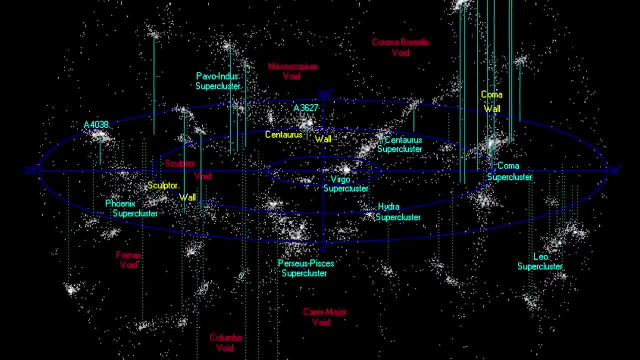 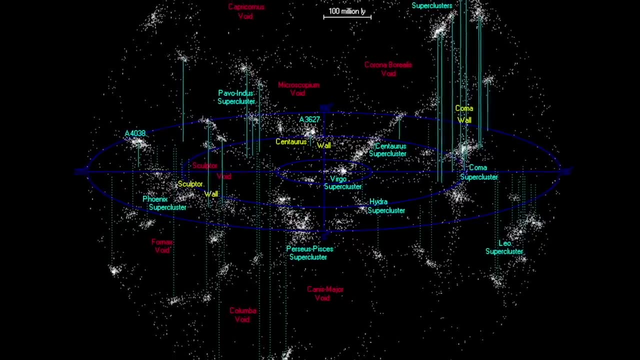 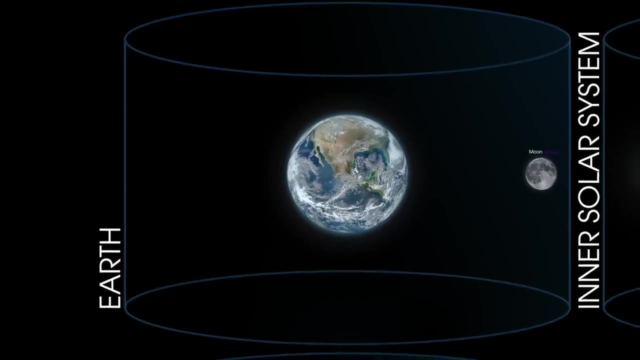 It lies kind of on the edge and we have these huge voids, billions of light years or Hundreds of millions of light years across within this foam like structure, and we're actually More on the outskirts of that than we are close to the center of any one of these huge 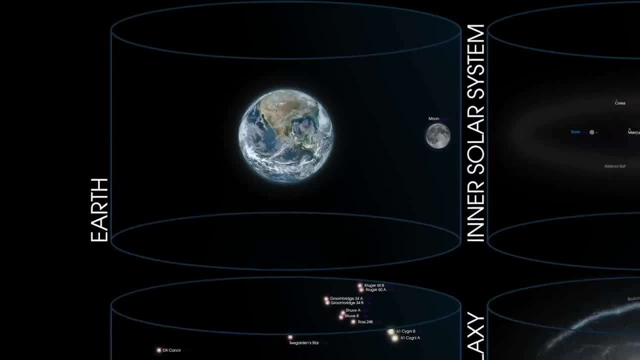 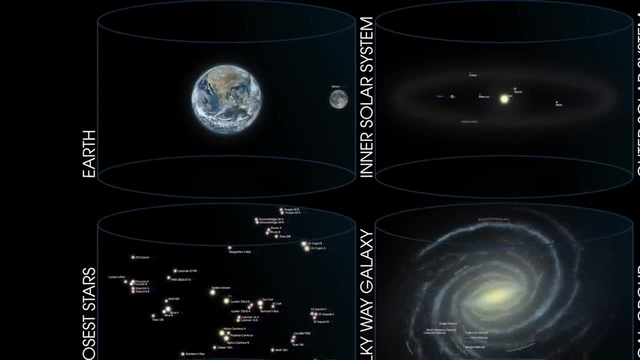 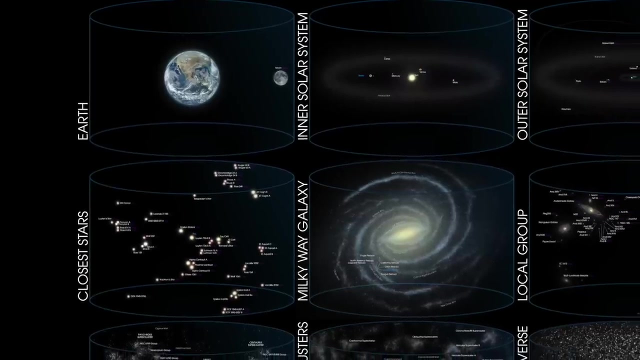 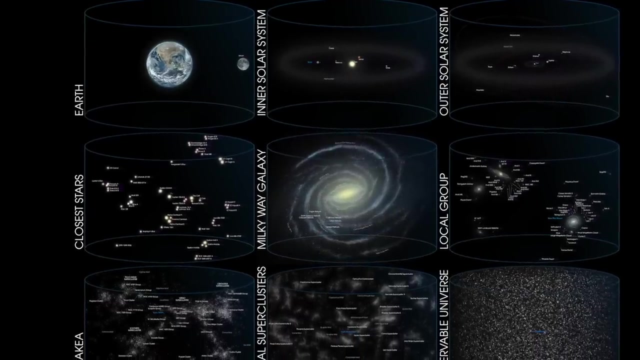 these dominant super cluster nodes that we see, and So we're outside from the fray. and then not only that, our galaxy in particular is very habitable to life, so It's not likely we're gonna see aliens outside Of our galaxy, but within the billions of stars within our galaxy. It's very interesting to know that. 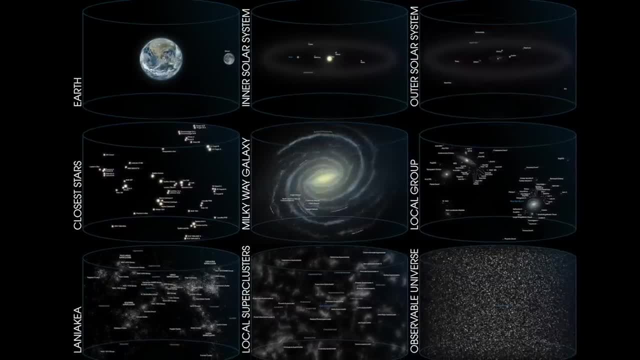 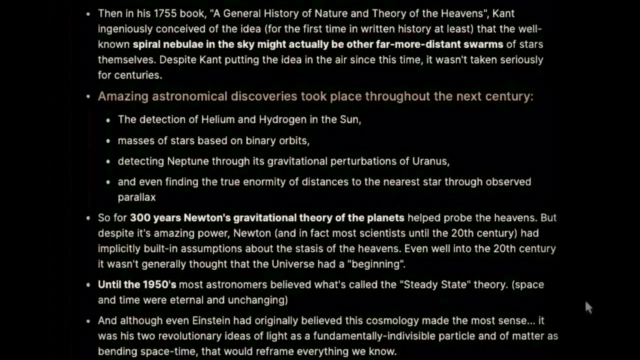 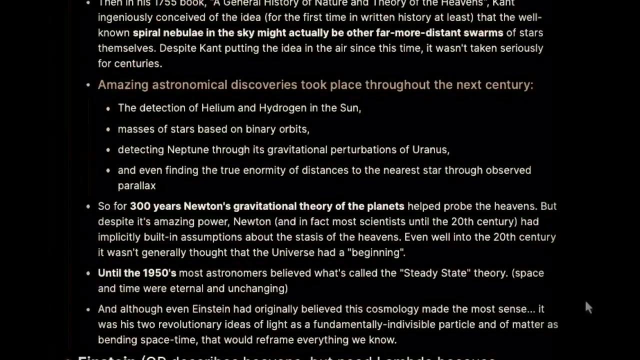 We have a very hospitable galaxy relative to many in the universe. Yeah, it's just amazing all the, All the discoveries we've been able to perform over the last Few hundred years of scientific investigation, and we've been able to detect Helium and hydrogen in the Sun, the masses of the stars based on binary orbits, and how they perturb each other's gravity. 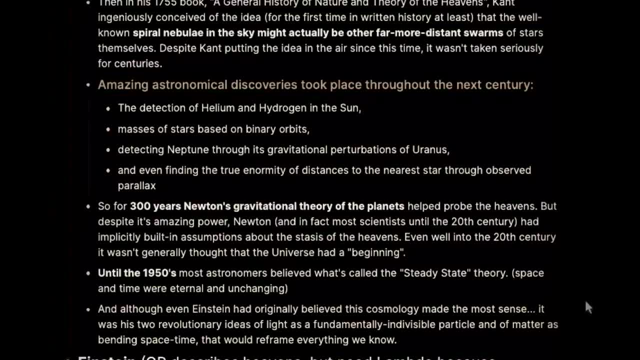 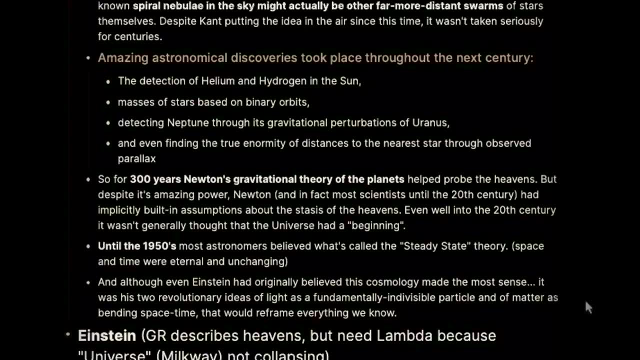 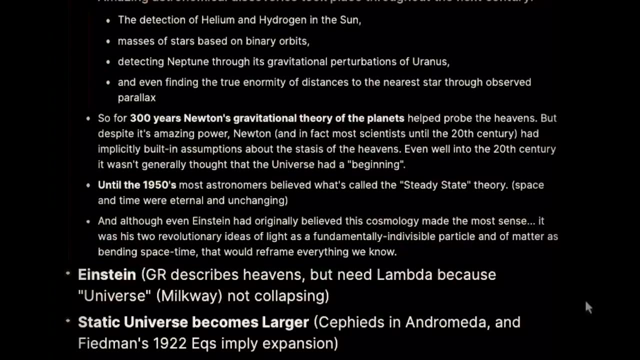 how gravitational perturbations Alerted us of the existence of a planet beyond Uranus, which ended up being Neptune that Herschel actually discovered- same guy who discovered infrared radiation- and Even in detecting the parallaxes. every six months we orbit the Sun and You can see my scale of the universe video for a little demonstration on parallax. how. 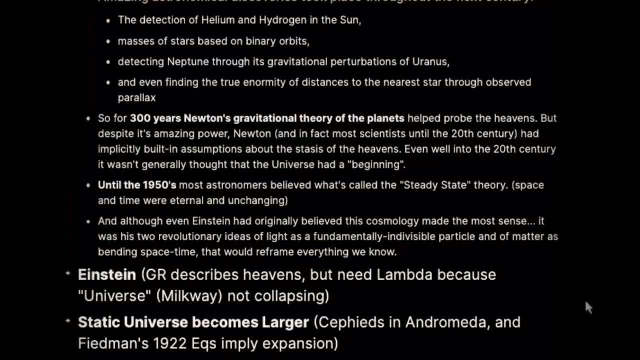 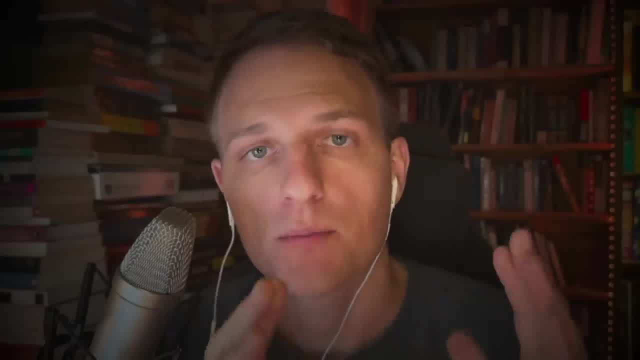 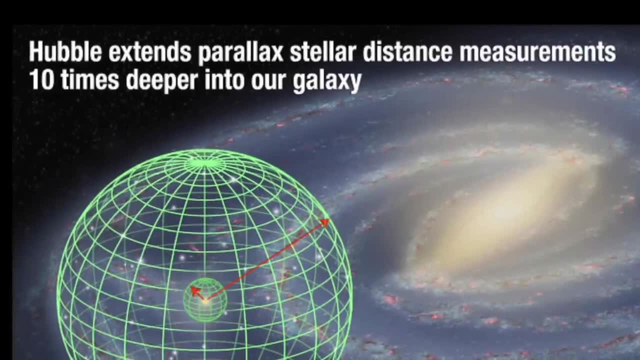 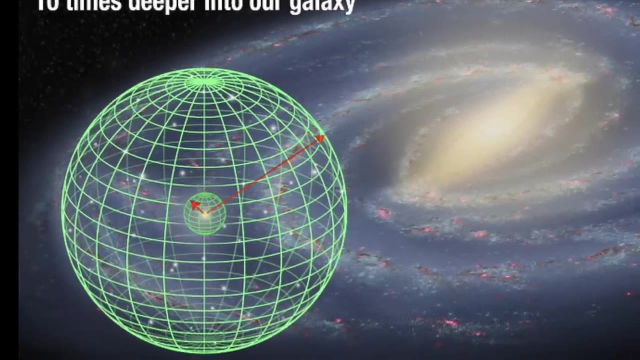 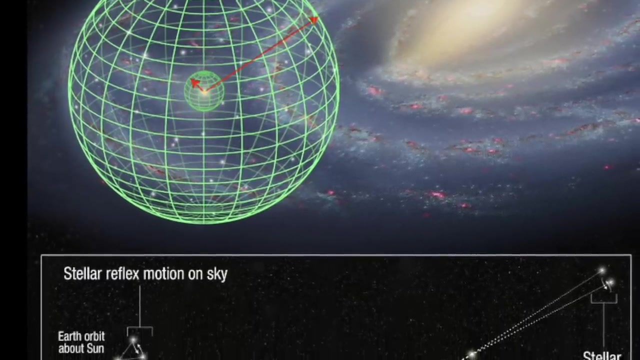 Amazing of a tool that really is to be able to see how Some trigonometry can give you the distances. and we have enough high precision telescopes now. Oh, Hubble was actually key in doing some parallax research to let us know the true, unequivocal distance to some of the most nearby stars, based on how it orbits around the Earth, or rather how it orbits the Earth along with the Earth in its orbit around the Sun. 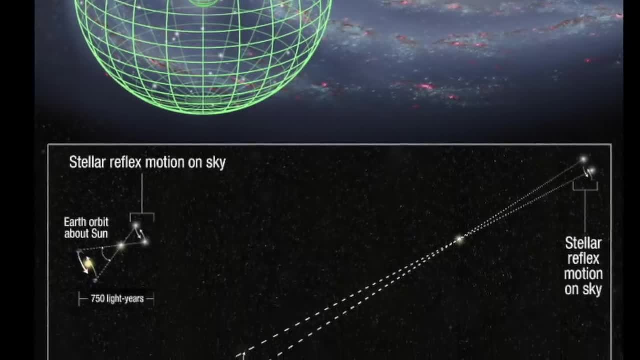 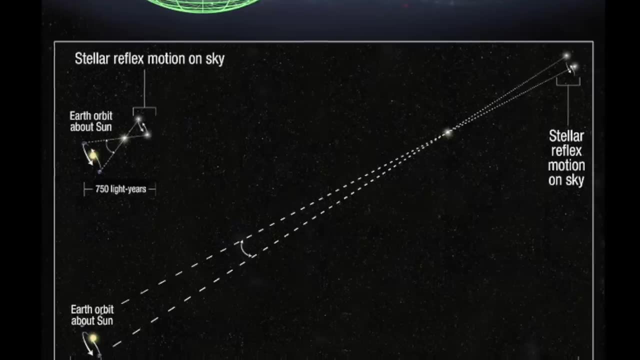 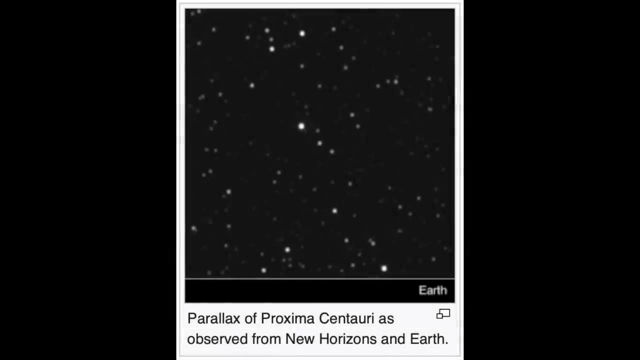 So every six months, Hubble is able to look at the same star and see a slight shift in the background stars relative to this nearby star, And so it's been able to vastly expand our knowledge of just how distant space is between the stars in our local neighborhood. 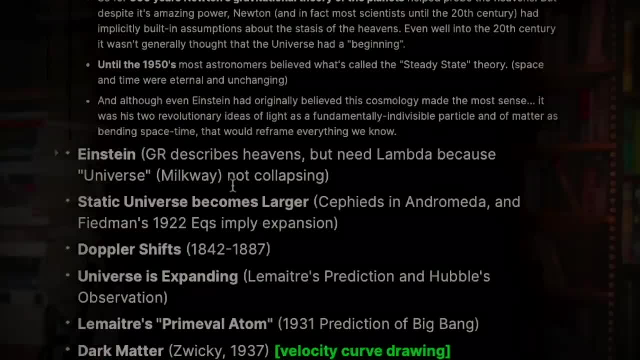 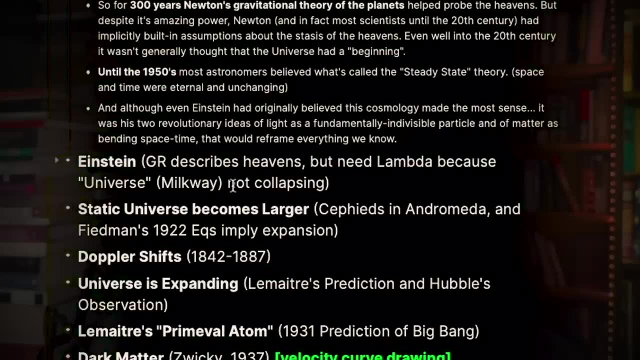 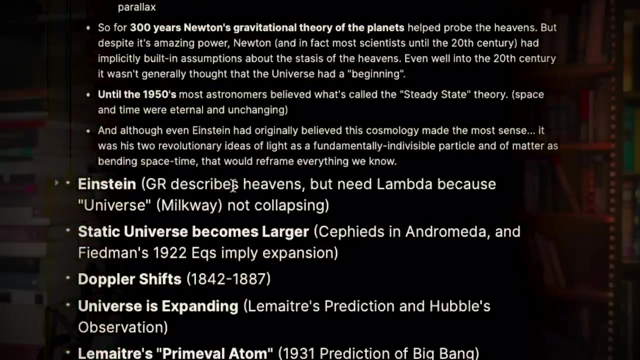 But really for 300 years, Newton's concept of gravity, his theory of gravity, dominated science and our understanding of astronomy. It was extremely effective and it explained everything in the solar system except Mercury. Mercury had an anomalous orbit and what that ended up being was an effect. 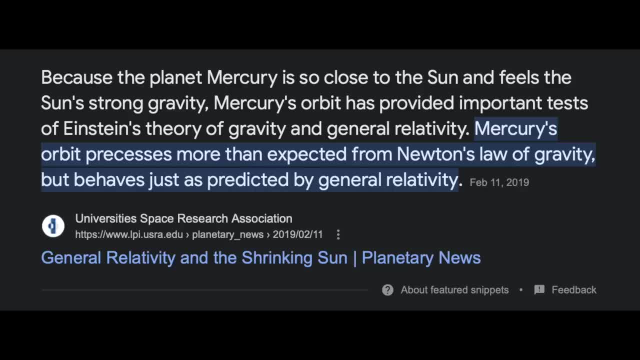 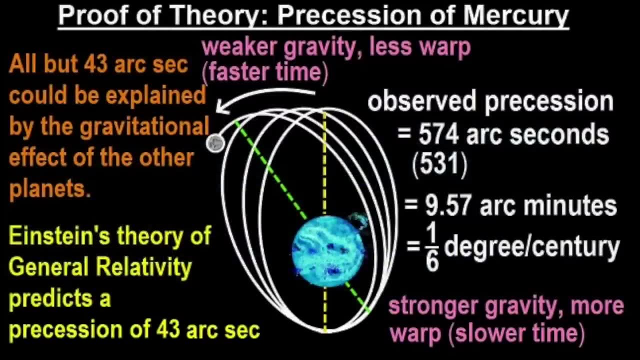 It was an effect of relativity, because Mercury is so close to the Sun that it's actually within the realm of observational relativistic effects from the Sun's gravity being so massive that it bends time and bends space around it in such a way that Newton's gravitational theory had not accounted for. 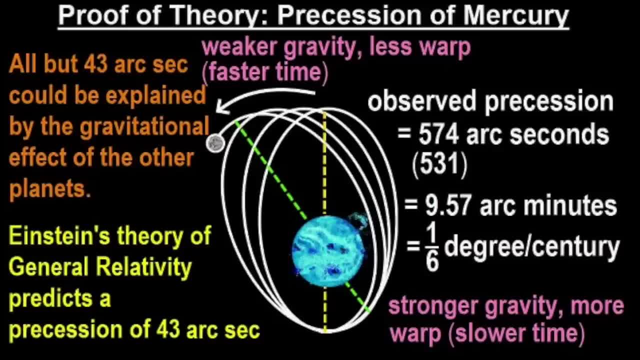 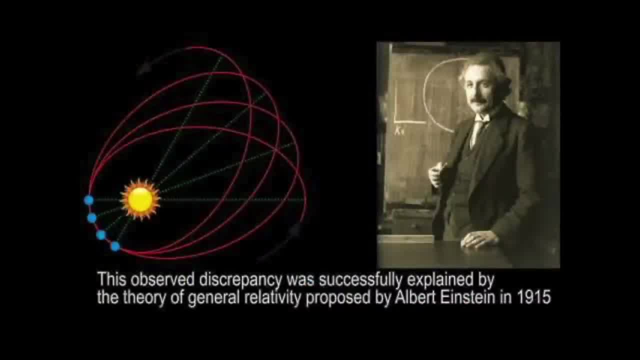 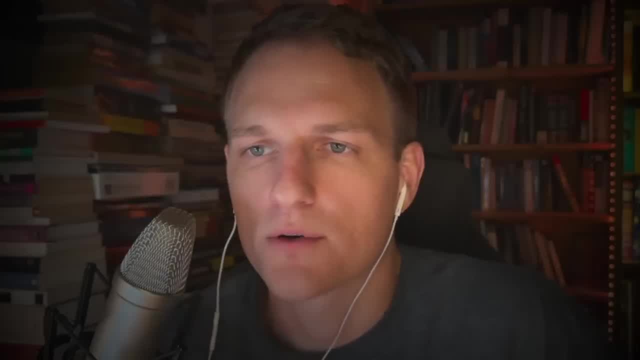 So there's a small variation, kind of a wobble in the procession of a- Yeah, I guess a procession of the elliptical orbit of Mercury. But that fit the model perfectly. But it was still amazing that it took 300 years to do. 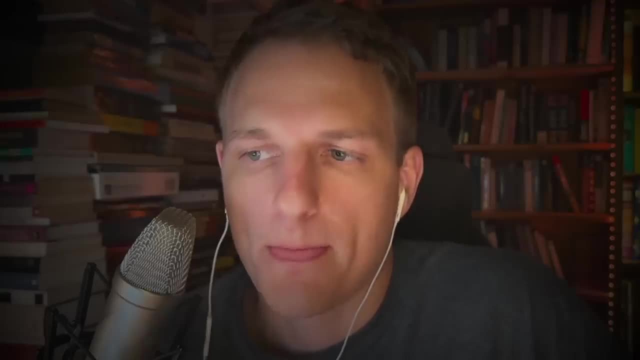 And what's maybe even more amazing is how, within that 300 years and even after it, even after Einstein comes, we have these conceptions of the grandest scale Of the universe, And one of them was this steady-state theory. Many, including Einstein, believe it or not, held on to a steady-state theory for a long time. Even after the expansion of the universe was discovered and the expansion of the velocity of galaxies traveling away from us was found out, we believed that the universe didn't come from anything. 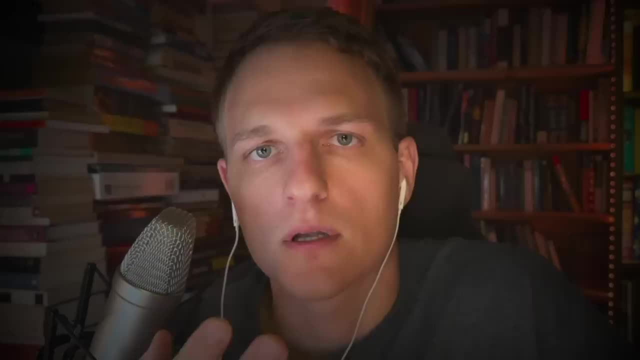 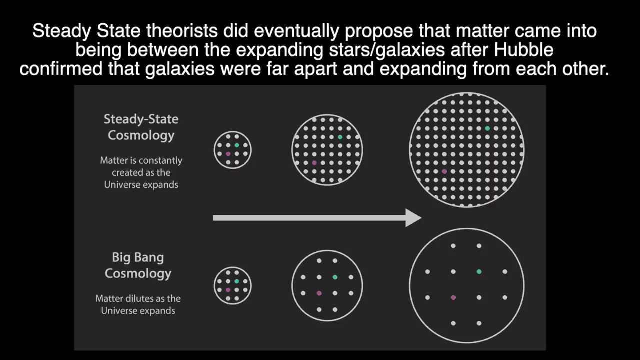 You know, it was just God. Einstein, in a religious context, had created the universe, And so it was unchanging. It was static. The galaxies were wherever they were, The stars remained where they were. Only the solar system had dynamism to it. 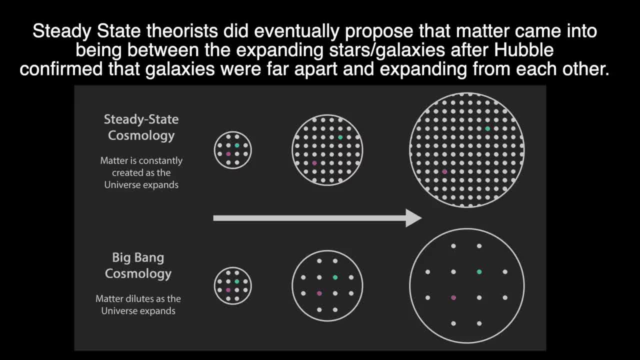 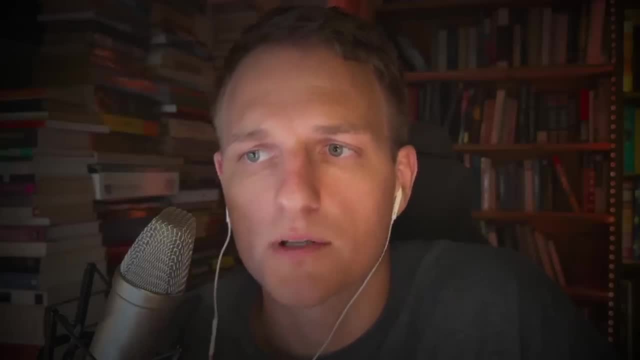 So Einstein initially even believed that this cosmology, this steady-state, infinite, you know, infinitude of cosmology, made the most sense. But it was his own two revolutionary ideas: The one of light as a fundamentally indivisible particle, a photon. 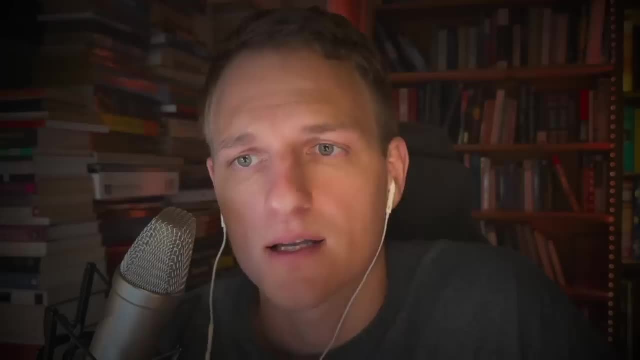 and of matter as bending spacetime And, of course, causing light to bend with it. That would reframe everything we know. So Einstein's new physics coming out of deep thought was the first of its kind, And it was the first of its kind. 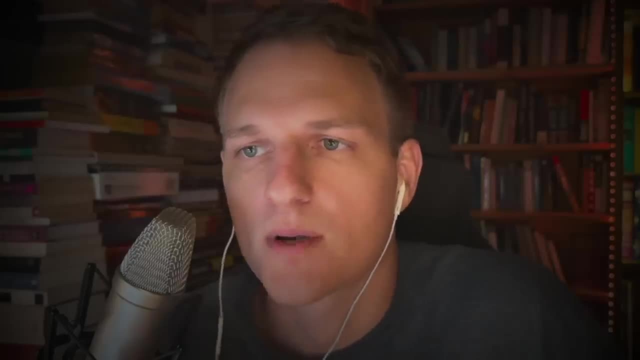 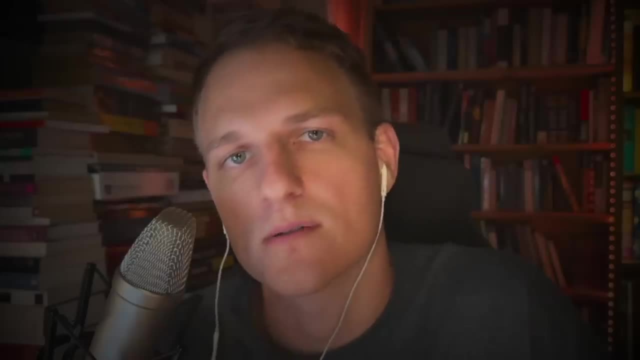 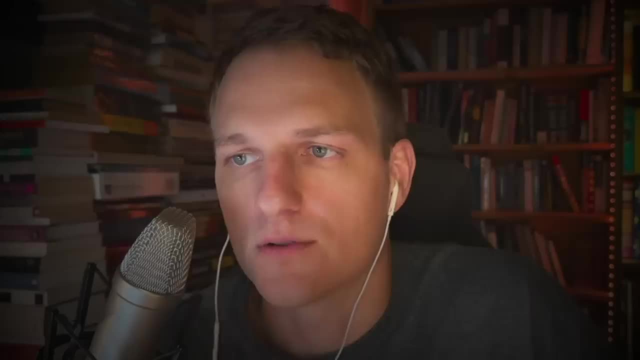 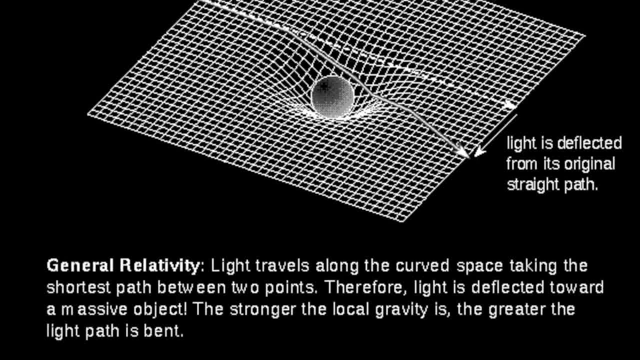 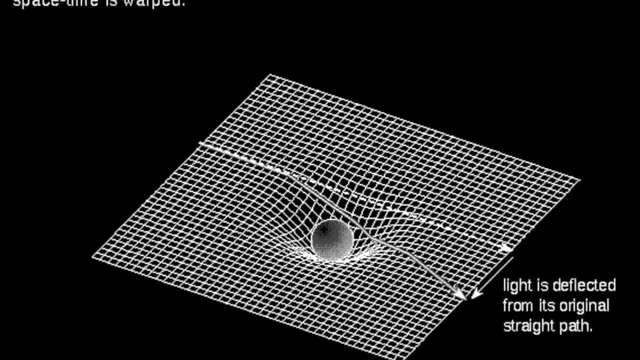 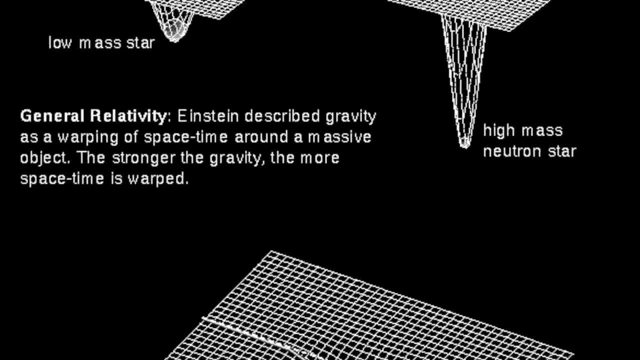 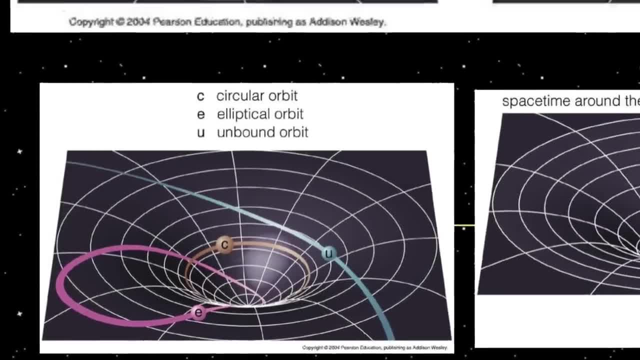 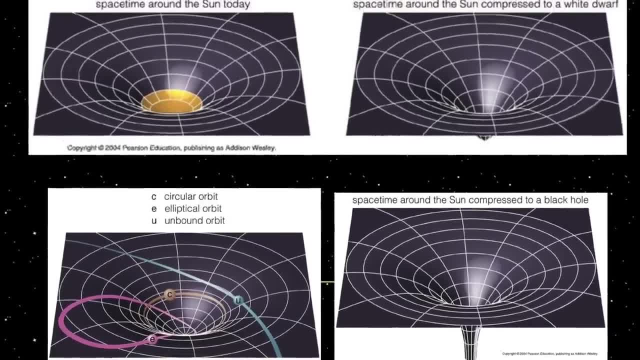 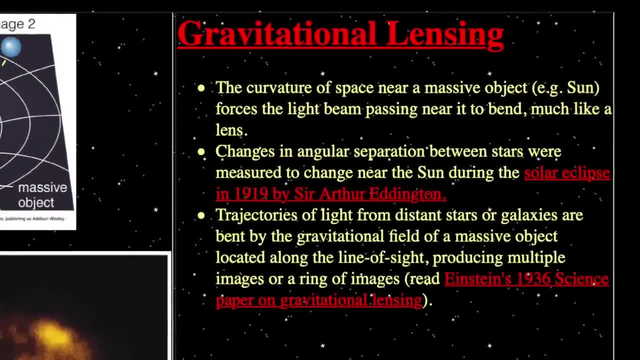 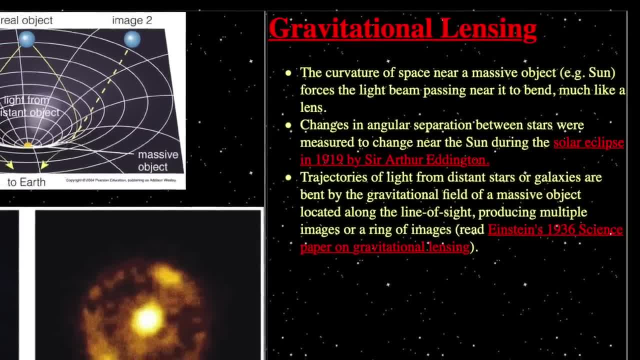 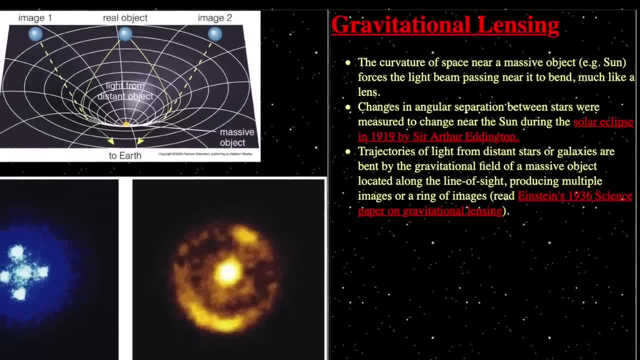 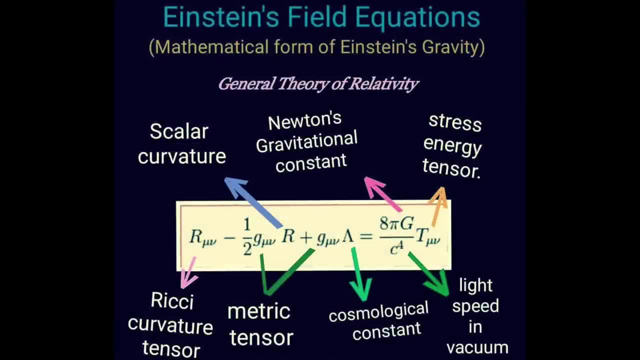 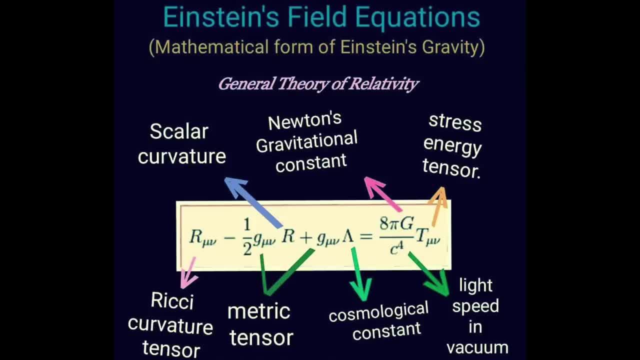 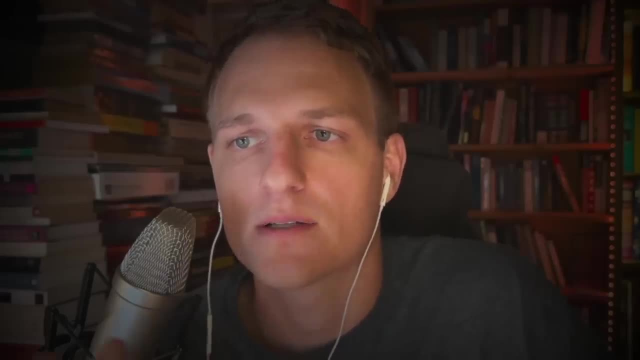 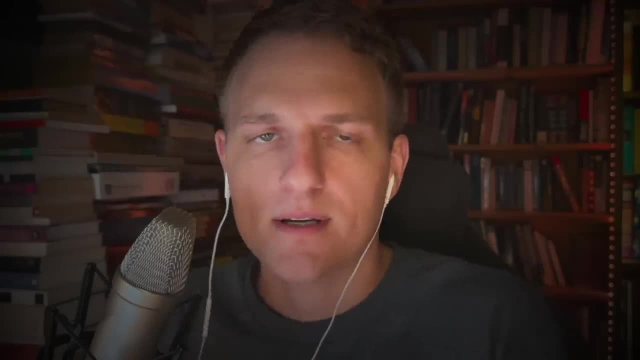 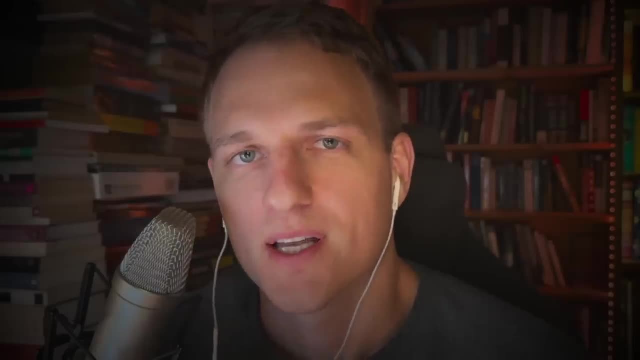 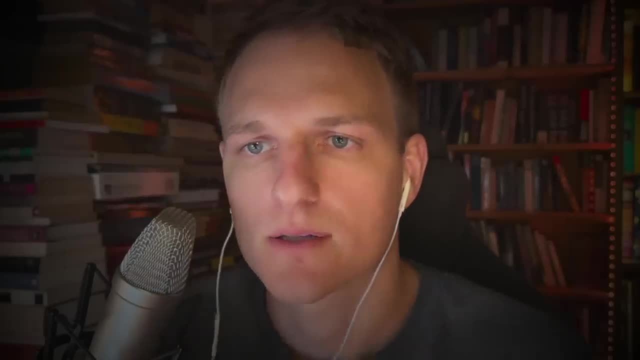 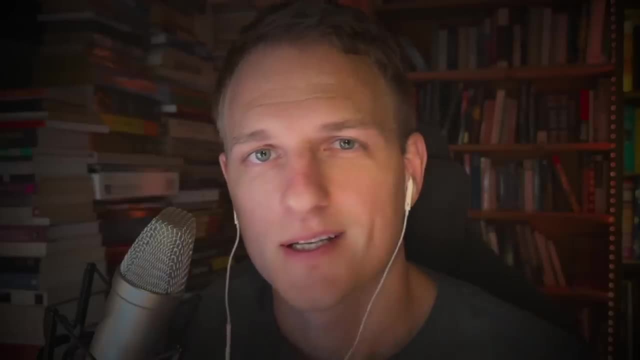 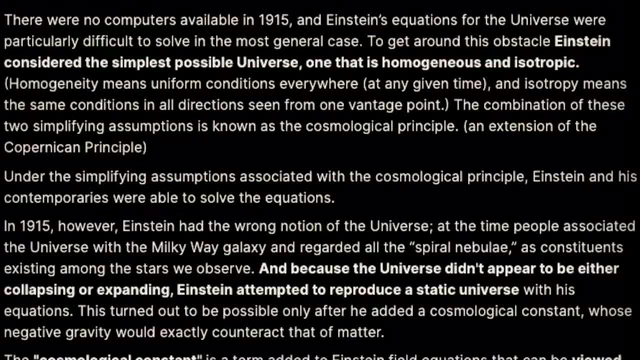 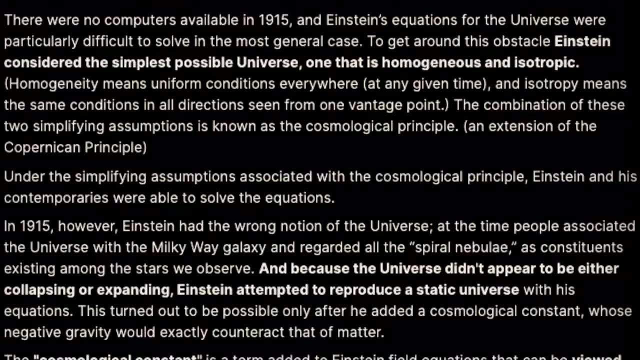 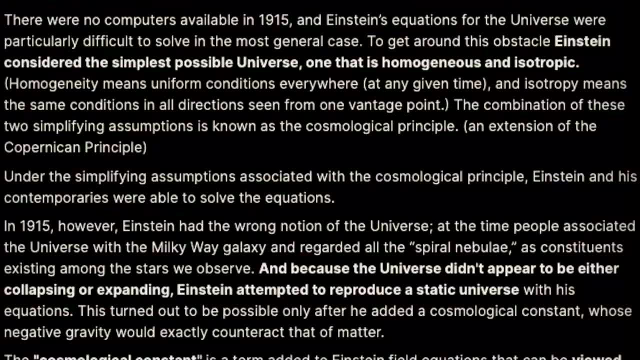 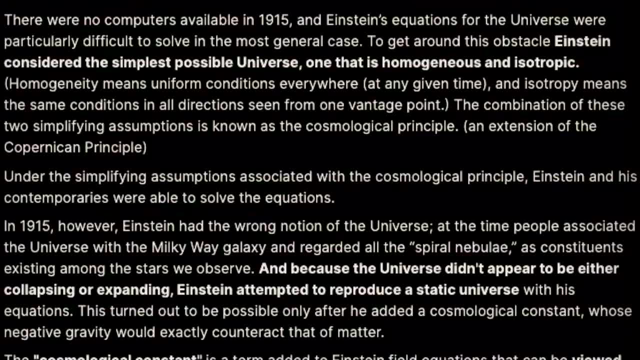 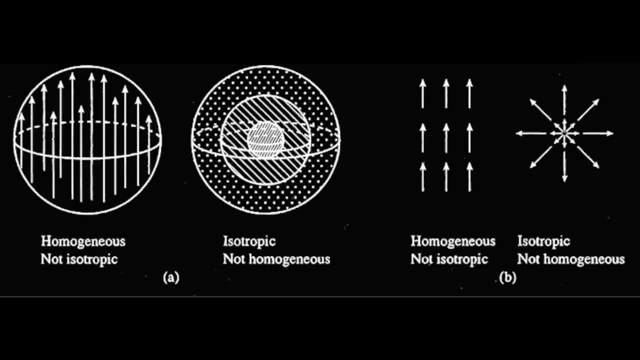 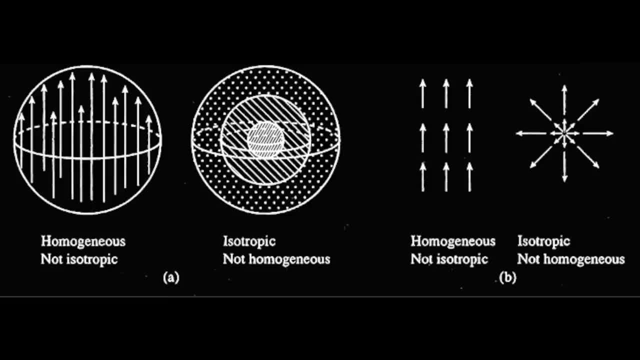 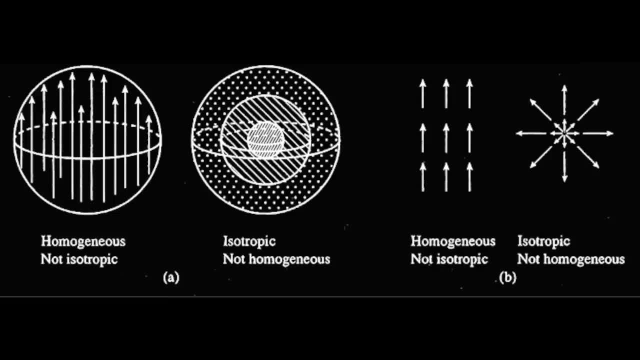 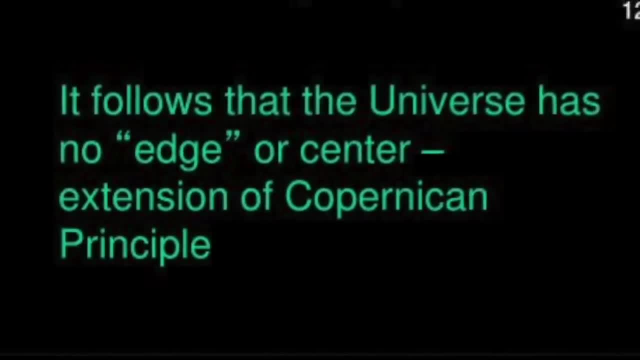 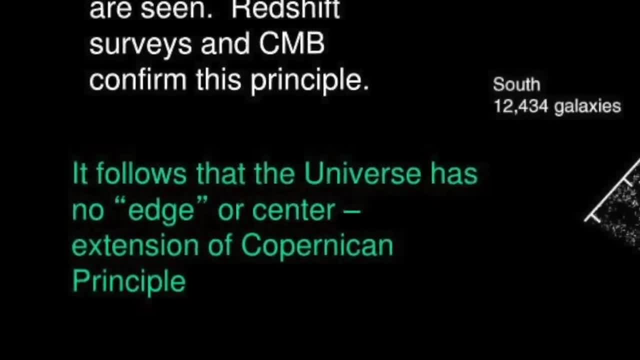 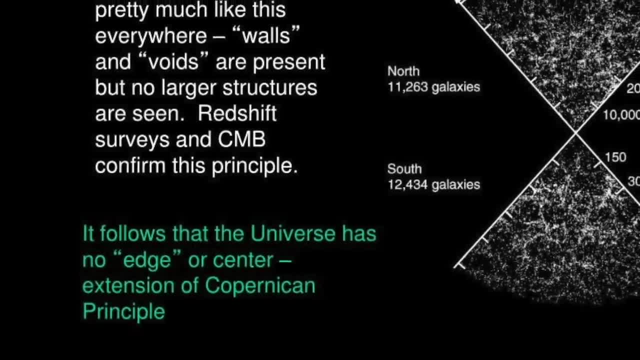 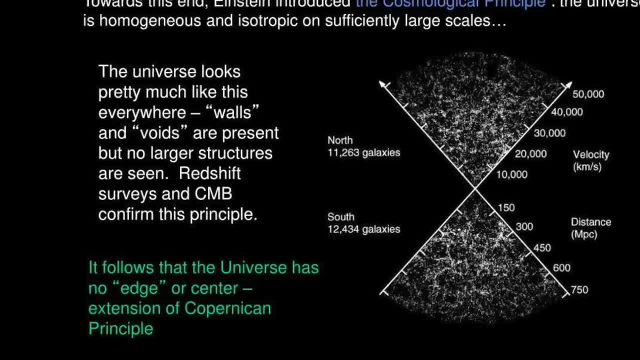 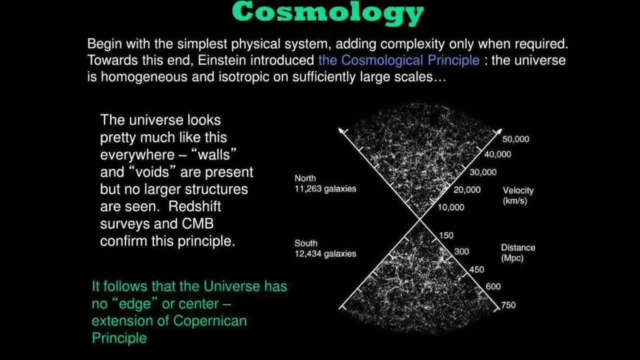 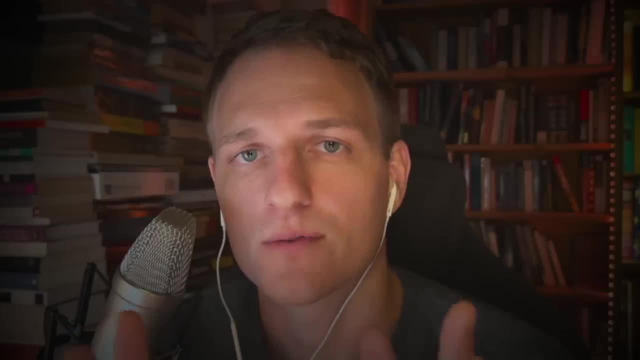 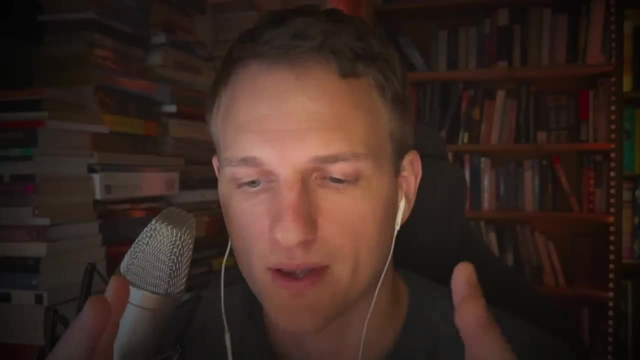 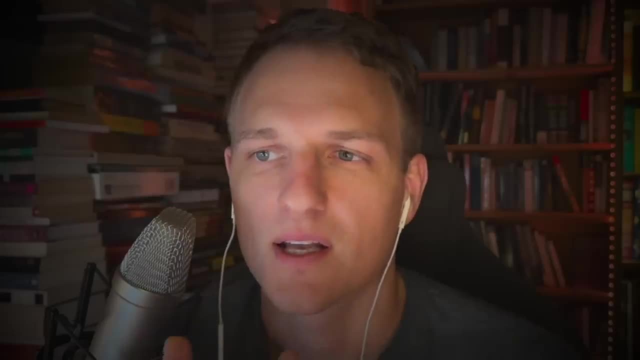 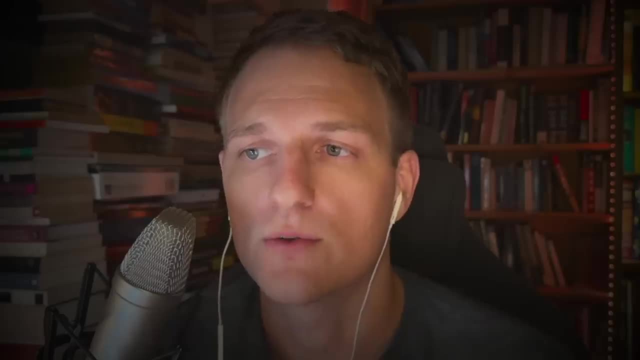 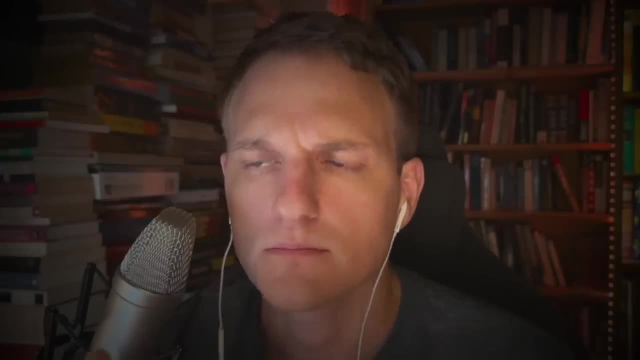 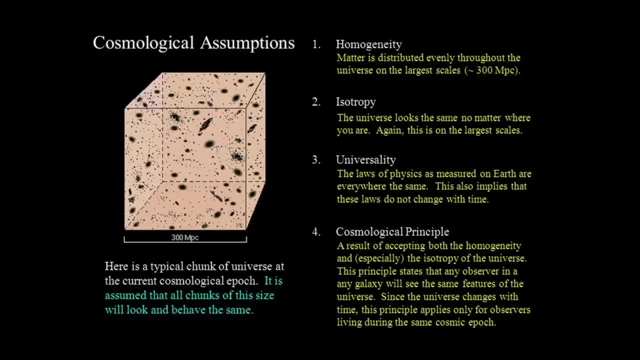 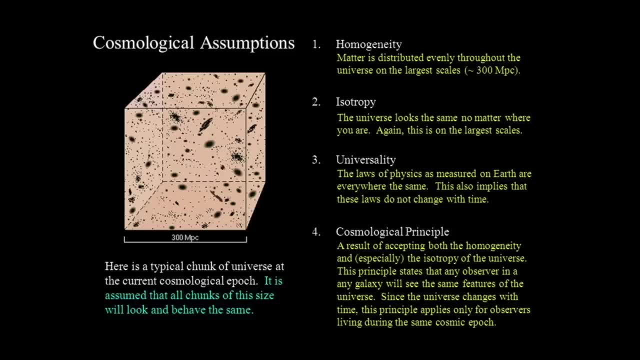 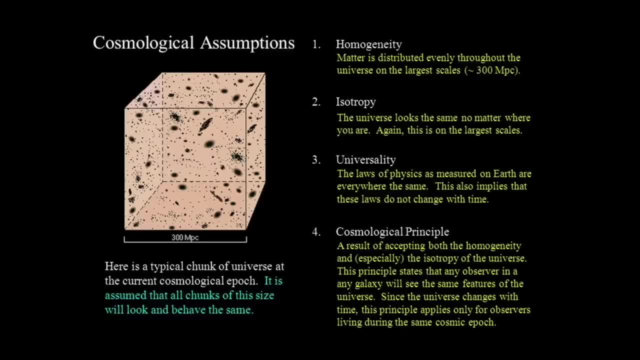 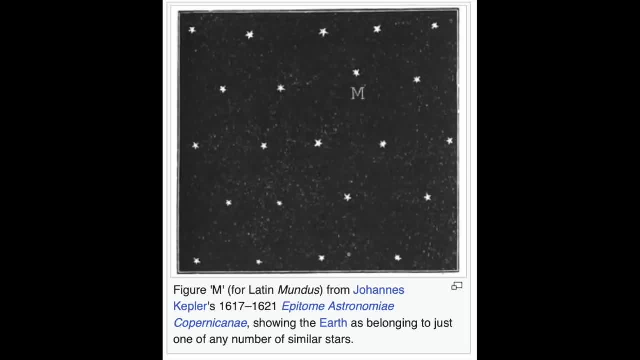 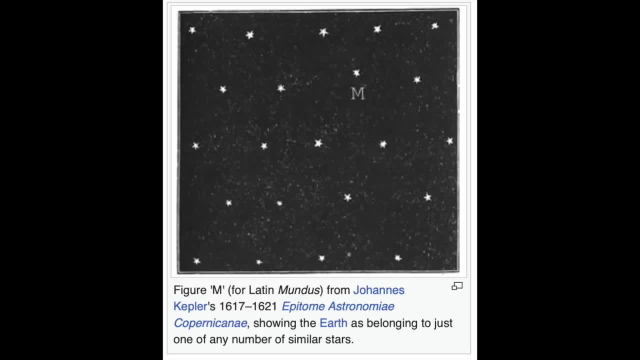 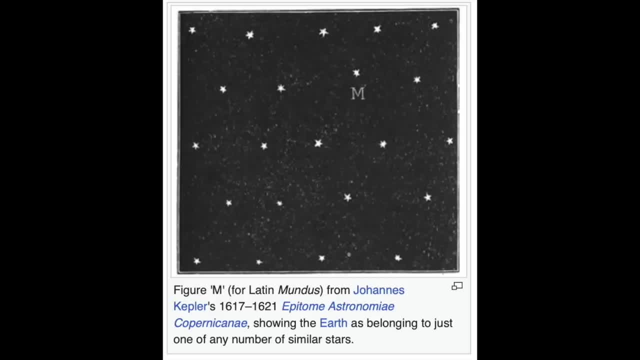 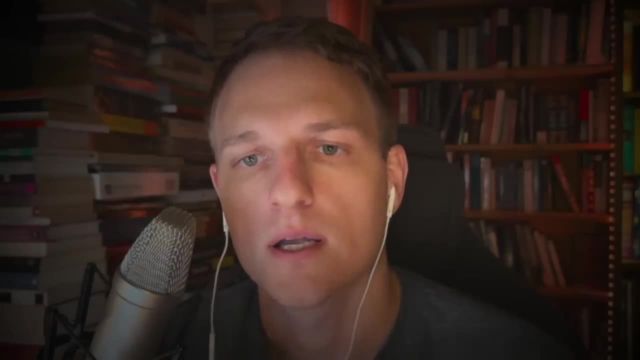 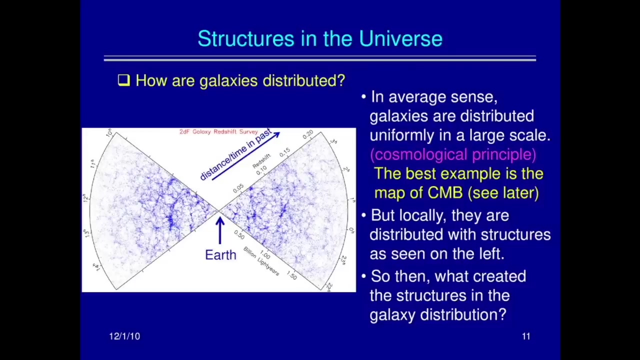 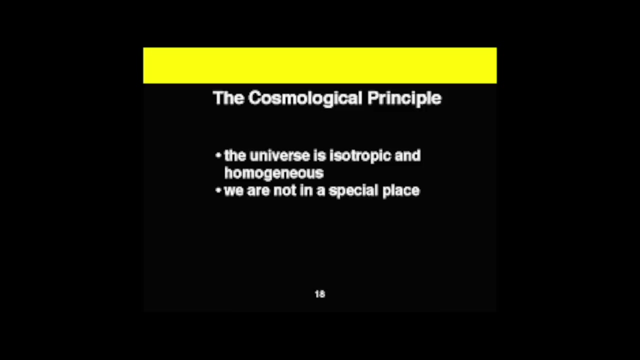 area and then the other. gravity isn't stronger in any particular area for the same amount of given mass. you know, one star of equal mass, 50 trillion light years away from here, is not a more gravitationally pulling on anything. then it is in this corner of the universe. but his notion, his, his perception, his. 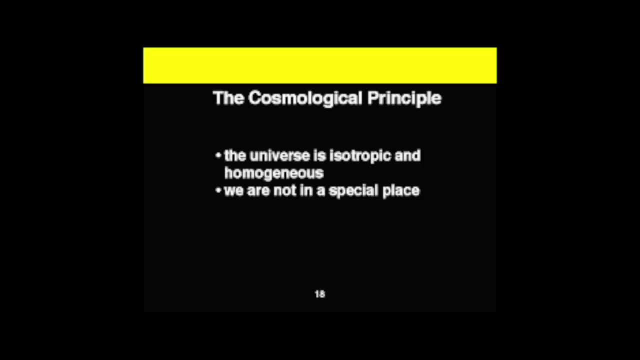 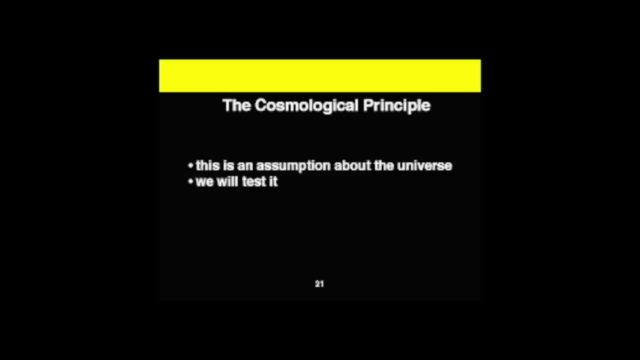 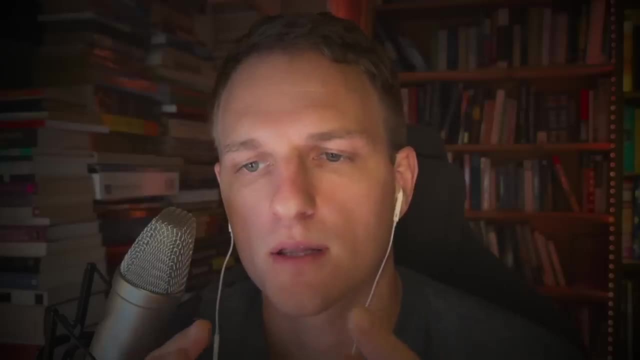 paradigm of the universe, Einstein's, was wrong, because at the time it would be 10 more years actually, until Hubble would come along and change this in the 1920s and before the stars that we see in the Milky Way and we got to remember the Milky Way is so vast that we can't even see stars much beyond. you know, a couple light years away with our naked eye. I guess that's that's true, it's that's not true. rather, we can see a few thousand light years away, I think, but it's 100, 150. 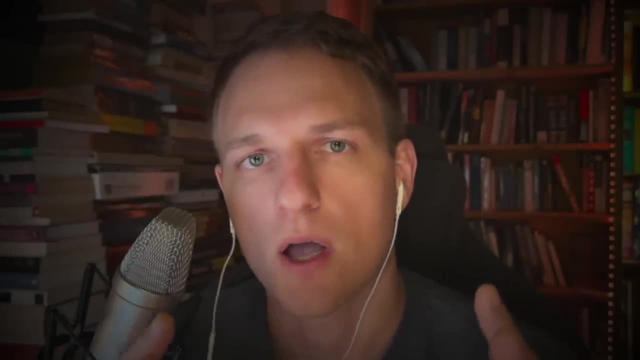 thousand light years across. so even with telescopes we're only seeing the nearest quadrant of stars in our galaxy. and now they were seeing these nebulous swirly, whirlpool looking things, but they thought at the time they didn't realize they were galaxies. they thought 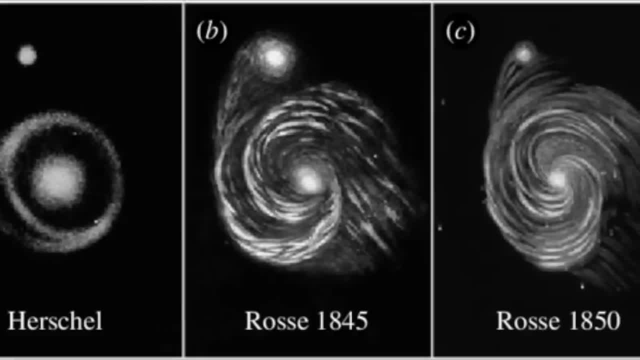 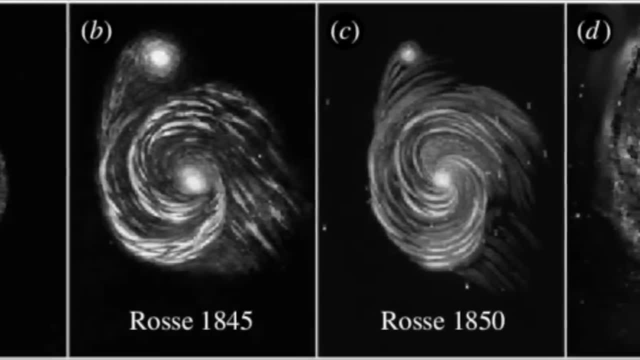 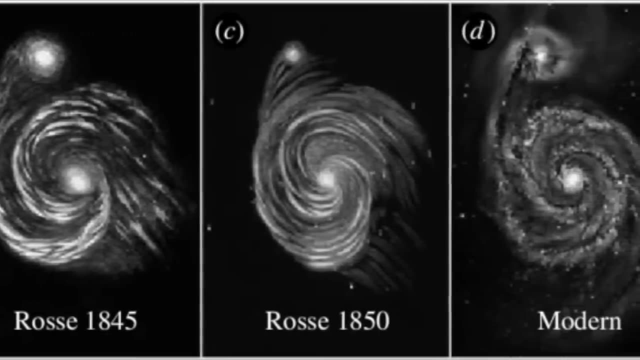 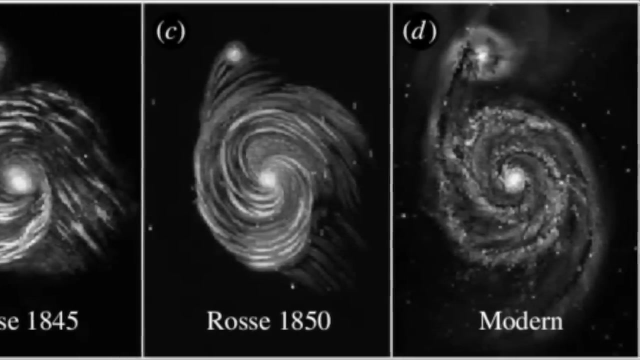 they were maybe just cloud structures in interstellar space among the stars. so for all of eternity, even after we had a couple hundred years in the 1800s and early 1900s, of observing the cosmic cosmos, the stars around us, all the universe appeared to be, was what we now. 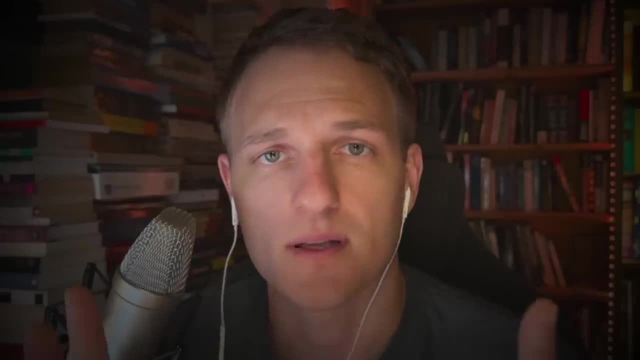 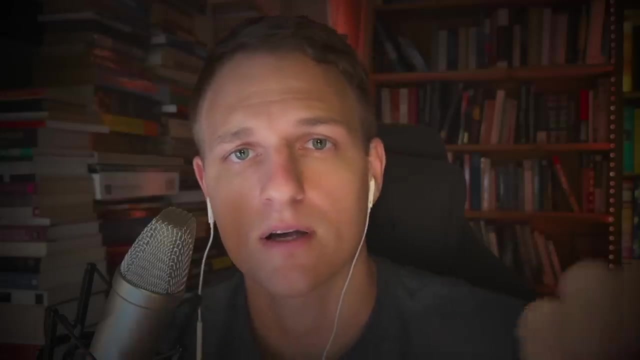 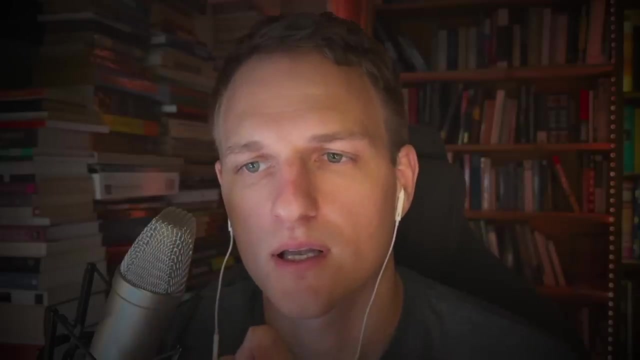 know is the Milky Way, but it was just for anybody. back then, Einstein included all astronomers, the entire universe, the entirety of existence was only what we could see which seemed to be stars. it didn't seem like there were any other islands or groups of stars anywhere else, and so that's all Einstein had to go off of. and because the 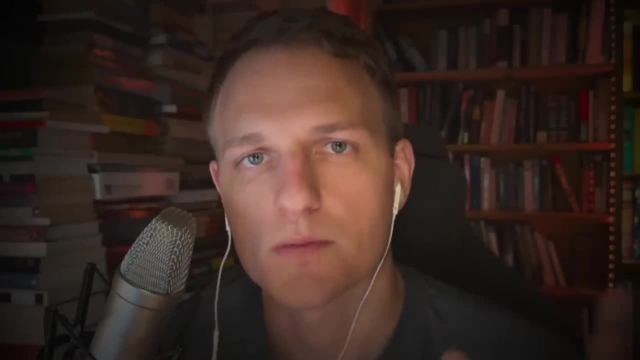 universe didn't appear to be collapsing or expanding, but this would be a one of those instances, again, just like the Sun and Moon appear to revolve around us, where our senses get in the way of finding the truth, you static universe. Einstein tried to attempt to recreate this mathematically. he 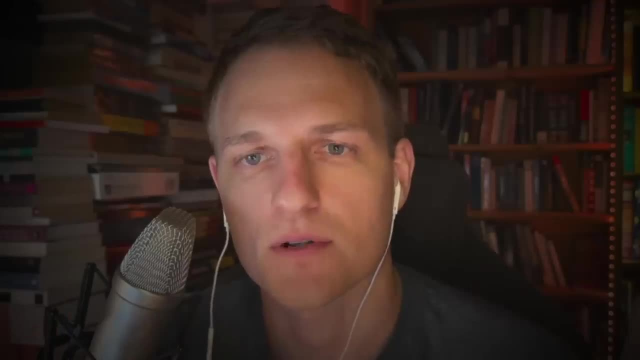 noticed, of course, with all the matter and the stars, that over time, for any experience, extended period of time, there would have been gradual collapse, ation of stars on themselves. so he figured there had to be some sort of repulsive force, like I mentioned, that he called his cosmological constant, that he 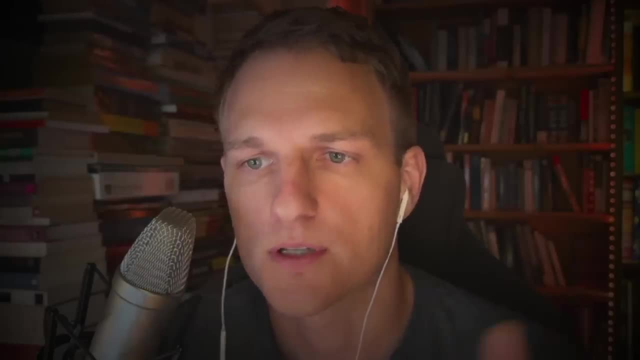 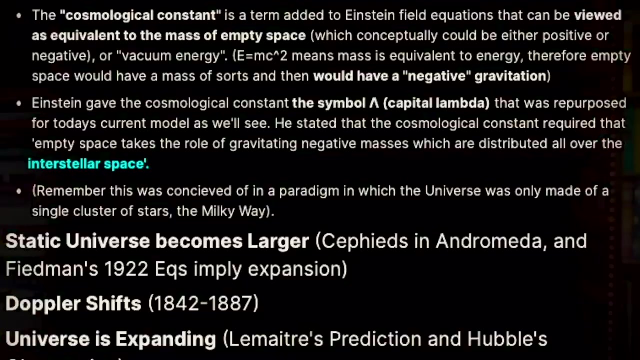 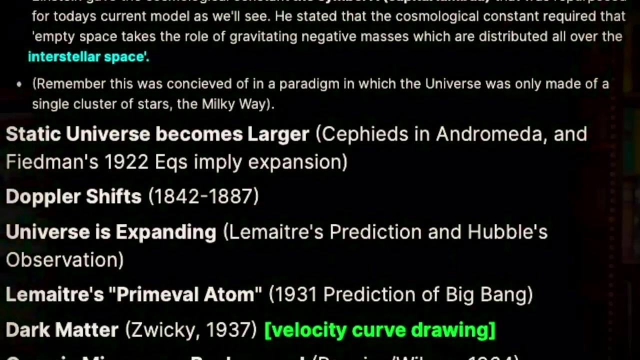 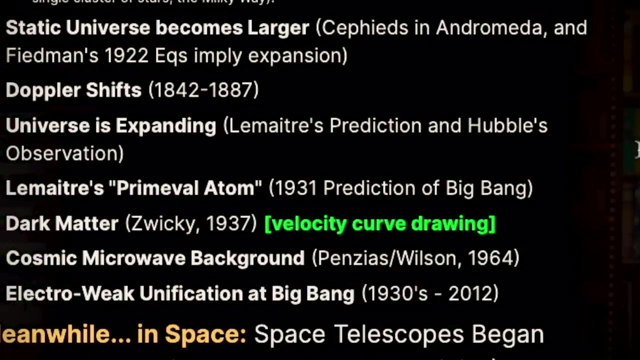 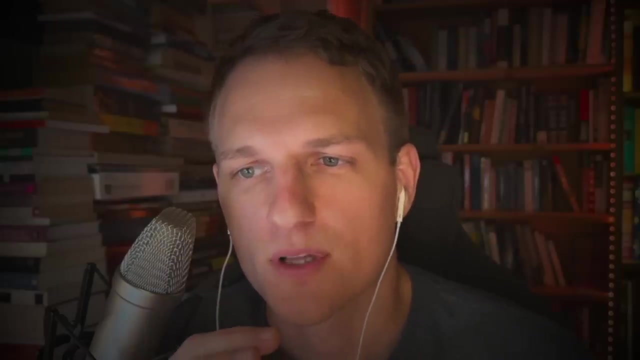 used the letter lambda. he said that conceptually could be considered as anti-gravity, really a gravity that repels rather than attracts. so what he considered was that empty space itself had this was permeated by this negative gravity, that would exactly counter matter, and we'll see that this was actually really prescient. he really came upon. 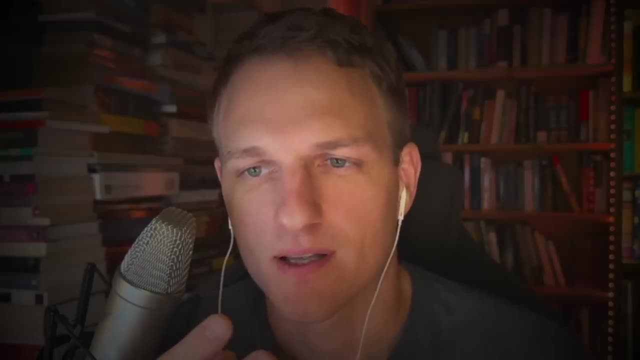 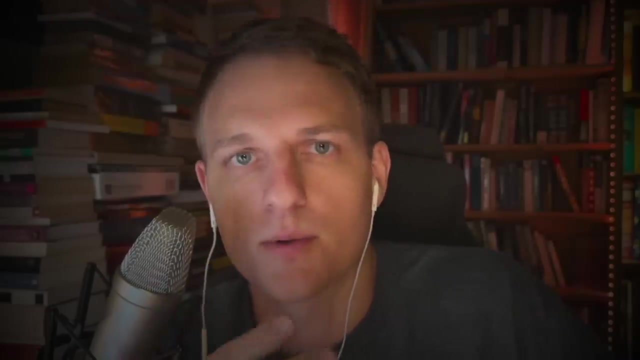 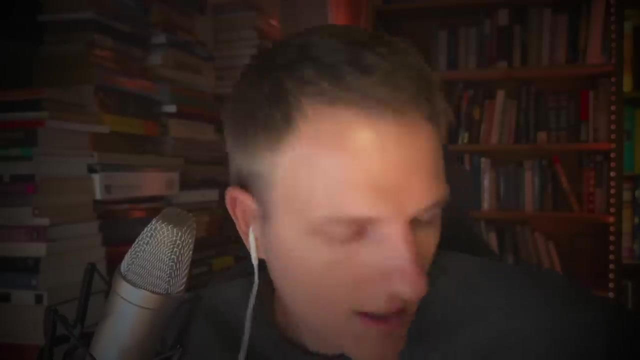 something in this thought experiment in researching physics. he, Einstein, truly observed, deserves his reputation for being, you know, the archetypal genius figure. he, he, he was a just a remarkable, remarkable thinker who never did it. and this object would be nothing but a lack of класс a. 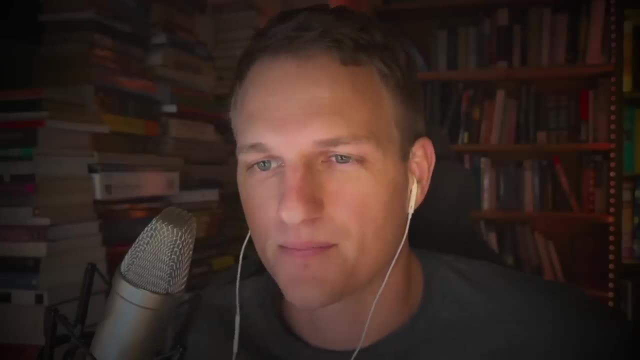 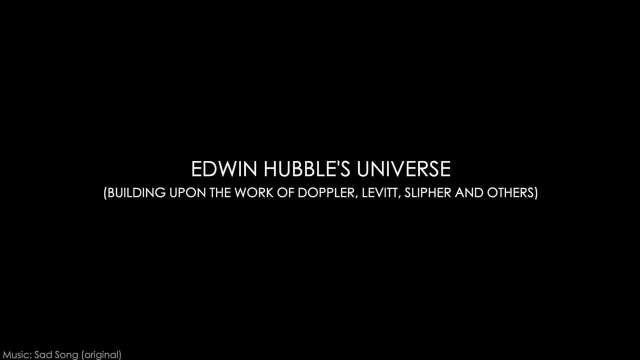 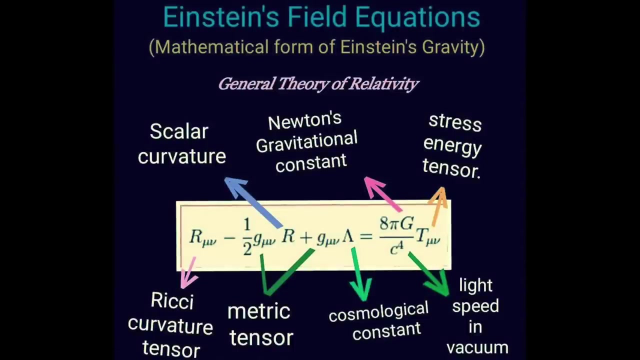 general, and this idea, it turns out this, it's either. and this idea it turns out this it's either, come back 100 years later. so, as a mention, lui, in the intro, So the static universe of Einstein's where you have is a perfect. you know, we didn't even know at the 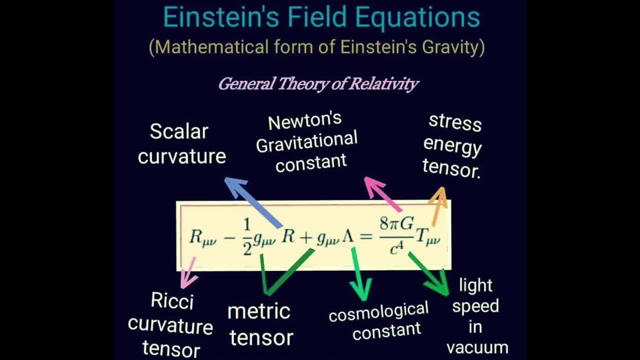 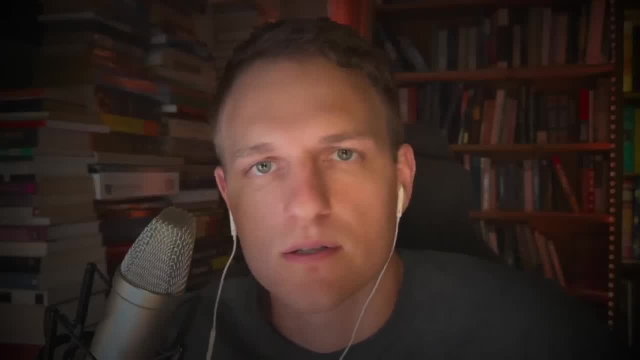 time we were part of a galaxy beneficial capableija field of stars static in position, and Einstein had to have this field penetrated, the interstellar space, in this field permeated by this negative repulsive gravitational force. However, less than a decade after Einstein had kind of theorized this, 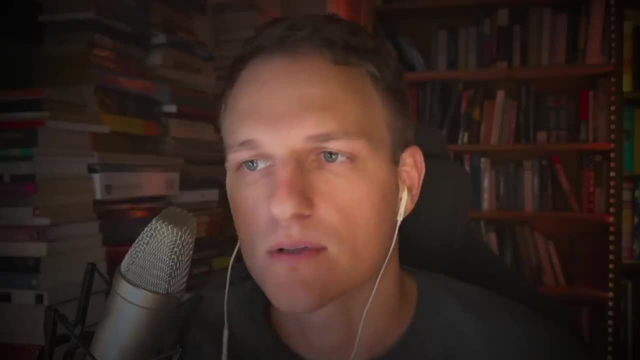 and came out with his general relativity field equations that seemed to perfectly explain all the light phenomenon that we're seeing. Edwin Hubble then made a discovery that would prove the universe is far larger than just the Milky Way Around 1900, probably 20 years earlier. 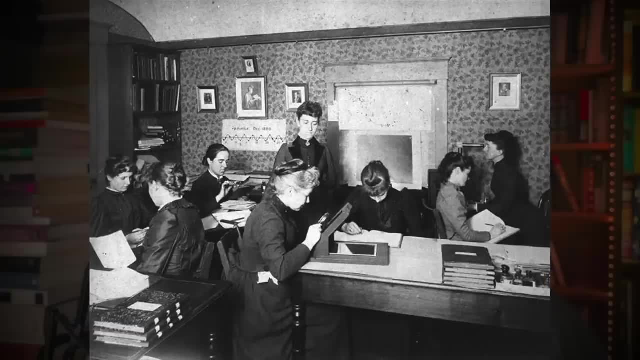 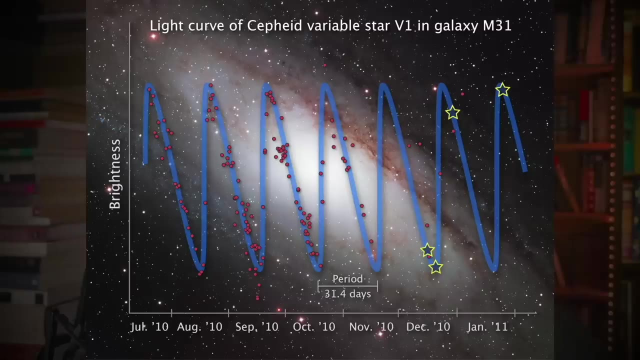 several variable stars had been meticulously studied by a woman named a female astronomer named Henrietta Leavitt of Harvard, and she'd found a firm relationship between the actual brightness of how fast their actual brightness and how fast their actual brightness and how fast they pulsed, because they were a periodic pulsing star. 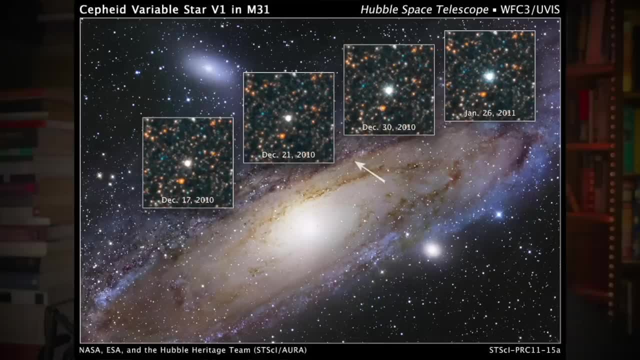 They consistently pulsed every consistent amount of days over, you know, anywhere from a couple days to a couple weeks and or maybe a couple hours, but they were exceptionally bright stars And what she found, for instance, was that for any given period, 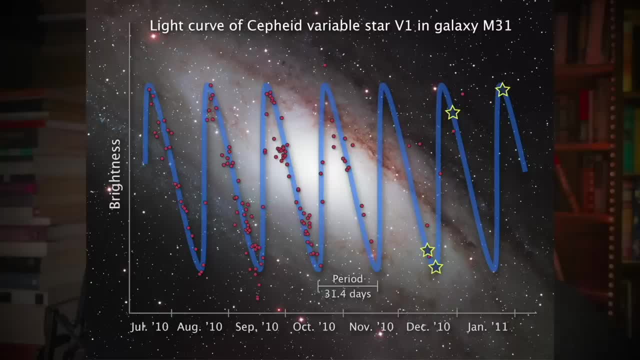 their magnitude that you could observe was always very consistent. So even on different parts of the sky, different stars, if they had roughly the same period, they would have roughly the same magnitude. And she studied thousands of these. So she developed a scheme and a map. 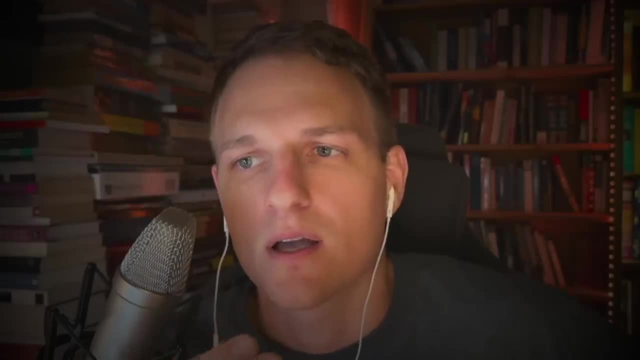 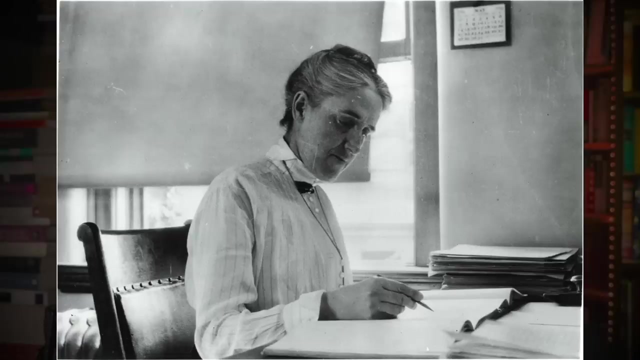 of actually being able to use these as standard candles. She compared their apparent luminosity to their intrinsic luminosity to give them a better understanding of the universe, To give their distance to Earth, And that's for another video to go into more. but it's really interesting how she deduced that. 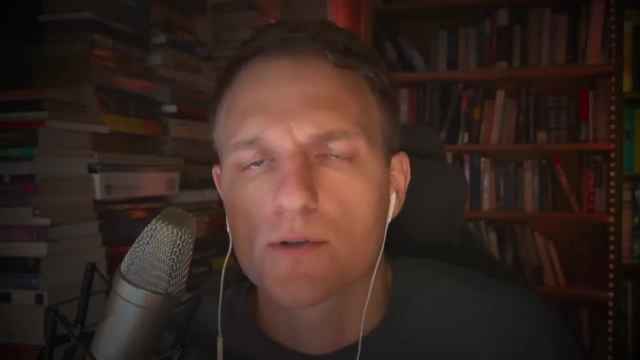 and figured it out. Hubble's first major discovery decades later, in the 20s, was to identify Cepheid variables in some of these larger spiral nebulae. What you know was considered just nearby, within the same you know, among the stars. 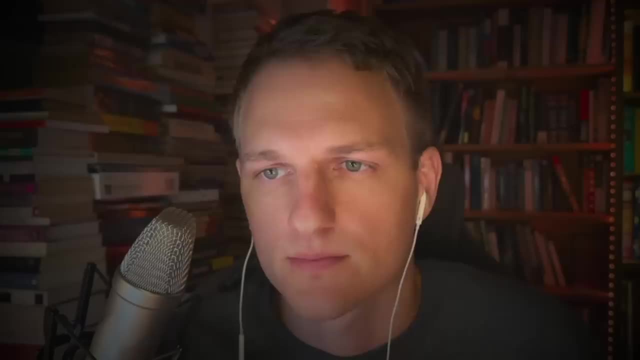 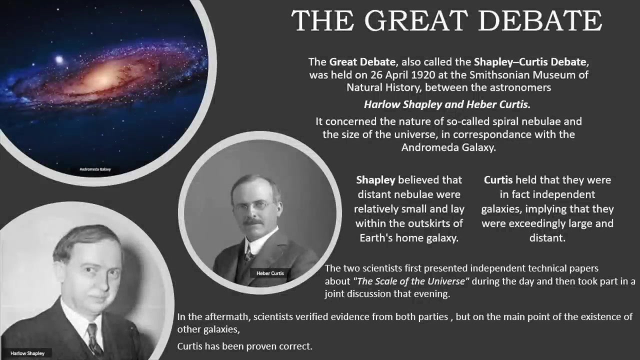 that we're observing And, most famously, he looked at one in Andromeda And when he compared their luminosity to the known standards, he found that they were way too distant to be in the Milky Way, And around the same time in the 20s. 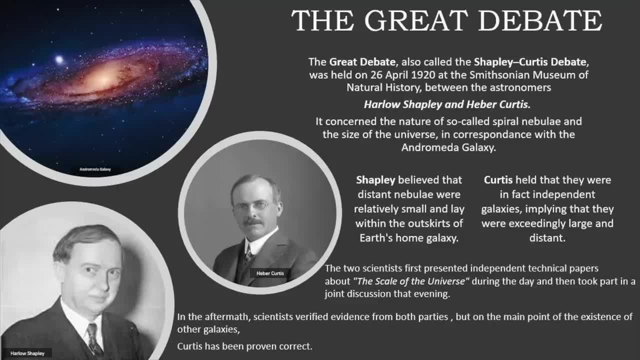 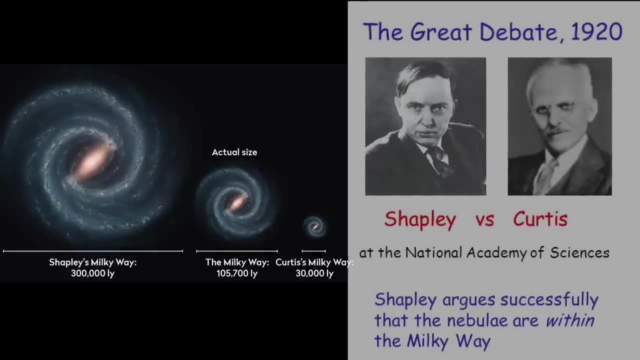 it had begun to actually be seriously theorized and famously even debated- And this famous debate here- Whether some spiral clouds of these might actually be distant star clusters. Until 1924, the universe, of course, had been the entire, or the Milky Way. 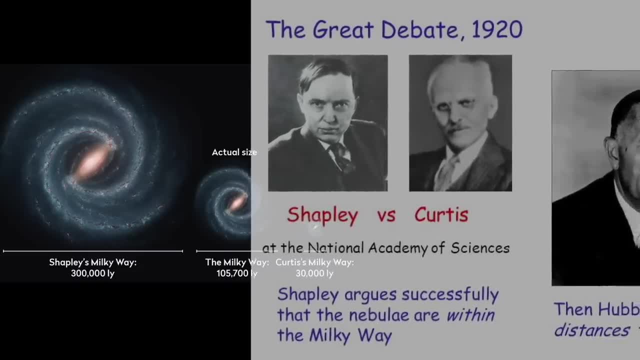 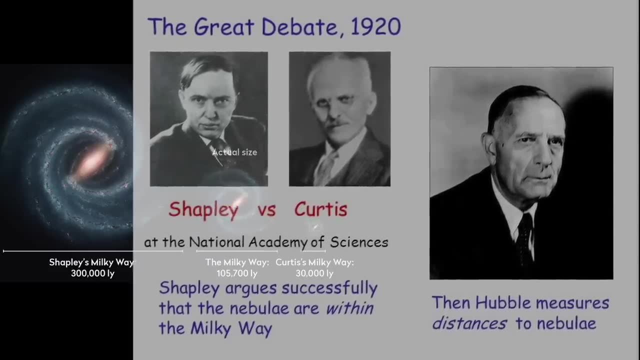 had been the entire universe. But that changed with Hubble's findings. The brightness and period of the Cepheid he had observed in Andromeda meant that it was not just thousands or even tens of thousands, even hundreds of thousands, It was millions. 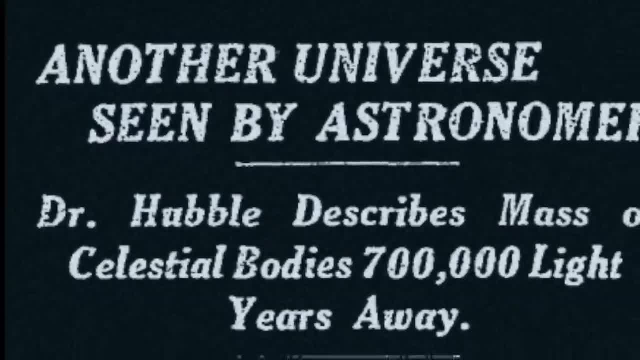 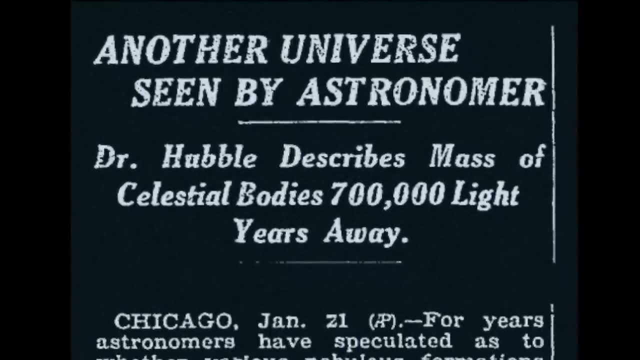 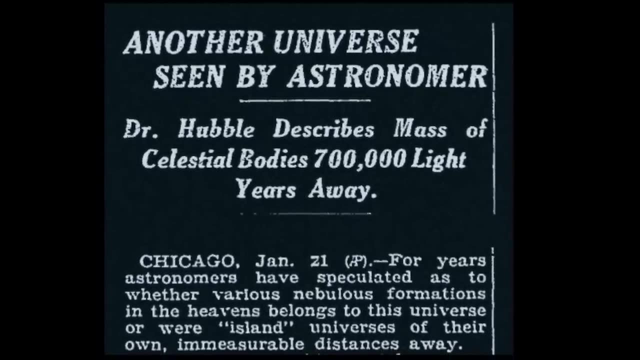 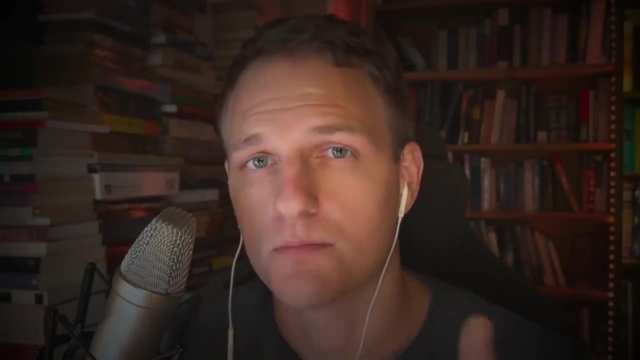 Millions of light years away And that just blew the lid off the current paradigm of cosmology. Even Einstein's theory, you know he hadn't expected the universe to be that vast, Remember we, you know, we know. now it's billions, almost 100 billion light years across. 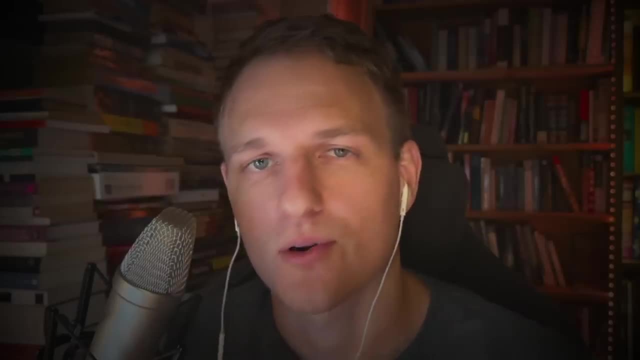 That's almost 10,000 times, you know, 10,000 times larger than what Hubble is blown away by. Cepheid variable was just because it was able to have the same period as a nearby variable with a similar period. 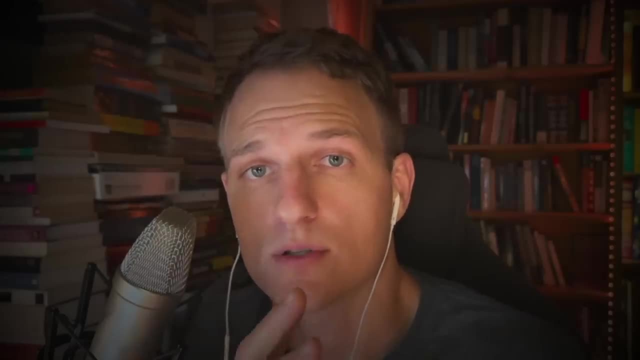 We saw how faint it was, which meant it was a. we could tell how distant it must be to be that faint, And it wasn't just a one-off. That was just the most prominent example. He studied, you know dozens and dozens of these to really 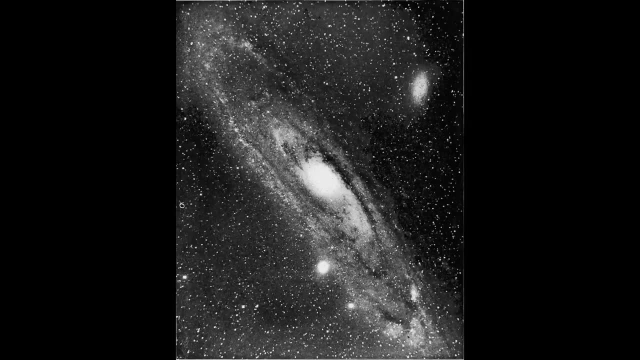 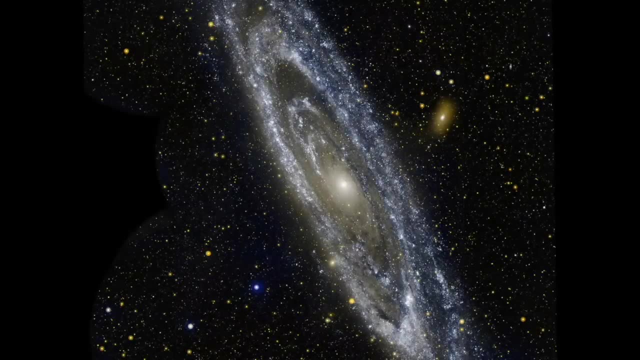 you know, hammer it down and make sure he had the numbers right. So now he had the universe blown up and said: oh, these nebulae, these spiral nebulae, are actually other islands, other swirling fields of stars, And they're way beyond the Milky Way. 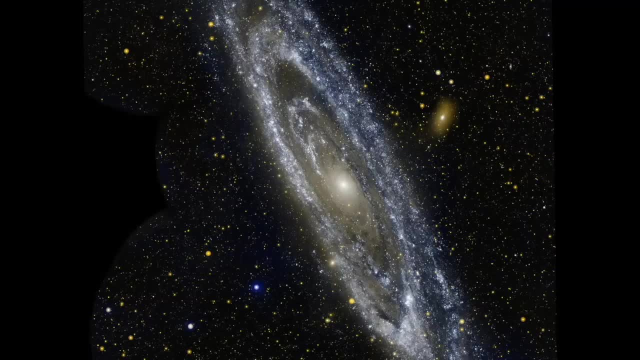 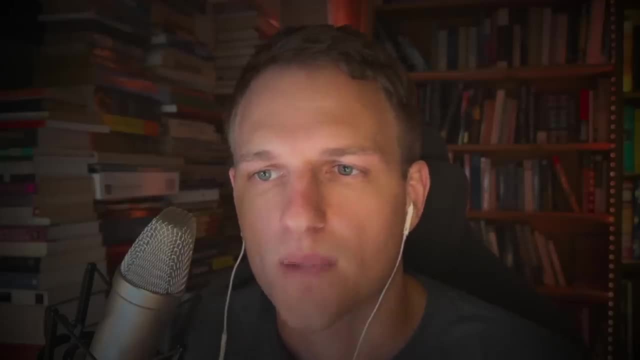 We must be in our own swirling field of stars, And these other ones are the only hints at the more distant ones. And so Einstein was pretty quick to grasp that if these field equations he had were true, then the static universe, even one balanced with a cosmological constant, 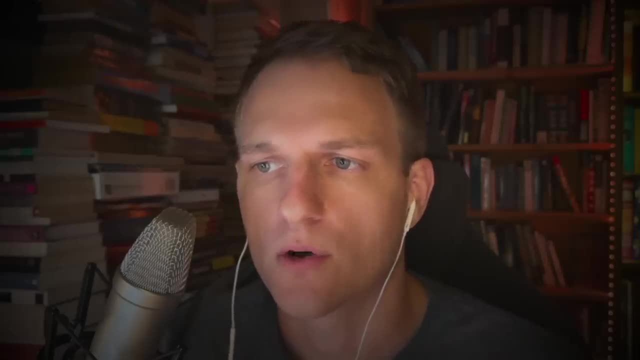 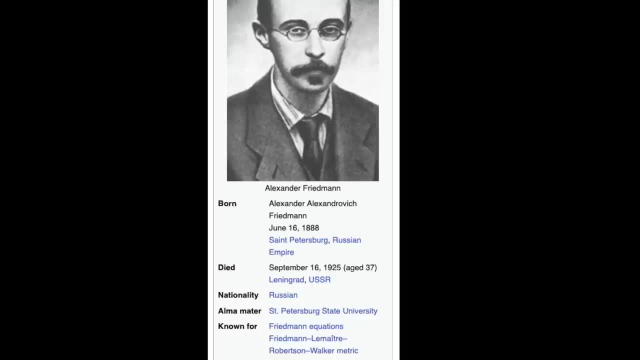 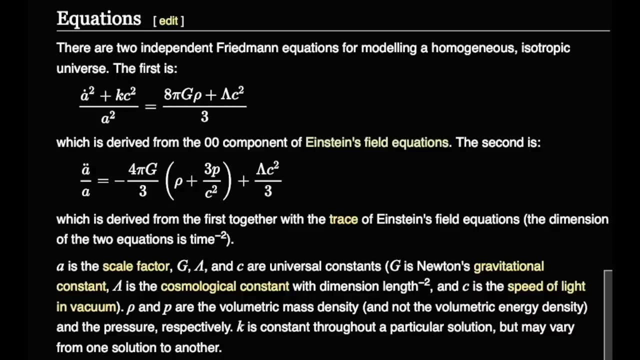 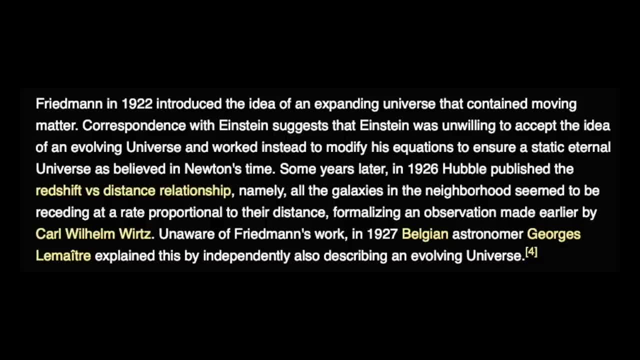 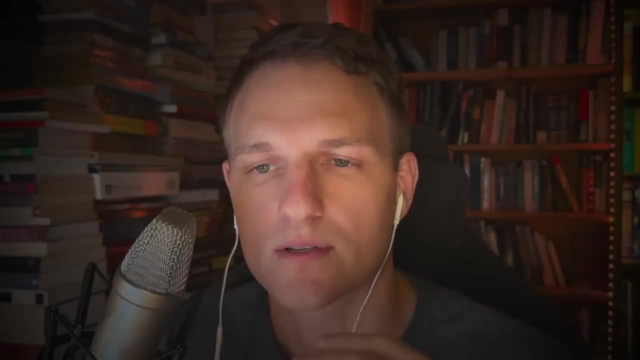 and applying those to Einstein's equations, might actually be expanding. But the stars nebulae in the universe weren't moving as fast either towards us or away from us as expansion would have made them. but two years later Hubble would make his great redshift discoveries. that would show just that Doppler, the guy who came. 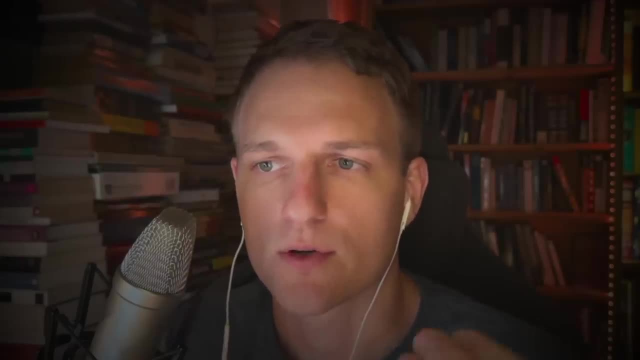 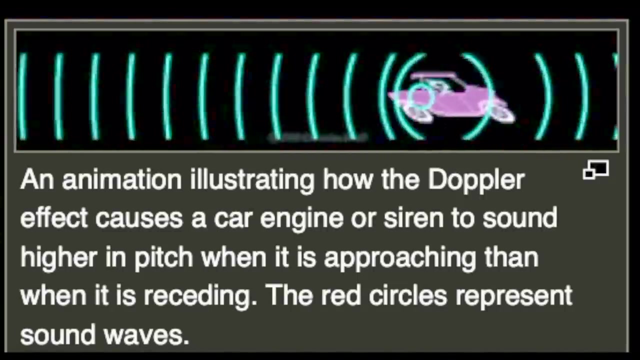 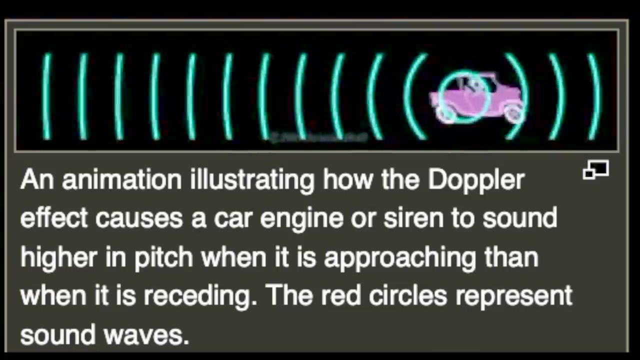 up with the concept of Doppler shifts. his name was actually Christian Doppler, Austrian physicist. he described the phenomenon way back almost 80 years before, in 1842, and he actually correctly predicted that this phenomena should apply to all waves, because, uh, you know, it has something to do with, of course. 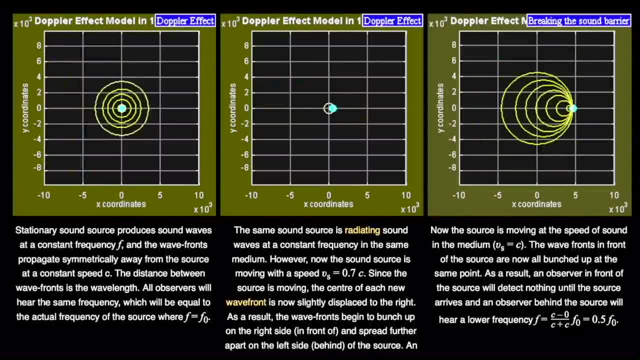 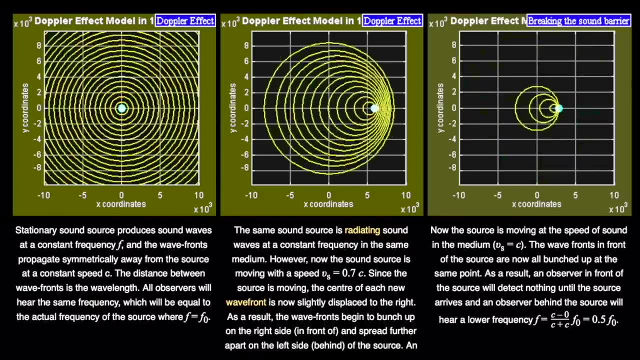 sound waves. that's the most intelligible example to us, but it applies to light waves too. and and he actually even predicted that the color shift would vary depending on how fast the waves would move. and so he actually predicted that the color shift would vary depending on how fast the waves would move, and so he actually even predicted that the color shift would. 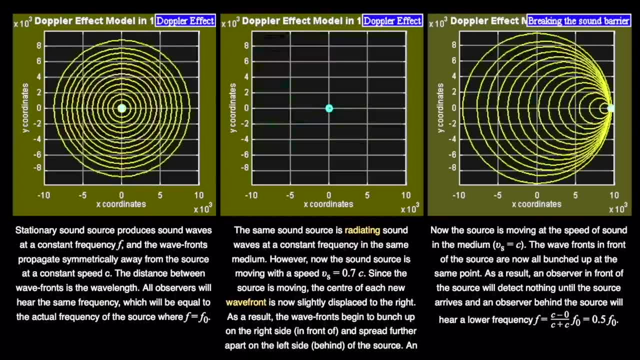 vary depending on how fast the waves would move. and so he actually predicted that the color shift would vary, but because of stars that were, you know, vary. but because of stars that were, you know, vary. but because of stars that were, you know, moving far away, they would shift to. 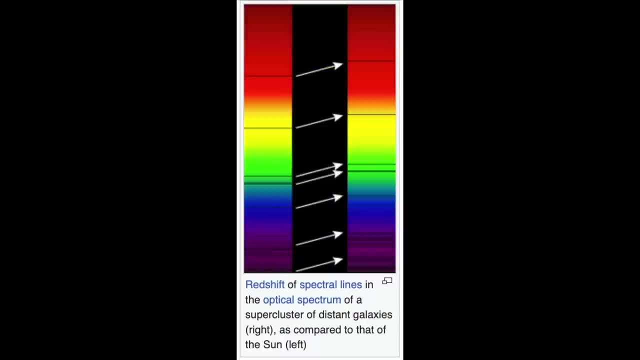 moving far away. they would shift to moving far away. they would shift to the red to a lower energy wavelength, or if the red to a lower energy wavelength, or if the red to a lower energy wavelength, or if they were traveling towards us, they, they were traveling towards us, they. 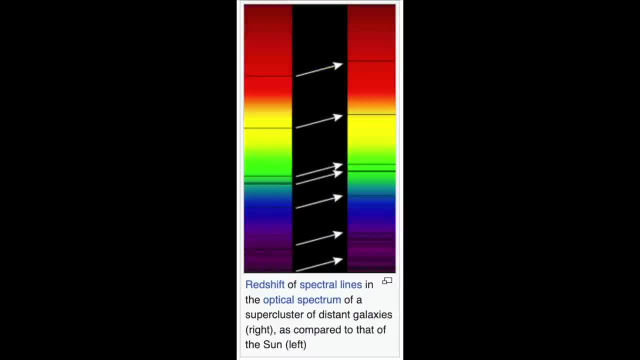 they were traveling towards us, they would get compressed and shift blue back would get compressed, and shift blue back would get compressed. and shift blue back in the 1800s, which was amazing because in the 1800s, which was amazing, because in the 1800s, which was amazing, because that was actually pretty right- galaxies. 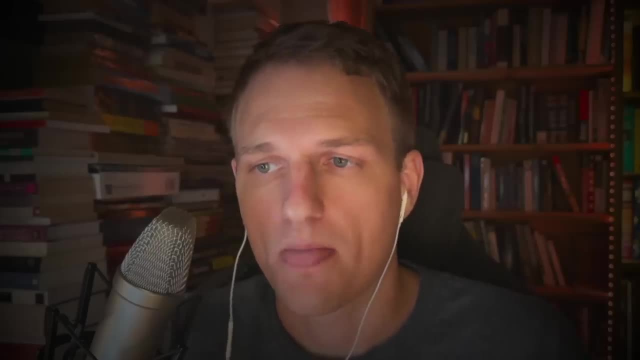 that was actually pretty right. galaxies, that was actually pretty right. galaxies: we don't see a lot of blue shifting. we don't see a lot of blue shifting. we don't see a lot of blue shifting galaxies, because they don't only a couple galaxies, because they don't only a couple. 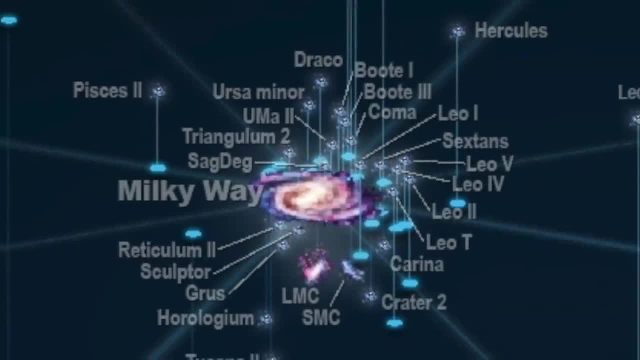 galaxies, because they don't only a couple- are traveling towards us like Andromeda are traveling towards us like Andromeda are traveling towards us like Andromeda. Triangulum but tons of galaxies from the Triangulum, but tons of galaxies from the Triangulum, but tons of galaxies from the expansion of the universe are traveling. 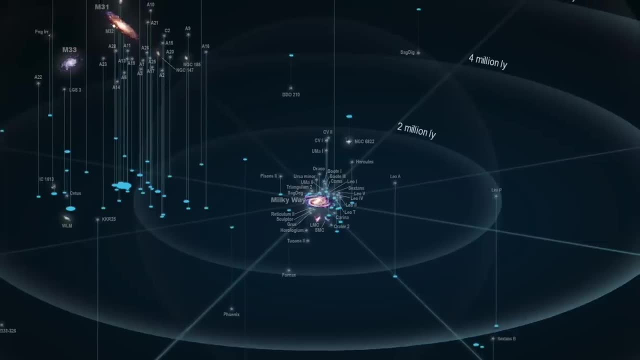 expansion of the universe are traveling. expansion of the universe are traveling very fast way faster than the speed of very fast, way faster than the speed of very fast, way faster than the speed of light. away from us, making them red light, away from us, making them red light, away from us, making them red. shifted, but his idea was actually shot. 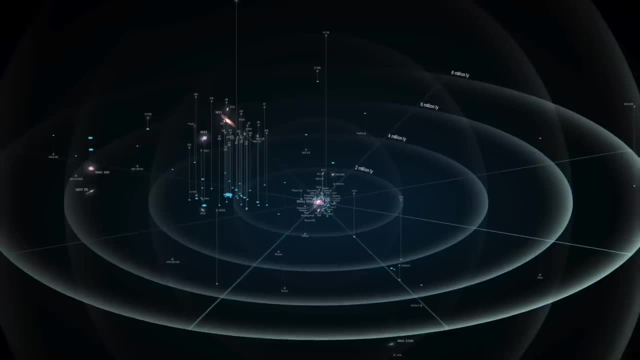 shifted, but his idea was actually shot, shifted, but his idea was actually shot down because, uh, actually, because of down, because of down, because of black body radiation was taken root and black body radiation was taken root, and black body radiation was taken root and there was a understanding that. 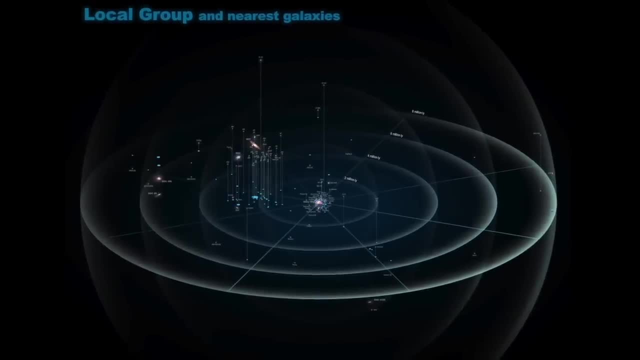 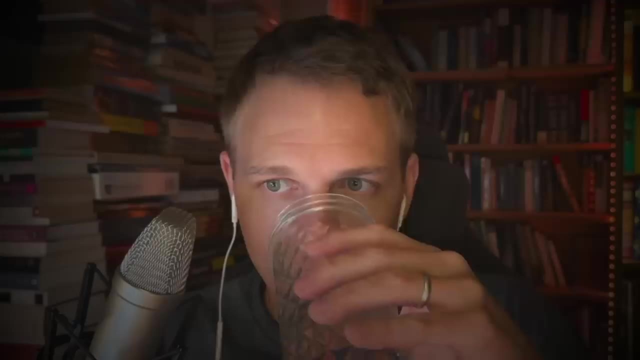 there was a understanding that. there was a understanding that temperature of course is correlated with temperature, of course is correlated with temperature. of course is correlated with color, which is true, but the Doppler color, which is true, but the Doppler color, which is true, but the Doppler effect was not taken into account. so 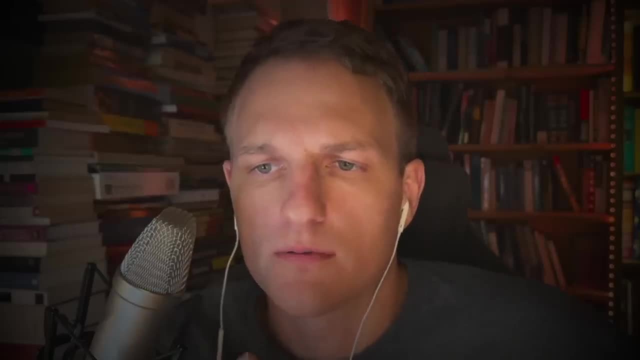 effect was not taken into account. so effect was not taken into account. so this: there was actually a long history. this: there was actually a long history, this: there was actually a long history of looking at stars. it was only a couple of looking at stars. it was only a couple. 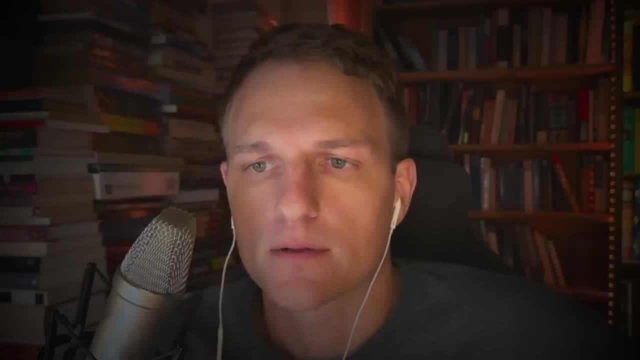 of looking at stars. it was only a couple, maybe a decade later, a couple decades, maybe a decade later, a couple decades, maybe a decade later, a couple decades later that the astronomers first. later that the astronomers first later that the astronomers first took Doppler's ideas about shifts and. 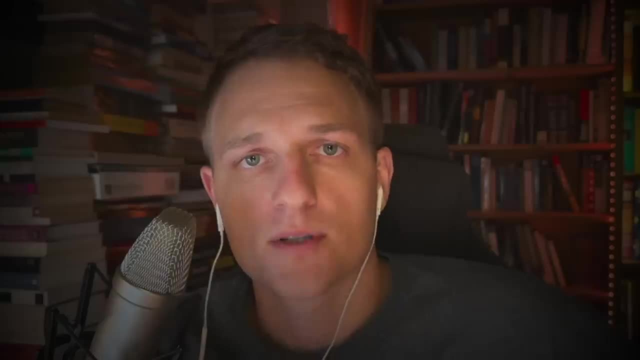 took Doppler's ideas about shifts and took Doppler's ideas about shifts and waves and applied them to the optical waves and applied them to the optical waves. and applied them to the optical Fraunhofer lines and other absorption. Fraunhofer lines and other absorption. 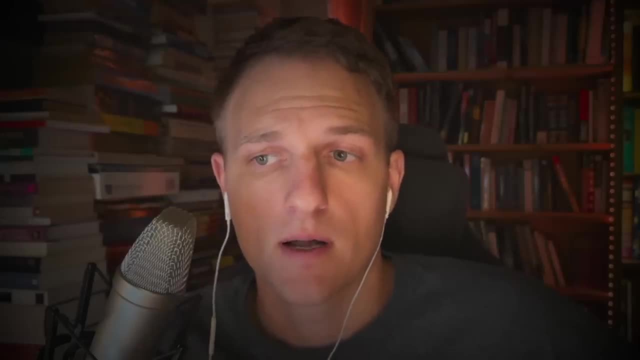 Fraunhofer lines and other absorption lines and stars. and recognize that, hey, lines and stars. and recognize that, hey, lines and stars. and recognize that, hey, they must be, they must be shifting you, they must be, they must be shifting you, they must be, they must be shifting. you know if they, based on their movement. 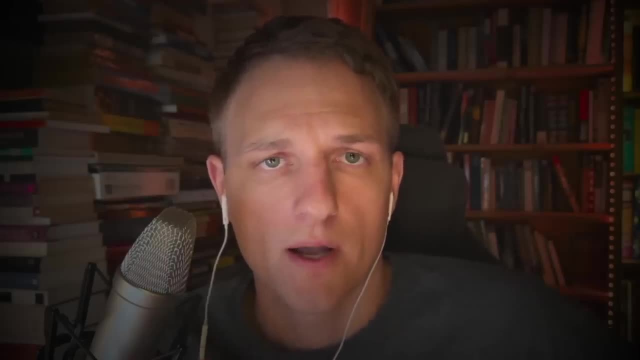 know if they, based on their movement, know if they, based on their movement, these lines should be. you know the these lines should be. you know the these lines should be. you know the wavelength for the absorption line of wavelength for the absorption line of wavelength for the absorption line of hydrogen should be at 121 nanometers. but 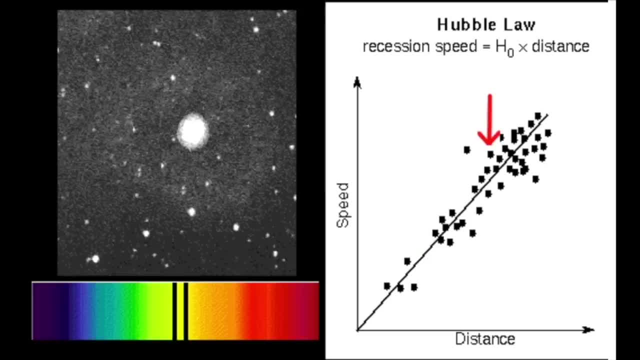 hydrogen should be at 121 nanometers. but hydrogen should be at 121 nanometers. but what's going on with that? and they kind what's going on with that and they kind what's going on with that and they kind of deduced that, oh, okay, and maybe it is. 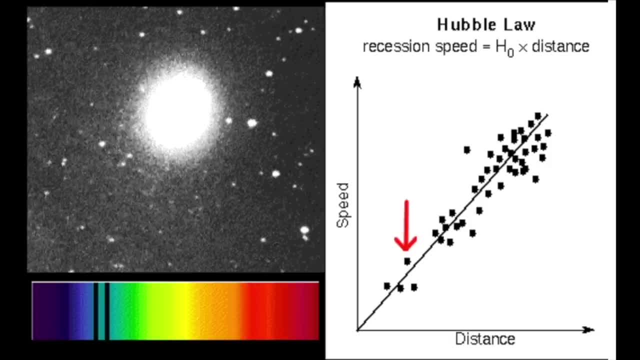 of deduced that, oh okay, and maybe it is of deduced that, oh okay, and maybe it is because they are traveling away, and so because they are traveling away, and so because they are traveling away, and so it's stretching the light out a little, it's stretching the light out a little. 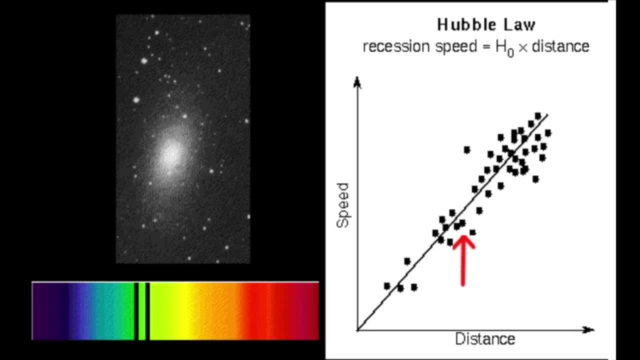 it's stretching the light out a little bit. and about ten years before Hubble bit, and about ten years before Hubble bit and about ten years before Hubble had made his famous Cepheid discovery, had made his famous Cepheid discovery, had made his famous Cepheid discovery and would go on to make some redshift. 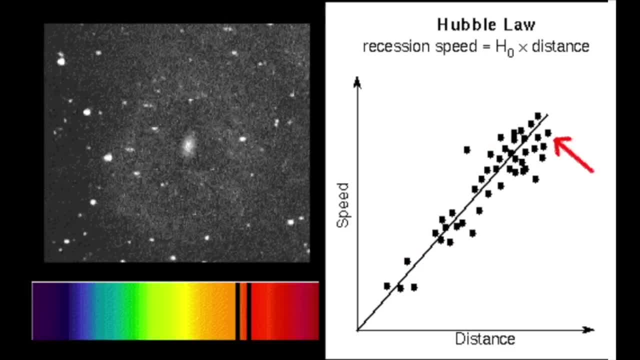 and would go on to make some redshift and would go on to make some redshift measurements, maybe closer to 20 festo measurements, maybe closer to 20 festo measurements, maybe closer to 20 festo. sliffer discovered that a lot of the sliffer discovered that a lot of the 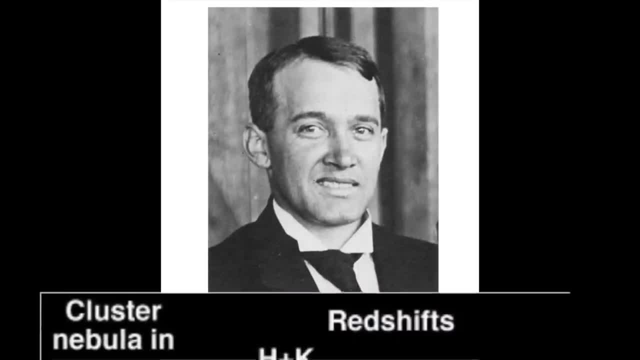 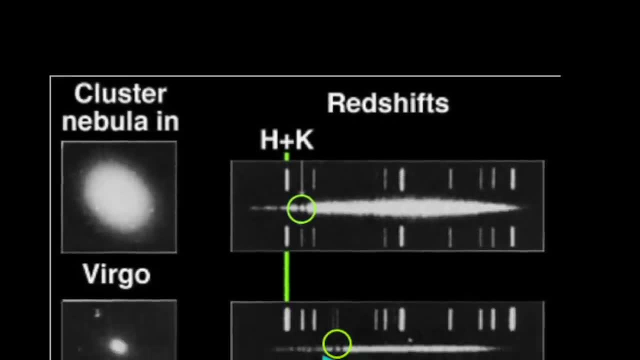 sliffer discovered that a lot of the spiral nebulae. he performed some spectra spiral nebulae. he performed some spectra spiral nebulae. he performed some spectra on them and he discovered that a lot of on them and he discovered that a lot of on them and he discovered that a lot of the spiral nebulae had considerable red. 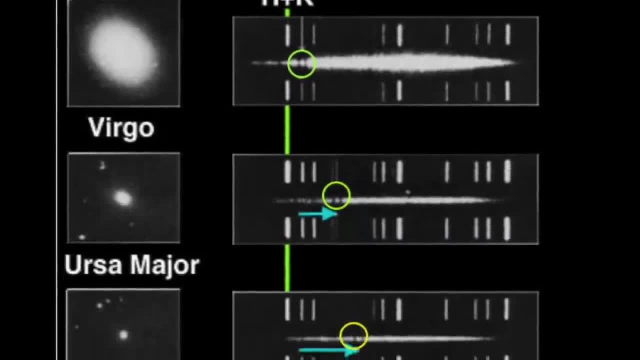 the spiral nebulae had considerable red. the spiral nebulae had considerable red shifts. he went on to record about 20 shifts. he went on to record about 20 shifts. he went on to record about 20 different galaxies that had mostly all different galaxies that had mostly all. 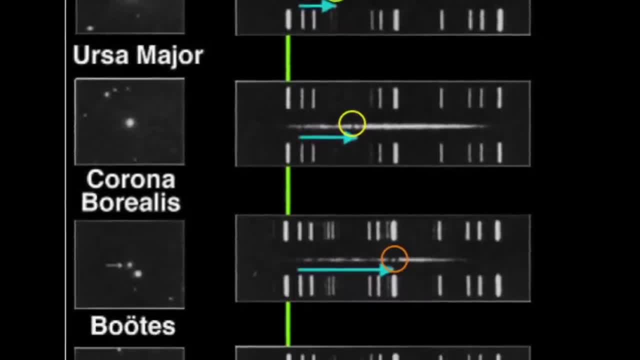 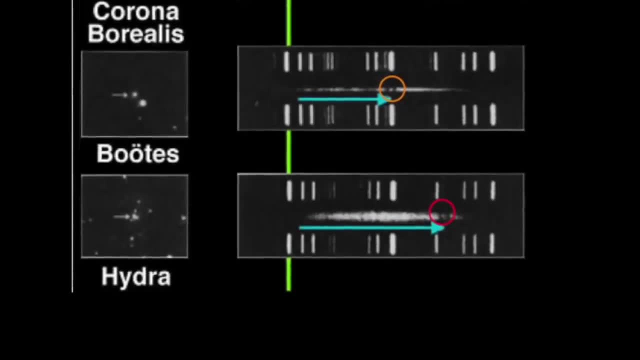 different galaxies that had mostly all red shifts, except for the few that were red shifts, except for the few that were red shifts, except for the few that were. unfortunately he didn't grasp the. unfortunately he didn't grasp the. unfortunately he didn't grasp the cosmological implications of this. 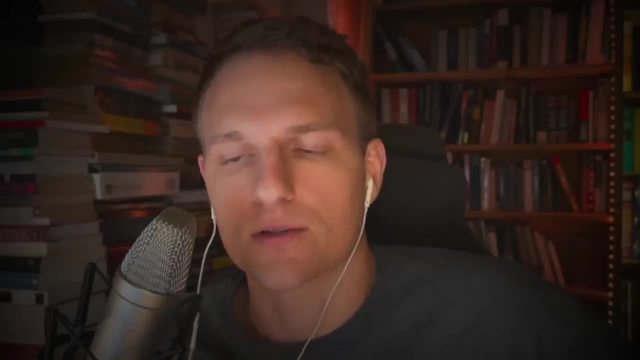 cosmological implications of this, cosmological implications of this, especially because at the time it was, especially because at the time it was, especially because at the time it was still, you know, controversial, whether or still you know, controversial, whether or still you know, controversial, whether or not he was doing this in the 19 teens. 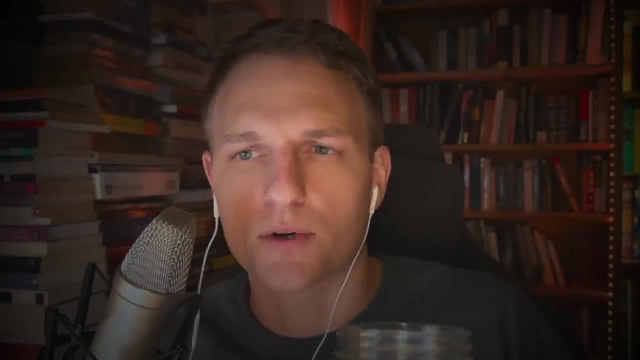 not, he was doing this in the 19 teens. not, he was doing this in the 19 teens before general relativity was even out, before general relativity was even out. before general relativity was even out. he was wondering, maybe probably thinking. he was wondering, maybe probably thinking. 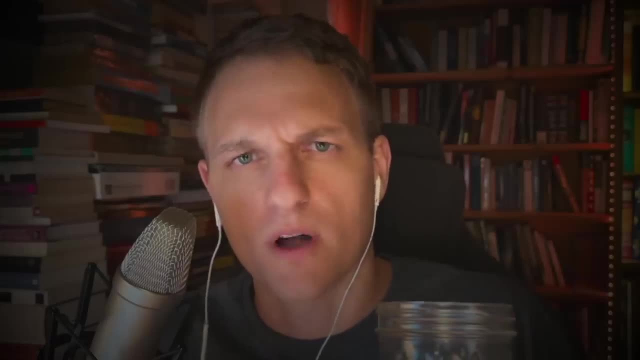 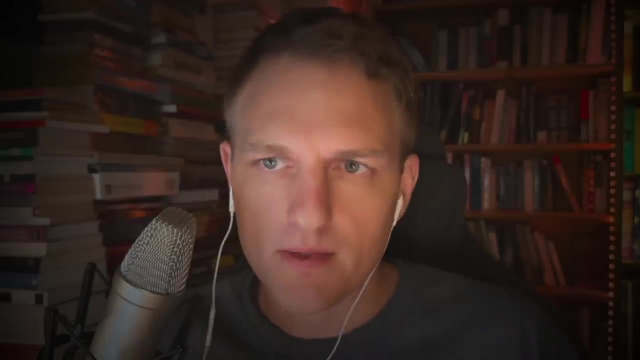 he was wondering, maybe probably thinking about them as nebulae amongst the stars, about them as nebulae amongst the stars, about them as nebulae amongst the stars, and wondering why they were traveling, and wondering why they were traveling and wondering why they were traveling so fast away, but in 1927, just a year or. 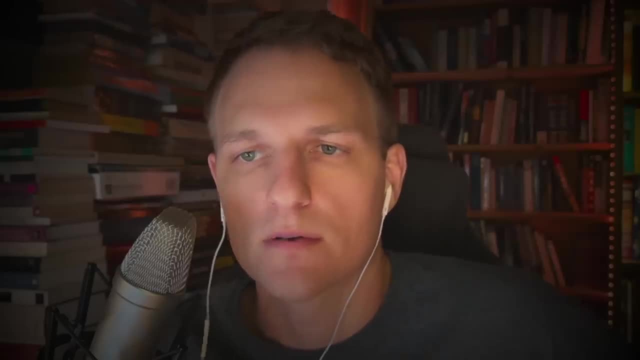 so after a few years after Hubble had so after a few years after Hubble had so, after a few years after Hubble had discovered Andromeda was 2 million light discovered. Andromeda was 2 million light discovered. Andromeda was 2 million light years away, blowing up the universe. but 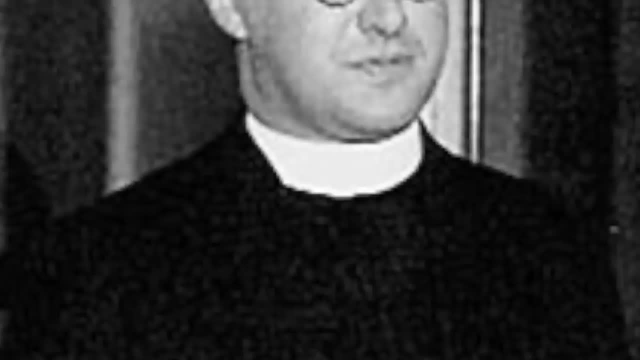 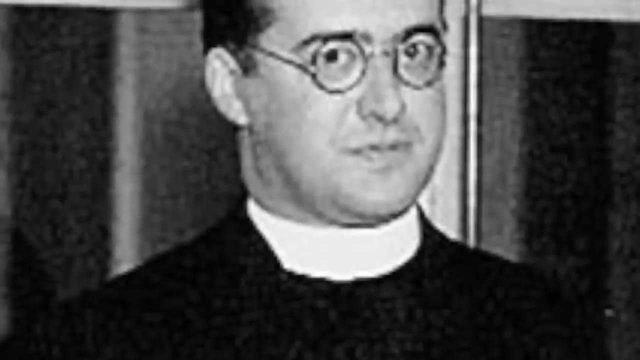 years away, blowing up the universe, but years away, blowing up the universe, but still the galaxy seemed static. a Belgian: still the galaxy seemed static. a Belgian: still the galaxy seemed static. a Belgian physicist. a humble, quaint Belgian physicist. a humble, quaint Belgian physicist. a humble, quaint Belgian physicist who was very interesting. they. 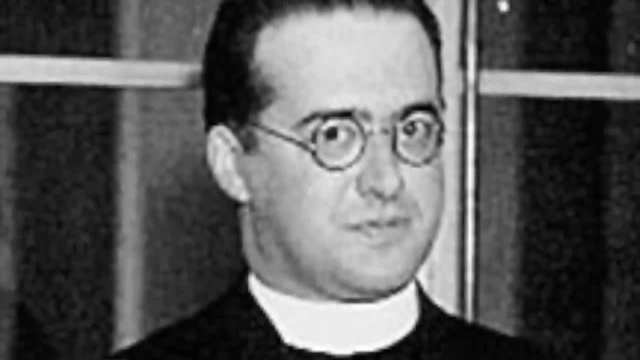 physicist who was very interesting. they physicist who was very interesting. they also also also a Roman Catholic priest named George. a Roman Catholic priest named George, a Roman Catholic priest named George Lamontre. he came into the picture here, Lamontre. he came into the picture here. 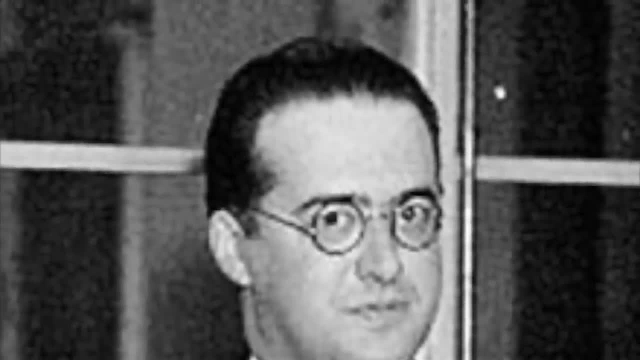 Lamontre. he came into the picture here and he'd preceded Hubble's next and he'd preceded Hubble's next and he'd preceded Hubble's next discovery by a couple years, but he wrote discovery by a couple years. but he wrote discovery by a couple years. but he wrote in some obscure journals and, of course, 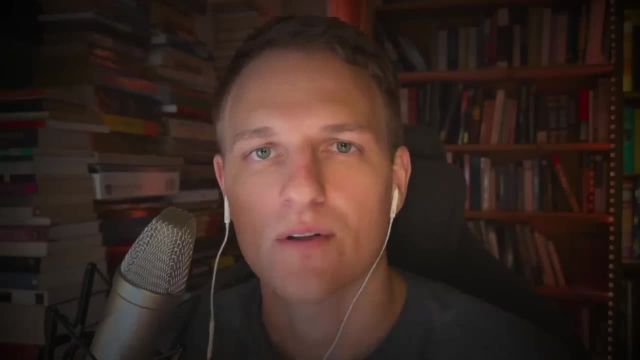 in some obscure journals and of course in some obscure journals and of course non-english language that didn't get non-english language, that didn't get non-english language, that didn't get acknowledged until afterwards. but he acknowledged until afterwards. but he acknowledged until afterwards, but he proved independently of Friedman even. 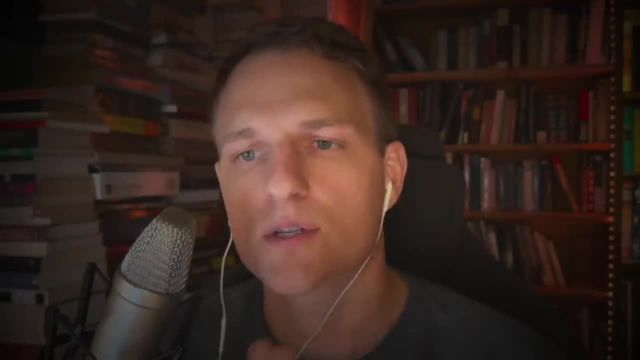 proved independently of Friedman, even proved independently of Friedman, even the even more fringe idea that the, the even more fringe idea that the, the even more fringe idea that the universe wasn't only millions of light, universe wasn't only millions of light, universe wasn't only millions of light years across now, but that it was also. 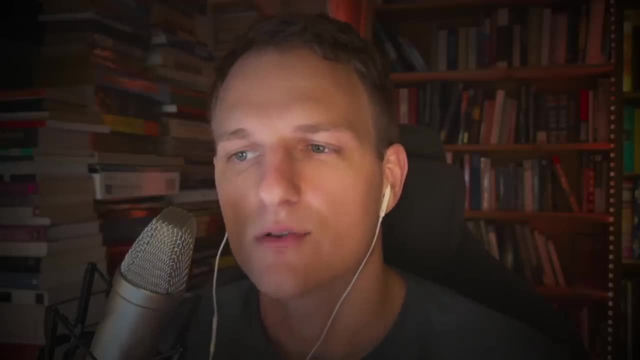 years across now, but that it was also years across now, but that it was also expanding using the equations. he directly expanding using the equations. he directly expanding using the equations. he directly derived from general relativity on his derived from general relativity, on his derived from general relativity on his own. he found a precise relation between 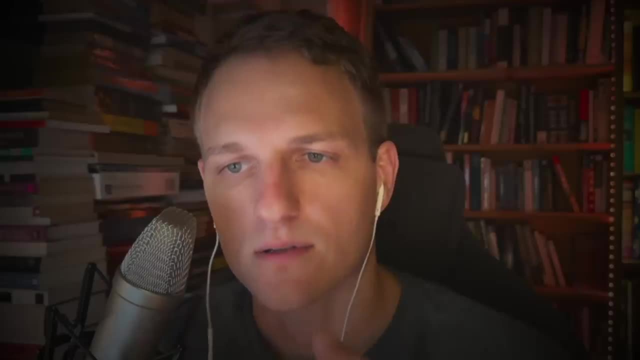 own. he found a precise relation between own. he found a precise relation between these vastly different distant galaxies, these vastly different distant galaxies, these vastly different distant galaxies, in how fast they were receding, and then in how fast they were receding, and then in how fast they were receding, and then, two years later, Hubble built upon. 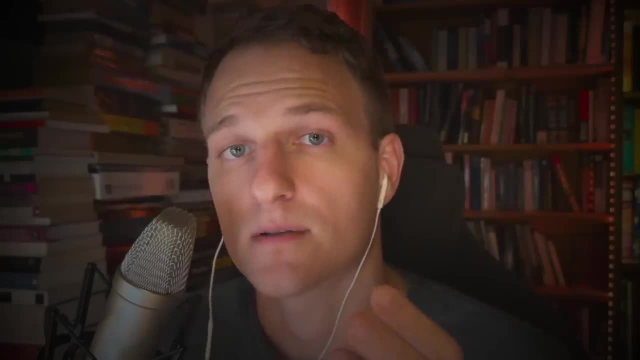 two years later, Hubble built upon. two years later, Hubble built upon slivers work and he provided these slivers work and he provided these slivers work and he provided these detailed observations to prove these detailed observations, to prove these detailed observations, to prove these ideas. he noticed that these newly 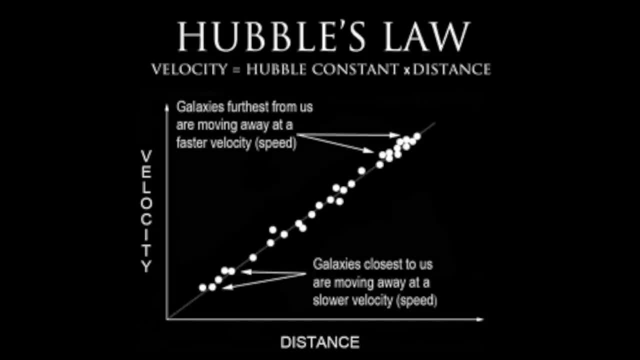 ideas. he noticed that these newly ideas, he noticed that these newly discovered galaxies were in fact discovered. galaxies were in fact discovered. galaxies were in fact redshifted in this, in fact, redshifted in this, in fact, redshifted in this in fact mathematically meant that they were. 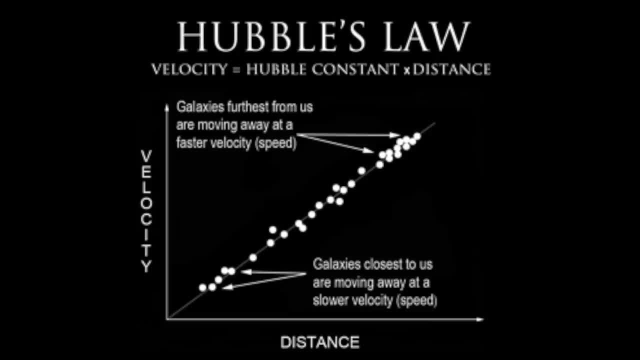 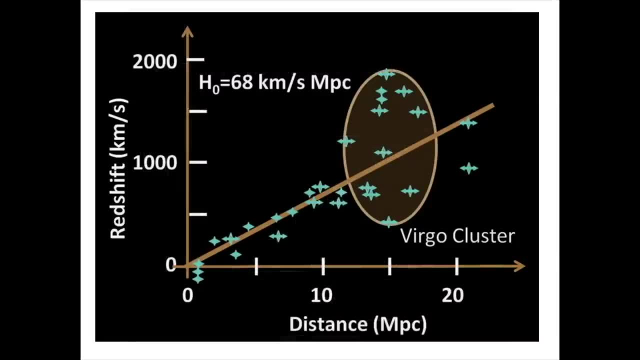 mathematically meant that they were mathematically meant that they were nearly all receding from the earth, that nearly all receding from the earth, that nearly all receding from the earth. that speeds exactly proportional. this is speeds exactly proportional. this is speeds exactly proportional. this is really cool here- to their distances. so 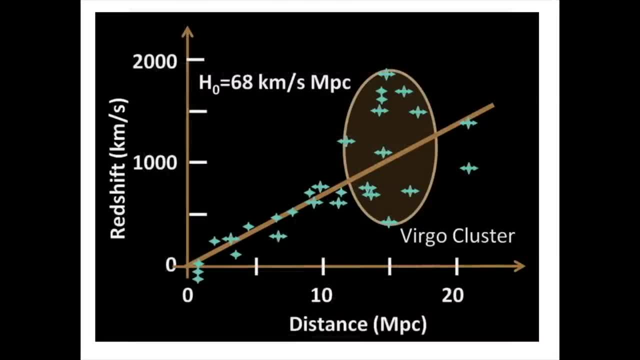 really cool here to their distances. so really cool here to their distances. so that the further you went, the further that, the further you went, the further that. the further you went, the further they appeared to be, the further they they appeared to be, the further they they appeared to be, the further they were were, the faster they were receding. 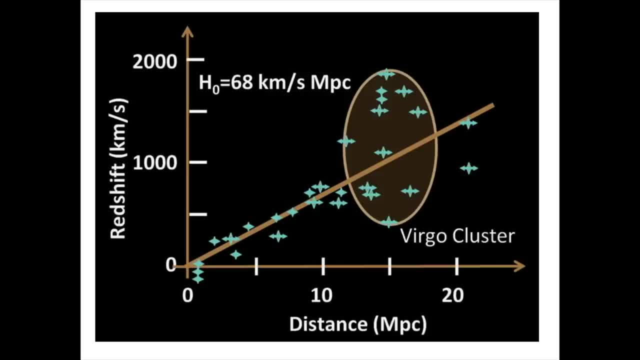 were were the faster they were receding. were were the faster they were receding. so the redshifts were it more and more so. the redshifts were it more and more so. the redshifts were it more and more exaggerated. so this wasn't a case where 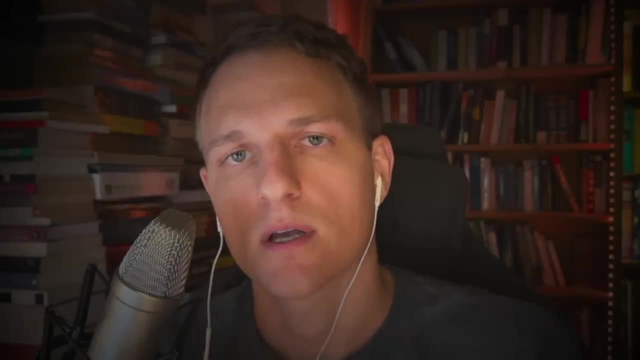 exaggerated so this wasn't a case where exaggerated so this wasn't a case where all galaxies were just receding at equal. all galaxies were just receding at equal. all galaxies were just receding at equal velocities. he was noticing that the velocities, he was noticing that the 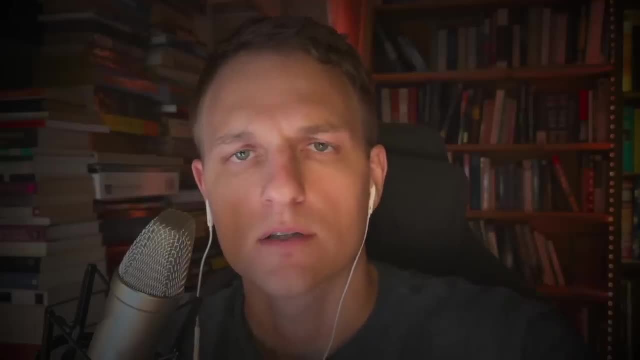 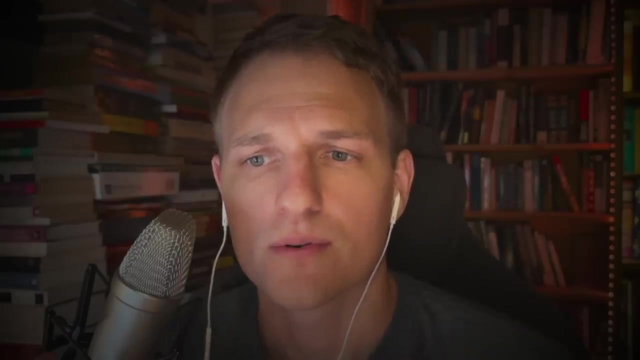 velocities. he was noticing that the further away ones were really going fast, further away ones were really going fast, further away ones were really going fast, and this was kind of hard to believe and and this was kind of hard to believe and and this was kind of hard to believe, and in fact a Hubble didn't even believe it. 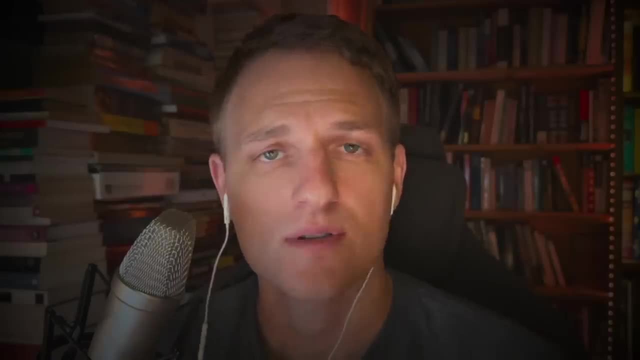 in fact, a Hubble didn't even believe it. in fact, a Hubble didn't even believe it until he, as far as I know, until as far until he, as far as I know, until as far until he, as far as I know, until as far as I read, both him and LaMontre, both. 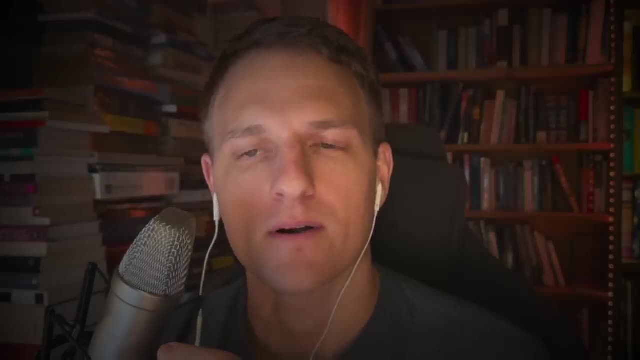 as I read both him and LaMontre both. as I read both him and LaMontre, both they didn't quite. it's kind of like they didn't quite. it's kind of like they didn't quite. it's kind of like Planck and, interestingly, Einstein was the. 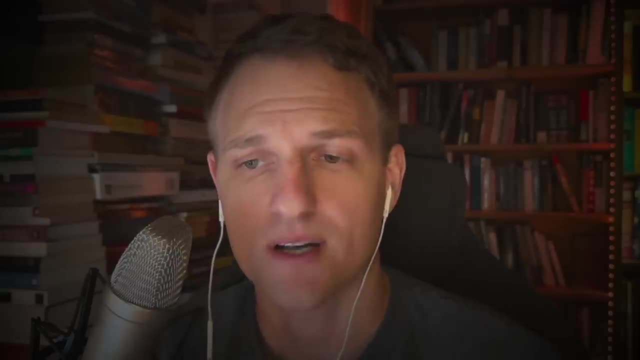 Planck and, interestingly, Einstein was the Planck and, interestingly, Einstein was the one who you know, he kind of latched one who you know, he kind of latched one who you know, he kind of latched onto it. he realized he made a mistake. 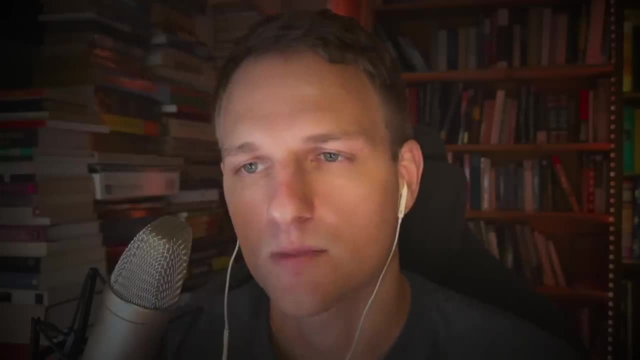 onto it. he realized he made a mistake. onto it. he realized he made a mistake trying to correct and make his universe, trying to correct and make his universe, trying to correct and make his universe static with his cosmological constant, static with his cosmological constant, static with his cosmological constant, balancing gravity, because he removed the 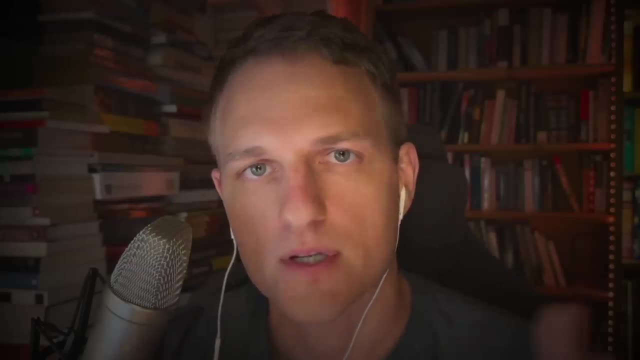 balancing gravity, because he removed the balancing gravity, because he removed the cosmological constant which allowed for cosmological constant, which allowed for cosmological constant, which allowed for the expansion of the universe. but it was the expansion of the universe. but it was the expansion of the universe. but it was interesting that the Hubble and LaMontre 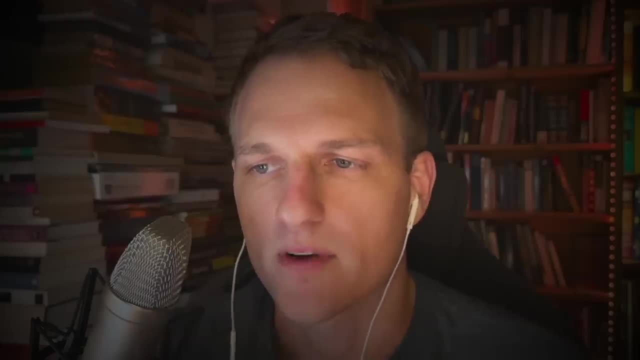 interesting that the Hubble and LaMontre. interesting that the Hubble and LaMontre both they did the math and they even both. they did the math and they even both. they did the math and they even made the observations, but they couldn't made the observations, but they couldn't. 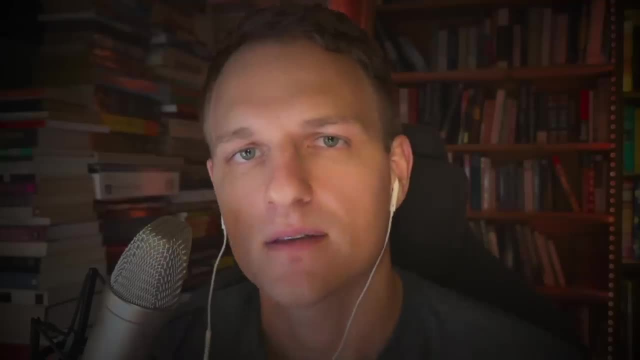 made the observations, but they couldn't quite come to terms with the fact that quite come to terms with the fact that quite come to terms with the fact that this might physically mean, or this might, this might physically mean, or this might this might physically mean, or this might actually mean, the galaxies were. 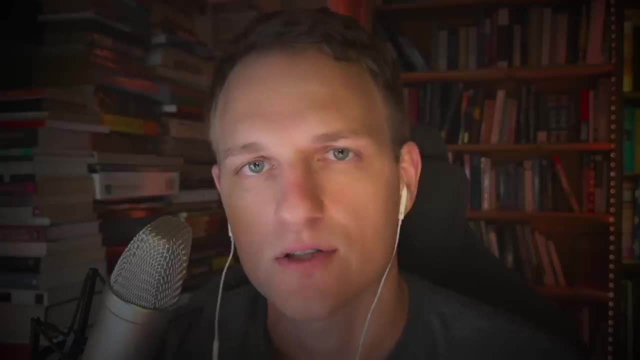 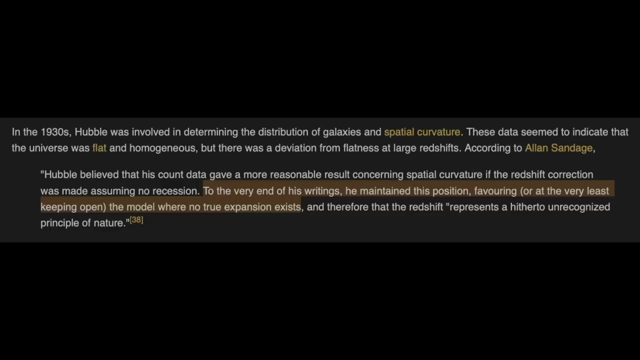 actually mean the galaxies were actually mean. the galaxies were physically receding away from us, like physically receding away from us, like physically receding away from us, like that, just in all directions. it's thought that, just in all directions. it's thought that just in all directions. it's thought even from at the end: he, he still. 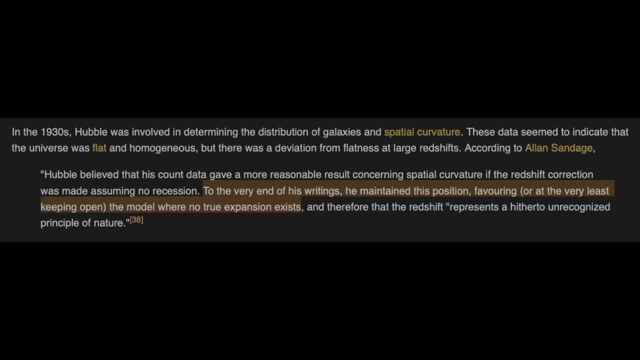 even from at the end, he, he still. even from at the end he, he still considered them just apparent velocities, considered them just apparent velocities, considered them just apparent velocities. he, he thought there was as of yet a he, he thought there was as of yet a. he, he thought there was as of yet a still undiscovered phenomenon, like some. 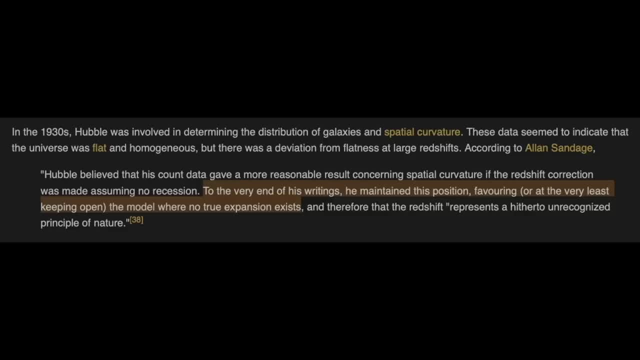 still undiscovered phenomenon, like some. still undiscovered phenomenon, like some. some reason other than the actual, some reason other than the actual, some reason other than the actual galaxies running away from us? that could galaxies running away from us, that could galaxies running away from us that could explain why their lines were so red? 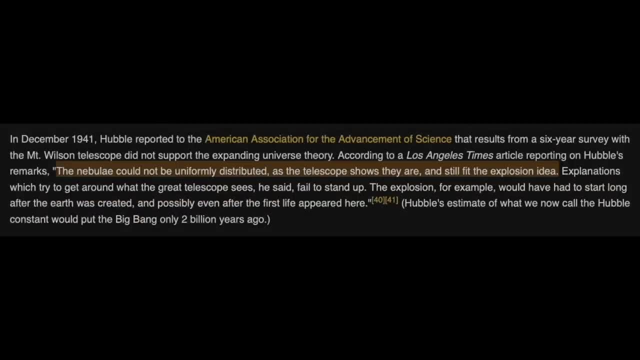 explain why their lines were so red. explain why their lines were so red. shifted like that. and in 1941 Hubble shifted like that. and in 1941, Hubble shifted like that. and in 1941 Hubble reported to the American Association for. reported to the American Association for. 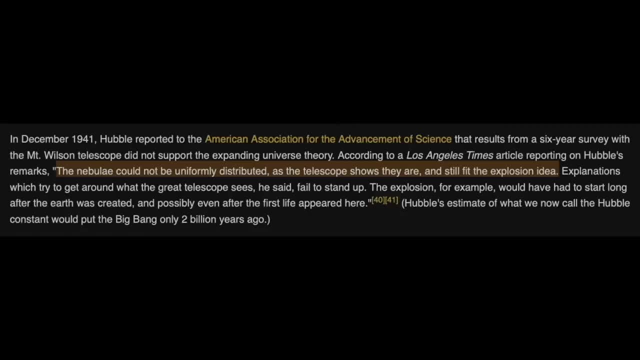 reported to the American Association for the advancement of science. results from the advancement of science, results from the advancement of science, results from a six-year survey at the Mount Wilson, a six-year survey at the Mount Wilson, a six-year survey at the Mount Wilson telescope. in fact, his own results, his 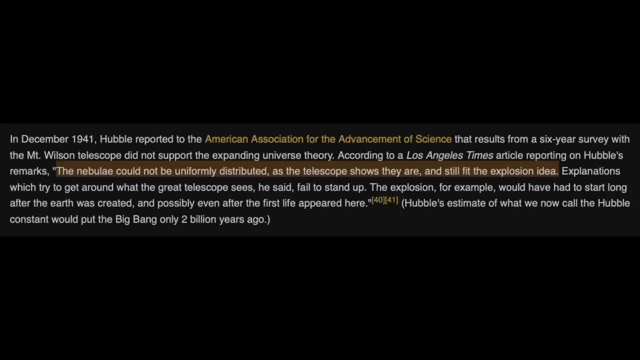 telescope, in fact his own results, his telescope, in fact his own results, his own data did not support the expanding own data, did not support the expanding own data, did not support the expanding universe theory, but meanwhile, like I, universe theory, but meanwhile, like I, universe theory, but meanwhile, like I said, Einstein grasped fairly quickly that. 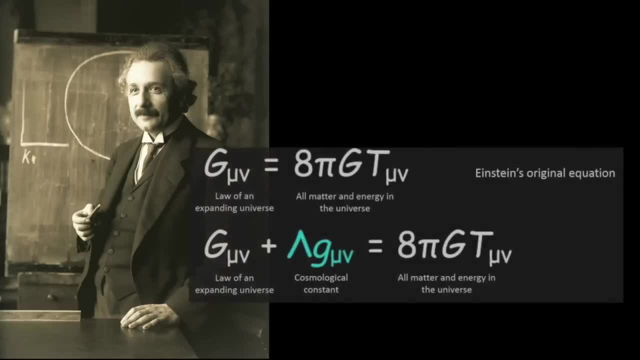 said, Einstein grasped fairly quickly. that said, Einstein grasped fairly quickly that he'd made what he even called his. he'd made what he even called his. he'd made what he even called his greatest blunder by simply not predicting greatest blunder, by simply not predicting. 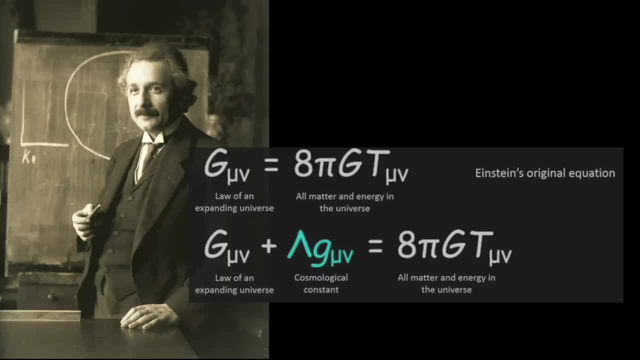 greatest blunder by simply not predicting the expansion as his equations showed. the expansion as his equations showed. the expansion as his equations showed him and predicted so they, they either him and predicted so they, they, either him and predicted so they, they either predicted. it was basically like a static. 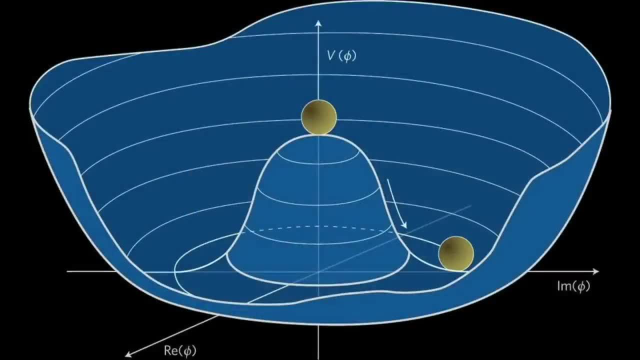 predicted it was basically like a static. predicted it was basically like a static universe would have been the ball universe would have been the ball universe would have been the ball sitting on a hill and it would have sitting on a hill and it would have sitting on a hill and it would have either had to, inevitably it wasn't. 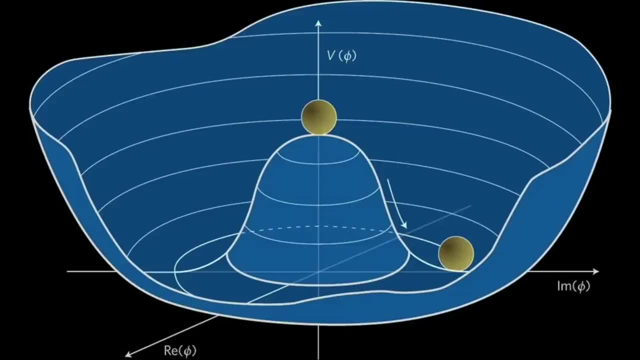 either had to inevitably it wasn't, either had to inevitably. it wasn't natural for that ball to just stay there. natural for that ball to just stay there. natural for that ball to just stay there. it was a very unstable situation, and so it was a very unstable situation, and so 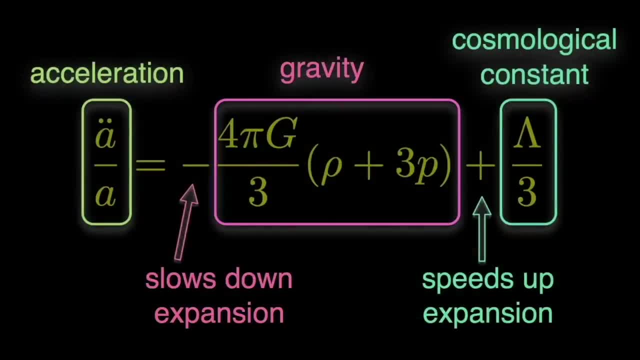 it was a very unstable situation, and so he, Einstein's equation, said that it's he Einstein's equation said that it's. he Einstein's equation said that it's either gonna roll this way and everything, either gonna roll this way and everything. either gonna roll this way and everything would collapse, or it would roll. 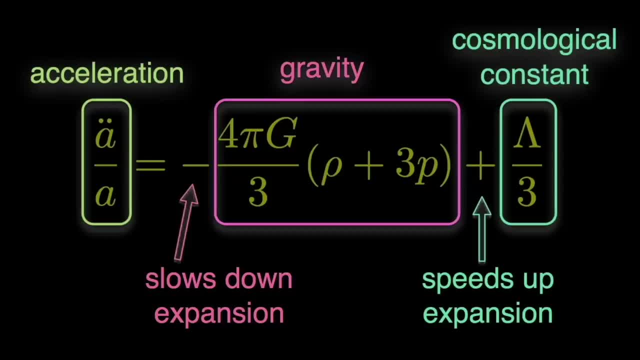 would collapse or it would roll. would collapse or it would roll this way and everything would be naturally this way and everything would be naturally this way and everything would be naturally just expanding. and so he felt just expanding. and so he felt just expanding and so he felt like it was: ah, such a, you know, such a missed. 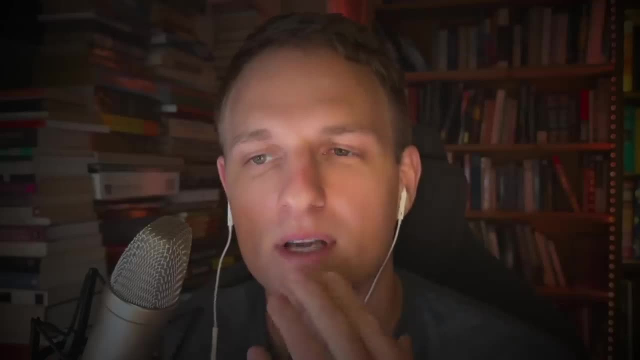 like it was- ah, such a, you know such a missed. like it was- ah, such a you know such a missed opportunity, but within a few years opportunity. but within a few years opportunity, but within a few years. this 2,000 year old belief in a static 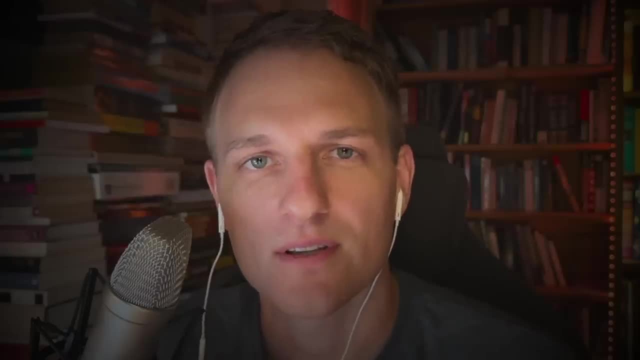 this 2,000 year old belief in a static, this 2,000 year old belief in a static universe, perfect and timeless, was universe, perfect and timeless, was universe, perfect and timeless, was shattered and it was now accepted fact. shattered and it was now accepted fact. 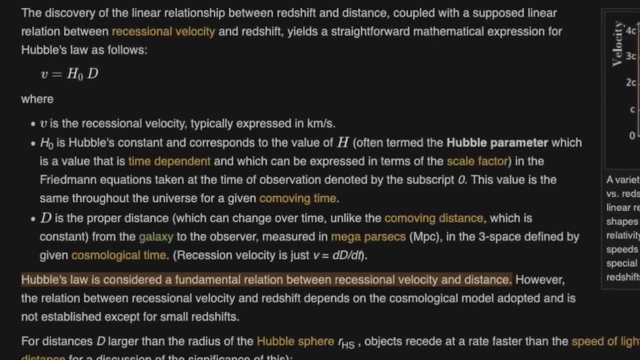 shattered and it was now accepted. fact: this equation combined with the, this equation combined with the, this equation combined with the well-fitting Friedman equations- Hubble's well-fitting Friedman equations, Hubble's well-fitting Friedman equations. Hubble's equation was basically: it was basically a. 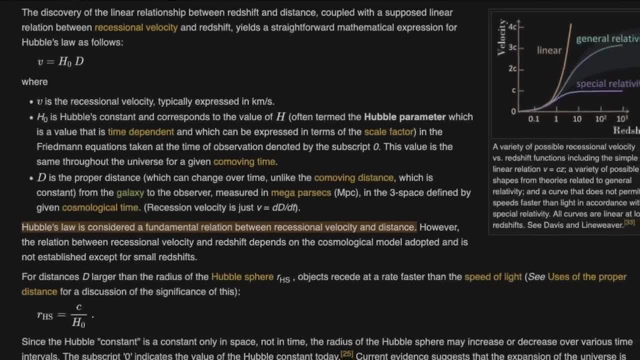 equation was basically: it was basically a equation was basically: it was basically a linear relationship, showing that linear relationship, showing that linear relationship, showing that velocity increased with distance. it velocity increased with distance, it velocity increased with distance. it cemented the theory of the expanding, cemented the theory of the expanding. 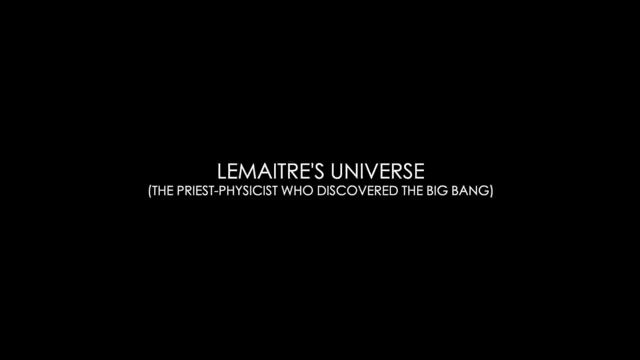 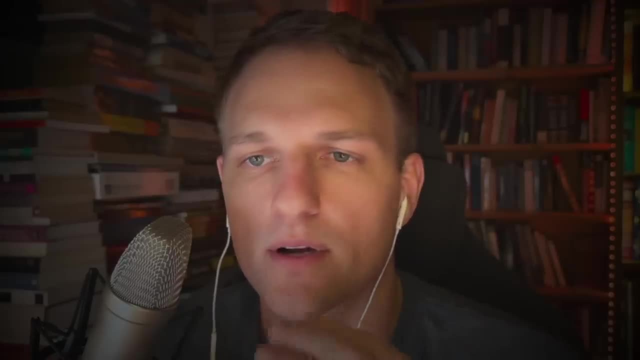 cemented the theory of the expanding universe. but what's interesting about Arthur key? but what's interesting about Arthur key? but what's interesting about Arthur key figure here, LaMontre was that he wasn't figure here. LaMontre was that he wasn't figure here. LaMontre was that he wasn't done. novel had shown that the distance. 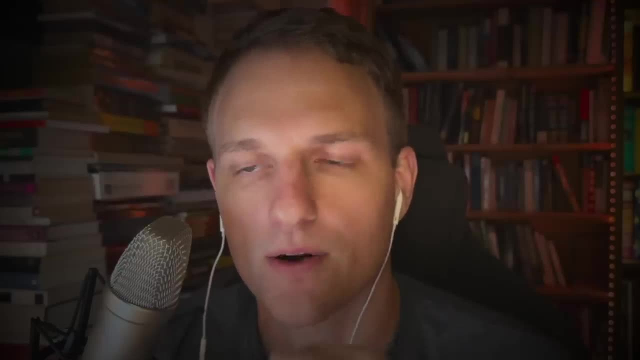 done novel had shown that the distance done novel had shown that the distance to galaxies were way further than sitting to galaxies were way further than sitting to galaxies were way further than sitting nearby our stars. and he, whether he nearby our stars and he, whether he nearby our stars and he, whether he believed it or not, he showed that the 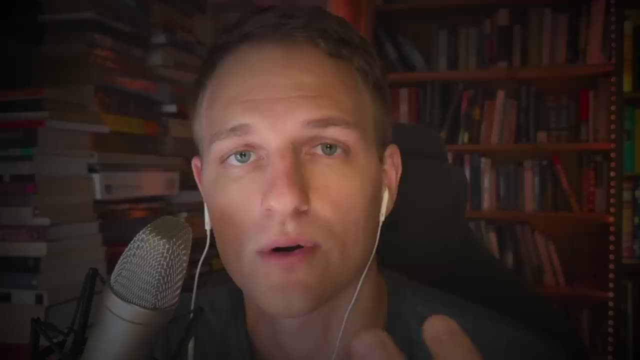 believed it or not, he showed that, the believed it or not, he showed that the universe in those galaxies, those distant universe in those galaxies, those distant universe in those galaxies, those distant galaxies were not only distant, but they galaxies were not only distant, but they galaxies were not only distant, but they were continuing to expand away from us. 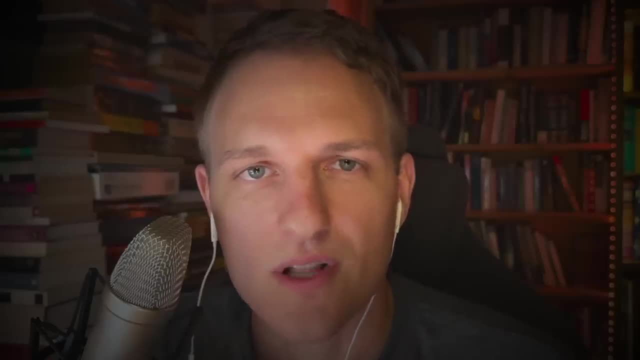 were continuing to expand away from us, were continuing to expand away from us, but LaMontre was still at it. he was a he, but LaMontre was still at it. he was a he, but LaMontre was still at it. he was a. he was a Roman Catholic priest. I can't get. 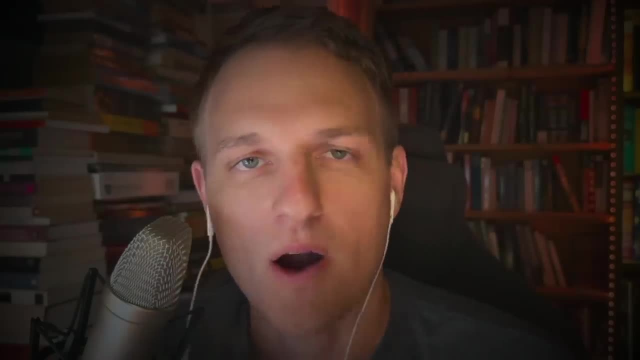 was a Roman Catholic priest I can't get was a Roman Catholic priest. I can't get this out of my head that he, he would this out of my head, that he, he would this out of my head, that he, he would have been inspired from a religious. 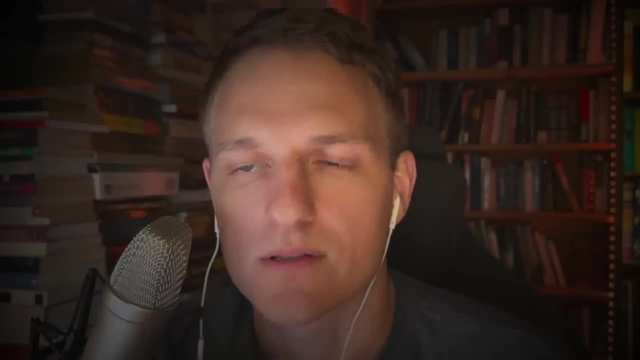 have been inspired from a religious, have been inspired from a religious perspective, to keep pursuing these perspective. to keep pursuing these perspective, to keep pursuing these cosmological ideas and, within two years, cosmological ideas and within two years, cosmological ideas and within two years of him and Hubble, you know, predicting. 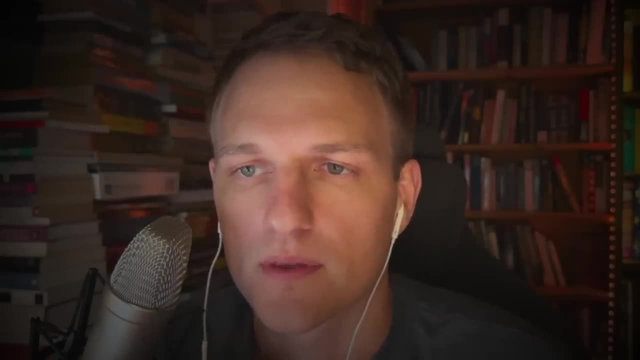 of him and Hubble you know. predicting of him and Hubble, you know. predicting and discovering the expansion of the and discovering the expansion of the and discovering the expansion of the universe, or the expansion of the universe or the expansion of the universe or the expansion of the recession of these galaxies away from us. 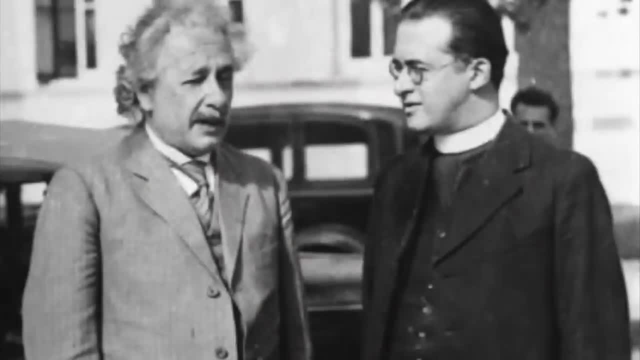 recession of these galaxies away from us. recession of these galaxies away from us in 1931. it was a breakthrough year, for in 1931 it was a breakthrough year for in 1931, it was a breakthrough year for Lemaitre and, along with Friedman, who'd 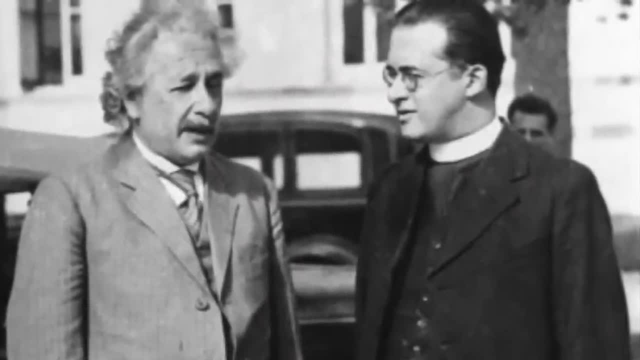 Lemaitre, and along with Friedman, who'd Lemaitre, and along with Friedman, who'd since died. he'd finally received some since died. he'd finally received some since died. he'd finally received some recognition for pioneering. a recognition for pioneering, a recognition for pioneering a relativistic cosmology which explained. 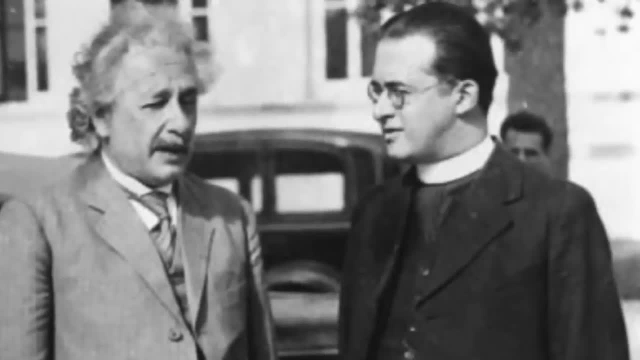 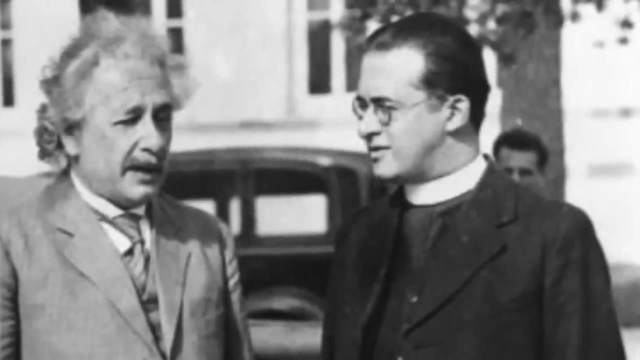 relativistic cosmology, which explained relativistic cosmology, which explained the observed redshifts of an expanding the observed redshifts of an expanding the observed redshifts of an expanding universe. but he pushed this idea, even universe. but he pushed this idea, even universe. but he pushed this idea even further. he explained it as this: this: 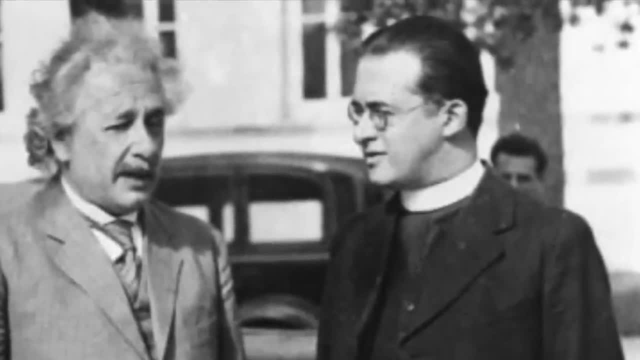 further, he explained it as this: this further, he explained it as this: this flow of energy, this flow of space, that flow of energy, this flow of space, that flow of energy, this flow of space that would have been repelling the galaxies, would have been repelling the galaxies. 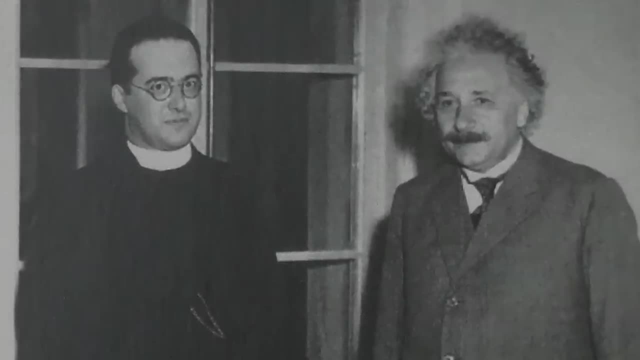 would have been repelling the galaxies away from one another, and he suggested away from one another. and he suggested away from one another. and he suggested that maybe this was evidence that if you that maybe this was evidence that, if you that maybe this was evidence that if you ran the projector backwards in time, 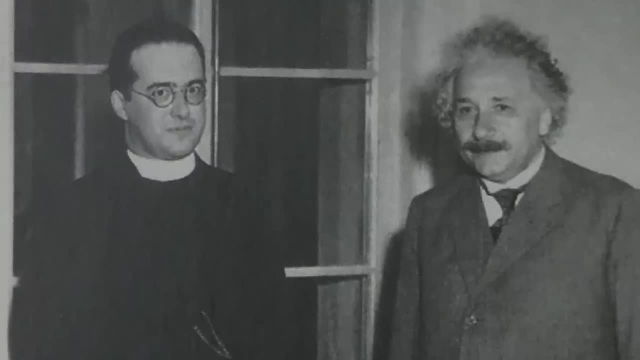 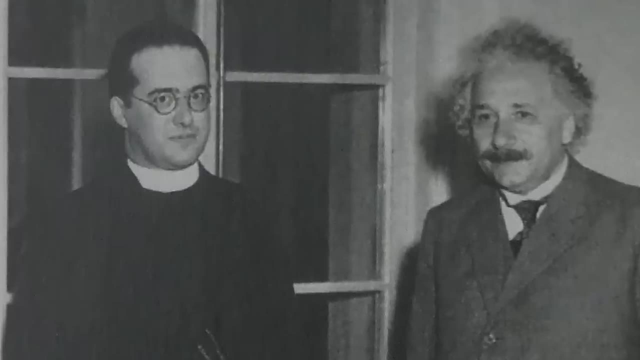 ran the projector backwards in time. ran the projector backwards in time, this expansion of space repulsion would this expansion of space repulsion would this expansion of space repulsion would turn into a gravitational attractor, turn into a gravitational attractor, turn into a gravitational attractor, meaning that there might be an initial 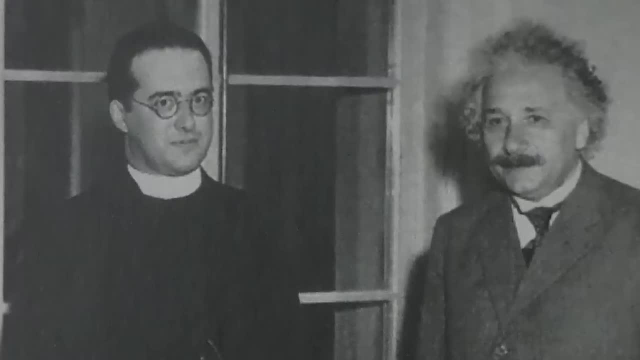 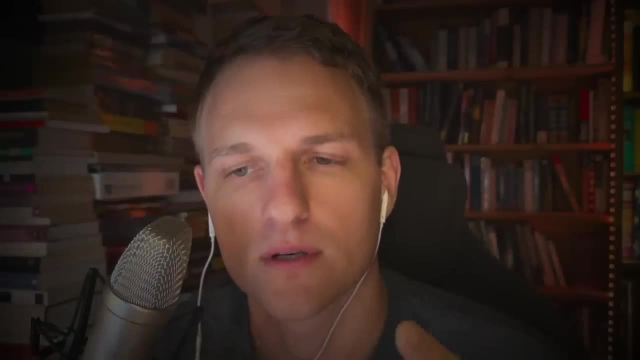 meaning that there might be an initial meaning, that there might be an initial creation like event. things would have creation like event. things would have creation like event. things would have gotten closer the universe in aggregate gotten closer the universe in aggregate gotten closer, the universe in aggregate would have heated up and they ultimately 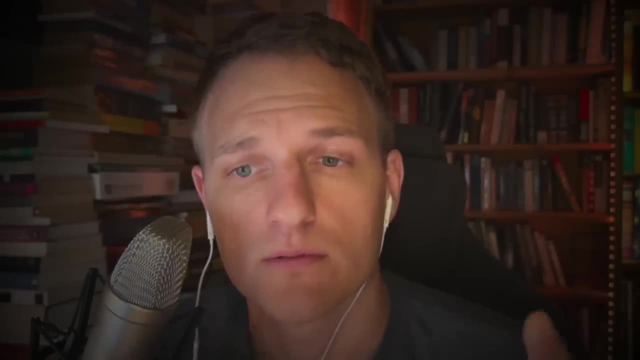 would have heated up and they ultimately would have heated up and they ultimately all matter. then, ultimately, all matter, all matter, then, ultimately all matter, all matter, then ultimately all matter would have coalesced and superimposed at, would have coalesced and superimposed at. 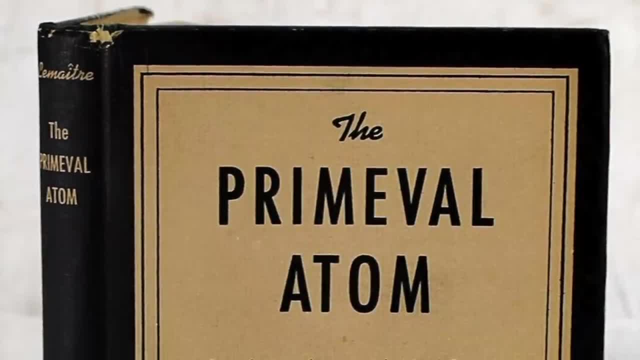 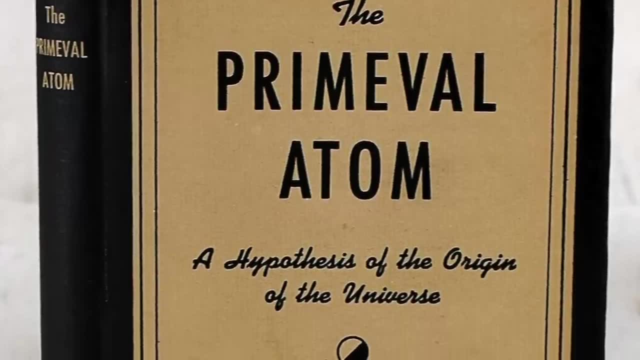 would have coalesced and superimposed at some singular, what he called primeval, some singular what he called primeval, some singular what he called primeval point, some primeval atom, and this in the point, some primeval atom, and this in the point, some primeval atom. and this, in the early 30s, was the first speculation. 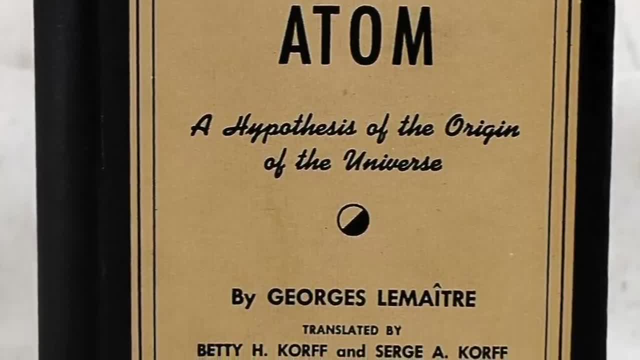 early 30s was the first speculation. early 30s was the first speculation about the Big Bang. we can tell our track about the Big Bang. we can tell our track about the Big Bang. we can tell our track record by now with Copernicus Newton. 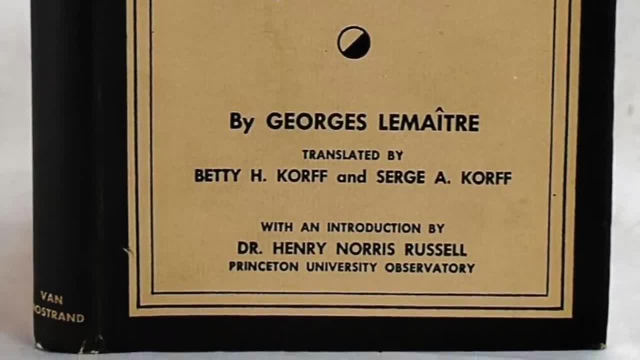 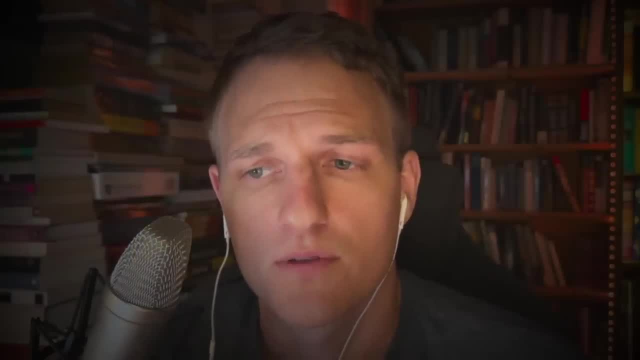 record by now with Copernicus Newton. record by now with Copernicus Newton, Einstein, Apple. the community wasn't Einstein Apple. the community wasn't Einstein Apple. the community wasn't eager to embrace this and it took almost eager to embrace this. and it took almost eager to embrace this, and it took almost 30 years for them all to finally grasp. 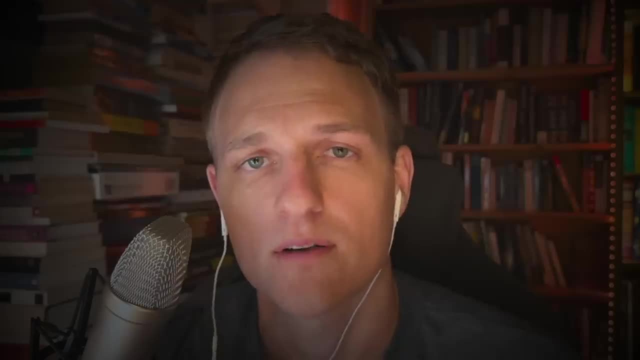 30 years for them all to finally grasp. 30 years for them all to finally grasp the implications and the fact that, okay, the implications and the fact that, okay, the implications and the fact that, okay, there was evidence of this and we'll be. there was evidence of this and we'll be. 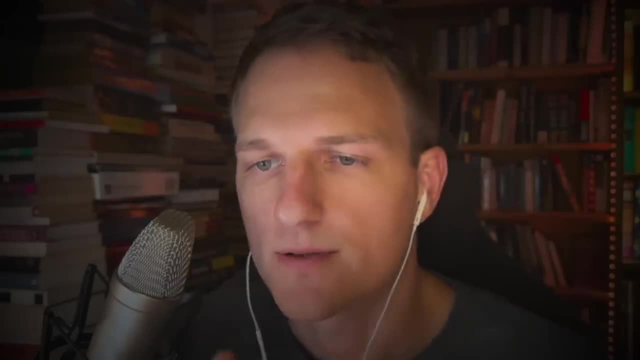 there was evidence of this and we'll be talking about that in a minute here, and talking about that in a minute here, and talking about that in a minute here, and it's hard to imagine that this wasn't. it's hard to imagine that this wasn't. 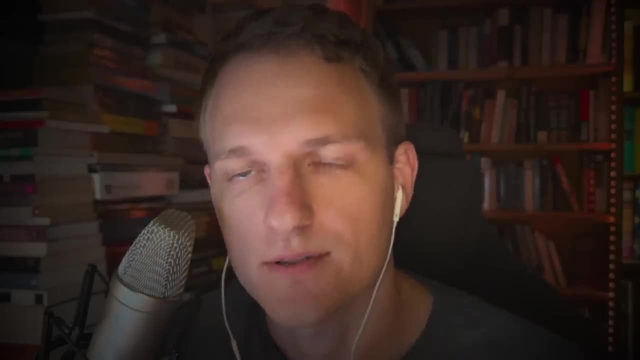 it's hard to imagine that this wasn't because he was a priest. he had some. because he was a priest, he had some. because he was a priest he had some religious inclination, and I think that's religious inclination, and I think that's religious inclination and I think that's a beautiful thing. because, well, I don't. 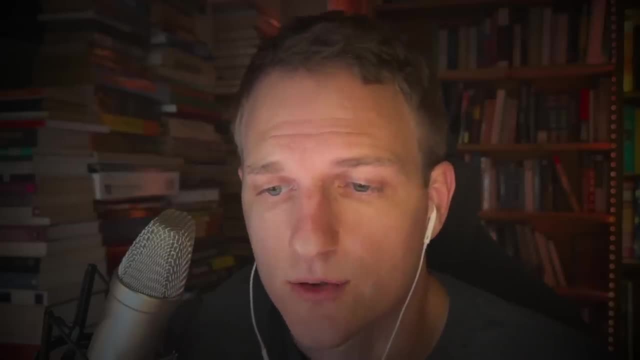 a beautiful thing because, well, I don't a beautiful thing because, well, I don't think it necessarily goes against. think it necessarily goes against, think it necessarily goes against creation like event. but you know creation like event, but you know creation like event, but you know, regardless, I, I, I don't want to. 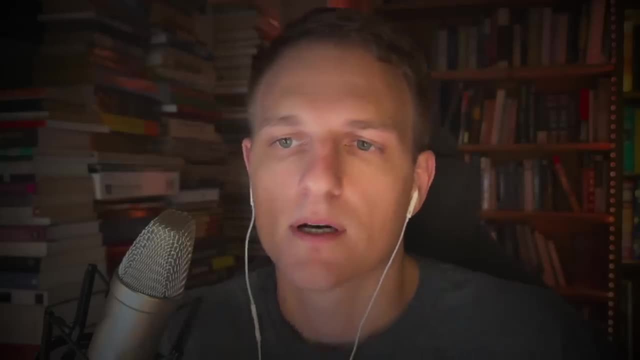 regardless I, I, I don't want to, regardless I, I, I don't want to oversimplify it. I don't think it is that oversimplify it. I don't think it is that oversimplify it. I don't think it is that simple and it doesn't even mean that the 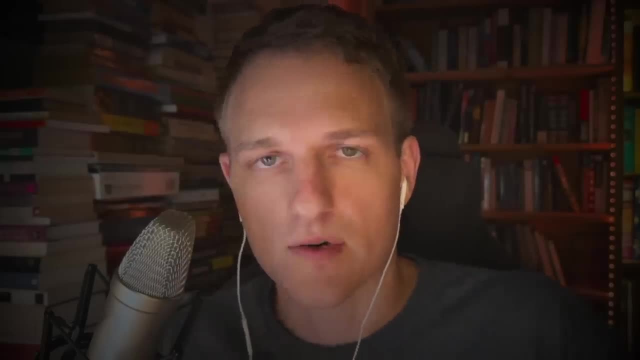 simple, and it doesn't even mean that the simple and it doesn't even mean that the Big Bang was the only iteration of the Big Bang, was the only iteration of the Big Bang was the only iteration of the universe. nonetheless, it's fascinating universe. nonetheless, it's fascinating. 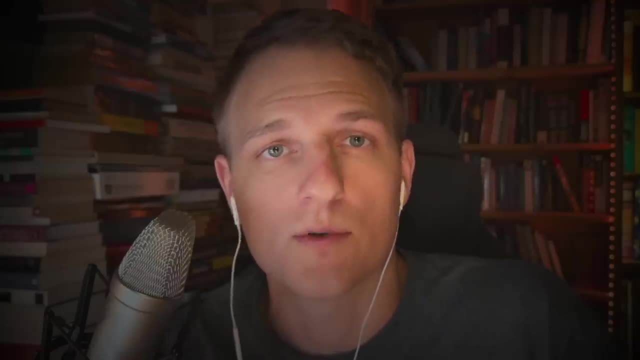 universe. nonetheless, it's fascinating that the universe isn't this. you know that the universe isn't this. you know that the universe isn't this. you know, kind of almost dull perfect, infinitely. kind of almost dull perfect infinitely. kind of almost dull perfect, infinitely. static, steady-state thing it actually is. 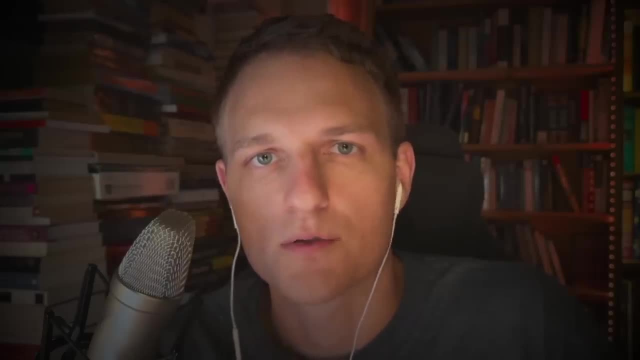 static, steady-state thing. it actually is static, steady-state thing. it actually is very dynamic. it exploded from some very dynamic. it exploded from some very dynamic. it exploded from some point. it was much hotter. it evolved the point. it was much hotter. it evolved the point. it was much hotter, it evolved, the things in it evolved and we're in the 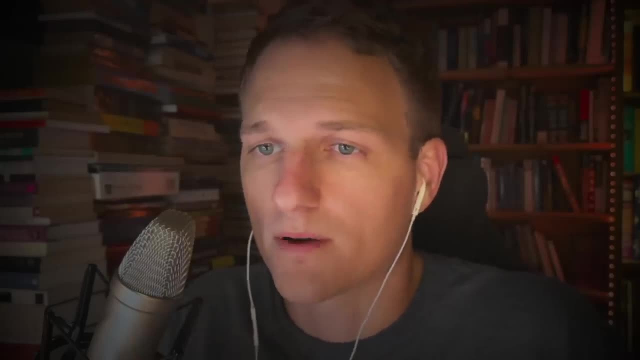 things in it evolved and we're in the things in it evolved and we're in the process of figuring out a whole lot more process of figuring out a whole lot more process of figuring out a whole lot more about it. so then you know, within about about it. so then you know within about. 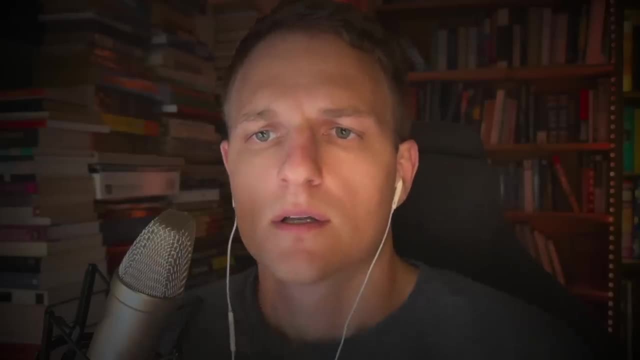 about it. so then you know, within about ten years of that we had. so it's crazy, ten years of that we had. so it's crazy, ten years of that we had. so it's crazy we have within, like within just 20 years. we have within, like within just 20 years. 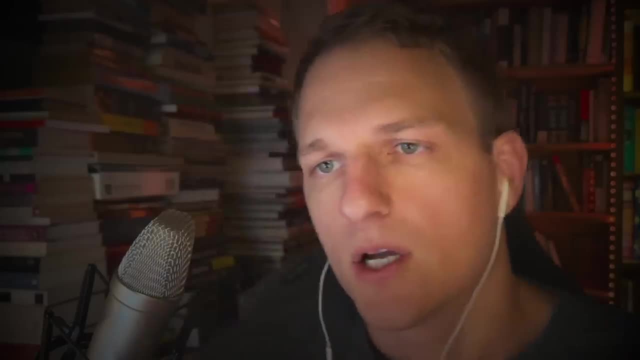 we have within, like within just 20 years. we have Einstein coming out with general. we have Einstein coming out with general. we have Einstein coming out with general relativity, relativity, relativity. we have Hubble discovering the expand. we have Hubble discovering the expand. we have Hubble discovering the expand, the, the, that the universe is these. 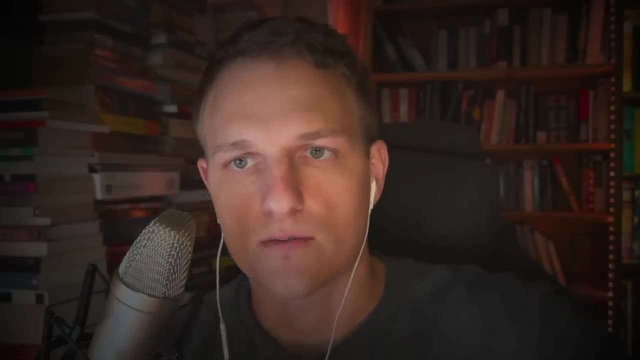 the, the that the universe is, these, the, the that the universe is, these galaxies are lying far outside. these galaxies are lying far outside. these galaxies are lying far outside these local stars of ours. so the universe, local stars of ours, so the universe, local stars of ours, so the universe explodes in size, and then just a couple. 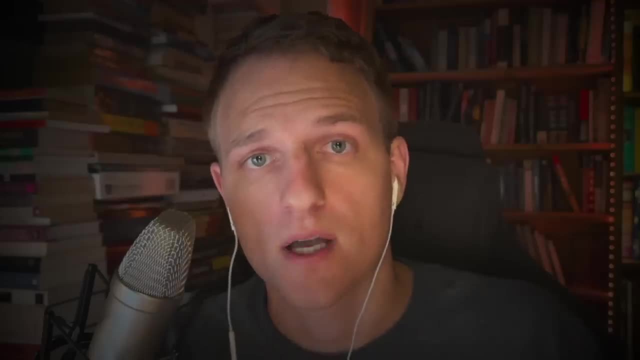 explodes in size and then just a couple explodes in size and then, just a couple years after that, it starts, literally years after that. it starts literally years after that. it starts literally exploding in space in the expansion of exploding in space, in the expansion of exploding in space, in the expansion of space propelling galaxies. apart then, we 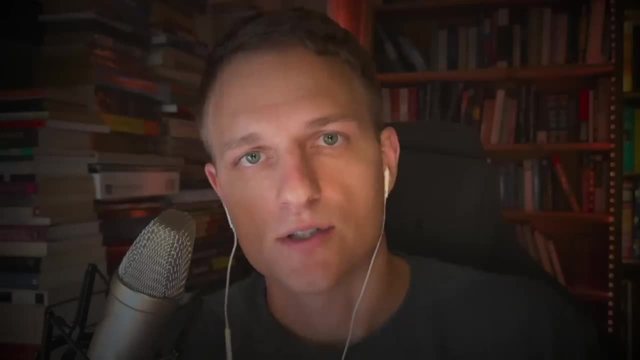 space propelling galaxies apart, then we space propelling galaxies apart, then we have the idea that maybe this expansion, have the idea that maybe this expansion, have the idea that maybe this expansion is the residual momentum of space from. is the residual momentum of space from? is the residual momentum of space from an initial explosion, like creation event. 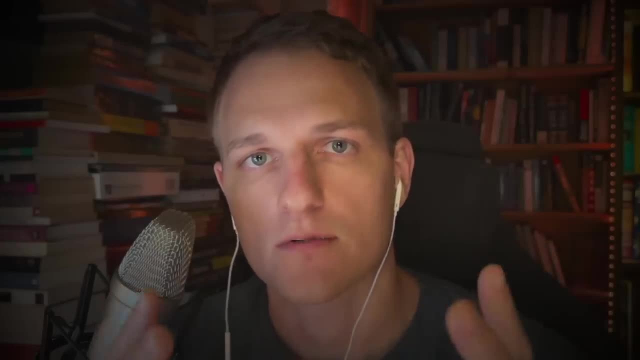 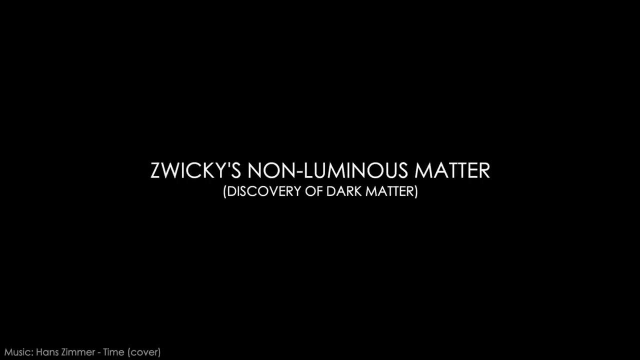 an initial explosion like creation event. an initial explosion like creation event, out of a of all matter and energy, out out of a of all matter and energy, out out of a of all matter and energy, out of a single primeval atom, and then, within just a few years from. 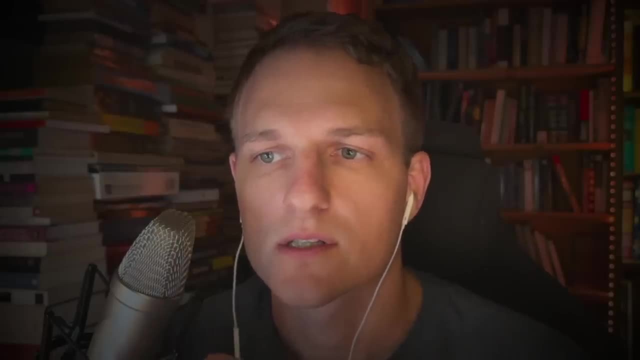 and then within just a few years from, and then within just a few years from this, this Swiss scientist, astronomer, this, this Swiss scientist, astronomer, this: this, this Swiss scientist, astronomer, Fritz Zwicky. in 1937, I was looking at Fritz Zwicky in 1937. I was looking at. 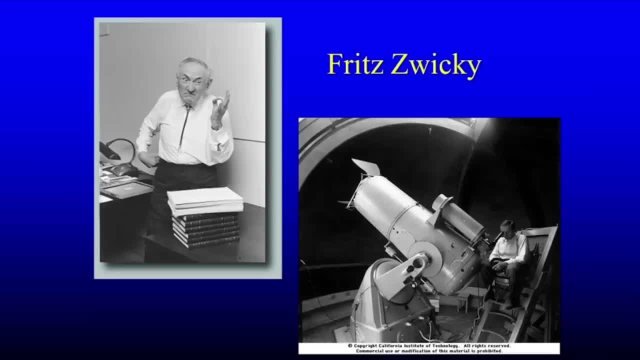 Fritz Zwicky in 1937 I was looking at galaxies and he's looking at spectra and galaxies. and he's looking at spectra and galaxies and he's looking at spectra and observing that they're rotating way, observing that they're rotating way, observing that they're rotating way faster than they ought to be. well, he's. 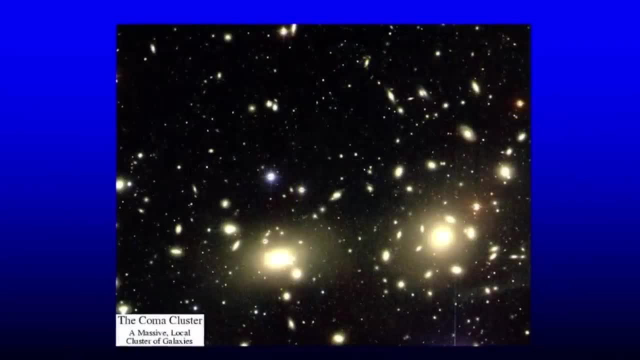 faster than they ought to be. well, he's faster than they ought to be. well, he's looking at clusters, rather he's looking, looking at clusters, rather he's looking. looking at clusters, rather. he's looking at the movement among clusters. he could, at the movement among clusters, he could. 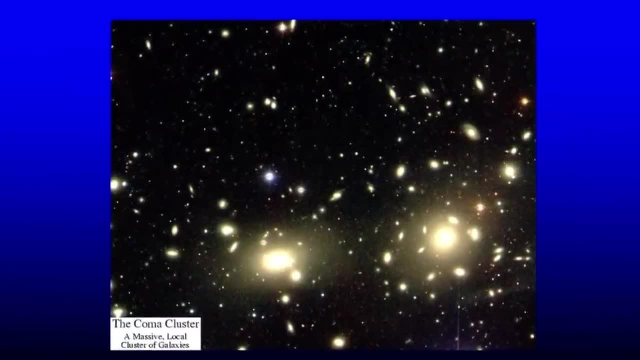 at the movement among clusters. he could see them blue shifting and red shifting. see them blue shifting and red shifting. see them blue shifting and red shifting. or you know less red shifting and more, or you know less red shifting and more, or you know less red shifting and more red shifting, as they swirl around each. 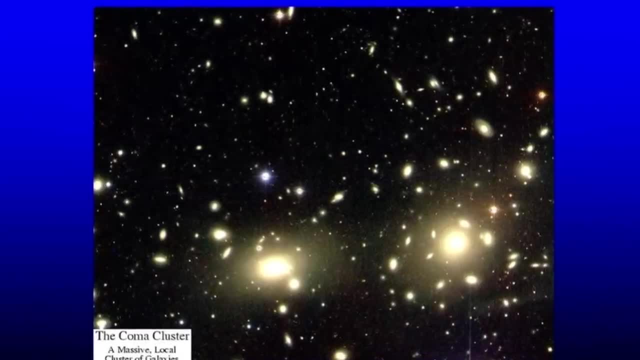 red shifting as they swirl around each red shifting as they swirl around each other. and he's noticing that the other, and he's noticing that the other, and he's noticing that the movements are way, way too much for the movements are way, way too much for the. 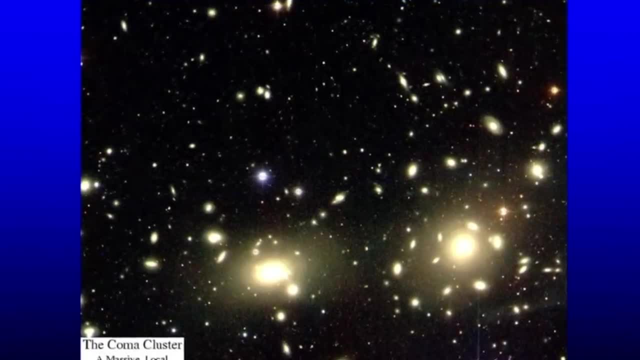 movements are way, way too much for the observed mass here. because spectra of observed mass here, because spectra of observed mass here, because spectra of galaxies look similar to stellar spectra. galaxies look similar to stellar spectra. galaxies look similar to stellar spectra and you know they are the combined light. 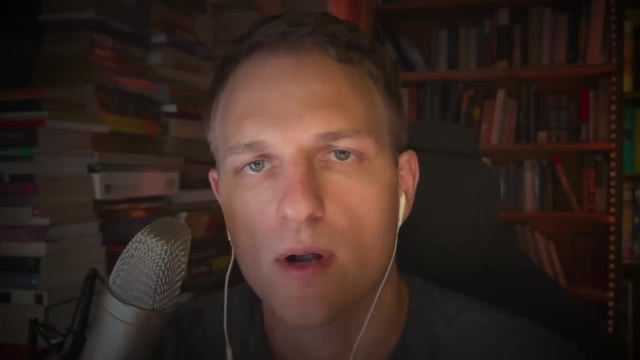 and you know they are the combined light and you know they are the combined light of billions of stars. so you can roughly of billions of stars. so you can roughly of billions of stars. so you can roughly. astronomers are able to. they have some. astronomers are able to, they have some. 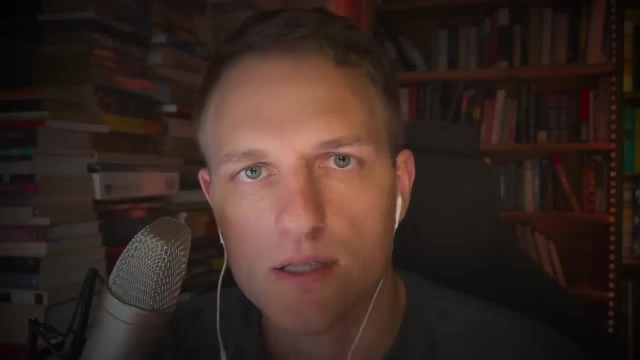 astronomers are able to, they have some methods by which they can estimate the methods by which they can estimate the methods by which they can estimate the rough mass, at least that within a rough mass, at least that within a rough mass, at least that within a magnitude of the right magnitude of 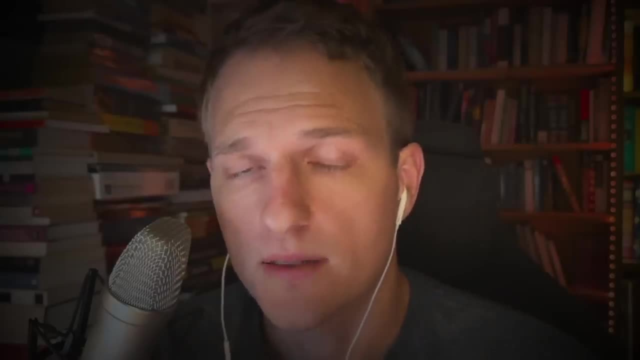 magnitude of the right magnitude of magnitude, of the right magnitude of individual galaxies and these galaxies, individual galaxies, and these galaxies, individual galaxies. and these galaxies weren't obeying that law. they were weren't obeying that law. they were weren't obeying that law. they were removing in such a way that looked like. removing in such a way that looked like removing in such a way that looked like they had they needed at least 20 times they had. they needed at least 20 times they had. they needed at least 20 times more galaxy mass in them, based on the. 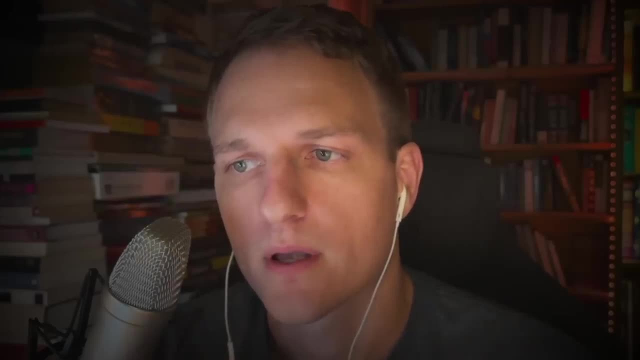 more galaxy mass in them, based on the more galaxy mass in them, based on the gravitational interaction among them and gravitational interaction among them and gravitational interaction among them. and so was Zwicky hypothesized. so was Zwicky hypothesized. so was Zwicky hypothesized, which I'm noticing, all these things. so 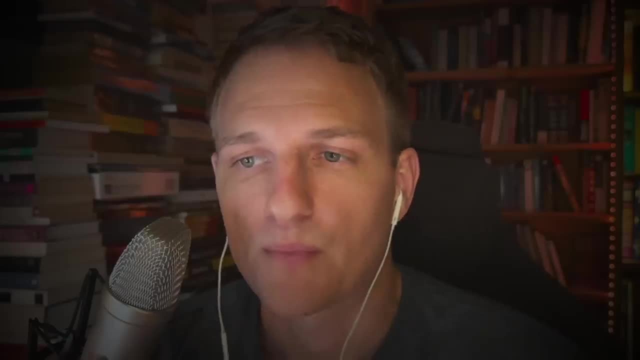 which I'm noticing all these things, so which I'm noticing all these things. so many scientists, and I think rightly so many scientists, and I think rightly so many scientists, and I think rightly so. you shouldn't be eager to speculate. you shouldn't be eager to speculate. 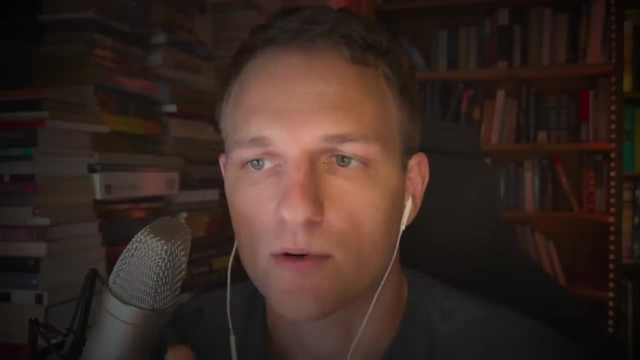 you shouldn't be eager to speculate without proper evidence. and Zwicky was without proper evidence. and Zwicky was without proper evidence. and Zwicky was one of them. he said he was along with a one of them. he said he was along with a one of them. he said he was along with a bunch. he went in in the same manner as 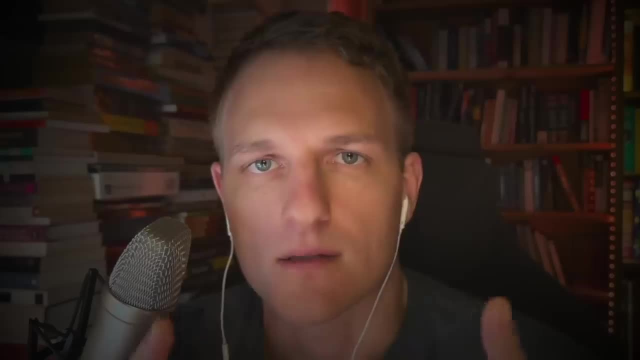 bunch. he went in in the same manner as bunch. he went in in the same manner as the others. you know being reticent to the others. you know being reticent to the others. you know being reticent to think that something exotic or crazy. 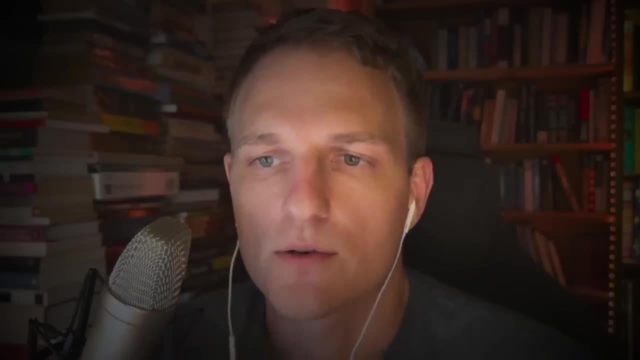 think that something exotic or crazy. think that something exotic or crazy, anomaly is the norm. he says that there, anomaly is the norm. he says that there, anomaly is the norm. he says that there might be just a great deal of non, might be just a great deal of non. 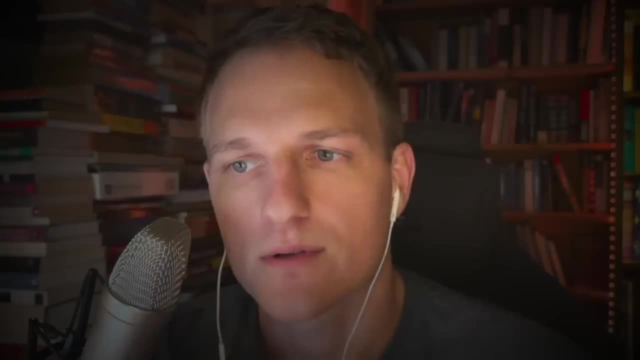 might be just a great deal of non luminous matter in the galaxy clusters, luminous matter in the galaxy clusters, luminous matter in the galaxy clusters, and what he initially meant, I believe, and what he initially meant I believe, and what he initially meant I believe was just, you know, matter that we 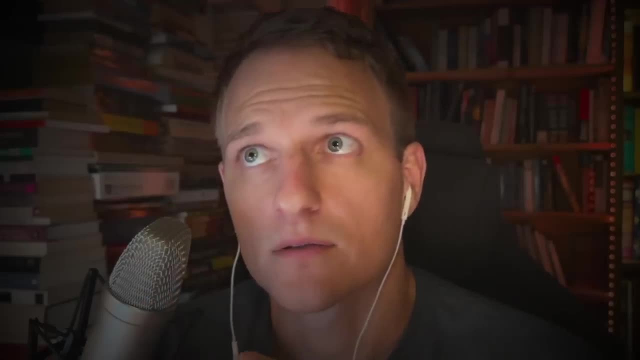 was just, you know, matter that we was just, you know, matter that we couldn't quite see and matter that was couldn't quite see and matter that was couldn't quite see and matter that was probably ordinary matter, but just probably ordinary matter, but just probably ordinary matter, but just invisible in the sense that it wasn't. 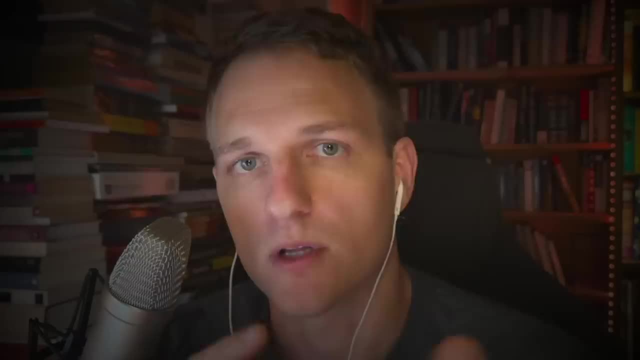 invisible in the sense that it wasn't visible in the sense that it wasn't lit up like stars, so we couldn't quite lit up like stars, so we couldn't quite lit up like stars, so we couldn't quite detect them visibly. but this became: detect them visibly, but this became. 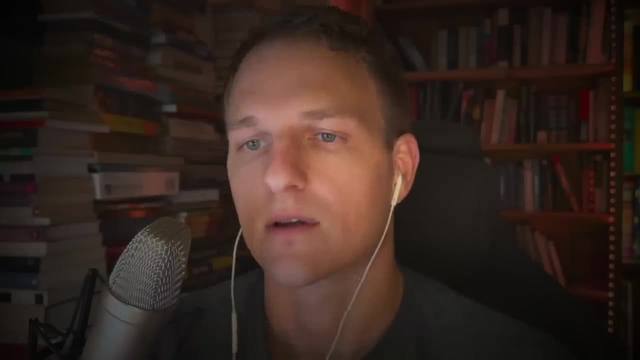 detect them visibly, but this became known as dark matter. this non luminous known as dark matter. this non luminous known as dark matter. this non luminous matter and within about 10 years matter. and within about 10 years matter and within about 10 years, observed dynamics within galaxies. 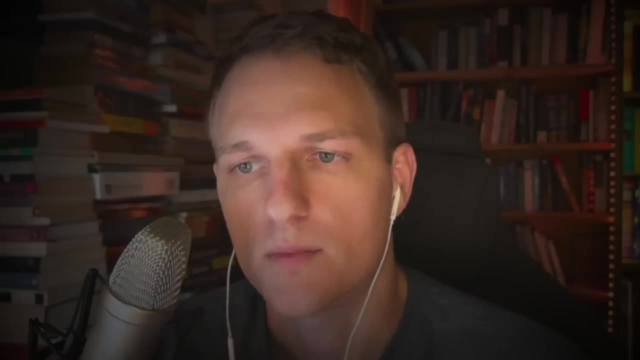 observed dynamics within galaxies. observed dynamics within galaxies everywhere astronomers looked, could be everywhere astronomers looked, could be everywhere astronomers looked. could be explained only if there was way like 10 explained, only if there was way like 10 explained, only if there was way like 10 to 30 times more gravity in them than 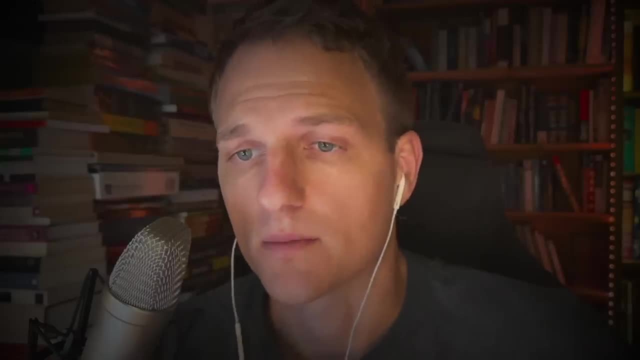 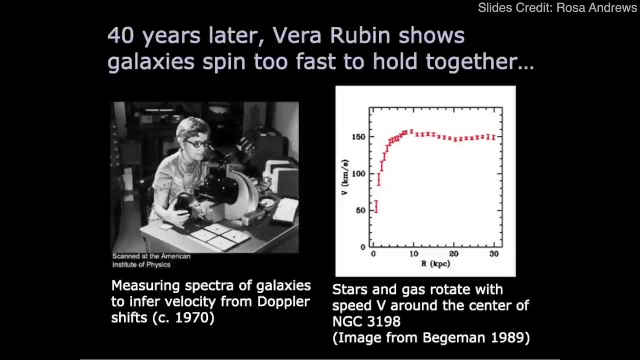 to 30 times more gravity in them than to 30 times more gravity in them than the galaxies. the galaxies: the galaxies. light was showing 40 years later in the light was showing 40 years later in. the light was showing 40 years later in the 70s. scientists even calculated that. 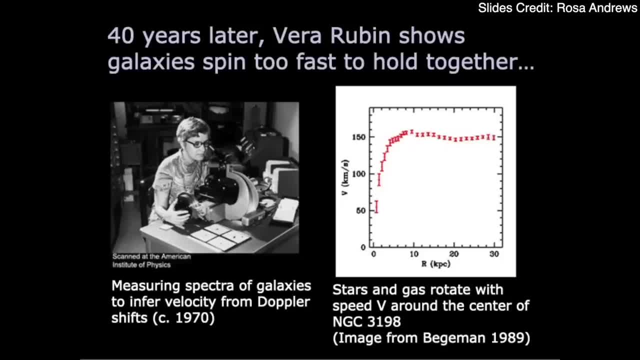 70s scientists even calculated that 70s scientists even calculated that that rotating galactic disks containing that rotating galactic disks containing that rotating galactic disks containing only stars and other material like gas, only stars and other material like gas, only stars and other material like gas and dust and planets- should actually 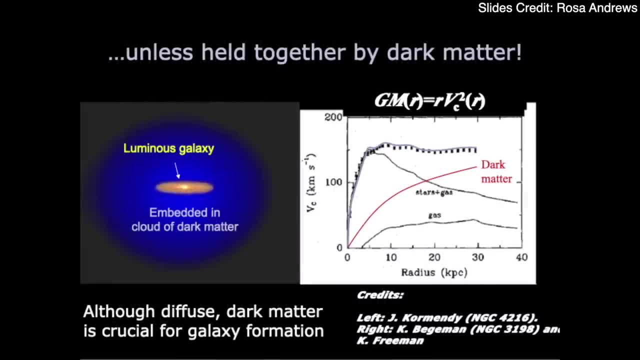 and dust and planets should actually- and dust and planets should actually become unstable and swell into spheres, become unstable and swell into spheres, become unstable and swell into spheres and not be these flat rotating disks and not be these flat rotating disks and not be these flat rotating disks that they are now if they didn't have. 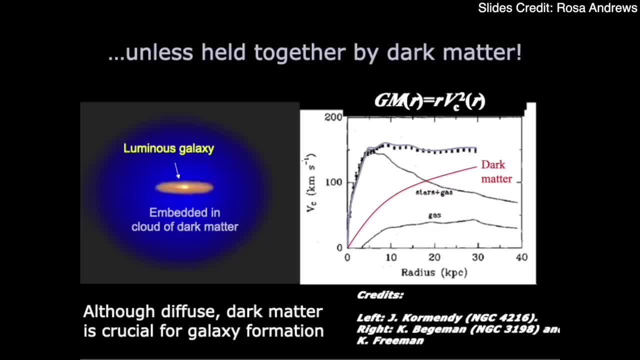 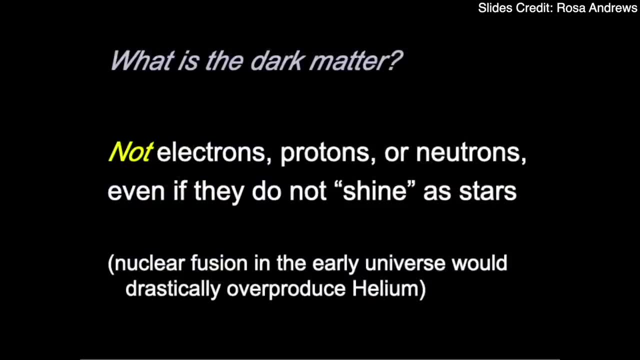 that they are now, if they didn't have that they are now, if they didn't have all this extra gravity in these halos, all this extra gravity in these halos, all this extra gravity in these halos, corralling them into flat disks and so corralling them into flat disks, and so. 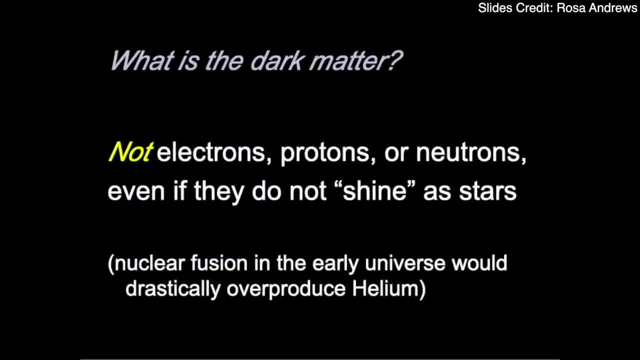 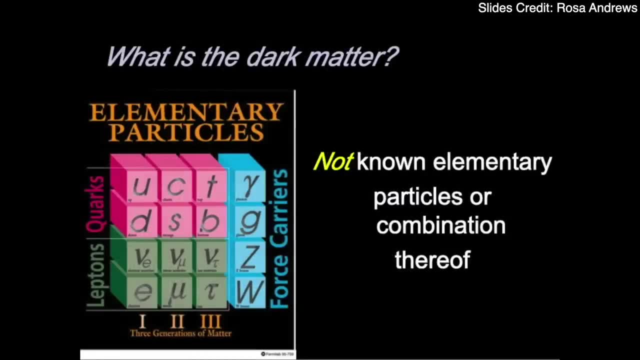 corralling them into flat disks. and so since his discoveries wiki in the 30s, since his discoveries wiki in the 30s, since his discoveries wiki in the 30s, the theory of dark matter has actually the theory of dark matter, has actually the theory of dark matter has actually been a pretty prominent aspect of all. 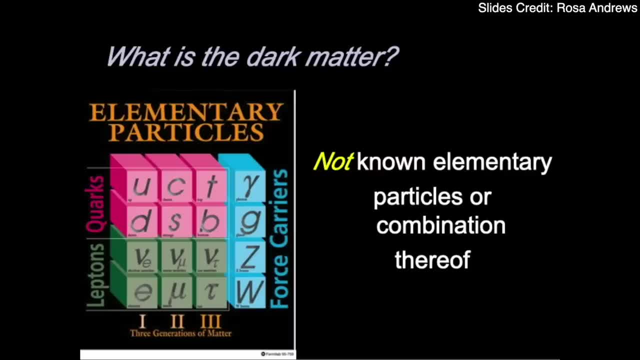 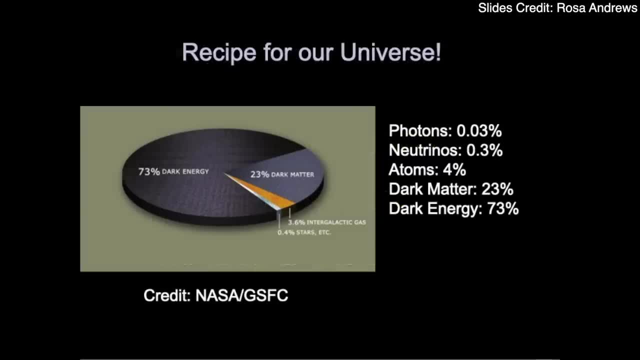 been a pretty prominent aspect of all, been a pretty prominent aspect of all major cosmological models since then. major cosmological models since then, major cosmological models since then. it's a thought that maybe most galaxies, it's a thought that maybe most galaxies, it's a thought that maybe most galaxies and most of the universe, in fact, is made. 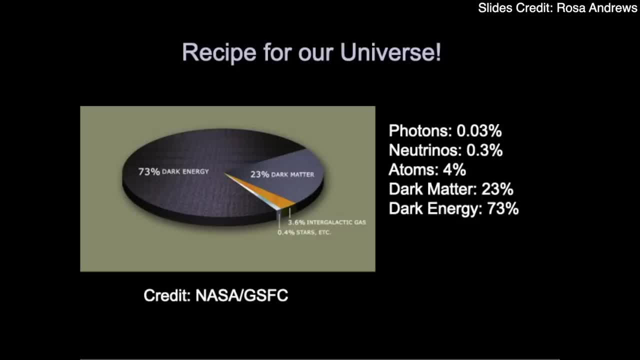 and most of the universe, in fact, is made, and most of the universe, in fact, is made up of dark matter, although interestingly up of dark matter, although interestingly up of dark matter, although, interestingly, I found I came across a 2003 study that I found I came across a 2003 study that 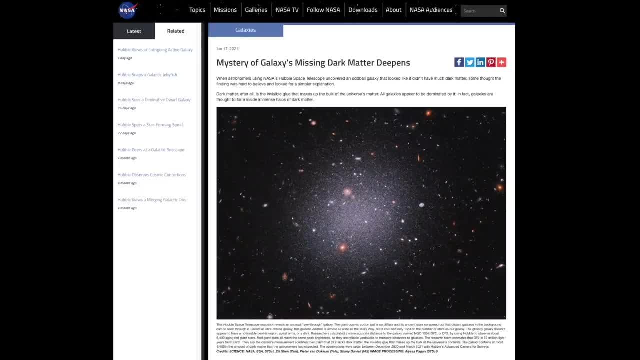 I found I came across a 2003 study that said four galaxies and GC 821, 33, 79, 44 said four galaxies and GC 821, 33, 79, 44 said four galaxies and GC 821, 33, 79, 44, 94 in 46, 97 were found to have little to. 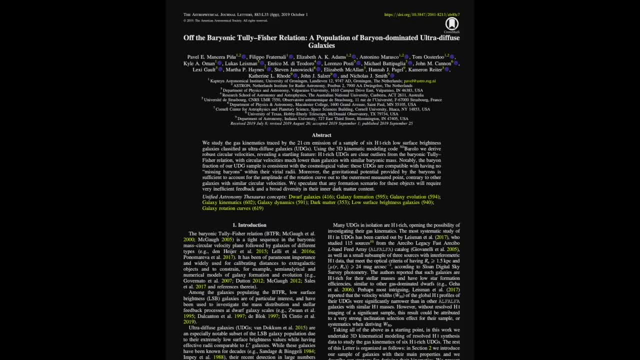 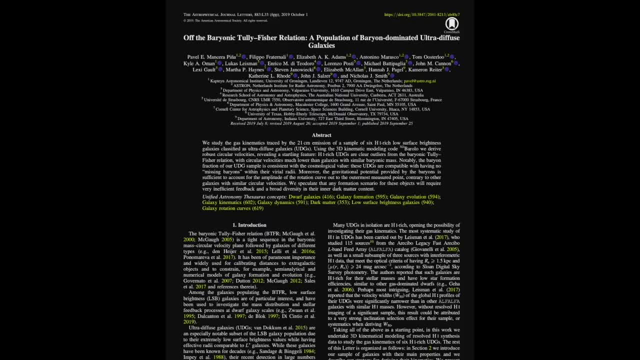 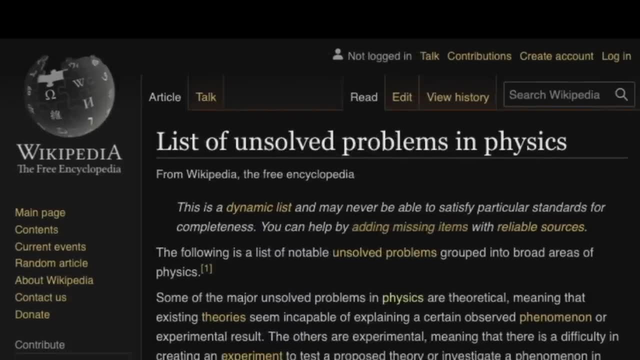 influencing the motion of their stars within them, and the reason behind this dark them and the reason behind this dark them and the reason behind this dark matter, this lack of dark matter is matter. this lack of dark matter is matter. this lack of dark matter is unknown, so there's actually a whole 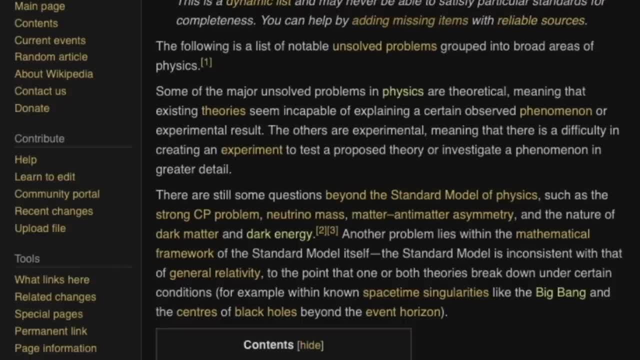 unknown, so there's actually a whole unknown, so there's actually a whole video I want to make on anomalies like video. I want to make on anomalies like video. I want to make on anomalies like this that either disprove or just don't. this that either disprove or just don't. 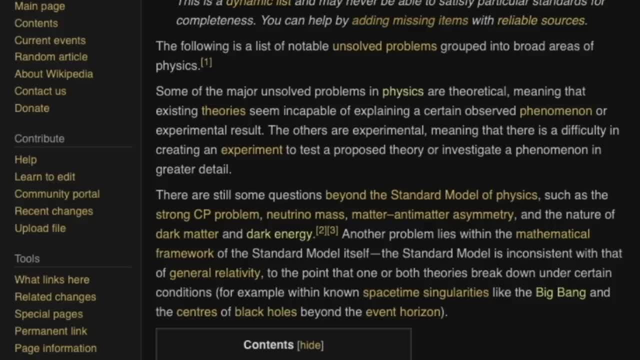 this that either disprove or just don't go along with the current theory, that I go along with the current theory, that I go along with the current theory, that I found it's. uh, if you guys want to check, found it's. uh, if you guys want to check. 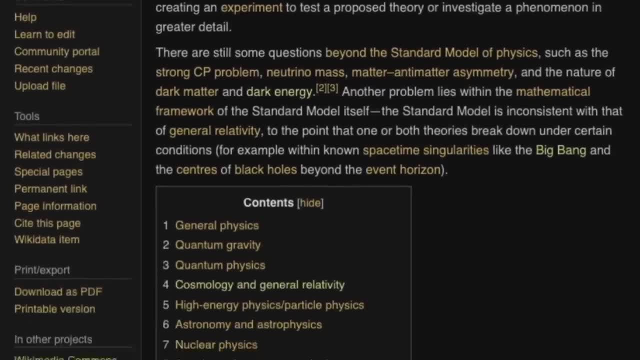 found it's. uh, if you guys want to check it out, just go to the Wikipedia page of it out. just go to the Wikipedia page of it out. just go to the Wikipedia page of. I think it's unsolved problems in. I think it's unsolved problems in. 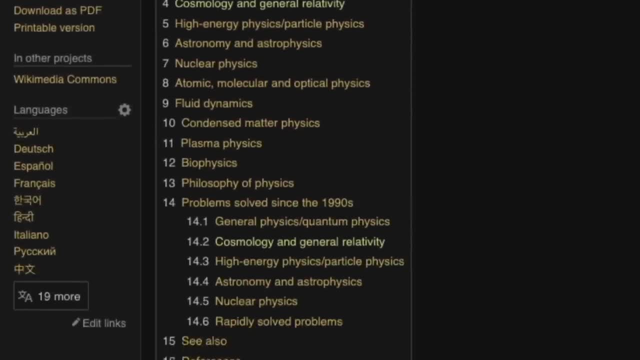 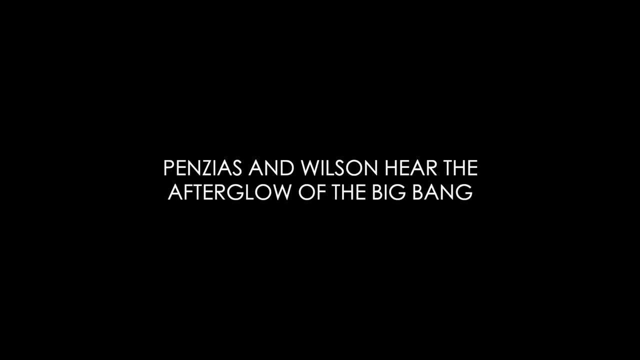 I think it's unsolved problems. in physics it's pretty, uh, it's pretty. physics it's pretty, uh, it's pretty. physics it's pretty, uh, it's pretty amazing to watch them to read through. amazing to watch them to read through. amazing to watch them to read through that. 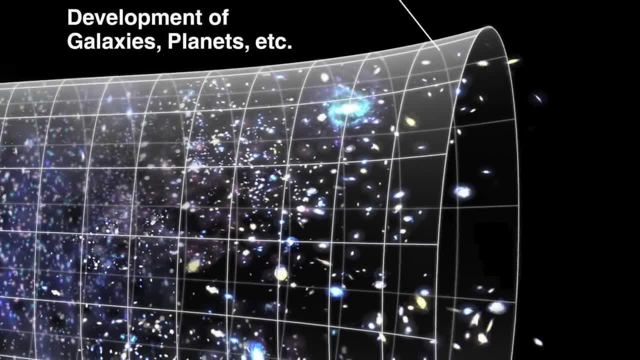 so then, just a couple years later? what so then, just a couple years later? what so then, just a couple years later? what would happen out of LaMontre's theory of would happen out of LaMontre's theory of would happen out of LaMontre's theory of the Big Bang? was that, you know by the 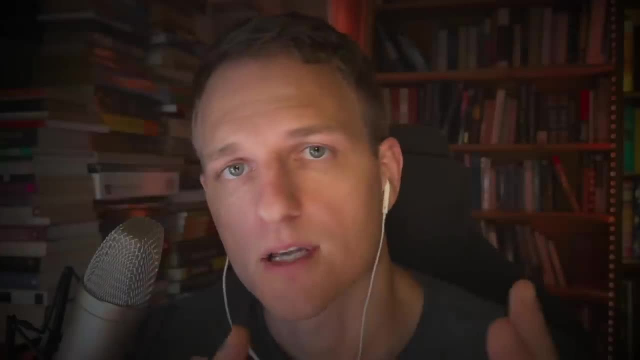 the Big Bang was that you know, by the. the Big Bang was that you know by the 20s and 30s particle physics, quantum 20s and 30s particle physics, quantum 20s and 30s particle physics, quantum mechanics had become full-fledged and was 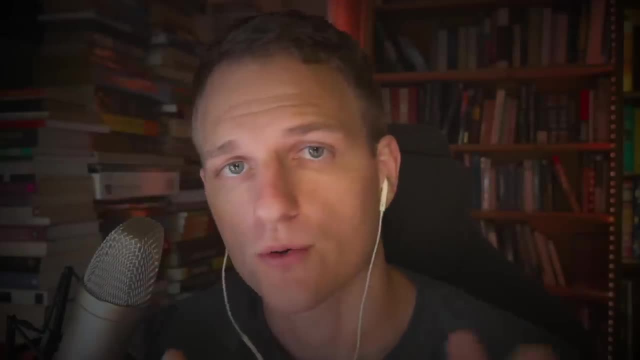 mechanics had become full-fledged and was mechanics had become full-fledged and was making predictions and discoveries, of making predictions and discoveries, of making predictions and discoveries of new particles. and so they were new particles, and so they were new particles, and so they were understanding, they were starting to. 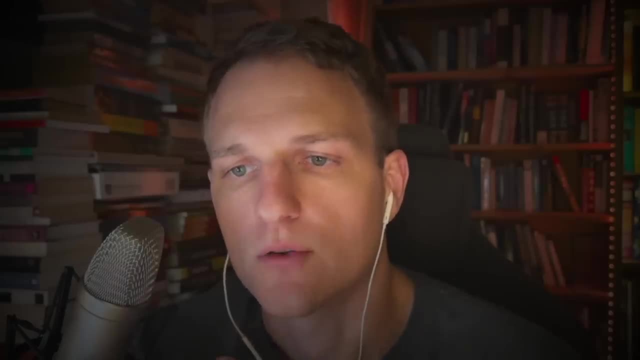 understanding. they were starting to understanding. they were starting to understand what happens at high energies. understand what happens at high energies. understand what happens at high energies and how particles matter break down, and and how particles matter break down, and. and how particles matter break down and forces like the electromagnetic electro. 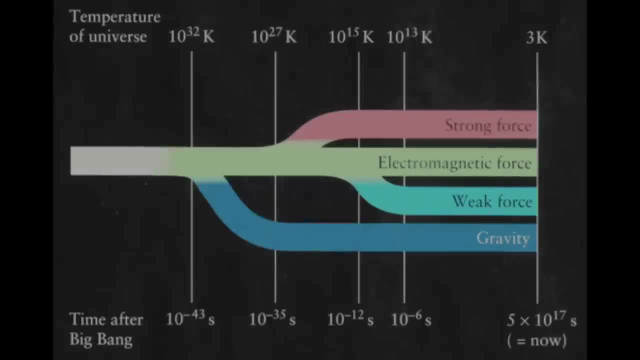 forces, like the electromagnetic electro forces, like the electromagnetic electro weak force, which was the combination of weak force, which was the combination of weak force, which was the combination of the weak force, nuclear force and the weak force, nuclear force and the weak force, nuclear force and electromagnetism. that used to be unified. 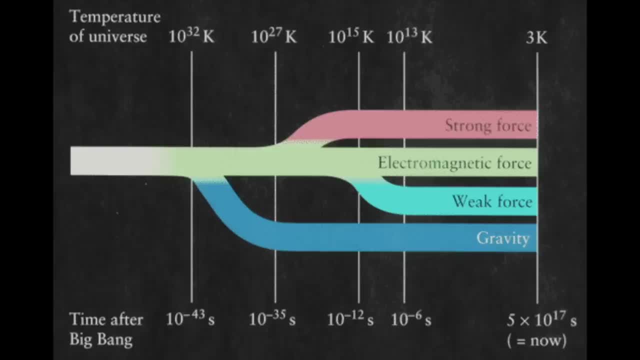 electromagnetism that used to be unified. electromagnetism that used to be unified at high enough energies that is unified at high enough energies that is unified at high enough energies that is unified. and later on it would be found out that, and later on it would be found out that. 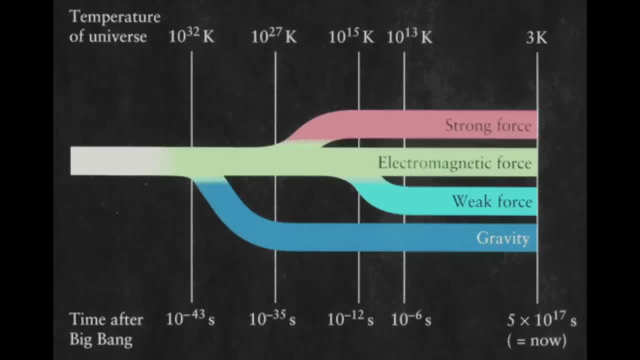 and later on it would be found out that the strong force holding protons and the strong force holding protons and the strong force holding protons and neutrons together in the nucleus, neutrons together in the nucleus, neutrons together in the nucleus, actually is a third phase transition, or I? 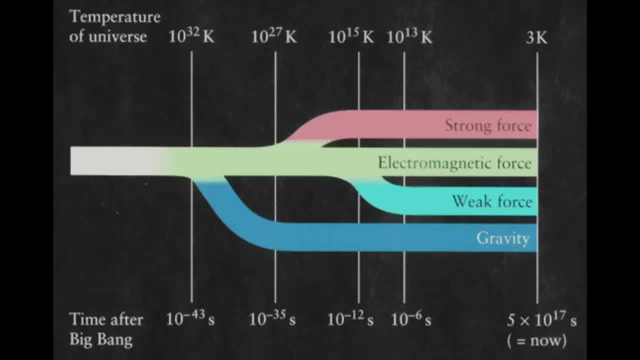 actually is a third phase transition, or I actually is a third phase transition, or I guess the second one. you'd say creating. guess the second one. you'd say creating. guess the second one. you'd say creating the unified atomic force forces, the unified atomic force forces, the unified atomic force forces altogether. and this, this understanding of 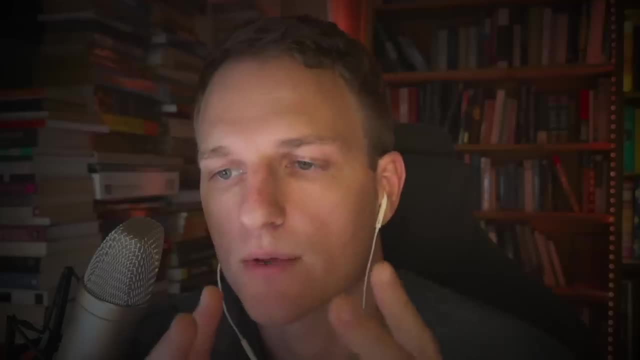 altogether. and this, this understanding of altogether, and this, this understanding of quantum mechanics and particle physics, quantum mechanics and particle physics, quantum mechanics and particle physics allowed them to make predictions. these allowed them to make predictions. these allowed them to make predictions. these people who were proponents of the Big Bang. 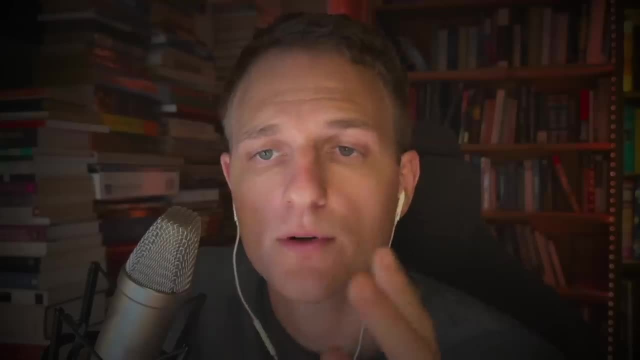 people who were proponents of the Big Bang, people who were proponents of the Big Bang model LaMontre's theory. they were model LaMontre's theory. they were model LaMontre's theory. they were saying that, well, the universe was hot enough. saying that, well, the universe was hot enough. 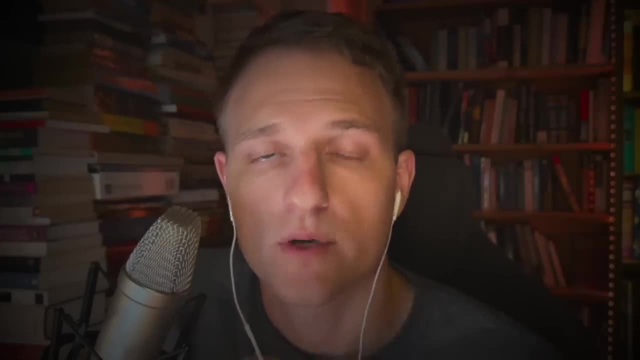 saying that, well, the universe was hot enough and everything was condensed enough, and everything was condensed enough, and everything was condensed enough. we could mean we should be able to have an. we could mean we should be able to have an. we could mean we should be able to have an idea of the rough state of things if 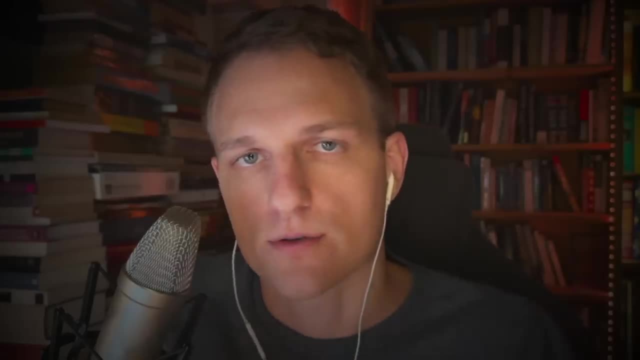 idea of the rough state of things. if idea of the rough state of things, if it gets hot enough at certain energies- it gets hot enough at certain energies, it gets hot enough at certain energies- certain features will appear and certain certain features will appear and certain certain features will appear and certain things will be able to be observed. and 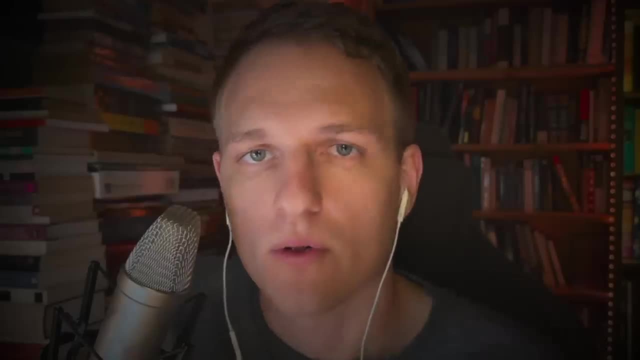 things will be able to be observed and things will be able to be observed, and one of them was that receding wall of one of them was that receding wall of one of them was that receding wall of white light. this, this essential, white light. this, this essential. 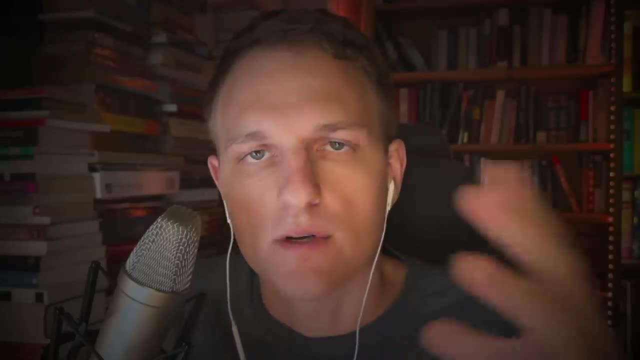 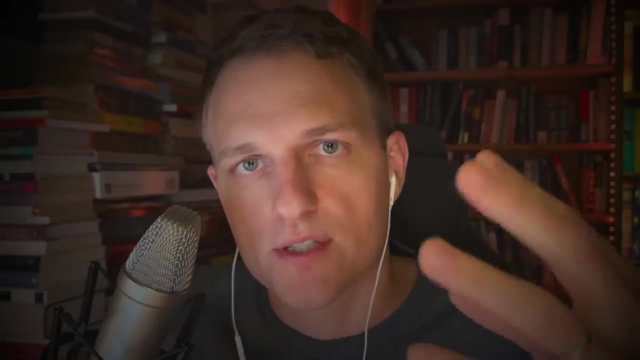 white light. this, this essential, essentially continuous infinite. as far as essentially continuous infinite, as far as essentially continuous infinite. as far as the universe was large field of black, the universe was large field of black. the universe was large field of black. body radiation, body radiation, body radiation still fizzing white-hot with the initial. still fizzing white-hot, with the initial, still fizzing white-hot, with the initial heat from the explosion of the Big Bang heat. from the explosion of the Big Bang heat, from the explosion of the Big Bang popping into existence gradually, over popping into existence gradually, over popping into existence gradually, over hundreds of thousands of years, cooling. 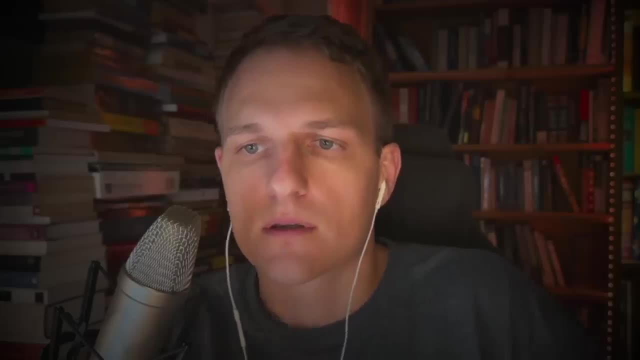 hundreds of thousands of years cooling, hundreds of thousands of years cooling down, and and it's not that this field down and and it's not that this field down and and it's not that this field should be cool enough now that it's far, should be cool enough now that it's far. 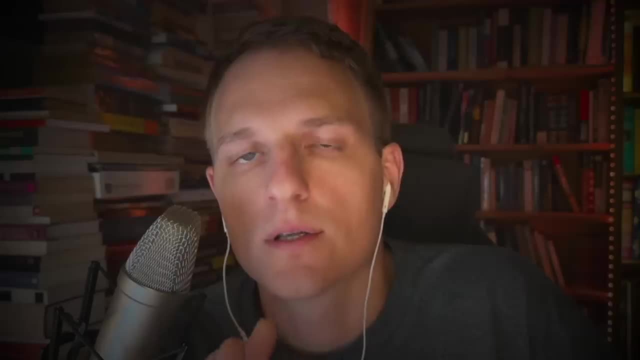 should be cool enough now that it's far and far enough away that it's shifted and far enough away that it's shifted and far enough away that it's shifted into the, into the, into the far, far, far infrared and even microwave region and infrared and even microwave region, and 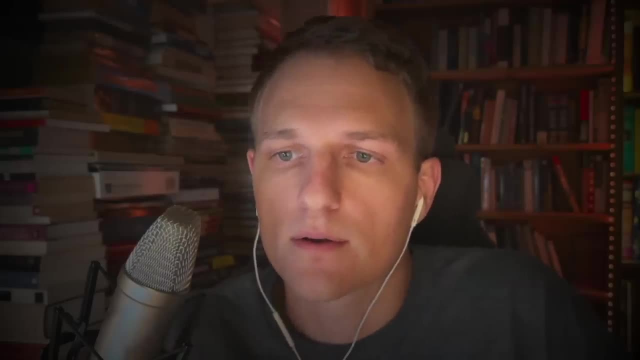 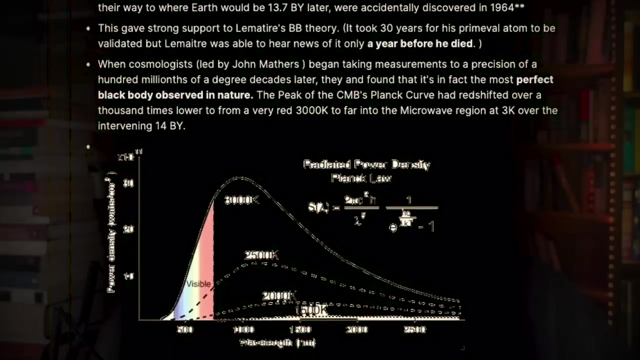 infrared and even microwave region. and that's exactly what happened in the 60s. that's exactly what happened in the 60s. that's exactly what happened in the 60s. 64- it was discovered that the cosmic 64. it was discovered that the cosmic 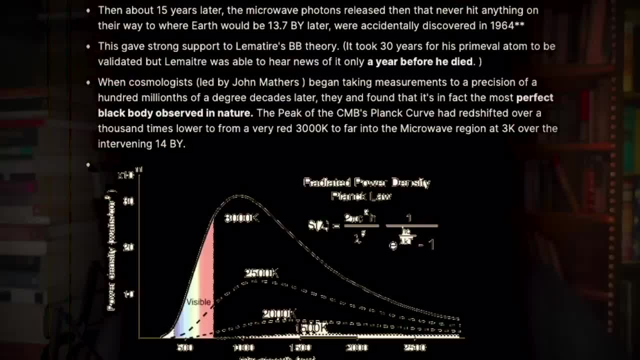 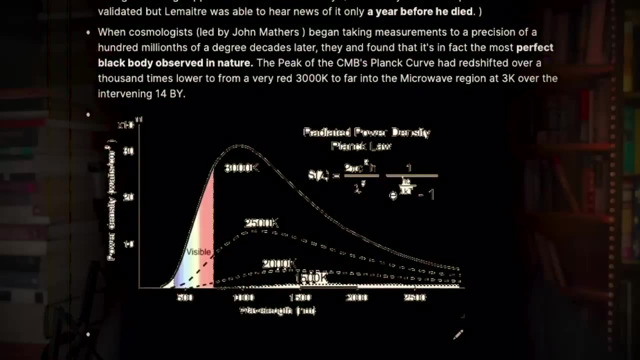 64, it was discovered that the cosmic microwave background is the most perfect microwave background, is the most perfect microwave background, is the most perfect black body curve found in nature, that black body curve found in nature, that black body curve found in nature that, exactly, exactly, exactly, exactly 2.7 degrees Kelvin it peaks in the microwave region and and I 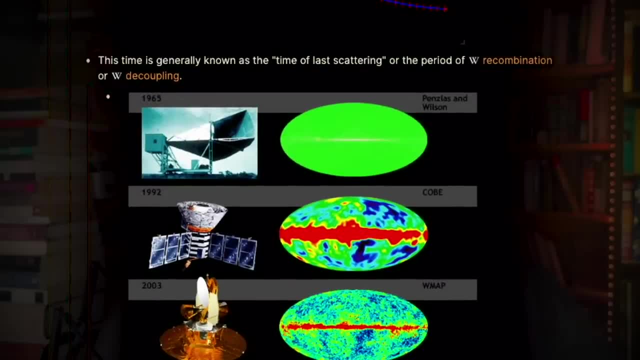 2.7 degrees Kelvin, it peaks in the microwave region. and and I, 2.7 degrees Kelvin, it peaks in the microwave region and and I always thought it was just a something, always thought it was just a something, always thought it was just a something they found and they kind of just try to 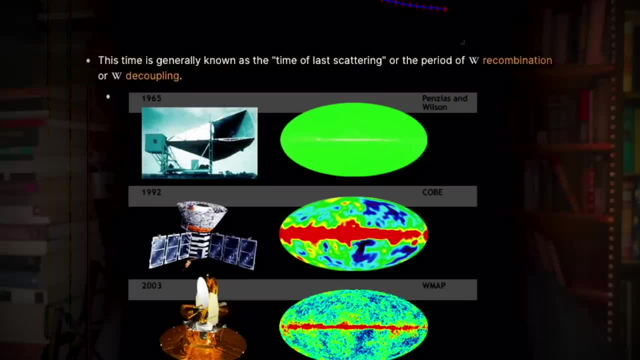 they found and they kind of just try to they found and they kind of just try to come up with a theory. but it's actually come up with a theory. but it's actually come up with a theory. but it's actually, it was actually a prediction and they. 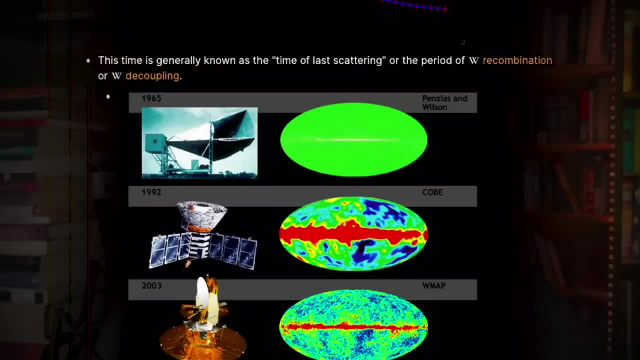 it was actually a prediction and they it was actually a prediction and they actually discovered that it matched, actually discovered that it matched, actually discovered that it matched perfectly with other predictions and the perfectly with other predictions and the perfectly with other predictions and the more they measure it. they. 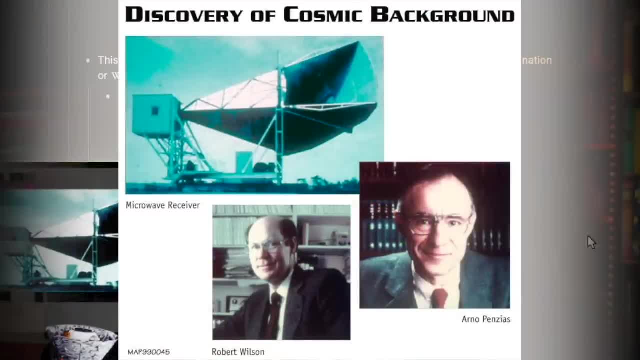 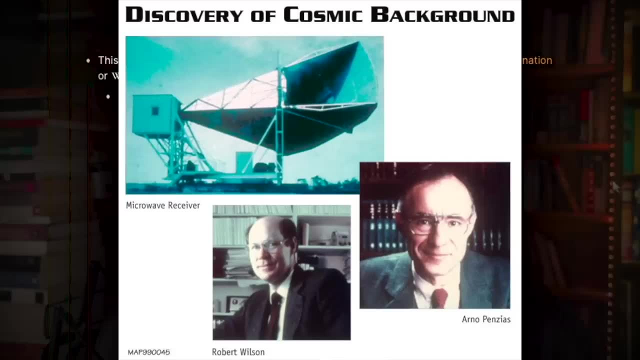 more they measure it, they more they measure it. they have the pensions and Wilk Wilson description. have the pensions and Wilk Wilson description. have the pensions and Wilk Wilson description- here we could see. or measurements here we could see, or measurements here we could see. or measurements. it's real weak. and then the Kobe. 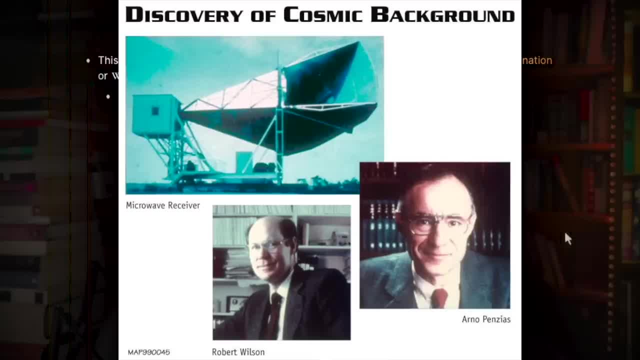 it's real weak, and then the Kobe: it's real weak, and then the Kobe satellite I mentioned in the 90s gave a satellite I mentioned in the 90s, gave a satellite I mentioned in the 90s, gave a much more precise measurement, and then 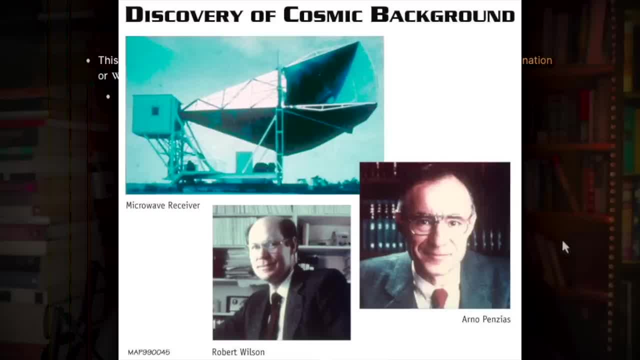 much more precise measurement, and then much more precise measurement, and then in the 2000s Planck or W map, and then in the 2000s Planck or W map, and then in the 2000s Planck or W map, and then even further in the what's I believe. 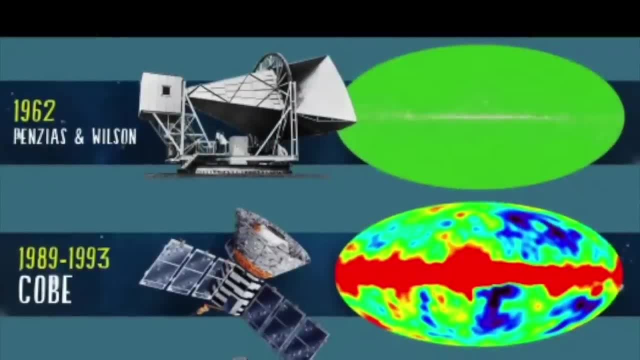 even further in the what's. I believe. even further in the what's. I believe it's still out there orbiting the Planck. it's still out there orbiting the Planck. it's still out there orbiting the Planck measurement, the Planck satellite. 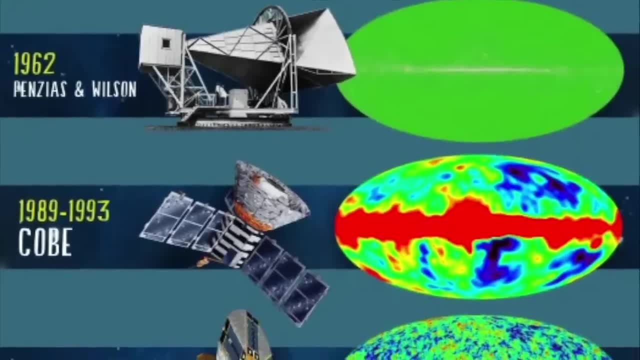 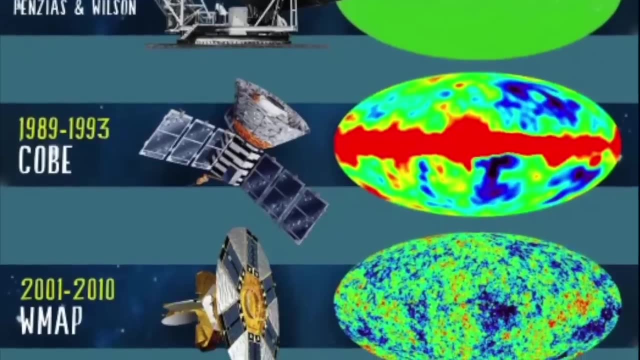 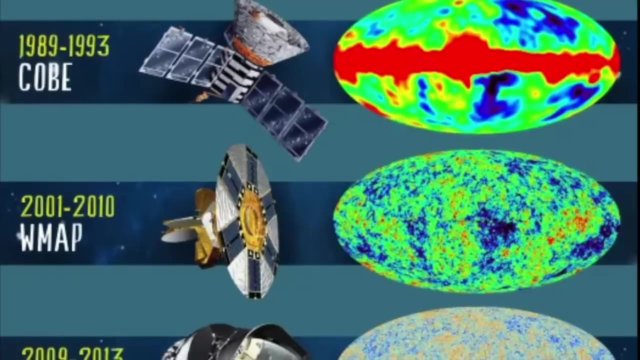 measurement, the Planck satellite measurement, the Planck satellite measuring, these, these background measuring, these, these background measuring, these, these background anomalies from the early heat. just the anomalies from the early heat, just the anomalies from the early heat, just the radiating environment of a steady, glowing universe. 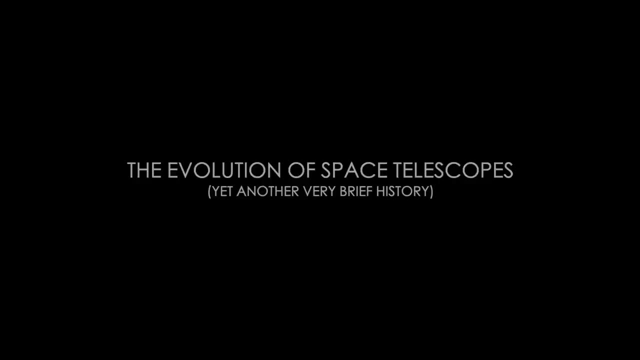 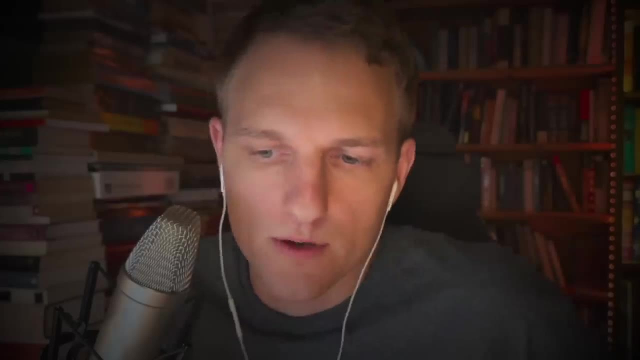 I thought it was relevant here to take. I thought it was relevant here to take. I thought it was relevant here to take- a brief detour in space telescopes. and why a brief detour in space telescopes? and why a brief detour in space telescopes and why is it that they're so important? I 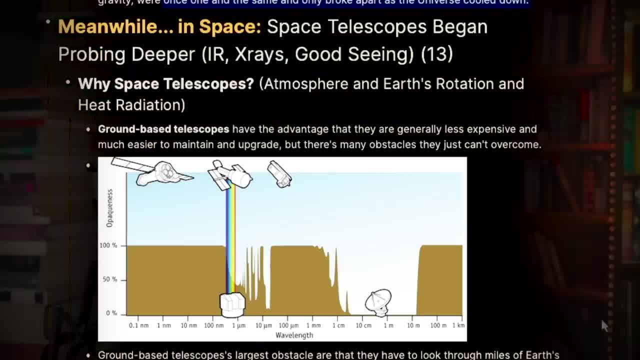 is it that they're so important? I is it that they're so important? I mean this graph here. we touched upon it. mean this graph here. we touched upon it. mean this graph here. we touched upon it. before the atmosphere absorbs a ton of, before the atmosphere absorbs a ton of. 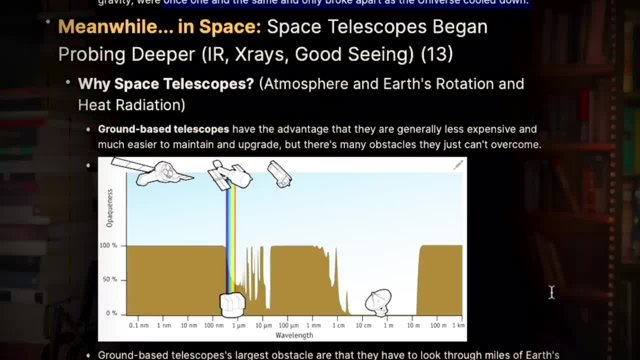 before. the atmosphere absorbs a ton of different wavelengths and this graph different wavelengths and this graph different wavelengths. and this graph here perfectly illustrates that could see here. perfectly illustrates that could see here, perfectly illustrates that could see here in the radio spectrum, the here in the radio spectrum, the. 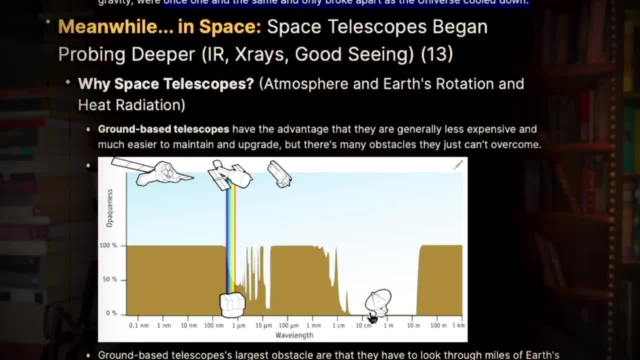 here in the radio spectrum, the essentially the background that touches essentially the background, that touches essentially the background that touches the ground here means that it has the. the ground here means that it has the. the ground here means that it has. the atmosphere is fully transparent to this. 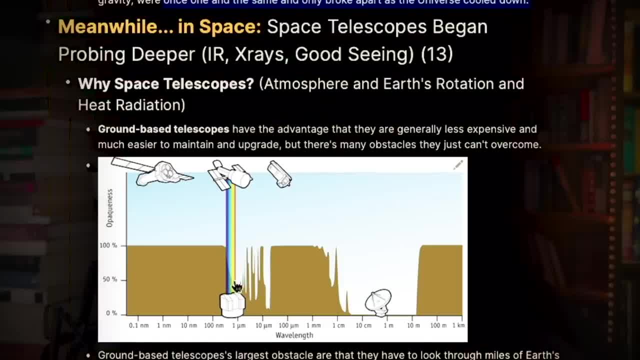 atmosphere is fully transparent to this. atmosphere is fully transparent to this section of the electromagnetic bands, so section of the electromagnetic bands, so section of the electromagnetic bands. so it's only partially transparent to. it's only partially transparent to. it's only partially transparent to visible. it reflects a lot of it back. 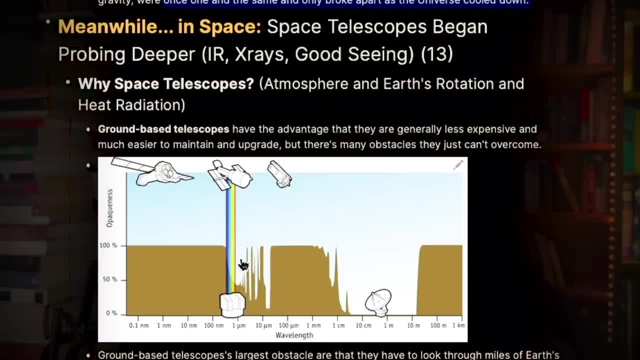 visible: it reflects a lot of it back. visible: it reflects a lot of it back: about 50% and then a ton of infrared, about 50%, and then a ton of infrared, about 50% and then a ton of infrared. over here is only sparsely. 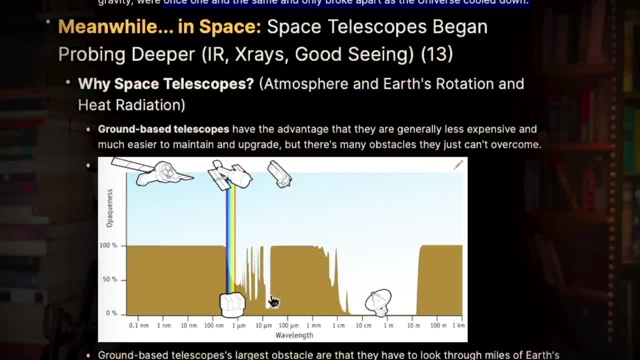 over here is only sparsely over here is only sparsely again available, like a little bit around again. available, like a little bit around again available like a little bit around the 20 micrometer band, but then this, the 20 micrometer band, but then this: 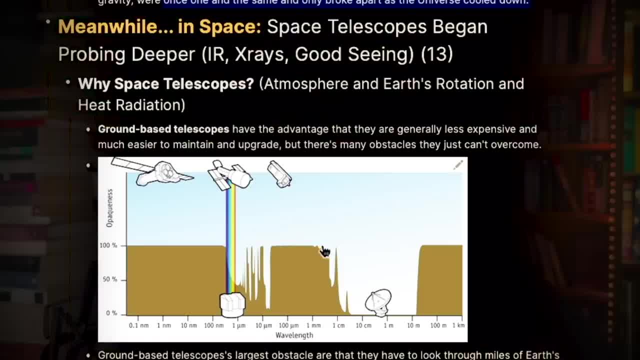 the 20 micrometer band. but then this huge chunk all the way through the huge chunk, all the way through the huge chunk, all the way through the microwave and far infrared is completely microwave and far infrared is completely microwave and far infrared is completely opaque, meaning it does not allow light. 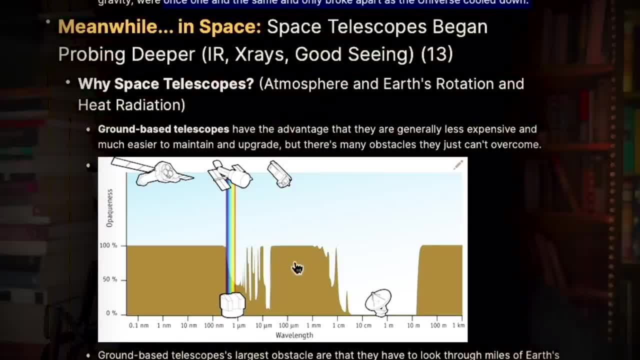 opaque meaning it does not allow light. opaque meaning it does not allow light to pass this particular type of light to pass this particular type of light, to pass this particular type of light. here to pass and reach the ground. so here to pass and reach the ground. so. 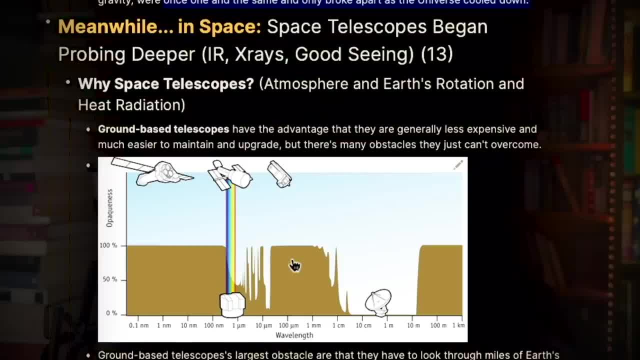 here to pass and reach the ground. so they have telescopes like the Keck and they have telescopes like the Keck and they have telescopes like the Keck and in decent, and these ones in Chile and in decent, and these ones in Chile and 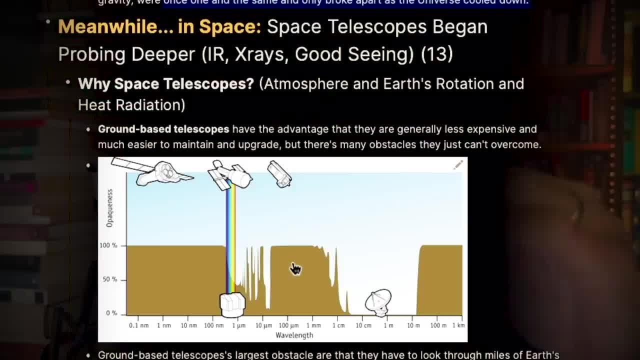 in decent, and these ones in Chile and other mountaintops around the world, of other mountaintops around the world, of other mountaintops around the world, of course, are high up enough where they're course are high up enough where they're course are high up enough. where they're not having to, they can pick up more. 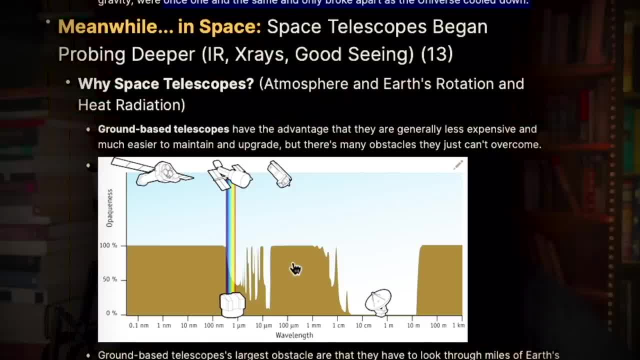 not having to, they can pick up more. not having to, they can pick up more infrared radiation. because it's not infrared radiation, because it's not infrared radiation, because it's not going through as much atmosphere, doesn't going through as much atmosphere doesn't going through as much atmosphere doesn't completely go extinct, but you can see. 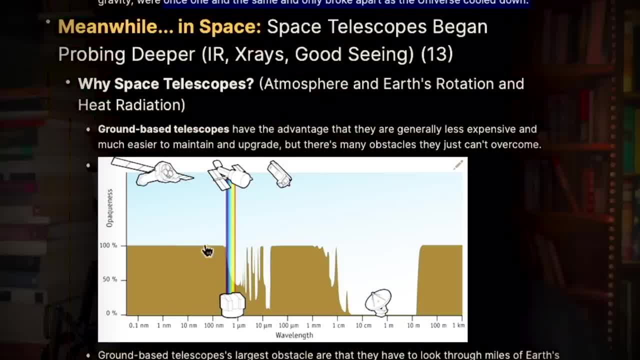 completely go extinct. but you can see completely go extinct. but you can see the gamma ray and x-ray and ultraviolet, the gamma ray and x-ray and ultraviolet, the gamma ray and x-ray and ultraviolet range, the infrared and then the far range, the infrared and then the far. 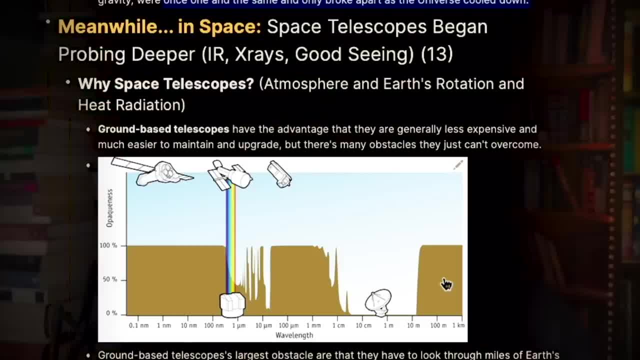 range, the infrared and then the far radio, but that's not really that big a radio. but that's not really that big a radio. but that's not really that big a deal because it's easy to make massive deal, because it's easy to make massive deal, because it's easy to make massive radio telescopes. so it's really just the. 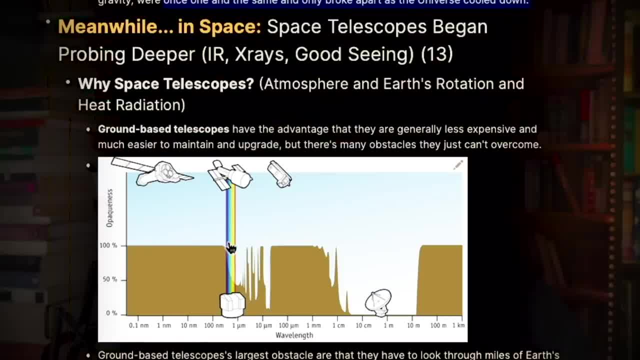 radio telescopes. so it's really just the radio telescopes. so it's really just the x-ray some of the visible. that's why x-ray some of the visible. that's why x-ray some of the visible. that's why Hubble is able to see so much better. 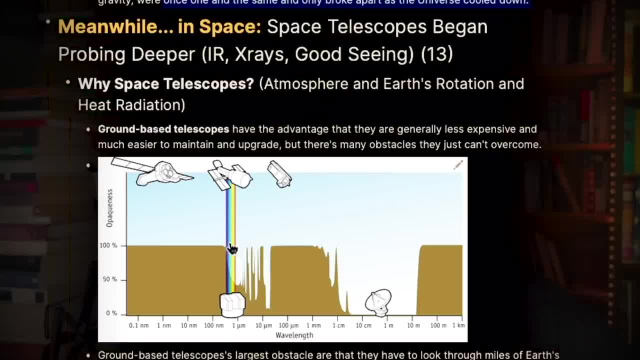 Hubble is able to see so much better. Hubble is able to see so much better than most telescopes, at least as of than most telescopes, at least as of than most telescopes, at least as of recently and until recently, rather in recently and until recently, rather in. 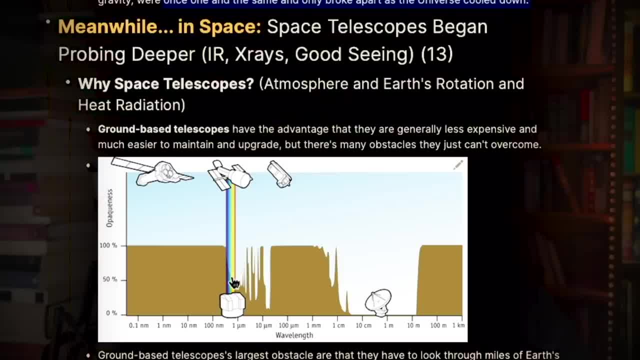 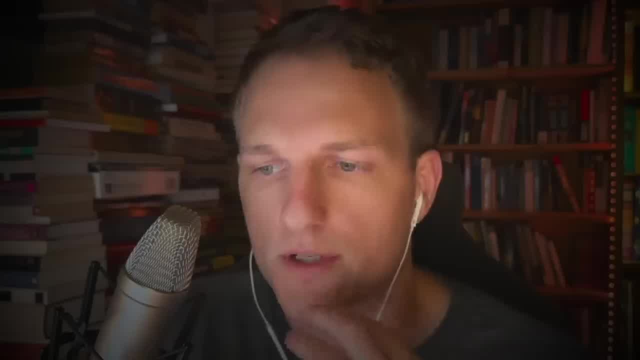 recently and until recently, rather, in the new advanced electronic digital, the new advanced electronic digital, the new advanced electronic digital. error correction called adaptive optics. error correction called adaptive optics. error correction called adaptive optics. thank you, script right there. yeah, it's. thank you, script right there. yeah, it's. 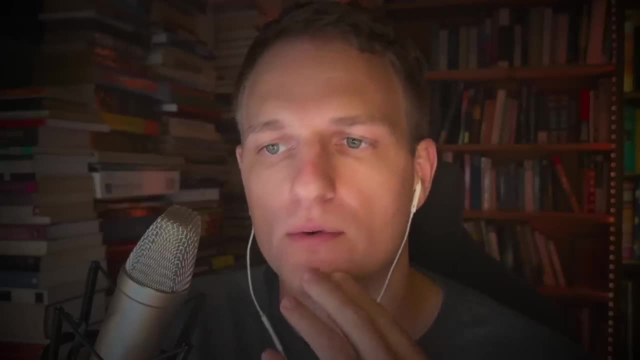 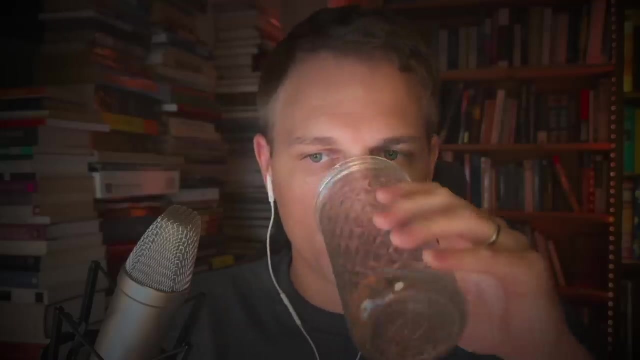 thank you, script right there. yeah, it's these telescopes in these ranges here. these telescopes in these ranges here, these telescopes in these ranges here- x-ray through infrared are really x-ray through infrared, are really x-ray through infrared- are really important to send out in the space. 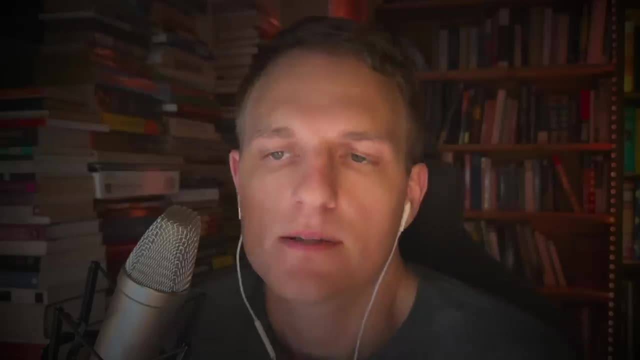 important to send out in the space. important to send out in the space. it's amazing to think that well, it's amazing of track ideas: the. it's amazing to think that well, it's amazing of track ideas, the. it's amazing to think that well, it's amazing of track ideas, the first ideas and how they come to. 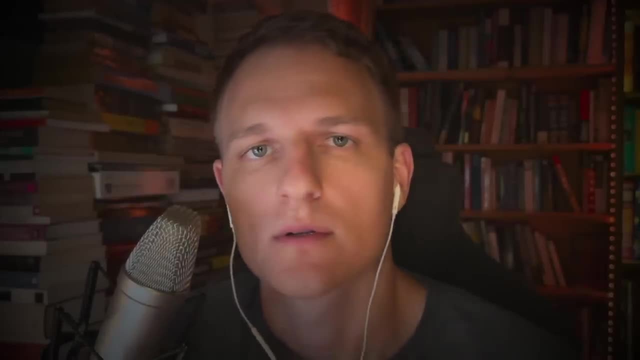 first ideas and how they come to first ideas and how they come to fruition, because there's always these fruition, because there's always these fruition, because there's always these dreamers and thinkers that of course put dreamers and thinkers, that of course put dreamers and thinkers that of course put things in in writing and put things in. 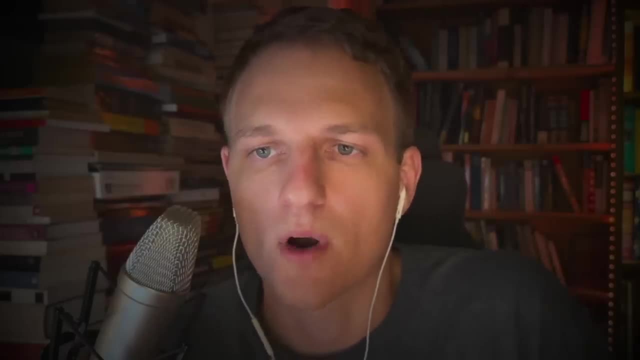 things in in writing and put things in things in in writing and put things in the air before they get made. you know the air before they get made. you know the air before they get made. you know the idea has to come from somewhere, and the idea has to come from somewhere and 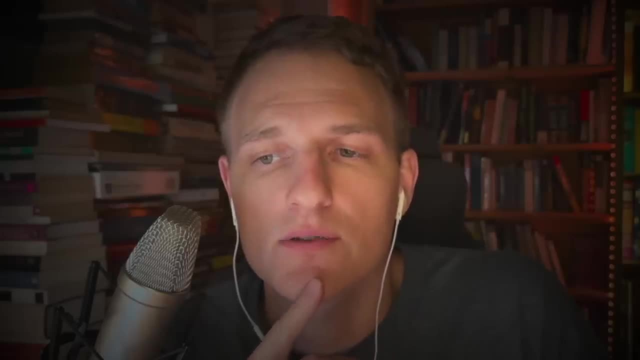 the idea has to come from somewhere, and oftentimes I found it's it's from ideas. oftentimes I found it's it's from ideas. oftentimes I found it's it's from ideas. they've been floating around for a long. they've been floating around for a long. 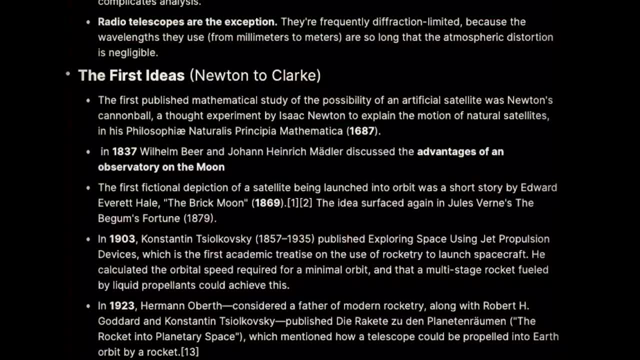 they've been floating around for a long time then Newton was possibly one of the time. then Newton was possibly one of the time then Newton was possibly one of the first to consider an artificial first to consider an artificial first, to consider an artificial satellite. he had a. it first published. 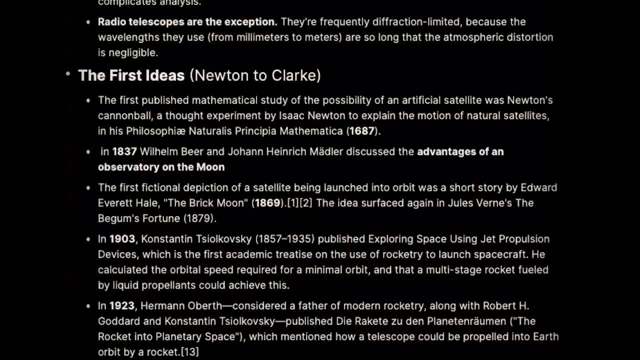 satellite. he had a? it first published satellite. he had a? it first published mathematical study of the possibility of mathematical study, of the possibility of mathematical study of the possibility of an artificial satellite as a cannonball, an artificial satellite as a cannonball, an artificial satellite as a cannonball. just a thought experiment to explain the. 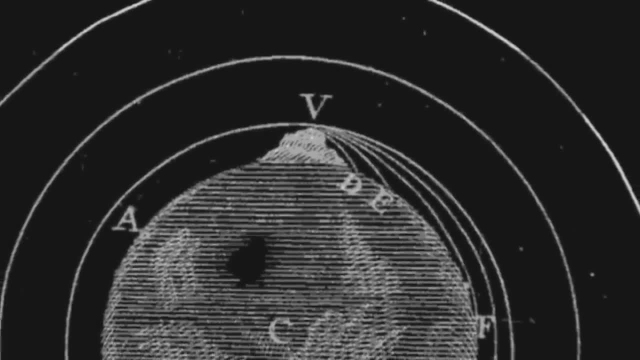 just a thought experiment to explain the. just a thought experiment to explain the motion of natural satellites, in his motion of natural satellites, in his motion of natural satellites, in his Principia Mathematica 1687 stating that a. Principia Mathematica 1687 stating that a. 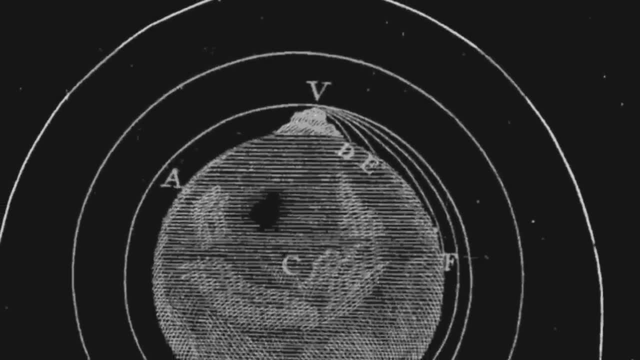 Principia Mathematica 1687 stating that a cannonball within the velocity initial cannonball within the velocity initial cannonball within the velocity initial velocity would be able to shoot out you velocity would be able to shoot out. you velocity would be able to shoot out. you know, I have enough altitude that it. 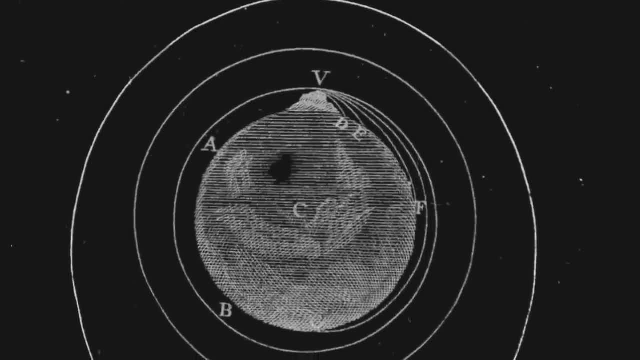 know I have enough altitude, that it know I have enough altitude that it completely relieves the Earth's, completely relieves the Earth's, completely relieves the Earth's atmosphere, and as it falls it would be atmosphere, and as it falls it would be atmosphere, and as it falls it would be going so far that it would never it. 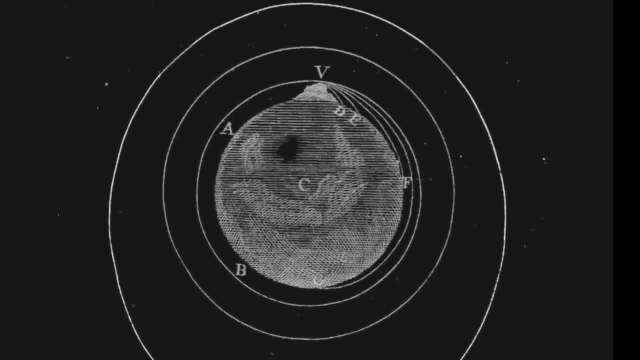 going so far that it would never. it going so far that it would never. it would go and overshoot the earth itself, would go and overshoot the earth itself, would go and overshoot the earth itself, and what that translates to is an orbit, and what that translates to is an orbit. 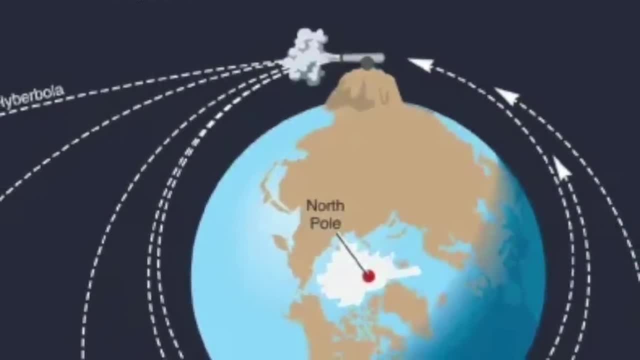 and what that translates to is an orbit. actually so, wouldn't. it wouldn't lob up, actually so, wouldn't? it wouldn't lob up, actually so wouldn't. it wouldn't lob up and hit the ground. it would be going so and hit the ground. it would be going so. 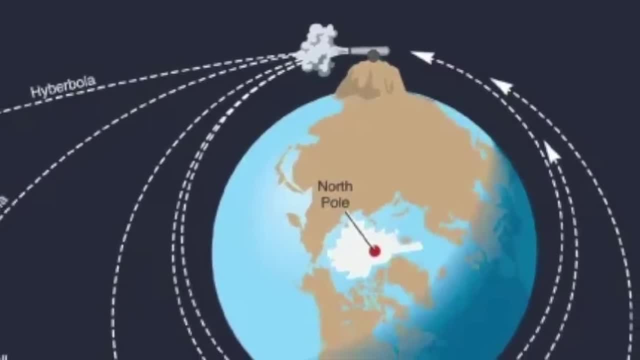 and hit the ground. it would be going so far that, by the time it came down, it far, that, by the time it came down, it far that, by the time it came down, it would follow the curvature, it would would follow the curvature, it would would follow the curvature. it would still be under the influence of Earth's. 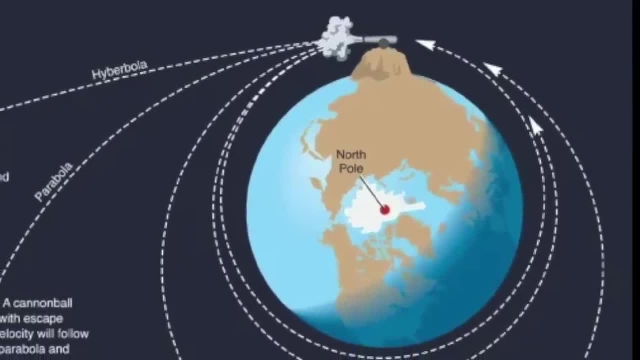 still be under the influence of Earth's, still be under the influence of Earth's gravity, but it would follow the gravity, but it would follow the gravity, but it would follow the curvature of the earth itself, going so curvature of the earth itself, going so curvature of the earth itself, going so far beyond it that it would fall into. 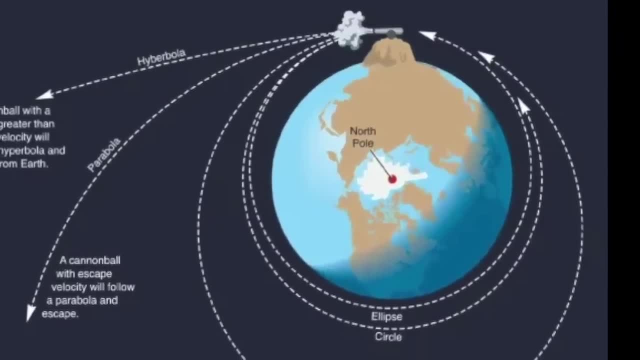 far beyond it that it would fall into, far beyond it that it would fall into an orbit and therefore it would become a, an orbit, and therefore it would become a, an orbit, and therefore it would become a satellite and then a little bit under satellite and then a little bit under. 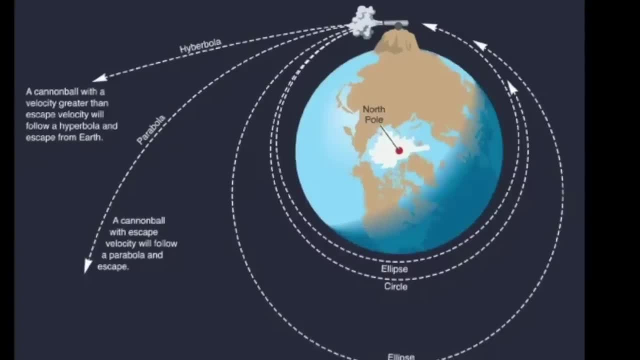 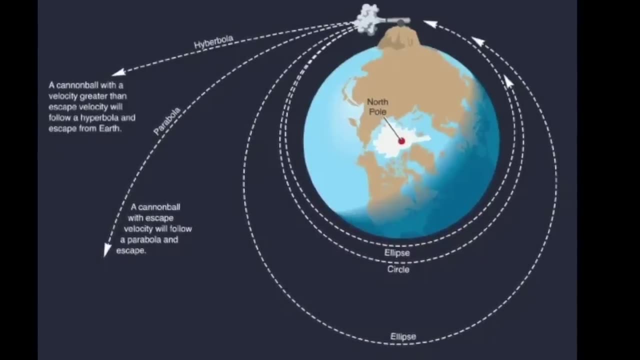 satellite and then, a little bit under 200 years later, another instance of 200 years later, another instance of 200 years later, another instance of probably the first true discussion of a. probably the first true discussion of a, probably the first true discussion of a telescope outside the earth, was by 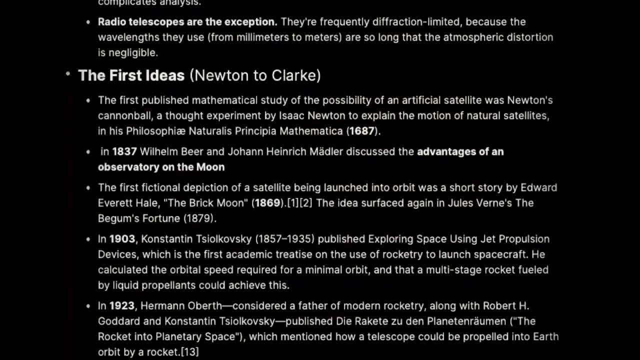 telescope outside the earth was by. telescope outside the earth was by Wilhelm beer and Johan Heinrich Madler. Wilhelm beer and Johan Heinrich Madler. Wilhelm beer and Johan Heinrich Madler. and discussing the advantages of an. and discussing the advantages of an. and discussing the advantages of an absorber. 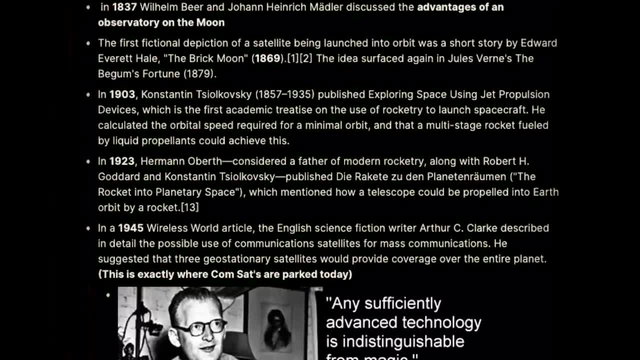 absorber. absorber: Tori on the moon, and then some fiction by Tori on the moon, and then some fiction by Tori on the moon, and then some fiction by ever it hailed and brick moon in 1869. ever it hailed and brick moon in 1869. 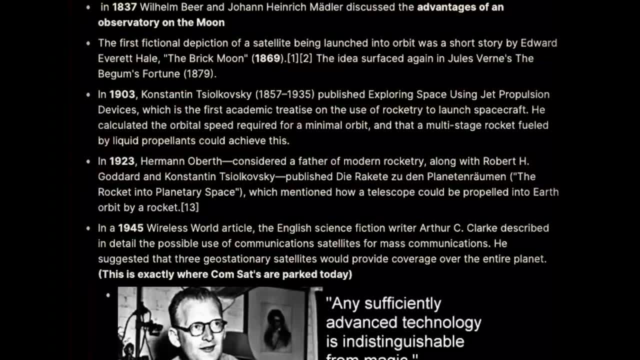 ever it hailed and brick moon in 1869. Jules Verne's. Jules Verne's the Belgium, Jules Verne's Jules Verne's the Belgium, Jules Verne's, Jules Verne's the Belgium, or the Begum fortune. ten years later, 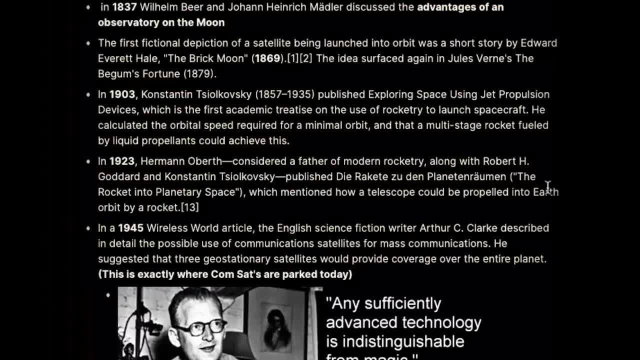 or the Begum fortune ten years later, or the Begum fortune ten years later: depicted: a satellite being launched into. depicted a satellite being launched into. depicted a satellite being launched into orbit. and then in 1903, Konstantin orbit. and then in 1903, Konstantin. 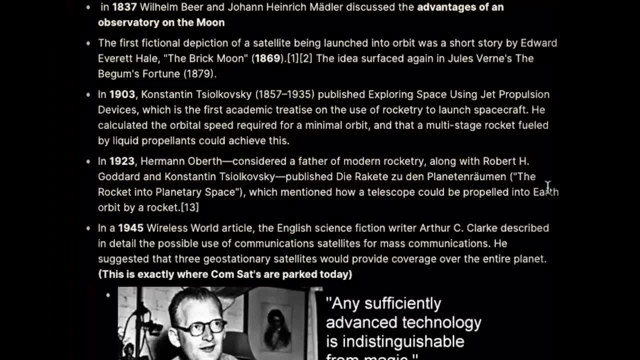 orbit. and then in 1903, Konstantin Sokovsky, Sokovsky, Sokovsky, Sokovsky, Sokovsky published exploring space using jet. published exploring space using jet, published exploring space using jet propulsion devices, and this was the propulsion devices and this was the propulsion devices and this was the first academic treatise on the use of. 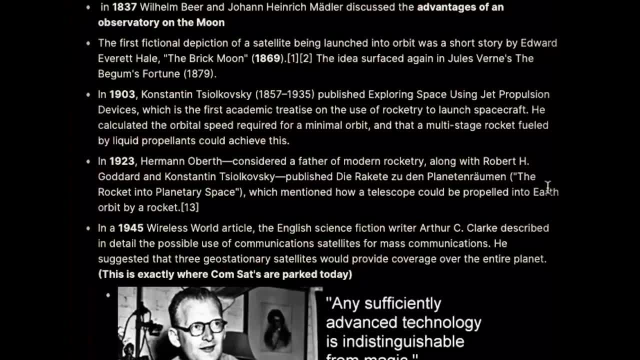 first academic treatise on the use of. first academic treatise on the use of rocketry to launch spacecraft, and then rocketry to launch spacecraft, and then rocketry to launch spacecraft, and then, much later, approaching the actual date, much later approaching the actual date, much later approaching the actual date that we started launching rockets in to. 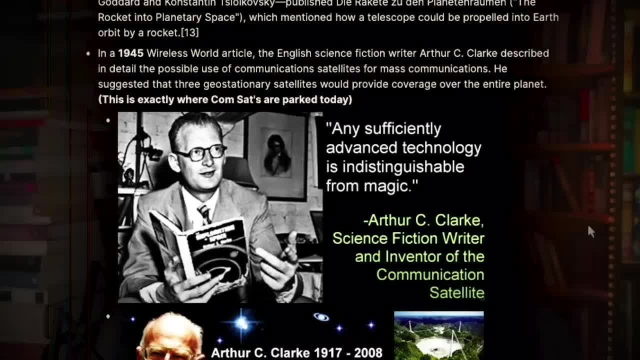 that we started launching rockets in to that. we started launching rockets in to space in 1945 in an article English space in 1945 in an article English space in 1945 in an article English science fiction writer Arthur C Clarke. science fiction writer Arthur C Clarke. 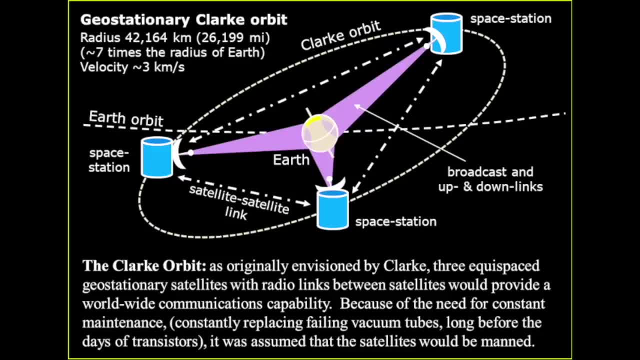 science fiction writer Arthur C Clarke, described in detail the possible, described in detail the possible, described in detail the possible use of communication satellites for mass use of communication satellites for mass use of communication satellites for mass communications. and so amazingly he communications. and so amazingly he communications and so amazingly he explained it perfectly- has three geo. 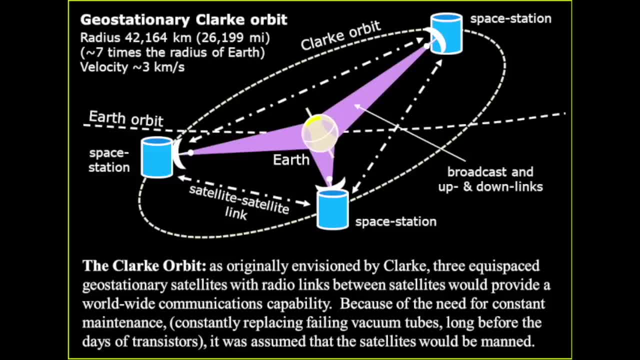 explained it perfectly- has three geo- explained it perfectly- has three geo stationary comm satellites that were stationary comm satellites, that were stationary comm satellites that were within range of each other, the whole within range of each other, the whole within range of each other, the whole time. so, anyways, 1946, I thought that was. 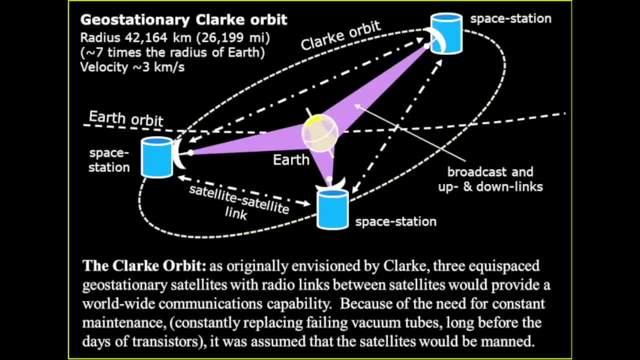 time. so anyways 1946. I thought that was time. so anyways 1946. I thought that was just cool to track the you know quick. just cool to track the you know quick. just cool to track the you know quick. subject: trajectory of how. subject: trajectory of how. 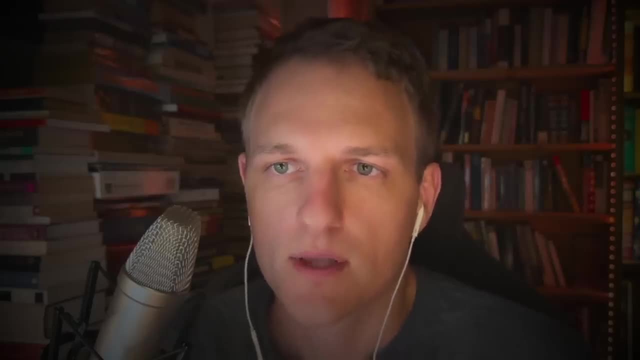 subject: trajectory of how long it's been in the air to make these, then long it's been in the air to make these, then long it's been in the air to make these then. Lyman Spitzer: he's one of the the. Lyman Spitzer, he's one of the the. 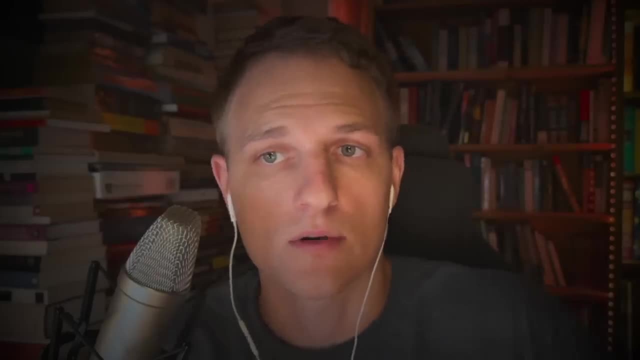 Lyman Spitzer. he's one of the the predecessor to Webb as far as an infrared predecessor to Webb, as far as an infrared predecessor to Webb as far as an infrared telescope goes. was named after telescope goes. was named after telescope goes. was named after Spitzer because Spitzer was. he played a. 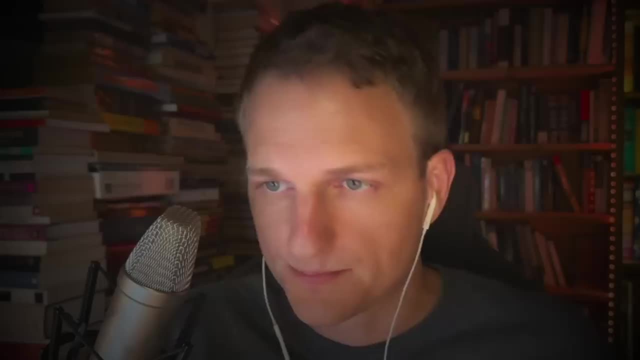 Spitzer. because Spitzer was, he played a Spitzer. because Spitzer was, he played a major role in the birth of space. major role in the birth of space. major role in the birth of space. telescopes in general in 1946 a year. telescopes in general in 1946 a year. 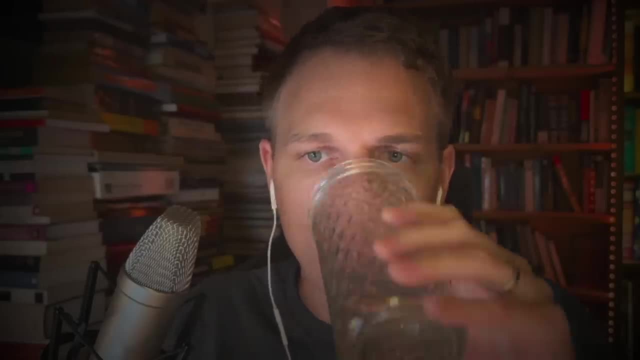 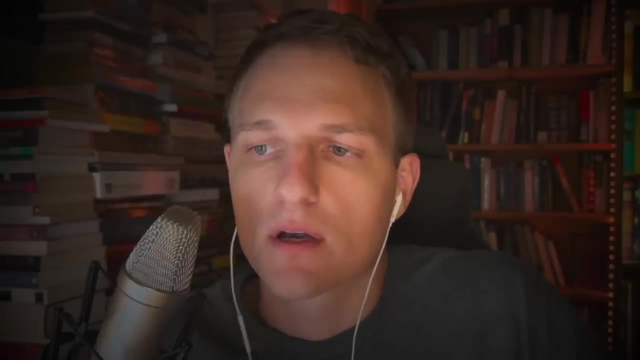 telescopes in general. in 1946, a year after Arthur C Clarke's article, after Arthur C Clarke's article, after Arthur C Clarke's article, Spitzer published astronomical Spitzer published astronomical Spitzer published astronomical advantages of an extraterrestrial- advantages of an extraterrestrial. 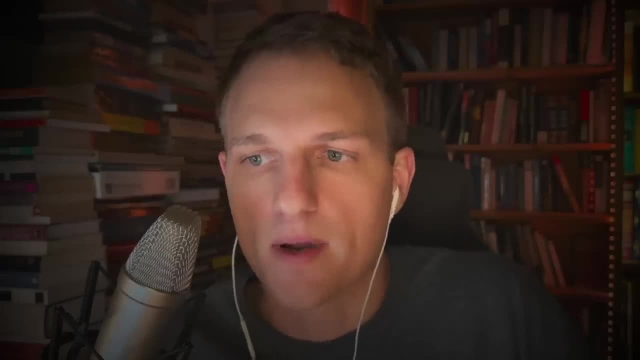 advantages of an extraterrestrial observatory, and then he discussed the observatory, and then he discussed the observatory, and then he discussed the two main advantages that it would have, two main advantages that it would have, two main advantages that it would have over ground-based telescopes. you know, 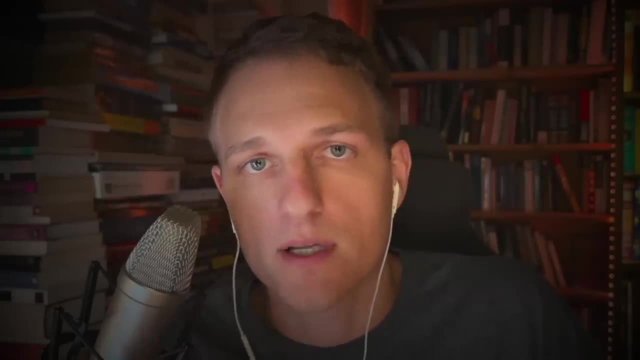 over ground-based telescopes. you know, over ground-based telescopes. you know, the angular resolution first would be one. the angular resolution first would be one. the angular resolution first would be one: you wouldn't have any atmospheric, you wouldn't have any atmospheric, you wouldn't have any atmospheric distortions. and then the second would be: 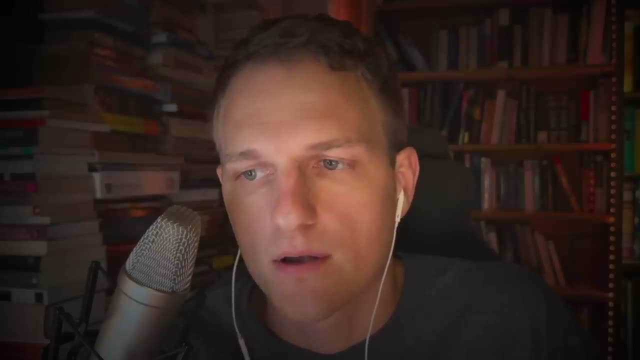 distortions, and then the second would be distortions, and then the second would be that you wouldn't have any atmospheric, that you wouldn't have any atmospheric, that you wouldn't have any atmospheric blocking from ultraviolet light. you know, blocking from ultraviolet light, you know. 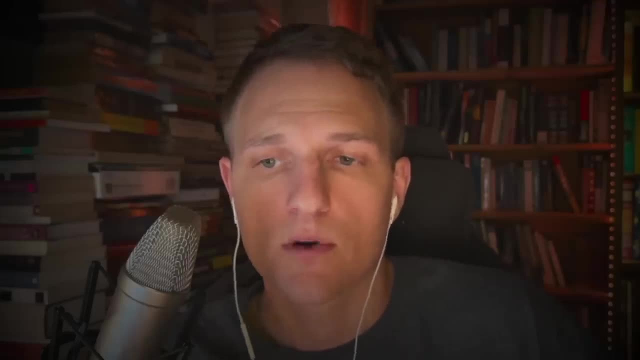 blocking from ultraviolet light. you know, a third he made, maybe mentioned. but a third he made, maybe mentioned. but a third he made, maybe mentioned, but didn't think about, would be if would be, didn't think about, would be, if would be, didn't think about, would be if would be, basically not being bound to the earth. 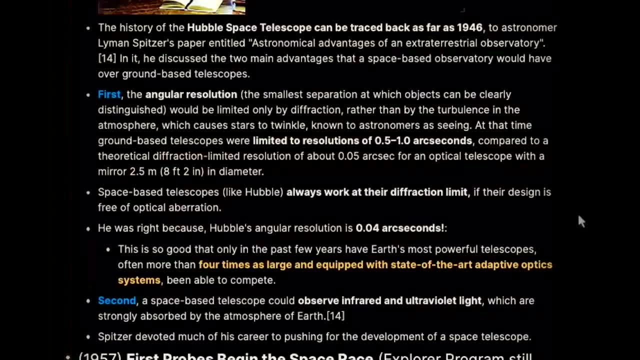 basically not being bound to the earth, basically not being bound to the earth, so you could always have constant. so you could always have constant, so you could always have constant observation of a particular object for observation of a particular object, for observation of a particular object, for way longer than just, you know, 10 hour. 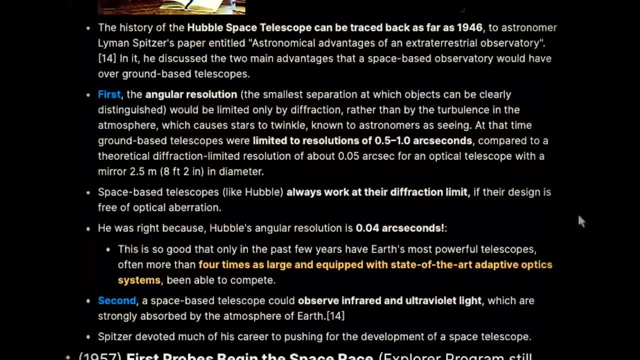 way longer than just you know: 10 hour, way longer than just you know. 10 hour, 8 or 10 hours, however long it might be, 8 or 10 hours, however long it might be, 8 or 10 hours, however long it might be visible on the surface as the earth. 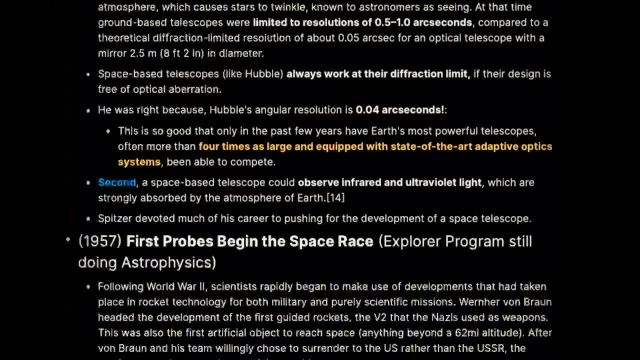 visible on the surface as the earth. visible on the surface as the earth rotates. so over the 50s and 60s we had rotates. so over the 50s and 60s we had rotates. so over the 50s and 60s we had the space race and tons of satellites. 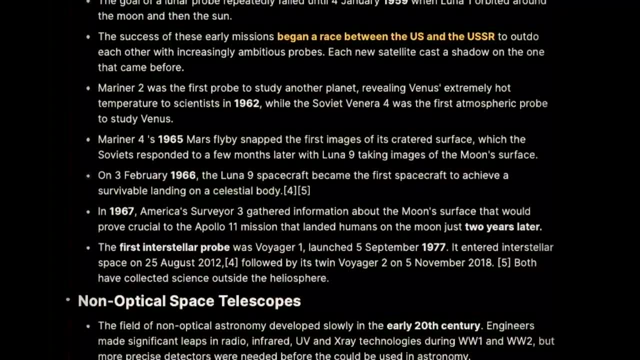 the space race and tons of satellites. the space race and tons of satellites starting to go up and gradually it starting to go up and gradually it starting to go up and gradually it became more and more apparent, that became more and more apparent, that became more and more apparent that non-optical telescopes were going to be. 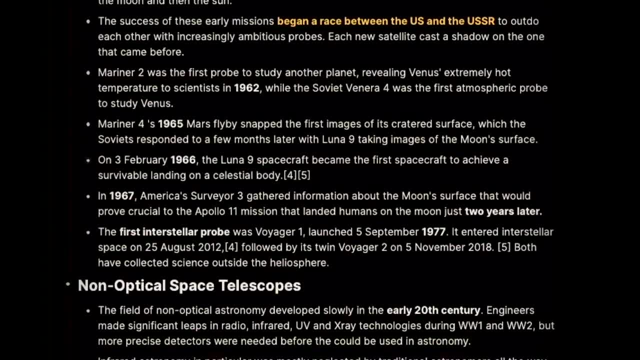 non-optical telescopes were going to be. non-optical telescopes were going to be extremely important for astronomy in the extremely important for astronomy, in the extremely important for astronomy in the 60s, 60s, 60s. we had the, we had the. 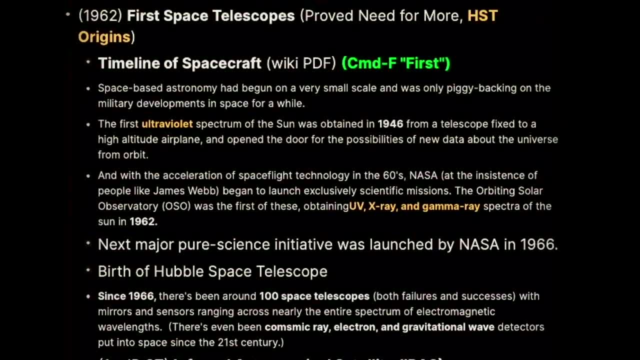 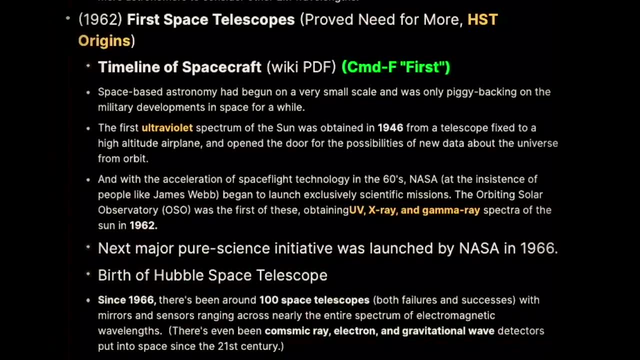 we had the space-based astronomy because it was space-based astronomy, because it was space-based astronomy because it was initially just satellites, and then of initially just satellites, and then of initially just satellites and then, of course, man satellites in the 60s and 50s. 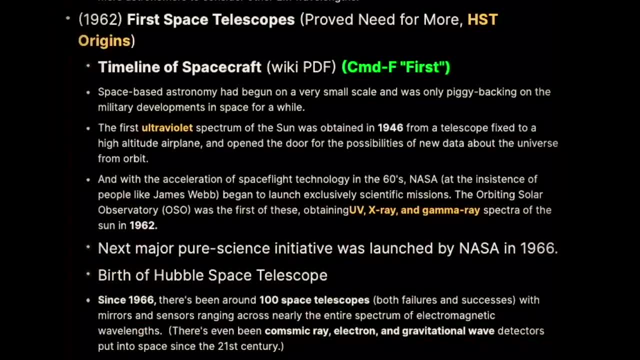 course man satellites in the 60s and 50s, course man satellites in the 60s and 50s, and, and then with James Webb instituting, and, and then with James Webb instituting, and, and then with James Webb instituting the prioritization of pure science. 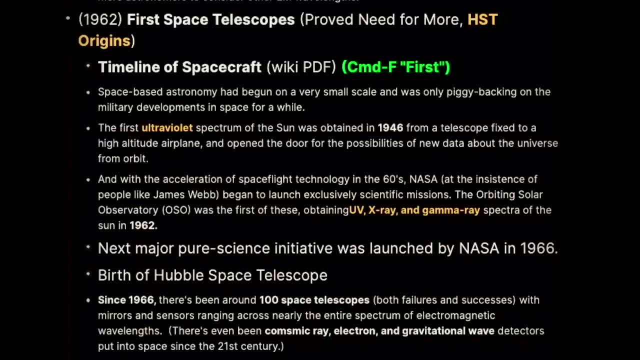 the prioritization of pure science. the prioritization of pure science. experiments along with many other people, experiments along with many other people, experiments along with many other people. but he was a huge factor in it along, but he was a huge factor in it along, but he was a huge factor in it along with the Apollo missions. we had these. 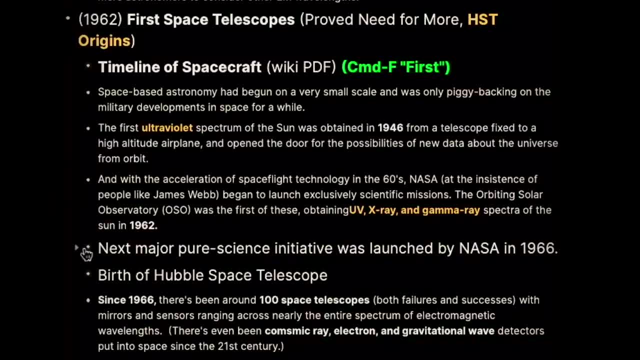 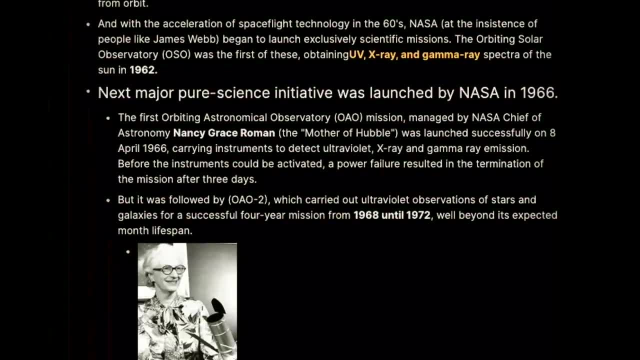 with the Apollo missions, we had these. with the Apollo missions, we had these pure, pure, pure science initiatives launched by NASA. science initiatives launched by NASA. science initiatives launched by NASA. this was the birth of the Explorer. this was the birth of the Explorer. this was the birth of the Explorer program and a woman named in the air, an. 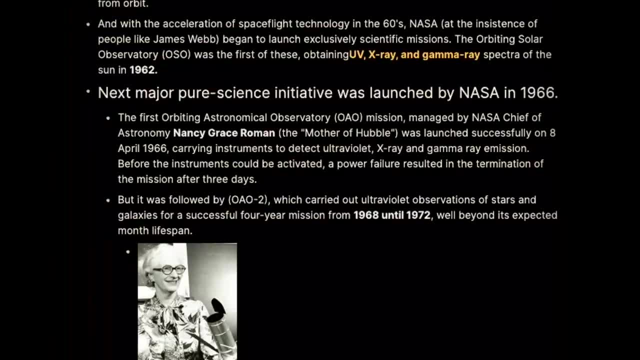 program and a woman named in the air an program and a woman named in the air, an astronomer. I say woman because I saw her astronomer. I say woman because I saw her astronomer. I say woman because I saw her picture here, Nancy Grace Roman, and she's. 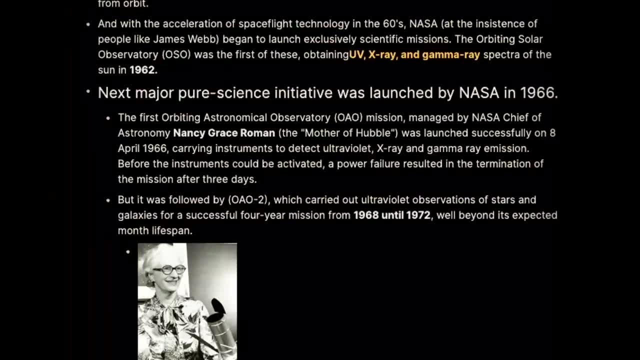 picture here, Nancy Grace Roman, and she's picture here, Nancy Grace Roman, and she's called the mother of Hubble. she's, uh, she called the mother of Hubble. she's, uh, she called the mother of Hubble. she's, uh, she was the chief NASA chief of astronomy of. 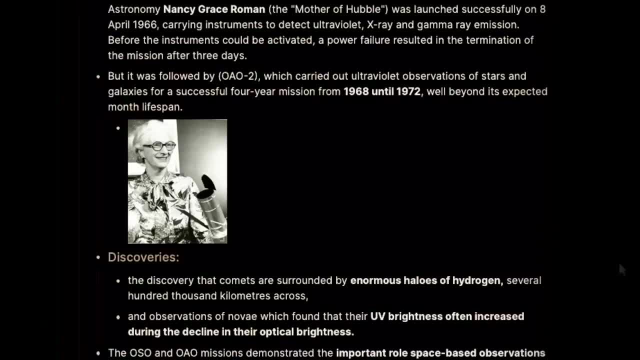 was the chief NASA chief of astronomy of. was the chief NASA chief of astronomy of these early scientific missions. she got these early scientific missions. she got these early scientific missions. she got to be seen here. see a picture of her. to be seen here: see a picture of her. 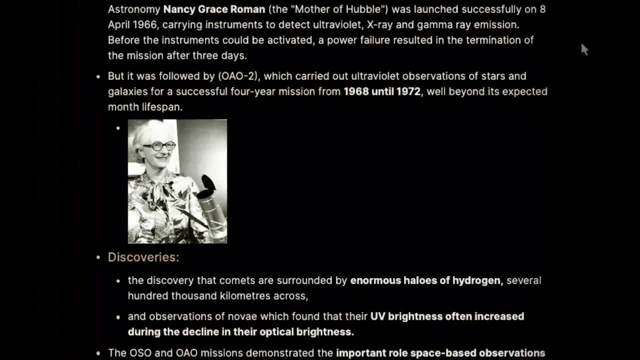 to be seen here. see a picture of her holding an early prototype of Hubble, but holding an early prototype of Hubble, but holding an early prototype of Hubble, but she's considered the mother of Hubble. she's considered the mother of Hubble, she's considered the mother of Hubble and Spitzer is considered the father. 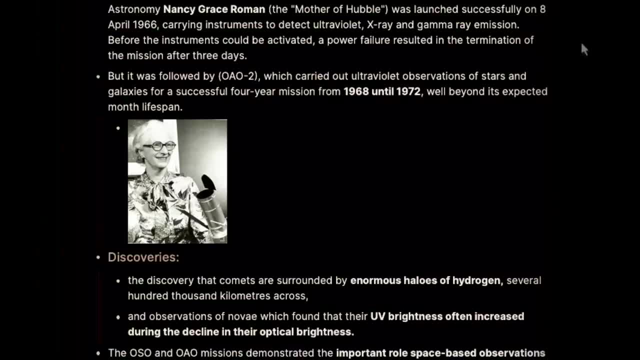 and Spitzer is considered the father and Spitzer is considered the father because they both were proponents for, because they both were proponents for, because they both were proponents for getting a. you know really putting some getting a. you know really putting some getting a. you know really putting some serious money into a telescope going. 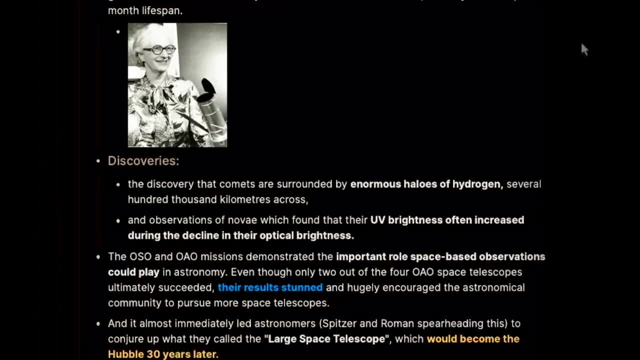 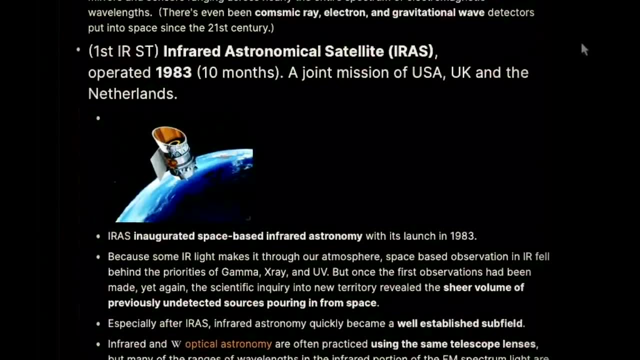 serious money into a telescope, going serious money into a telescope, going far beyond these small little. you know, far beyond these small little. you know far beyond these small little. you know foot wide telescopes, that they had sent foot wide telescopes, that they had sent foot wide telescopes that they had sent into space before then and about 30. 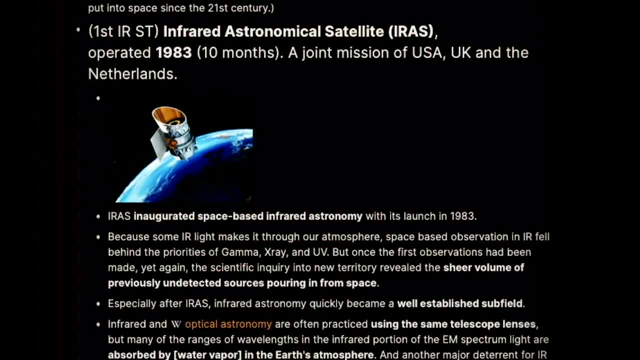 into space before then and about 30 into space before then, and about 30 years later we'd see the birth of. years later we'd see the birth of years later. we'd see the birth of Hubble in 1962, a report by the US. 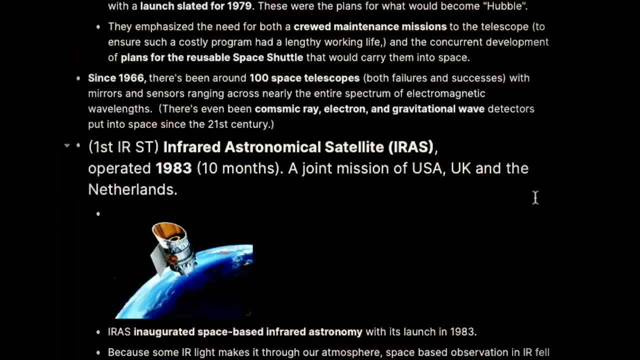 Hubble in 1962. a report by the US Hubble in 1962. a report by the US National Academy of Sciences, National Academy of Sciences, National Academy of Sciences recommended the development of a more recommended the development of a more recommended the development of a more advanced space telescope as part of the 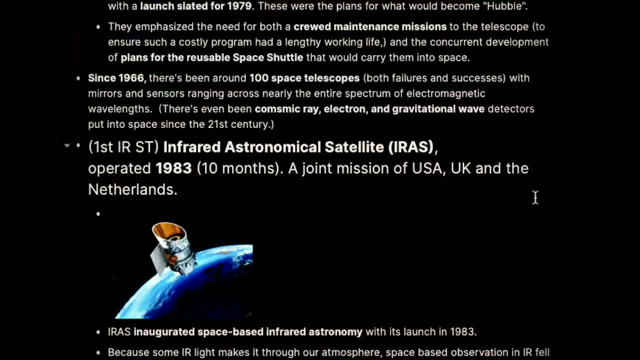 advanced space telescope as part of the advanced space telescope, as part of the new NASA space program to the moon and new NASA space program to the moon and new NASA space program to the moon. and in 1965, Spitzer was appointed as head of. in 1965, Spitzer was appointed as head of. 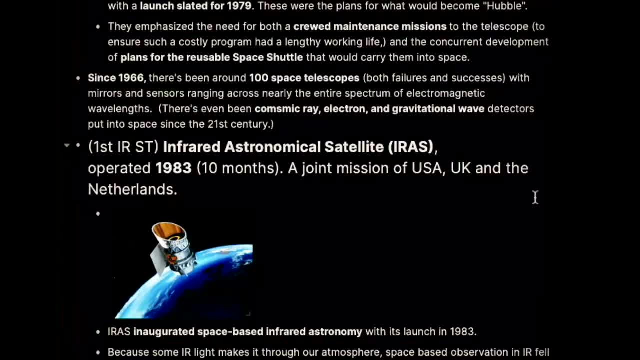 in 1965, Spitzer was appointed as head of the committee and given the task of the committee, and given the task of the committee, and given the task of defining scientific objectives, for what? defining scientific objectives for what? defining scientific objectives for what would become Hubble, a large space. 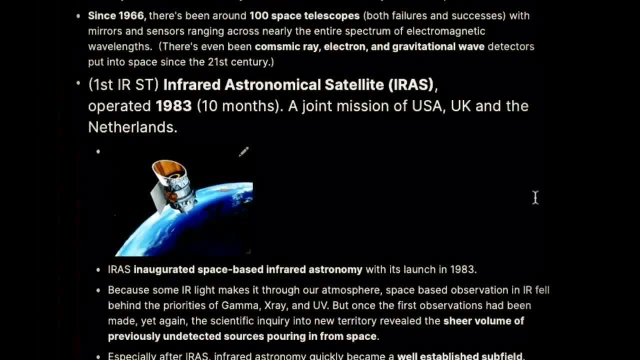 would become Hubble. a large space would become Hubble, a large space telescope. supposed to be 10 feet in telescope. supposed to be 10 feet in telescope. supposed to be 10 feet in diameter. that got scaled back a little. diameter. that got scaled back a little. 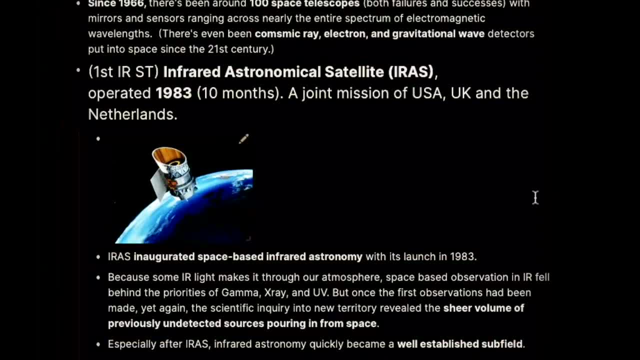 diameter, that got scaled back a little bit. the launch slated for 1979- that got bit. the launch slated for 1979- that got bit. the launch slated for 1979- that got scaled back 11 years. but that's for. scaled back 11 years, but that's for. 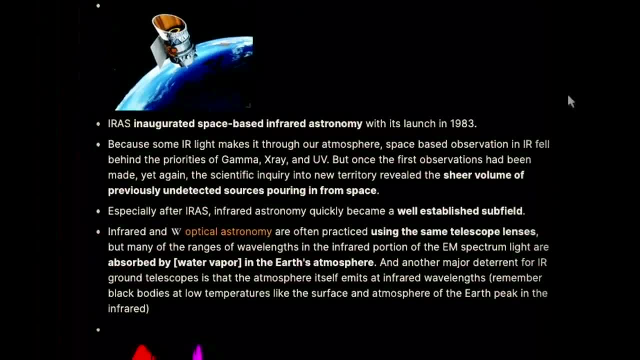 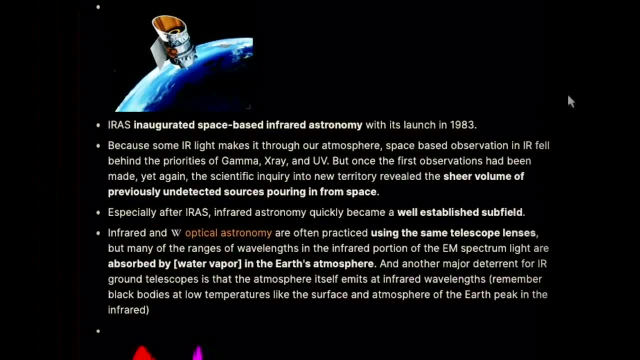 scaled back 11 years, but that's for another time. there's been about a another time. there's been about a another time. there's been about a hundred space telescopes since the hundred space telescopes, since the hundred space telescopes since the sixties, that have been launched and we 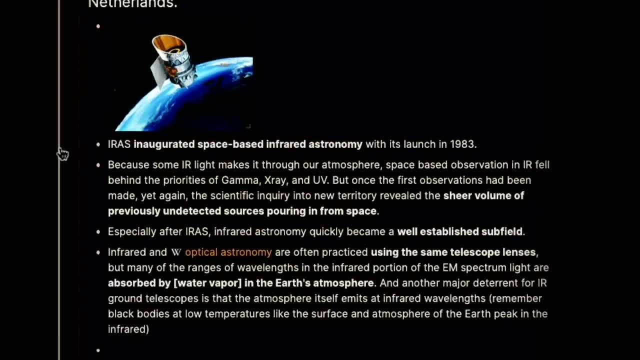 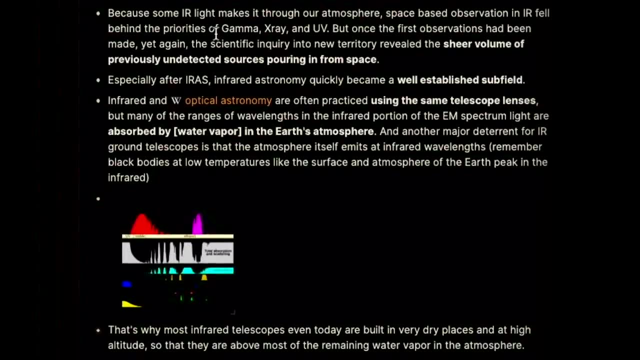 sixties that have been launched and we sixties that have been launched and we we saw our first strictly infrared. we saw our first strictly infrared. we saw our first strictly infrared telescope launched in 1983 and this telescope launched in 1983. and this telescope launched in 1983 and this inaugurated the space-based infrared. 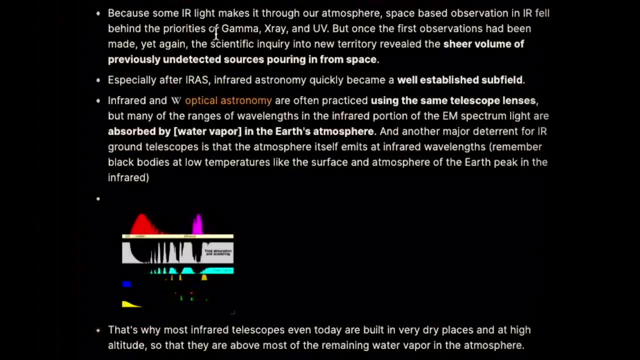 inaugurated the space-based infrared, inaugurated the space-based infrared astronomy, which blew open the minds of astronomy, which blew open the minds of astronomy, which blew open the minds of scientists who realized, oh yeah, there's scientists who realized, oh yeah, there's scientists who realized, oh yeah, there's a ton of infrared radiation pouring in. 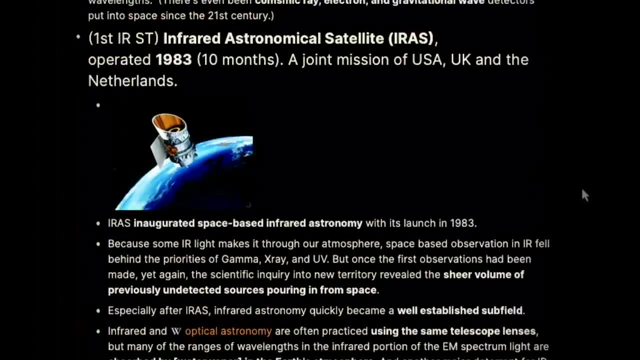 a ton of infrared radiation pouring in a ton of infrared radiation pouring in from space, from space, from space. this was called IRAs the infrared. this was called IRAs the infrared. this was called IRAs the infrared. astronomical satellite joint mission by. astronomical satellite joint mission by. 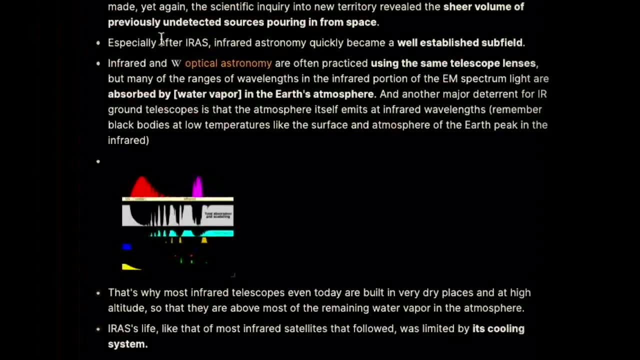 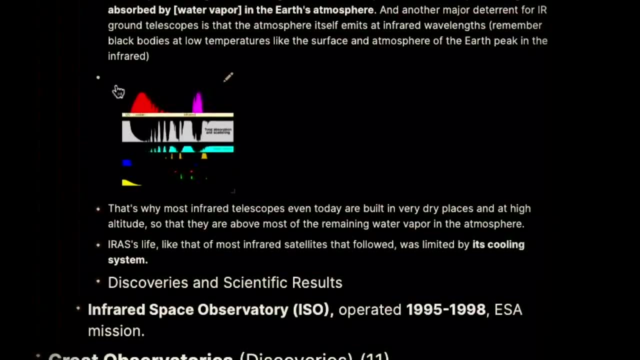 astronomical satellite joint mission by the US- UK and the Netherlands too, and the US UK and the Netherlands too, and the US UK and the Netherlands too, and this was a really accelerated further. this was a really accelerated further. this was a really accelerated further future missions. and then we had the ISO. 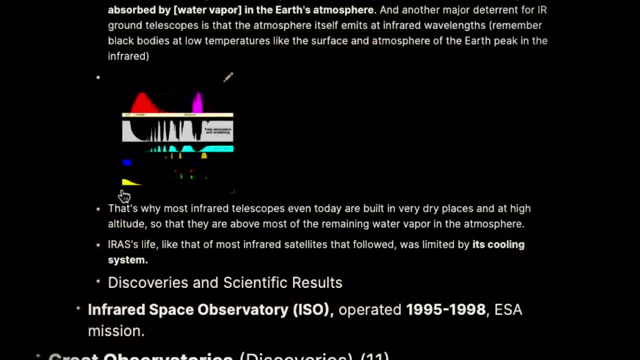 future missions. and then we had the ISO future missions. and then we had the ISO that would be launched about ten years. that would be launched about ten years, that would be launched about ten years later, and then ten years after that, we later- and then ten years after that, we. 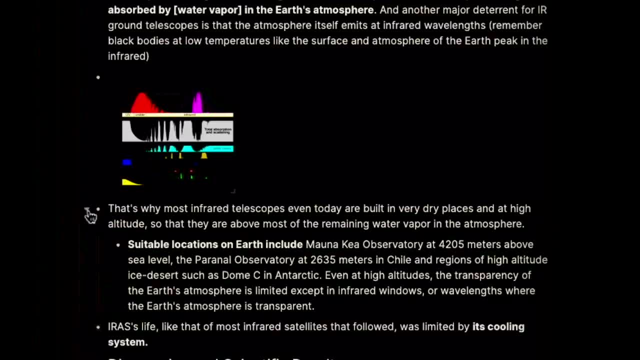 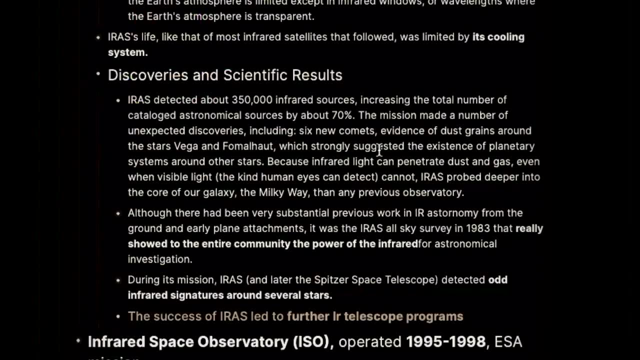 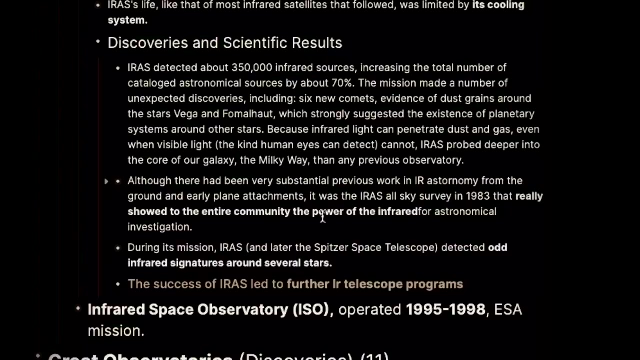 later, and then ten years after that, we had the spitzer, had the spitzer Space Telescope. This detected about 350,000 infrared sources cataloged, increased the catalog number by about 70%. It gave us the first look into the core of our galaxy and 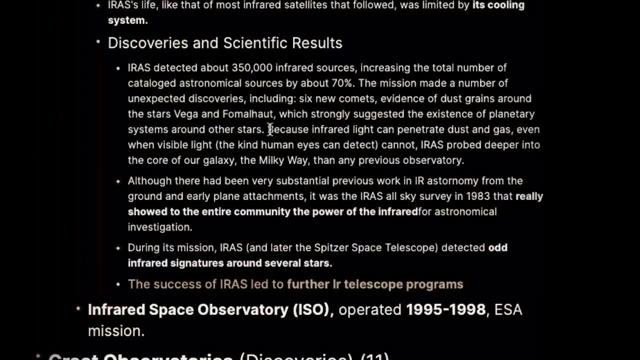 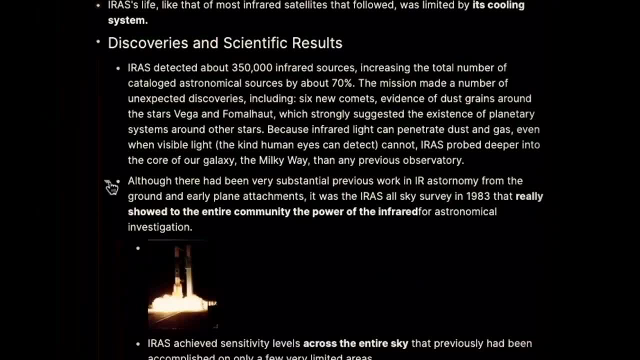 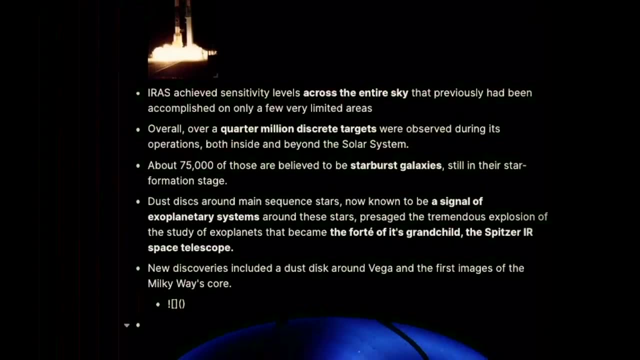 of course, showed that you could penetrate gas clouds and dusty circumstellar disks. you know protostars that we just couldn't see from Earth or in just visible light in general, And this made it extremely important to get new missions off the ground, And these 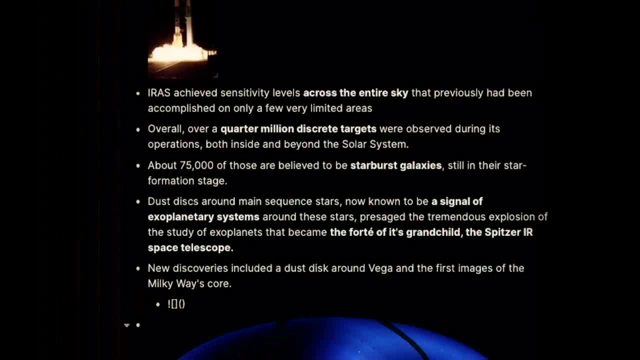 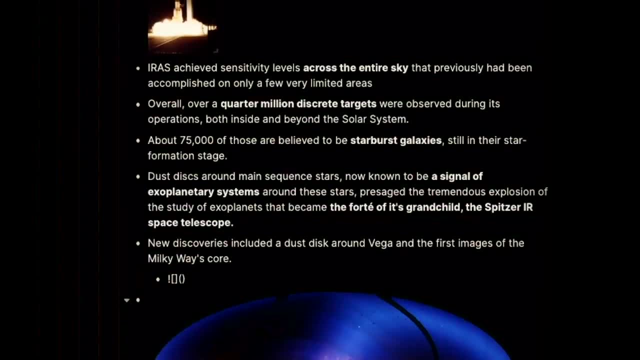 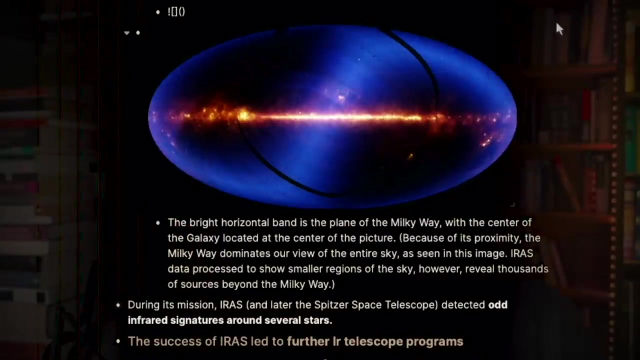 infrared telescope missions throughout the 80s and 90s really planted the seeds for the importance of a much larger, much more sophisticated galaxy. The first exoplanet wasn't discovered until the 90s- officially, but data from these, because the way telescopes work, I found out, is that they just take tons of data and, of course, 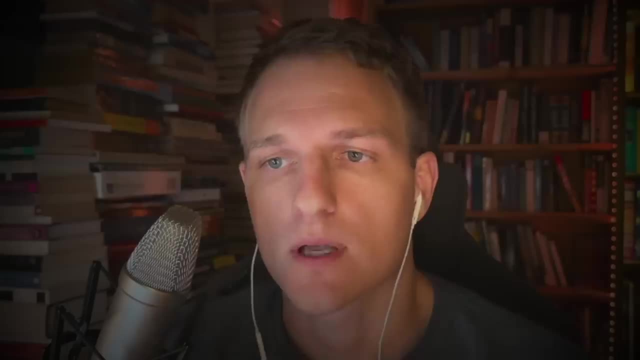 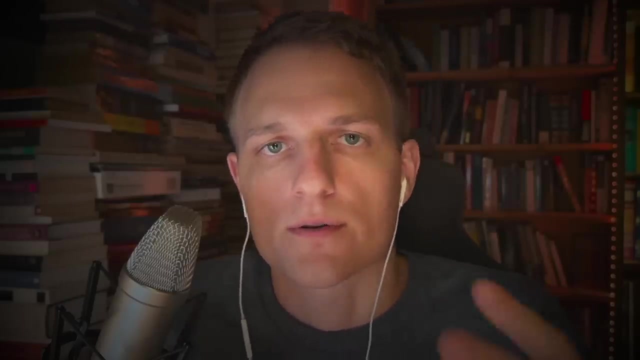 they make images, but there's also a ton of data within the images And for every image you see, there's, you know, hours and maybe gigabytes of data and other images that go along with it, And over years these data get probed and mined and sometimes there's. 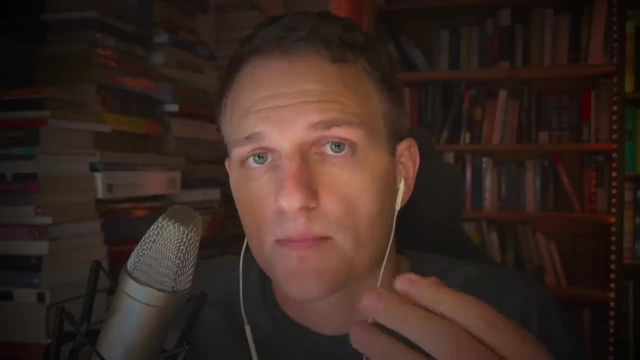 objects in the images that just weren't thought to be looked at until later. another telescope, more sophisticated, looks at it and sees something there, and you want to have to go back and compare, And so it's really important to have these massive images. 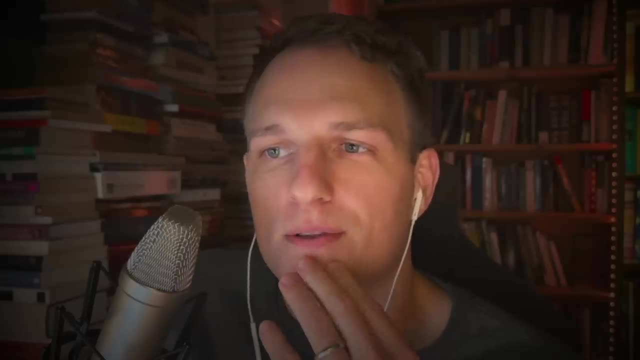 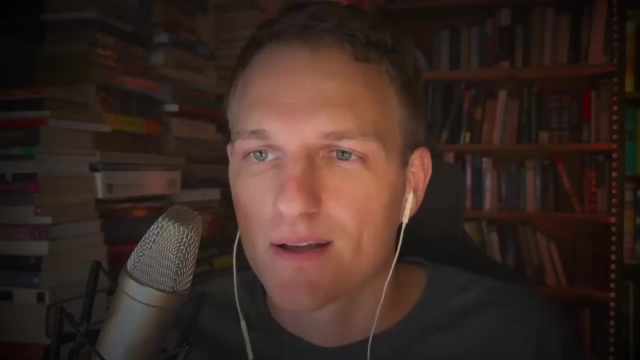 And it turns out that in the 80s one of the exoplanets discovered in the late 90s was actually imaged, but it was just a little too faint to be recognized as an exoplanet back then by IRAS. But it just makes you wonder what kind of you know what information. 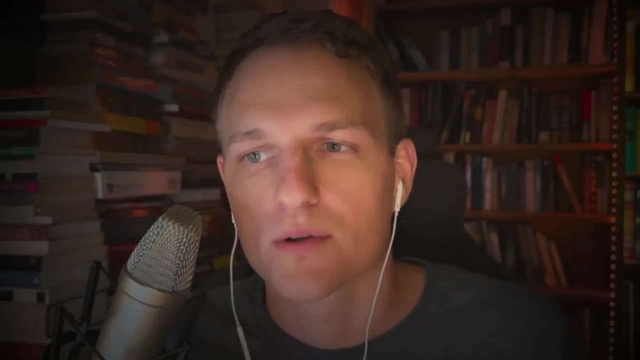 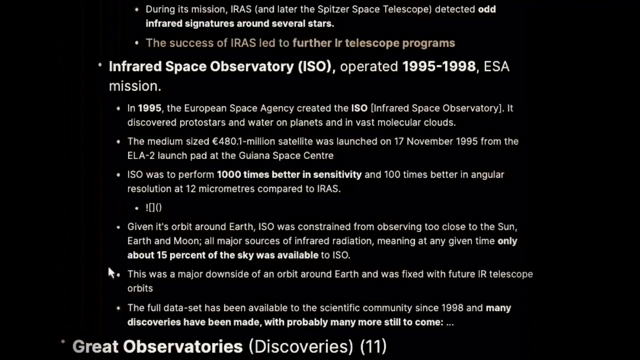 we're already aware of, We're just not aware That we have it on record. And then in the 90s, of course, we had the ISO, and that's the Infrared Space Absorbitory, a strictly European ESA mission. 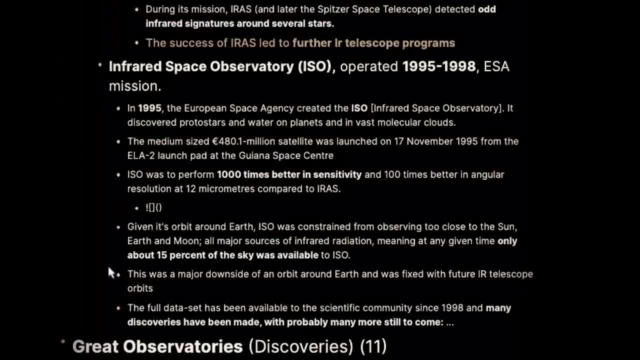 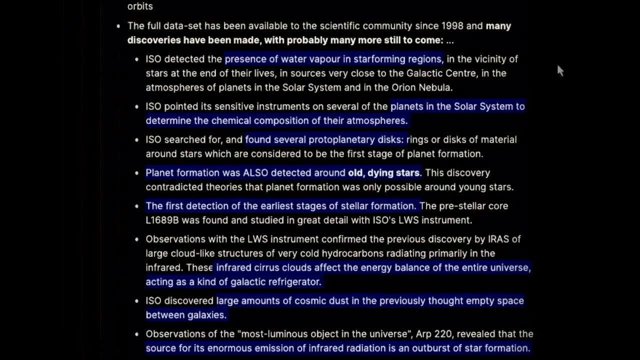 And this was a thousand times better in sensitivity and a hundred times better in angular resolution than IRAS, And, of course, James Webb is probably about a million times better. This made some amazing discoveries, though. ISO detected The presence of water vapor in star-forming regions, indicating that you know that's. 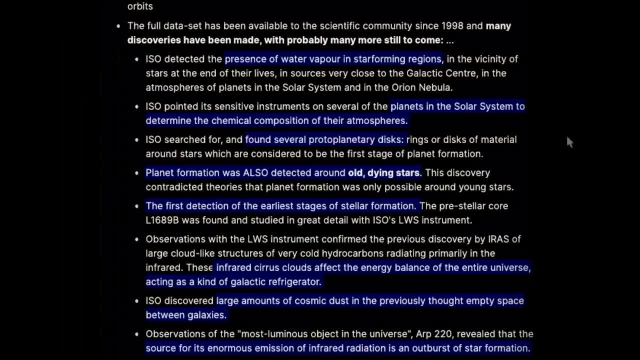 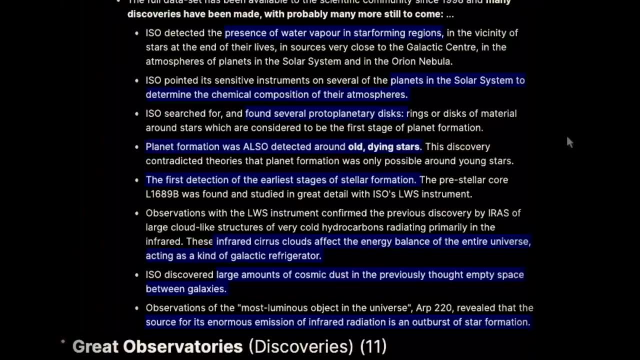 definitely a way we could have gotten water on our planet. It was able to locate several protoplanetary disks of material around stars, which are considered to be the first stages of star formation. It detected old, dying stars too. It's um with uh with planets forming around them still. 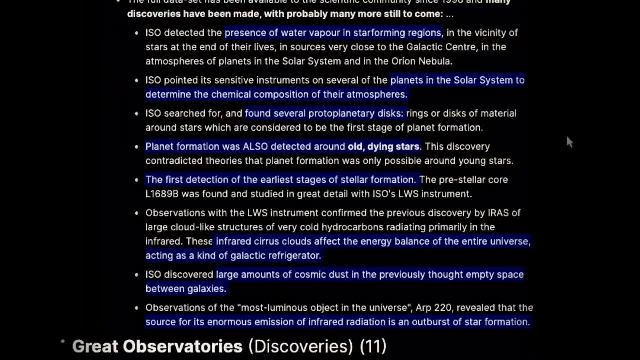 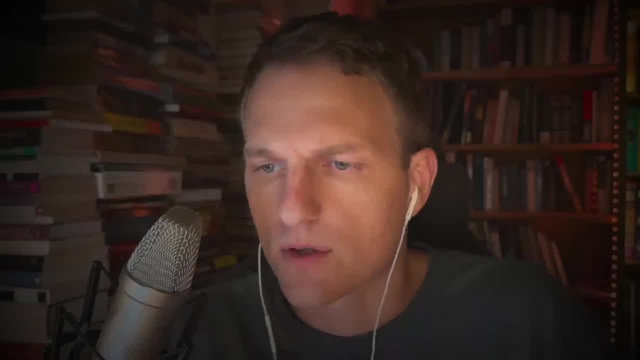 So it completely contradicted theories that planet formation was only possible around young stars. And yeah, there's so much other cool things, but, um, I think maybe one is ARP-220,, the most luminous object in the universe, was discovered by ISO. 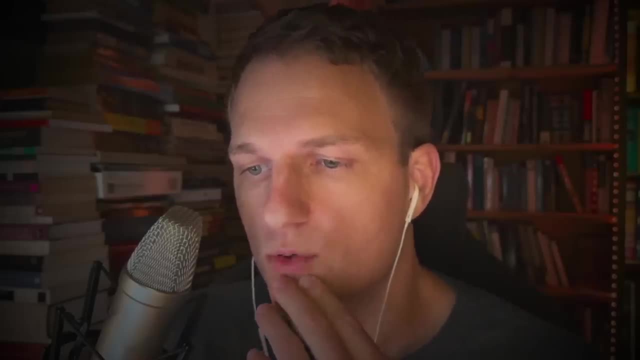 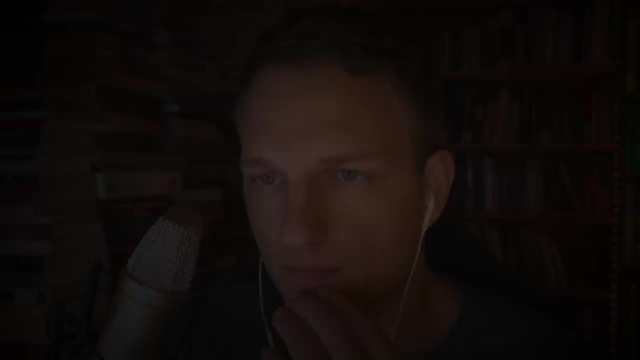 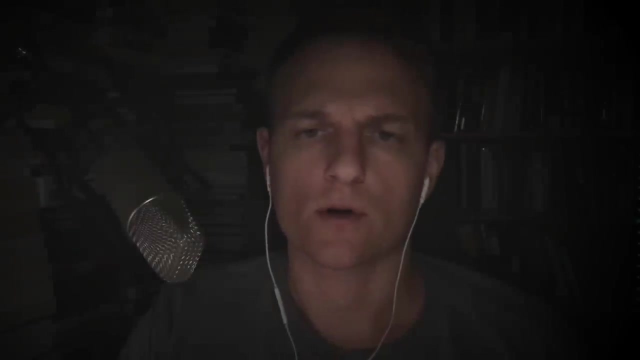 Revealed that the source for this enormous emission of infrared radiation is an outburst of star formation. So dark matter is um a huge part of the universe, and we still don't know what it is. We've been speculating about it for almost a hundred years now. 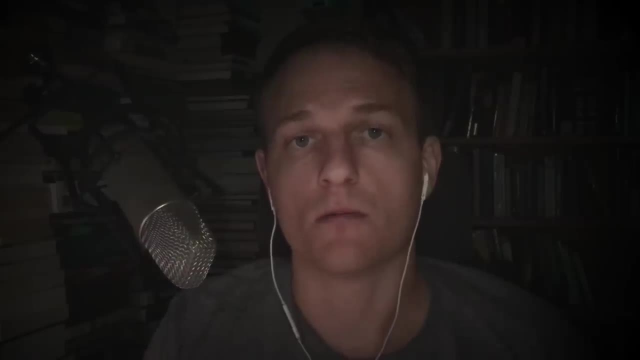 And the current cosmic, The current cosmic, The current cosmic, The current cosmological model of the universe is called the Lambda. It's called the Lambda LCDM model, the Lambda Cold Dark Matter, Big Bang model. And the cold part of the dark matter is: 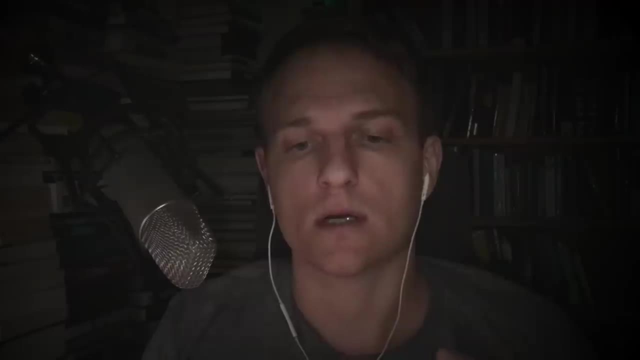 Indicates that the matter, the dark matter, doesn't re-interact with regular normal matter or the radiation, the light coming off of normal matter as well. So it's- um, It's definitely a dark foreign substance that we haven't detected yet. 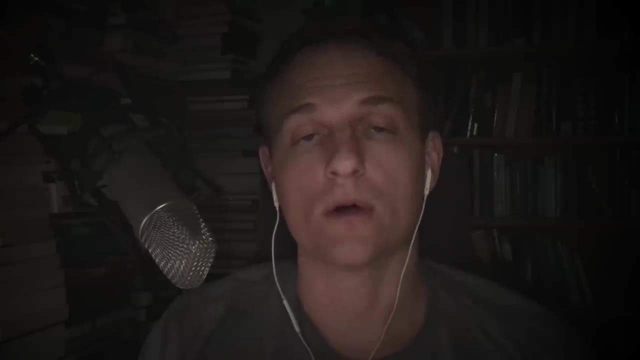 And particle accelerators on Earth are really one of the huge hopes is that one of these days we'll be able to detect some signs of it in a lab And, uh, we're going to see. Now we're going to talk about dark energy. 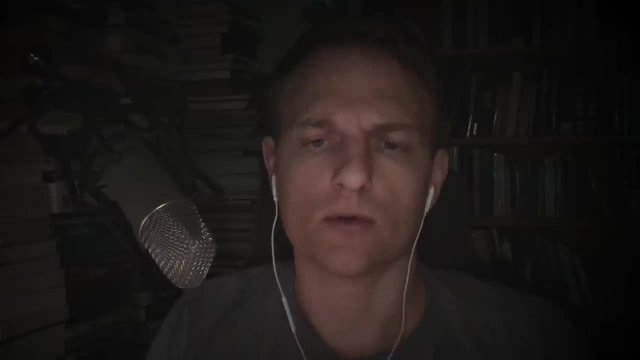 And now that's revolutionized cosmology. Hubble only was looking through optical, you know old-fashioned telescopes, we'd say. And uh came up with his theory. It turned out that that theory of constant expansion held true only up to a certain redshift. at which the universe appeared to be expanding even faster than just a constant velocity. It now appeared to have an acceleration to it. So in the mid-90s Hubble started really making strides in astronomy and cosmology, once it got its lens fixed. 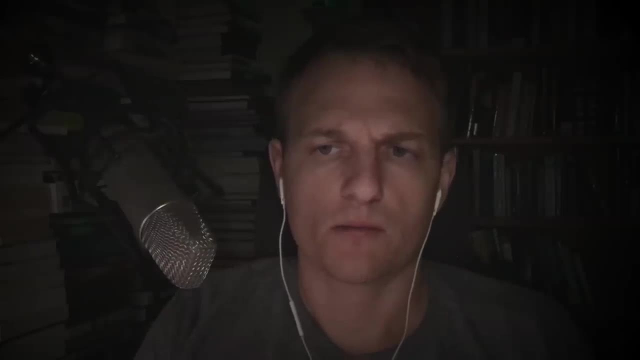 But let's talk about where cosmology went once Lemaître was vindicated in the 60s From his 1930s hypothesis about the primeval atom, the Big Bang, his first, uh, being the first one to talk about the Big Bang. 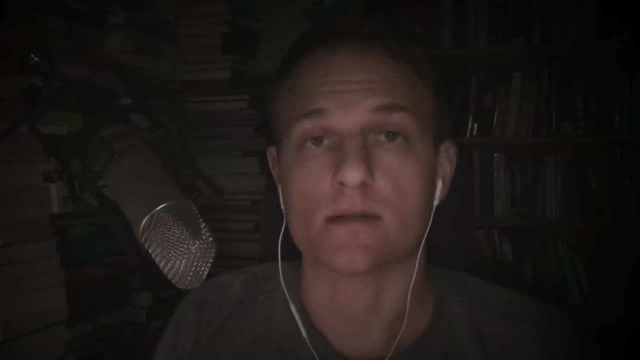 Since then, um, in the 60s, when Penzias and Wilson discovered the first evidence data of the cosmic microwave background, we realized: okay, this was predicted from Lemaître's theory about the Big Bang where, if it did come from a- uh, a single point of origin, then there would be this, this state of the early hot. 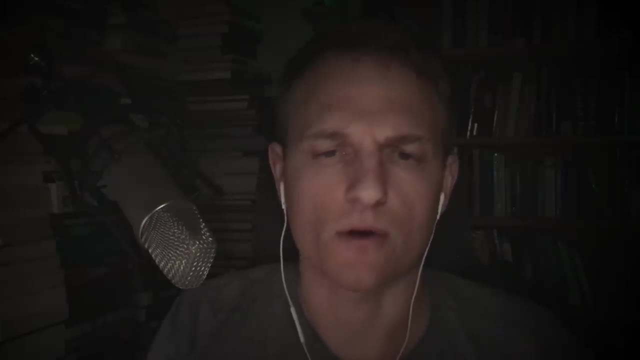 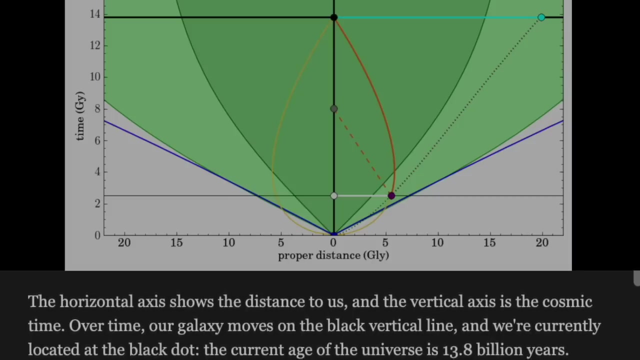 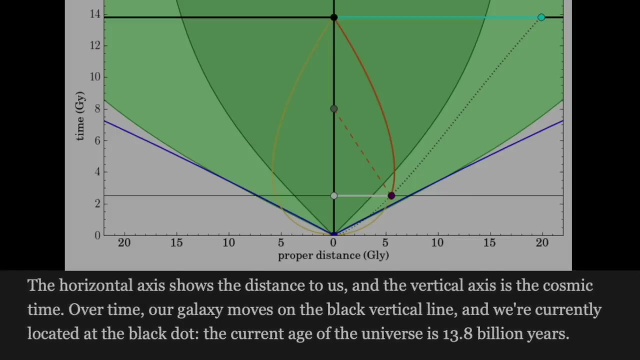 And this is really important here- I I never had really heard or maybe paid attention to it, But this idea that what I find fascinating is the idea that space-time itself, if it's expanding, that means that further back in time it gets more and more. 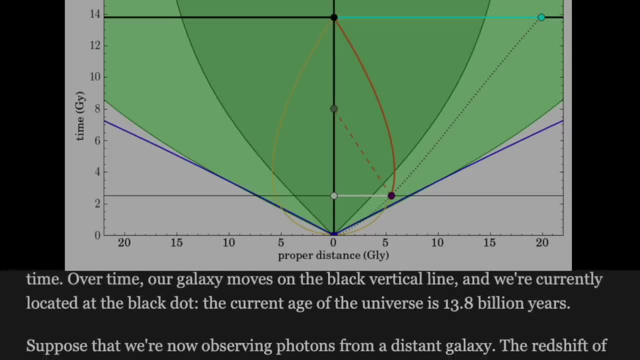 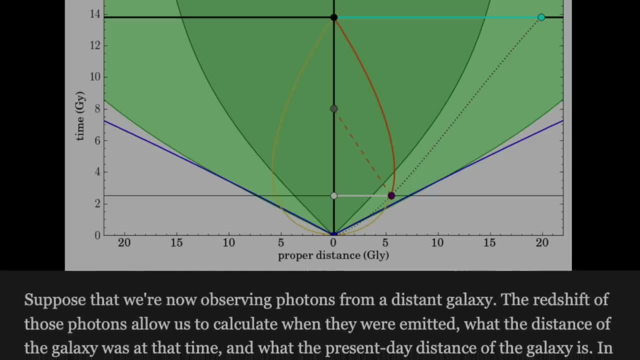 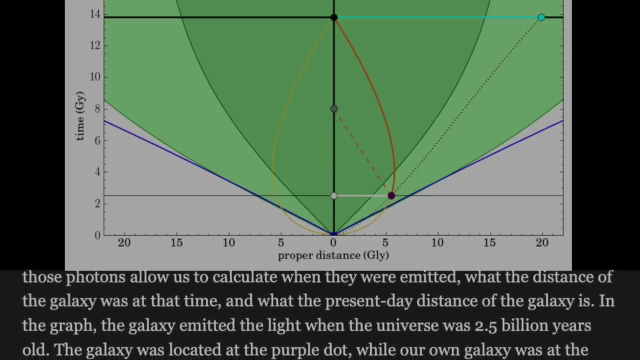 It gets more and more condensed, And that doesn't mean the space between matter is is just um. it doesn't mean that particles are further apart. Or it doesn't just mean that It means that the space, the fabric, the, the, whatever, the, the nature of space-time itself is. 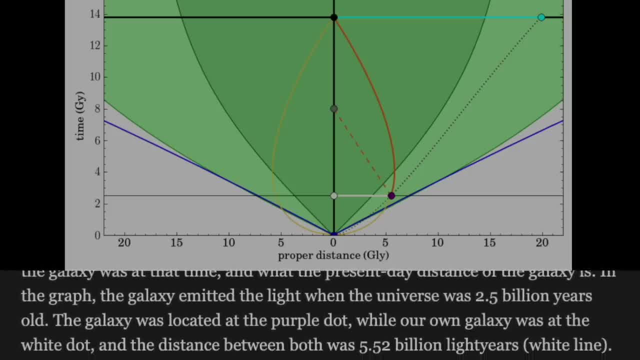 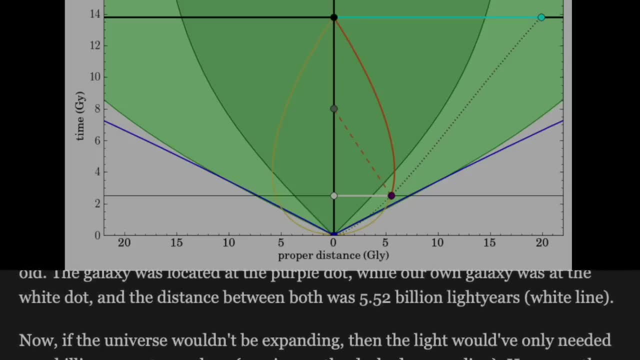 the thing that bends and distorts light through heavy, massive objects, whatever the nature of that, is that thing. that metric is the thing that bends and distorts light through heavy, massive objects. It's the thing that bends and distorts light through heavy, massive objects. 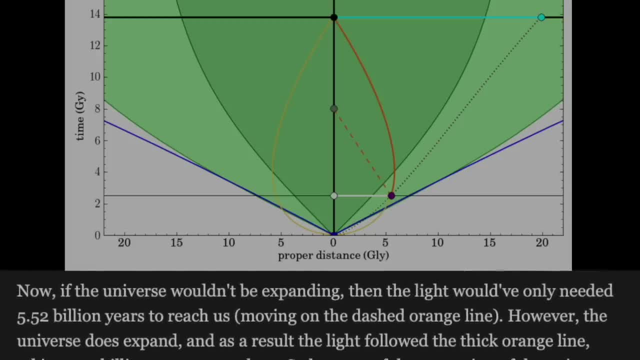 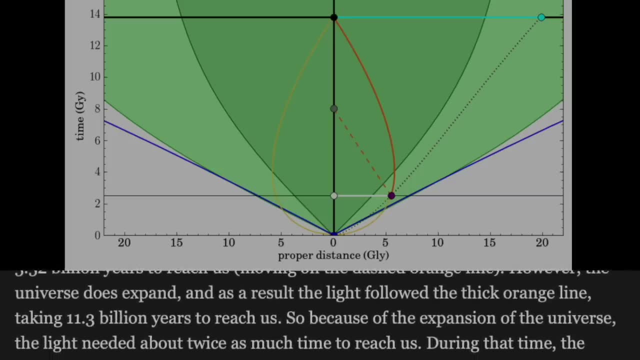 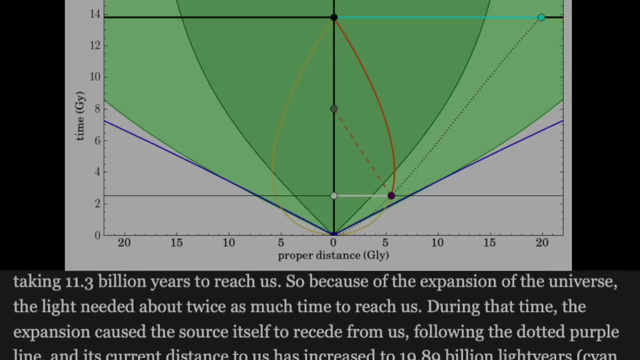 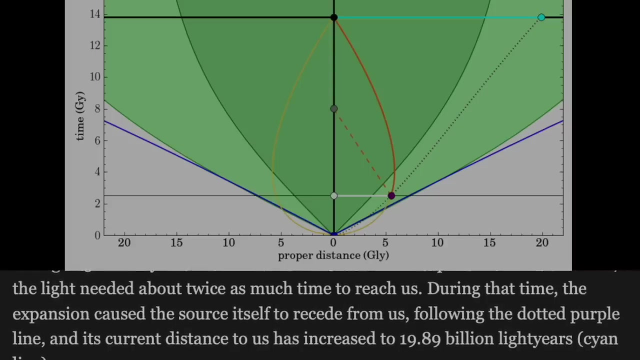 Condensed, And it means essentially that the radiation emitted from galaxies of the earliest and furthest galaxies was emitted. Since then, the space across and in which that light is traveling has expanded, And so an interesting effect that cosmologists all agree upon right now. as of now, 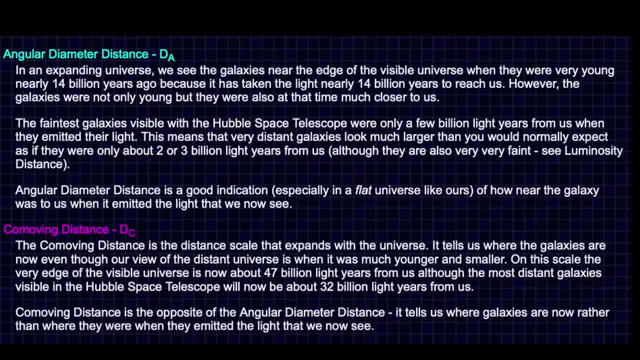 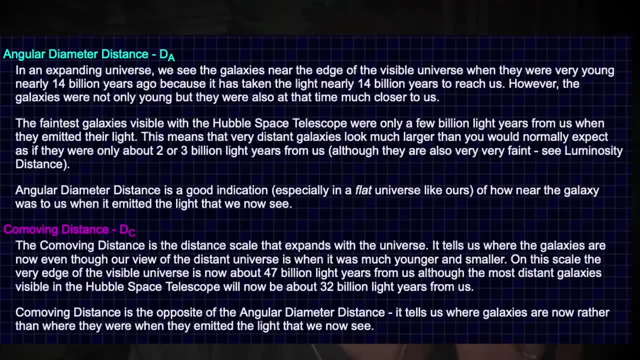 until James Wynn breaks this whole theory. is that galaxies way in the past because space is accelerating in expansion. they actually the radiation, the light coming off those distant galaxies that are now, you know, 30 billion light years away from us. 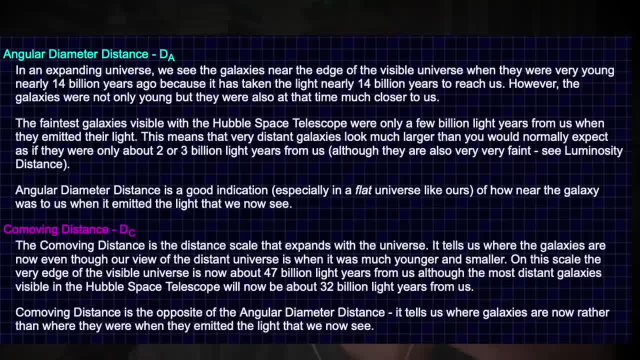 appear larger than they otherwise would in a universe that has not been expanding. Even in Hubble's universe of constant expansion, those galaxies would look much physically smaller on the sky, But because of the actual expansion of space they are magnified. 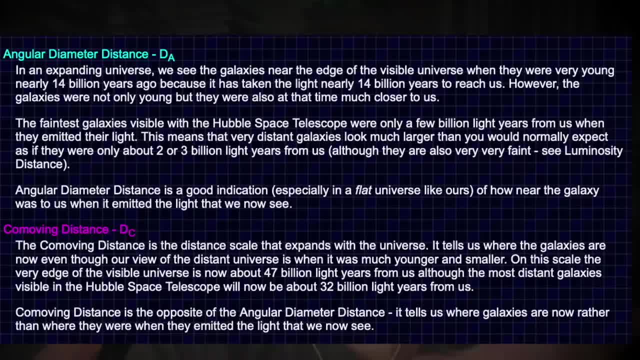 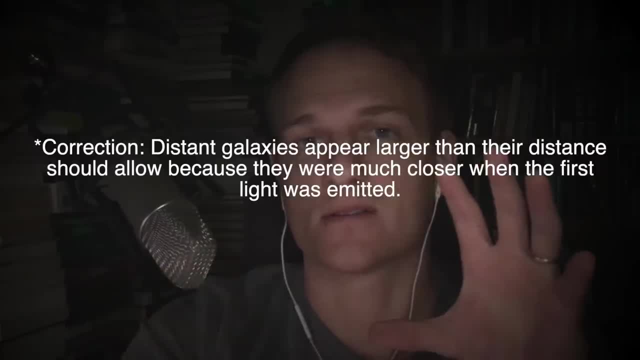 So not even through gravitational lensing or anything like that. That's additional magnification. These galaxies are just magnified because of how far, how old the light is and across how much expanding, accelerating expansion of space they've been traveling, And because light 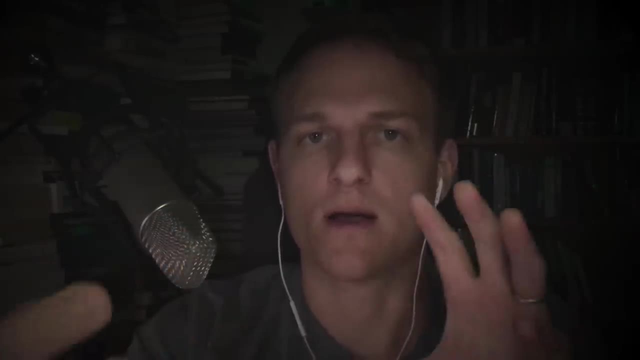 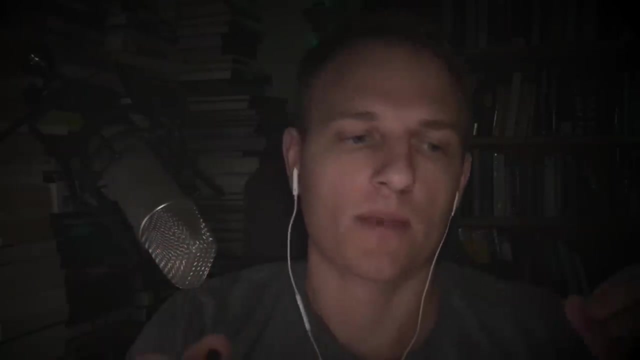 another fascinating thing to think about is that the way we view the current paradigm of the universe is that light is connected with space-time itself, So it expands as space-time itself expands. So if you have a wavelength with a frequency of a billion hertz, 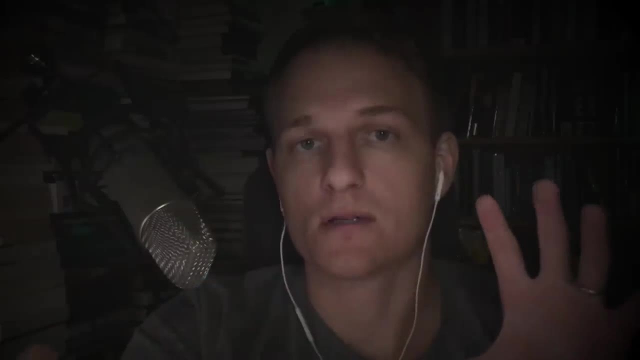 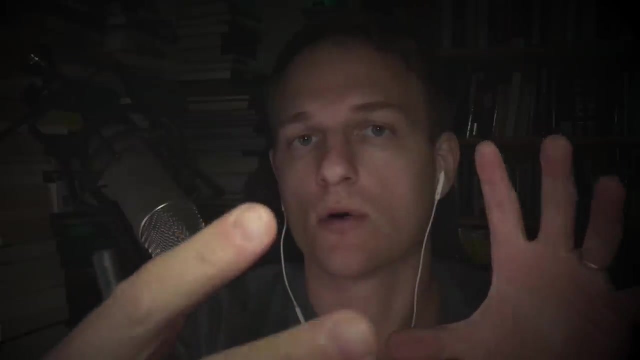 that frequency as it travels across billions of galaxies, over billions of light years of space, over billions of years, that frequency is going to go and get shifted to a lower, longer wavelength, a lower frequency, I think, at the furthest distances. 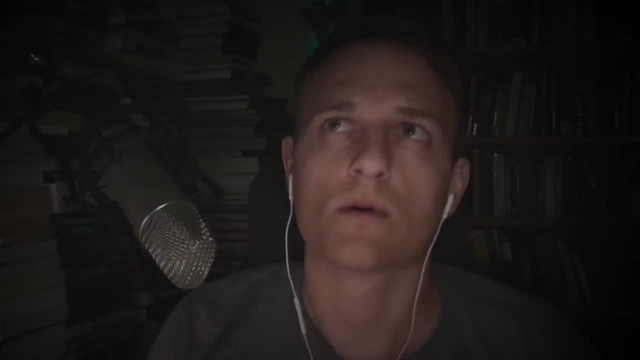 it is a shift of a thousand. Is it ten times more than a redshift of one? It just corresponds to a different distance. Yeah, I think so. So, yeah, it could be shifted from a billion hertz. Yeah, I think so. So, yeah, it could be shifted from a billion hertz. 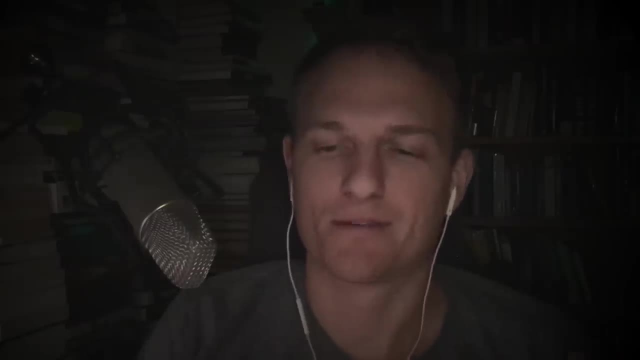 It's my understanding as a physicist. I mean, if you're watching this and you're a physicist, You're definitely not watching it for my expertise. So I guess I won't feel too bad about making some minor errors here. Hopefully it's not too egregious. 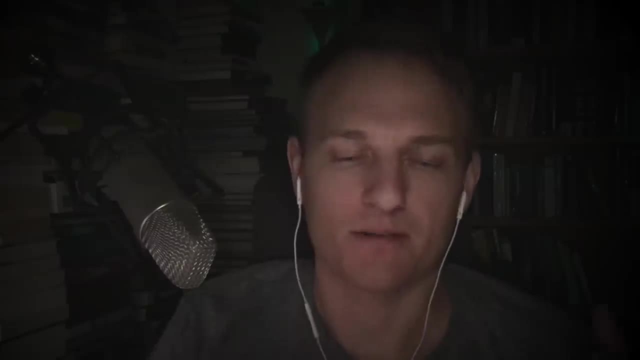 If we have a billion hertz, basically it might shift, it might downshift, redshift, downshift, redshift to maybe a hundred million hertz, redshift to maybe a hundred million hertz. It's just astounding. It's just astounding. 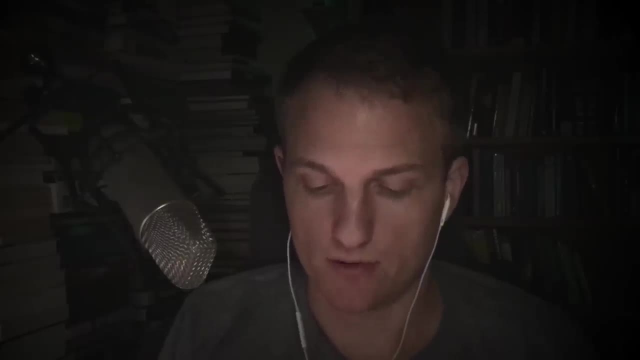 nature of our universe. space-time itself expands and distorts, not only distorts the size of, but it slows down the light being transmitted across space-time, so that light, so those galaxies and things in those galaxies appear, I think, something like twice as slow as they actually happened to us across 13. 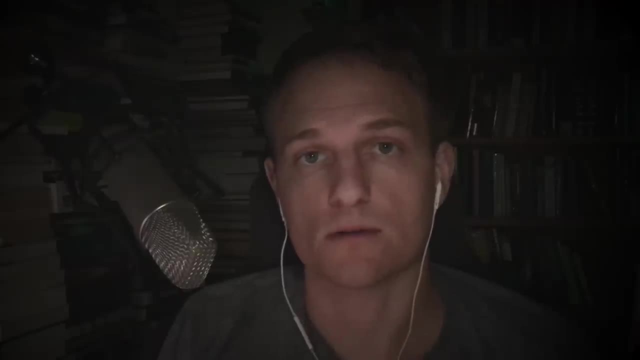 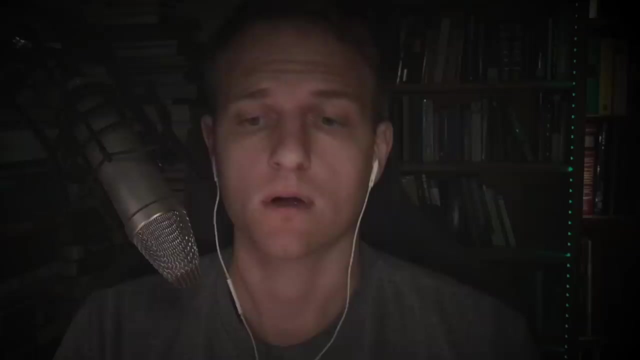 billion years of cosmic history and 30 billion years, billion light-years of distance expansion, expanding space, the the rate at which things happen appear to go about twice as slow. it was really important to know that you, although we hear a lot about dark energy, that wasn't even a theory, because 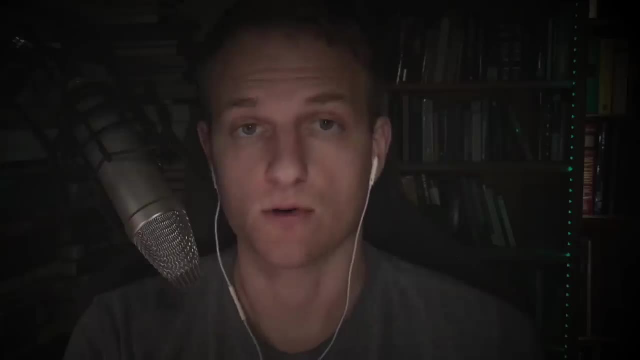 it because its effects weren't observed, observed until Hubble performed some deep fields in the late 90s and until then throughout the 70s, 60s, 70s and 80s, with all scientists had, all cosmologists had, were the theories of cosmic, the 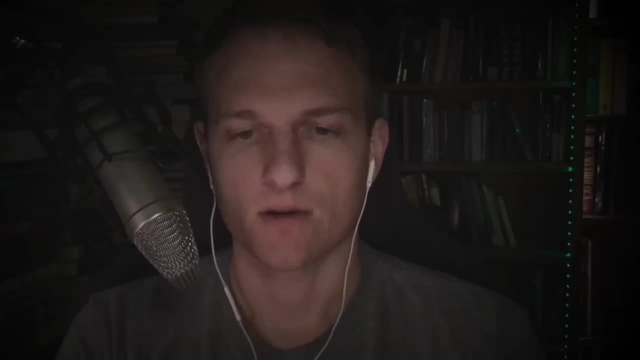 cosmic microwave background or, sorry, the dark energy theory. for the last 20 decades, the number of stars in this matter waslardan okay, and also one of the more complex mysteries that you can move around and see their upside down as they go. you all the observations. they had to go on with. the two biggest cosmological phenomenon were other than theolutions. they had to go on which a two biggest cosmological phenomenon were, other than observing galaxies and their dynamics, was the Cosmic microwave background, which told us a lot about the very first light. the furthest back we can go the the opaque wall. 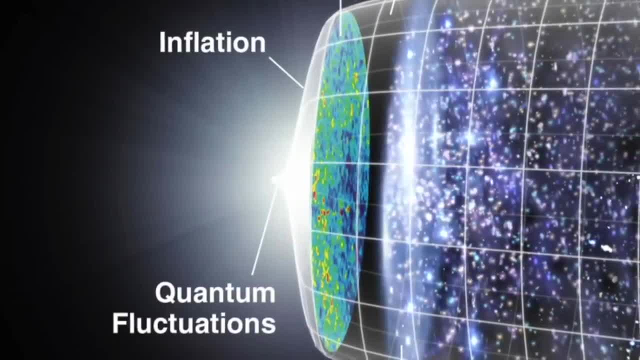 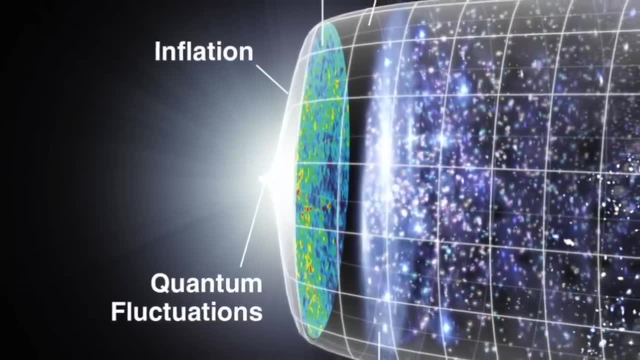 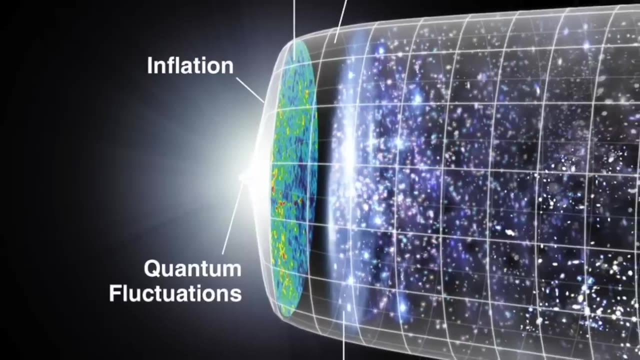 it's beyond which we'll never be able to see. So it happened everywhere. but as the universe evolved, it evolved into stable atoms locally, and then, of course, it takes light time to travel from distant objects towards us. So it appears like the universe. 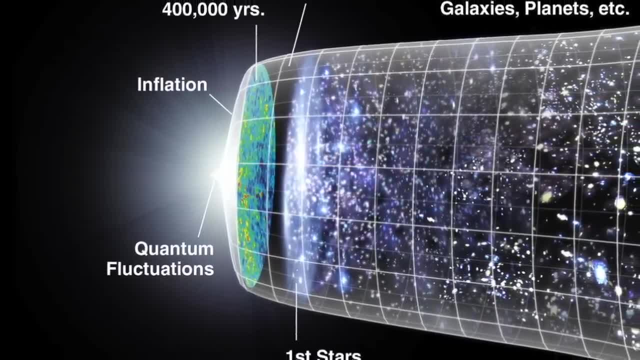 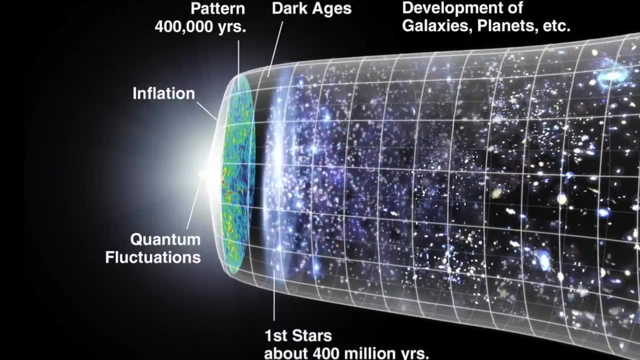 well, it's basically. we're seeing the universe as it was at earlier stages of its evolution. the further back we look, until the earliest possible stage we can ever see is this sphere that was 40 million light years away, 80 million light years in diameter. 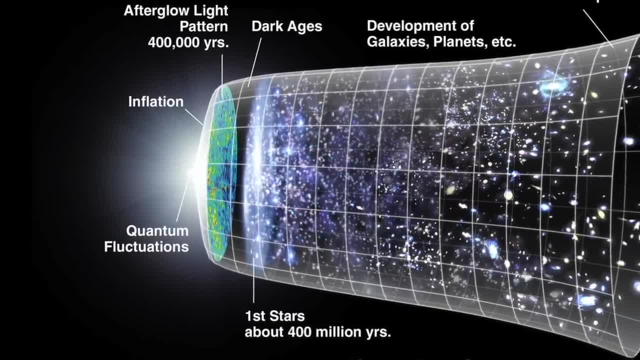 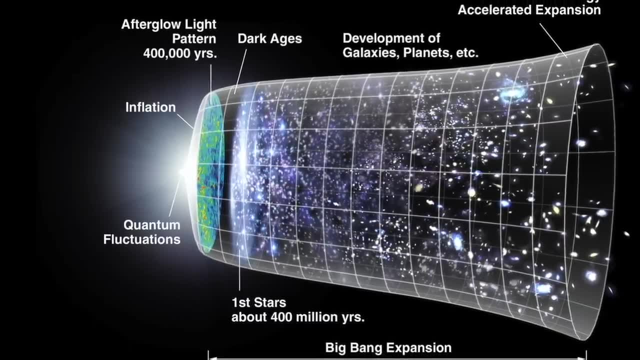 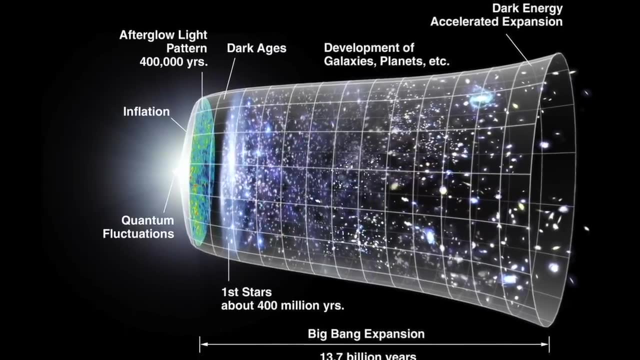 and has now expanded to 93 billion light years in diameter, about 46 billion light years away. That's the boundary of the observable universe. It's not the boundary. we don't even know if there exists a boundary of the universe, but that's. 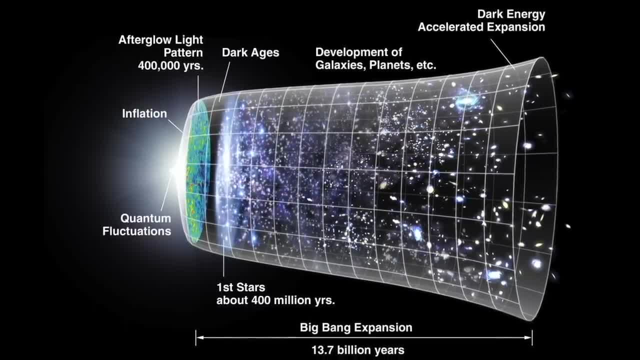 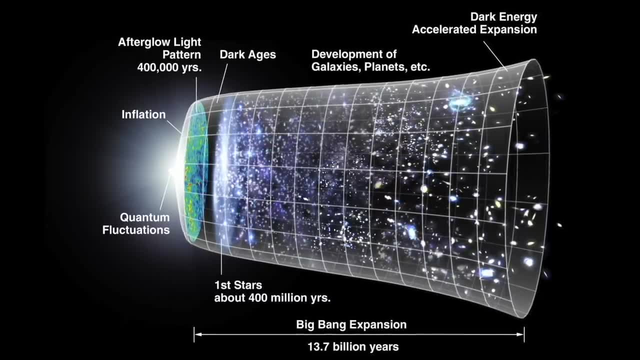 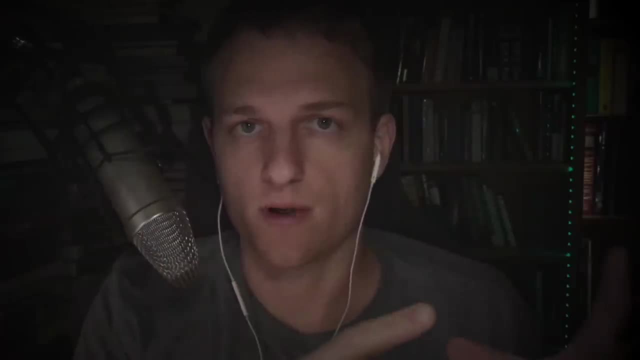 that is the particle horizon of our universe that we exist within. So until the discovery of dark energy in the late 90s, all we had was the cosmic microwave background and this knowledge, this observation of galaxies that move faster, that appear to move with more gravity. 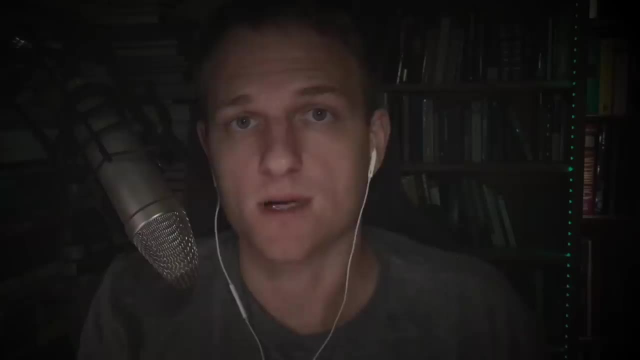 and under the influence of more- about 10 to 20 times more gravity than their luminous matter suggests. So that's why we hypothesized this dark matter And that that influenced the cosmological models that have been created ever since. We only thought, hey, ordinary matter was about, I think, something like 20%, and dark matter was like 80%. 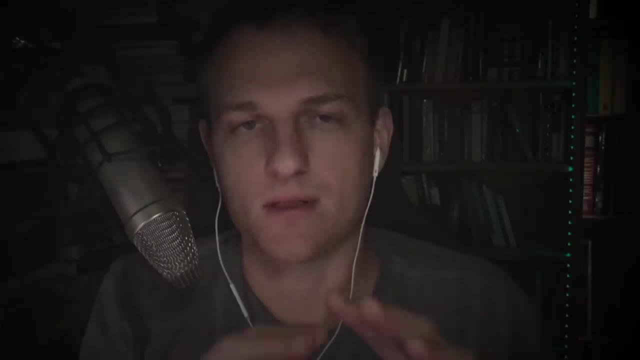 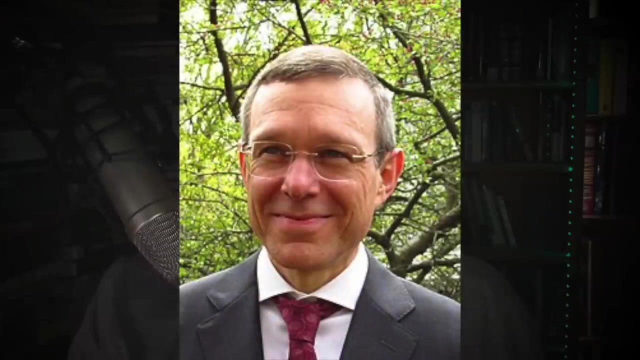 Nowadays. well, let's just put it there until we discover what dark energy really is and how it came to be known. But I think Harvard astronomy professor I mentioned earlier, Abbey Loeb. he has been on Lex Friedman's podcast, I think, once or twice. 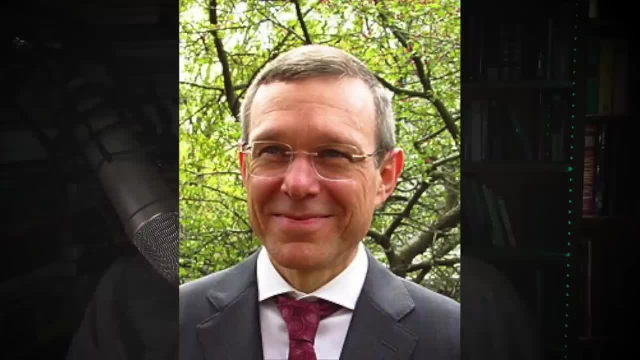 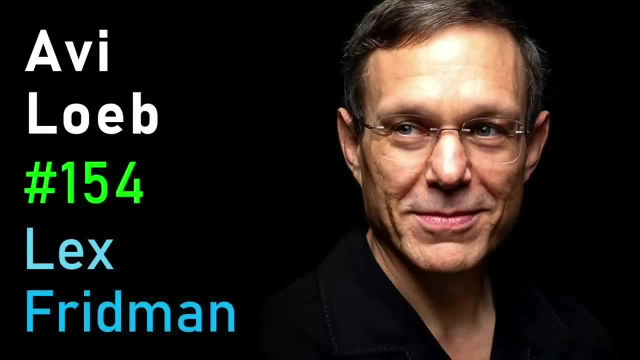 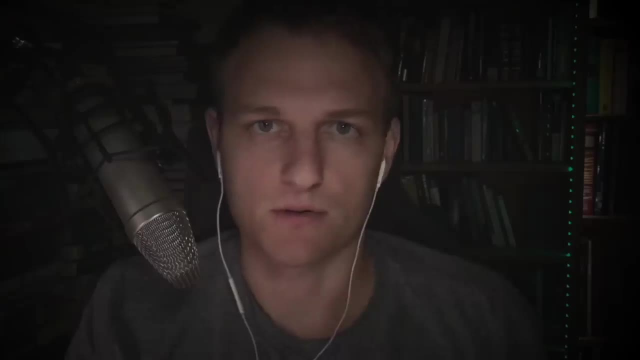 and he's been on a couple other. Dr Brian Keating. he's been on that podcast a couple times. He's a really interesting guy to listen to talk about aliens or the early cosmology. I would highly recommend him. He said it's tantalizing to contemplate in his book The First Galaxies. 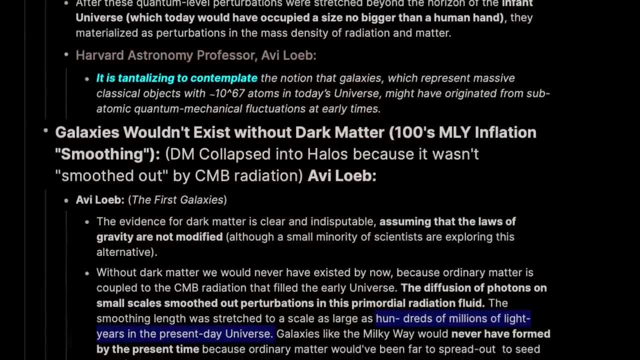 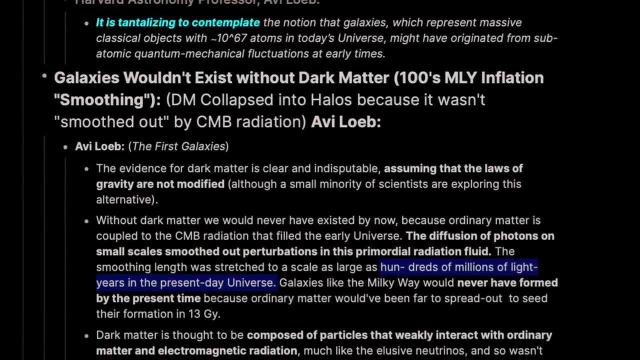 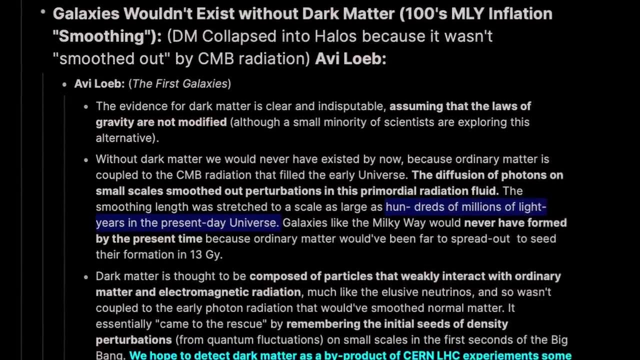 He said it's tantalizing to contemplate the notion that galaxies, which represent massive classical objects- 10 on the order of 10 to 67 to the 67th power atoms- that many atoms is an unimaginable amount in today's universe- might have originated in subatomic quantum mechanics. 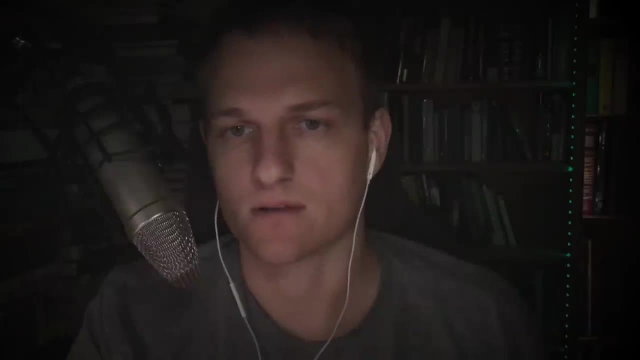 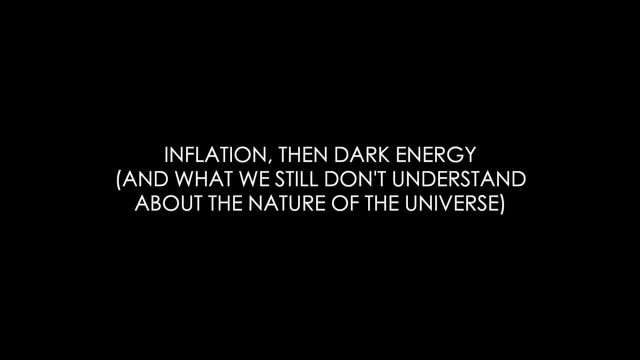 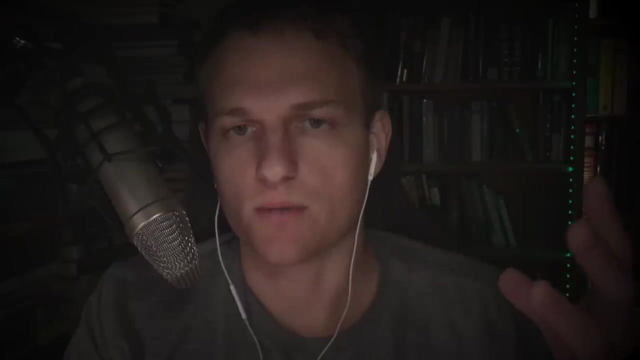 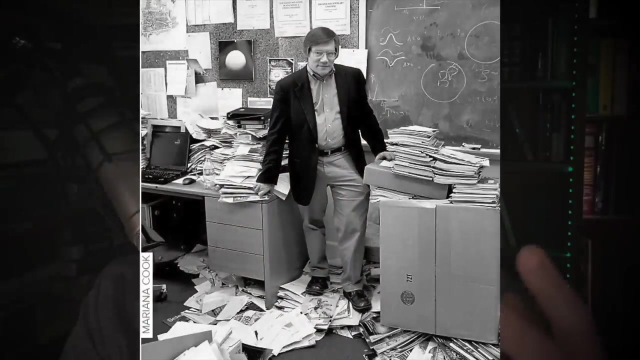 And mechanical fluctuations at these earliest seconds of the universe, before inflation. So we had in the 1980s, before dark energy was known, this guy, Alan Guth, was looking at expansion of the universe and wondering why gravity in the universe hadn't contracted it. 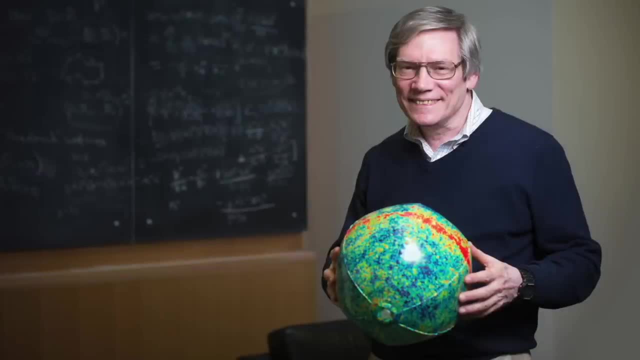 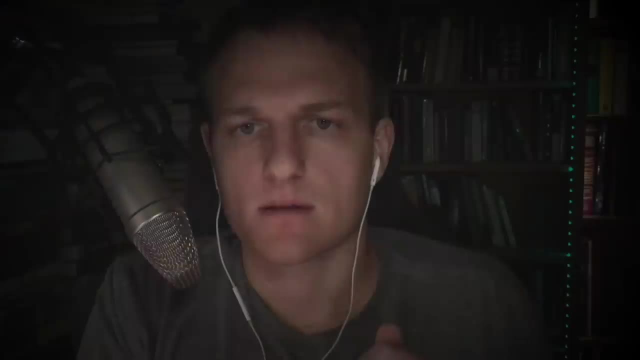 So, even though we hadn't contracted it, even though we hadn't contracted it, he said that even though the early Big Bang- because inflation wasn't a thing- and the earliest models of the Big Bang theory didn't incorporate the inflation that I mentioned in the beginning of the universe, 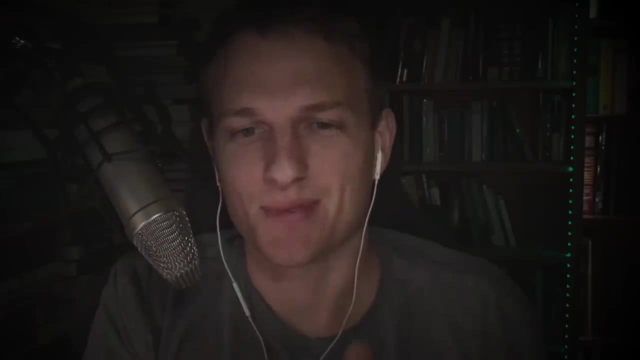 in the beginning of what seems like the length of the universe. now What I mentioned in the beginning, where it swelled up from the size of a you know dna to 10 light years across, or the size of a cell to, was it, 110 000 light years across. 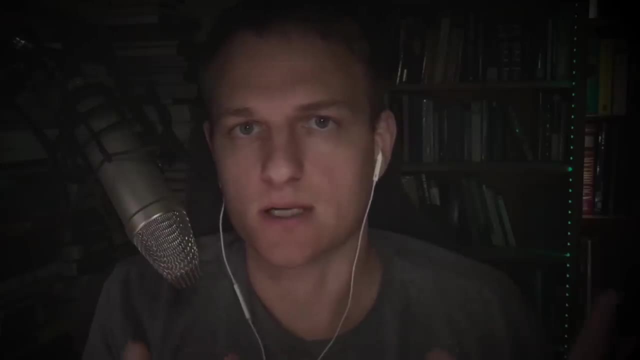 that was originally not until the 1980s. that was not a part of the big bang model. the big bang model was a, an expansion of the universe out of a single point, but it didn't have that other additional component of inflated expansion over the, you know, over a millionth of a second. 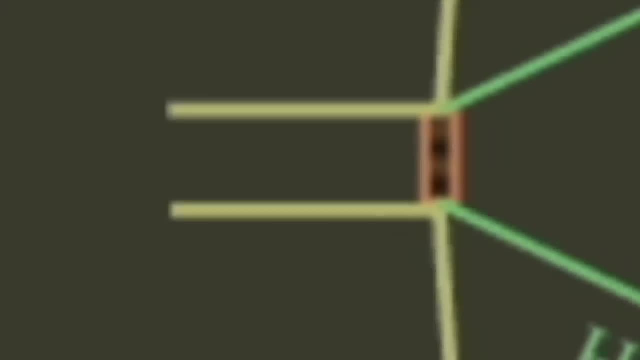 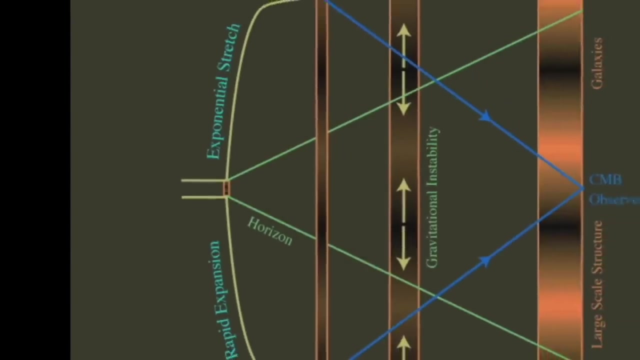 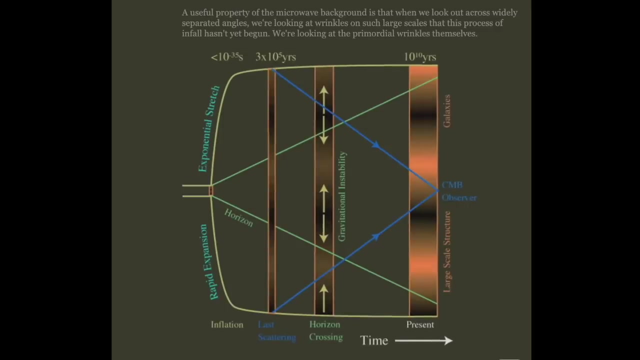 that inflated the universe right after right around the origin, first trillions of a second, and then the universe stopped inflating that. that inflation stopped continuing, it just expanded. the universe began a trillionth of a second later, or so. it inflated at an even faster rate, an exponentially just, tremendous rate. 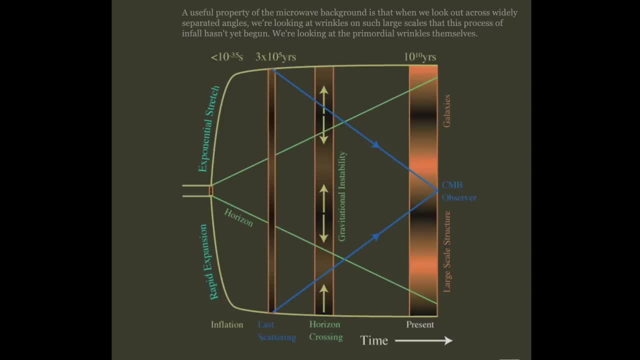 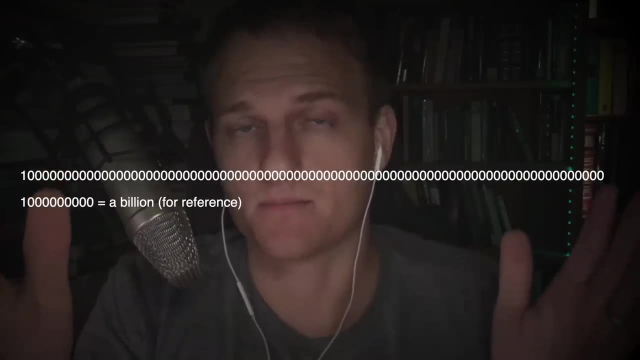 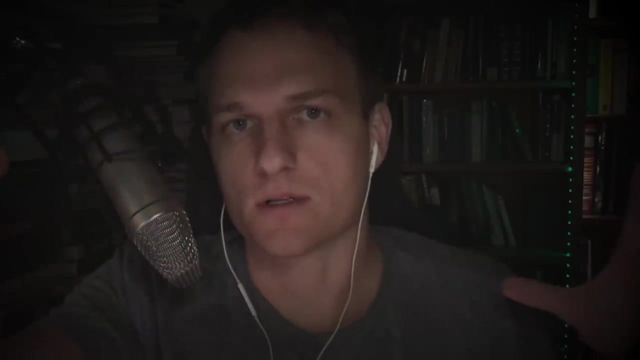 that we. you know, I try my best to explain- 10 to the 78th power, That's literally a 10 with 77 zeros coming after it. That's an enormous, unimaginably enormous scale of inflation. And then from there, the residual momentum of that inflation apparently kept the universe expanding. 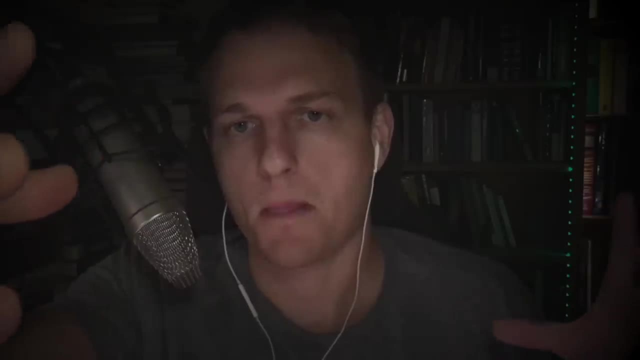 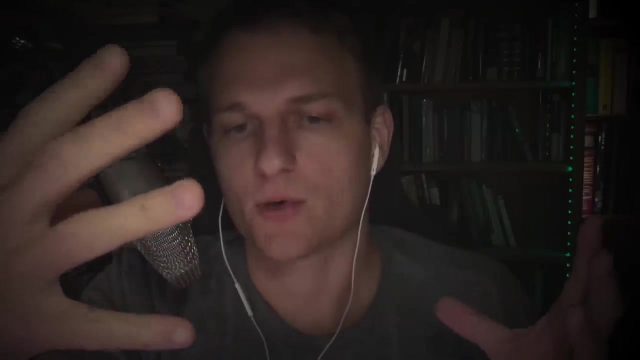 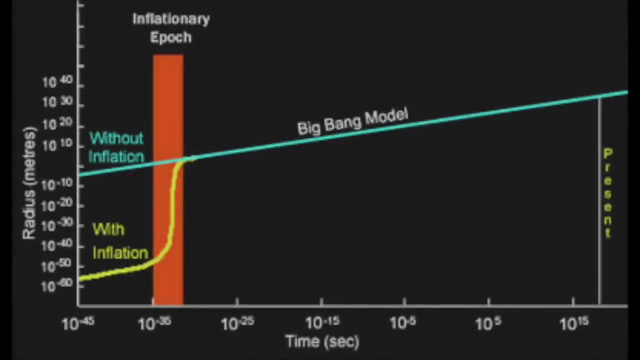 That's the current theory. But back in the 1980s, before inflation was hypothesized, we just assumed the universe kind of expanded at a pretty constant rate, And so this cosmologist, Alan Guth, was right Wondering why gravity hadn't at least slowed the expansion. 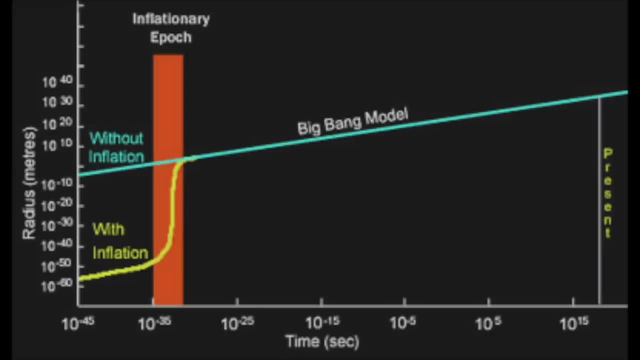 If not collapsed, you know, began a collapse of it altogether, of the universe. And so throughout the 80s and then the 90s, when Hubble began looking, began showing cosmologists and astronomers that, oh, we can look way further back than we realized. 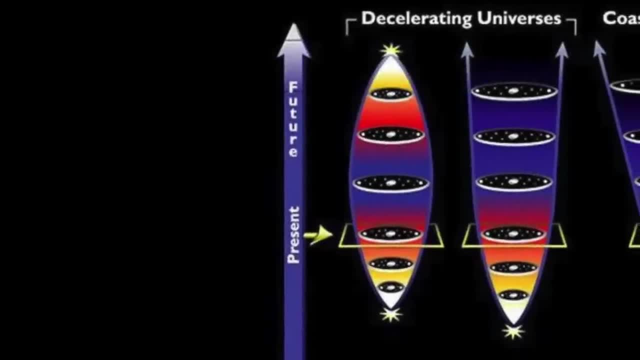 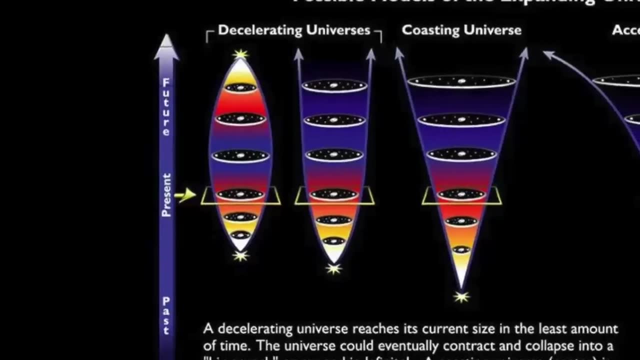 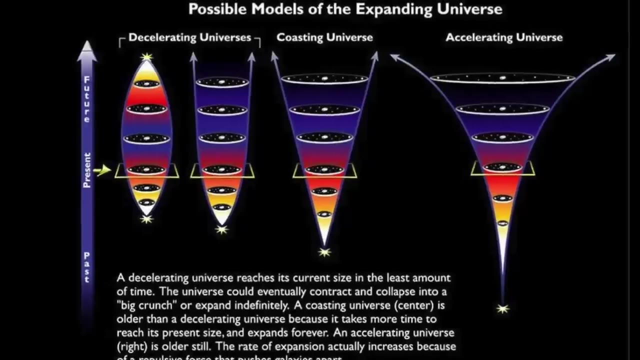 The goal was actually to find deceleration of the universe at the largest scales. It was to say, OK, if, unless there's some other force keeping the universe propelled apart, there needs to be some sort of slowing down at the largest scales. 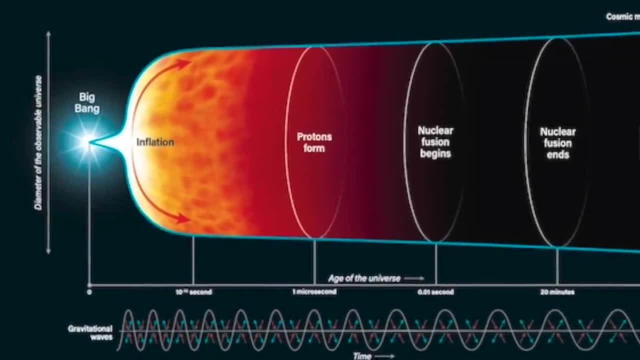 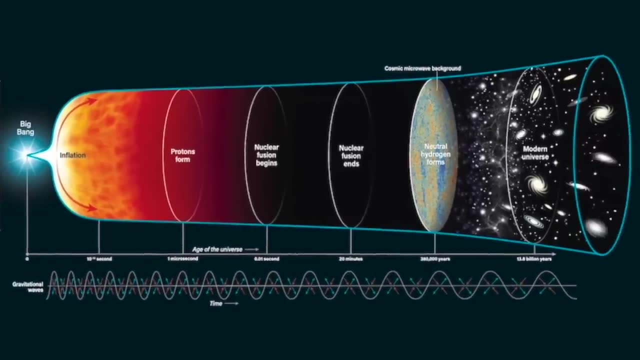 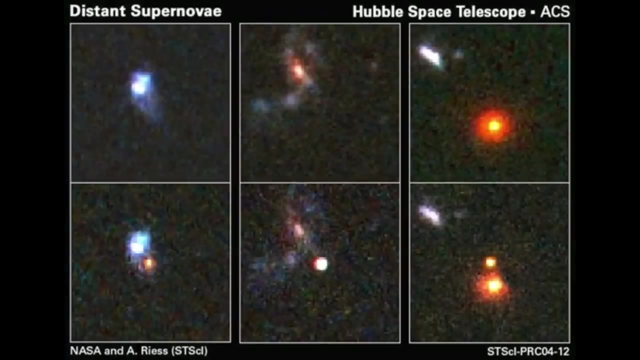 We should see galaxies start to appear less redshifted- And you know the rate at which they redshift should start to decrease at a certain point, And they They look at supernovas, distant supernovae that shine brighter than their entire galaxies. 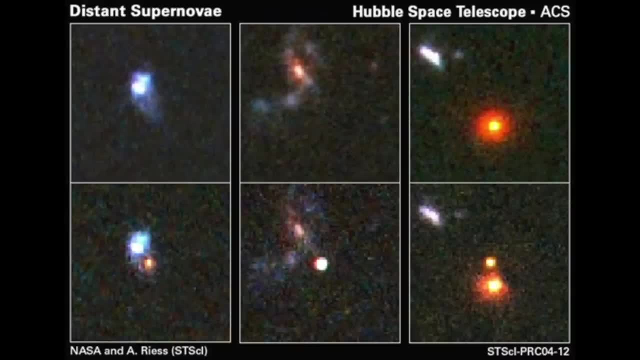 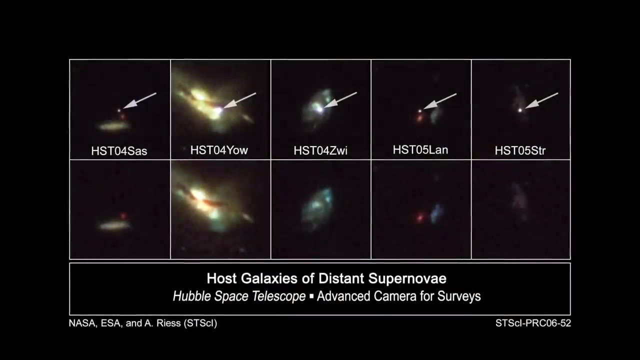 for a few days or weeks or hours to tell them how redshifted or how far away certain galaxies are, And then they can look at the redshift and say that OK, these are inappropriately mounted, appropriately mounted galaxies. 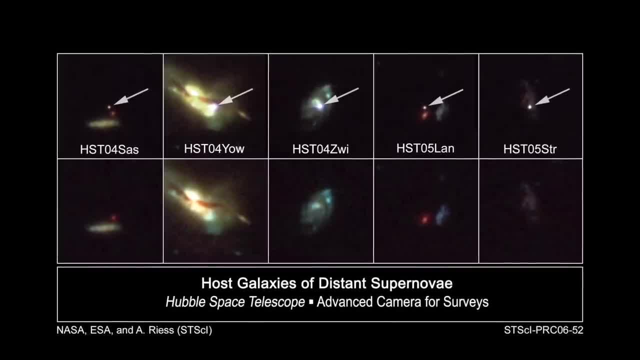 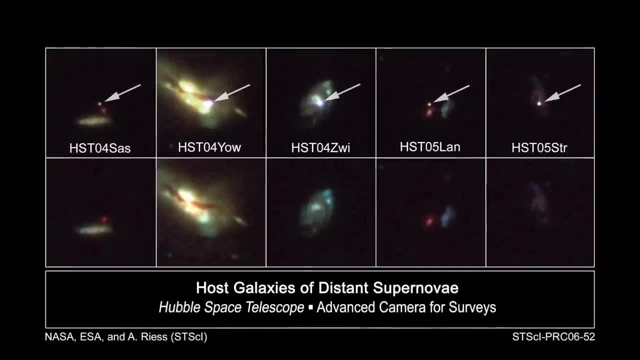 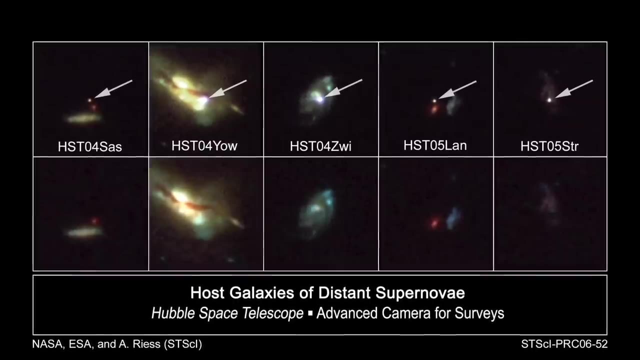 These are inappropriately redshifted galaxies for how far they are away or their velocity is way, way more or way less. They were looking to see a deceleration. They were looking for velocities much less than the local receding velocities of galaxies within you know, a billion light years or so. 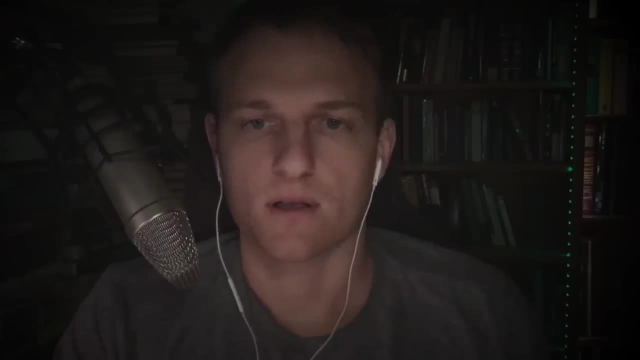 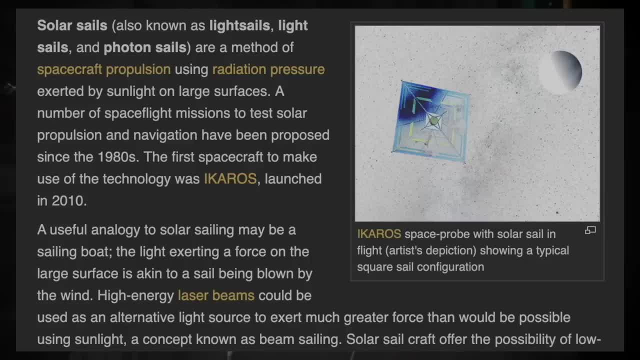 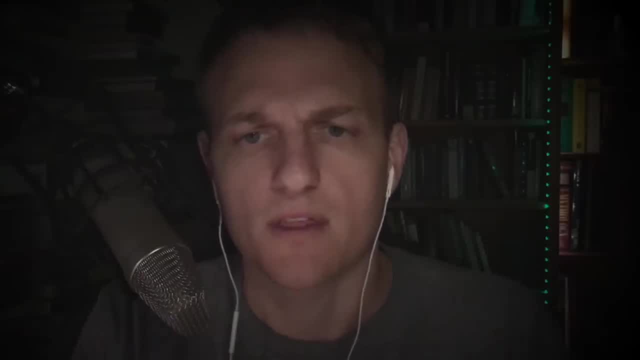 sun, and so there is an outward force, even though it's small. but of course, like we said, i think it's something on the order of a thousand times more photons than all the stars in all the galaxies in the 14 billion years of the entire universe. a thousand times more than that amount. 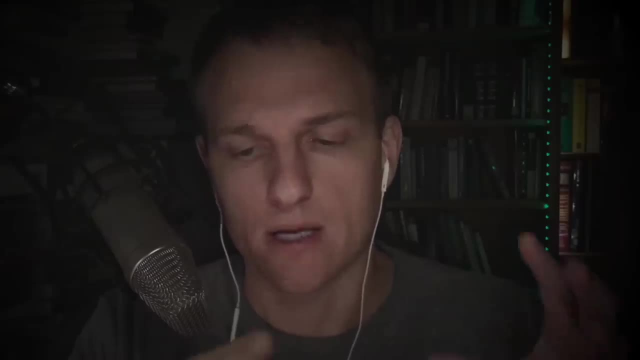 of photons was how much light was emitted by this cosmic microwave background at the time of last scattering. so that tells you it's a lot. those photons add up to quite the force on the original field of hydrogen in the universe that went on to make up the stars and you know matter the rest of. 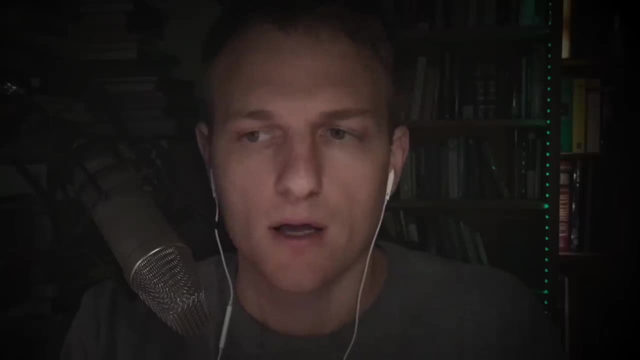 the matter, you of the universe. this radiation would have smoothed out the distribution of matter so much that even gravity itself, even over 14 billion years, wouldn't have had time to allow the stars to condense and or the matter to condense into the first stars. so they're wondering how? 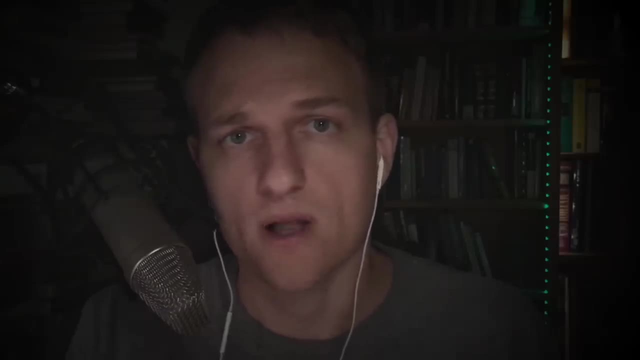 star formation and galaxy formation got underway so quickly in the beginning and this idea of here, the explained for the world is said to be quietly, but this idea of inflation helped explain at by saying that the universe to explain expanded so rapidly in such a brief moment of time is. 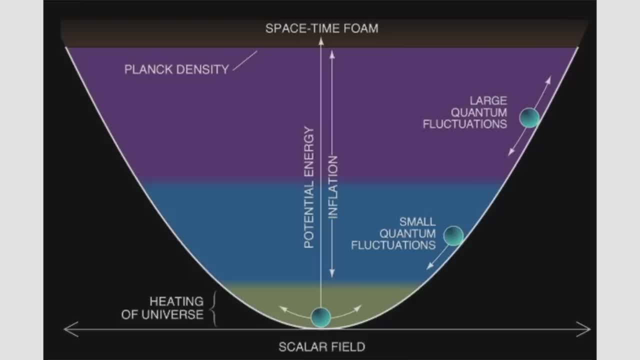 so soon after the big bang, it originated everything that it froze into place through quantum mechanical fluctuations that just naturally exist, or and in random fluctuations in the vacuums, in just the nature of into the netter. just a part of reality is the nature of powerful space. it's just as it. 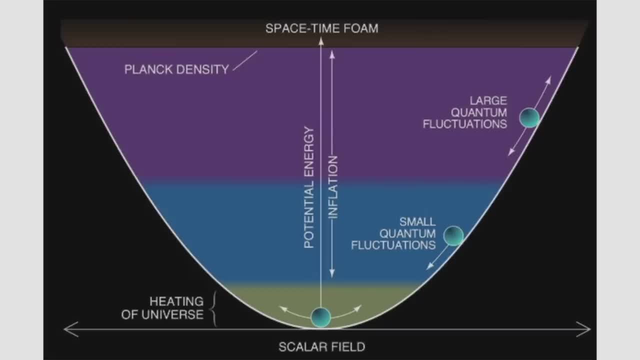 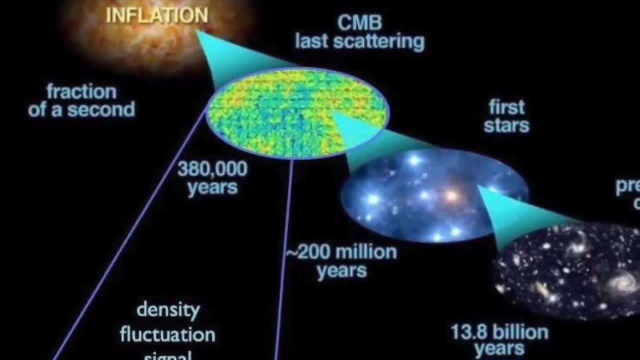 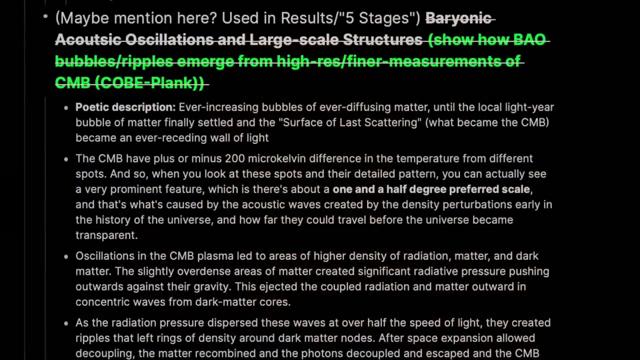 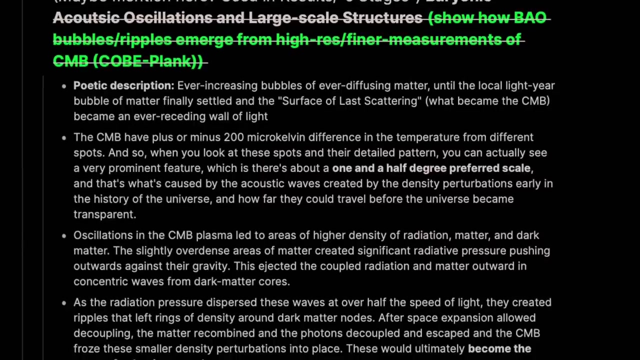 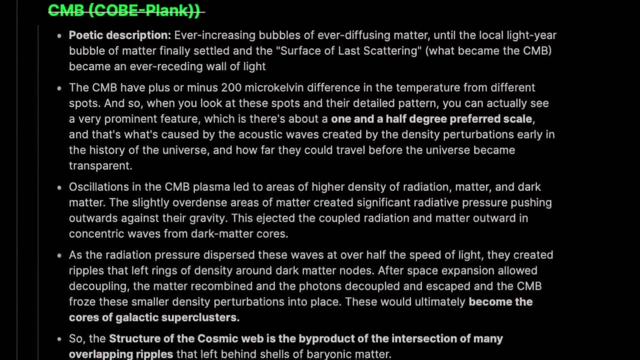 part of reality at small enough levels because the universe expanded so rapidly. these fluctuations that rule in the realm of the small quantum, they got frozen to place. and dark matter, the theory, the reason they call it cold, is because dark matter is not hypothesized to interact or be pushed by that force imparted by the photons, by that massive field of photons. 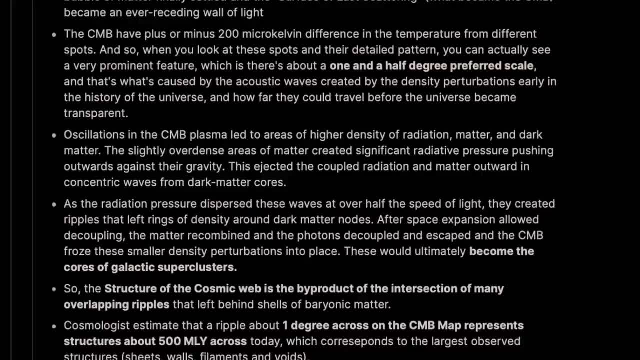 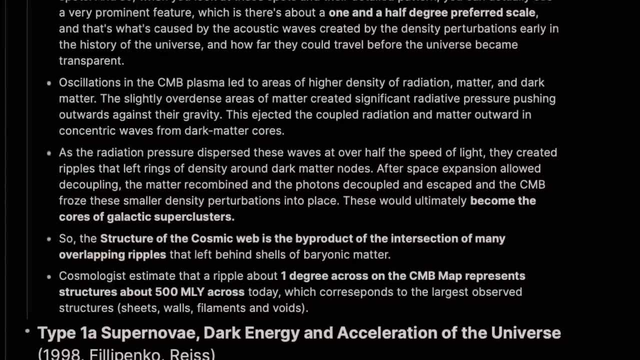 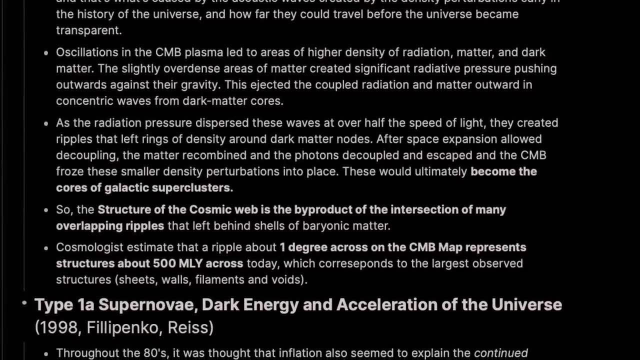 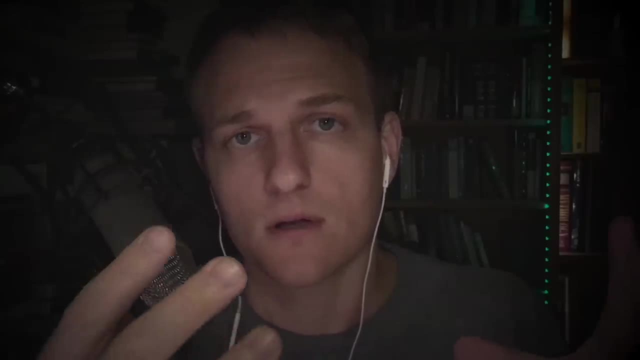 that was circulating around in the early universe. so dark matter, cold dark matter- was actually able to be condensed into the pockets of higher density that the quantum fluctuations froze into space, and then it was around that over a few, you know, over millions of years, it was around that matter, that, uh, that dark matter, those dark matter pockets. 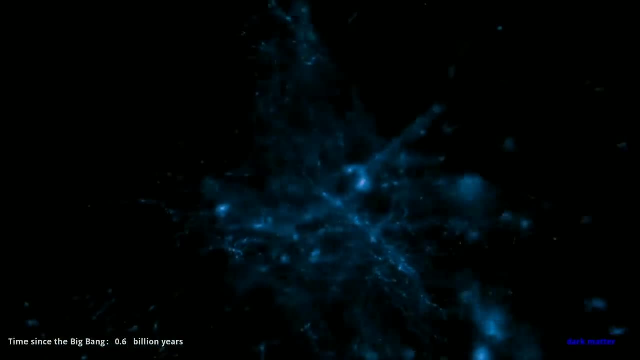 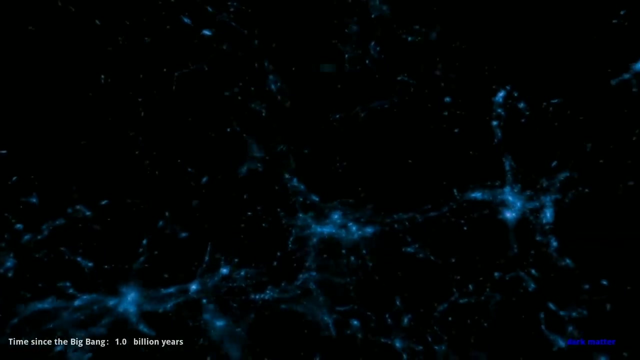 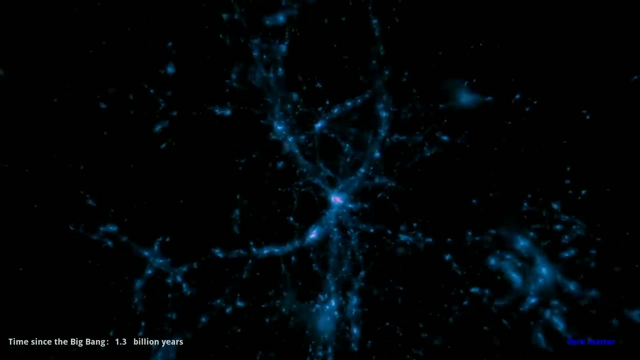 nodes in the universe, that the filaments that make up the cosmic web on the grandest of scales, the filaments of matter, that it began to form these super clusters of galaxies, and so it's thought that, um, actually, it's literally what. this is right here. 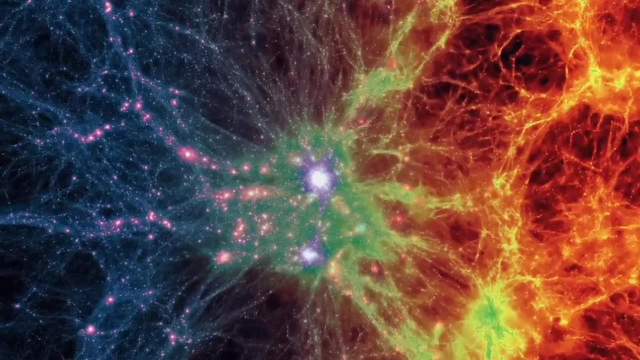 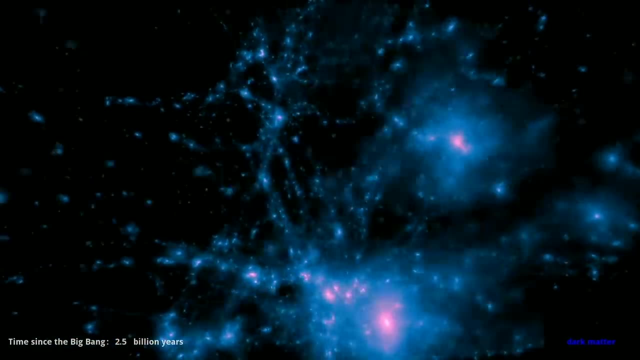 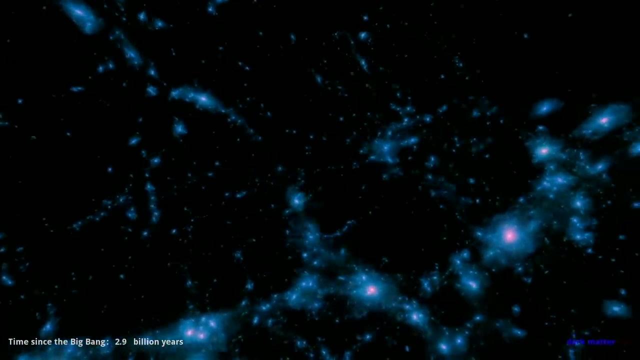 it's just really interesting to me to to understand that we thought we had it mostly figured out and there's been multiple times in the history where we've thought we had it figured out. i think, um, i forget what it was. i think in the 1800s it might have been lord. 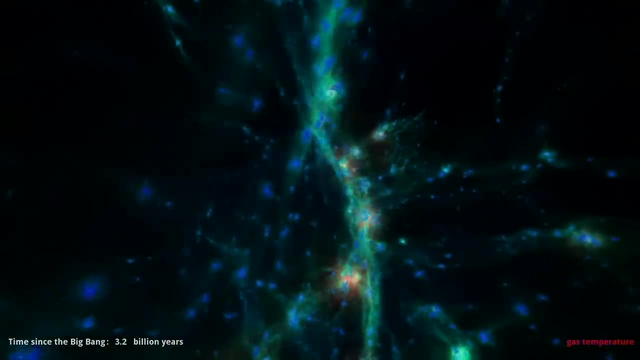 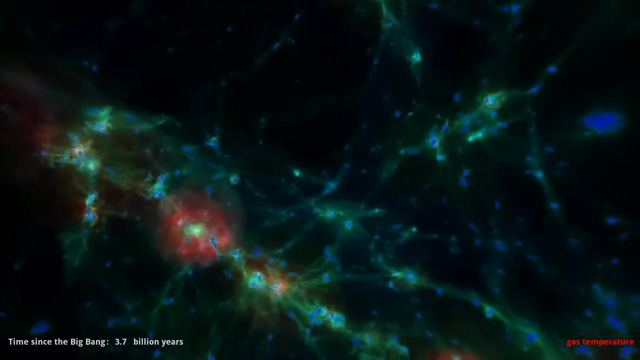 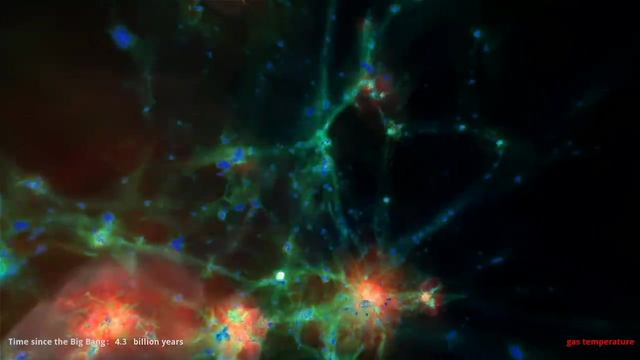 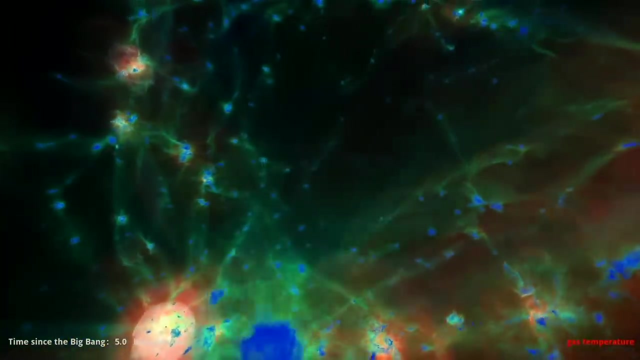 calvin- it was one of the famous, famous uh scientists of european the enlightenment age- thought that they basically just had a few small gaps in our scientific knowledge to fill in. this was way before quantum mechanics and the uv catastrophe and um relativity was even a thing. 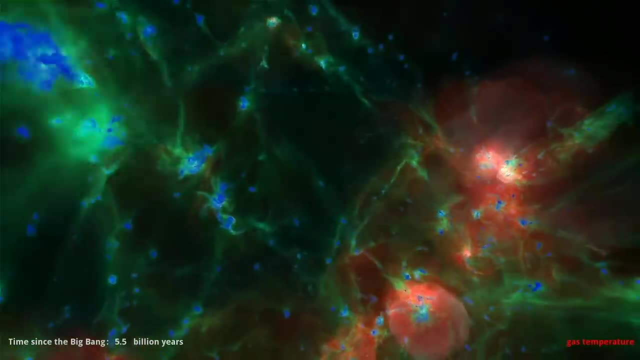 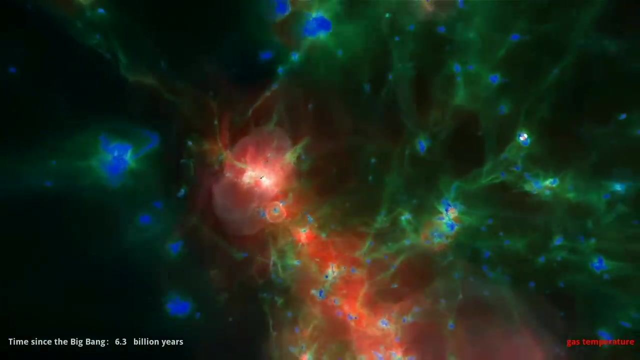 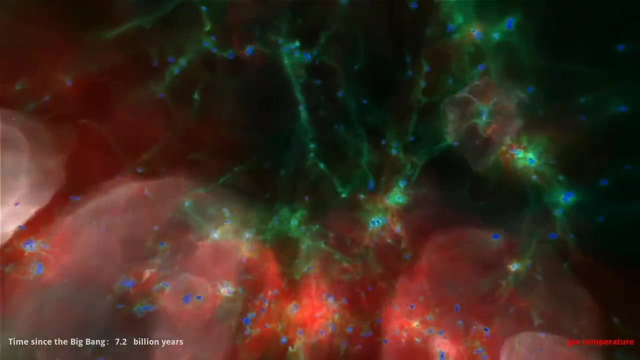 100, 100 or at least 50 years before, there's been an arrogance in science and just it's almost understandable because of how much we know and how well our mathematics describe the universe. I mean, think about that One of the Lagrange points, or sorry, Lagrange. whom the points are named after, famous French mathematician. he found out about those. He mathematically deduced those based on Newton's laws of gravity in the 1700s, And we weren't able to experimentally confirm them by literally putting satellites there or observing Trojan. 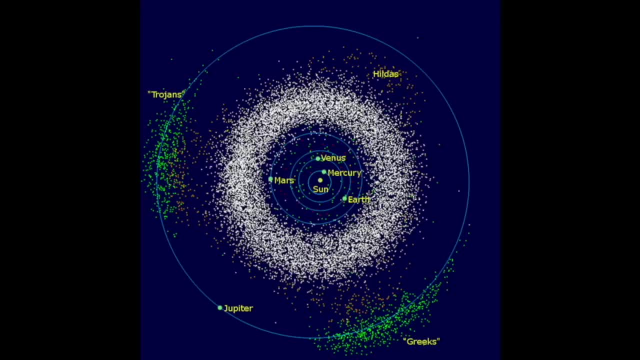 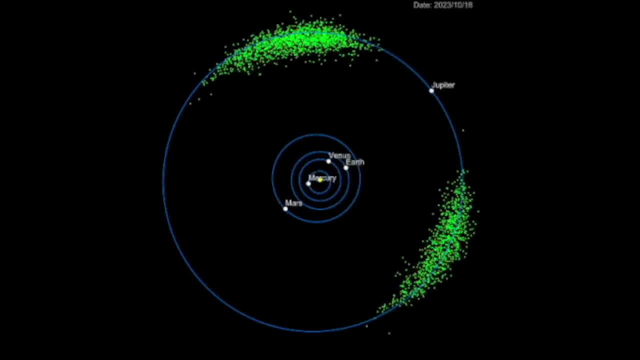 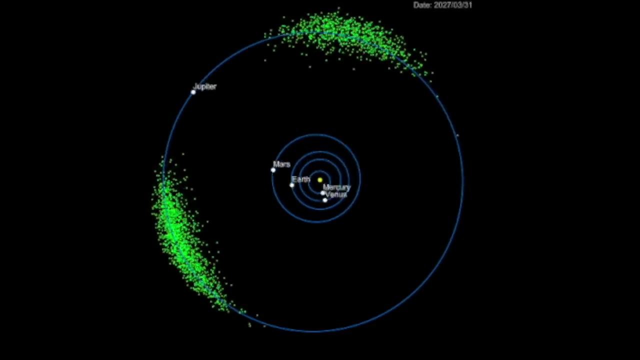 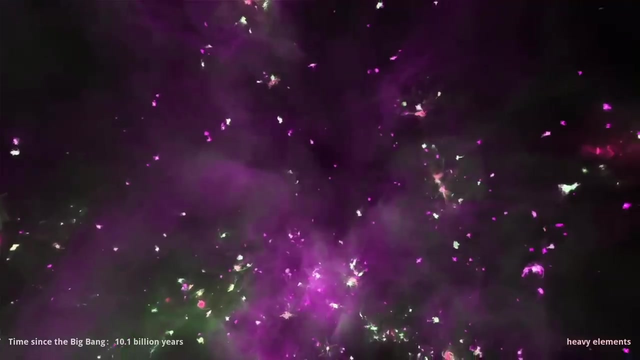 and were they Hellenic? I forget what the other one's called Groups of asteroids circling, orbiting with Jupiter, in front of and behind Jupiter, in its orbit. at those Lagrange points We weren't able to determine, test them out experimentally, And we literally are sending satellites there nowadays. And this 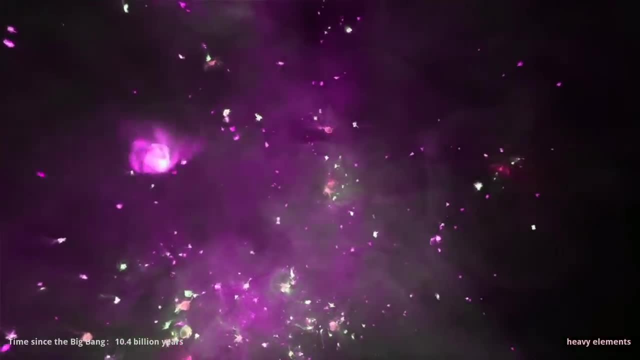 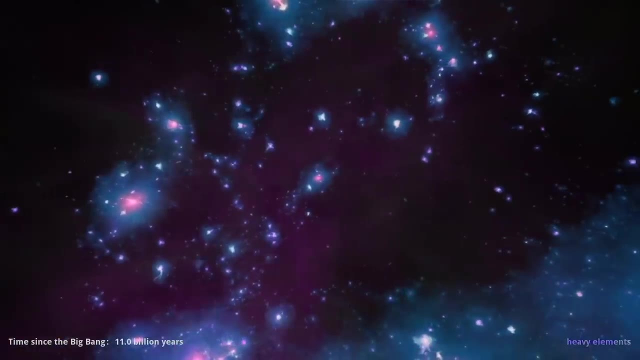 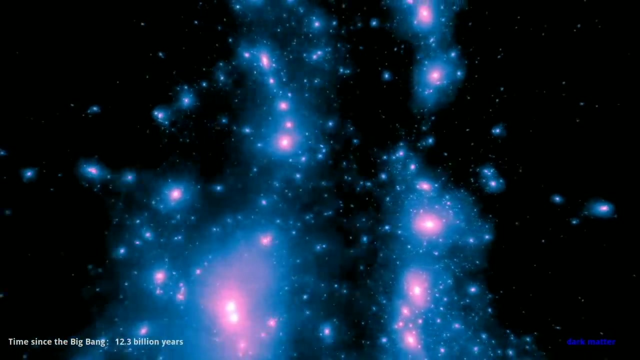 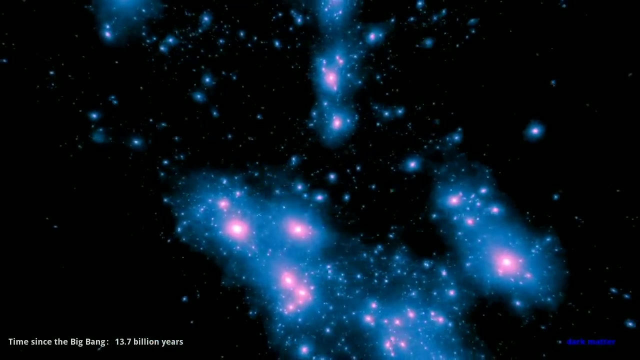 mathematics is so powerful And physical experiments are so revealing about the nature of the universe, We've had just numerous instances where we thought we were really pretty much done figuring it out, out the universe. and now here we have another, another instance of that almost being the case. 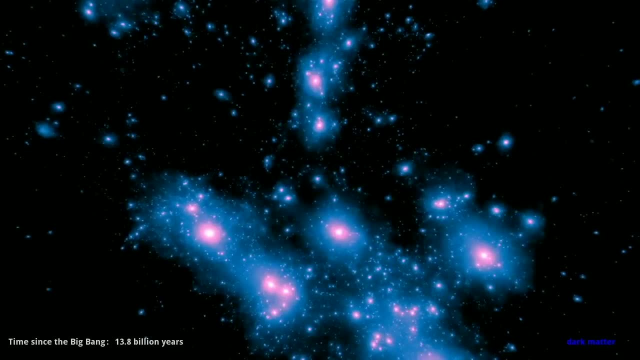 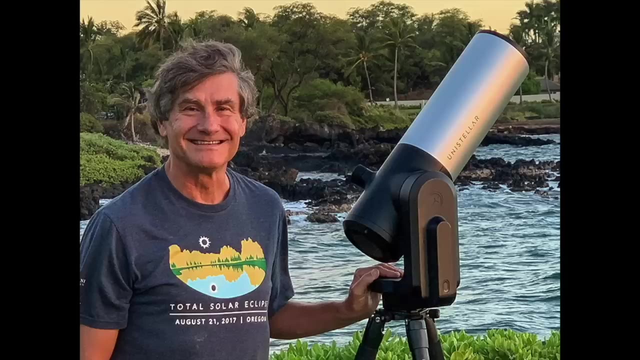 we just thought we had to kind of fine-tune some parameters about how the universe is probably slowing at the largest scales. and in 1998, alex filip filipenko- he's just such a, he seems like such a cool, easygoing guy, such a fun guy um him. and this guy, reese, adam reese, uh, who actually won. 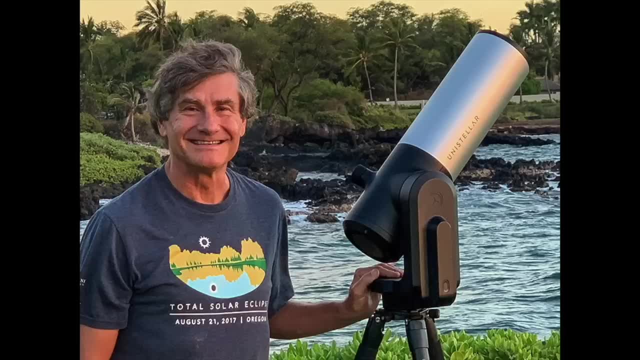 the nobel prize for this? filipenko, didn't? it turns out that him and lex friedman talked about that in the interview, but i guess there was a team of like dozens of people, so it's you know. filipenko was like: yeah, i get it. you know, i wasn't the third. you only get only three people get. 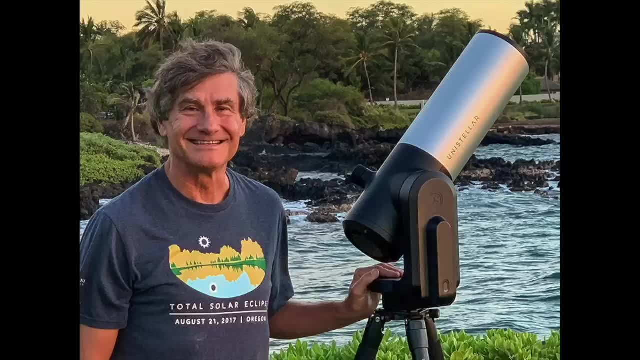 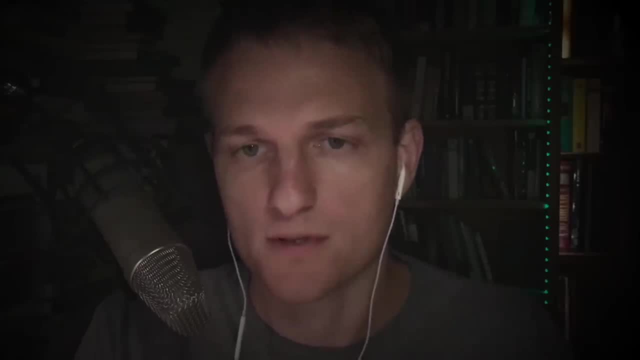 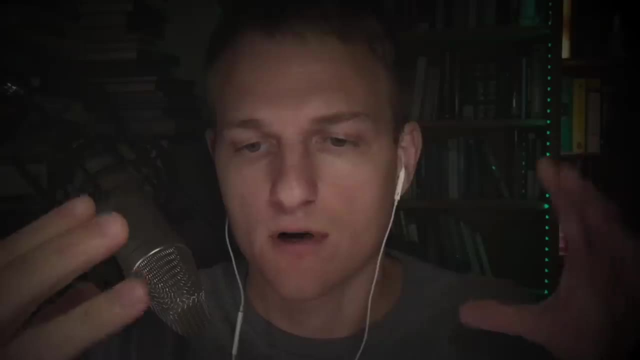 awarded for any specific discovery, a maximum of three, rather so filipenko wasn't in the top three of people being important for the discovery. but, um, you know, in the late 90s, as they were looking for evidence of cosmological deceleration, saying that, 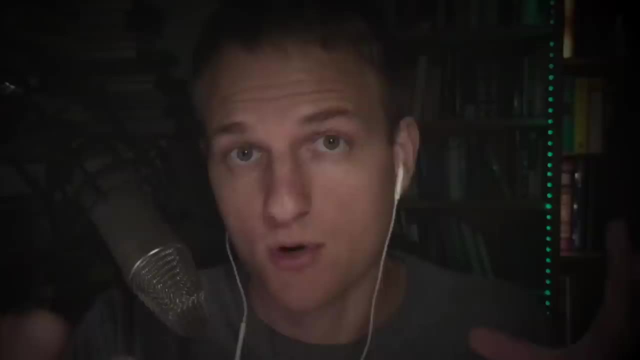 gravity from dark matter and matter- mostly dark matter- makes up, you know, 70 at the time, 30 dark matter or something like that should have ex. should have slowed the expansion. and as they're measuring the supernova, they noticed it was red shifted, not less, but about 15 percent more than they expected. and so this blew cosmology apart yet again. so the universe went from being just a couple thousand light years across to two million, to a few million, and the galaxies were expanding away to billions of light years across, but kind of at a constant expansion from an event that happened at the beginning of time. 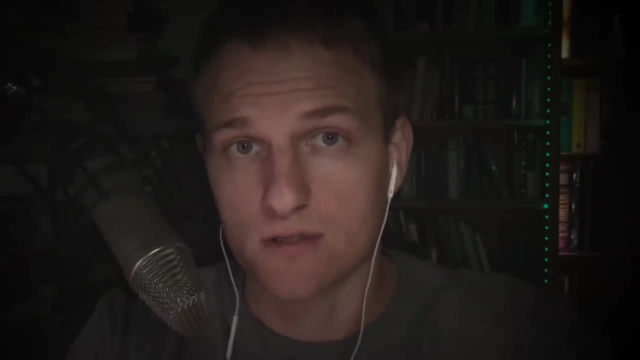 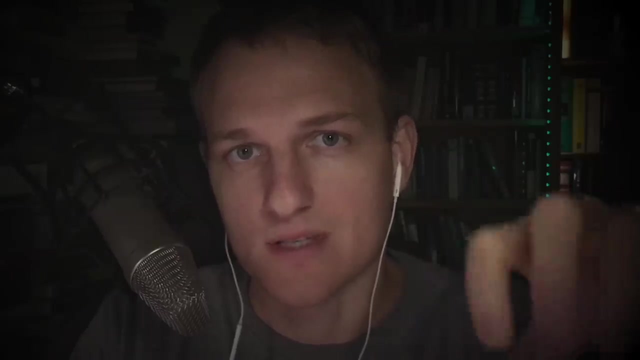 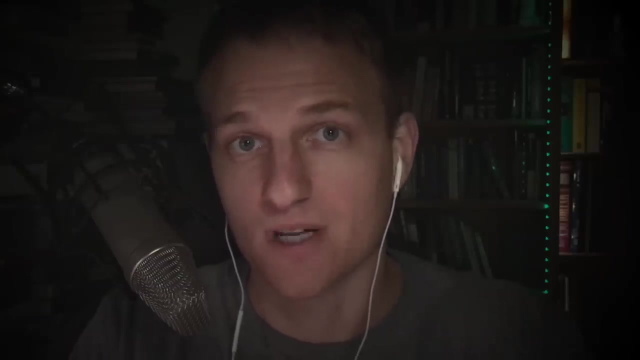 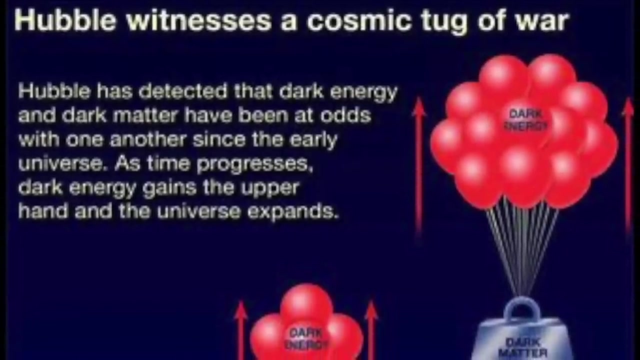 to now, an acceleration of expansion at the furthest, most extreme distances that indicated that there was an active element in the universe completely unknown and undetected before 1998, causing space-time to continue and even quicken in its expansion. This became dark energy. 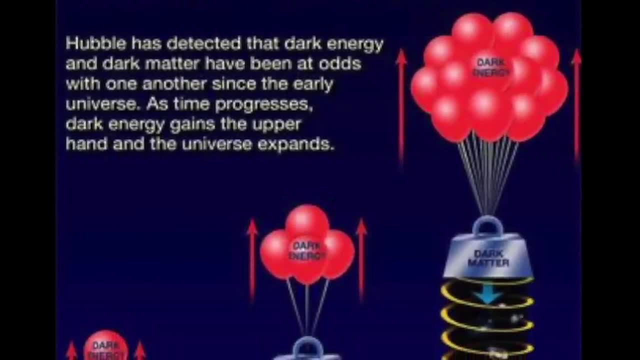 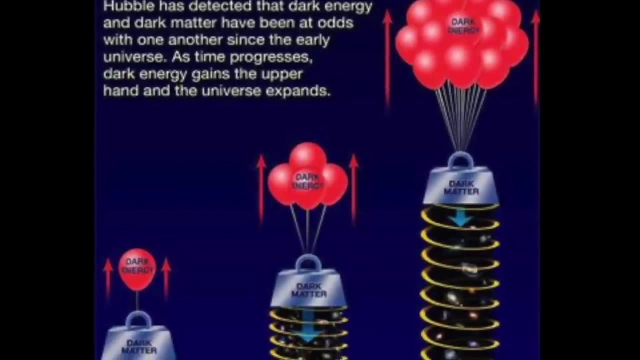 It was an acceleration of space-time. It's really fascinating. I'll have to do another video about just all the other stuff I'm skipping over here about how we know how we can use Type I supernovae, because there's different types. 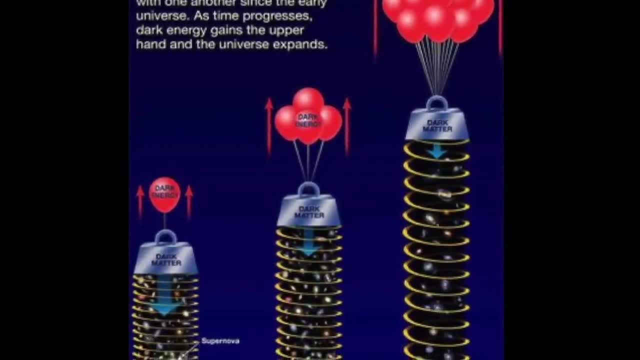 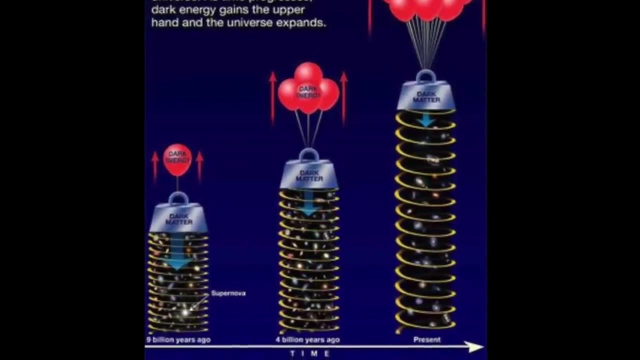 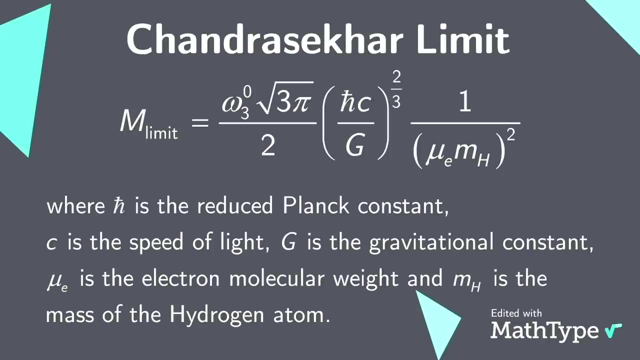 but there's one in particular that a famous Indian scientist, Shana, under SACAR, derived from quantum mechanics and atomic physics, actually about the way stars, about limits of the mass of certain stars before they can't handle their own pressure. 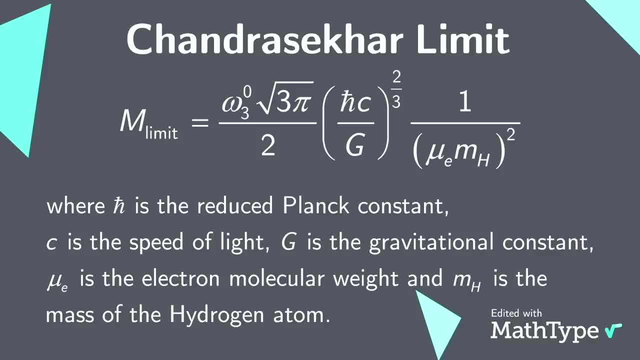 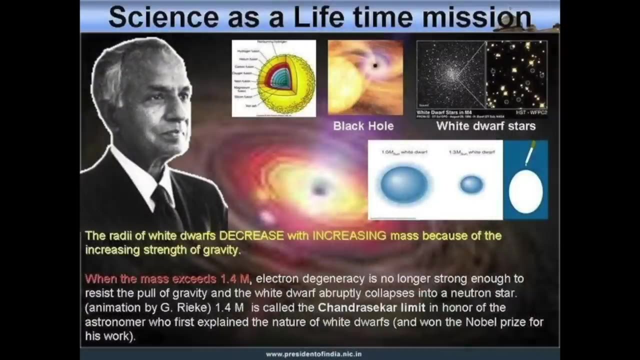 gravitational pressure and they explode. It tells scientists that a predictive amount of luminosity will be given, given off by stars that explode in this specific way, called Type Ia supernovae, Once they pass what is now called the Chandra-SACAR limit. 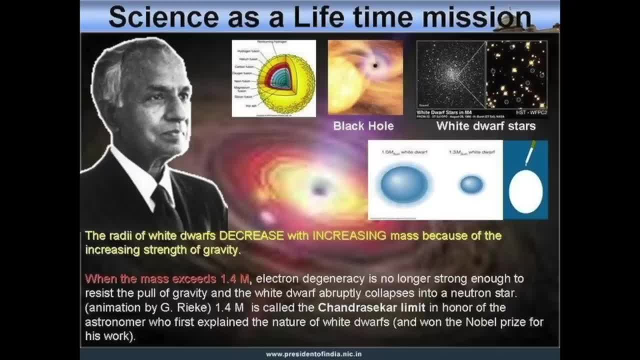 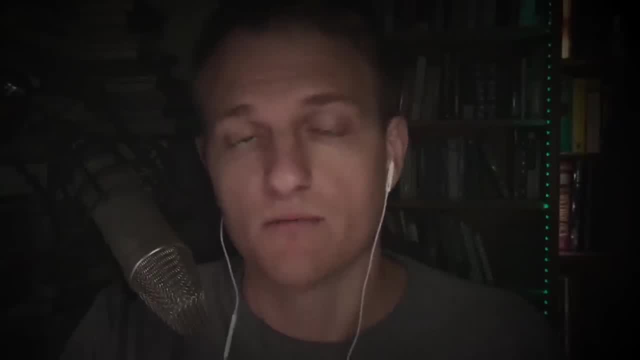 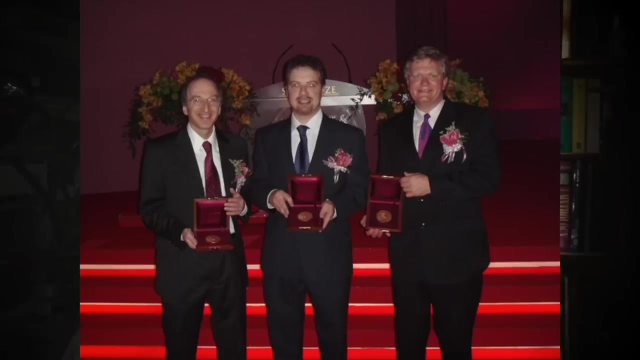 In 2003,. observations of the cosmic microwave background and the redshift intrinsic to it confirmed this expansion, this accelerated expansion, and then 2011,. a Nobel Prize was given to Adam Riess, Brian Schmidt and Sal Perlmutter. 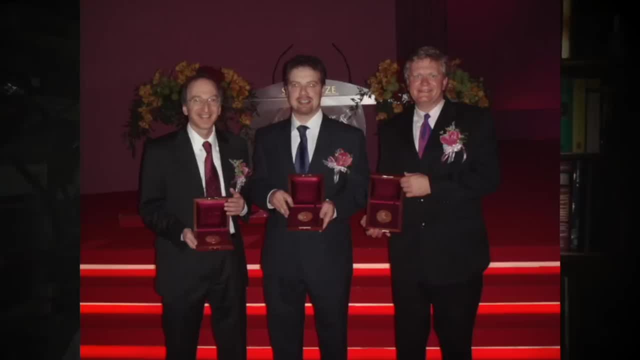 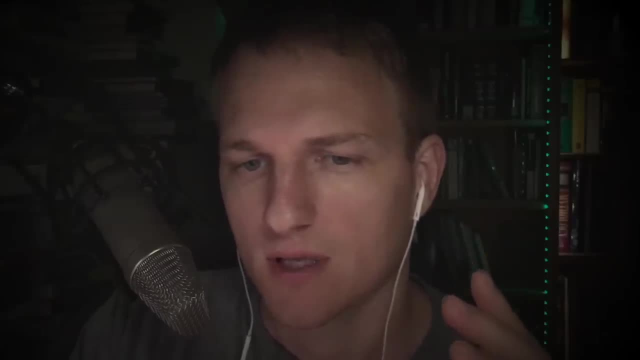 for the discovery of dark energy, But not only was- and I think the point I'm trying to reiterate over and over again by saying that I'm trying to find the motivation, the, the, the, the, a truly inspiring. 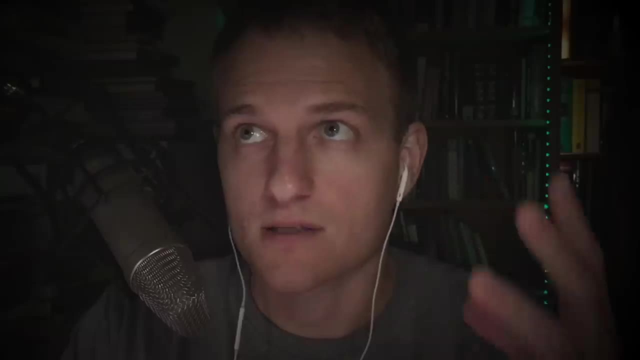 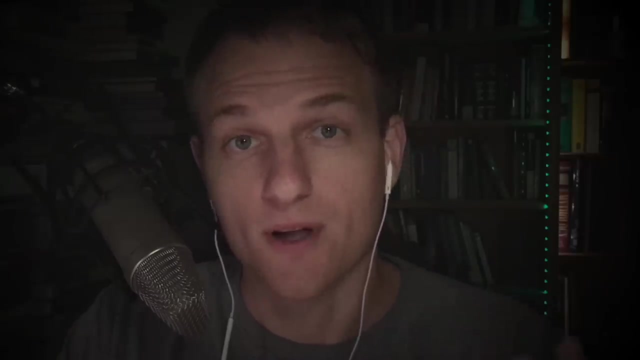 interesting, insightful the the fascinating and exciting aspect of James Webb I'm trying to convey. what I've found is that there's so much we do not know about the universe and our existence And there's so many more mysteries that keep opening up. 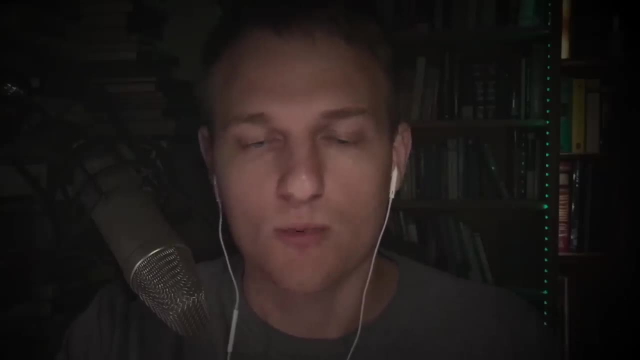 with new discoveries that James Webb will most certainly push further. So it's John Mather being the lead scientist for James Webb. He's been interviewed quite a bit and in multiple articles and interviews he's given he stated that even though there's all these expected things, 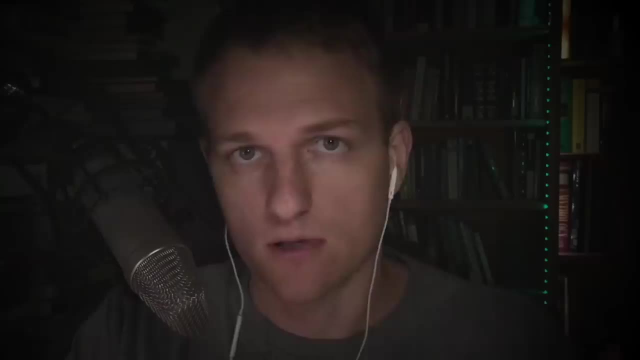 coming from James Webb, based on its abilities and technological advancement of its instruments. there's also the unknown aspect, which is why I opened this video with the quote by TH Huxley about the unknown. John Mather says it's not just what we know Webb can do. 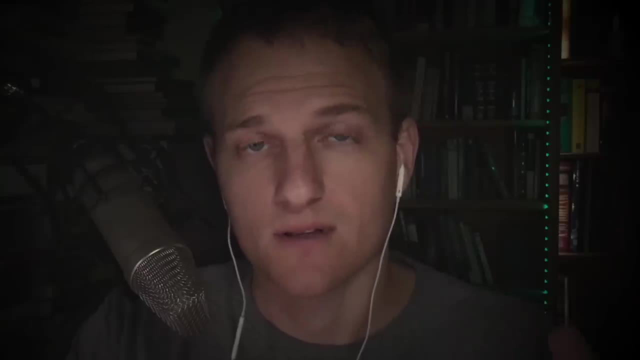 but it's the things that we haven't even yet thought to expect, that it will most undoubtedly, most undoubtedly discover, Just the way Webb or Hubble discovered: the universe was lit up at redshift six through its first deep field, And then a couple of years, just a couple of years later. 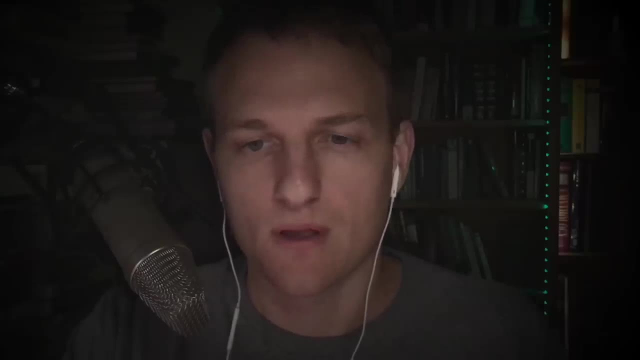 we're used to things you know sometimes happening, At least big breakthroughs not happening until you know- every 20 years, But it's like just three years after the first deep field we discovered that There's an energy in the universe intrinsic to space-time. 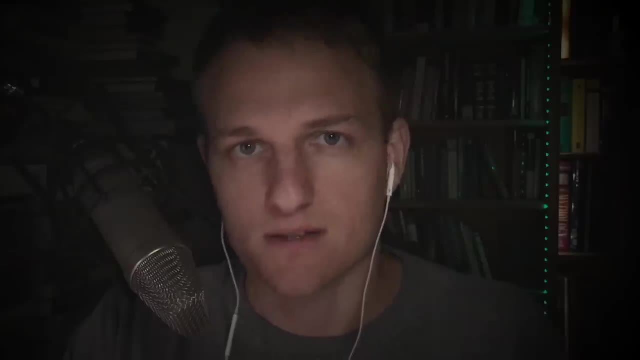 So something that physics essentially missed on Earth in our experiments in particle accelerators here, that makes up 70% of the entire energy of the universe and affects the way galaxies evolve, And so that wasn't expected. We thought well, well, you know these discoveries. 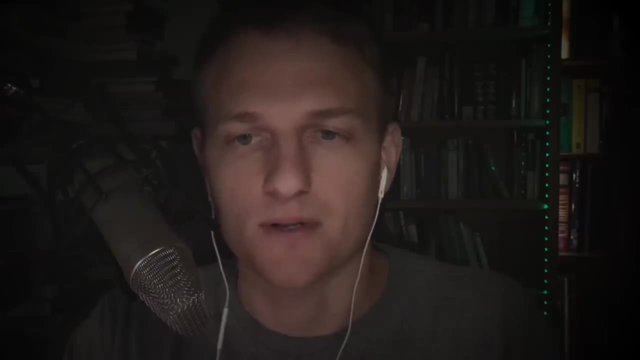 it was expected that we would find more about the universe out, but these were unexpected discoveries, And so it's natural now to expect Webb to make some observations that are going to really challenge, And that's why they built it in, actually, to a lot of the reports. 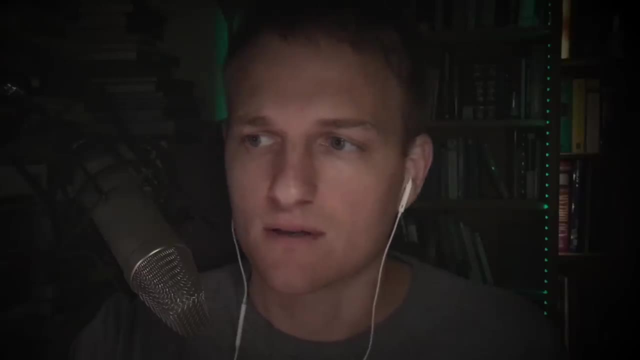 Webb is. let's see, I have a. one of Webb's primary goals is to either verify or challenge the current benchmark model for the age of the universe, the lambda-gold-dark-matter-big-bane theory. This is so we measure. Z the redshift. 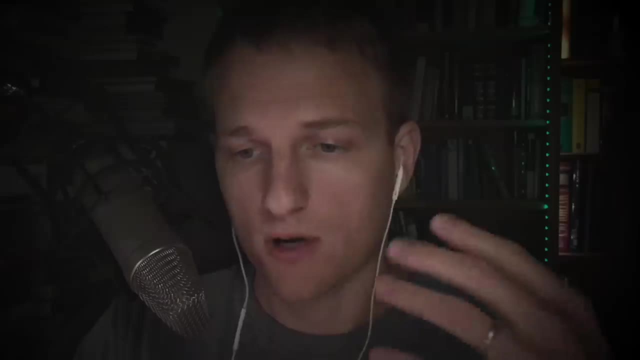 but it's depending on what model of the universe, what mathematical equations and parameters, what values of the variables we put in those parameters are that tell us how to interpret the redshift into distance and time, and also, more often, more esoteric things like the curvature of space-time. 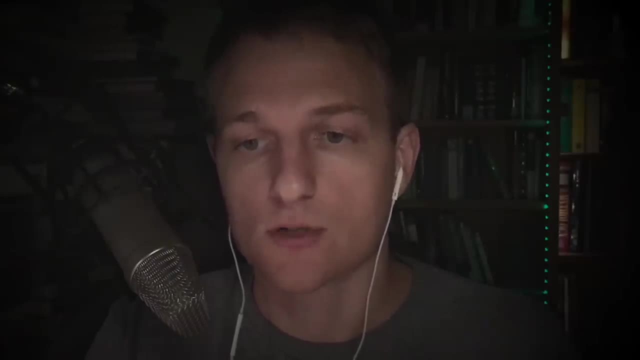 that we mentioned a little bit earlier. So we're all of these things are expected to either be: either confirm the current model, which is 70% dark energy, you know, 30% dark matter, roughly 25%, 5% regular matter. 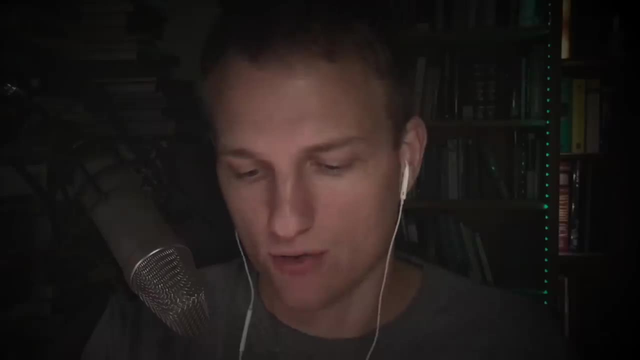 But now we're getting wiser, we're in our old age And a lot of people are outwardly saying, yeah, maybe Webb's goal isn't to confirm it, but actually rattle it up and, you know, shake the foundations. 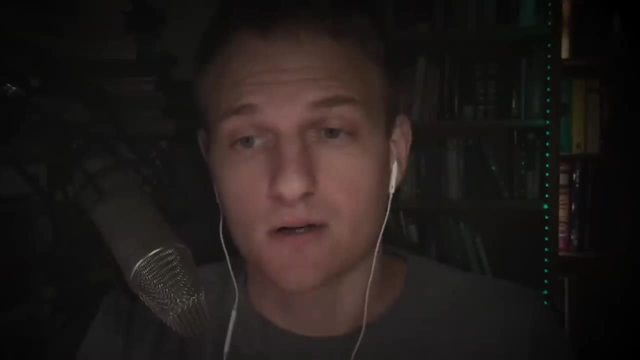 of our current cosmological model and cause make a need for a new physics. even So, it's really, it's really exciting To hear that happen. And so, just 20 years ago, we had a new, completely unexpected aspect of the universe. 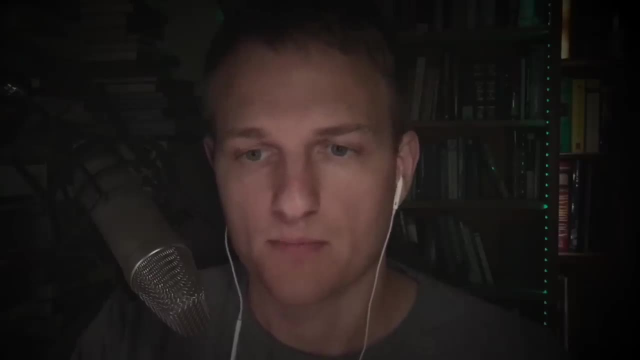 called dark energy come into play. And what's even crazier is that, like I said, cosmology and physics have been going hand in hand, trying to reinforce each other's theories And, if one, if there's huge discrepancies, like between gravity and quantum mechanics. 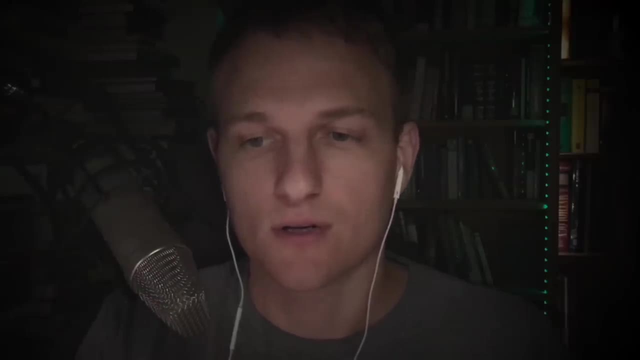 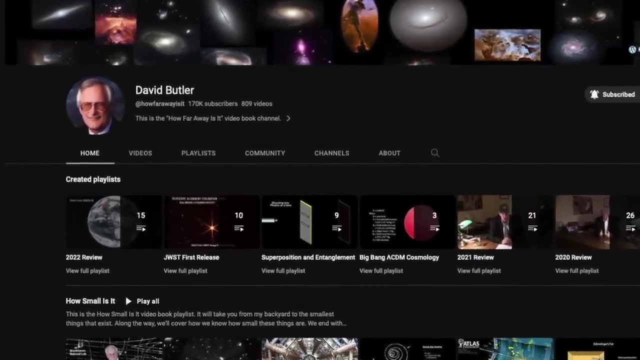 that's clearly an area we have to reconcile, And one thing about dark energy is that- and David Butler goes into it and explains why- we have a fairly good grasp of maybe the origin of dark energy, And it's. it's essentially that. 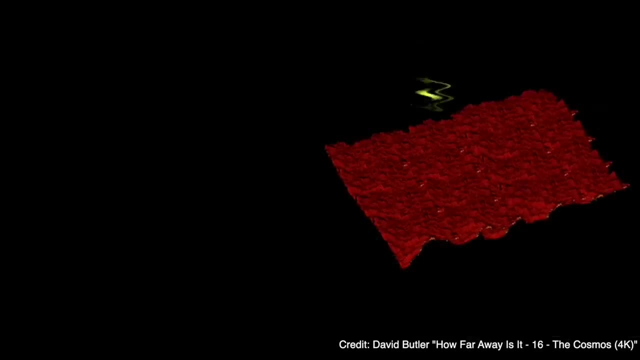 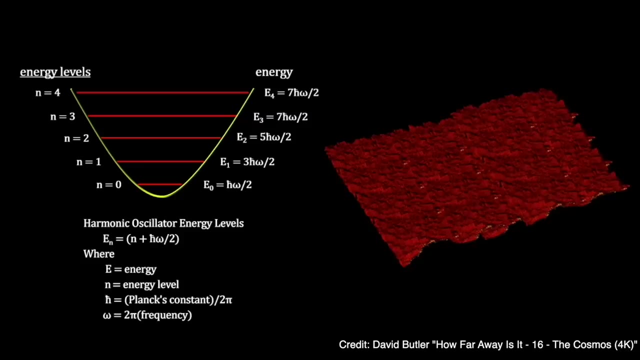 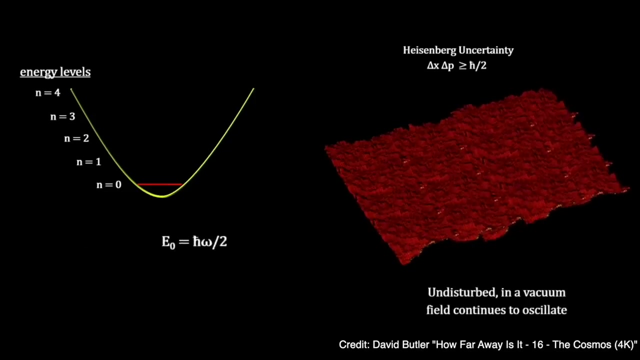 that that there. it's, essentially that the, the nature of space itself, at the smallest scales, has these forces, these quantum mechanical field energies and other energies too, always bubbling around and bubbling in and interacting with each other at different nodes. 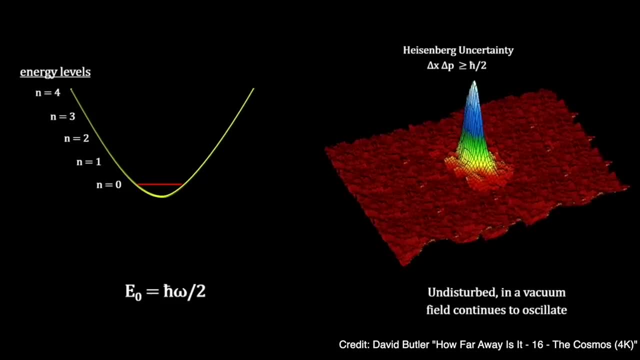 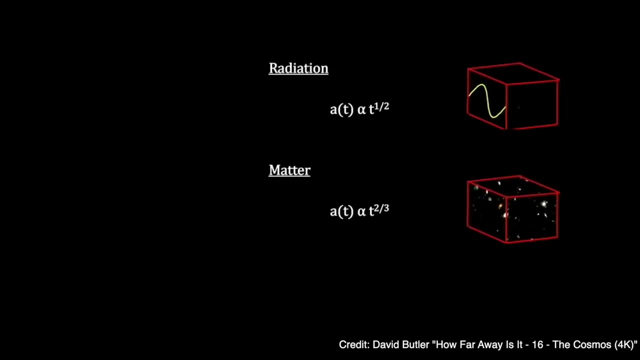 And occasionally they'll, they'll create a spike in energy, And this as the universe has expanded and as the universe has expanded and as the universe has expanded and as the universe has expanded, from residual inflationary expansion, the momentum left over from that. 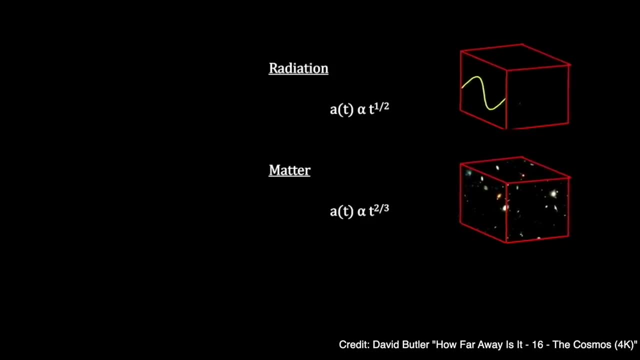 for about 10 billion years expansion happened pretty consistently, But at around the 10 billion year old mark the universe became, became expanded enough, or enough extra space was added to it that these energies, these vacuum energies and the quantum field fluctuations 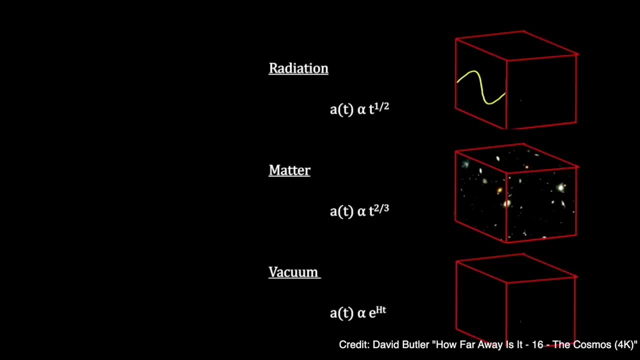 they began adding up over billions and billions of light years. you know 40,, 50,, 60 billion light years. At that point they added up to start accelerating the expansion that was already happening. And he actually goes into. I'll recommend that to. 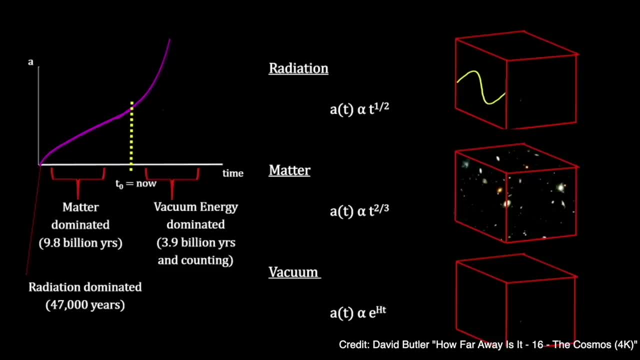 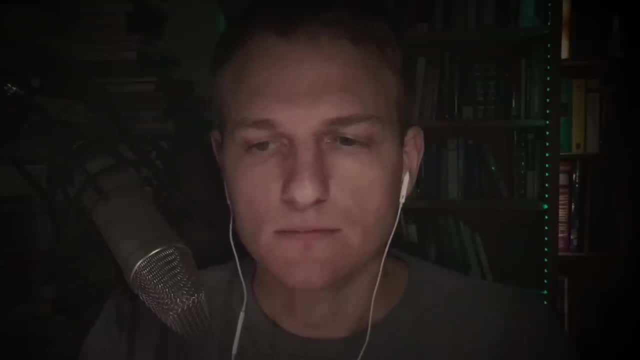 you know the actual equations behind it. So it's not just speculation. It's pretty, you know it's mathematically tight. but one thing: so they think they have a general idea of it and they have mathematics to back it up. 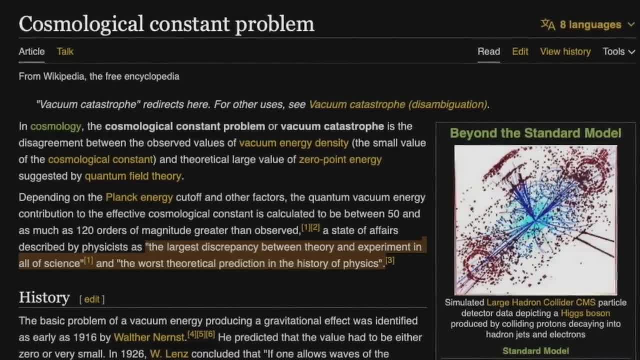 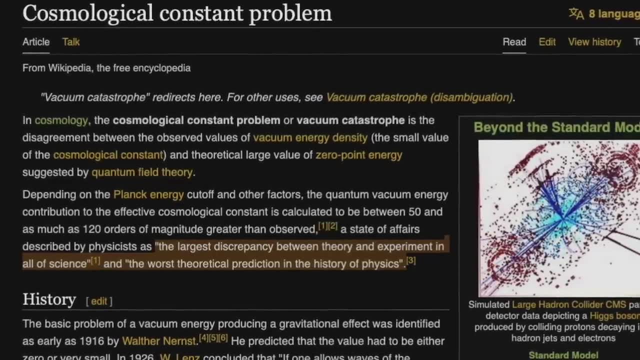 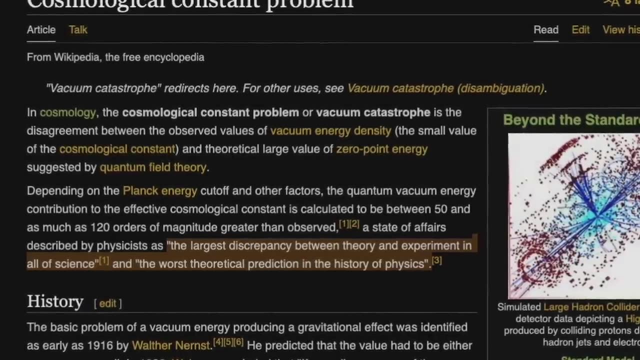 except they're off by a scale of 120.. No, no, sorry, It's a little bit of a difference here. Off by a scale of 10 to the power of 120. So there's a huge discrepancy, Quantum mechanics tells us. 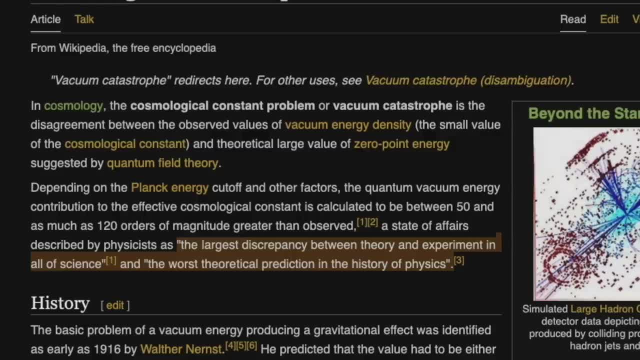 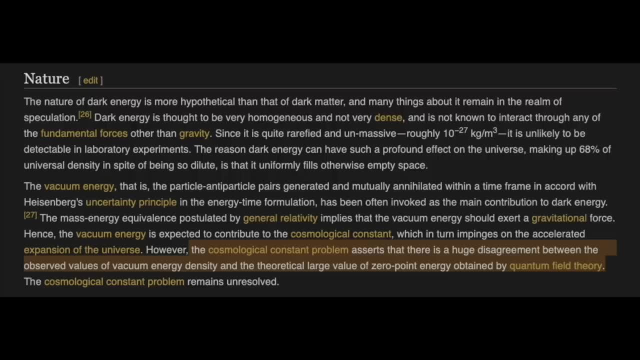 that the source of this vacuum energy might be tiny elementary particles that flicker in and out of existence everywhere throughout the universe, And various attempts have been made to calculate just how big the effects of this vacuum energy should be. But so far the order of magnitude of theoretical estimates. 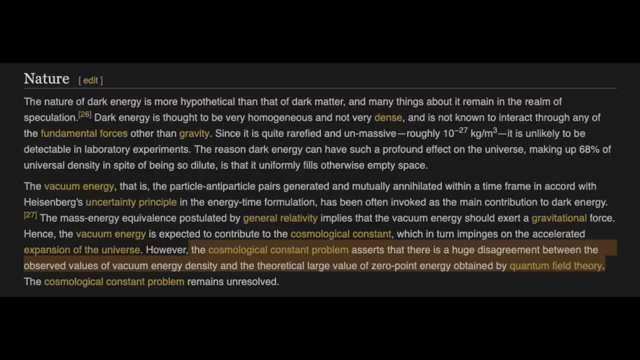 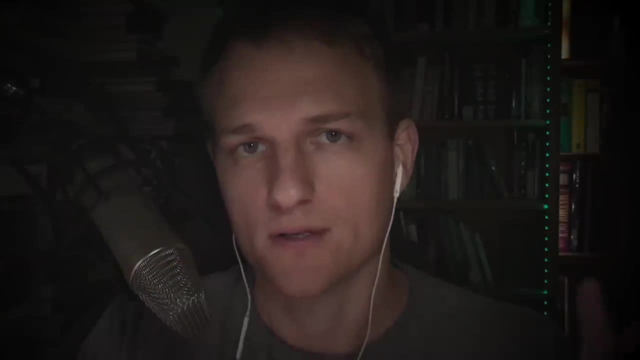 and the value required to account for the acceleration observed by the supernova. measurements are off by 10 to the power of 120. So although there's compelling evidence that dark energy exists, we have no idea of the source of such a large magnitude of it. 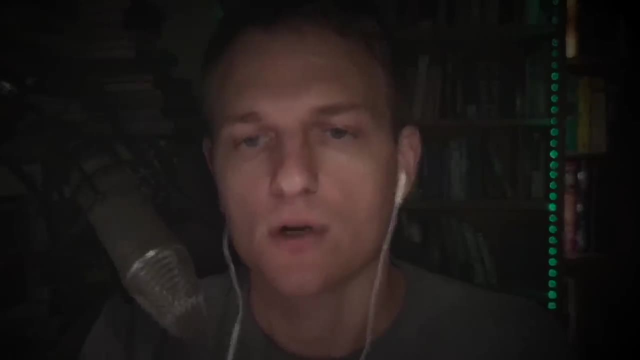 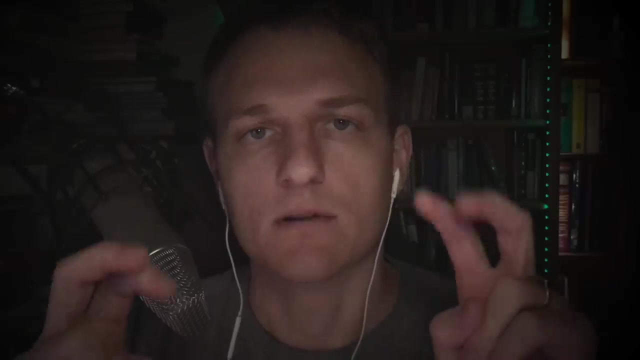 Yeah, Another fact I learned from David Butler's video: dark energy's density is very low. It's much less than the density of ordinary matter and dark matter. But an example is it's negative gravity, of course, because it's an outward repulsive force counteracting 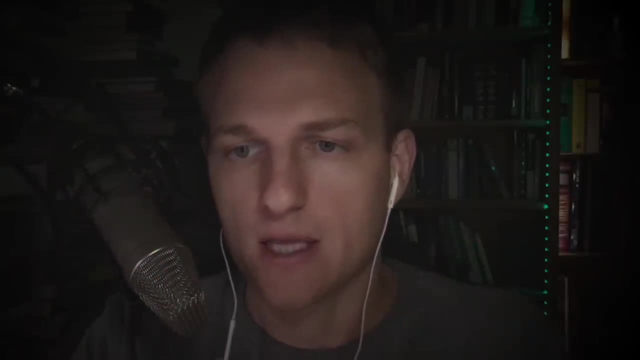 the attraction of gravity. It can't be observed on human scales. We can't observe it. We're only observing the effects on cosmological scales, of course, of 40 billion light years and 14 billion years. All that empty space in there is the compounded effect. 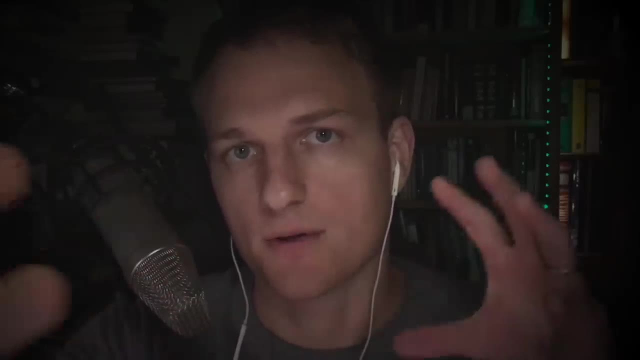 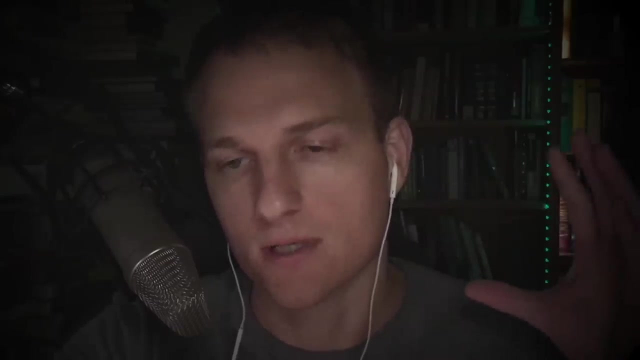 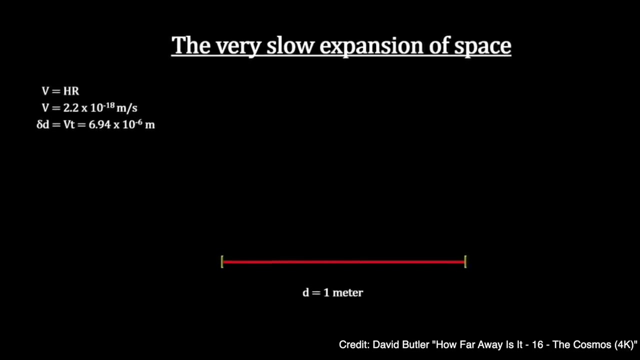 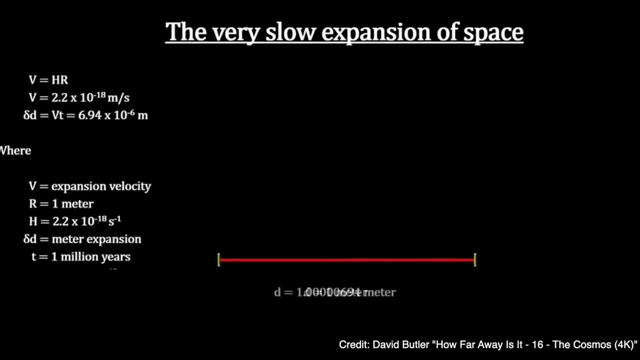 The accelerated expansion is the compounded effect of this energy taking effect over 40 billion- 93 billion light years of empty space. So this negative gravity can't be observed on our scales because it would take a million years for a meter three feet to expand just seven millionths of a meter. 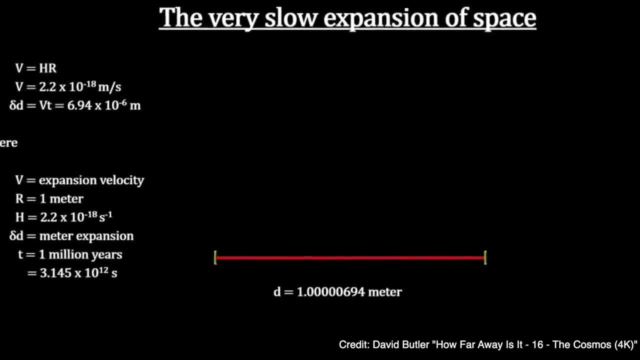 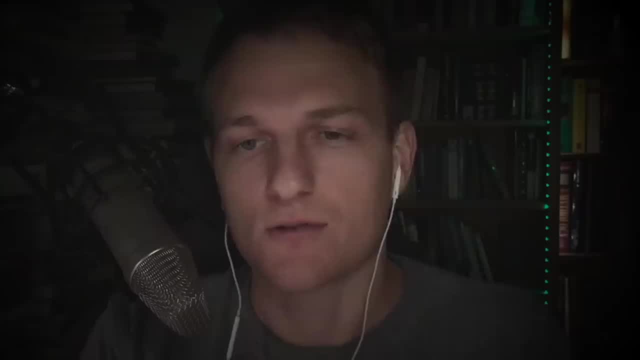 So it would take a million years to expand just seven millionths of a meter for a meter to expand by that much more So of course that's not even measurable on anything even approximating what our current technology and our current human lifetimes exist within. 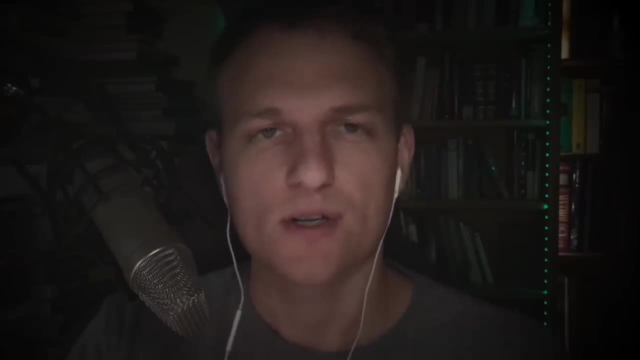 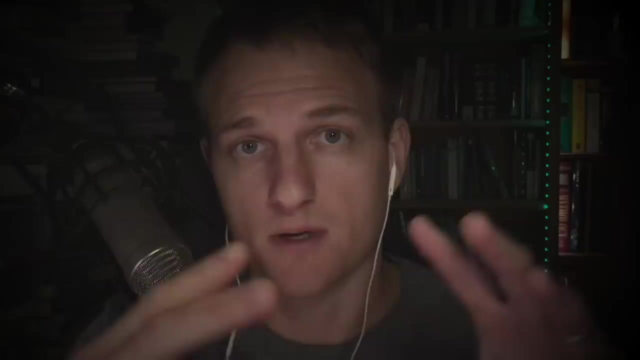 But it's a cool historical note that dark energy proved Lemaître right because he did have on top of the theory, the Big Bang theory that the universe might have actually been. if it is expanding, it might actually have been come from a single point out of which it expanded. 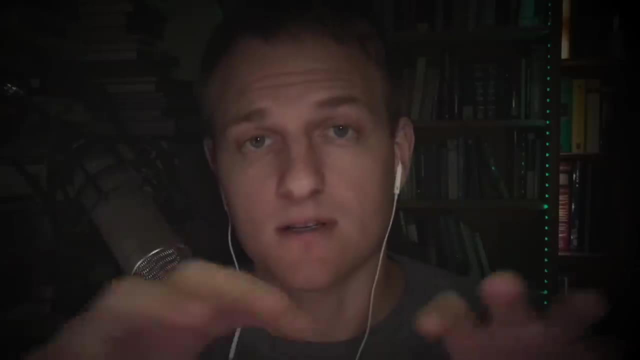 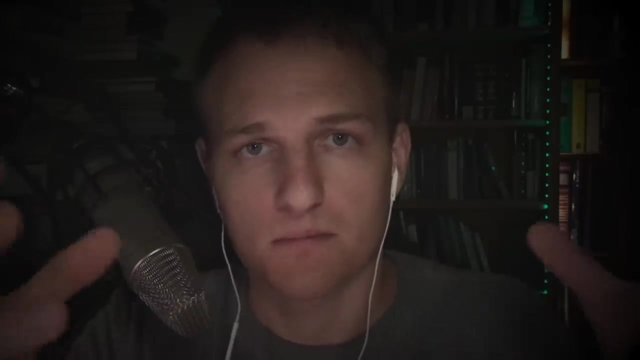 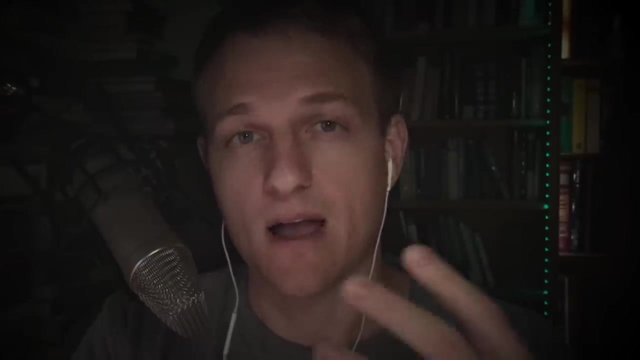 He also- separately- or not separately, but as a completely equal, equally amazing feat of contemplation and theoretical work- he predicted that the universe was actually accelerating, or at least that he outlined equations that predicted that. Whether or not he actually believed that, that was a different story. 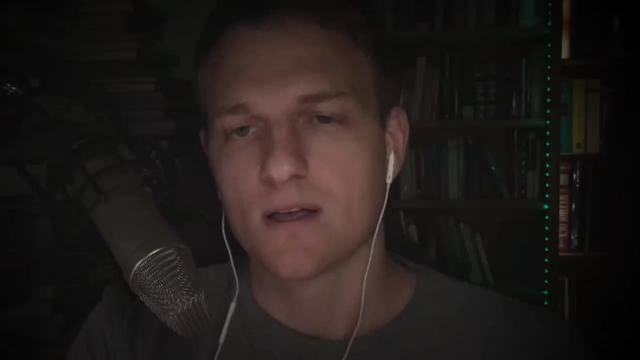 because apparently he didn't. He was like Hubble and didn't really believe that that was a tangible fact, so much as just a way to interpret the data. One extra little note I'll add about dark energy is that Alex Filippenko was. 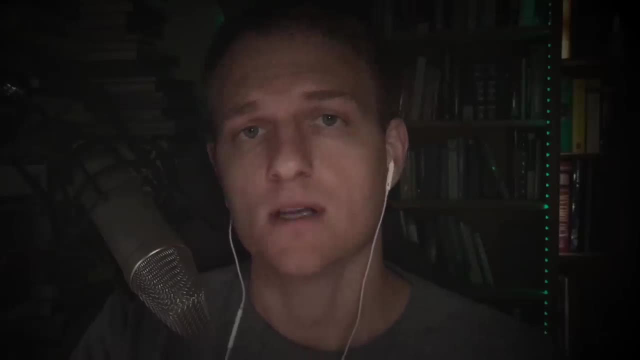 again in the Lex Friedman interview he actually said that maybe, given that the inflaton field that caused inflation and then rapidly just dissipated and actually interacted with reality, to actually be some sort of causation of matter and other particles after that fact, 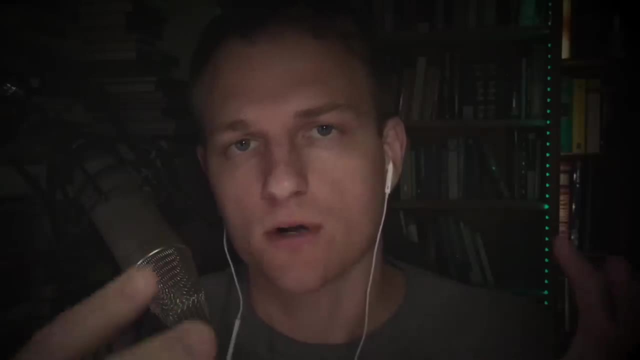 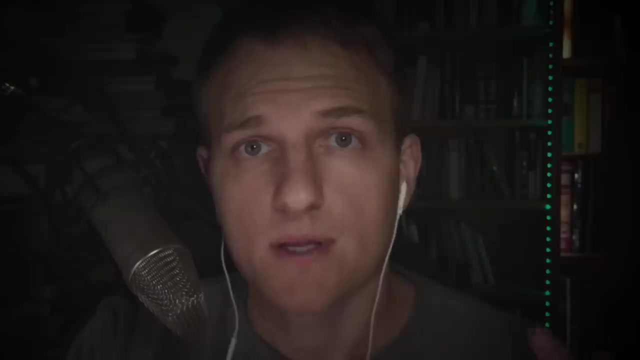 maybe possibly after. What dark energy implies is that after long enough time scales, there are other fields, other things, or maybe the inflation, the inflaton came, is coming back into existence. So in other words, he's saying he doesn't know what it is. 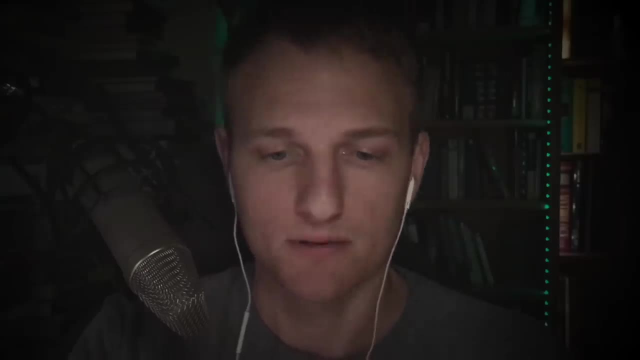 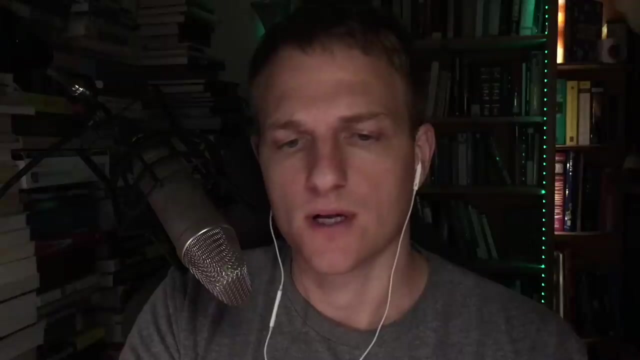 but that there may be a connection between inflation and the current acceleration that dark energy is causing. So that's the one thing I wanted to say about dark energy. Thank you very much, And it's probably one of the main goals of James Webb. 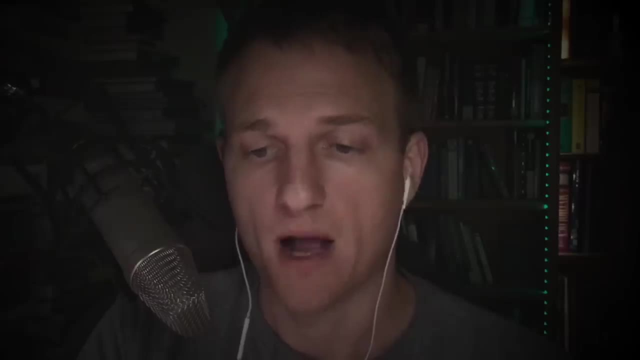 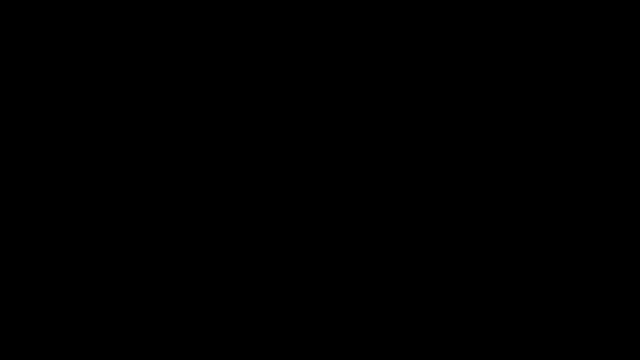 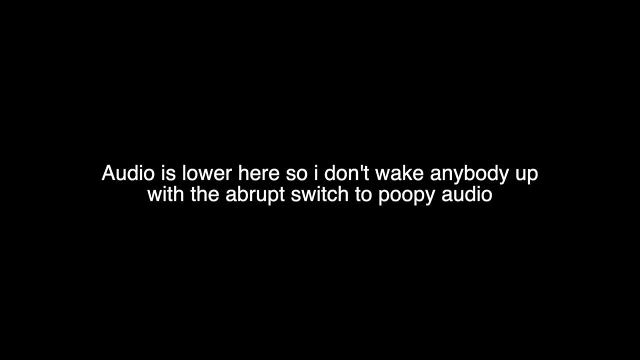 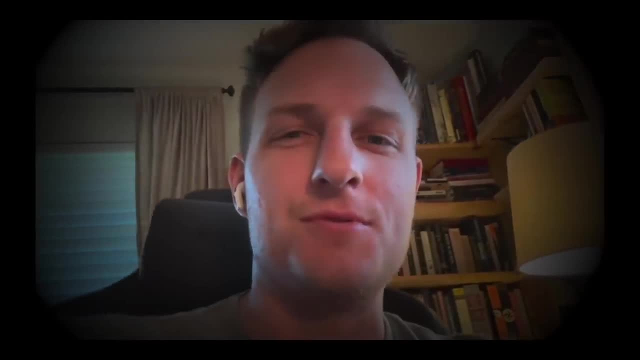 The Planck Telescope. if you made it this far um, I guess. oh, if I haven't put it in the description, I'll clue you guys into uh material I didn't use for the James Webb Space Telescope video. I had written this. 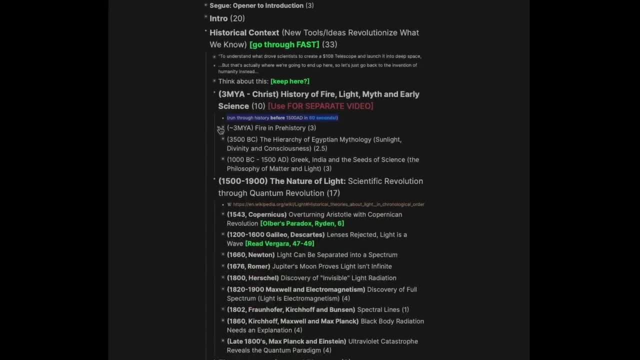 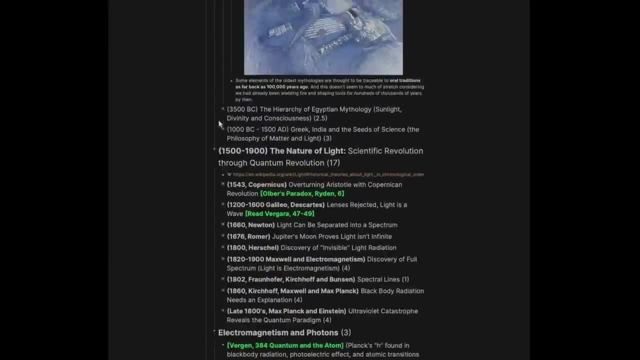 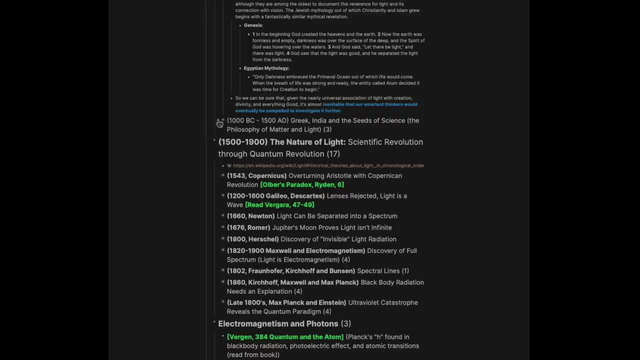 huge. well, I'd written this and a couple other real big um background kind of contexts that the Webb Telescope sits within and historically there's a whole nother one where it's it's. I'll probably have to redo it because it's just I don't think I did a very good job on it, but 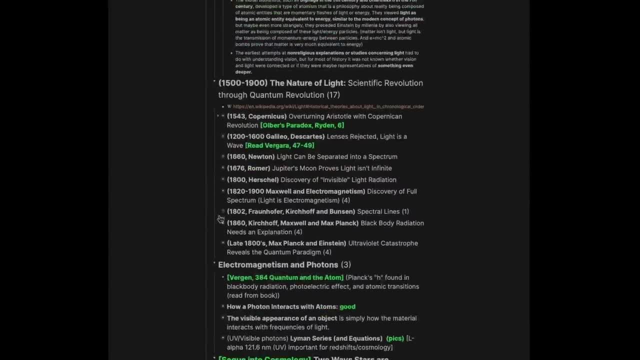 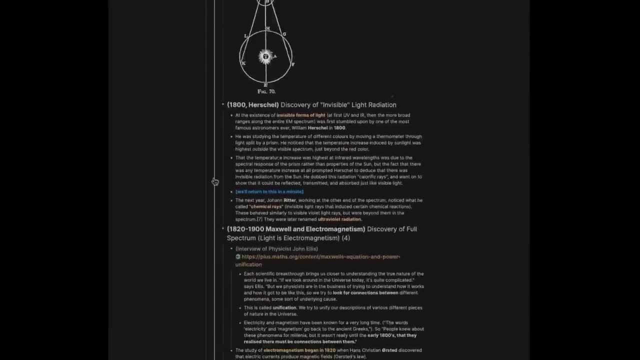 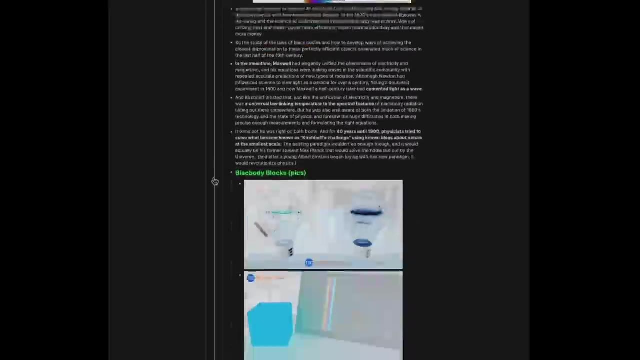 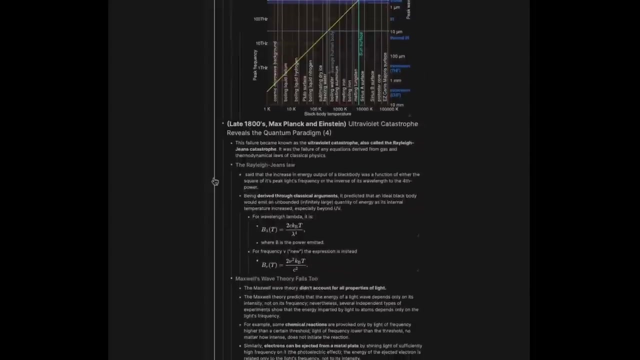 uh, this was kind of the science, the cosmology background and context of Webb and its purpose for existing being made, and the other one was a historical, um kind of a context of the, the, the, the concept of light in ancient history and how you know our origins in fire. I kind of. 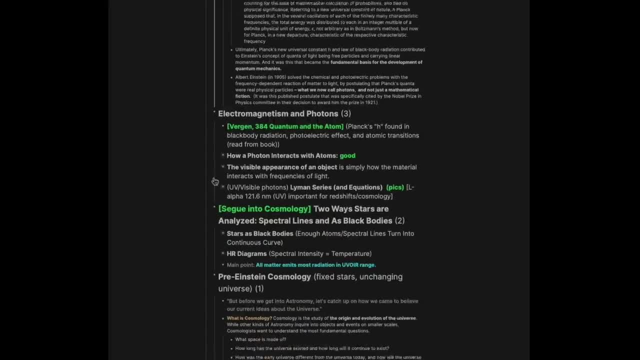 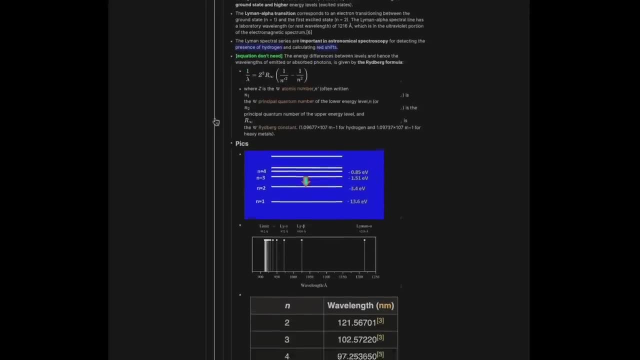 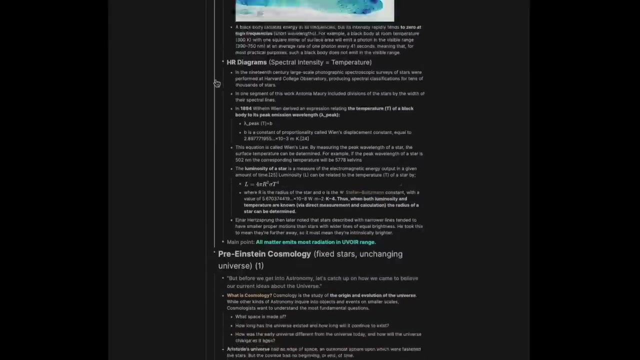 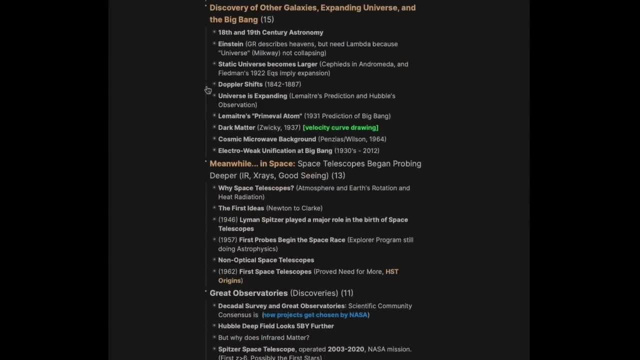 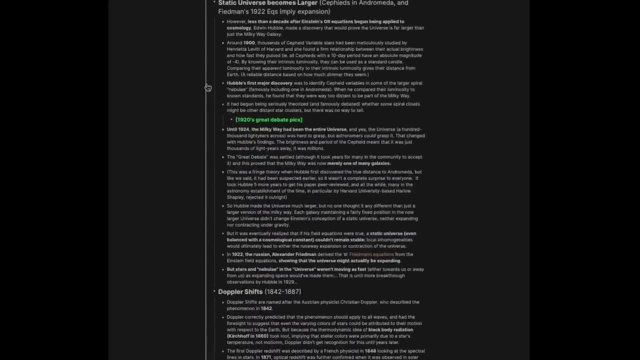 it wasn't anything, uh, extremely illuminating, I guess you might say, uh, in regards to mythology. so it's, I don't think it's really worth putting out, but I'll definitely touch upon it and maybe if I could do some more research and flush it out some more, um it uh. 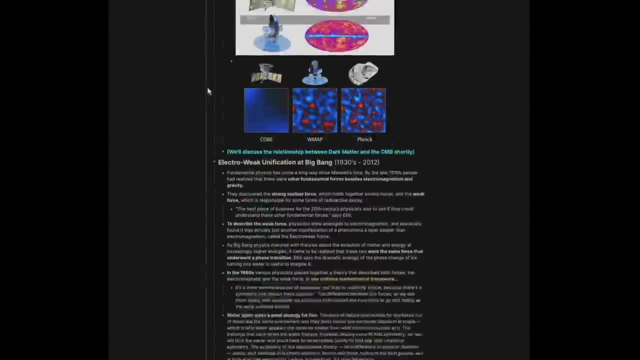 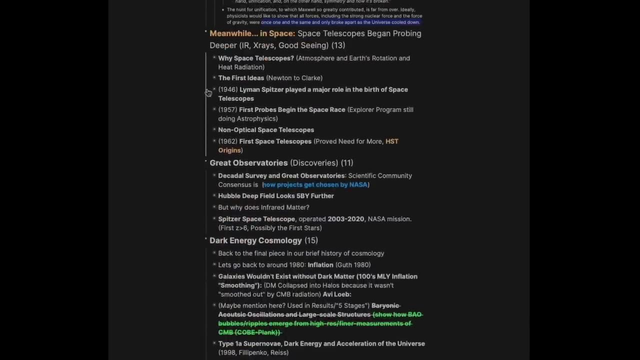 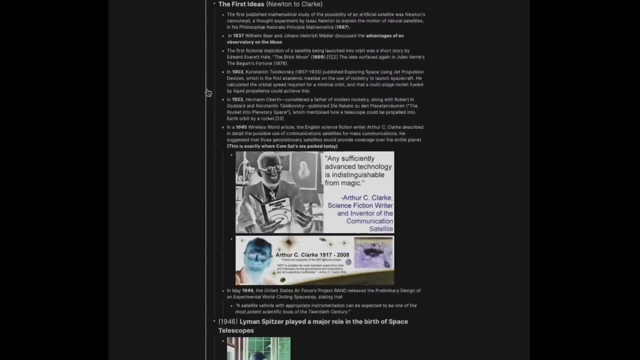 it was very cool and, and Webb, I think I have a. I might have ADHD or something, but um, as I was learning about Webb, I wanted to understand its background and the physics in astronomy, and then I got into the history of astronomy, which led me into the history. 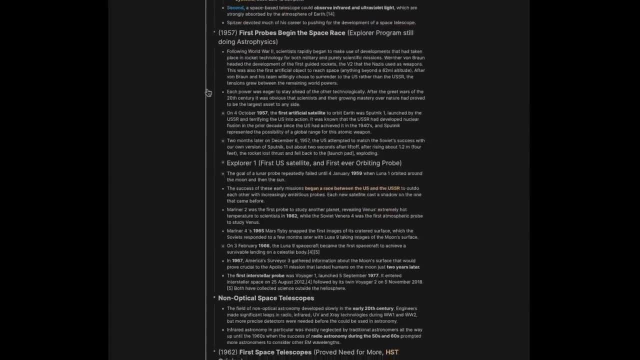 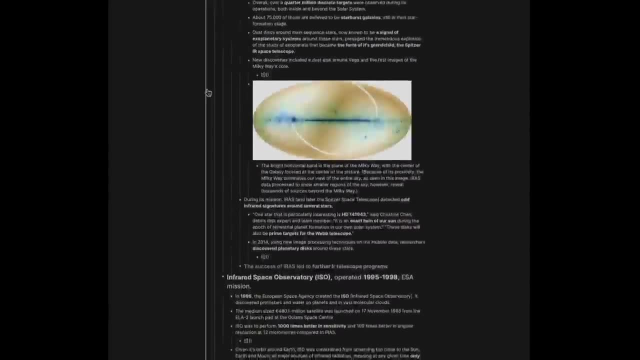 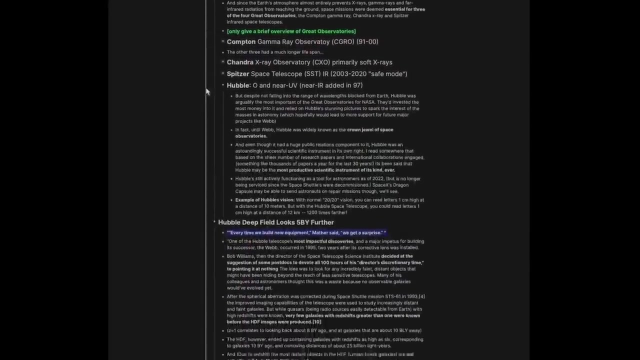 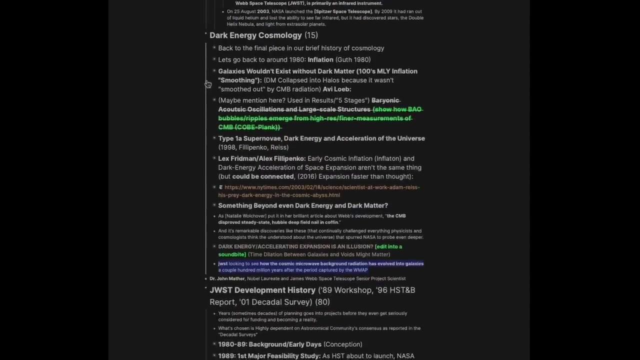 of you know, astronomy is just goes so far back in human history, so that was a subject I started kind of dabbling in and anyways it was fun. but there was a lot in my final script that I wrote and this is part of that fruit, I guess, of the script that didn't. 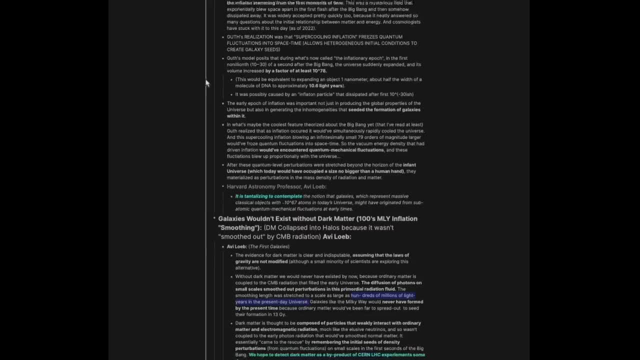 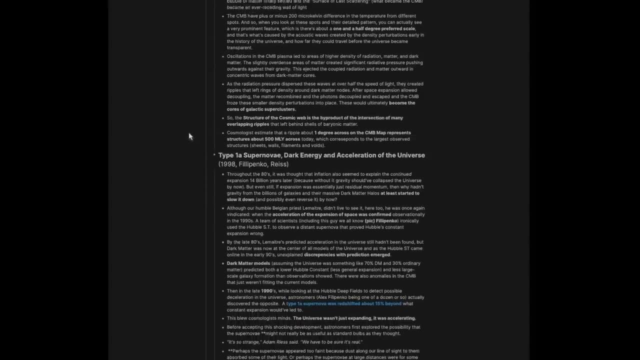 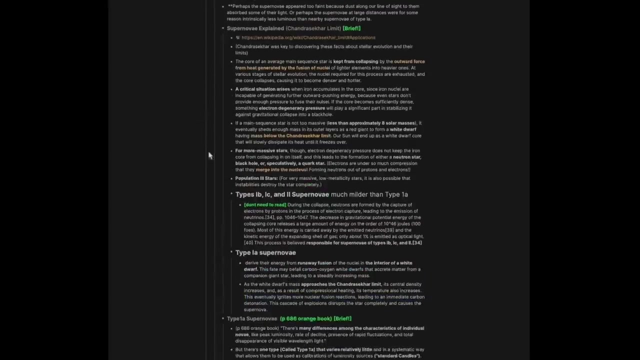 quite make it into the web, so I hope, if you guys liked this, I would love to do some more kind of histories and broad overviews of astronomy and science. there's a whole other hour-long segment that I about electromagnetism and its separate specific development. 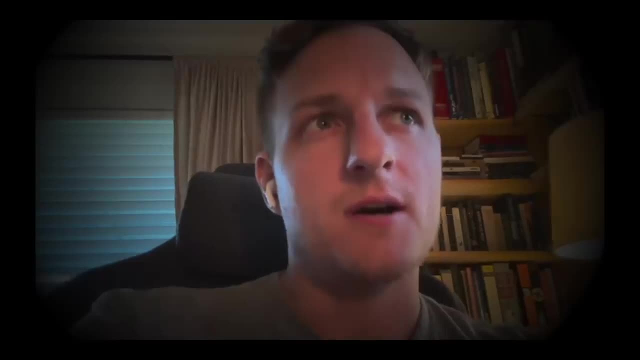 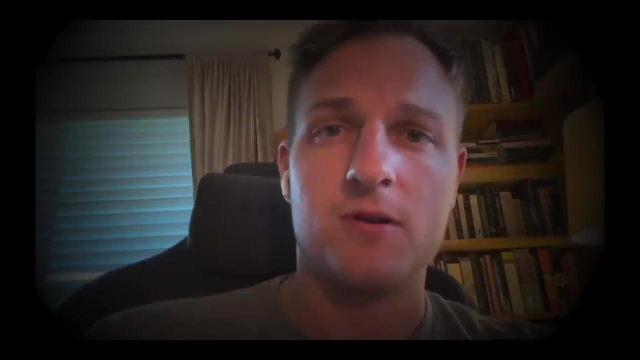 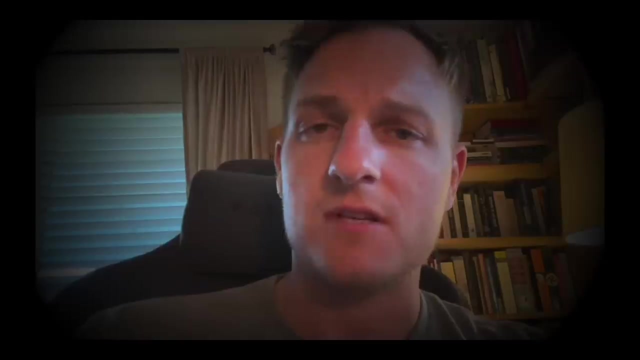 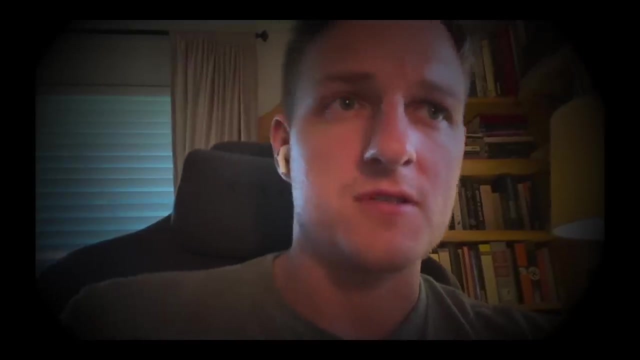 apart from cosmology, just yeah, the train of thought from around Descartes. a little bit after him, Newton came along on the scene and he became the chief reason why his investigations into light, became the chief reason that, for 200 years after him, all physicists, most physicists, 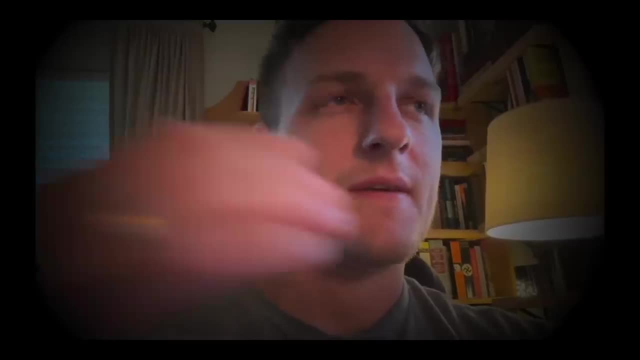 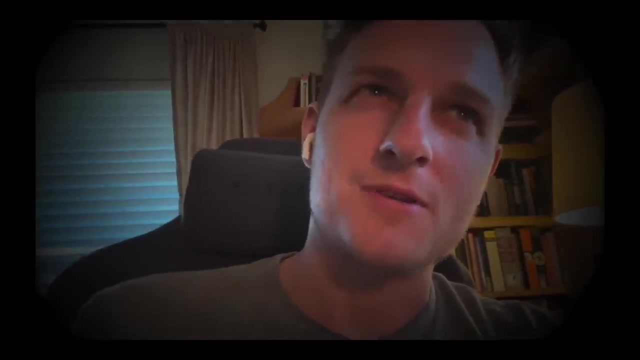 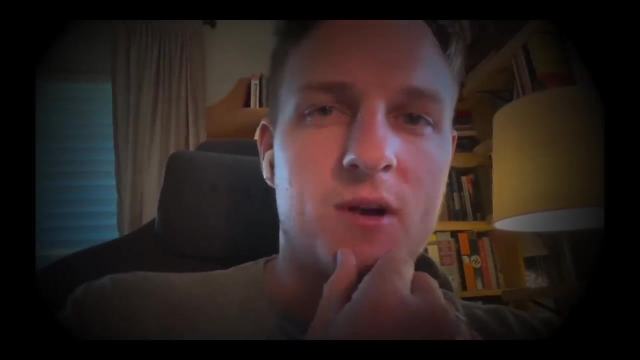 thought that light was particulate. How was it The other way around? it needs to be a separate video regardless. Newton thought it was. I think Newton thought it was corpuscular. he thought it was particles. so everybody thought it was possibly particles. yeah, and Descartes thought it was waves. one of those. 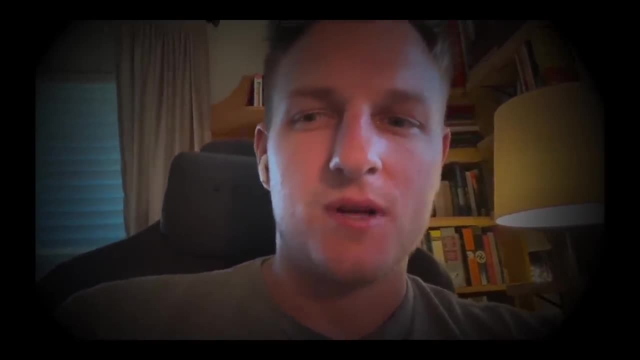 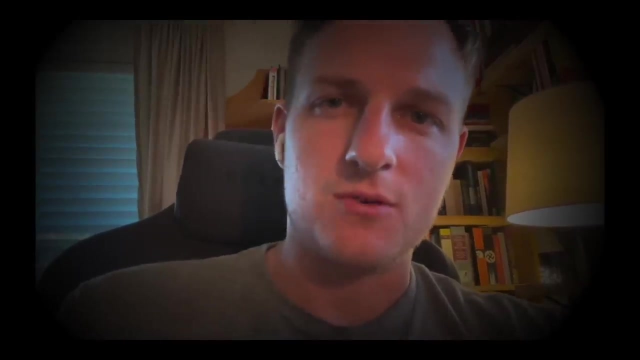 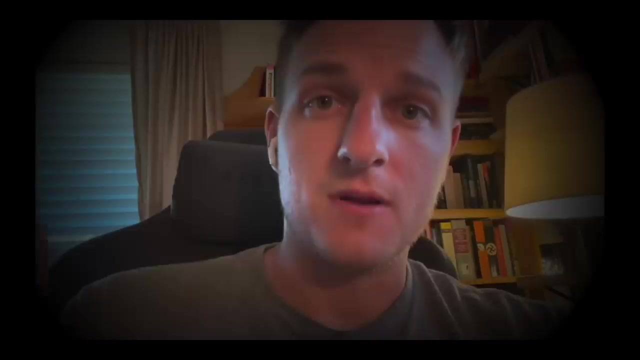 two, but the whole after the 1800s, the whole history of light is. you know, it's fascinating how, from Maxwell and his equations and Faraday's experiments before Maxwell and then her in his lab, confirming the existence of radio waves that Maxwell had predicted, and then 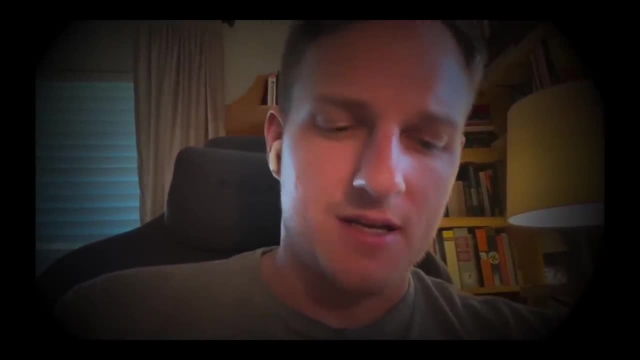 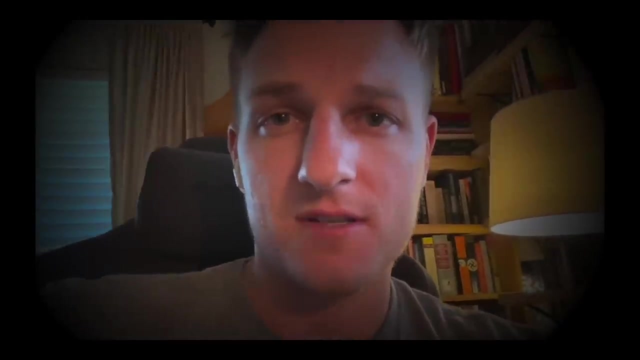 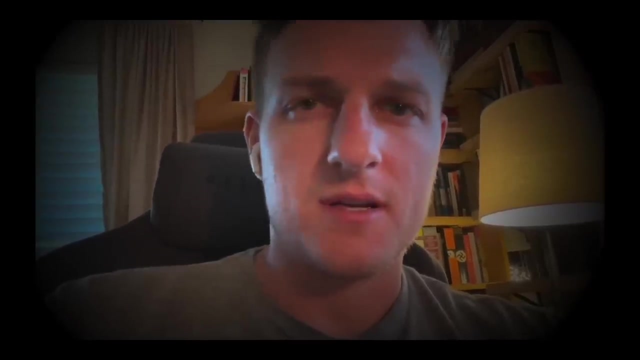 on up to 1900, when, you know, Planck had figured out that light had to have a quantum smallest amount of energy that it could exist within. that light could deliver, I guess the exchange between matter, particles, atoms. 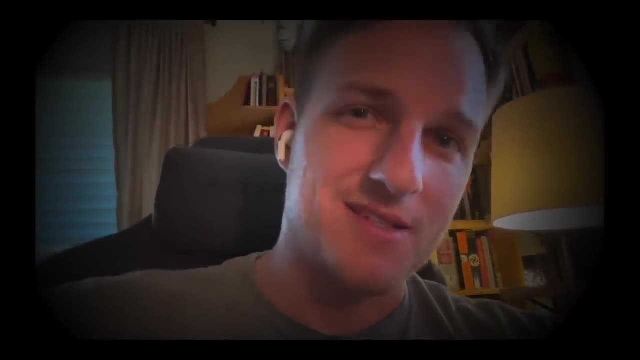 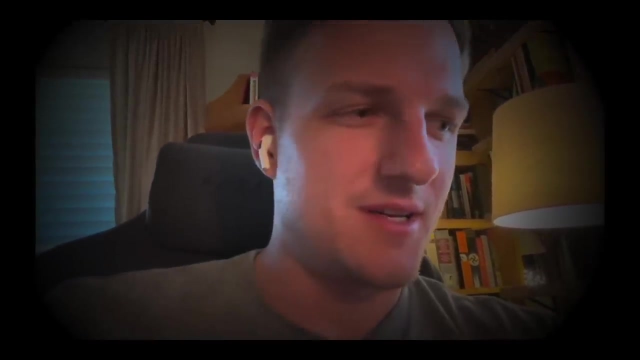 Anyways, that whole history is fascinating and I tried to do that. obviously, I don't retain much of it, so I probably didn't. that means I probably didn't do a very good job of well, not only learning it, but even what I wrote down wasn't enough, wasn't good. 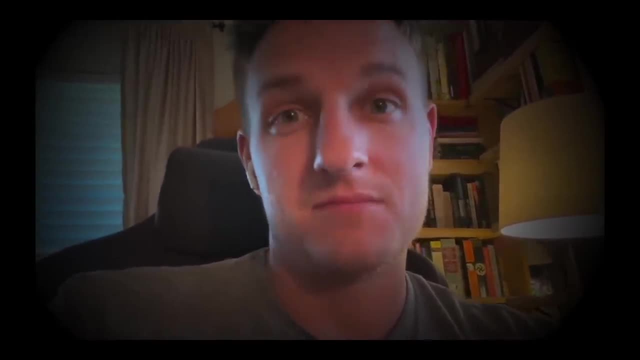 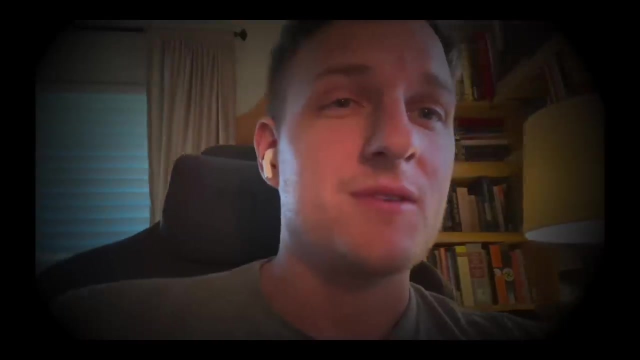 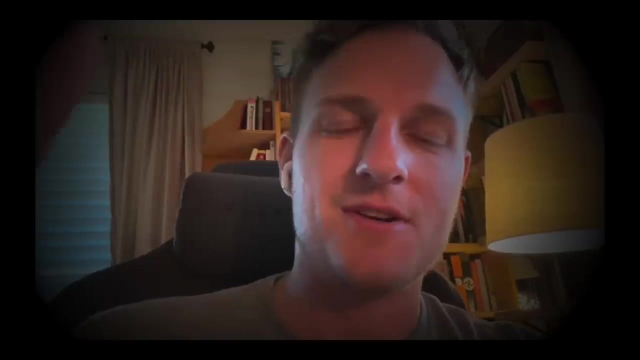 enough for me to really be able to explain it, obviously. so that's a whole other video. I'd like to do the whole history of light, but regardless, this is my really long way of trying to wrap this video up in editing here, realizing that it's a chunk of you. 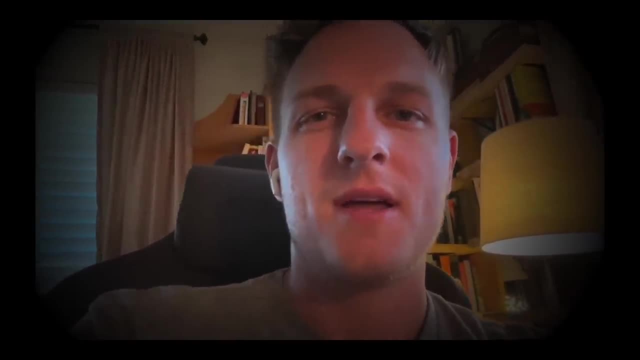 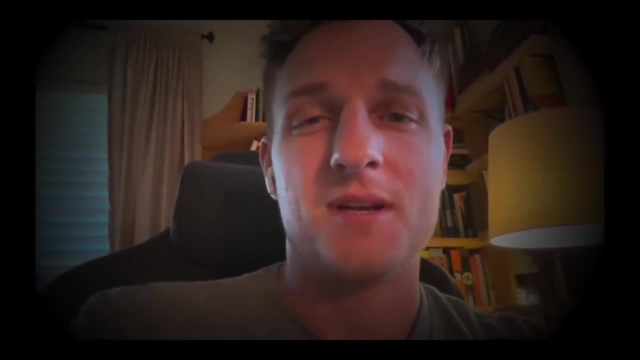 know existing material that I just didn't get to use for web, and so I wanted to say wrap it up by saying thanks for watching guys and for showing yet again so much gratitude for all of you who do watch, who show love in the comments, support the channel. 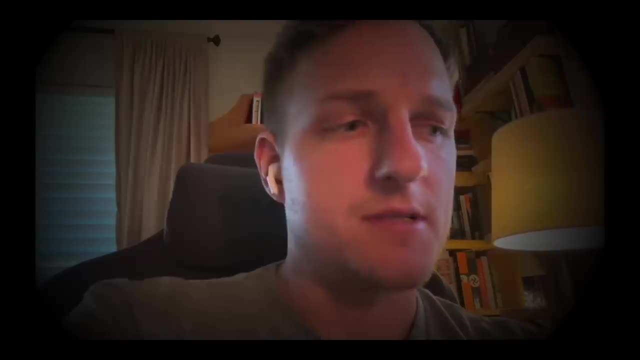 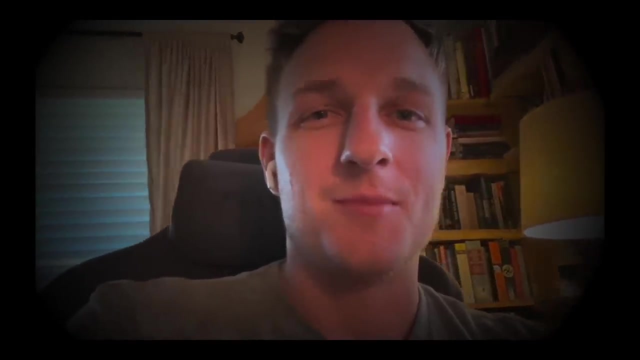 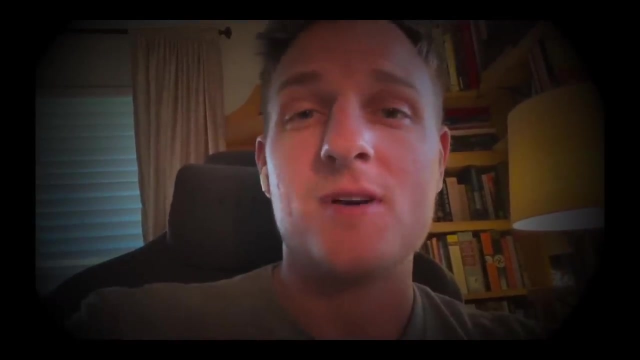 financially through all the avenues. You guys, it really means a lot. and thanks for the well wishes on baby number two. we got coming probably tomorrow as of the time I'm recording this video, so by the time you guys see it, it should probably be here. we don't know whether it's a boy or a girl. 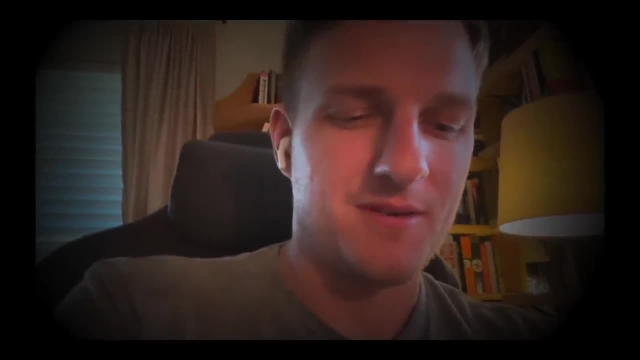 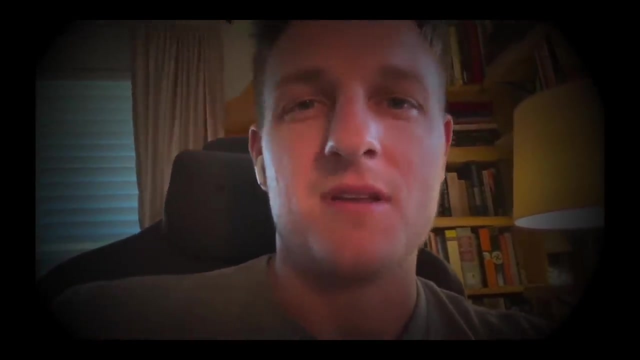 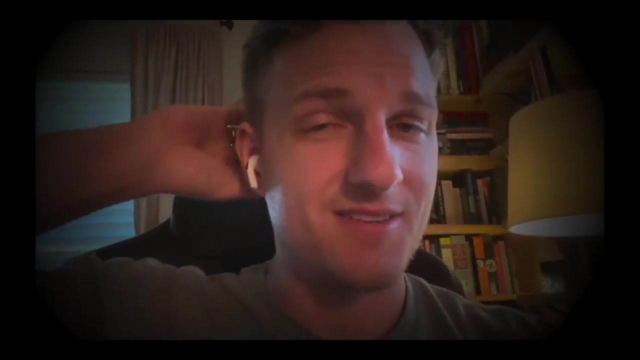 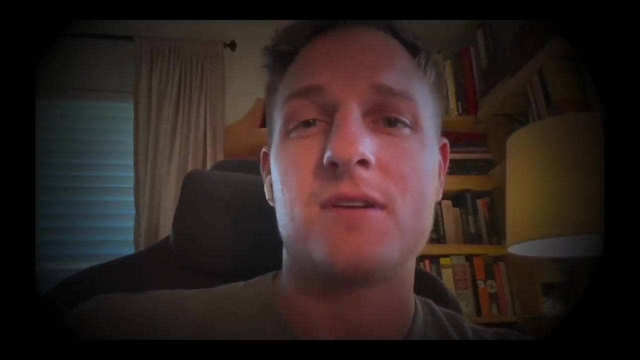 at this moment, but we're very happy and, yeah, this is a really fun topic and obviously learning more and more about it as I make these videos, and that's part of the reason why it's so much fun and meaningful for me to do this, and meaningful that you guys enjoy. 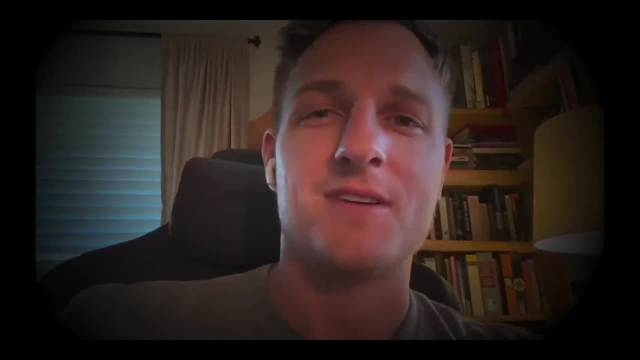 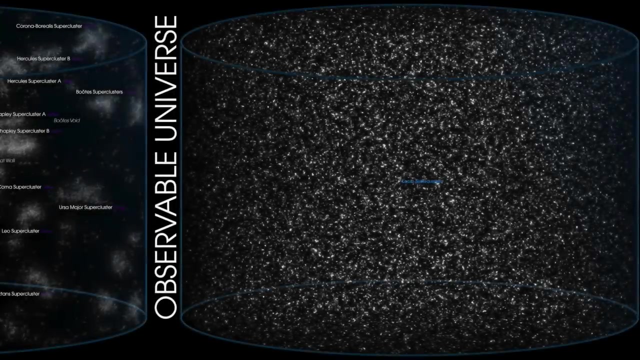 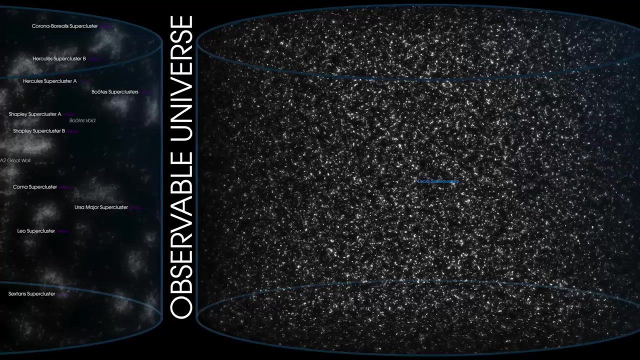 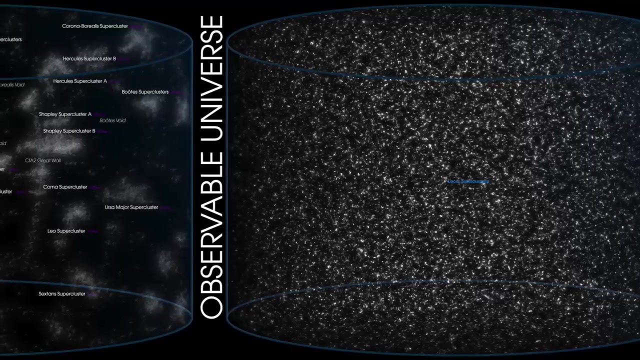 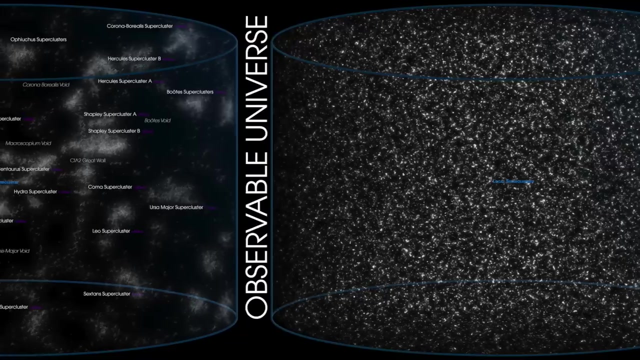 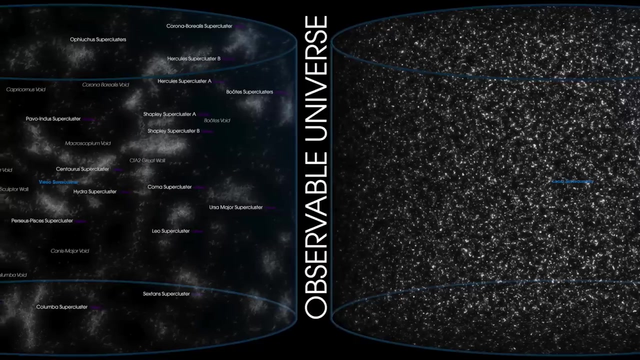 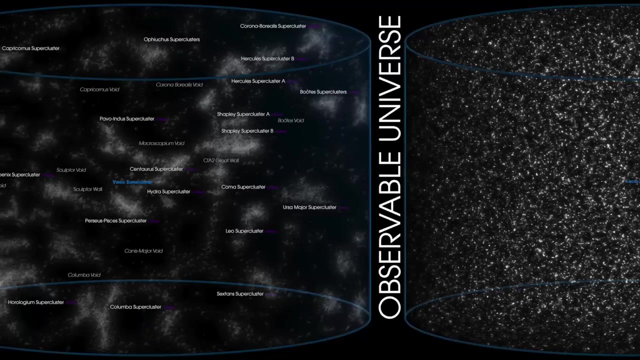 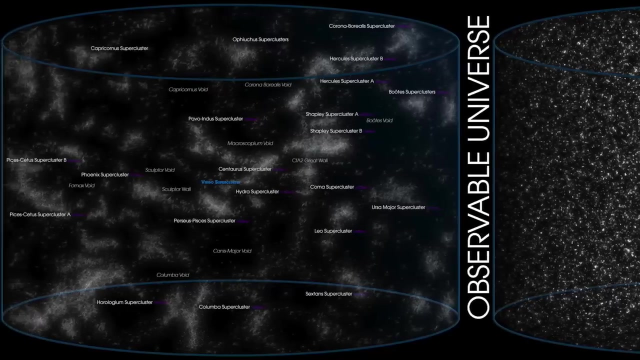 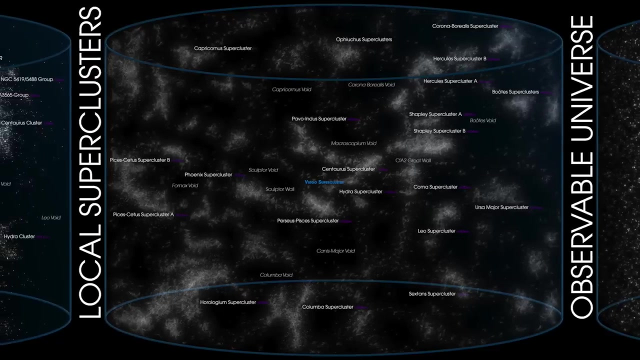 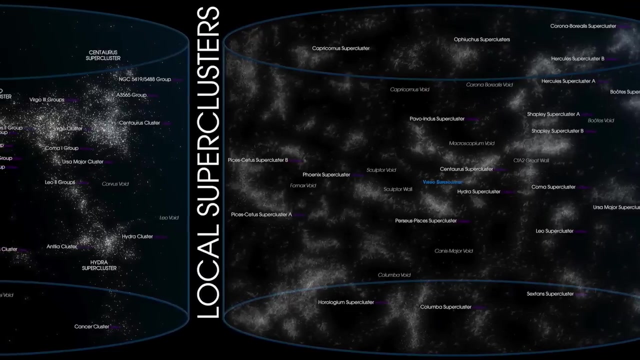 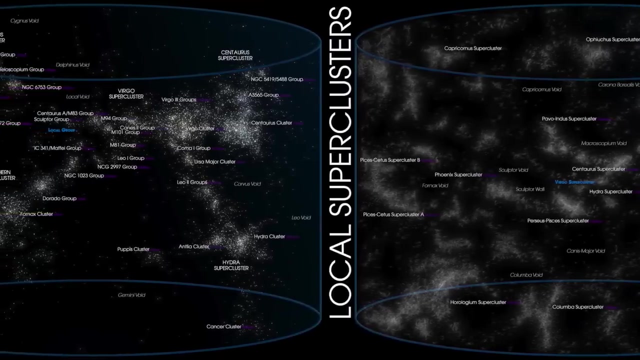 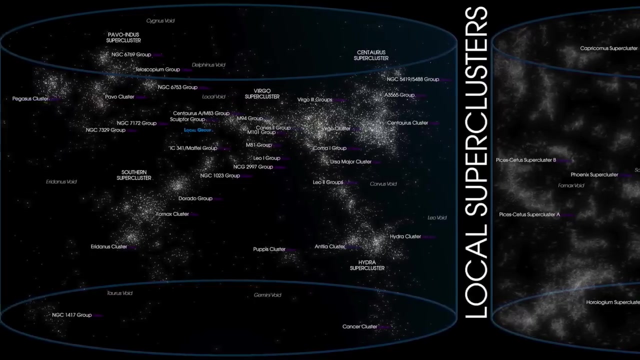 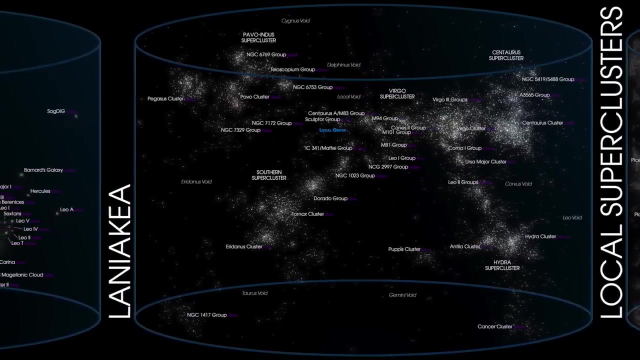 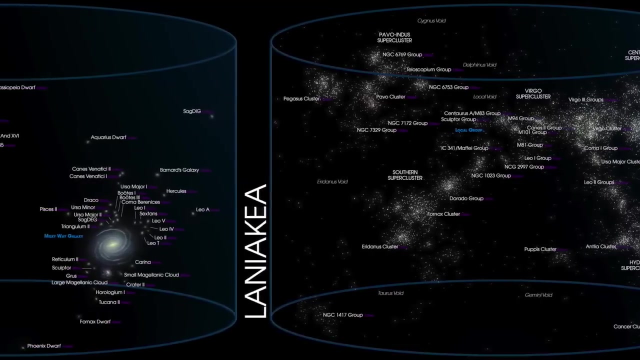 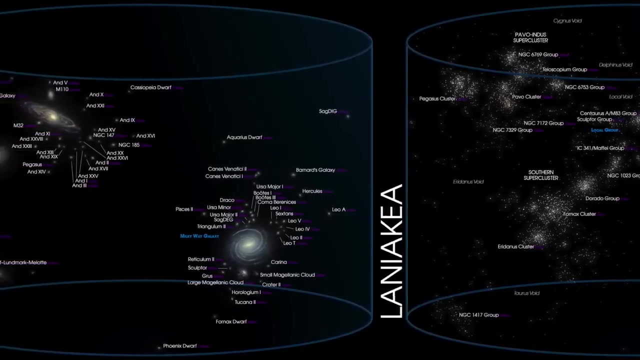 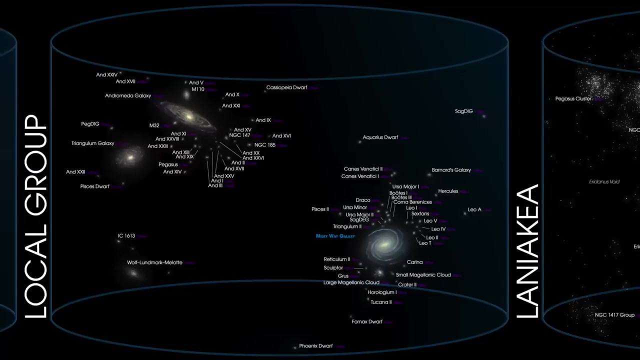 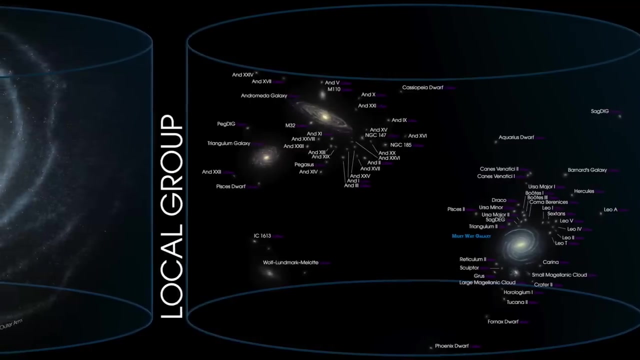 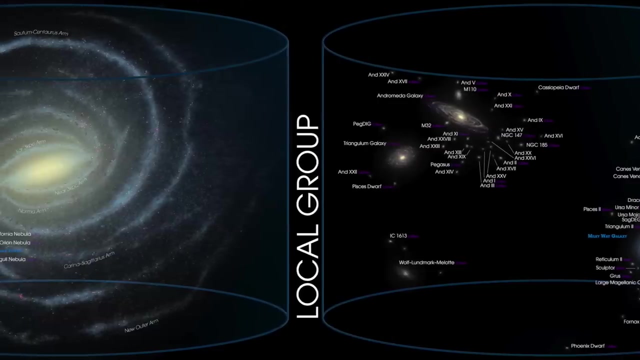 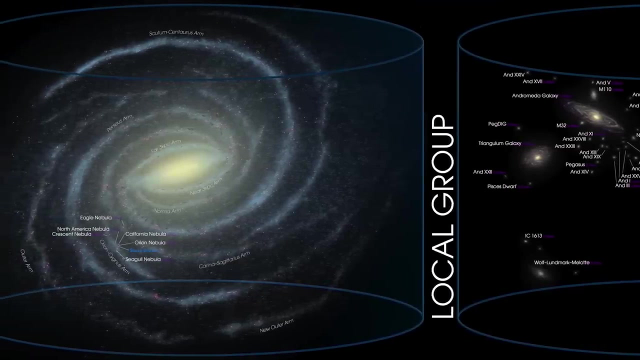 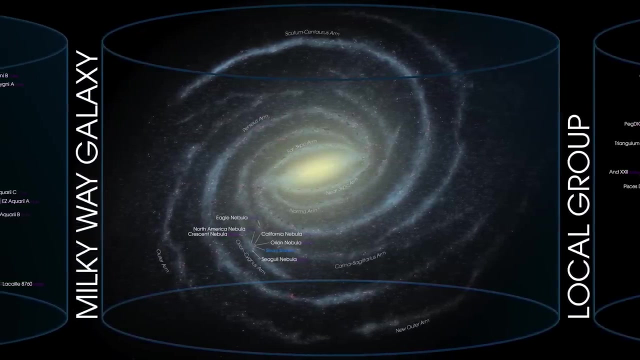 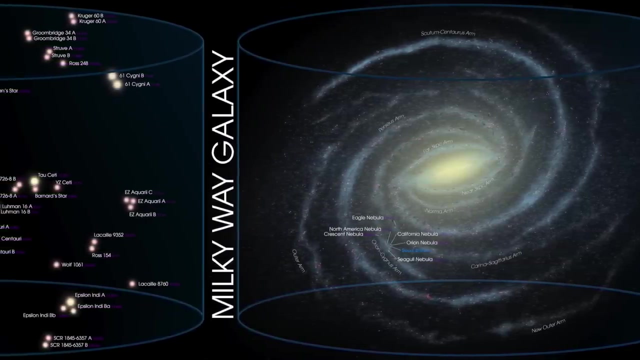 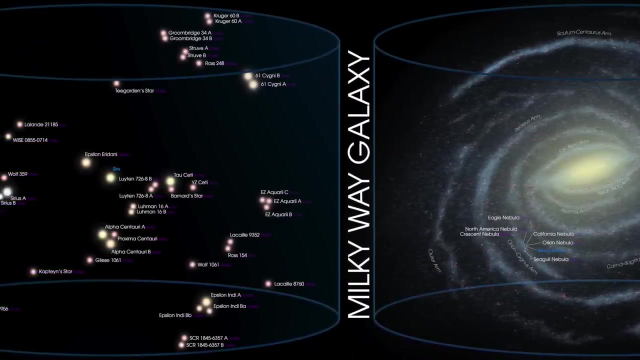 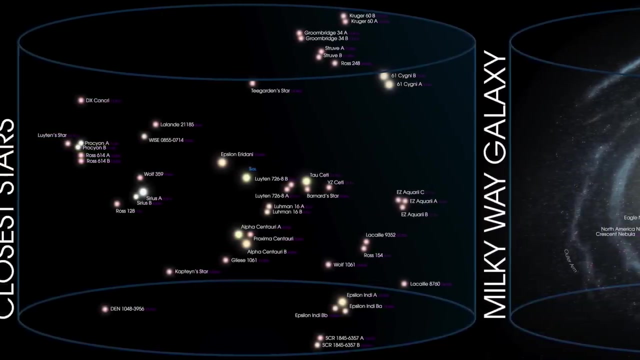 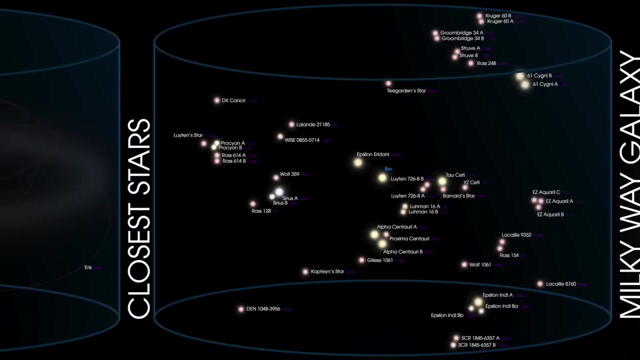 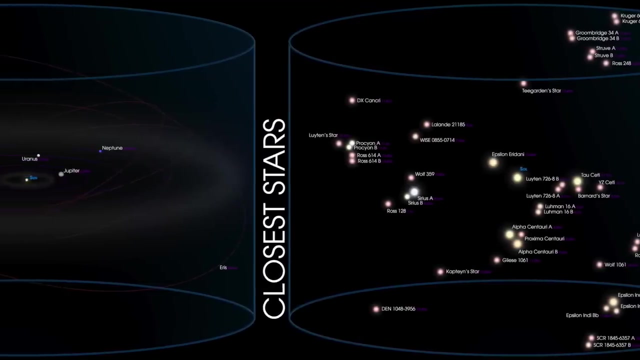 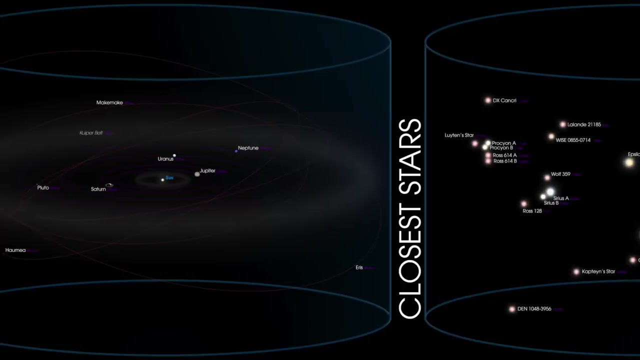 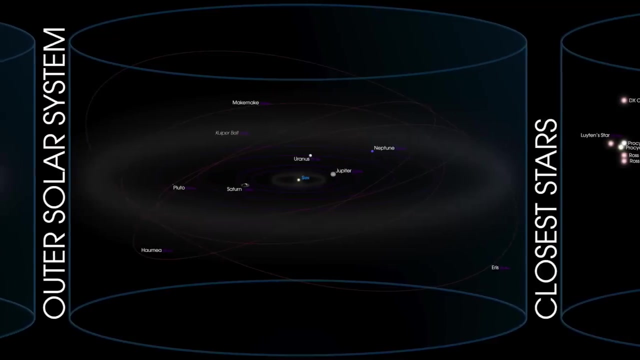 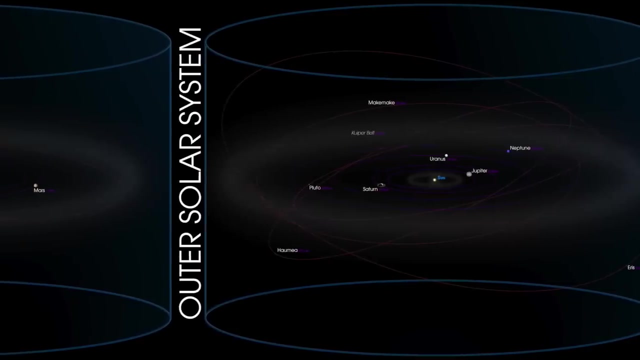 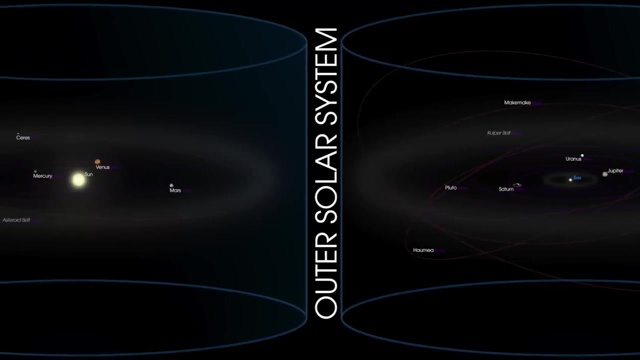 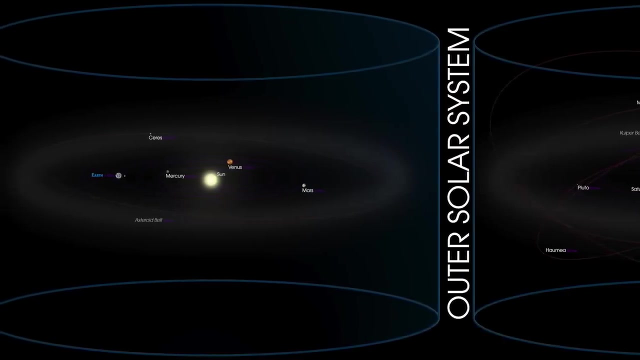 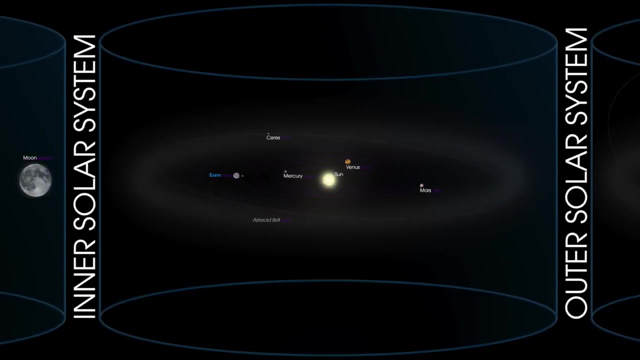 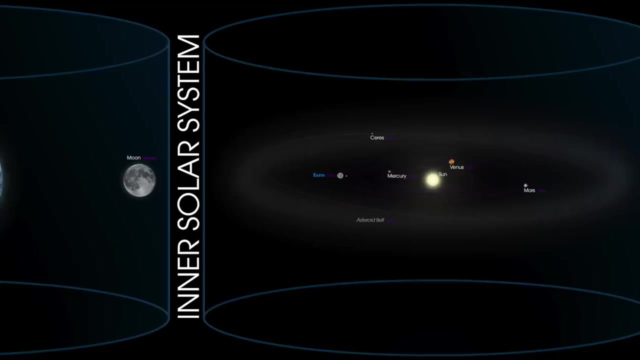 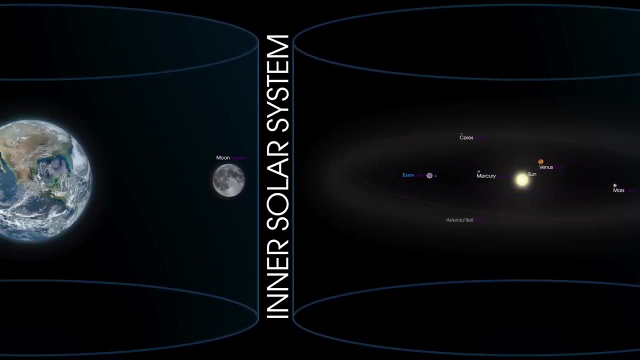 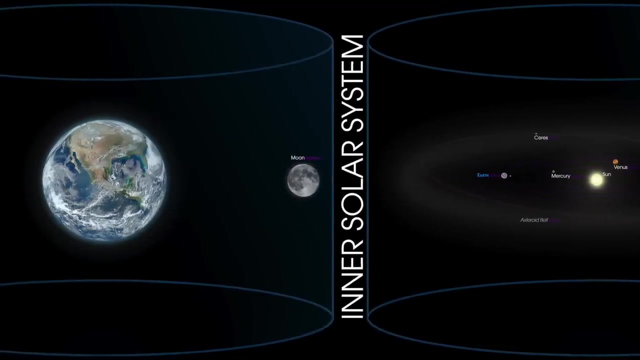 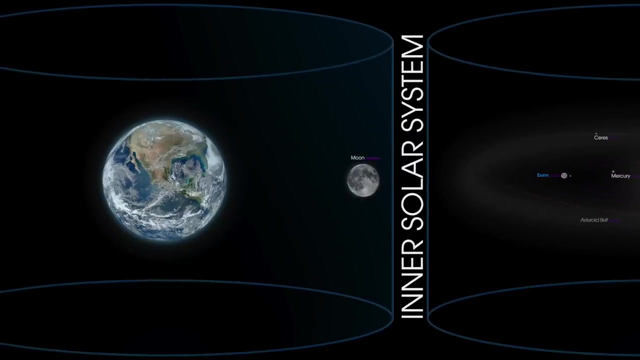 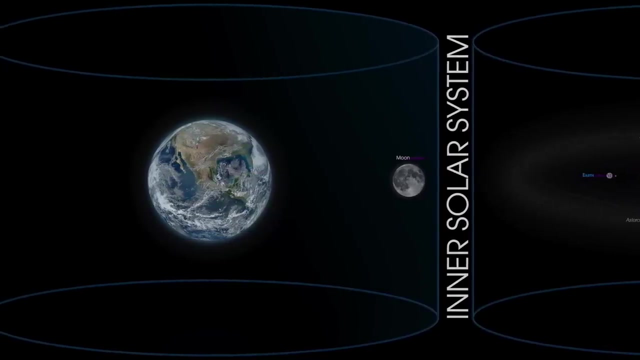 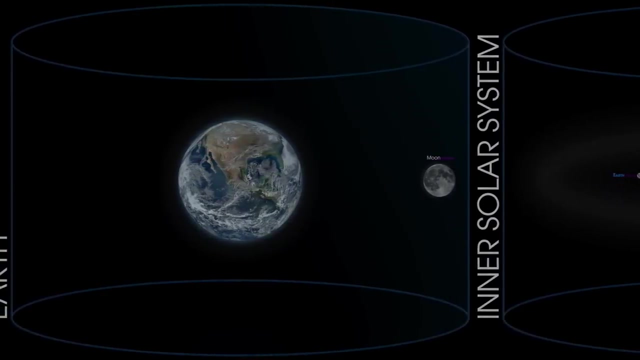 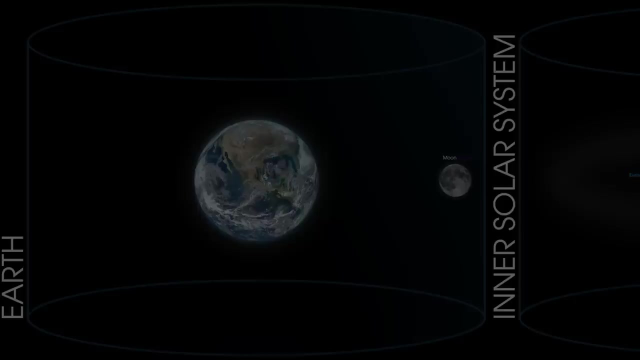